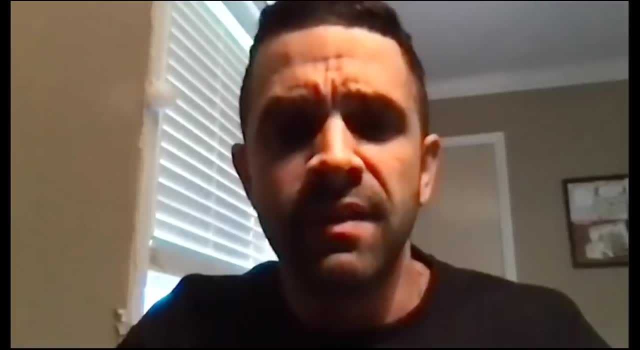 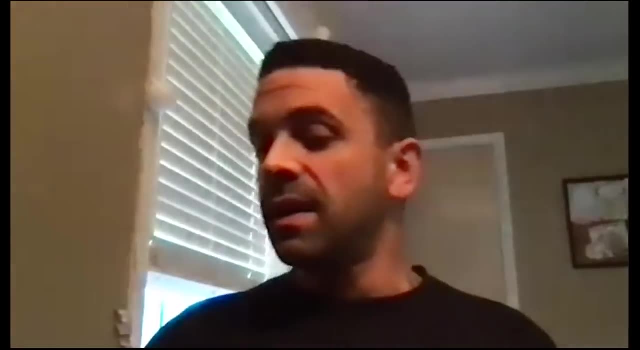 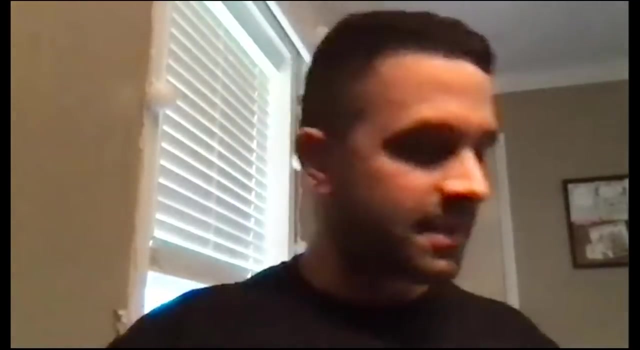 accidentally kicked the plug that holds the fucking modem in. I was just testing you, All right. So what the fuck is this? All right? so, as I was saying, I'm going to need a couple pee breaks and drink too much coffee, you know. 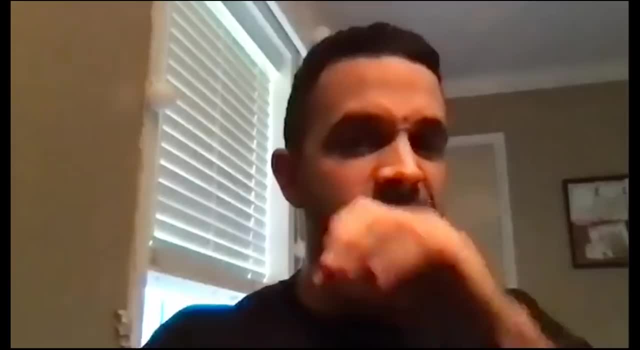 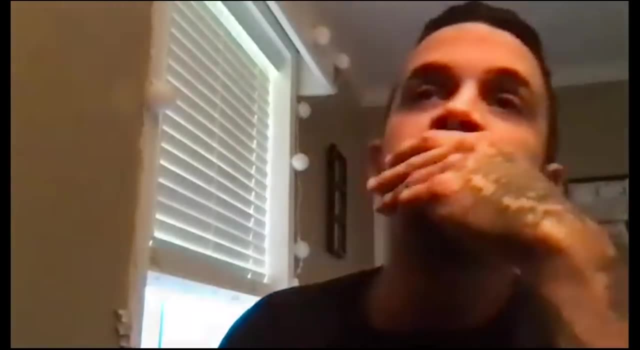 So what we're going to start? I got a little slide presentation prepared. We'll start, hit record. Okay, it's recording already, So we'll fucking. we'll start off with a just general plant ID And then towards the end, for anyone who's struggling, I mean I talked for a while, So 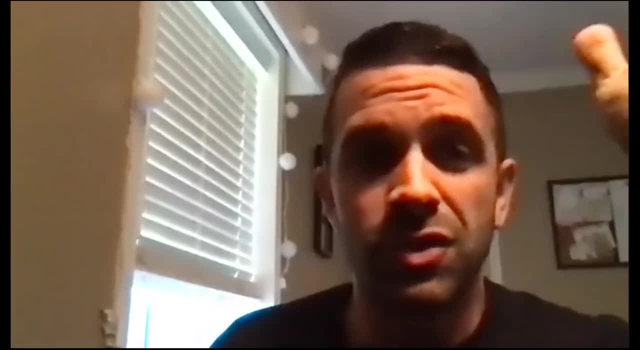 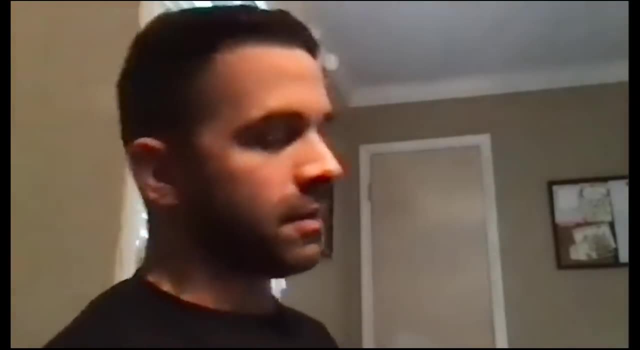 this will go longer than an hour. If you need to dip out, of course, just fucking do it. You can watch the recording later, Just hit me up for it. We'll talk about all the technical stuff And then we'll get into. I'll show a bunch of plant porn, just different photos of. I got a 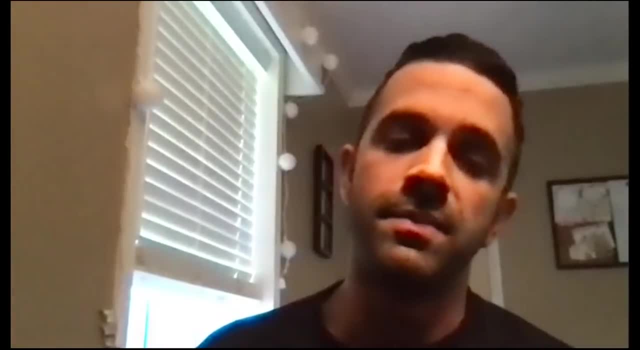 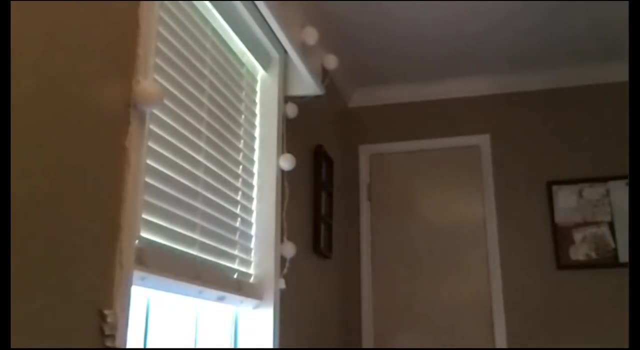 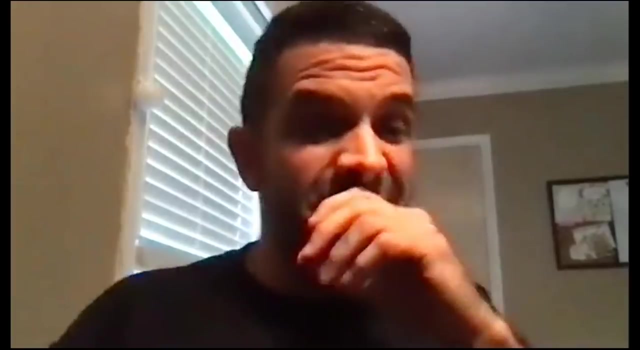 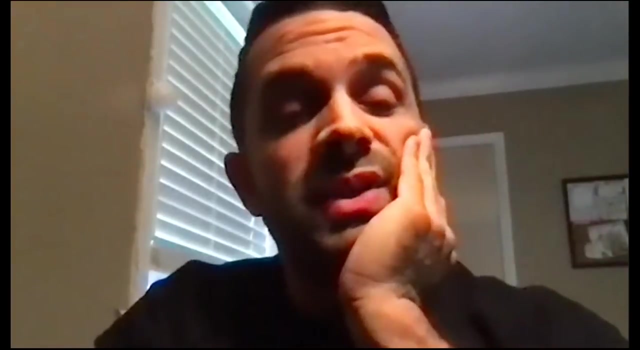 New Caledonia presentation. I got a bunch of shit from the Southwest And let me get this. I got a list of books too, So hopefully everybody downloaded iNat, because that's going to be. that's going to be. your most useful tool is looking at iNaturalist, because you can use. 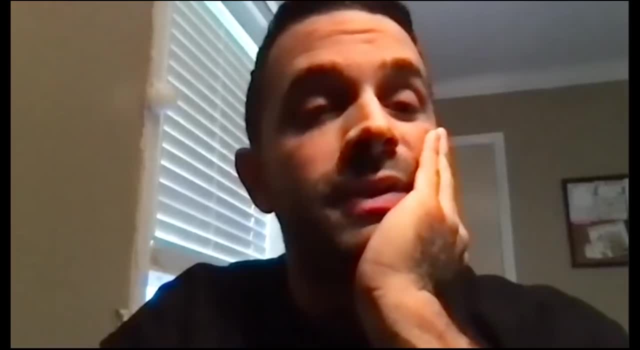 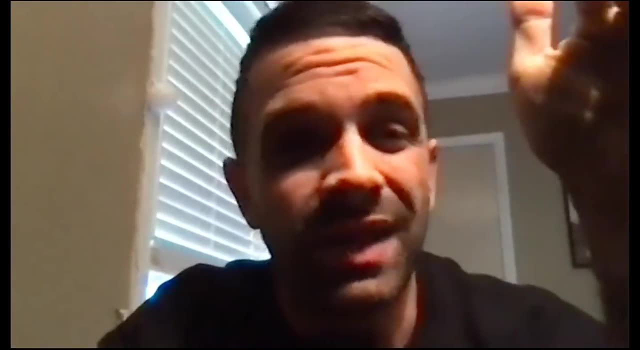 that explore feature. You don't even need to upload shit, You could just use that explore feature and you know all the taxonomies there, et cetera. So I mean, it's really you know, especially if you're stuck in like a Northern latitude where it's fucking, you know, winter. 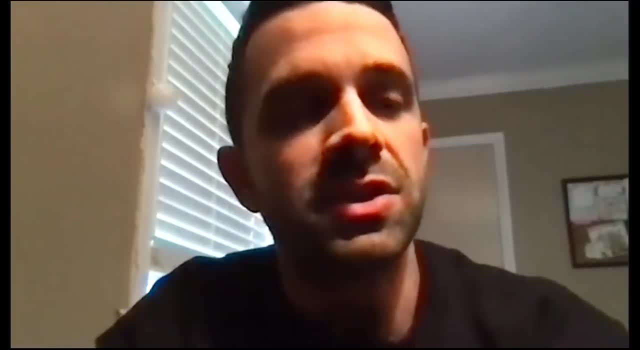 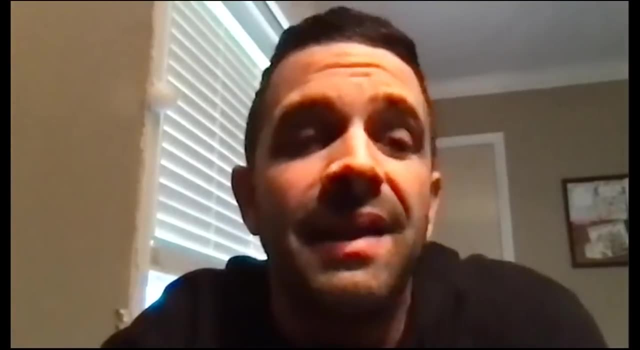 you can't go outside, you could still explore it. So I mean, it's really you know, especially if you're in places like you know- West Australia, where it's summer right now, you know, or Chile, or whatever. see what people are logging. A lot of a lot of photos are shit on iNaturalist. 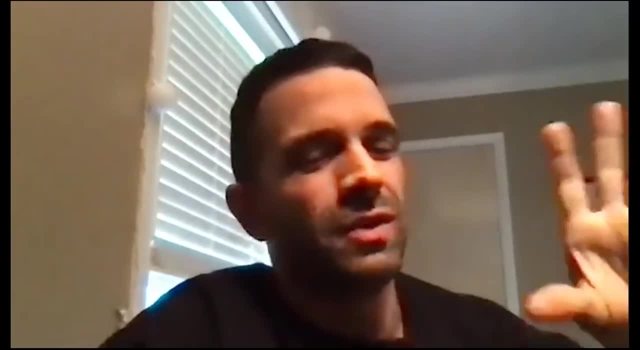 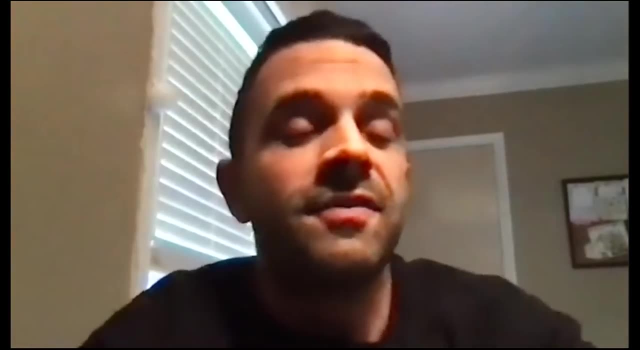 but at least you know cause people will take like blurry cell phone photos, and only one, And some guy just discovered like a new species or species of rock daisy that hadn't been seen in like 50 years, And the photos he took were like blurry and fucking, you know, three feet back. 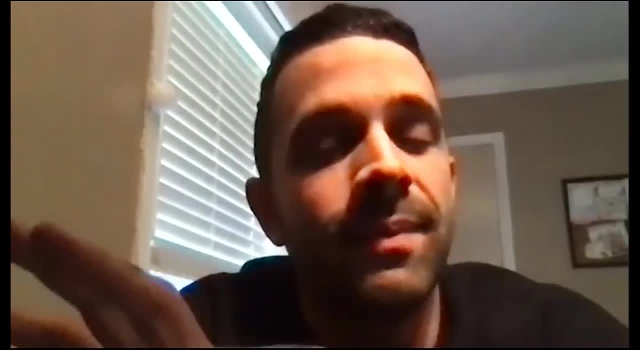 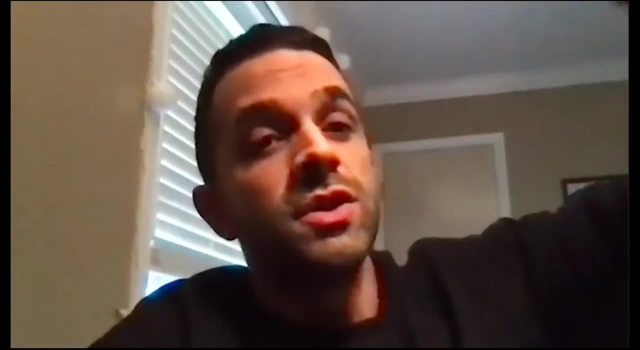 It was like really, But you know, you still get the name of the plant. and then there's a way to you know, hit the view children button. Children is just, you know, the the word they use for all the lower taxa of. you know, like a genus, If you're. 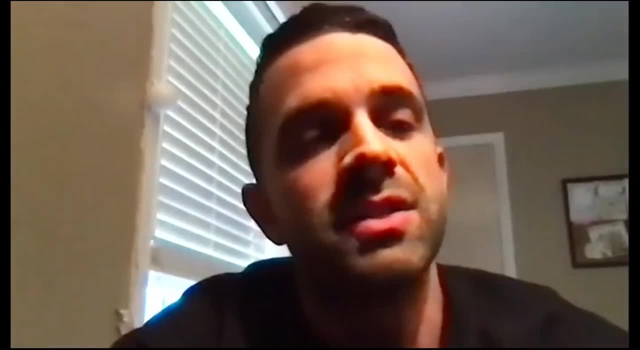 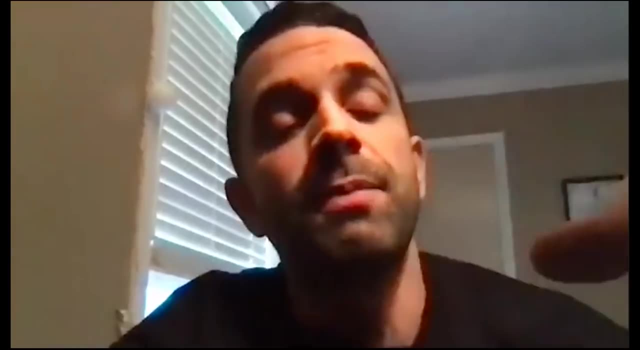 looking at a genus. it'll say: view children. You hit, view children. you could see all the species in that genus. but we'll get to all that. If you don't understand what the fuck I'm talking about, that's fine. I'll uh. every couple of slides, I'll stop and you can ask questions. Uh, please. 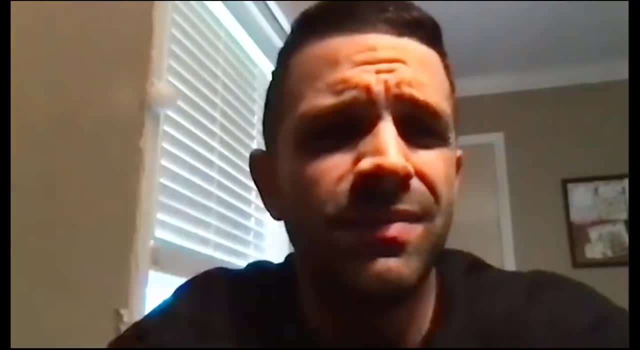 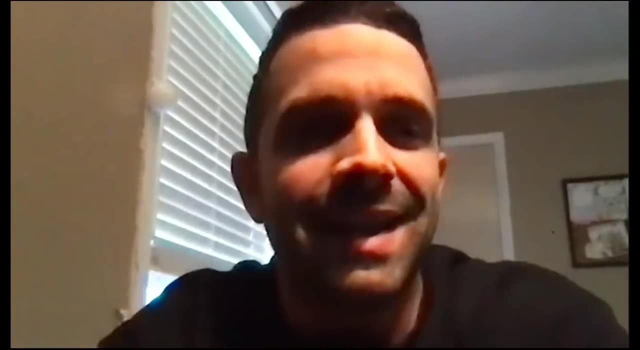 everybody. mute your, your camera too, if you can cause. it's fucking. you know someone's puking in the background or someone farts or something. you know someone's dog's barking or some shit It's. it's very distracting And I got- I got- bad ADD already, So, uh, mute. 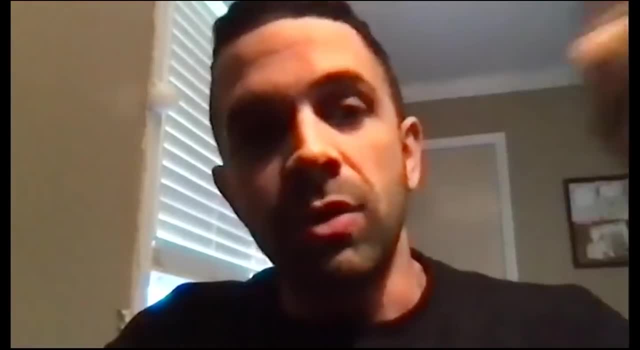 your, mute your mics, And then if you want to talk, you know, just unmute them and ask a question, whatever. So, um, but like I was saying, if you don't understand any of these terms, don't trip. 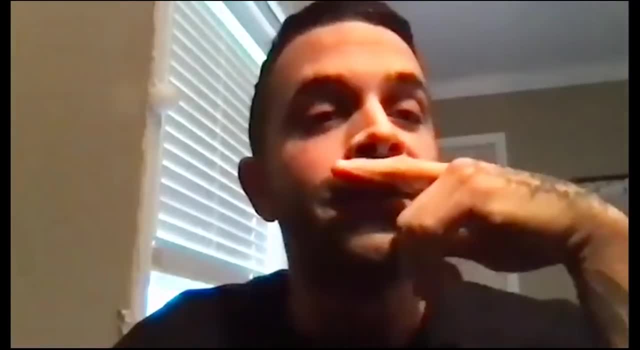 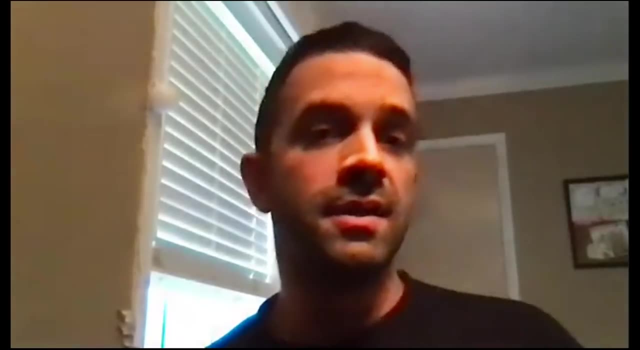 you just, you know, take notes, write them down. You can watch the video later. Uh, the key, the thing I want to do is just put these words out there and throw them at you So you can look them up later, So you don't need to memorize everything now. I don't feel you know all the 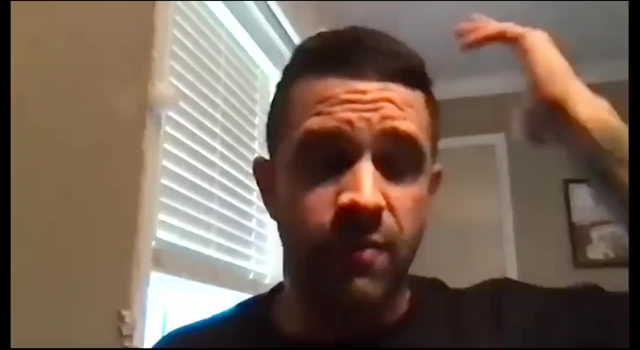 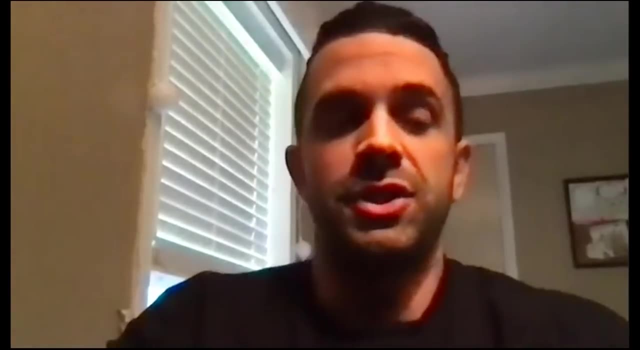 pressure I got to get this all down. What the fuck is he talking about? I don't understand. It's way over my head. You get the ideas, you get the keywords, and then you could just look them up later, And I mean that's how I taught myself all this shit, You know? I mean just 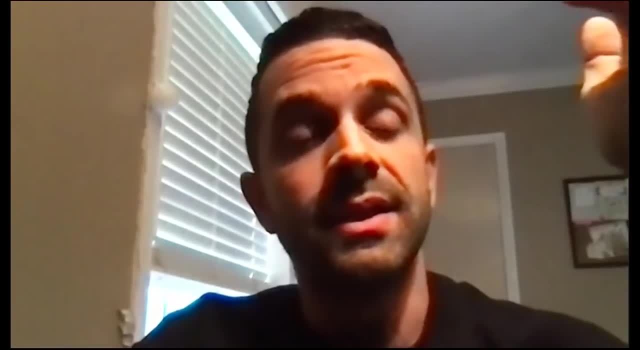 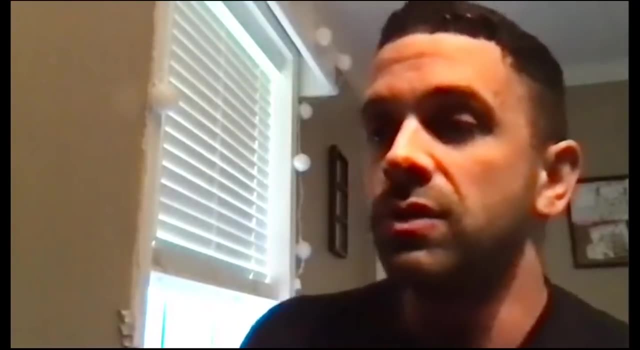 anytime you encounter something, you don't know what the fuck it means. You just look it up. I mean, it's just, that's mental exercise, trying to understand new concepts, new ideas. the same way, you know, you got to do physical exercise to keep your your ass in shape. 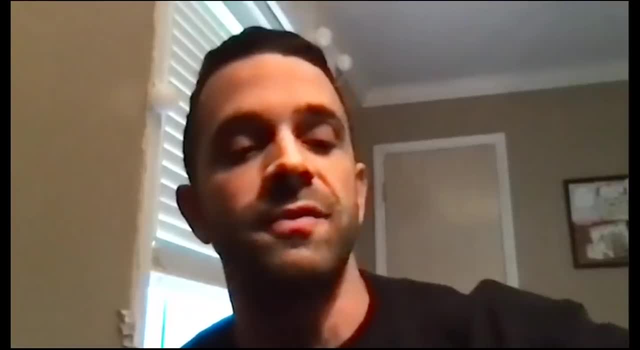 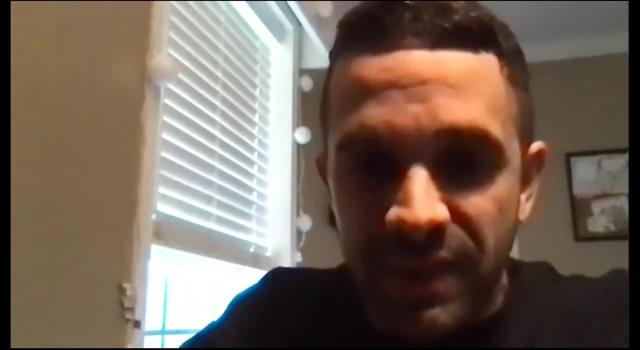 heart up. Uh, you got to do mental exercise too, So you don't atrophy, So your mind doesn't atrophy, you know? Um, so anyway, with that we'll get started. uh, pardon, grandpa, while he. 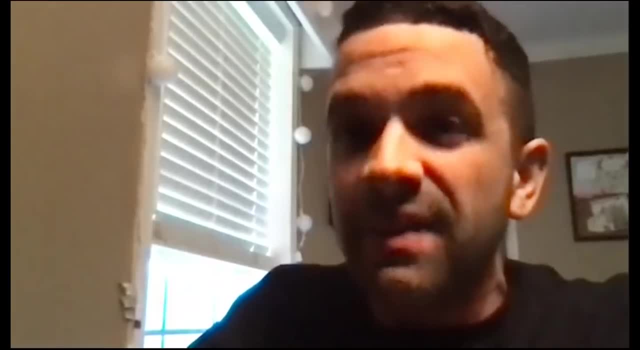 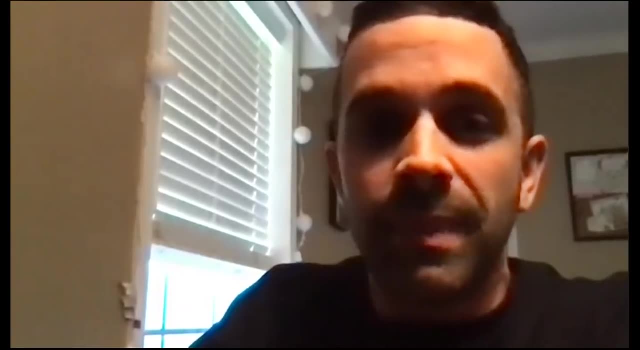 figures out how the fuck did see share screen. Let me put this presentation up. Oh, it's a fuck. I'm using a Mac. This is my computer too. I'm using a Mac. I can't. uh. Oh God, There we go. 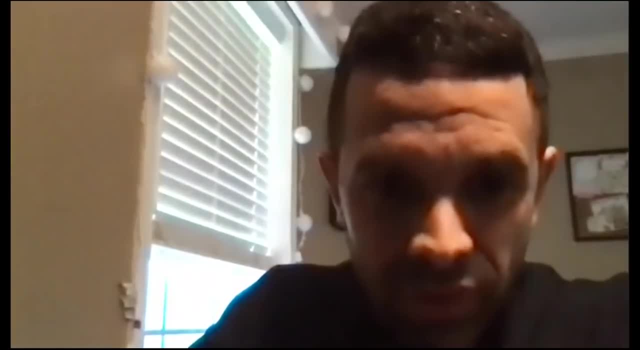 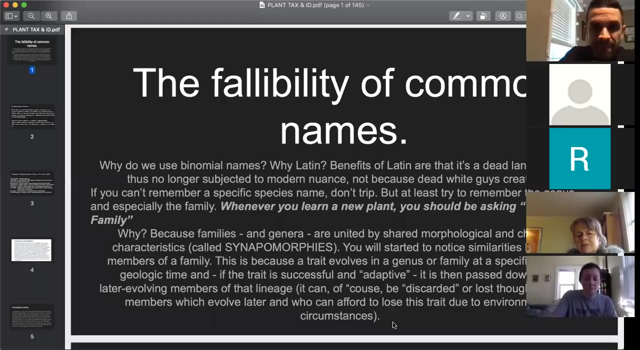 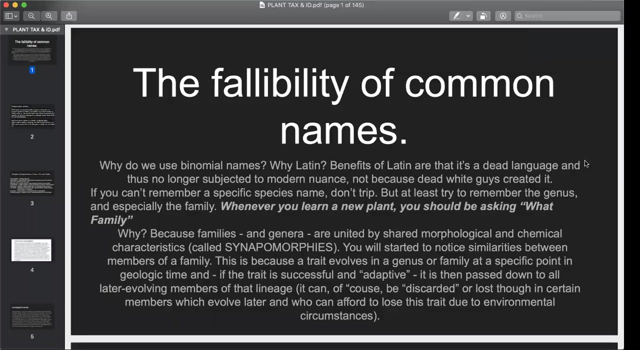 Plant tax and ID And we'll do share screen. What, Oh, just this. Okay, How do I do minimize this? And then, how the fuck? you paid zoom money just to watch some guys scream in a computer? How, uh, how do I full screen this? Jesus Christ? 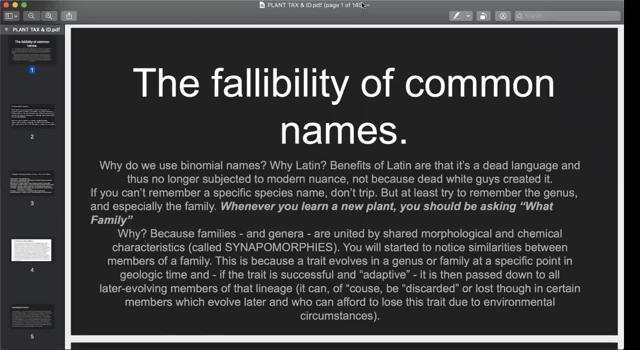 Oh, hold on, Hold on, Hold on, Here we go. Just got to hit the full screen button. Oh yeah, So this is there. They're seeing everything that's in the green. So for them, how do I? there's no way to- you want to? Oh, okay, They're seeing everything, Yeah. 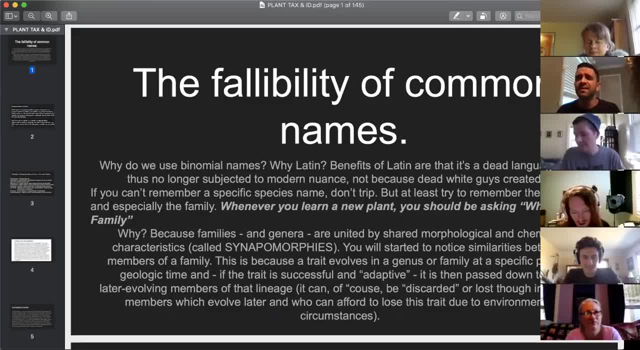 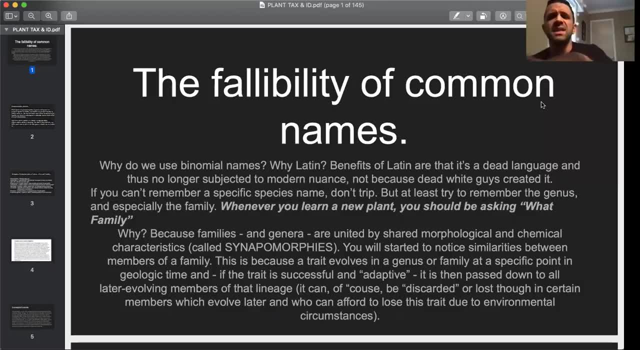 So you can do this. Okay, So they're not seeing. you guys aren't seeing anything but this slide. I got up right. Could someone on mute and just give me a heads up? Yeah, Just you in the slide. Okay, All right. Cool, And if we get a shit poster or a troll, then we'll have some fun. 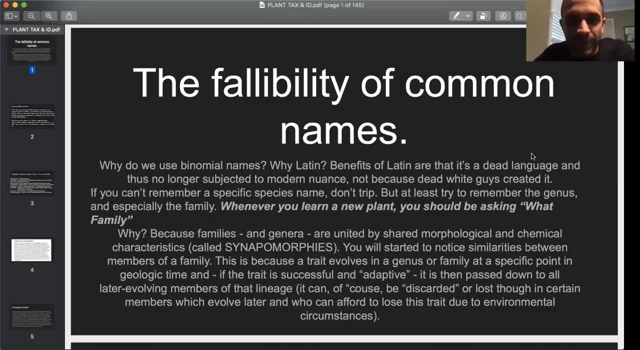 with them and throw them out. If I can, you know, get the adult back in the room to show me how to do it. Okay, So this the thing I want to teach you. all this. it's not just so you can impress your. 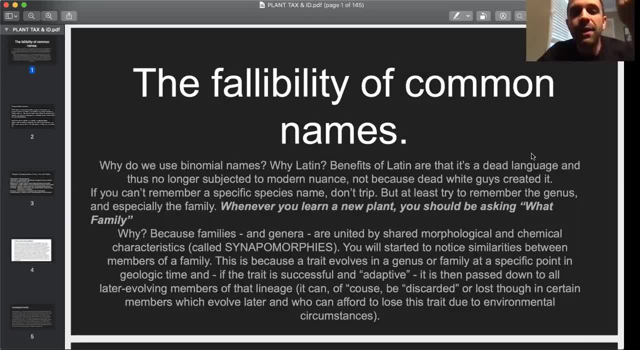 friends and know all the fucking Latin names and everything, And so you can get a better understanding of, uh, of life on earth. Cause this stuff, the principles I'm going to try to show you, don't just apply to plants, They apply to everything, They apply to you, They apply to 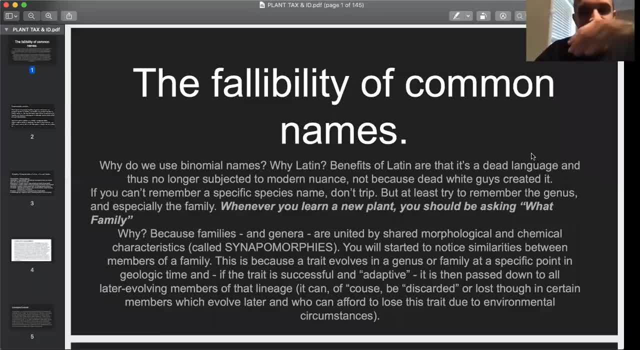 your Simeon relatives, you know, chimps, chimps and bonobos, Uh, they apply to, uh, to bacteria, viruses, everything. So it's, it's just the you know, it's, it's evolution, It's this, uh, still relatively new concept, only 150 years. 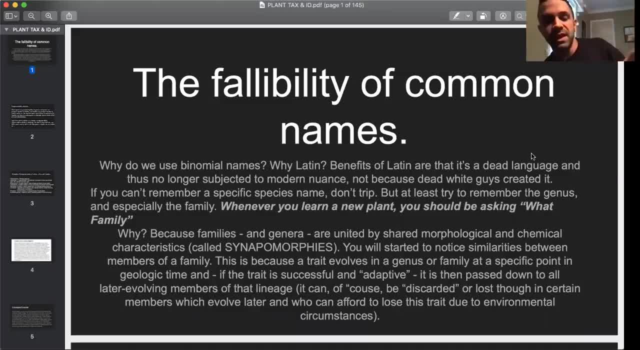 old, Uh, and it's. it's amazing. I mean, when you learn this, it makes you know whatever droll fucking world you're, you're you're living in, you're immersed in, you know whether it's. 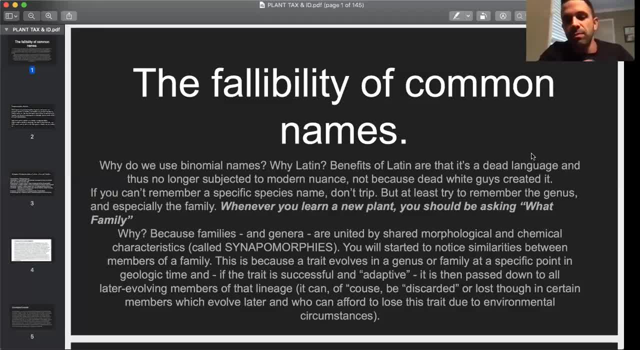 cul-de-sacs and strip malls or you know something, even more bleak. it makes it, you know, it gives you kind of a a a perspective on everything else around you. You know everything else that's been here for the past 4.6 billion years of of uh, of earth history. 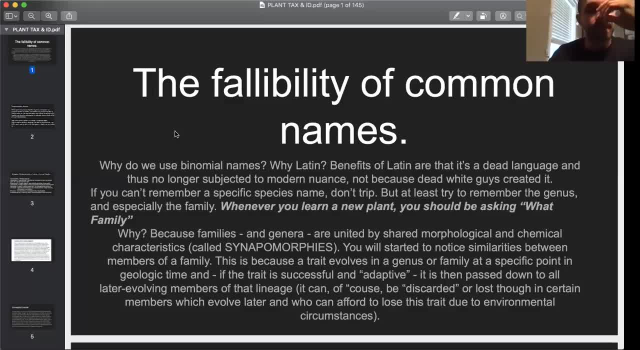 so, um, anyway, we'll start off with the fallibility of common names. You know the reason I don't like to use common names. this is probably elementary for some of you, but it's because you know a word like cedar can refer to refer to six different uh, unrelated. 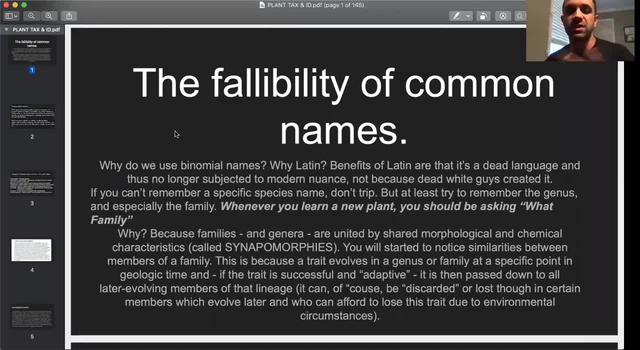 plants, You know. it can refer to Thuja, the Arborvitaes. it can refute a salt, refer to salt cedar. Tamaris can refer to uh, juniper, And then you have the true cedars, none of which are native. 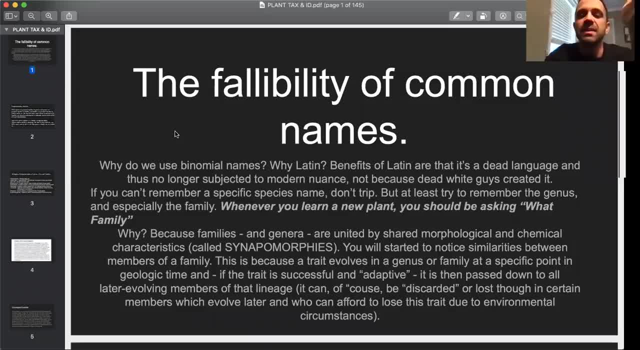 to North America in the genus Cedrus. So common names can be confusing, like a plant like Turk's cap, for instance, can refer to six different plants too. They don't tell you anything. The point of using taxonomy and Latin names is that a species is connected to a genus. 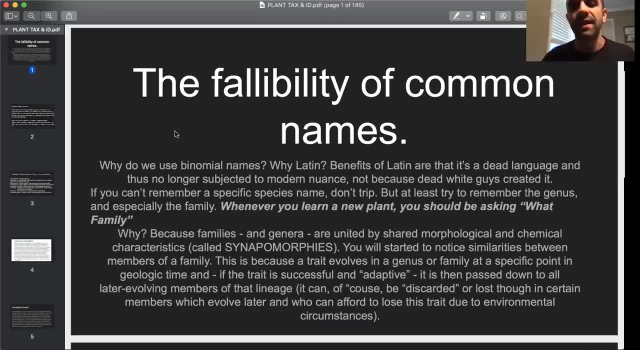 And then that genus is united- And we'll get into this again- by shared traits, both molecular in terms of DNA, but, more importantly, things you can directly observe, like flower morphology. So I can be in a new place I've never been before and see a plant I've never seen before and know. 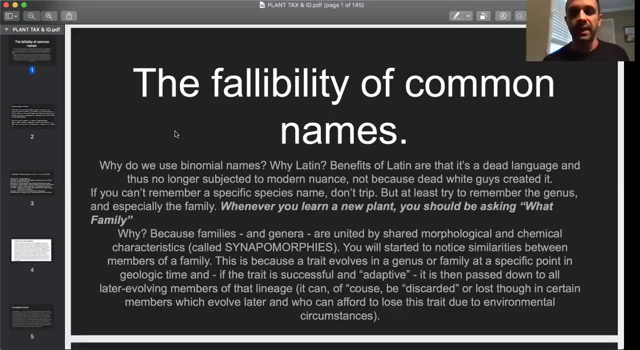 Oh, that's in the verbenaceae, That's in the verbena Family, in the order Lameales, And so there's these shared traits, uh, you know. so I'll know that it's probably got opposite leaves, It's probably got a, uh, probably a pleasant stench. 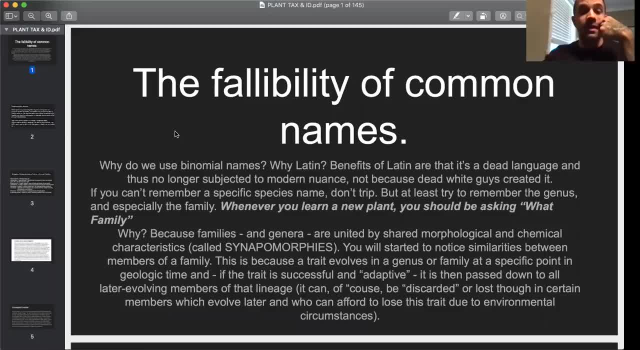 to it. you know, cause that's the Lameales, is the order of mints, et cetera. So there's a lot you know once you know what are the traits that unite a genus or a family or an order. 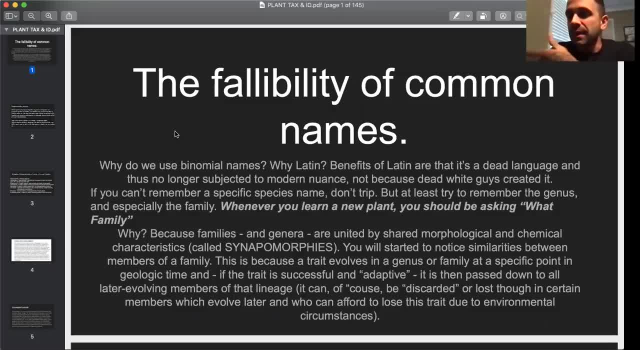 you already know more about the plant you're looking at Once you can place it by looking at its flowers, you know. you can say: Oh well, it's got so many stamens and the flowers, you can fold them, uh, longitudinally, but not not horizontally. 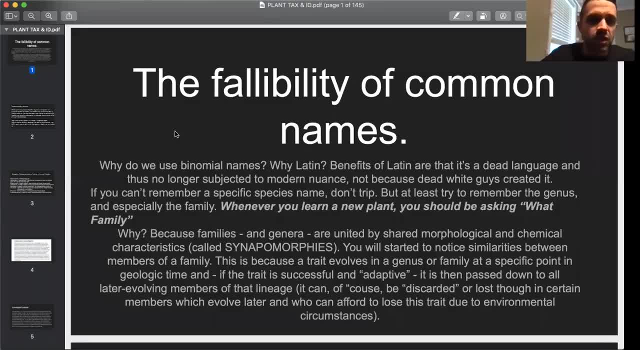 you know, so it's bilaterally symmetrical. It's a good chances related to this, you know. and then, uh, you know, once you get uh, familiar enough with it, you get really good at it. You can, you can just automatically start. 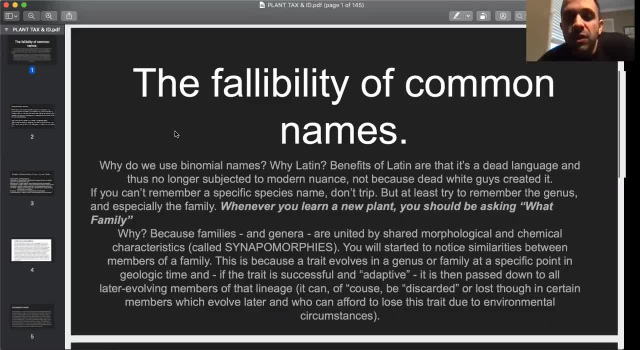 IDing stuff. You may not know what species it in, but it's in, but you'll know what genus, uh, and what family and order, et cetera. So there's a story there And that's the thing I. 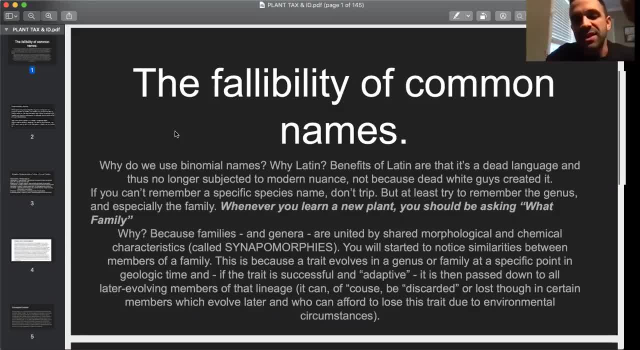 want to, I want to get across is we use taxonomy because there's a story with every genus, with every family, et cetera. There's, there's a bunch of traits that you know, little footnotes in that, in that, uh, that name, So uh, anyway, these shared traits are called synapomorphies, All. 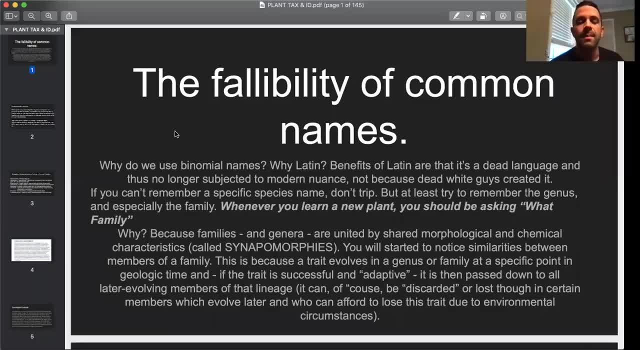 right, And that should be the first word. write it down, remember it, memorize it. I mean, these are the shared traits that, uh, that that unite things under, uh, under a taxon level, Like a genus or family, whatever. So, um, let's move on. You could read that that this is: 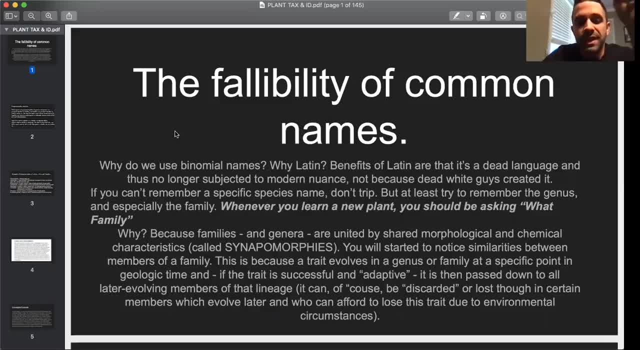 because a trait evolves in a genus or family at a specific point in geologic, geologic time, And if the trait is successful and adaptive, uh, that trait is then passed down to all later evolving members of that lineage. Now, of course, these traits can be lost later, Like if it proves 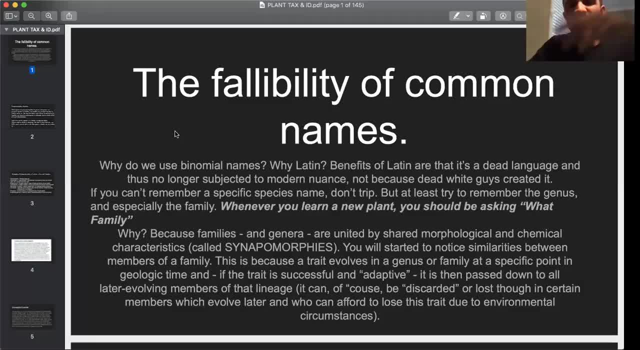 you know you'll get like, uh, caryophyllales, for instance, the order of cactus beets, spinach, ice plant, uh the four o'clock family, they're all in the order of caryophyllales, A lot of. 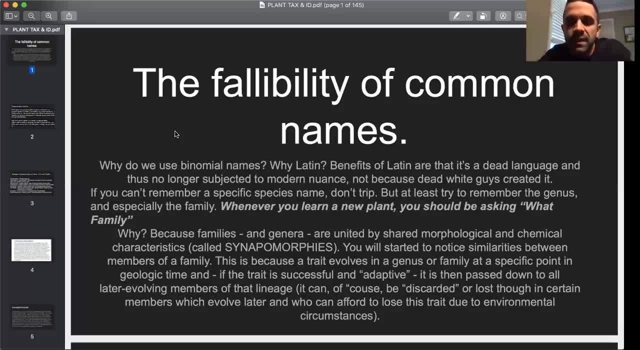 members of caryophyllales. like 95% of them, uh produce beta lane pigments, which is a type of pigment. Once you learn what it is, you'll oftentimes be able to just tell if it's a beta lane pigment by looking at it. that you know when you take a shit after you ate some. 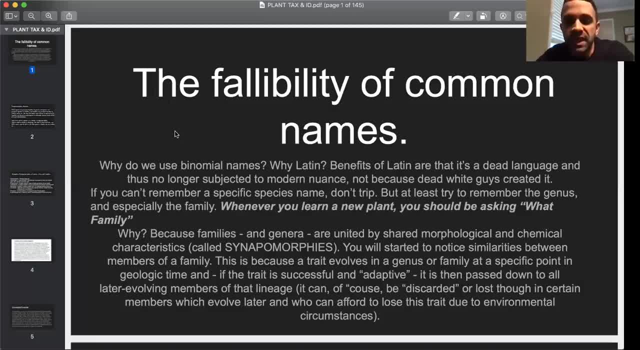 beets, those red pigments, uh, that you see, that make you think you got colon cancer and you're dying. those are beta lane pigments. Okay, They're the same uh, red, You see, in cactus or an ice plant or in bitter root. they're beta lane pigments, Beta lane. 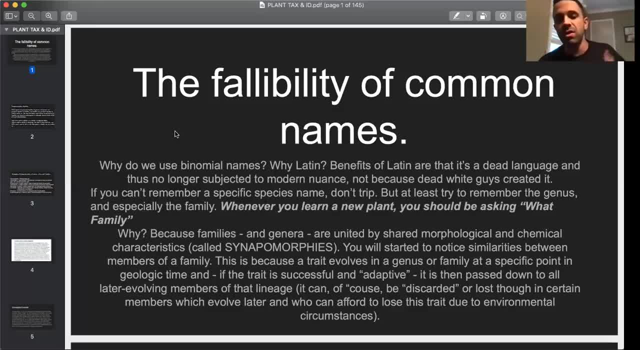 pigments are a synapomorphy of caryophyllales, but not all families and caryophyllales have beta lane pigments. Some lost them. They just didn't prove adaptive. A mutation occurred, uh. that mutation, you know, was the loss of beta lane pigments, And so you know. 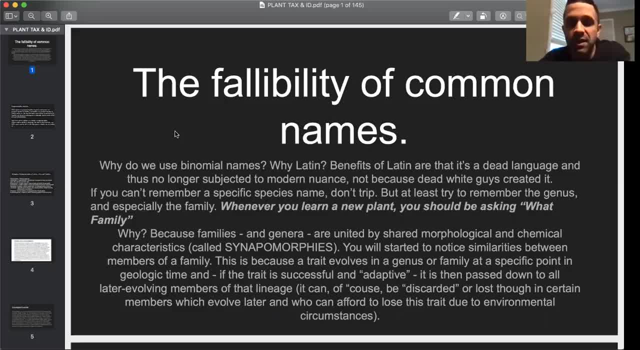 they were secondarily lost. That's the word for it- secondarily lost. But generally you get the idea. you know that that trade is passed down and all descendants have it. you know it's like I got a giant fucking schnoz. I could fit quarters in my. 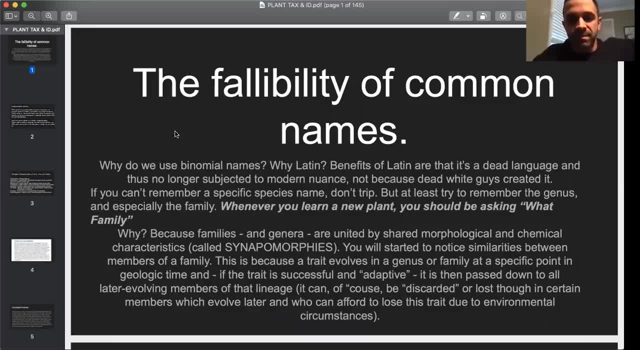 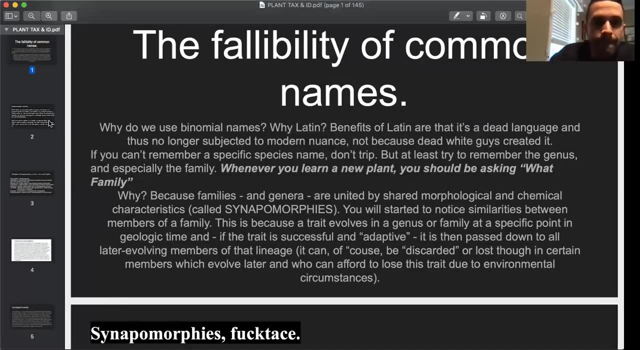 nostrils. That's because my dad also had a giant Italian schnoz and he could fit quarters in his nostrils too. Okay, General, general idea, just you know to make an analogy. So, moving right along, how the fuck? here we go, There you go. Synapomorphies, fucktastes. I did this last night. 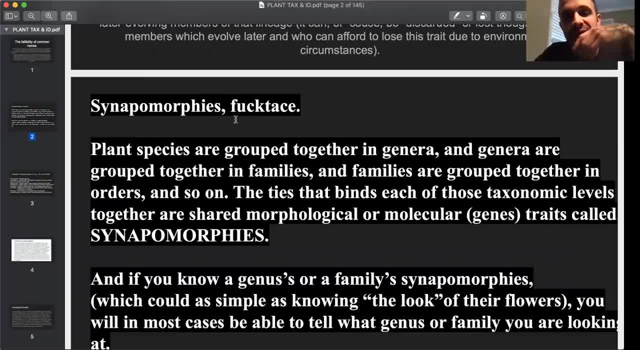 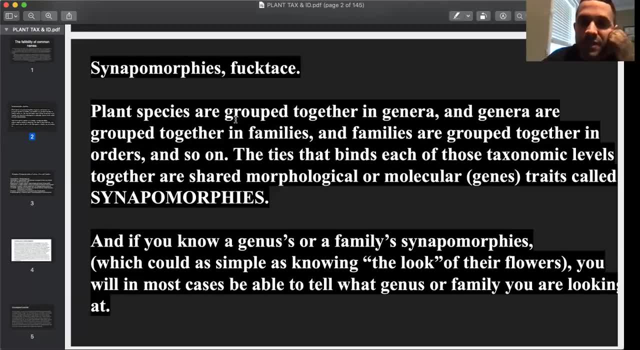 I put this present, this slide together when I was like running around a track typing on my phone. So typing is a double layer of hell for me. Uh, but anyway, there you go. New word: uh, plant species are grouped together in. 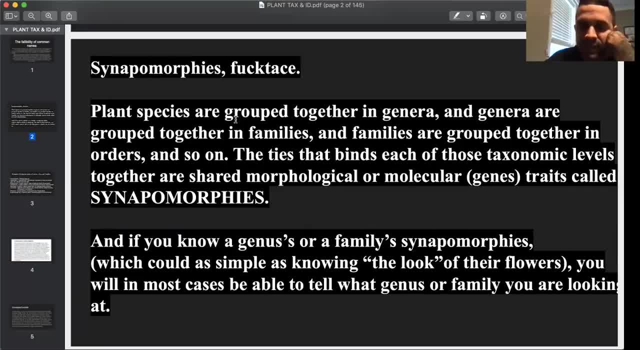 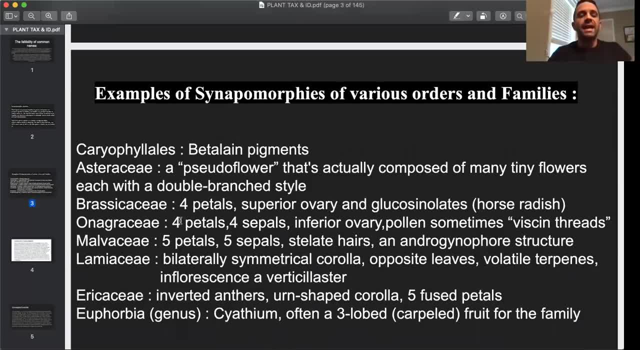 genera- This is what we just talked about- Synapomorphies, et cetera, Moving right along. Uh, here's some examples of synapomorphies, So like Asteraceae, and we'll get to this later. 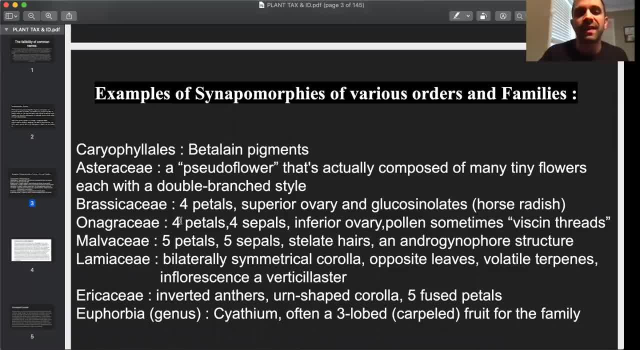 the sunflower family, a pseudoflower, a pseudanthium- uh. that's actually composed of many tiny flowers, each with a double branch style. Now, other families will do this too. They'll, they'll make a, they'll group a bunch of tiny. 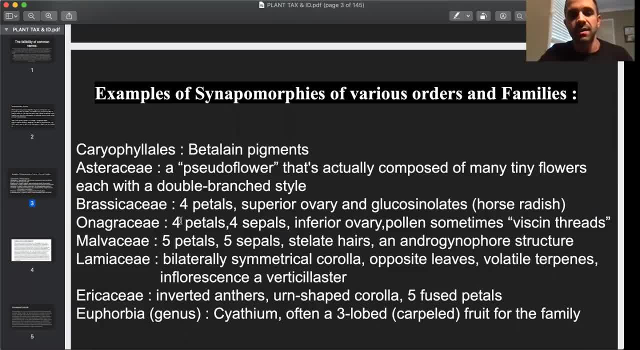 flowers together to make it look like one flower, because that's a better pollinator attracting. but nobody does it like Asteraceae does, with the same arrangement of bracts, the same shapes, the same, you know, bifid, double branch style that looks like a Y, et cetera. Brasticaceae, 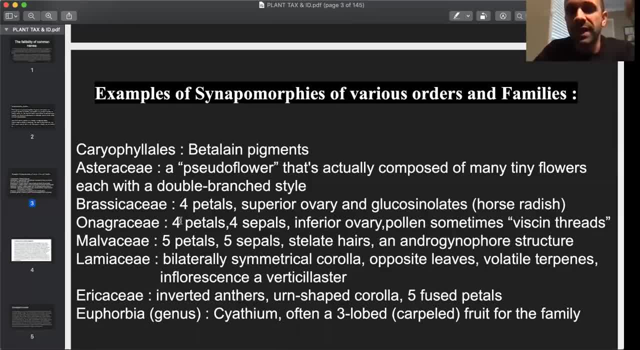 the mustard family, four petals, superior ovary and glucosinolase, which are a chemical. uh that you know. horseradish is a good example. It's like a basically like a sulfur containing compound with a stink to it, And of course, that discourages animals from wanting to gnaw on it. 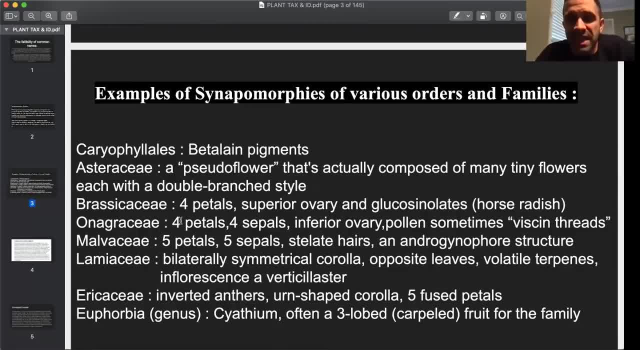 So glucosinolase is an idea. It's an example of a chemical synapomorphy. Um, you'll see a lot of numbers here: Onagraciae, four petals, four sepals. You always want to pay attention to numbers and we'll get into this too. 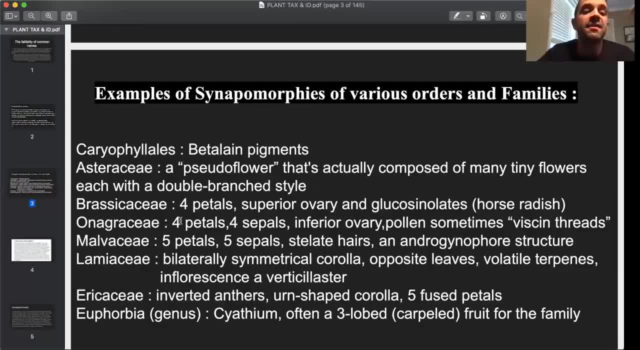 when you're looking at a flower and trying to figure out what the fuck you're looking at. Onagraciae: five petals, five sepals, stellate hairs. There should be two L's there. Stellate hairs just mean stellate, just means star shaped, So it's like a star shaped hair. 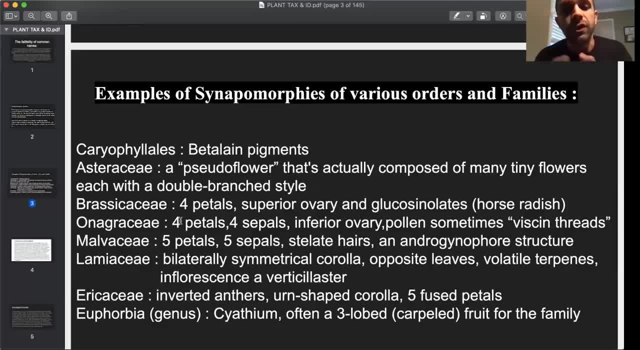 It's a very particular style of hair, or trichome, that you'll see on a lot of members of uh, the cotton family. You know, I think you look at you live in California. you know the plant, flannel bush. it's called flannel bush because the leaves are covered in stellate hairs. 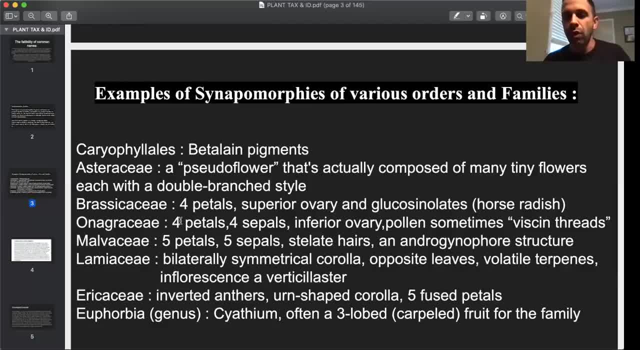 And androgynophore. you don't need to memorize that word. It's just the type of structure, a type of structure that applies to flowers. But uh, you know, that's if you see an androgynophore. 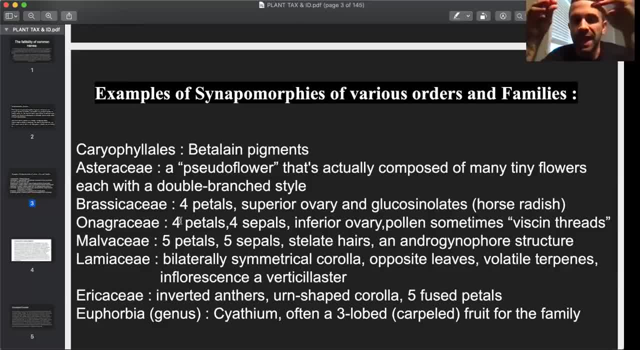 like: look at a hibiscus flower, you've got all those little, what look like little hairs at the top of a column, in the center of the flower, And then at the top of that is the female part, the pistillate part, the stigma: Androgynophore again. the word androgynophore is just the human. 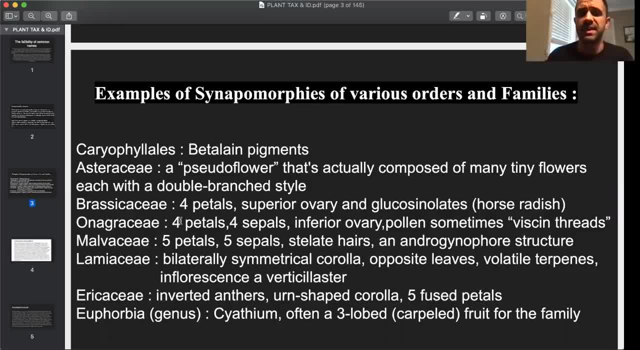 way to think of this type of flower structure, the way that the stamens and pistil are arranged, But that particular type, if you look at like a hibiscus flower, that, the center of that, that androgynophore that is specific to Malvasiae. 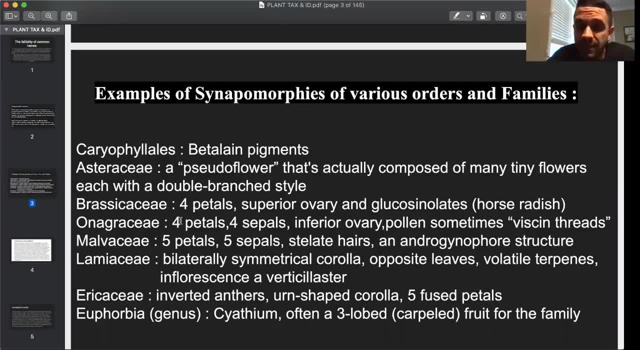 not all Malvasiae have it, but a lot do. And if you see it, you're looking at a fucking member of the cotton family, Malvasiae Lamiaceae. bilaterally symmetrical corolla. opposite leaves: volatile terpenes. you know just a fancy word for this thing: Fucking stinks. 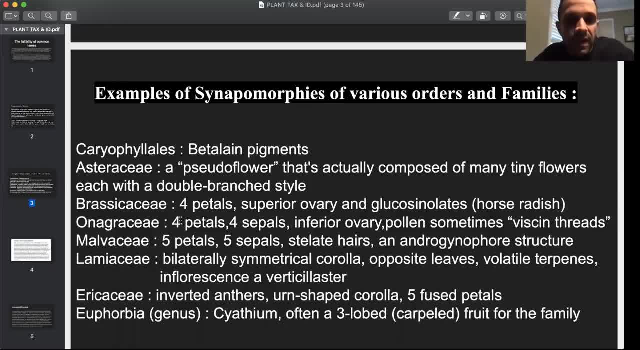 It often smells pleasant, at least to humans. uh, and inflorescence is a verticillaster. Again, verticillaster is just a, a form of a grouping of flowers. You know, you can look that up later. It doesn't matter, right now It's just. 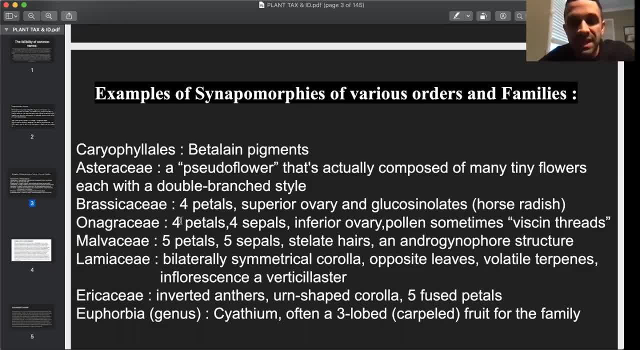 often. uh, you know, if you see some of the verticillaster, there's a good chance it's in Lamiaceae or in, uh, sometimes in Lamiales. Budleia is in the order, Lamiales, and that they. 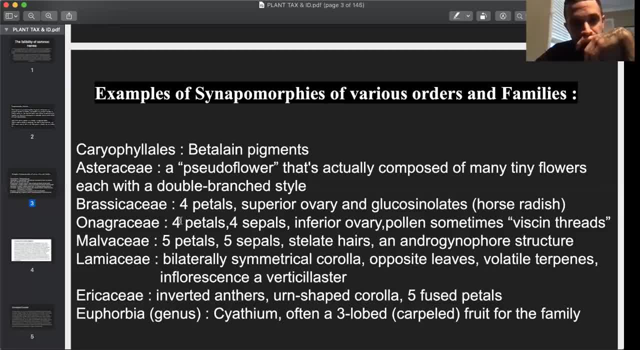 have, uh, often have- verticillasters too. Um, and we'll go through all the taxonomic levels too. you know, or at least the four you need to fucking remember: Arachaceae, blueberry family, inverted anthers. You'll see that with a hand lens. 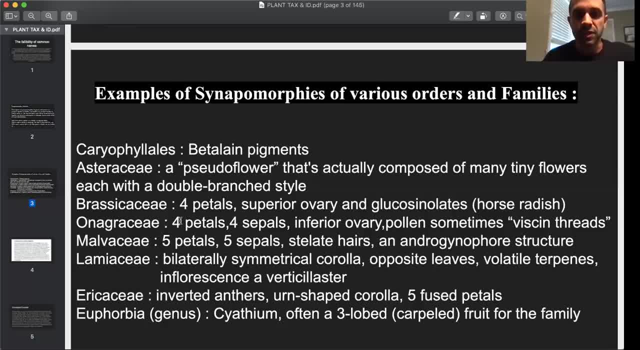 You know, you get one of these jeweler loops like 10 bucks from Jeff Bezos is creepy ass or wherever you know, and those are. they're fucking great. They're cool. Just in general. to look at anything, It's like a mini microscope- uh, you know, a low power microscope in your 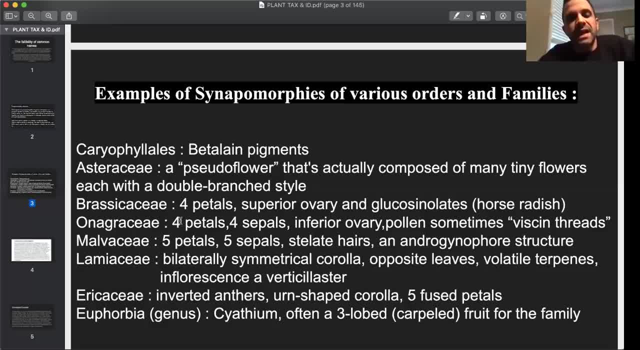 pocket. I carry one around with me all the time, but especially for looking at flowers. there's a lot of shit. you can see that you you may not see. I had a tiny tick on me the other day. Didn't bite me yet, but I couldn't figure out if that's exactly what it was or some other bug. 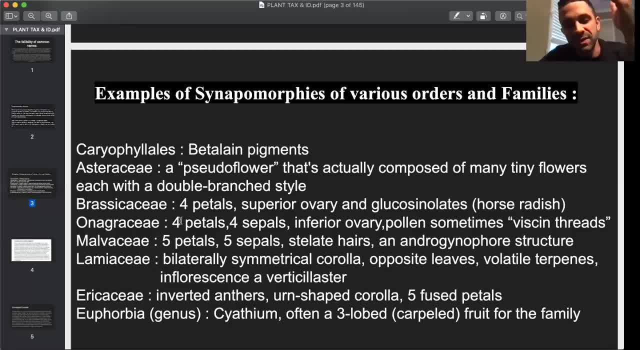 Took out my jeweler's loop. Sure enough, I was like, oh my God, I'm going to die. I'm going to die. If it was a little nymphal tick, it was fucking gross. I set the fucker on fire and that was it. 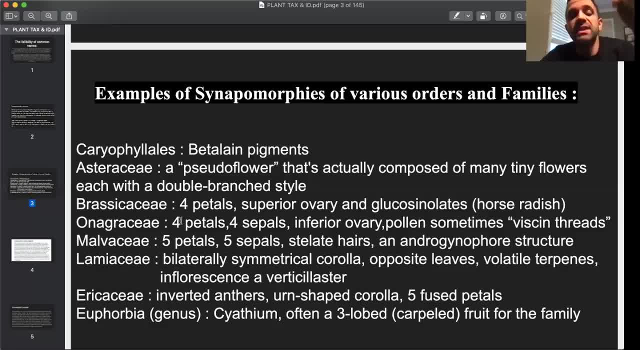 Uh, euphorbia, they have a cyanthium. If you see a cyanthium, it's in the genus euphorbia, the poinsettia genus um, often a three lobed carpal fruit, et cetera. But again, don't be. 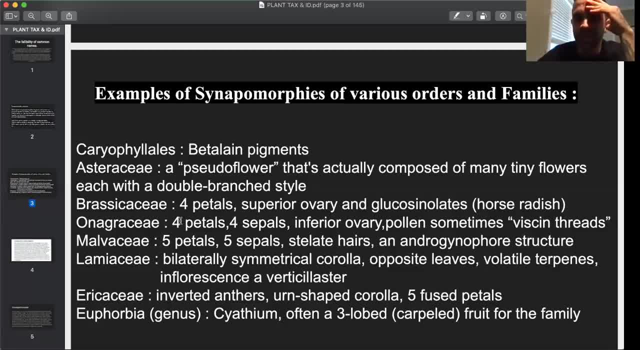 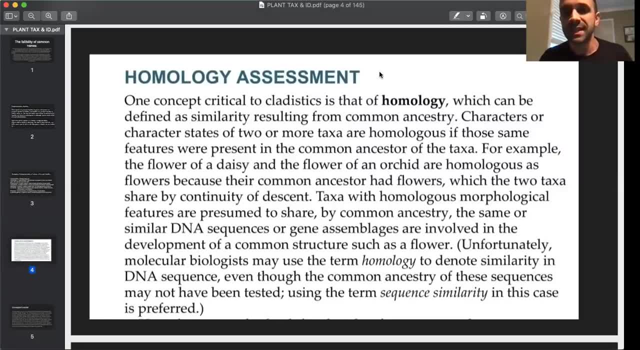 intimidated by all this technical talk, man Cause you can. you can look this shit up and teach us of it. Homology assessment: Homology is just a fancy word for saying that two traits, or the traits that two different species or genera have, are that both those two individuals have those. 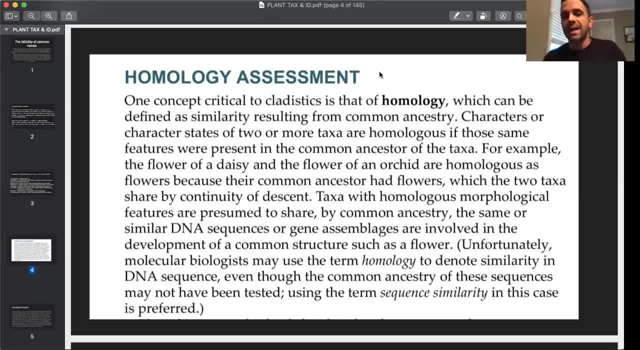 traits because of shared ancestry. Okay, Again, we'll go back to like the big daggo nose that I have. you know, my half brother also has a big David, big daigle nose. Okay, It's cause our dad had a big Italian schnoz and apparently that allele was dominant. So anyway, the homology. 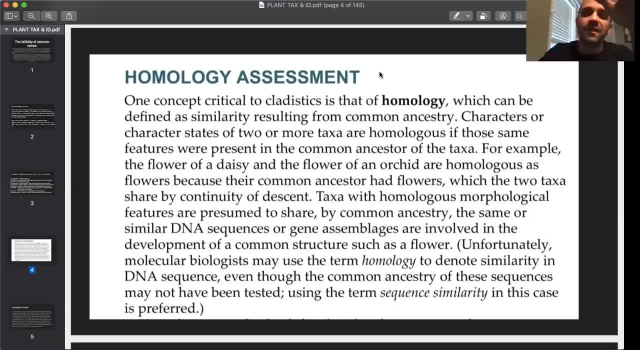 is just another word for a synapa morphine, Homology. Anyways, homology is just another word for synapomorphy, kind of they're they're somewhat synonymous. the opposite of homology, which we're going to talk about, is homoplacy, which means that these two plants- and this is what we're going to- this is 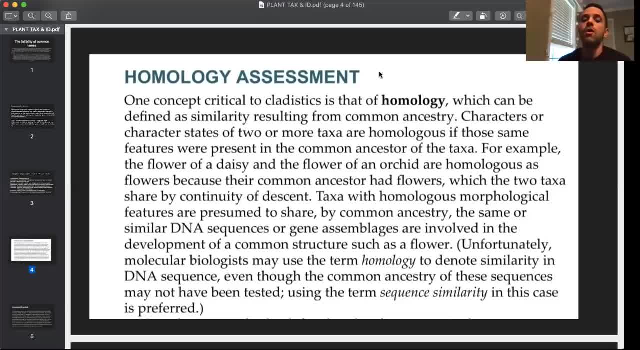 important idea to understand too: convergent evolution. so homoplacy applies to convergent evolution. it's, you know, a great example people always use is cacti and euphorbia, like the south african euphorbs which you'll see planted a lot in los angeles, you know, a lot of people see them. 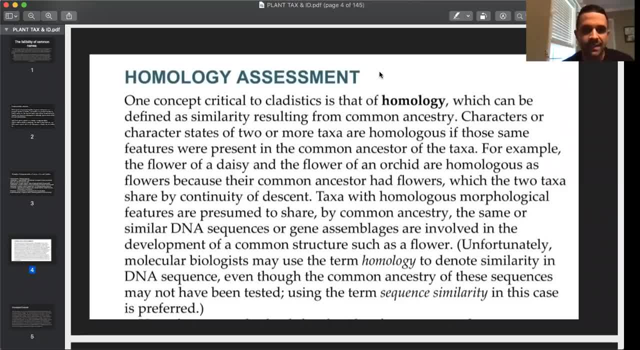 and they think they're cacti. they look like cacti, but they're not related. they're not directly related at all. they've just both evolved similar traits due to similar environmental conditions, and i'll show you some examples of this. anybody got any questions so far? 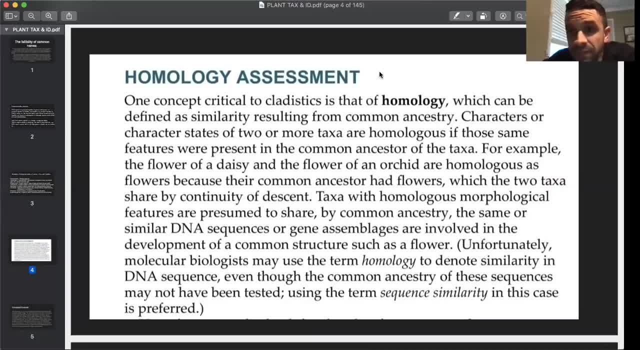 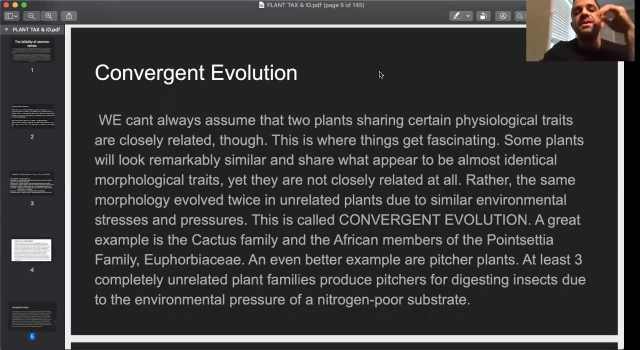 no, no, thank you. it's nice, clear. thank you for coming. okay, here we go. evolution: we can't always assume- this is just what i was talking about- that two plants sharing certain physiological traits are closely related. okay, this is what will fuck you up. people always send me pictures. and, on another note, somewhat 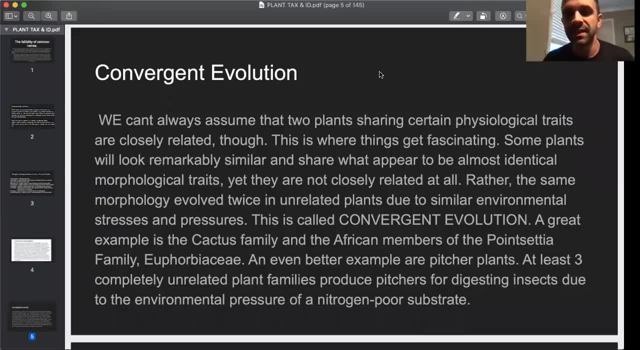 related. people will send me pictures of leaves and be like: what is this? you know, and the dudes in fucking asia or something i don't know. i know, send me a picture of flowers and i can tell you what it is, but just leaves i don't know. a lot of plants have similar looking leaves. 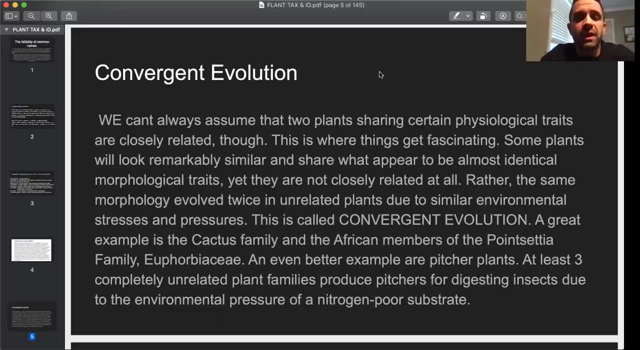 you can look at leaves and be like that's a fucking blah, blah, blah, but generally you need flowers anyway. we'll get to that later, uh, but this is where things get fascinating. the convergent evolution, though it can be frustrating if you're trying to learn- uh, you know, plant taxonomy or 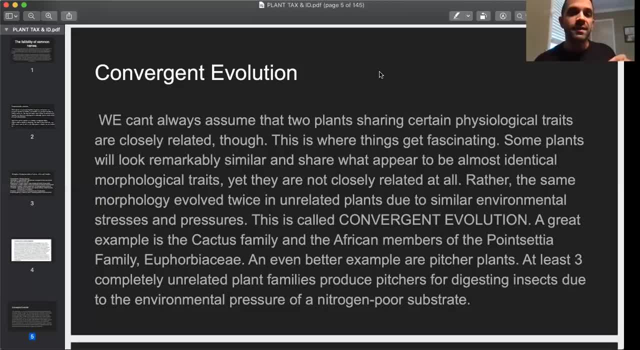 plant id. it can also be fucking fascinating- and this is what, to use the term wet. my whistle about evolution is seeing that two things look so remarkably similar but weren't related at all. and why did they look so similar? because the same environmental stresses that uh- to use a somewhat uneloquent term- sculpt those traits out, the same environmental conditions. 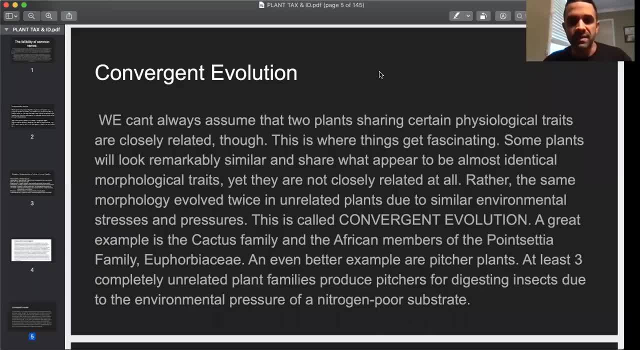 existed in each respective plant's environment. now, by environment i mean you could talk about you. you can mention climate geology. herbivores are part of the environment. pollinators are part of the environment. these are all stresses or or beneficial. you know what's the? 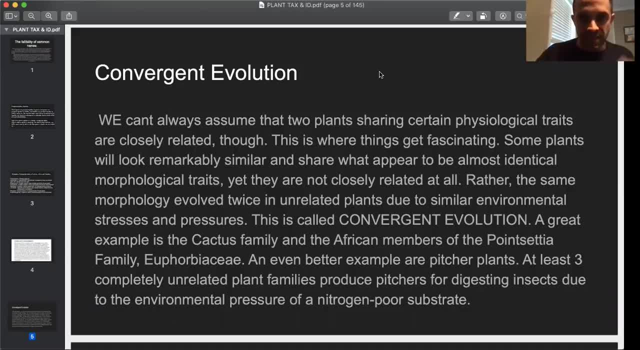 how do you say it? how do you say it? stress things that can accentuate alleles and and traits and plants. so you know this whole idea. the idea i want you to get is that the environment sculpts new species and can also cause the extinction of species. so the environment is responsible for how plants evolve and what 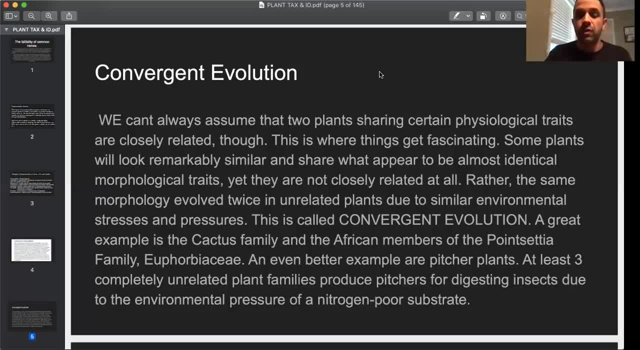 succeeds and what fails. now, of course, we're part of the environment too, and we're causing a mass extinction right now. uh, you know the kt meteor that hit 66 million years ago that was. that was an environmental stress that caused a lot of extinction. but there's also, you know, the hummingbirds growing in an area in the in the. 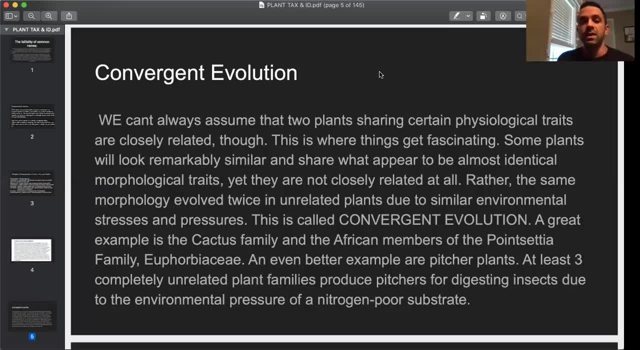 andes with a high hummingbird diversity. that's also, uh, a part of the environment. and that what is? what's the result of hummingbirds being abundant in your environment? you're going to start to evolve red tubular flowers which insects can't really see- at least bees can't, because they don't see that. 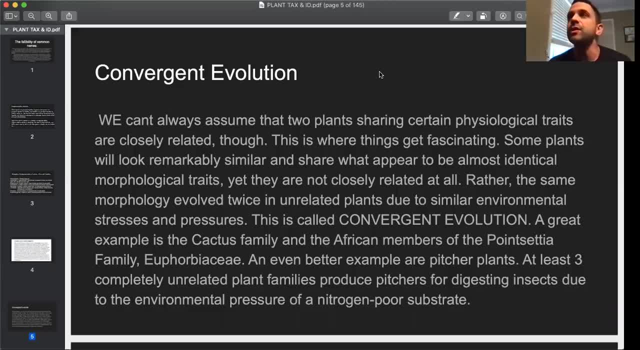 pigment. but hummingbirds, do you know? i mean anytime you see a red tubular flower you're like that thing's pollinated by hummingbirds, maybe if it's in, you know, south africa, there's no hummingbirds in the quote old world, but it's pollinated by a bird. it's pretty. it's pretty fucking cool. and these 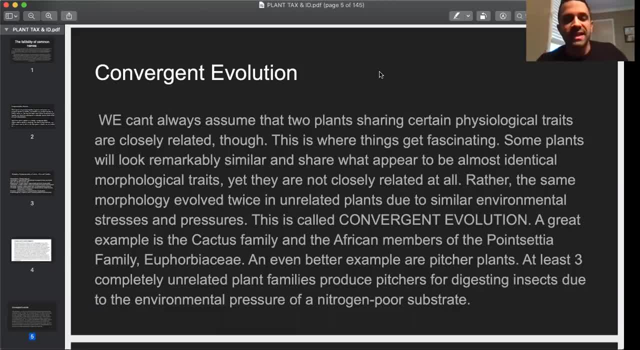 are the things that really you know. get you, get at least me, get me fascinated with the world. it's like everything is connected, everything is influencing everything else, um, so anyway, this is called convergent evolution. a great example. we already talked about cactus family and euphorbia family. even better example- and this, this fucking blew my mind when i see it- is this one. so 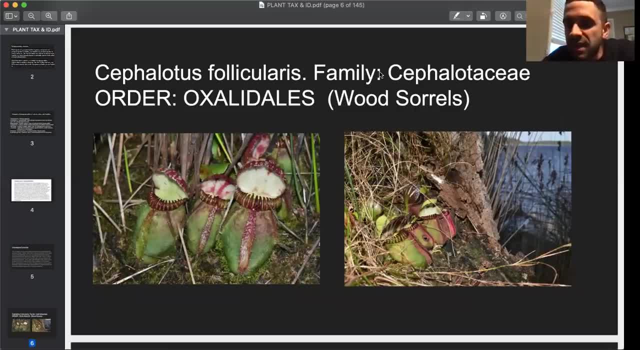 this is a plant- cephalotus follicularis- it's uh, from western australia- grows in a relatively small area. i was there last- the fuck, was it a year and a half ago, october. these things are relatively small. they're, like you know, two inches at most, just growing right on the this, this embankment. 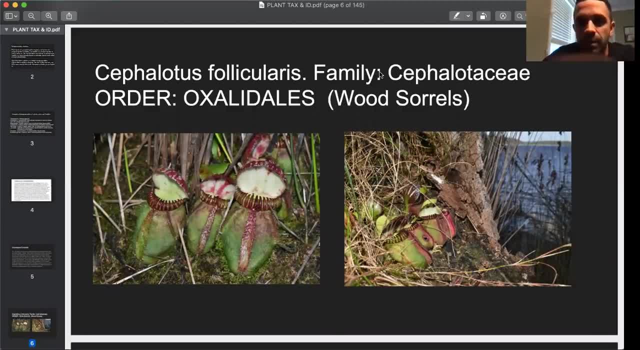 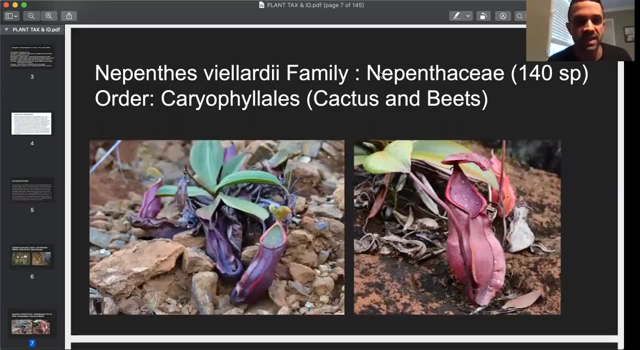 this seep, uh, near this estuary or bay. they look almost, i mean, to someone who's not familiar with botany. they look almost identical to this guy, uh, kind of look like saracenia purpurea too. right same thing, if you want another example. 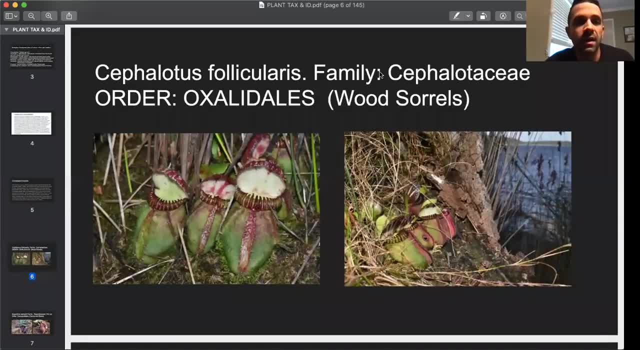 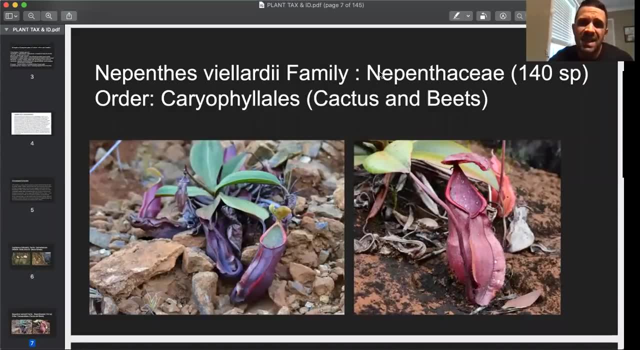 all: saracenia, nepenthes, uh uh, cephalotus, they're all they're. none of them are directly related. they're all just morphological responses. saracenia is in. is that in caryophyllales or ericales? i forget either way. 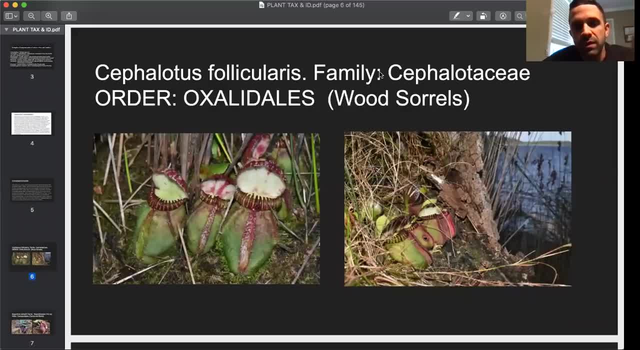 um, they're not directly related. these, these are both: this form, this morphology, these are things that just evolved, uh, evolved on their own, independently, on each of these lineages. and what was the thing that caused it? a, you know, shitty soil, lack of nitrogen in the soil. you know, with any carnivorous plant there wasn't enough nitrogen and so you know, maybe, uh, maybe, a you know at first started to curl and an insect got trapped in it or insect got stuck to it or whatever. and then that proved adaptive, that trait got accentuated. 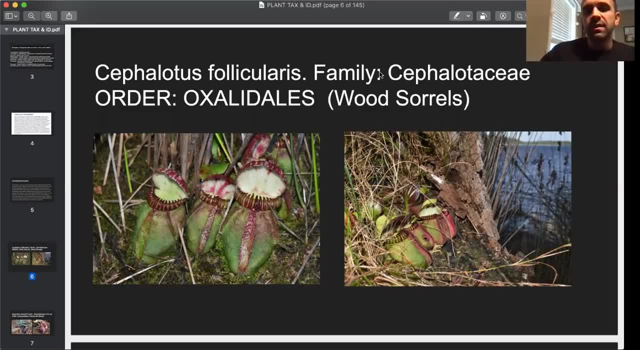 the plants that had that trait, uh, that mutation, uh thrived, and the ones that didn't have that trait didn't thrive as much, uh, or they went extinct. and so just these little baby steps. generally, sometimes they're big steps, but these little baby steps end up leading to this, i mean. 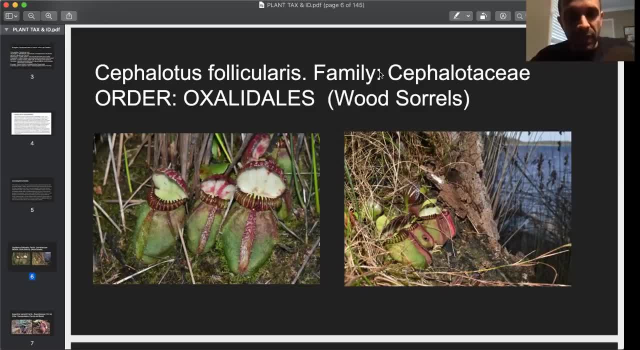 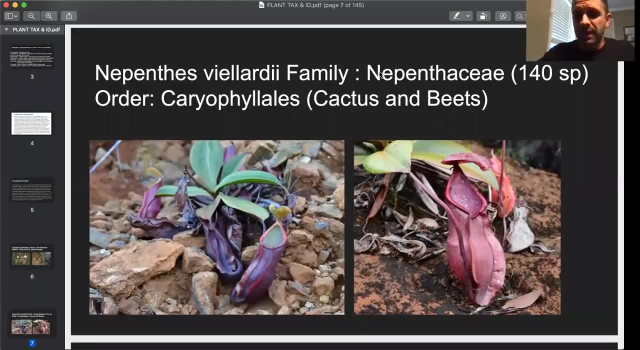 you could look this cephalotus even has that lip. you know, that ribbed lip, the peristome that nepenthes had. this doesn't isn't a great example, but it's a great example of what's going to happen in the future. but there's some species of nepenthes that have like a really prominent peristome with those ruffled ridges. 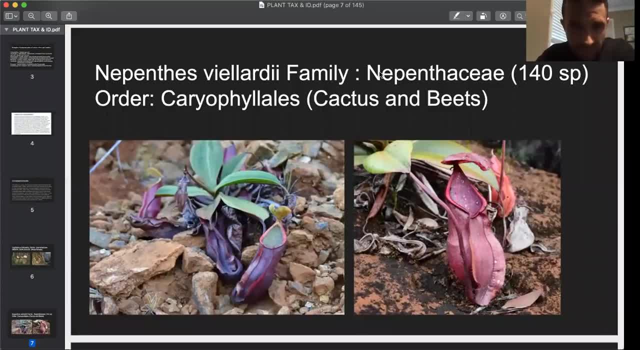 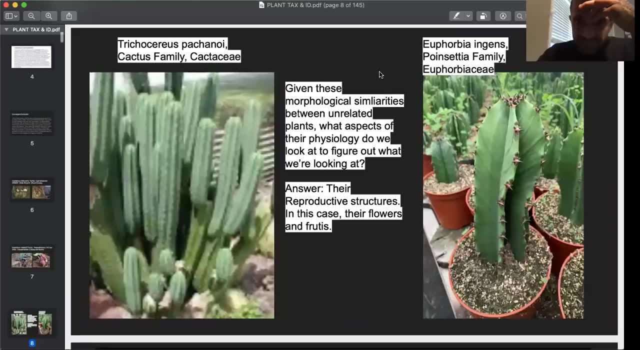 this is nepenthes viardii. this is from new caledonia. it's the new. it's the only species of nepenthes that grows on on new caledonia. this is a shitty photo because i stole from the internet. this is trichocereus pacanoi, the one that 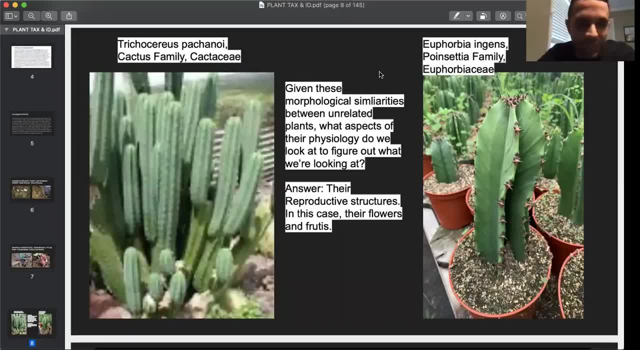 all the the druggies love, right, that's whatever your gateway drug is into botany. you know i'm for it. you know. you see, these guys who got like big cat, all their photos are just of like trichocereus and peyote. 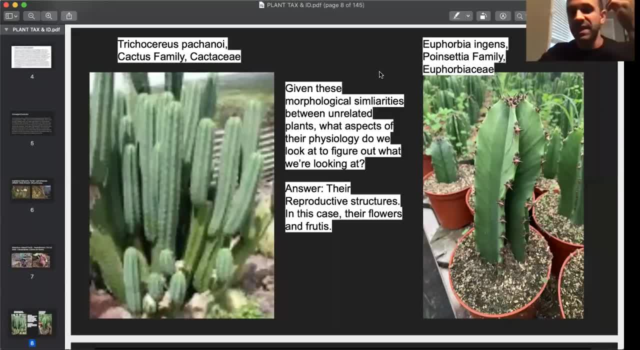 all right, okay, you know, try to get them looking at things a little differently, looking a little deeper, looking at plants that can't be used for psychedelic purposes, but anyway, trichocereus pacanoi- uh, you know, looks exactly like this plant on the right, not related to it at all. 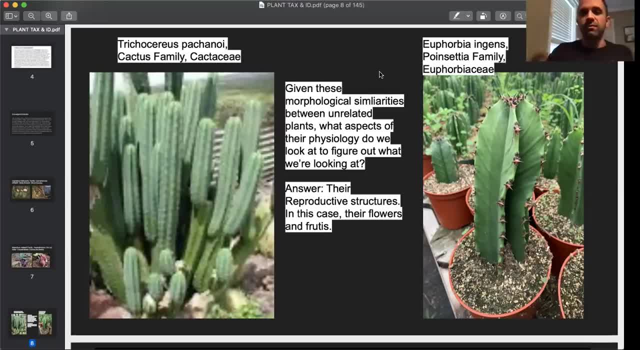 not even in the same order, but again, they just evolved these similar morphological responses because they were the only green thing on the menu in an otherwise relatively comparatively barren environment. you know, these big photosynthetic organisms, an area with no trees- no big trees at least- and so they're going to be the first thing that herbivores try to. 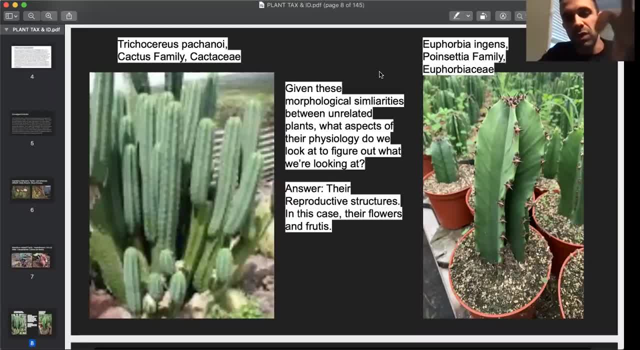 go on. so or you've got this immense selective pressure of herbivores just gnawing anything down that doesn't have these spines, or or harsh chemistry- a lot of cacti have you know secondary metabolites, chemistry. in them they produce compounds that you know, like mescaline is a. 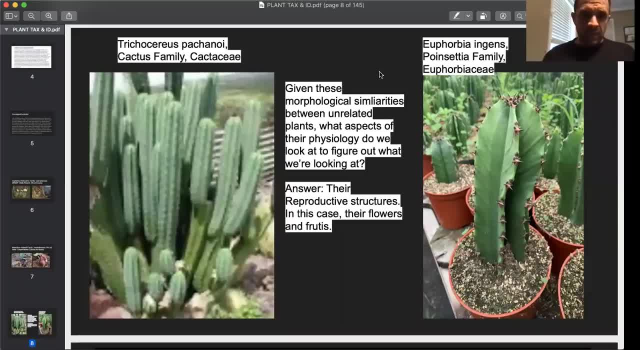 sample like you. sure humans can use it to, you know, have vision, quests or experience, uh, altered states, whatever. but if you're a rabbit and you eat mescaline, you're going to have a fucking bad day. and so that mescaline was a beneficial, the production of mescaline was an adaptive. 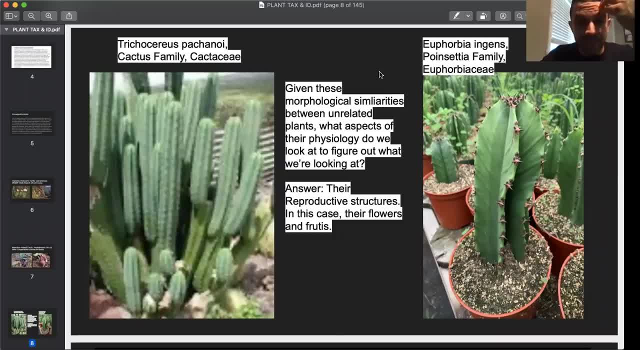 trait for many cacti. many cacti produce mescaline, not just trichocereus and not just peyote. in peyote the concentration is really high. in trichocereus it's a little bit less, but even like some of the stenocereus. 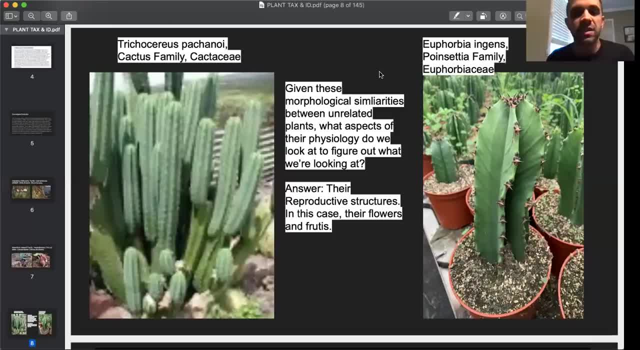 produce mescaline, not in any really usable amount to a person. but you know- and that brings up another point which i don't want to diverge on this too much- but you know, some families in genera almost seem pre-adapted to evolve. not just once, but sometimes dozens of times the same response. 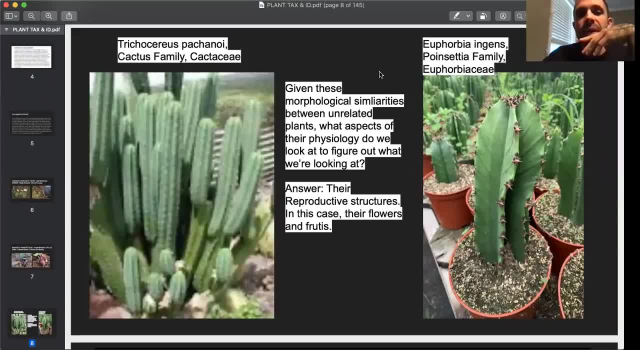 to, you know, a fucked up soil, or or, uh, the same response to herbivore pressure. so you know, this production of mescaline might have evolved, you know, a number of times, but in the cactus family, so it's not necessarily that, that, uh, that you know everything that has. 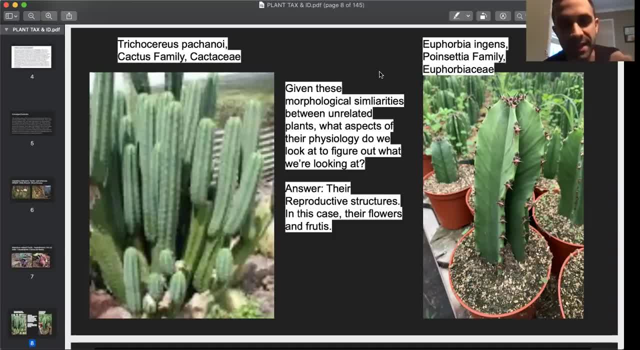 mescaline is directly related and shares a common, immediate common ancestor. sometimes they just, you know, evolve it, uh, on their own, independently, you know. another good example of that is the genus streptanthus which i got photos of later. got some nice money shats. i'll show you streptanthus. 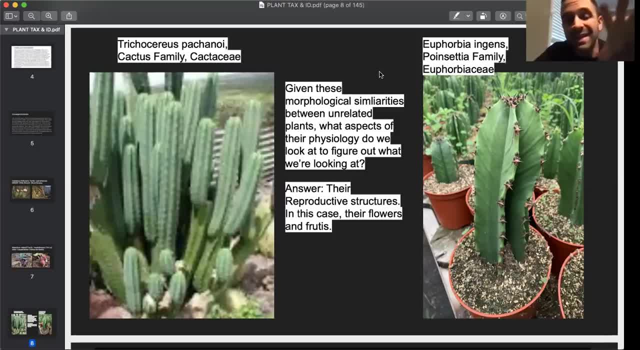 you know, in the genus streptanthus, which is in the mustard family, that genus has evolved tolerance to the fucked up chemistry of serpentine soil, like six different times, you know, and this has been. this has been figured out just from looking at dna sequences and comparing them. i mean it's. 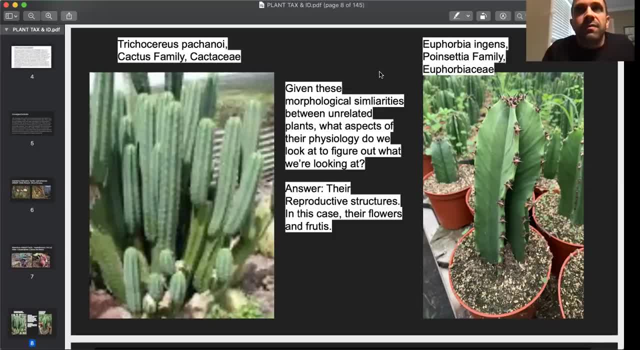 it's a pretty remarkable thing. so you know- and i've talked to my friend tom gibnish about this too- there's there. in some cases there's all almost a pre-adaptation. a pre-adaptation, the genetic toolbox is already there and it just ends up working itself out over time. another reason i 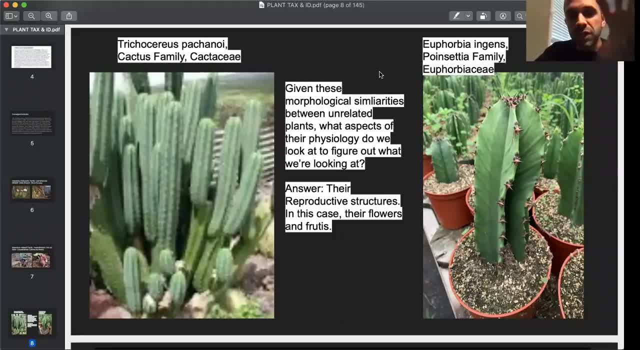 love thinking about evolution is that there's a lot of people who are thinking about evolution is because you know, when you think about evolution, you're just de facto going to be thinking about deep time, these immense amounts of time, uh, that it takes for these things to evolve. 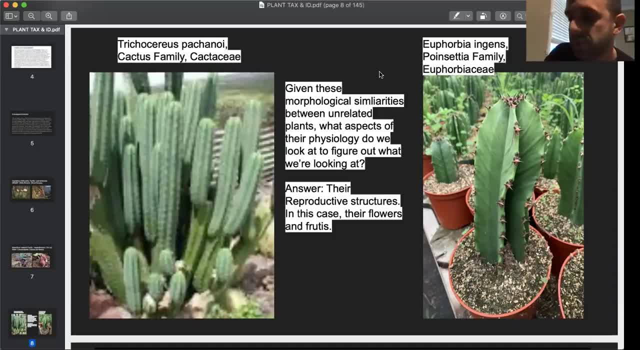 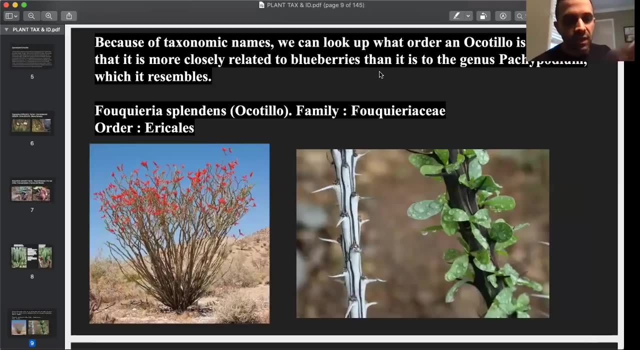 you know, or for these relationships to evolve. sometimes evolution happens pretty fast. oftentimes it happens relatively gradually, you know, over many, many, many human lifespans. so moving right along, okay, another great example of a convergent evolution: you got ocatillo. anyone fucked around in the southwest deserts in north america, uh, is familiar with this genus: 12 species. 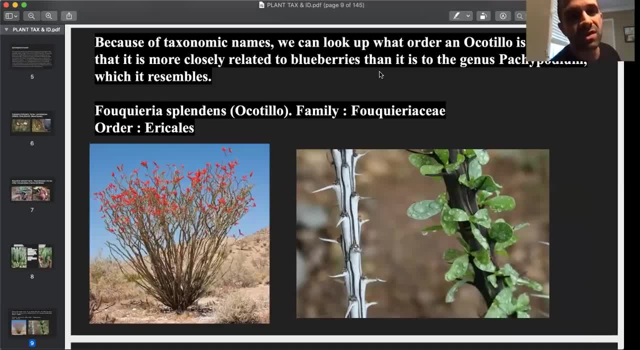 in this genus most people only know focaria splendens, which is the only one that grows in the united states. here you go, little uh, mildly succulent, it, it drops its, uh, it drops its leaves in, uh, and you know it's like drought deciduous, which you explain that to someone who lives in. 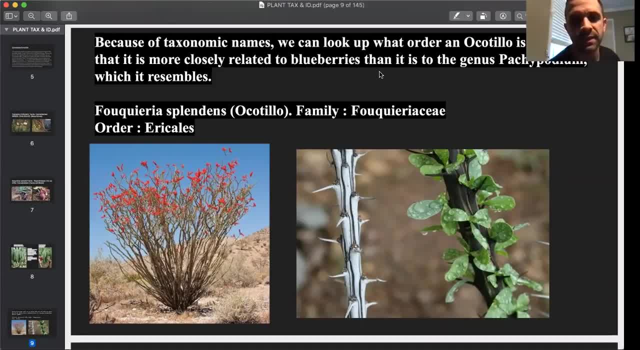 minneapolis. they're like plants: drop their leaves due to heat too, no shit, and they survive. they're just adapted to that. yeah, a lot of forests from india to mexico, to wherever you know, seasonally dry forests, do this. to madagascar, etc. to australia, do this. they will drop their leaves and go dormant when it's just too fucking. 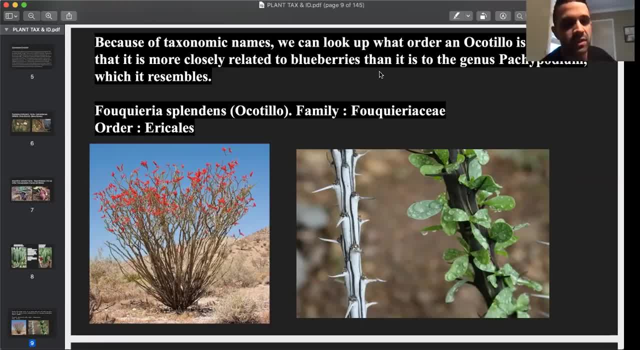 hot and rains, you know not going to be arriving anytime soon. anyway, ocatillo- uh, you know you can see these, these spikes, that's drought, deciduous red flowers. looks remarkably similar to another completely unrelated plant, ocatillo's, or also in the order: eric kelly's, the blueberry order. 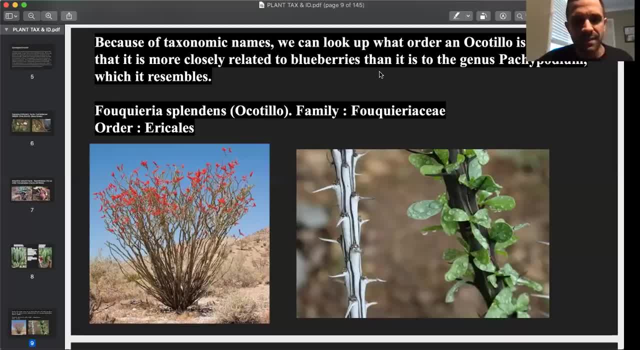 and i just called the blueberry order, not because you know blueberry shares any sort of evolutionary novelty for this order, but just to get human beings, uh, an idea of what. okay, that's the blueberry order. they can, you know, connect it, just to give them a mental connection to a plant. 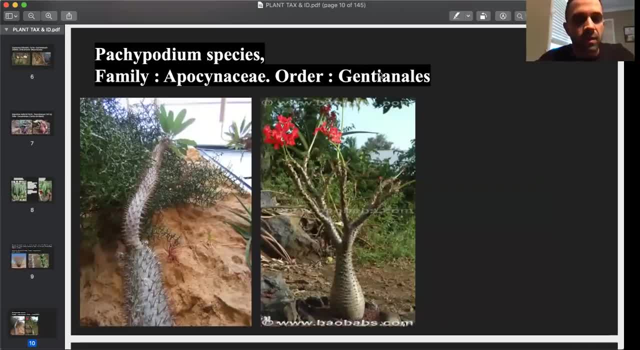 that everyone's familiar with. so ocatillo looks remarkably similar to this. okay, i mean, to me it doesn't, because i'm familiar with both of them, but there's someone who's who doesn't know yet- maybe your grandpa or something- they'd be like: oh, it's an ocatillo. 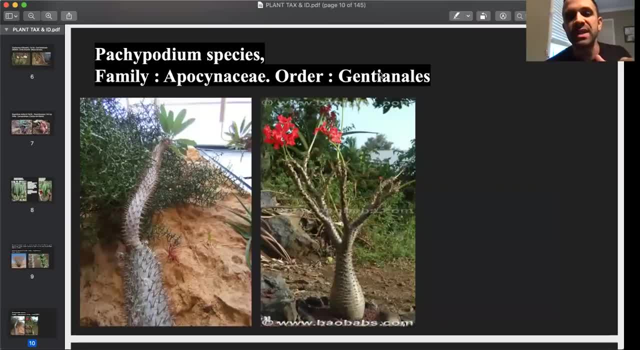 i mean no, they just again convergent evolution. similar traits evolve in response to similar environmental stresses. this is pachypodium. this is i forget what species it is, don't really care. not i like them, but i just. until i see a plant in habitat, it's hard for me to get. 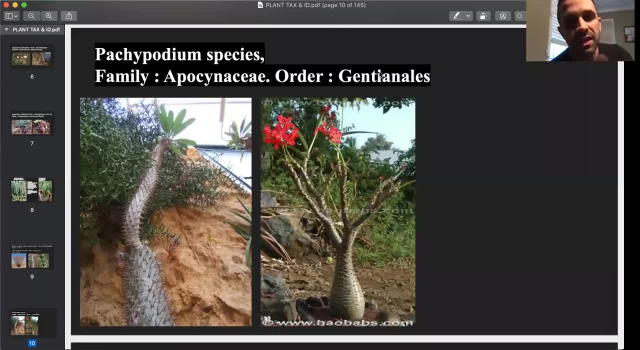 enthralled about it, but regardless, this, uh, this species, i believe, is from madagascar, it's it's more closely related to oleander than it is to ocatillo, and ocatillo is more closely related to blueberries than it is to blueberries, so it's more closely related to blueberries than it is to. 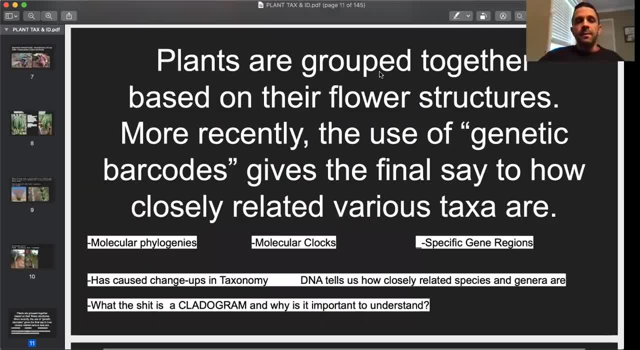 this. uh, plant right here, uh, before we go into this. anybody got any questions? no, okay, am i talking too fast or is any of this shit flying too far over your head? don't be afraid to speak up. my job is to fucking teach you this shit, not to uh, you know. 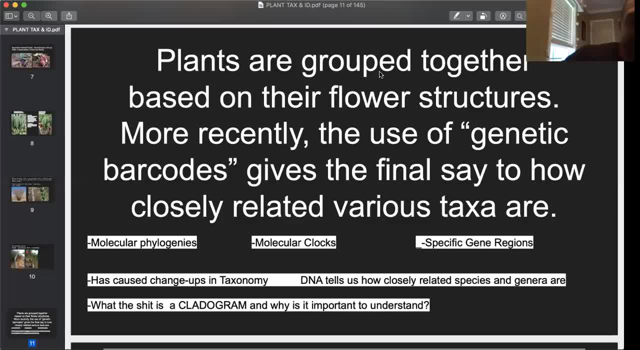 all right, fine, to me, all right, yeah. yeah, i've got one, uh, and maybe you're gonna go over this later, but so if we're trying to use this plant right now, we're gonna use this plant right now to ID things based on family, but also families can look similar due to convergent evolution. 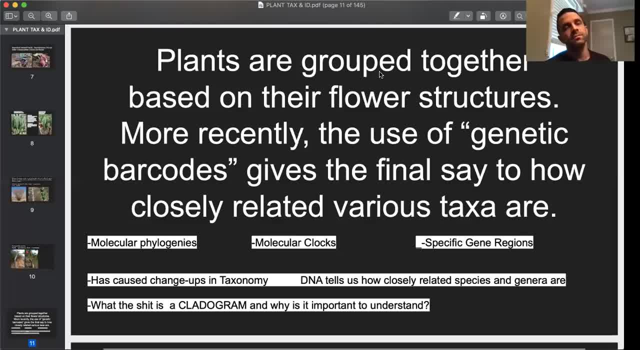 um, how do you kind of get around that when you're, when you're trying to, to use, you know more plant morphology, to to do an ID or at least identify a family? that's a good question, and i could be pissing in a bottle right now and you wouldn't know it, because i'm just kidding. uh the well. 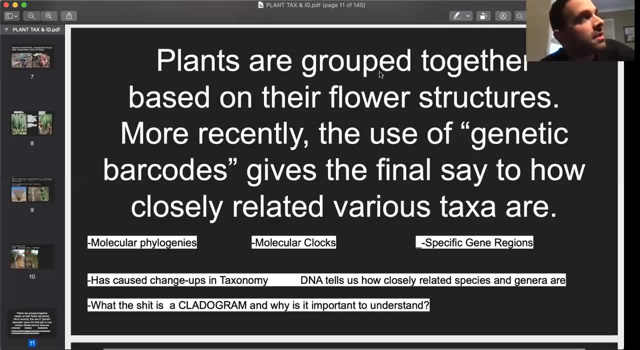 that's just part of the. uh, you know, there's, there's books, there's books that you can find. you have to books help. but you know, i guess the idea with convergent evolution is you just got to look closer, like with euphorbia. are the spines really the same if you look close? are the spines? 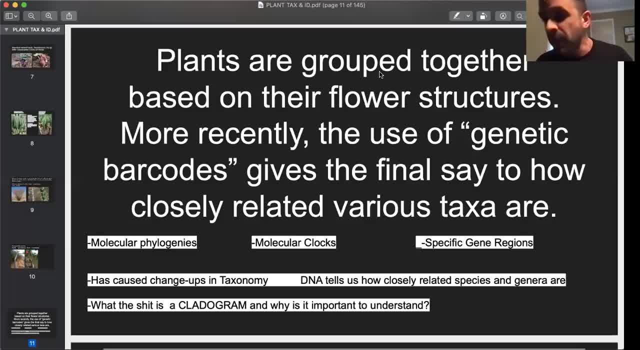 really the same as the spines you see in a cactus? no, what is the base tissue? you know, if you look close, like i, can look at a euphorbia and be like that's a fucking euphorbia. there's maybe one or two times i've looked at one and been like: is that a fucking euphorbia? or a cactus like there? 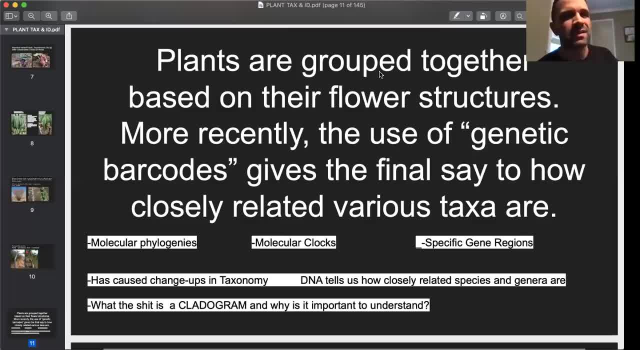 i remember there i was in the highlands of not highlands, it was like two thousand feet of Oaxaca, near the Oaxaca- Puebla border, and i saw a plant and i was- i knew it was a cactus, because those big columnar euphorbia are native to north america- uh, but i looked at it and i was like that. 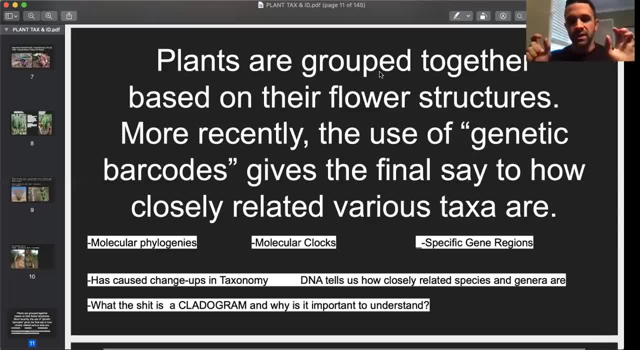 is fucking. it looks so much like a euphorbia because its spines were somewhat reduced. they weren't that long. uh, the texture of the stem, you know, i was like it was on a steep hill, i was like 12 feet away, but it's like that looks so much like a euphorbia. the species name was euphorbia. 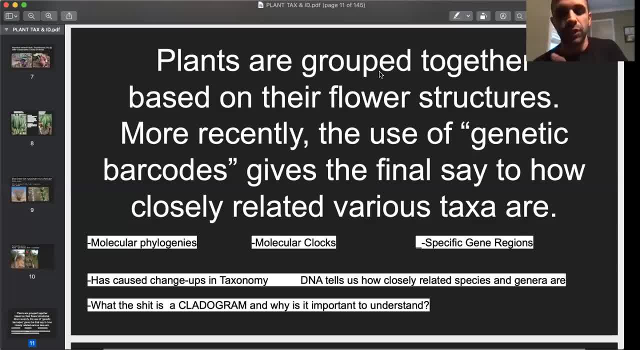 coincidentally you anytime you see that oides. it means looks like like coia glyptostroboides. it's called that because it looks like glyptostrobus, which is a related genus in the redwood family. but anyway, the point was, you know most of the time if you look close. 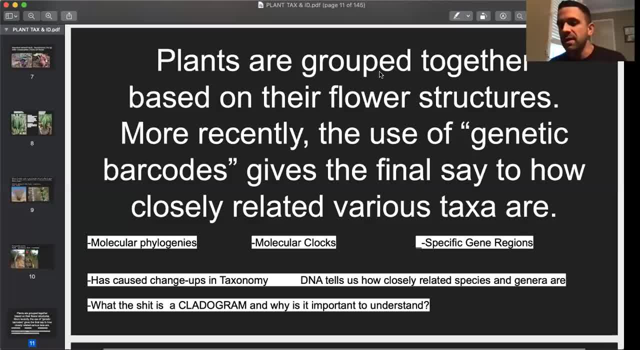 you can be like, ah, you know, something seems off euphorbia. if you look at them long enough, you know, or if you've been looking at them for, or studying this stuff, or just paying attention to it. eventually you start to pick up on those differences. the base tissue that spines are. 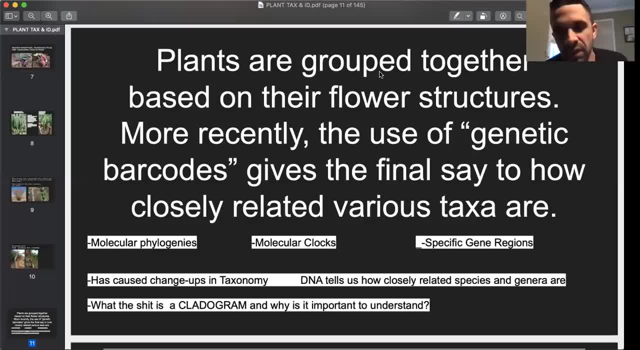 derived from in in the euphorbia genus are stipules which are like a type of brack that kind of protects emerging leaf tissue. okay, in cacti, the the spines, people say cactus spines are leaves. not quite, they're axillary leaf buds, but if you look at them close enough you. 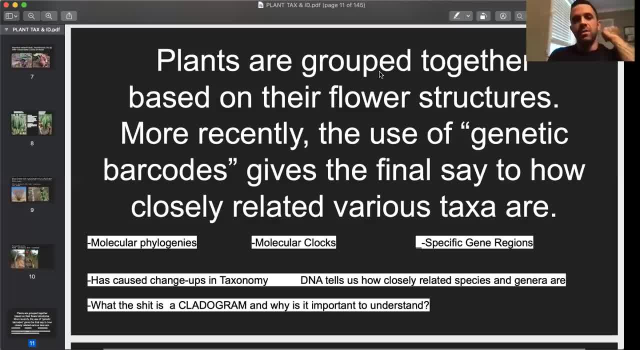 could see the differences where they, where they are, uh, in terms of, uh, you know that, that bud tissue, or whatever. so, and then, of course, the way to get around it, and this is what i'm getting to here. the main way to get around it is flower structure. a euphorbia flower in no way looks like a cactus. 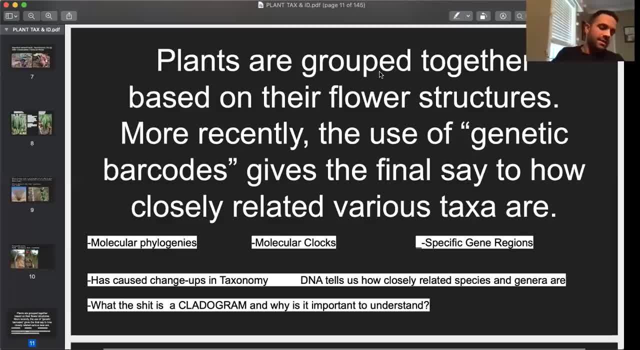 flower completely different. so that's why i'll say: you know, this is the thing to get across too, and it when i first got into plants, you know it took me a while before someone told me this too. this is like 10 or 12 years ago. so like, yeah, plants are generally grouped together on the way. 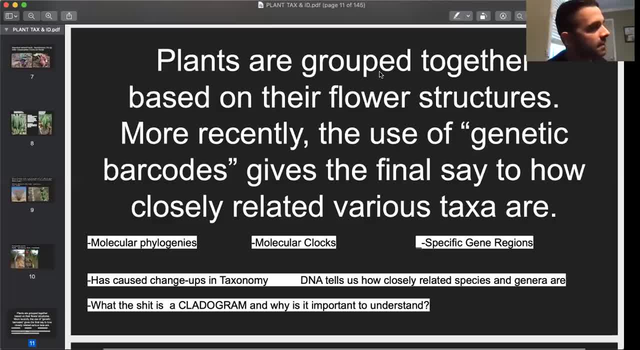 their flowers. look, and this was a thing that got uh linnus in trouble because he was like: i want to group plants together and their fuck parts, you know, and how they look and and puritanical. when was it 1600s or 1700s? whenever that pissed a lot of? 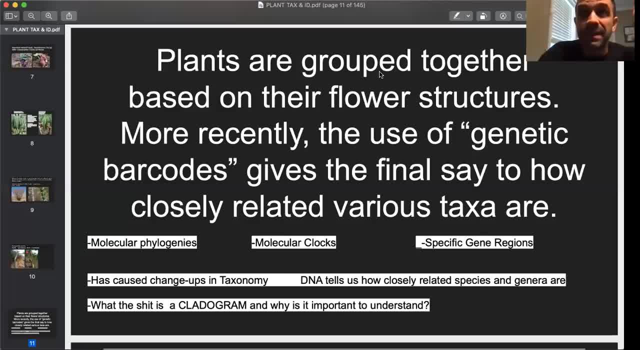 people off, you know? um, can you imagine being alive back then too? i would have been fucking beheaded 10 years ago. but uh, you know that pissed a lot of people off because it was like that's the shit you have to talk about. it was, you know, really prude. uh, square society, you know. 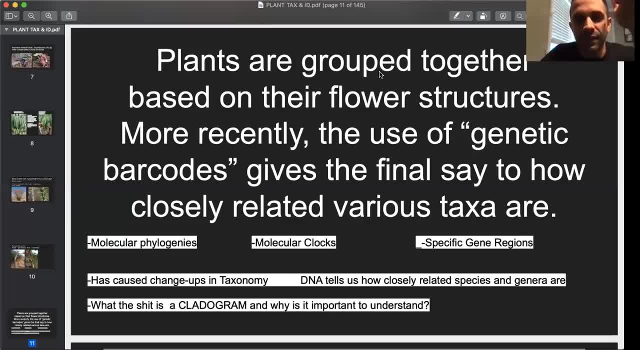 um, i, the theory of evolution was still, you know, 200 years away, so, but you know, he was the first one that looked at that and was like, okay, i see what's going on like. this is the one thing that's generally similar flower structure, because flower structures can't- they can't change too much, you know. 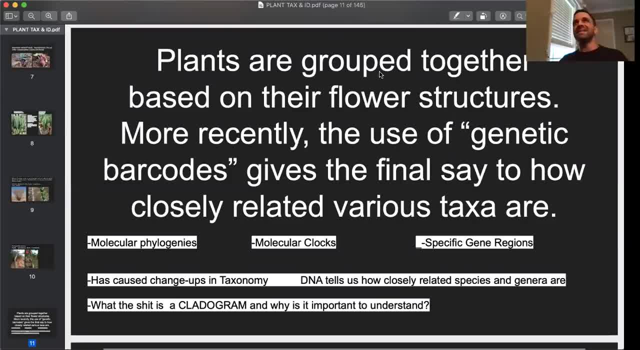 uh, and have things relating to. well, that's not the right way to put it, too trying to say they can't. you know, if you, if you, if you get a big mutation in flower structure- oftentimes it's not adaptive- it'll, it'll cause that lineage to go extinct. uh, when it is adaptive. 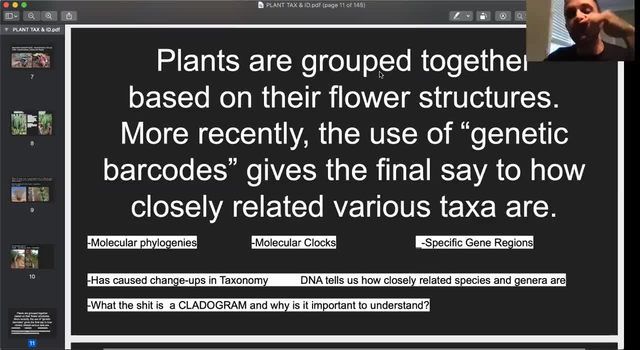 then you get a new family or a new genus, whatever. but the point is, flowers are what you look at. uh, not just leaves, you know. so, like you wouldn't just look at, oh, it's a stem succulent with spines. i mean you, you know that. give you hints. when you look closer, you could look at the spines. 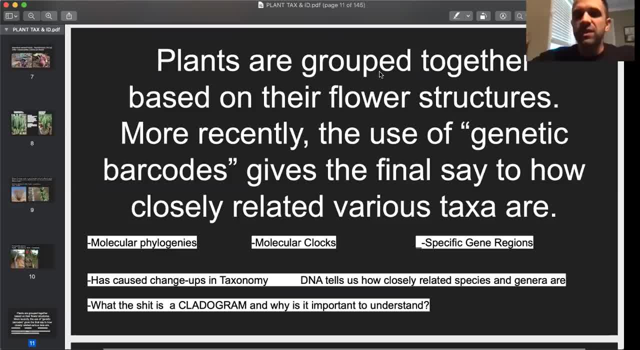 tell the differences, but when that thing blooms, or if you get a fruit, even just the dried fruit, flowers and fruits both, because every flower matures into a fruit. so either one of those that'll give you a that'll, that'll be the final word, and then sometimes that's not even enough. 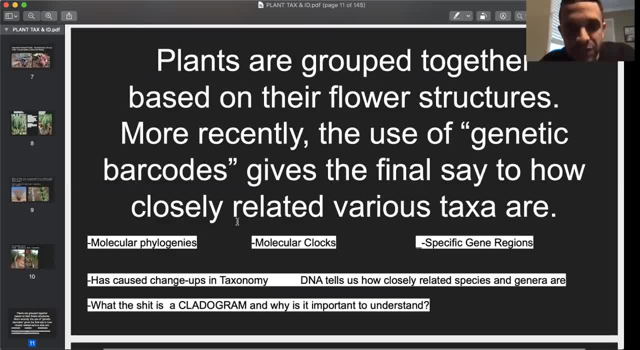 and that's where this shit comes. that comes in molecular phylogenies, molecular clocks, looking at specific gene regions. just think of it like barcodes holding one barcode up to another. nice reference from a consumer society, right, holding barcodes up to each other- genetic barcodes. 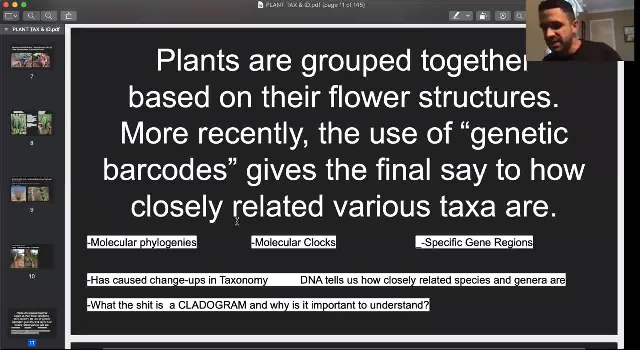 as to what dna is okay, series, atcg, atcg. um, you know there are areas, there are gene regions. uh, you look at different gene regions to look at different levels of relatedness, like are two in the same genus versus comparing, uh, two different families, right? so there's, if this flies over your 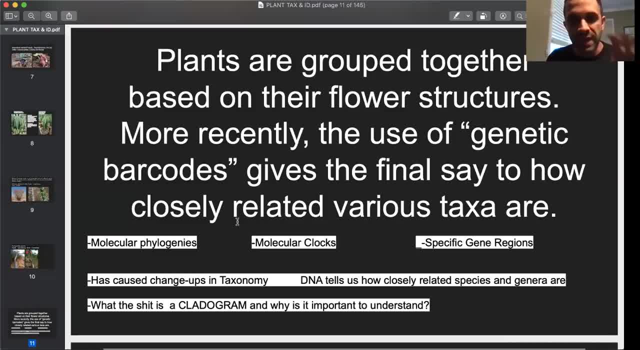 head. don't worry, it's a fucking abstract thing to think about because you can't directly see it. but i'm just trying to plant the seed. so dna is the final word. that's why a lot of things have been switched up lately. you might hear older botanists and horticulturalists talking about it. my friend, 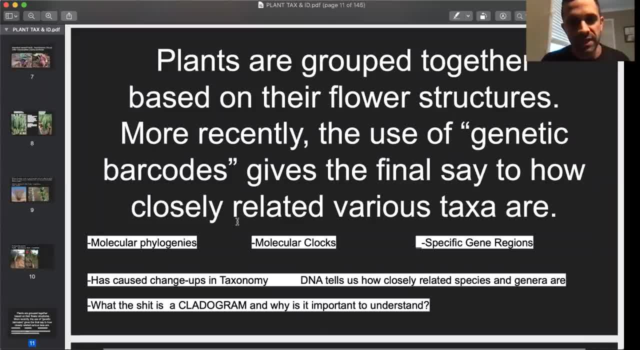 ken hates it and he's like: i don't even know what they changed that genus to now. it used to be in this. i just call it whatever you know- at least i know the species. the species will stay the same, but they'll change the genus name. 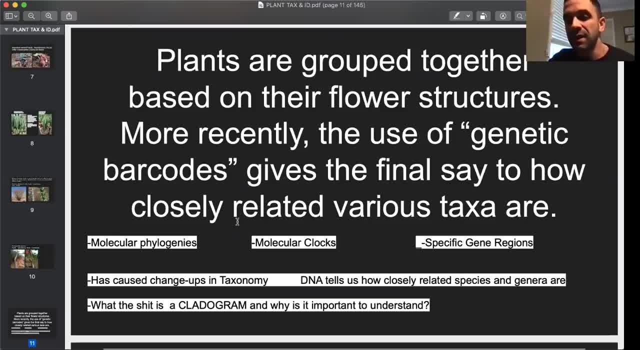 or they'll change the family. this is a great example. yucca joshua trees. yucca used to be placed in uh, the lily family, which is fucking insane. you know you go back to like old taxonomy books. 60 years ago they were classified. some of them classified them in the lily aca, which is like 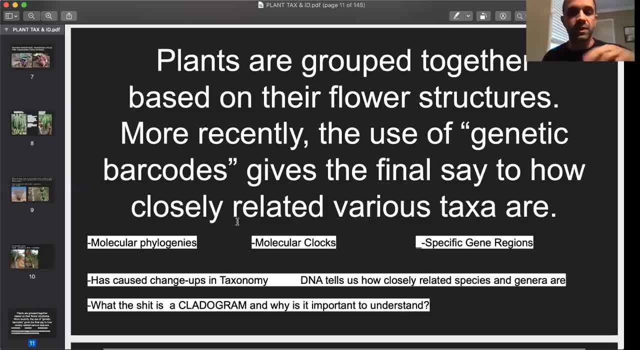 you know the lilies you might buy at the the grocery store, which is insane. it was just based on the same number of of stamens and what was thought to be a similar flower arrangement, but then of course, i mean later on, people, people caught that fuck up before dna came about. but 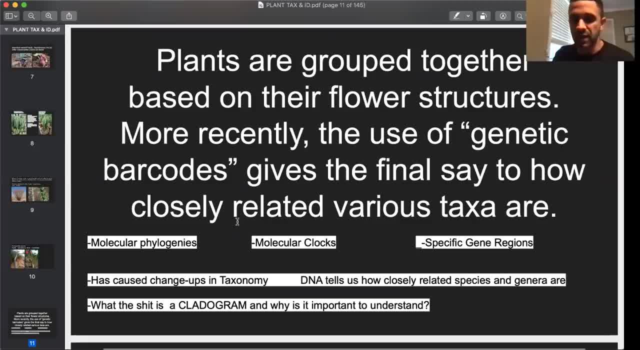 dna has really been in use the last 10 or 20 years, so that's why you're getting all these these, these swapping these switches of uh. you know this genus was in this family and now it's in this family because we, in many ways, dna can elucidate. it can shed light on interrelatedness. 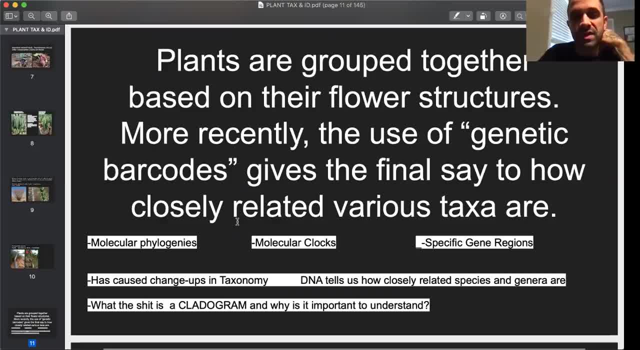 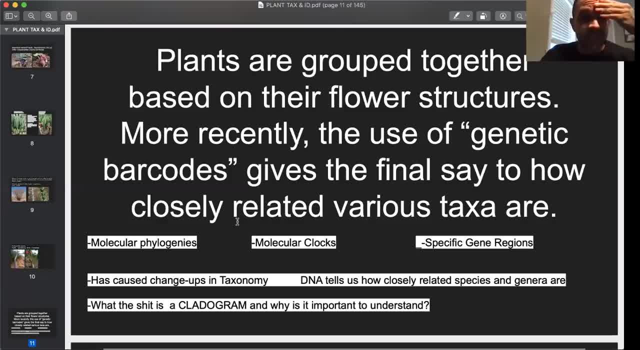 so, uh, anyway, what the shit is a cladogram and why is it important to understand? so a cladogram is just a fancy word for a family tree. there can be different, there can be different ways to illustrate a family tree. it can be like: you know 90 degree angles, uh, you know branching like a 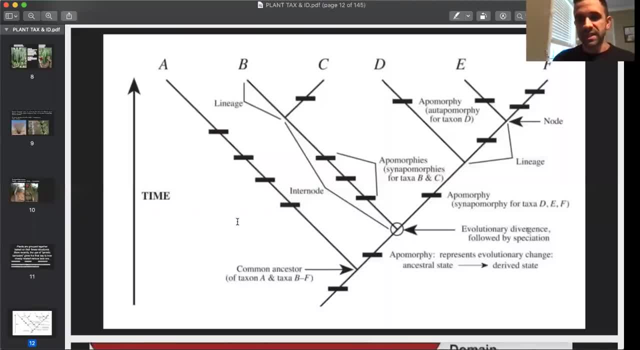 family tree. it can be pyramid shaped. whatever this one is a pyramid shaped. this is just a prototype. there's no plan here. it's just a prototype. the black lines are synapomorphies. um, you know so. and then, of course, you look up. uh, at the top, you got time on the left, so older. 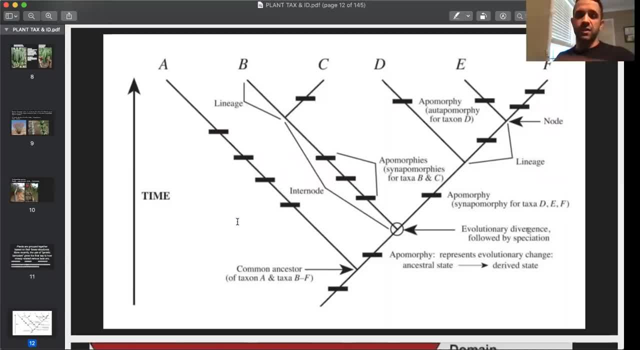 you know lineages that are older or have changed or gone extinct. well, if they go extinct, it's a. you know, they've morphed. they morph through evolution, in the way that the, the environment, causes things to evolve. so, uh, this is a. this is the way it looks. it obviously up by the letters at the top of the. 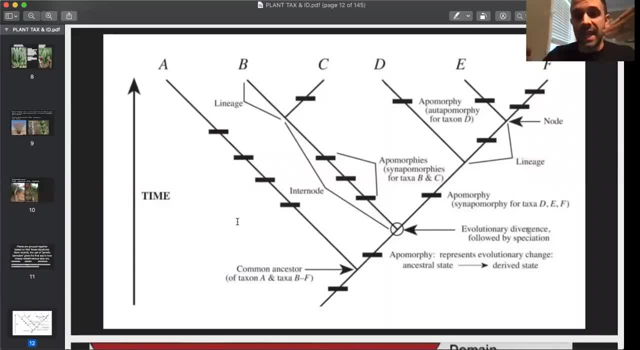 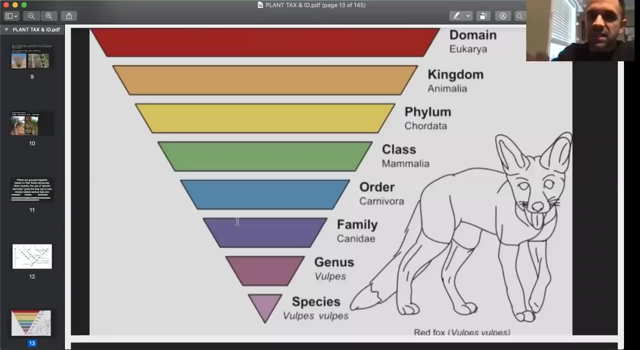 screen. that would be, uh, in general today, where we're at today with these lineages, but it's a cladogram. uh, again, it's just a human way to think about how things evolve and how lineages evolve. okay, so there we go. so here's. here's the general list of tax taxonomic nomenclature. 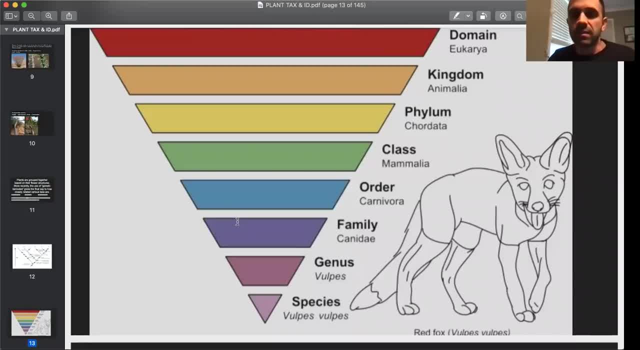 you got domain kingdom phylum class. don't even need to go through the list of taxonomic nomenclature. don't fuck yourself up thinking about all that. i generally only work with order down. you don't even need to focus on order now, because that'll fuck you up too if you're just getting started. 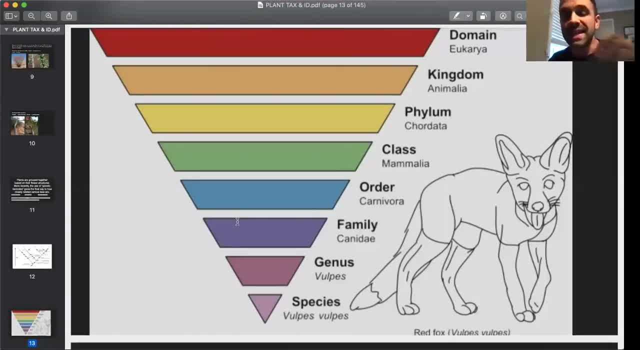 just focus on family, genus and species. anytime you see a plant, you should be asking yourself: what family is it in, instead of asking things like: oh, what does it do for me if i make a poultice and put it- you know- on my, my knee that i scraped? or what does it do if i make a potion? 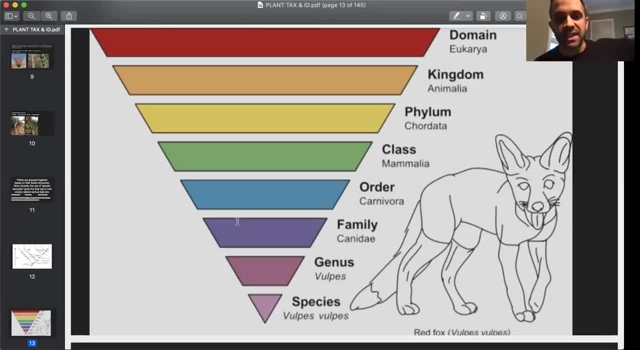 out of it and ingest it. uh, you know. so like you're selling on etsy, for, you know, 100 bucks for a skin cream. well, you got a hustle going on. i want to interfere with that, but the point i'm trying to make is is: uh, anytime you see a plane, you should be asking what family. 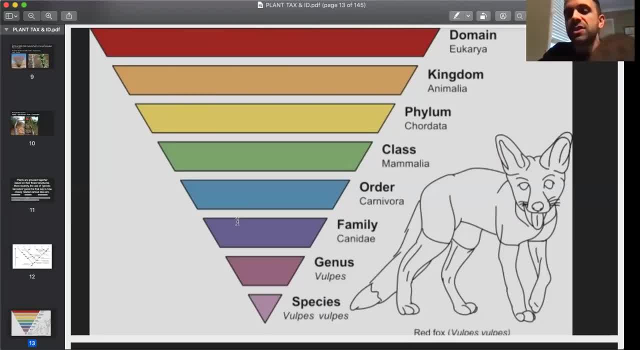 is it in? because if you do this long enough, eventually you'll start to notice traits like: oh yeah, this is in the same family i you know. before i even looked it up, i look, i saw that flower and i was like it looks like it's in this family and it turns out i was right. um, that's the. 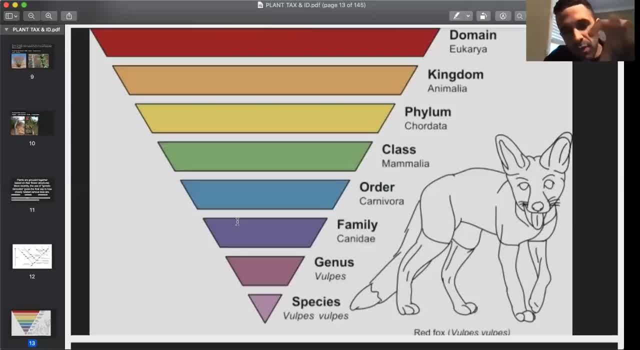 big thing to take away, you know, is that what you start to notice, these synapomorphies, these traits, and that's what makes it fucking exciting, because you can go to a shitty dirt lot, a vacant lot, or go to a fucking train yard or, like, be at a shitty shopping mall and look at their. 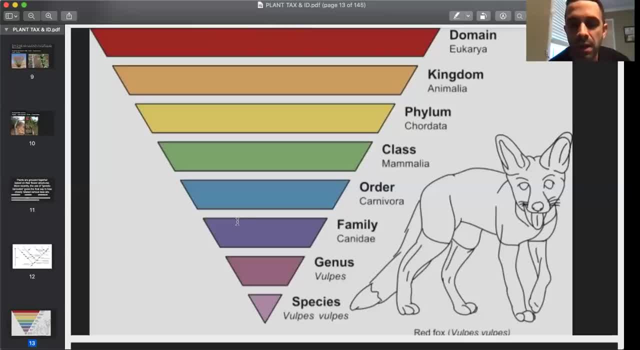 tacky landscaping. if something's flowering, you could be like: huh, look at that flower, look at the way it's arranged, look at the sepals, the petals. why is it arranged like that? why is it this color? uh, why are the stamens and the pistol at different? uh, why are they different lengths? 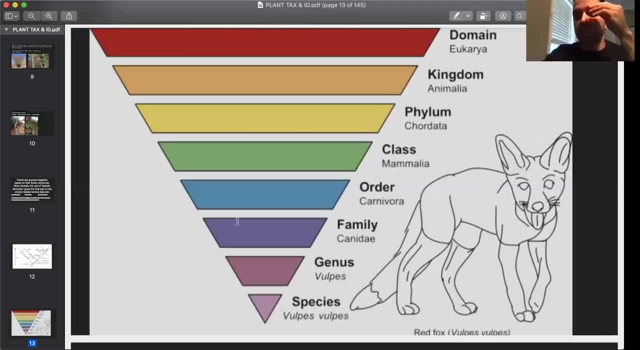 um, and you can guess, you can start to notice things that you know. oh, it's in this family. wow, how about that? that's cool. that's a weird variation on a theme you always hear me talking about in videos. variation on a theme- what the fuck is variation? 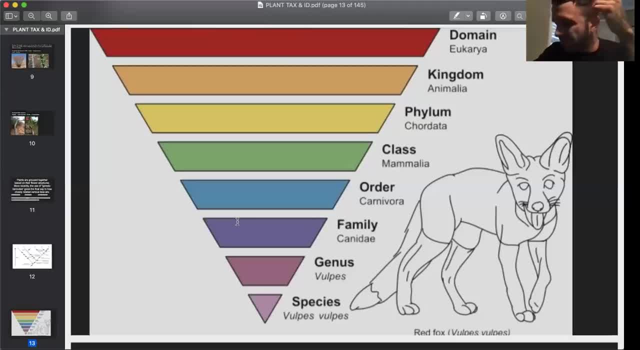 on a theme. i think it was. i forget who coined it. it might have been darwin, i don't know. darwin was endless forms, most beautiful, but the, the, i guess that's an emo band too, but i never listened to him. the point is: variations on a theme. that's what really sparks the imagination. 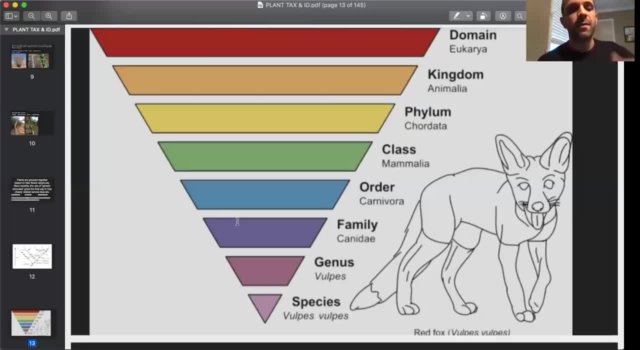 of any biologist you know, because you get to see, you're familiar with us, to say you're, you're right, you live in tucson or phoenix. you're like, i love saguaros. i don't know just something about them: the way they look, the, the, you know the when they bloom and the bats like, and then the fruits. 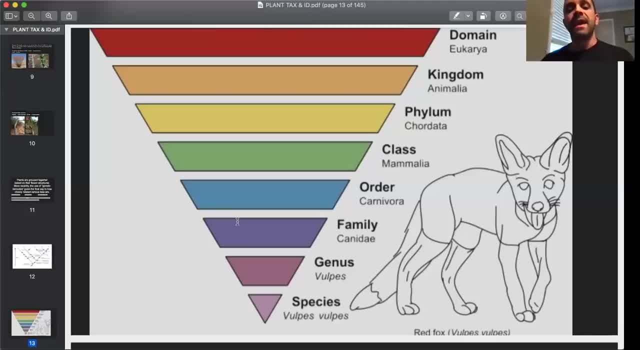 and they're just fucking cool. you know i just like i love the way they look on the landscape. eventually your imagination, if you're really into it, will start- want you know- wandering to other different types of columnar cacti, like neobux, bamiya, like what is? wow, that's a cool. i've never 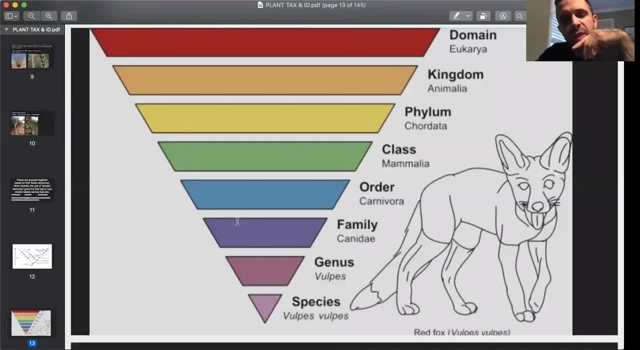 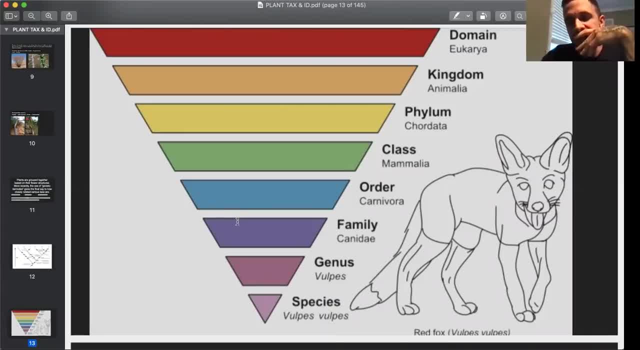 where, where it grows, you know, uh, down there in oaxaca or central mexico, wherever. so you, you start that imagination gets sparked and you want to start learning about you know, you get curious. what other forms have evolved over the last five or six million years, maybe less, i forget how old. 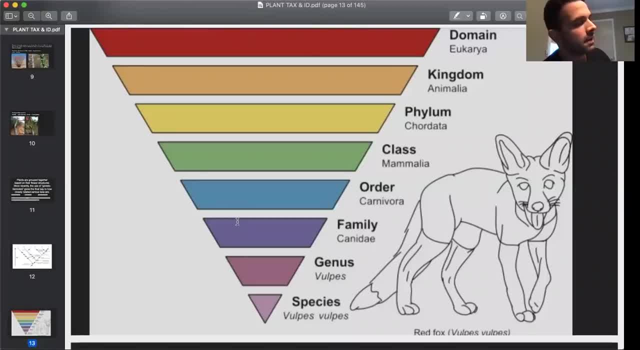 that cactus family's been in north america. i think it's primarily it originated in south america. but you know what? what different forms have evolved over deep time. you know, it's fucking fascinating and that's one thing that gets me stoked about exploring. you know, i can. i can walk up a barren. 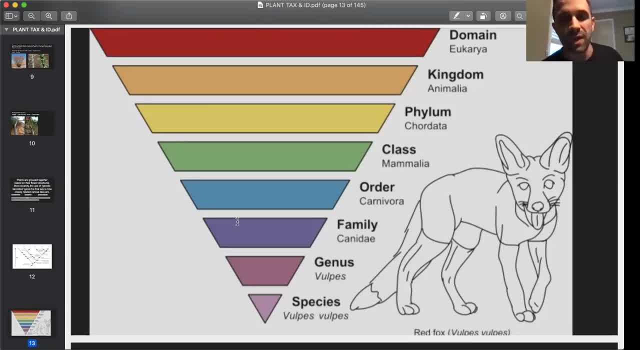 hillside in the desert that someone who's not into plants might see and be like, wow, it just looks so dead and dry and i'll walk up it and i'll see. you know, plants that have evolved. their leaves are the same color as the fucking rock they're growing in, and that blows my mind, so it 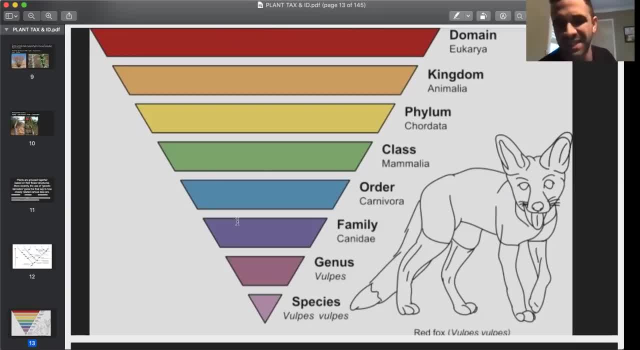 might be a genus that i'm familiar with, but i've never seen one that does that and i've never seen this that has leaves that turn fucking orange with speckled purple, because they grow on orange volcanic rock. it's fucking wild and you'll see the same thing, uh, with certain snakes will do that. 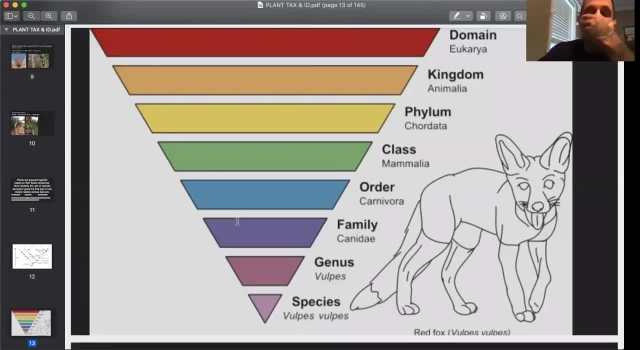 certain snakes. i mean there's speckled rattlesnakes, it's a species in, uh, the mojave and sonoran desert and, uh, what's blown my mind about those fucking snakes- i mean, aside from almost stepping on them and getting bit uh- is that each different population will come to. 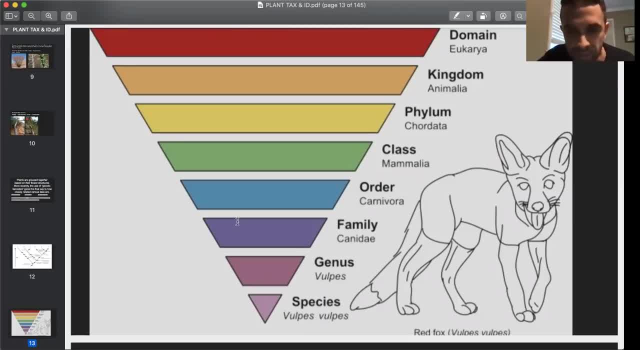 you know, if you're on like purple rhyolite, you'll see purple speckled rattlesnakes. if you're on a grayish limestone, you'll see grayish colored rattlesnakes. it's fucking wild, you know, and you think about how long did it take for that trait to evolve? you know. and they don't change color. 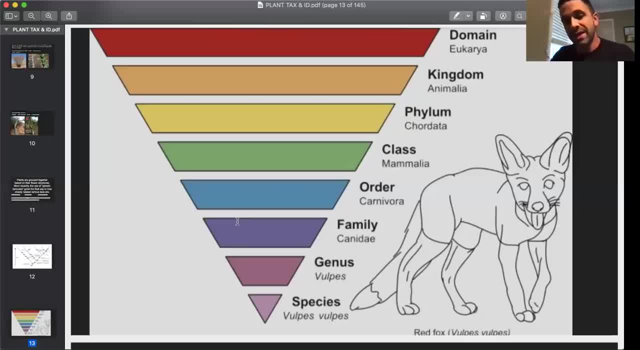 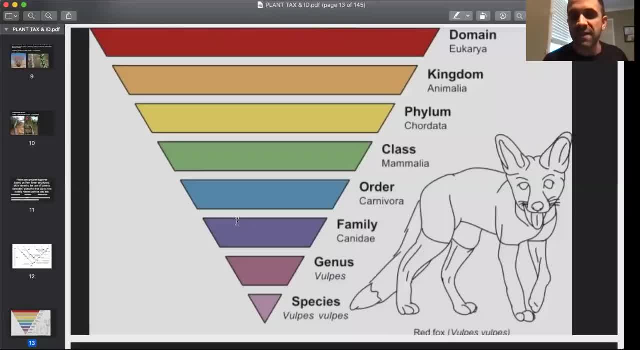 fucking cool to think about and in a way it's almost philosophically fulfilling, because you're like this shit, this depressing shit. you know everybody saw the fucking gravy seals invade the capital yesterday. the world's going to shit pandemic. you know, half the fucking country doesn't. 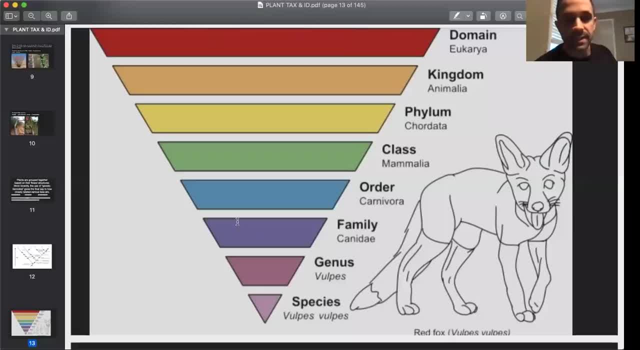 believe in science anymore. you kind of come to realize this is all this temporary bullshit. i mean, you know, i mean i don't want to let it soothe you too much. there's still a lot of need that you know to to try to affect change. but it's philosophically 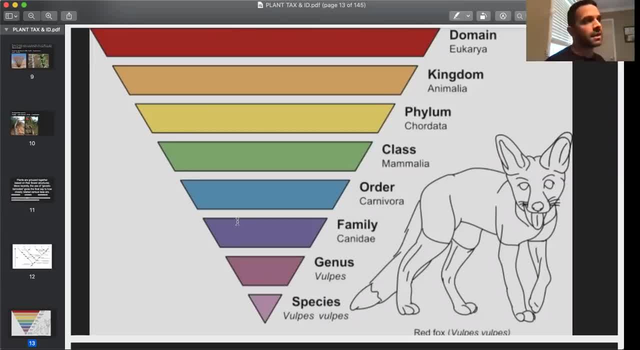 fulfilling in its own way. you're like you know what, uh, things are generally going to be okay. maybe not for me, we're all going to die one day, but just, you know, just broadens your perspective on the world around you and takes you out of this depressing synthetic world we've created. 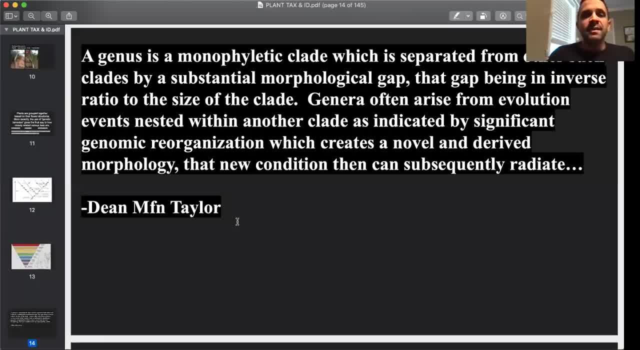 so, anyway, enough of that moving right along. uh, this was uh a quote by my friend dean, who just died, uh in november, and it was basically his way because we were getting into this conversation. like you know, we're going to die one day. we're going to die one day. we're going to die one day. 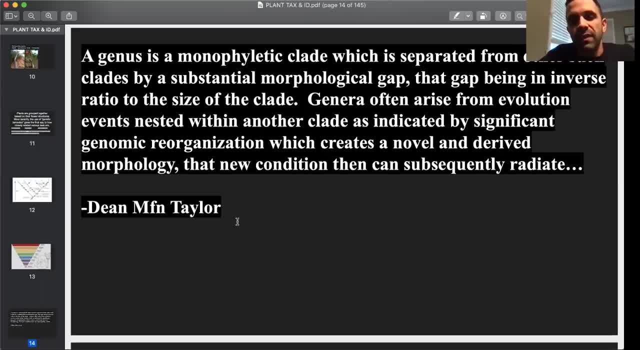 you know what is a fucking genius? what's the family? these are just things that humans come up with. right? we're humans trying to draw boxes and classify things. draw boxes around and classify things that nature doesn't classify, nature doesn't. nature doesn't play by our rule, our rules of 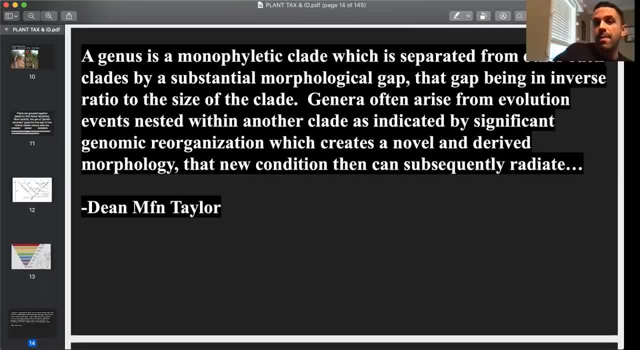 taxonomy, so in his way that he came up, came up about it, and you could apply this to family or whatever. but a genus is a monophyletic clade which is separated from other such such clades, other such groups, uh, by a substantial morphogenesis. 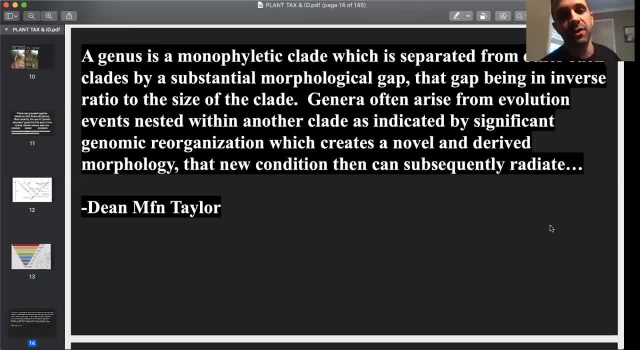 so that's just saying it's got to be different enough from other genera, um, to be considered a new genus, right? so in in some cases things aren't different enough and so they end up getting lumped together in the same genus, whatever, and you end up pissing off a bunch of old botanists and 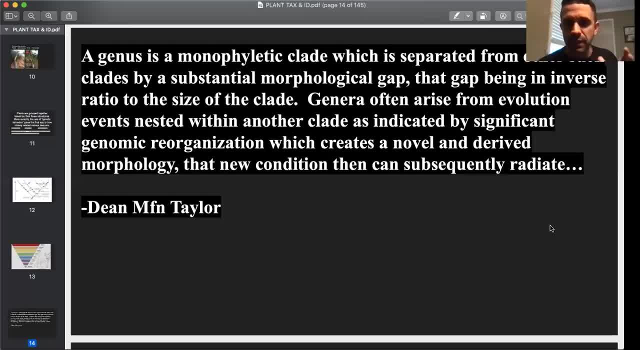 horticulturalists. but it's just a way you got to keep it loose, right? you got to keep it loose when you're thinking about this stuff, uh, kind of like how you got to keep it loose when you're thinking about geology, like there's just you know, you got to understand at the root of it that there's a 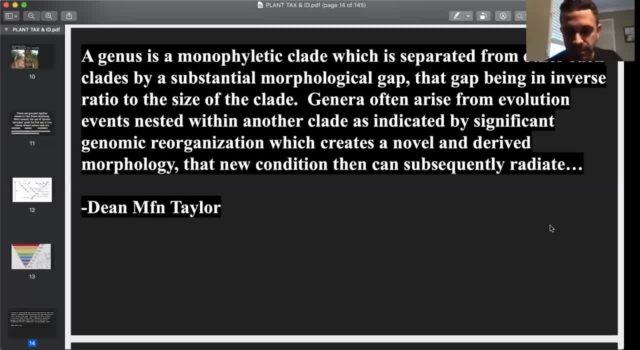 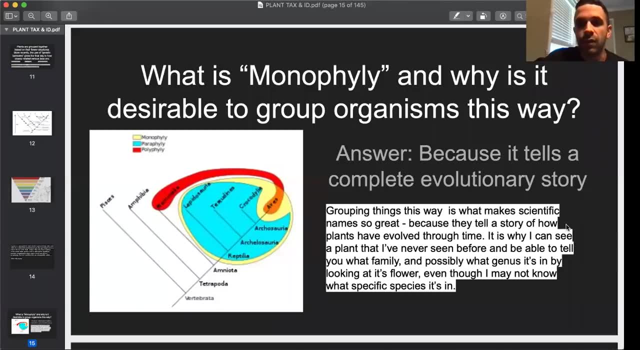 these are attempts of humans, of of us fucking primates, to put boxes around things that may not be as crystal clear as we want them to be. uh, anyway, what the fuck? why is this not working? next slide, here we go. what is monophily and why is it desirable to group organisms this way? 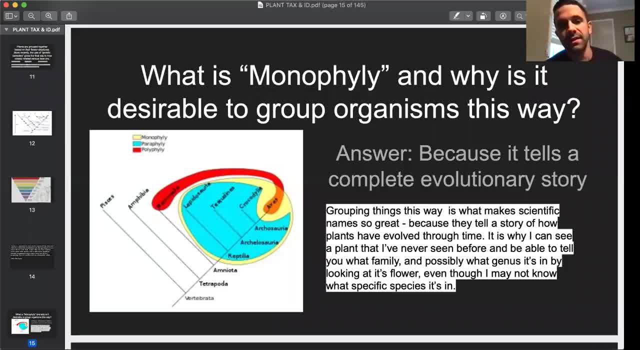 okay. monophily is uh just means if you have a monophyletic clade, it means everything in that clade uh shares a common ancestor. so you have monophily, paraphily and polyphily. monophily is what you want, paraphily and polyphily are ways to. 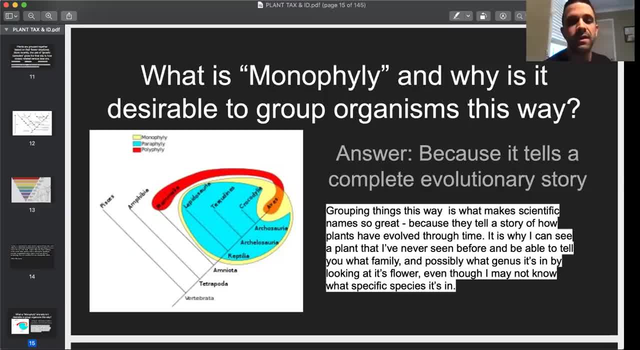 fuck things up. you know when you're before. you have, uh, had it elucidated, these relationships elucidated. so like, um, let's see paraphily. i'll get into this later too. i'll give examples of each. but monophily is really what you want. it means everything in that group and that genus in that. 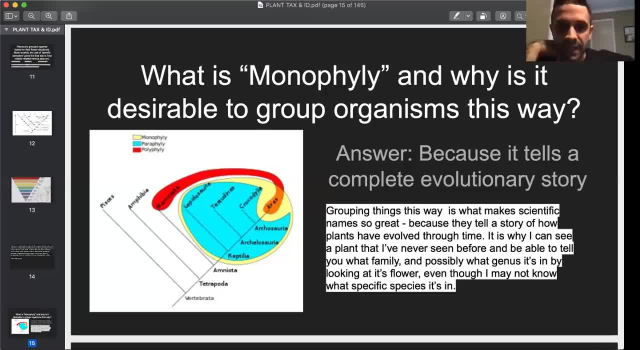 family shares a common ancestor. you're not leaving anybody out. it's a direct descendant of, uh, the last common ancestor that they all shared. it's the same thing with people, bacteria, fish. if you go far back enough, we're all related. you've got that luca. 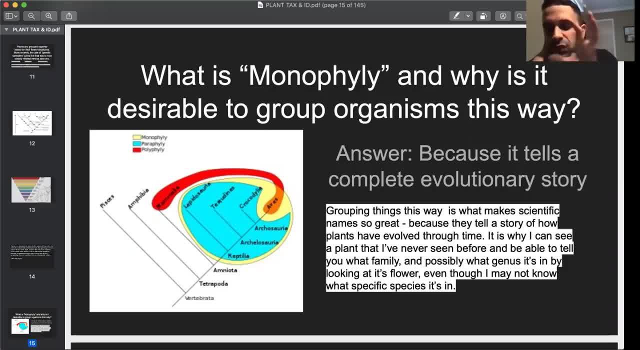 that last universal common ancestor. okay, but anyway, sticking to a smaller scale, more recent things are grouped together in monophyletic clades. so that's that's what you want. you want everything to be grouped together taxonomically, on how, on the ways in which evolution worked. 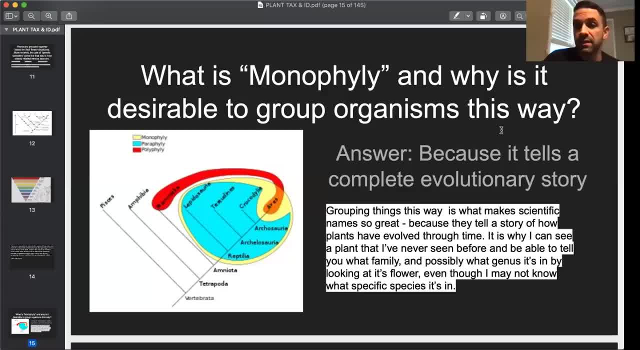 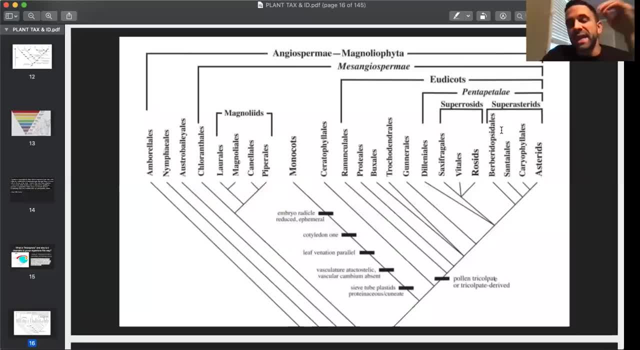 itself. out, there we go. so here's an example of the flowering plant monophyletic clade. right, it used to be, everything was just grouped in monocots and dicots, and then, once we look closer, we realize: you, you've got these magnoliids and some of these more basal angiosperms that are in. 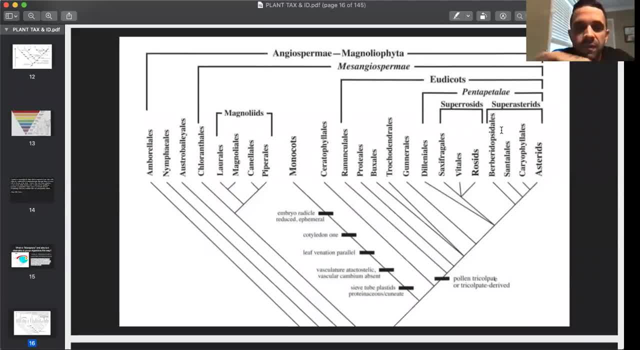 they're more closely related to monocots than they are to other flowering plants. so you know a good here's and here's the apomorphies, right? so, uh, paraphily is a group of monocots that are parallel leaf venation. if you look on that, that one black rectangle beneath monocots, you know that's. 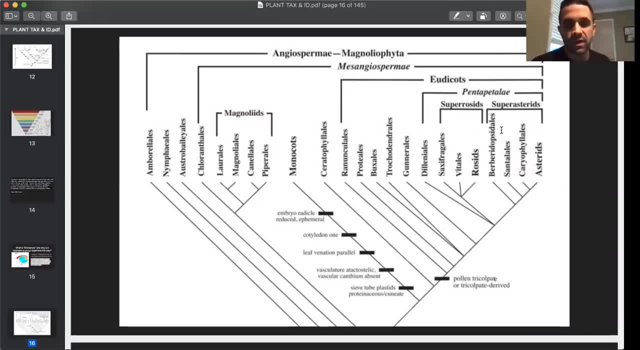 a good way to tell if something's not flowering, if you know if it's a monocotal leading or not. monocots are grasses, palms, asparagus, agave, orchids, lilies. you look at the leaves of all those and the veins. you know you got the the light green leaf with the darker veins in most cases. 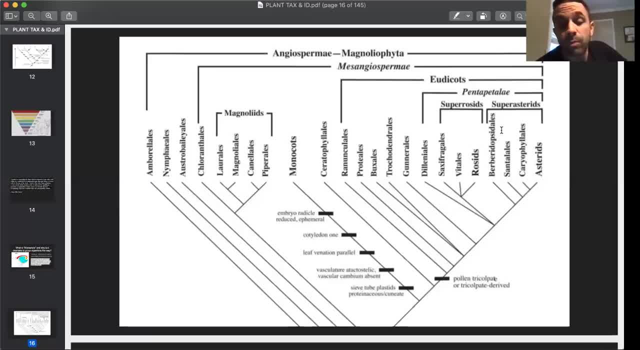 the leaves are parallel, it's a monocot. so boom, you got one one, you're going to have a monocot. you're one step, you're one clue, uh closer in your detective novel of figuring out what the that plant is. okay, parallel, uh, leaf venation. okay, vasculature attack. i don't even know what. 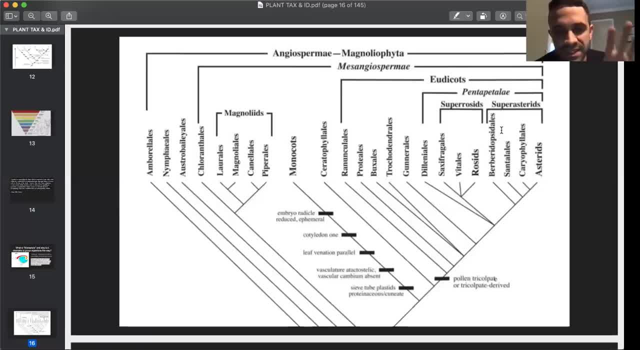 a tactile stelic means. but these are all things. obviously you can't see, unless you, you know, get in there and dissect it in a microscope, sieve, tube, plastic, same thing, um, you know, microscope for all that. but leaf, parallel leaf, venation, parallel, cotyledon one, it sends up one leaf. 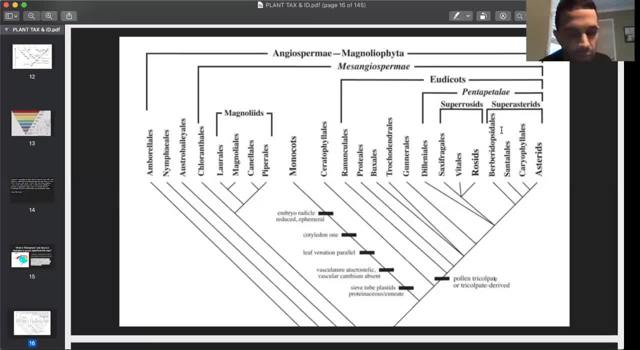 so if you grow- if i grow grown agave from seed, it's cool- you get one little leaf coming up. it just looks like a tiny little mini grass and then, uh you know, eventually it starts to get this rosette. one another leaf forms to the right, another leaf forms to the right. they whirl around. 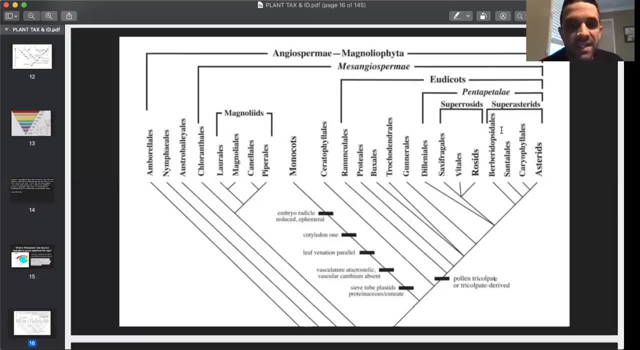 uh, etc. so you got monocots. then, to the left of that, you got, uh, ambarella, which i'll show you. i think i put a slide of that in here. you got ambarella, which is, you know, a. really it's like a dinosaur, it's like a living dinosaur. a lot of people don't like it, but it's a living dinosaur. 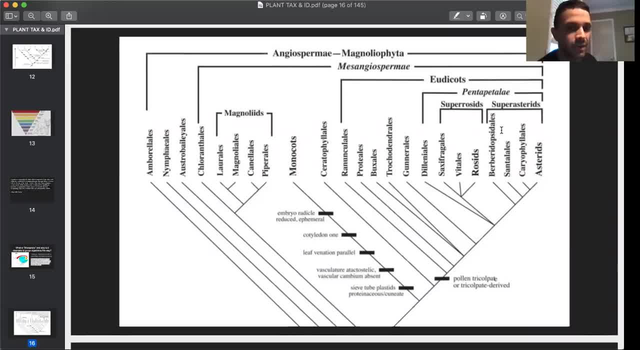 i don't like that term, but for all intents and purposes it works. for people who are just getting into it: uh, it's a living dinosaur of plants, a living fossil, so it's a really old lineage. i mean the way that that ambarella transports water. the structures that it uses are so fucking different. 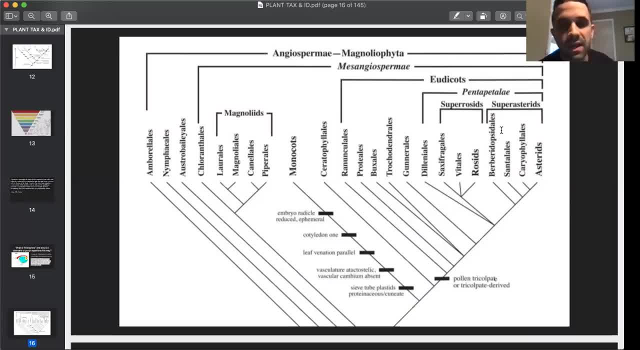 they're more closely related to conifers than they are to the rest of flowering plants, so this is a really old lineage. uh, i actually actually got one growing from seed back in california right now, collected seed of it, but it's- uh, you know it's one of those. ambarella is one of those plants you're gonna see every conservatory. 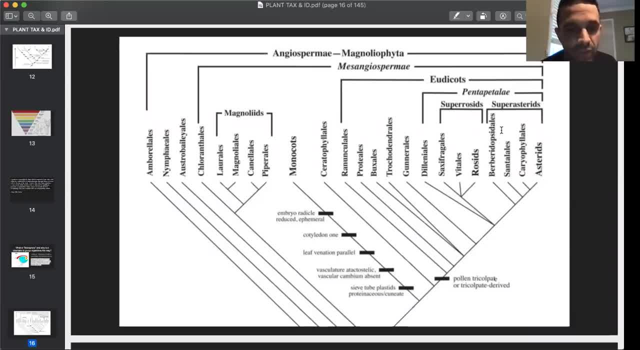 should have one. every fucking uh college greenhouse should have one. it's a massively important plant, uh, in terms of the evolution of life on earth, not just flowering plants, but, you know, all life on earth, considering that that you know, plants are the base of the food chain, uh, nymphiales that's. 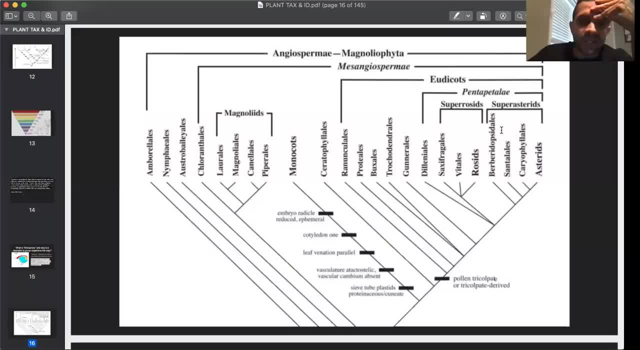 water lilies, austrobaliales, that's uh, elysium, you know, another kind of rare, like star anise. pretty sure, yeah, star anise is in austrobaliales, you know, used as a spice. it's actually a really weird, long, lonely branch- is a way to think of it. a flowering plant, evolution, cool fucking plant. 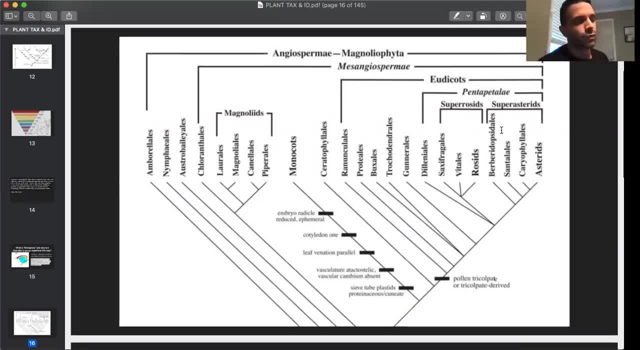 the really weird flowers and when you get up and you look at these flowers you realize there's there's some differences there. you know, avocado is in low rallies, it's a magnolia- again, another kind of basal lineages. lineage magnolia- same thing. piper, alias pepperomia- uh, same thing. 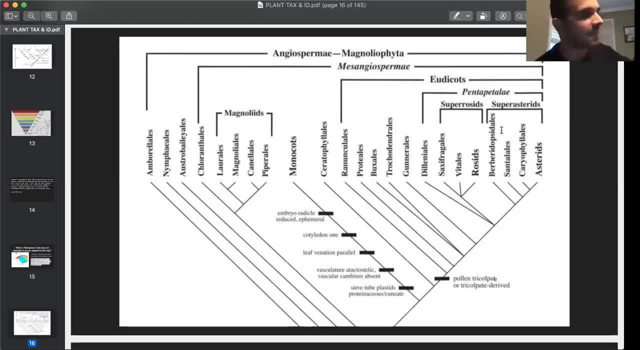 older lineage. i mean, it's so the the species itself is not left over from the fucking, you know, early cretaceous, but the lineages, so the descendants, uh, you know, are descended from this really old, uh, lineage, this that evolved a long time ago or first emerged a long time ago. 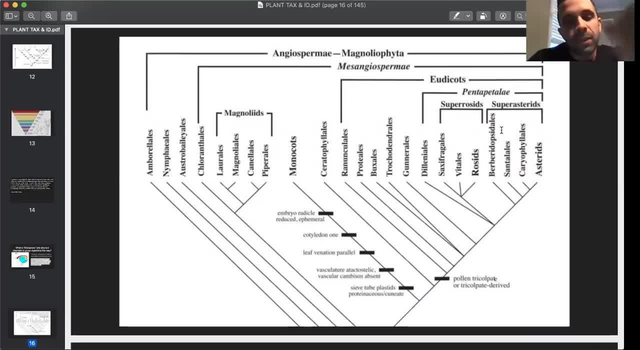 you know, if you look at like uh, look at like a, look at a magnolia flower up close, it'll blow your mind. it's fucking unreal. i mean, everything's arranged in this kind of cone-like structure. the? uh don't have a filament, they barely have a filament. they're kind of like they're not stocked. 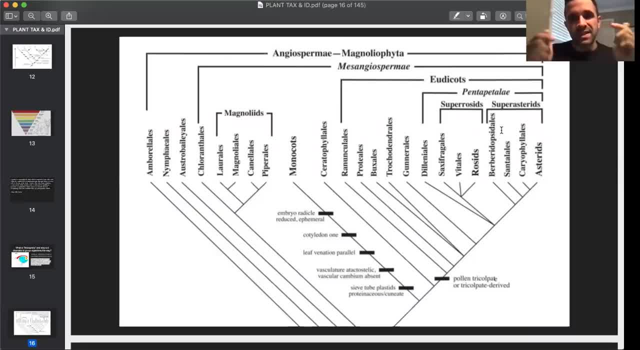 think of like a lily stamen. right, those antennas you got, we'll get into this later. you look at like a lily, those stamens are long. you know, if you got cats you want to keep the lilies out the house because those stamens hold the anthers and the anthers drop the pollen and it's poisonous, uh to. some animals. you know those things that you and they'll clip them off in lilies sometimes because of that they can be poisonous to animals. um, they'll clip those off those think of. compare that to a magnolia statement. i mean, get up close next time you get a magnolia flower. they should be. 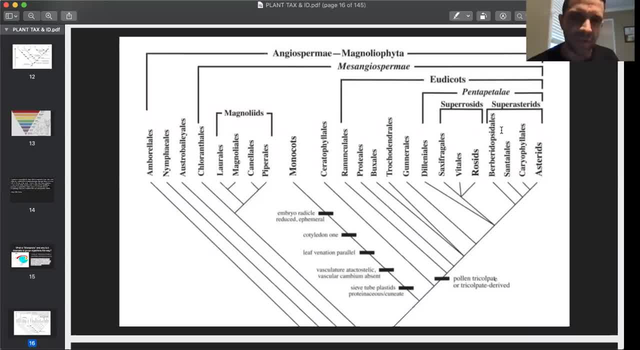 blooming. if you're in the south next couple months and look at it and you'll see how fucking weird it is. it's like this doesn't look. it almost looks like a conifer. it's a really old quote, old structure. and then on the right you got the more recently evolved things, the asteroids. 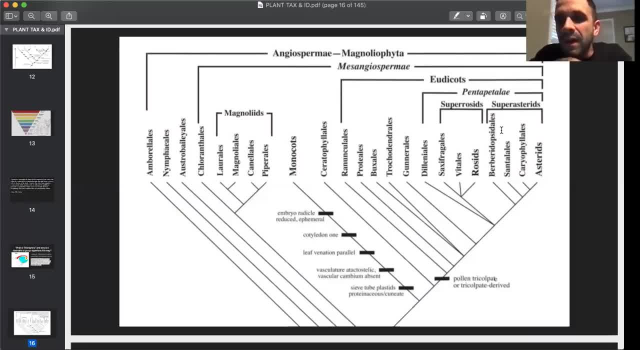 karyophyllales, which we just talked about, santa lalys, uh, which is entirely parasitic, really cool fucking family. all over the world mistletoes are in santa lalys, etc. so you mentioned earlier the importance of ideeing or capturing photos of plants in habitat, the 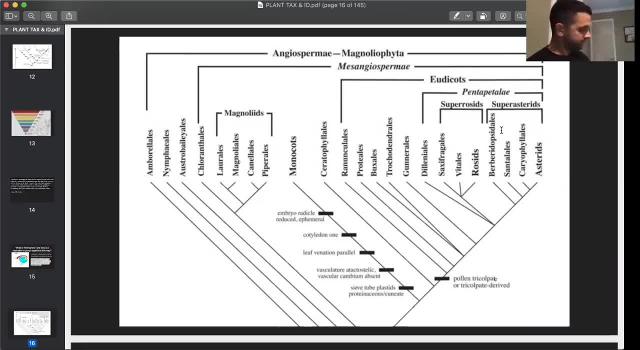 problem that i have is that some of the plants that i'm most interested in ideeing are in habitats that are, like, heavily disrupted. so, for example, i live in oregon, west of the cascades. we have a huge himalayan blackberry problem. it's fucking everywhere. oh, it's a terrible fucking. 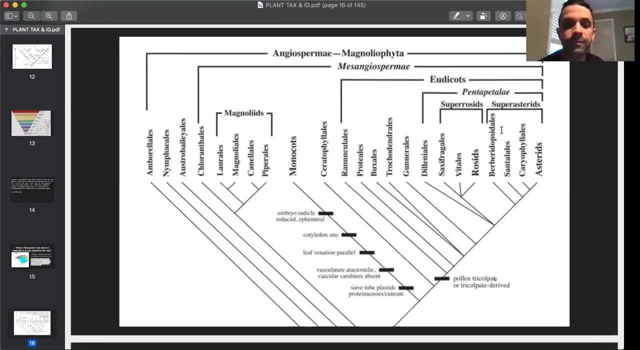 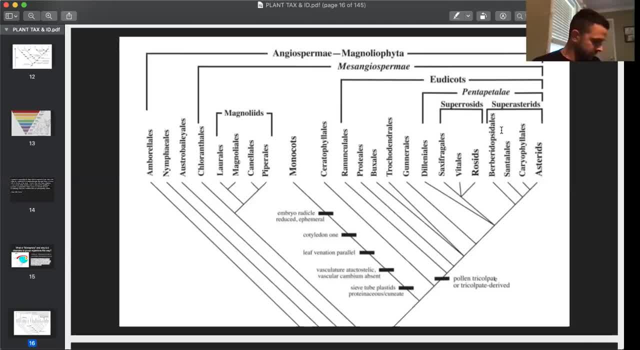 and it'll be completely grown over with invasives like blackberry and scotch broom and i'll see like one presumably native plant sticking up out of the monoculture and i'll be like, oh fascinating, what plants resilient enough to survive in the sea of invasive species. but i can't get to it. 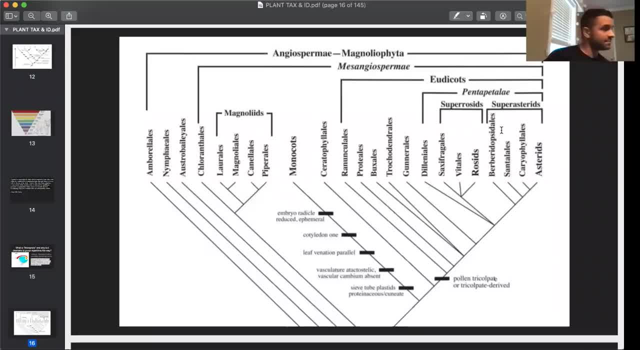 because i'm not going to get torn up trying to wade through blackberry bushes. all i can do is like take out my camera and zoom in as much as possible to try to get something clear like: what do you do then? how do you positively id a plant in that situation? 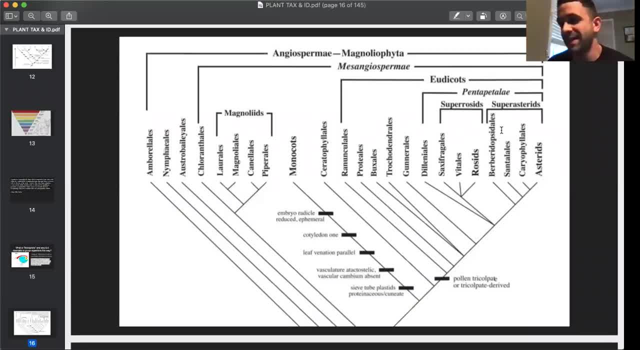 or are you just screwed? i don't know. you get some good boots, maybe i don't know machete, some cases you can't. you know. i mean blackberry is really fucked. a lot of the hippies and permaculture, let's no offense. don't like roundup or or, or you know, herbicides. this is going on kind. 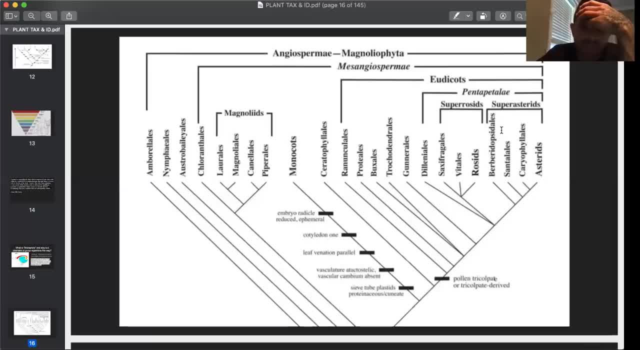 of a digression here, but, man, there's no fucking way to get rid of some of these plants without using it. the idea is to not use mass amounts of it to spot apply it. don't use a fucking sledgehammer, use a scalpel. but you know, in case the himalayan blackberry, you cut that thing, it's going to sprout. 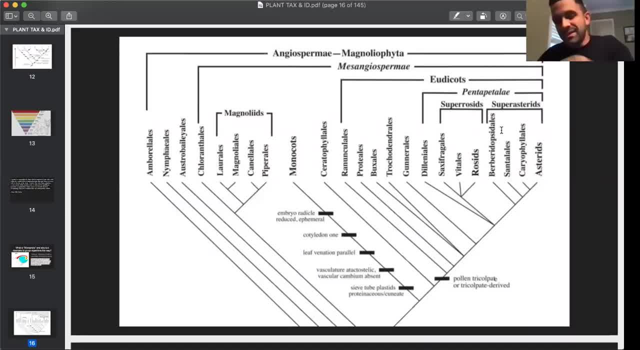 back up. so do you want to go and and wear gloves and dig the fucking root out, you know, and cut the shit out of yourself? or do you want to cut it and then, you know, spot apply, like with a paintbrush, some herbicide, i mean you know, yet habitats are disrupted. i mean i've, i've almost killed myself. 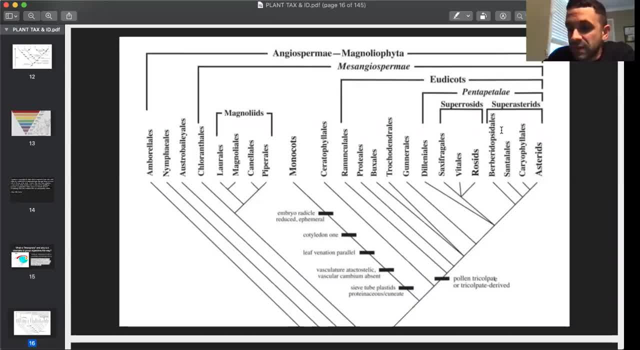 you know, dangling off cliffs to get pictures of flowers before just to to look at them. in some cases you can't, you're fucked. look for another, try to look for another one, you know. try to, uh, i don't know. i mean, there's, there's just ways. there's only so much you can do, don't. 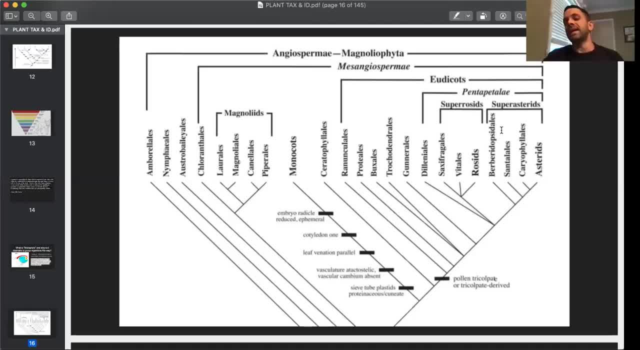 fuck yourself up. but uh, you know, in some cases there's just nothing you can do. so, but if you do get photos, get photos of the top, get photos of the sides, get photos of the underside, so you know if the petals are really big, if they're bigger than the sepals. you know you take one blurry. 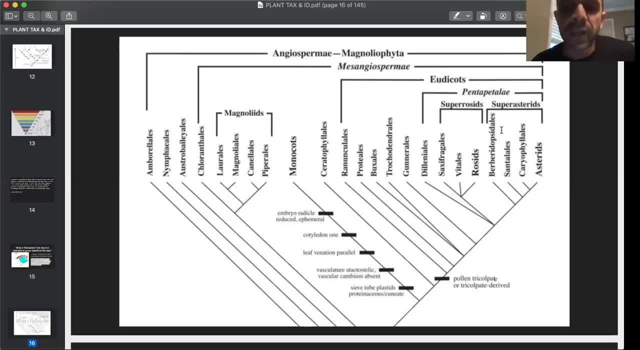 picture head on. you won't see those sepals sunflower family. get pictures of the sides of it, because a lot of members of the sunflower family just have yellow rays, right, they all look the same. so you can't just look at the. the fileries- and we'll get into that later. the fileries, those 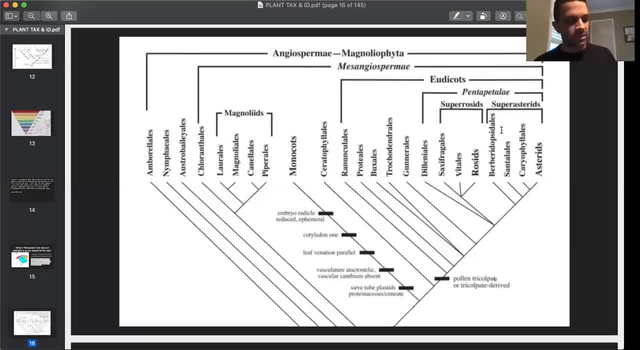 bracts on the side, which can be in one series or in multiple series. those are the things to look at. those can be diagnostic: the shape of them, whether they were curve or not, how many series you have, etc. so, um, anyway, any more questions? uh, yeah, um, so, when you were talking about related, but not. 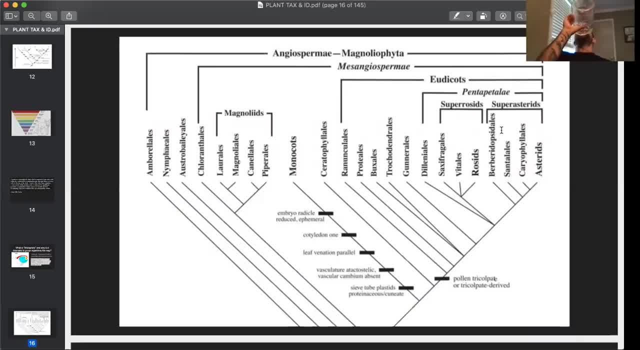 similar versus similar but not related types of plants. it made me think about ring species and uh in the arctic, where nearby populations are able to interbreed, but once you get like a certain, like enough of a distance, they lose that ability. i was wondering if that's something that we also 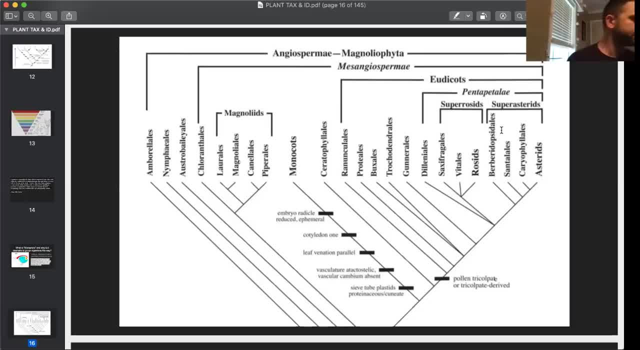 observed in plants. uh, somebody else had said that that, uh, they had. they see it in like cereals. i was wondering if that's a common thing or like more rare in the plant world. if they see it in cereal, what do you mean? i'm not like cereal grain. oh, i don't. i don't know about that. i mean, i don't know. 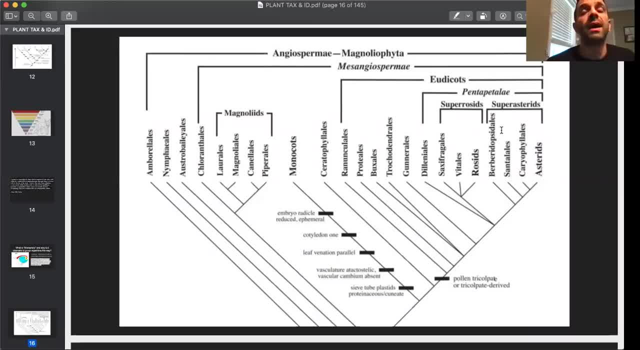 i do know that there are. there's cases of like you know. you take coranthodendron and flannel bush. right, those things grow a thousand to three thousand miles apart and they're in different genera, different genera not supposed to be able to interbreed coranthodendron and flannel bush can't. 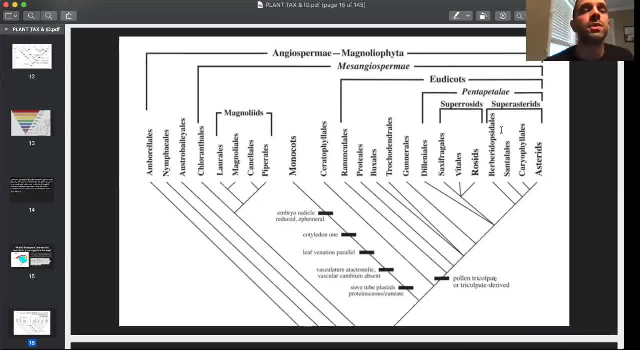 i mean, it's really just nothing. is that's what i'm trying to say? keep it loose when you think about this stuff, because nothing, nothing is solid. you know things are everything's subject to change, everything. you know there's no definite rules. rules can be broken, rules apply. 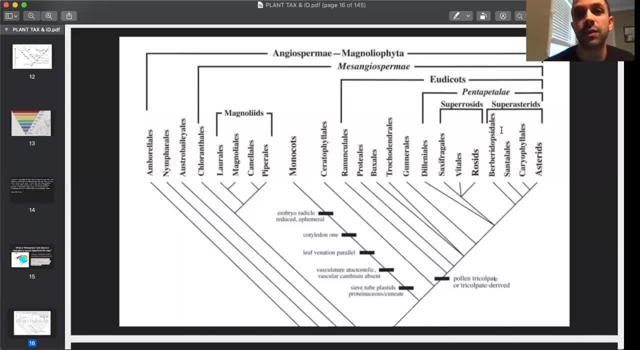 ninety five percent of the time, you know, but then there's a case where it doesn't. so you know the idea of, and again the idea that, uh, what's the way to think about this? that you know when gene flow breaks down, basically, um, your barriers to gene flow sometimes, sometimes they're, you know they're. mountains, sometimes they're deserts, sometimes there's things just flower at different times, but nothing, nothing's solid. sometimes things can still interbreed, even though they've their lineages have been separated- for you, you know, fucking millions of years. so, uh, i'm not familiar in the case with birds, but, um, you know. 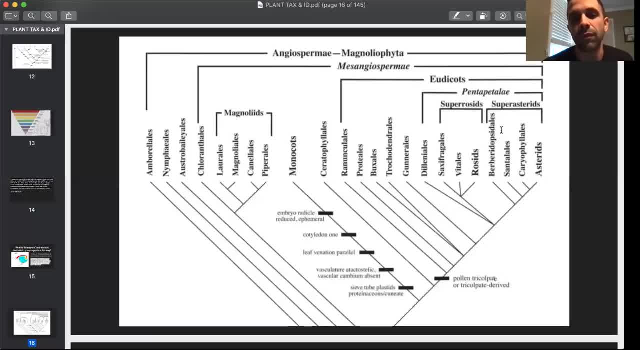 the thing, that the thing to take away is just like anything can really happen. i mean that fucking corny quote from jurassic park: life finds a way. i mean that really is the fucker. was that. whoever wrote that line, for whatever that actor's name is, that's. they were kind of right so 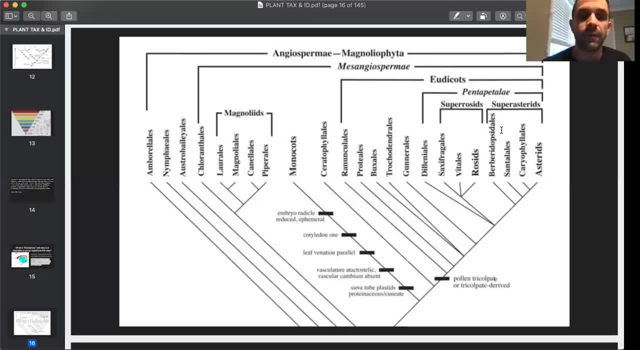 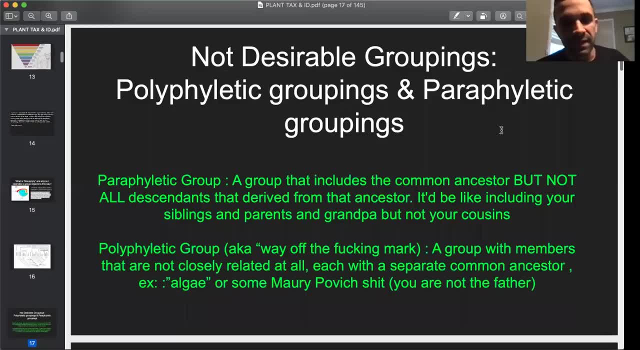 awesome, thank you, yeah, hopefully that quite that answered. i don't know, it was kind of kind of a rant, but uh, anyway, all right, so let's move on. uh, so not desirable grouping groupings, polyphilic groupings and paraphyletic groupings. now, this can be really hard. good way to remember it is paraphyletic, the. 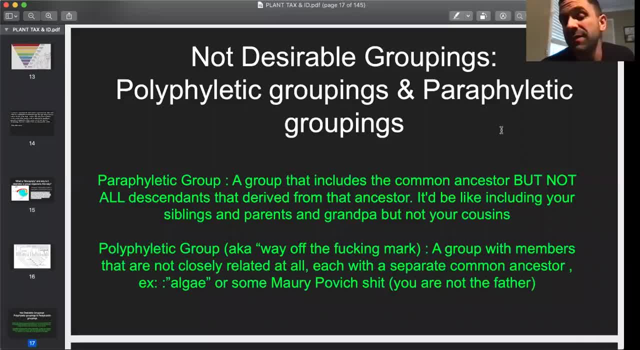 word has an a in it. uh, a can also. a is the first letter in the word ancestor, so paraphyletic: a group that includes the common ancestor but not all descendants that derive from that ancestor. the most perfect example of this that you see in evolution textbooks: 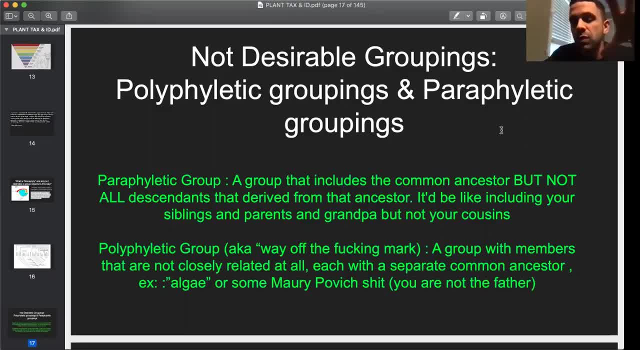 is birds, it's like reptiles. if you say, if you, if you reptilia the order, i've not even fucking, i should not a herper. but whatever the clade is for reptiles, if you don't include birds in it because they're technically a reptile, that's a paraphyletic clade. you got all the ancestors and most of the 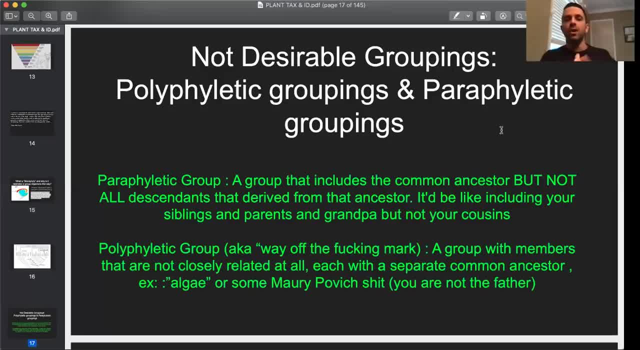 descendants save for one or two. so paraphyletic means you're kind of close when you're grouping these, but you're not on the mark, right? uh, so paraphyletic, it's got an a that word. ancestors, the common thing to group. they're the common ancestor but not all descendants ancestor. a paraphyletic also has an a, that's. 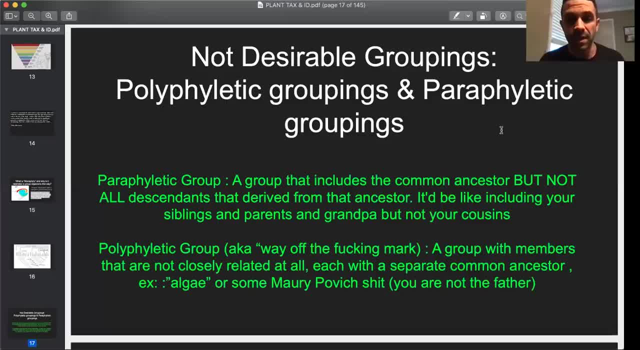 how i remember polyphyletic group, aka way off the fucking mark. you're putting yucca in the lily family, you know, or you're putting. you're putting paintbrush, indian indian paintbrush, in the- uh, the fucking what was it? what it used to be in scrofulary a say or something? way off the mark. 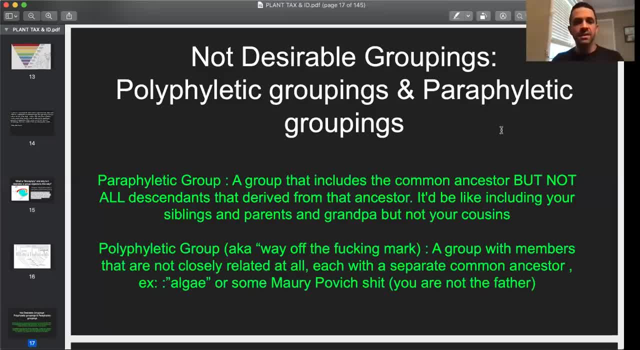 right. i mean they're in the same order, but you're way off the mark. so polyphyletic is groups that are not related at all, you know, and that's what? uh, that's what. that's where dna comes in. that's where i, that's when i like dna, because it really elucidates these relationships like for so long. 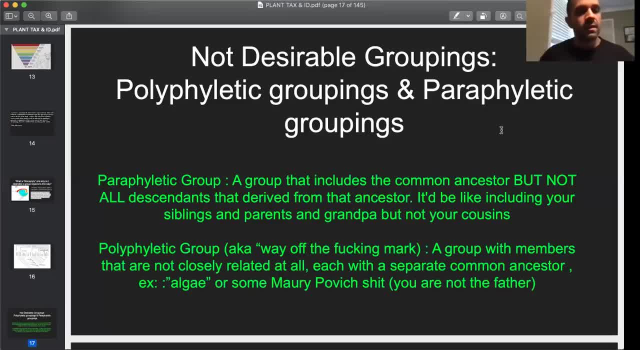 we thought, because these things looked similar, uh, or similar enough, that they were in the same family or genus. and then you know, boom, it turns out when you look at the dna test: uh, no, they're not, they're not related at all. you know, it's like the mori povich. you know, you are not the father. 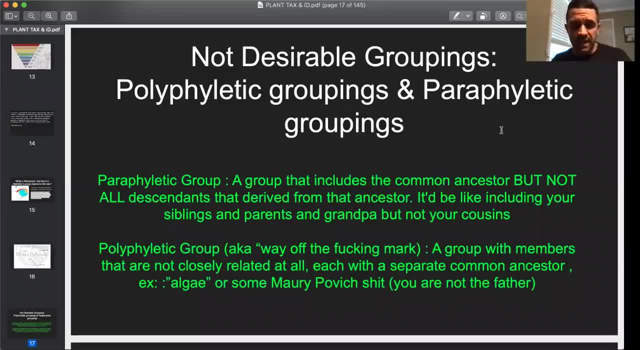 on stage. real nice good example. that's polypháfic, right um. so those are the things you got: monophilic, paraphyletic, polyphaletic, monophilics, desirable paraphyletics like: oh, you just need a slight adjustment- and polyph detergent. you really work on structure. você é tudo tipo there. 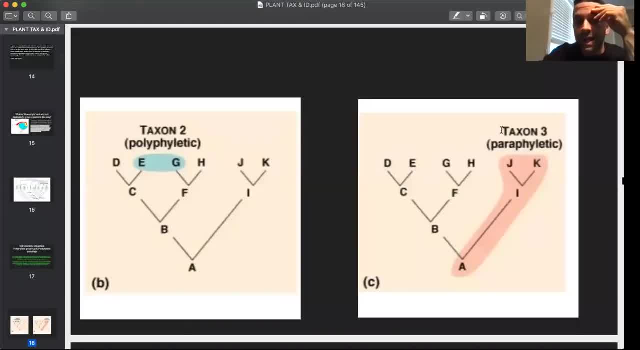 fuck this up. you have no idea what you're talking about. and here's the clay to gram example of each polyphometric. you could see e and g are presumed to be more closely related than they actually are. it turns out e is actually more closely related to d, then it is to g. 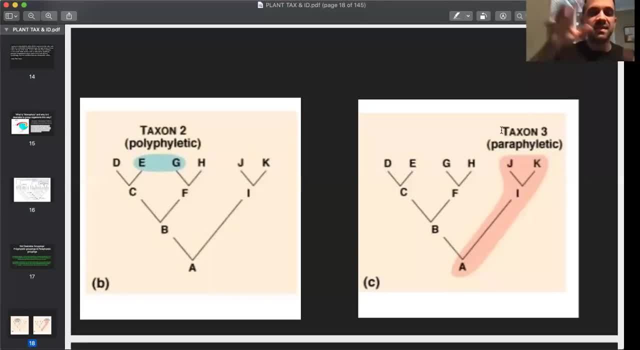 And of course, the idea would be that you know E and D are placed in different, are mistakenly placed in different genera or family, whereas E and G are placed in the same family And it turns out: boom, that's way, way wrong. Paraphilitic, here you go. Good example: This is the reptiles. 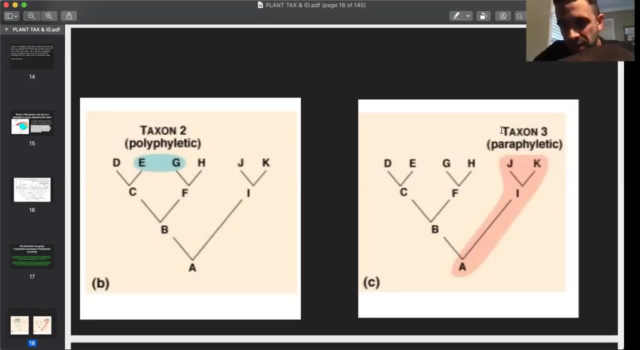 and birds thing. okay, Say, the B is all the birds and you know you're calling A and I, J and K, all reptiles, but you're not including birds. So that's paraphaletic. You've got the ancestor. 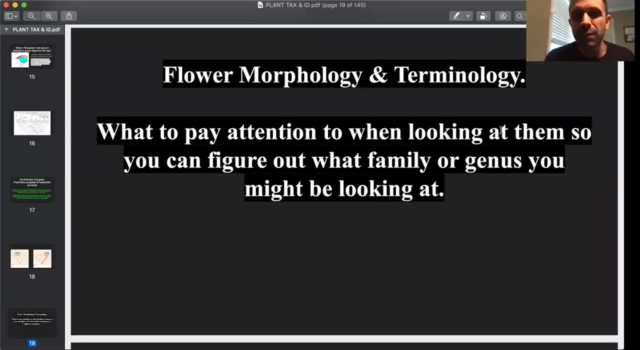 but you don't have all the descendants. So here we go. Here's the juice Flower morphology and terminology. So what to pay attention to when looking at them, so you can figure out what family or genes you might be looking at. Now, the best way to do this is not from listening to my ass. 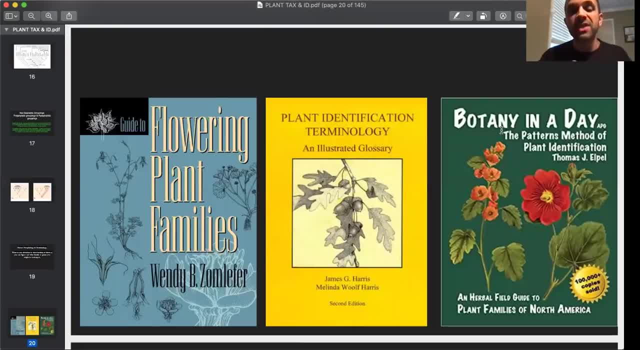 talk about it or reading a fucking book and just studying on paper. The best way to do this is to go out there and challenge yourself by looking at weird shit: Plants in a vacant lot, Plants in a conservatory. Go sneak into the botanic garden, Pay if you can, but don't worry about it, okay. 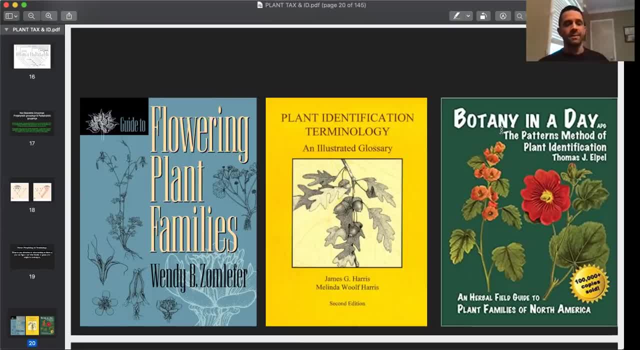 It's like all that. That shit should be free, in my opinion, anyway. all right, Conservatories and fucking greenhouses, and it should all be free. That's like the library. These are the books I recommend to people. Botany in a day- not so much anymore, because it's a good introductory guide if you're. 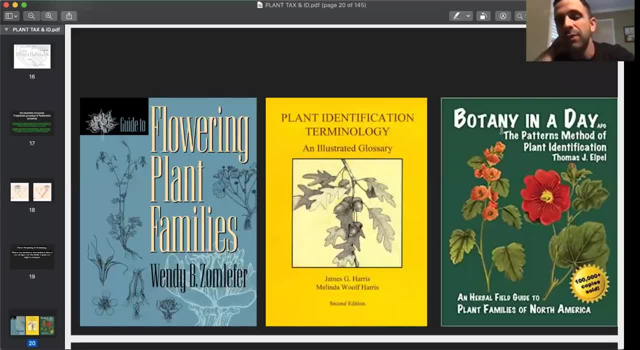 getting started but it was designed for herbalists. Some of the taxonomies off, but it really runs home the idea of looking at flowers and you know each page corresponds to a certain family or in some cases really big ass family. So if you're looking at a book, you're looking at a book. that's. 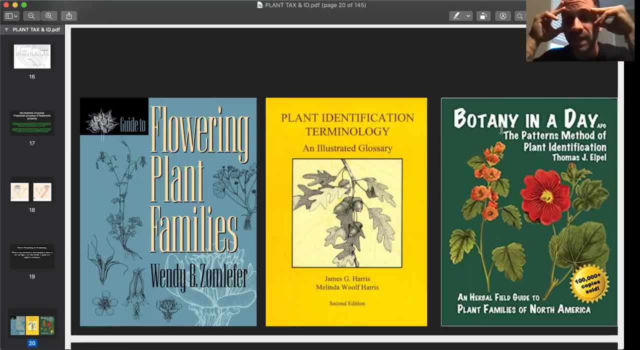 like the sunflower family, it corresponds to a subfamily, So it'll help you get the idea. you know, I think I heard the guy who wrote it. it's kind of a prick. you know he's whatever, but you. 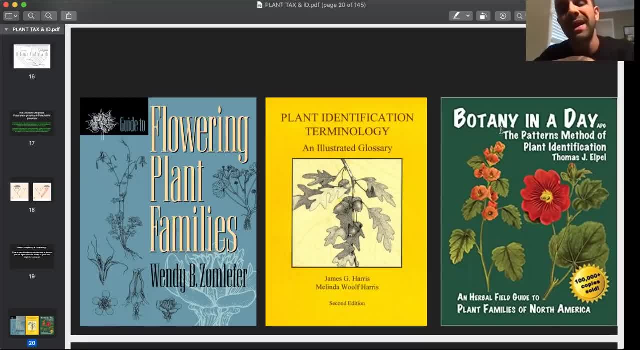 can steal it on LibGen. You don't want to pay for it. I would recommend the hard copy of any of these books though, because, again, you want to give the authors some credit. you know, The publishing- whatever The publishing- will get some of the money, but if you have the money, get it. It's. 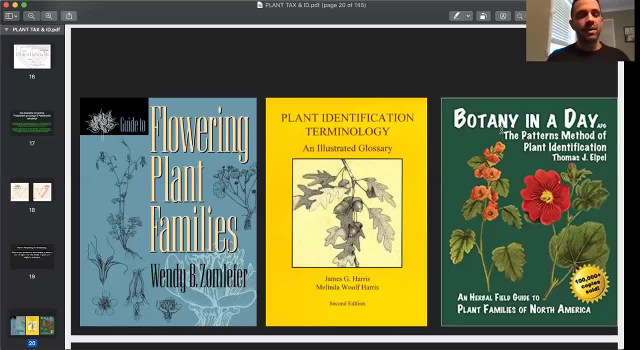 always better to look at a hard copy too. you know, I use this fucking tablet, this Android tablet, you know, because you can download a lot of stuff on LibGen. You can carry 70,000 pages in what amounts to a, you know, a pound and a half device. But you know, generally I like. 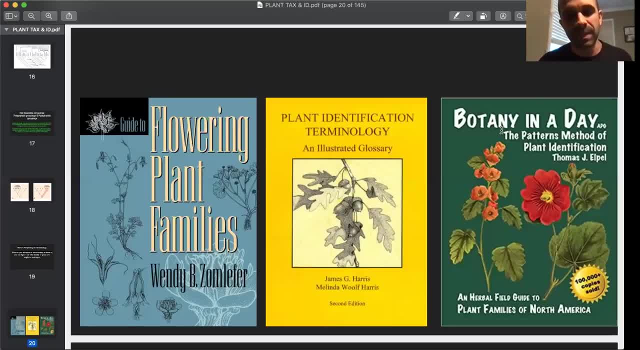 looking at hard copies, Flowering Plant Families gets a little bit more in-depth. That's on LibGen too, but the fucking hard copy is awesome If you can get it on used or I don't. even it might be out of print. This lady, I think she's in Georgia or something, but it's a great family and it goes. 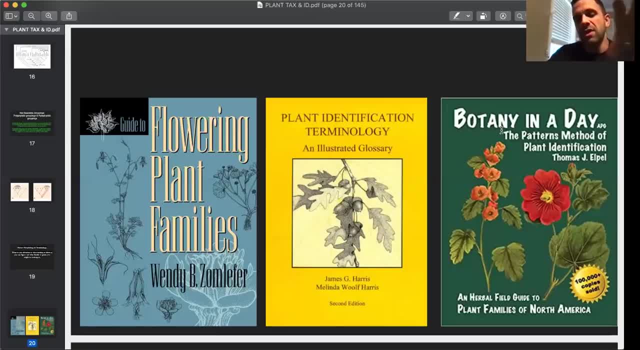 into a lot of, not just you know it's a great family, but it goes into a lot of you know, just morphological traits. But she even talks a little bit about habitats that they tend to occupy, because certain plant families will tend to occupy certain habitats And then plant 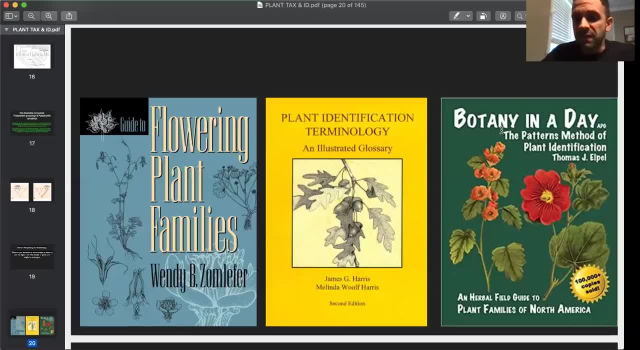 identification terminology. if you know, you're fucking yourself up trying to figure out what certain words mean And it's a whole different vocabulary when you're looking at this stuff. But you know, the way to learn it again is not just by. oh, I'm going to open up this glossary. 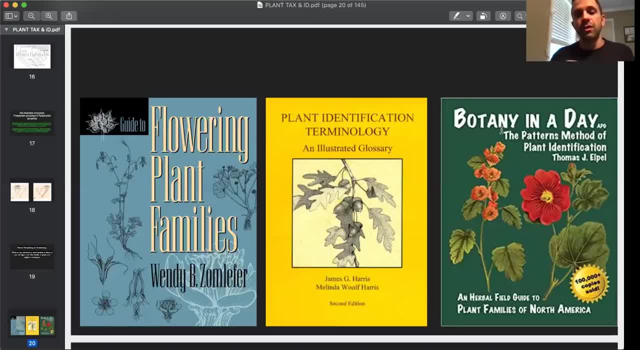 and just start memorizing the words. The way to learn it is to go out there and read these descriptions of plants and then be like, oh, I wonder what this word means. And then look it up, You know, say you see a member of the sunflower family trying to figure. 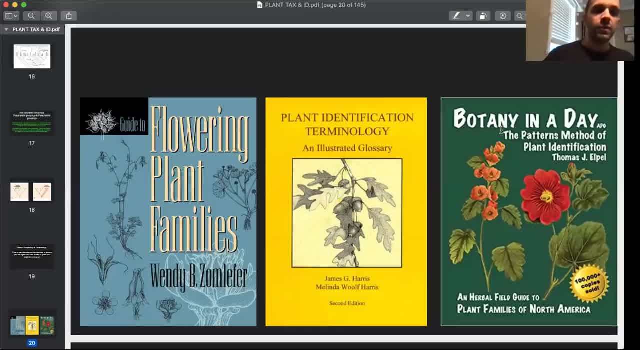 out what it is. Go to like a flora or a key and you see the written description of it and you encounter a word that you've never seen before. you know like Pele, and it's describing how the Pele look, And you're like: what the fuck is a Pele? You go to plant identification terminology. 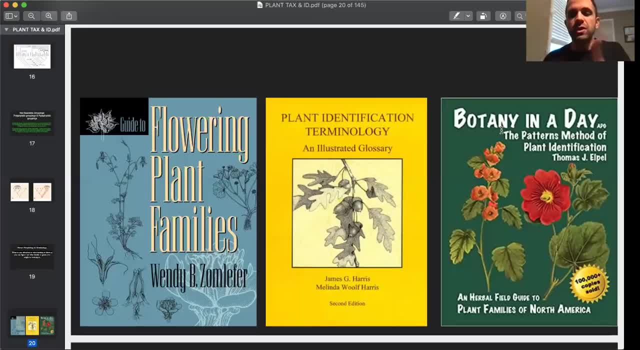 or look it up online, whatever Boom. you just learned it. Not only did you just see it written down, but you saw an example, if you're looking at a flower in your hand, of what it is. So with this too- and I got another slide for this- The fucking Lord of all books is the book. 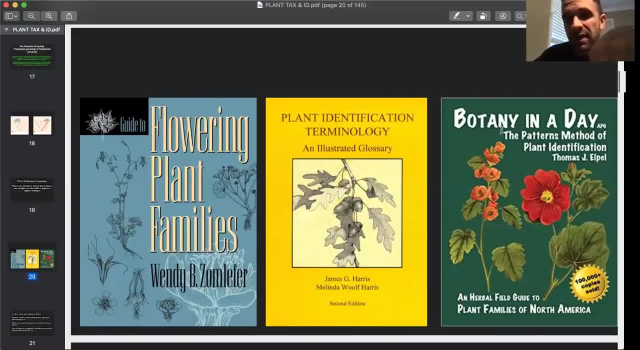 Plant Systematics by Michael Simpson. So these are all good, but Plant Systematics by Michael Simpson is really. it's like a textbook. You can get it used. He just came out with a new edition. If you got the money, it's definitely fucking worth it. You'll be using it for the next five. 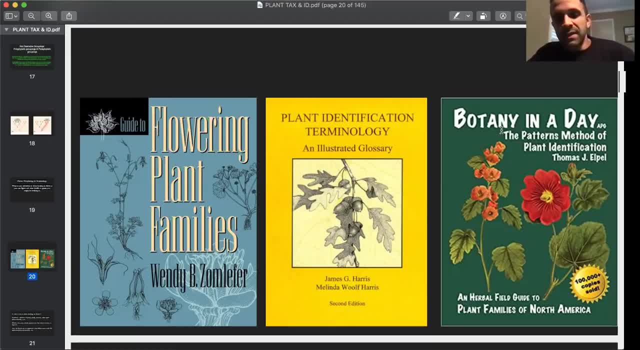 or 10 years if you stick with this shit. But it's also on LibGen- if you're broke and just can't afford it right now. So, and he's a fucking legend. So I'm going to go ahead and read this. 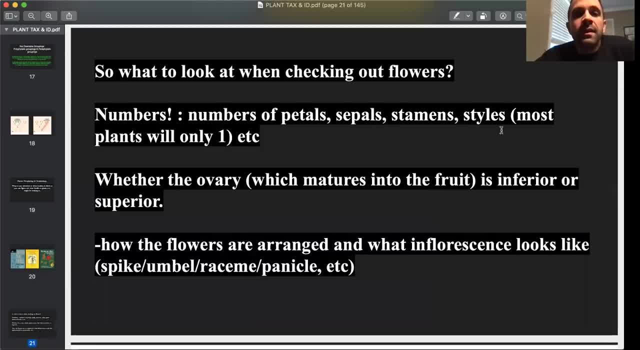 Cool guy. He's based out of San Diego, He just retired, Okay. So what to look at when you're checking out flowers? Numbers first, Easiest right: How many sepals, How many stamens, How? 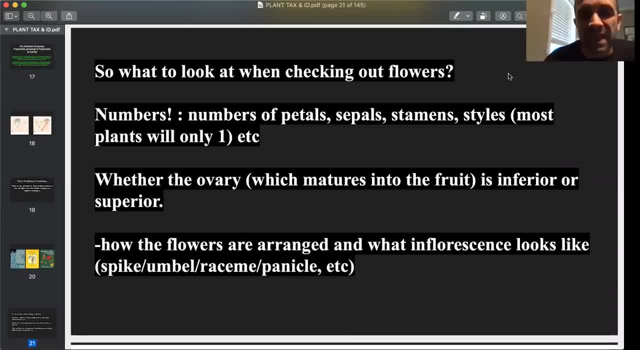 many petals? How many styles? In terms of styles, most plants only have one. Some members of caryophyllaceae have three, which is pretty unusual for plants, but it's a good way. You see three styles like: oh, this might be a caryophyllaceae, Whether the ovary which 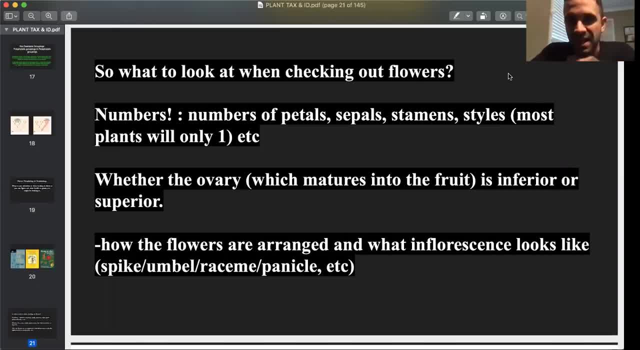 matures into the fruit ovary is just a fancy word for fruit. swollenovariescom is inferior or superior. These words inferior, superior- I'll show you coming up in a couple slides. but it just refers to where the ovary is in relation to the point of attachment of the 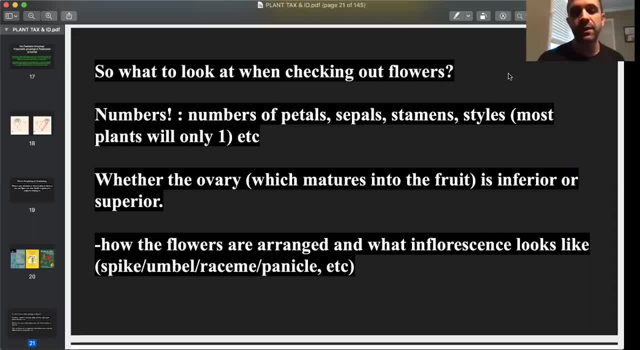 petals and sepals, And then also how the flowers are arranged, because few plants will just send up one flower. They're always grouped together on a stalk. It's a compound flower, an inflorescence. Look at the way an agave flowers. There's hundreds of flowers on an agave. 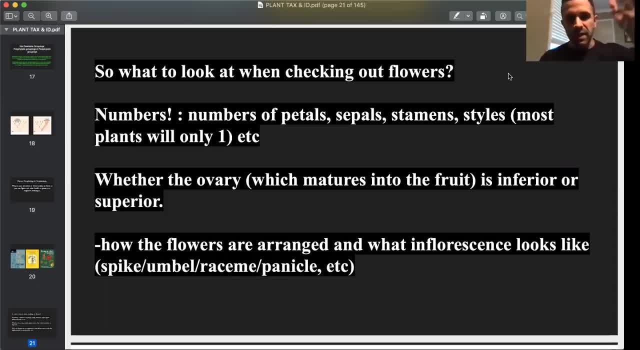 americana. You get that massive asparagus-looking stalk that sends up and then it branches and it's got flowers on each. I mean, look at the inflorescence. Don't stress yourself out trying to figure out what the name for the inflorescence is, because, remember, it's just 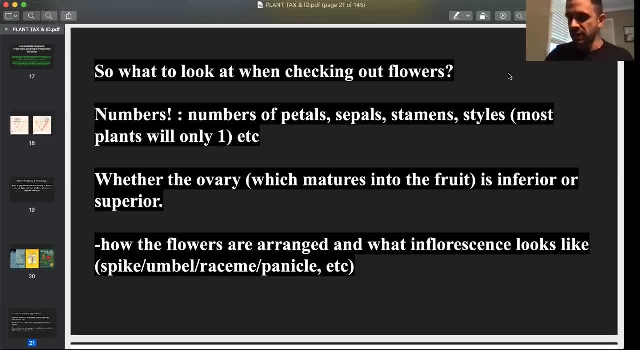 the human idea. It's the human way to connect the flower structure, consistencies and flower structures. Okay, just try to remember what that flower structure looks like, how it branches, how the flowers are arranged. Do they droop? Do they point up The many stalks that branch off? 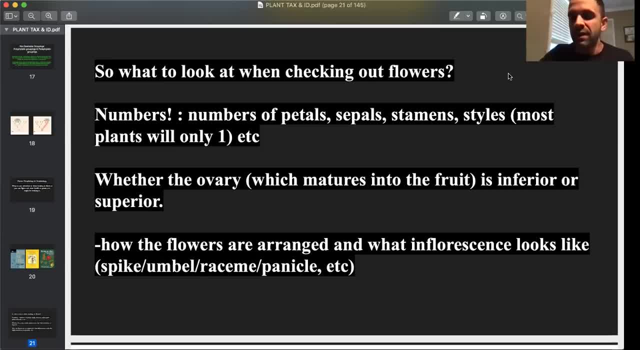 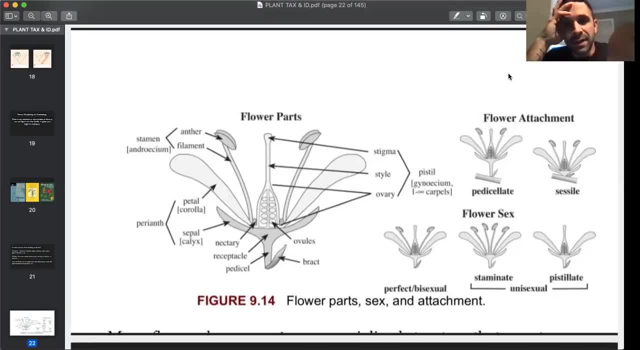 the main stalk. how long are they? Is there one at all, Whatever? So here's flower parts, right? So this is the thing that you got to learn. We're only going to focus on the diagram beneath the word flower parts and the diagram beneath the word flower sex, Staminate or pistillate. I just 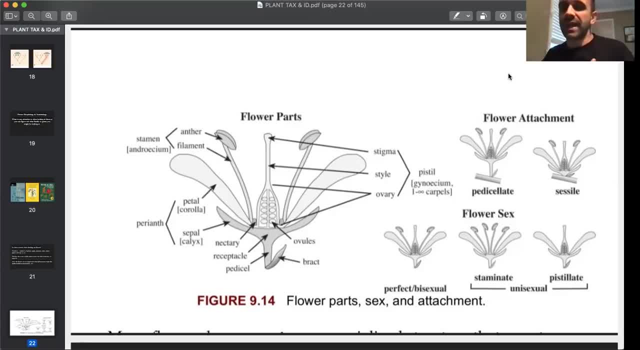 call it male and female, because that's the only way to do it. So I'm going to focus on the easy word to use. It's easy way to anthropomorphize this year. Remember it easier. Same reason: plumbers call certain pipes a male end and a female end of a pipe. So it's really easy way. 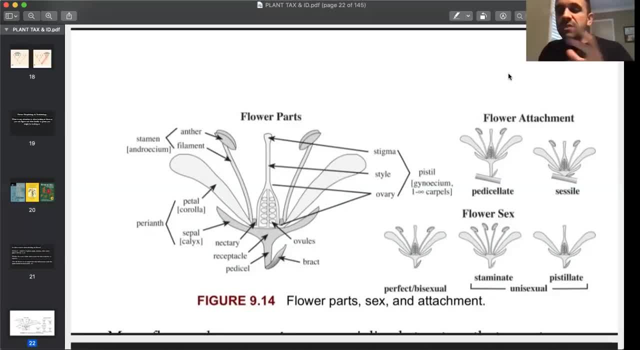 to anthropomorphize things and think about them. So most flowers are perfect. They'll be like this flower on the left, where you got male and female parts in the same flower, but you go to like cannabis, or you go to coyote bush, which is in the sunflower family. Those are dioecious plants. 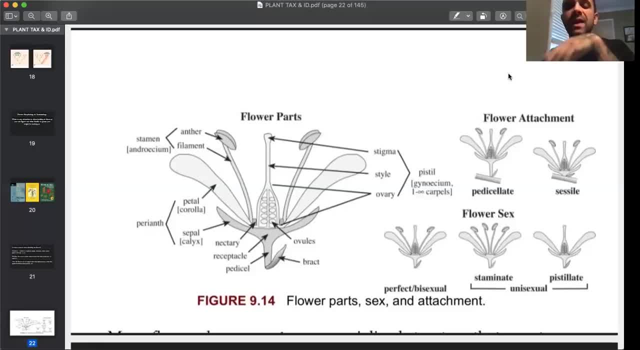 They will either have. they will either have. you know the plant will be consistent entirely of male flowers or entirely of female flowers. You also have monoecious plants, which means monoecious and dioecious. The thing that remember is just all that means is the flowers are not. 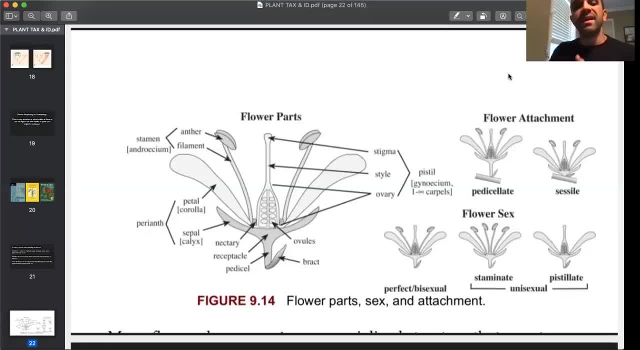 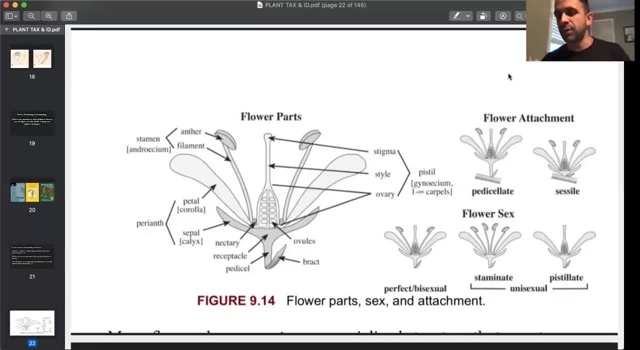 Dioecious means an individual plant produces only one kind of flower, either male or female. All right. But like I said, I think like 80 or 90% of plants have perfect bisexual flowers. In that case, this general structure we're looking at here under the flower parts diagram holds true There. 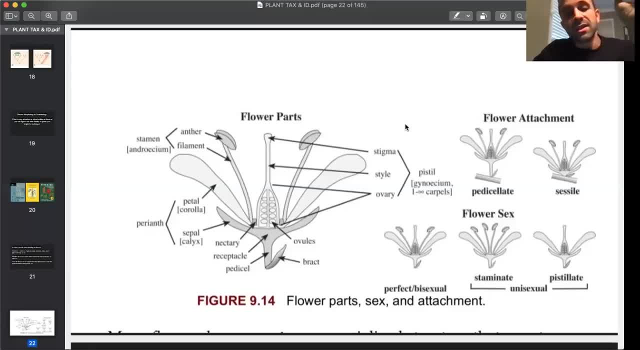 will be variations on it. Some plants won't have any sepals. Some plants won't have any petals. Uh, some plants will have three styles, Like I said. uh, whatever, but they're all going to have more stamens than they have. styles There's always going. 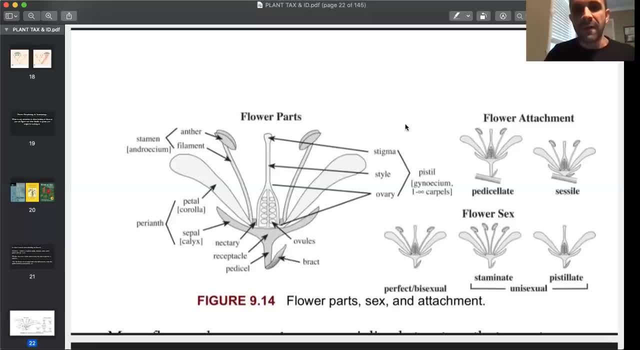 to be more, uh, male parts than there will be a female part, And generally there's only going to be one, one, ovary. Uh, so the thing this: you memorize this structure, you'll always understand, you'll always be able to see it and pick it out and know what the stamens are in any plant. 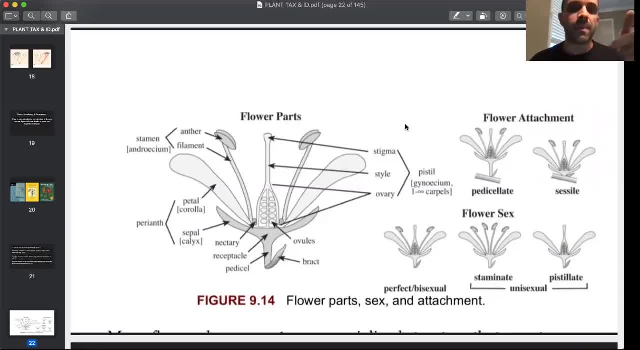 So we'll start with the stamen. Stamens consist of a pollen anthrofilament. Keep saying that to yourself: Pollen anthrofilament, pollen anthrofilament. nice prose, like a nice cadence, Just recite it yourself: Pollen anthrofilament. That's what I did. 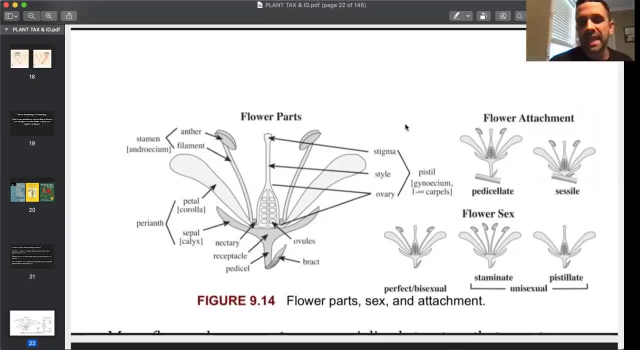 That's how I would remember stamens, When I was first learning this. I would see stamen, Okay. So you got the grouping, you got the word stamen and then you know, subtending that label, you have pollen anthrofilament, pollen anthrofilament, You say it. 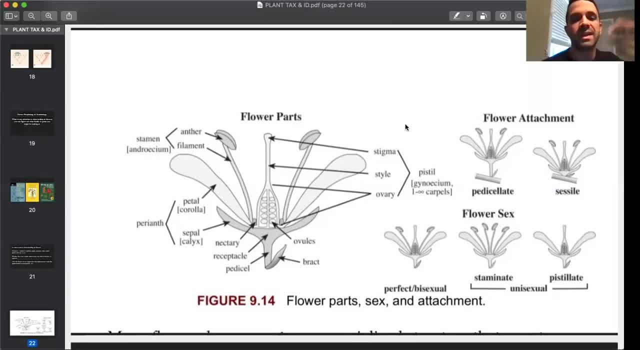 enough times. It's like remembering a song or remembering, you know, a cadence of the way someone says something. Conversely, on a pistol, which the technical term is gyno, But you don't need to think about that now. A pistol is the female part. This is the way I. 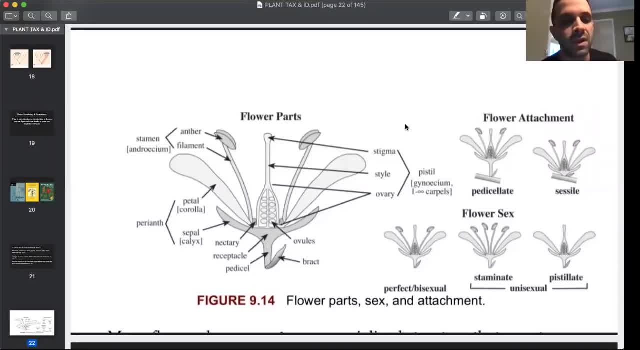 remembered that when I was first starting, was it's counterintuitive. You think pistol, you normally that's a very phallic tool. You normally think dick or dong, whatever, but it's counterintuitive, You just remember it's the opposite. So yeah, pistol would make you think. 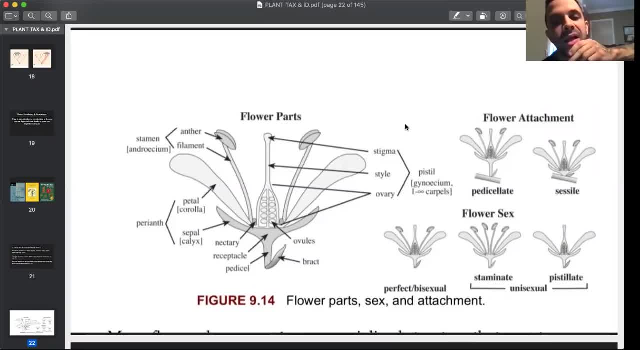 it's this, It's counterintuitive, It's the female part, It's where the ovary is, etc. And it's also spelled differently. But anyway, pista is stigma style ovary. Say it a bunch of fucking times, Write. 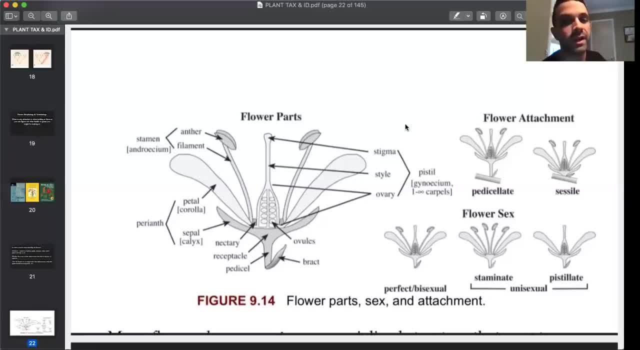 down: stigma style ovary. stigma style ovary. stigma style ovary. And eventually- you know you do it enough times- you'll be reading about plants to the pistol. Well, the pistol is arranged this way. Okay, what's pistol? Oh yeah, stigma style ovary, That's the way that sounds. 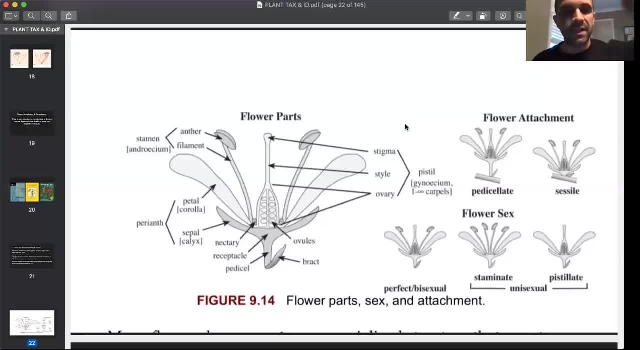 you know, And that's in subtending order from top to bottom. Same thing with pollen, anthrofilament subtending order: The pollen's at the top, pollen comes out of the anther. The anthers are those little banana shaped things at the end of the stalk. The stalk is the filament, etc. So you got. 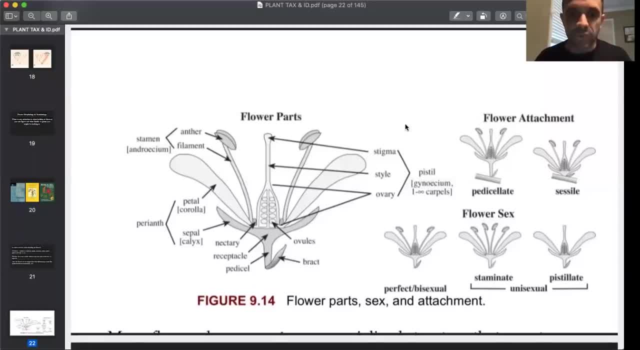 stamens. you got pistils Inside the ovary. you got the ovules. Ovules are just a fancy word for seed. You know, if you had a poppy bagel this morning, you ate some ovules. Okay, poppy seeds. 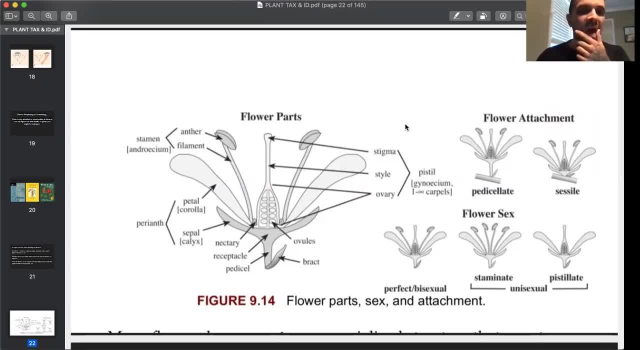 are ovules. Sunflower seeds are ovules. The perianth, the same way that a stamen consists of pollen, anthrofilament, a perianth is composed of petals and sepals. Petals are synonymous with corolla, Sepals are synonymous with corolla. So you got pistils, you got pistils, you got ovules. 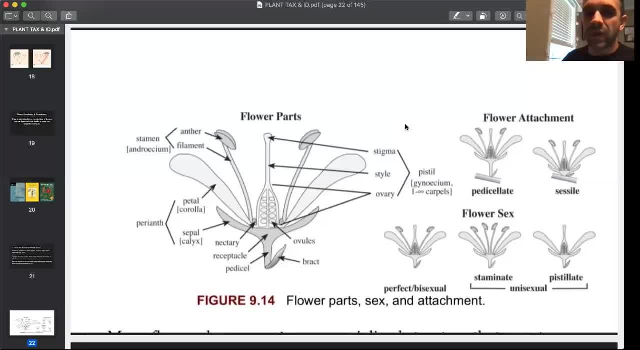 calyx. But again, you know some plants don't have petals and sepals, Like you look at like lilies, or you look at like proteas, which will really fuck you up. You're like Australia Southern Hemisphere family. you know you get them all over the South Africa. you get them in. 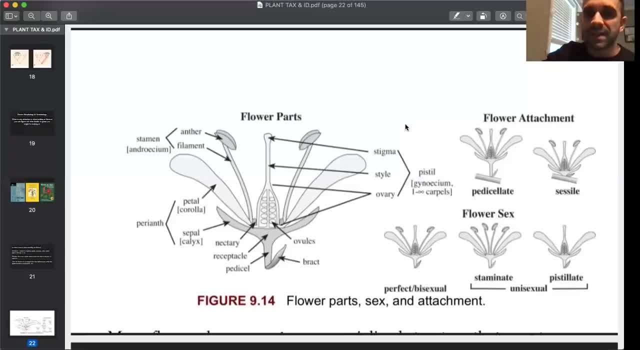 South America. you get them in Australia. Proteaceae does not abide by this. The sunflower family does not abide by this diagram. There's variations on it, But I brought up proteas because they're different. So again, this is the human way to think about the way that these floral 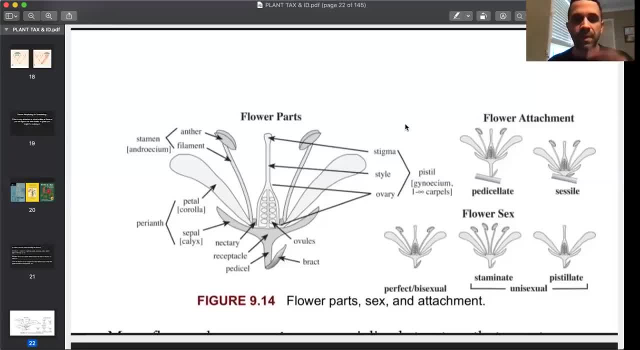 attractant. these modified leaves that have been, you know, pigmented and turned into floral attractants, are arranged So tepals. if you can't tell if it's a petal or a sepal- and they don't- they're not differentiated very much, they seem to just all be emerging from the same area. 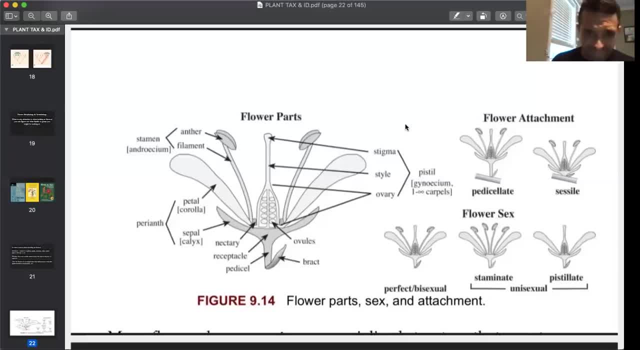 the same base tissue, then it's a tepal. Okay, So you got petal, sepal and tepals. Most plants will have petals and sepals Always up top, or, you know, distal from the axis of the plant, the sepals always closer to the 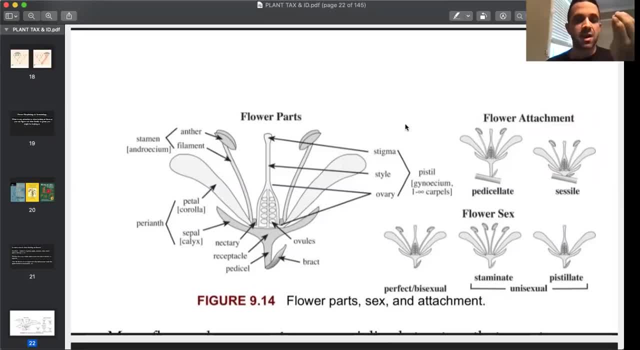 axis of the plant. you know where the that stalk that the flowers on comes from. So sepals are below petals are above. petal corresponds to corolla, sepal corresponds to calyx. Okay, and these are all fucking important If you're looking like a sage flower, a salvia flower, the calyx. 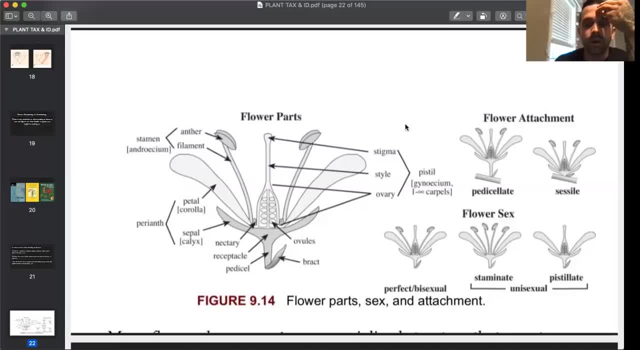 ends up holding the seed. you've got this superior ovary, That kind of rests inside this calyx, the petals, the you know, senesce, they, they get old and fall off once that flower is pollinated. And in the sage, in most cases the sage family you have. 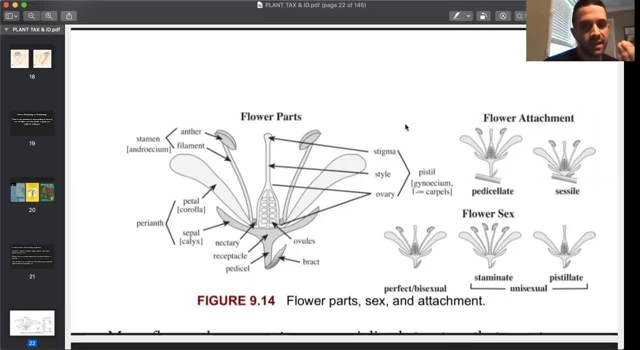 four ovules inside that ovary which is nested in the calyx, you know, and the calyx in the sage family is often not very attractive. It's just a structural thing. It doesn't serve in attracting, attracting pollinators. So any questions on this? 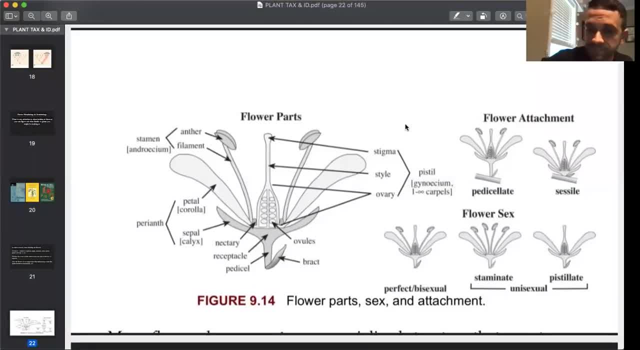 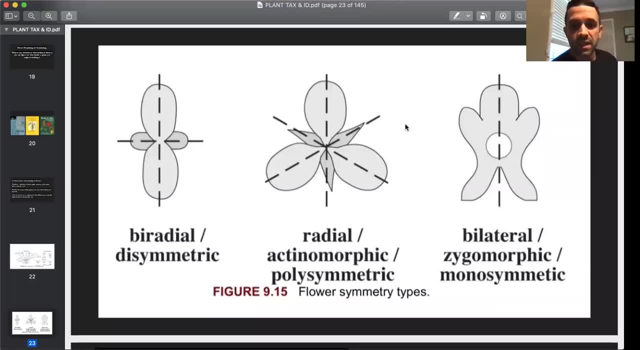 No, all right, And if I'm moving too fast, you know, give me a heads up. Okay, this is the last thing to focus on with flower structure, So we're not. don't focus too much on biradial, just focus. 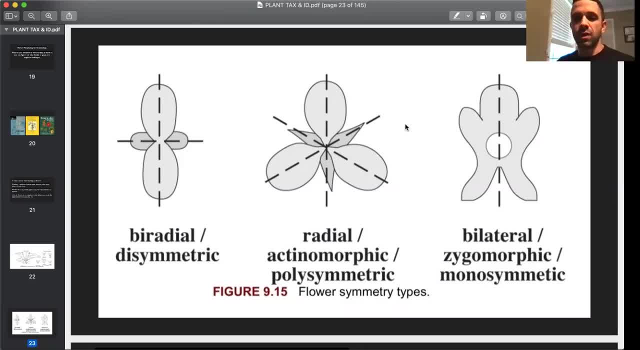 on actinomorphic and zygomorphic, which again are just fancy words for radial. Can you cut it? If you cut it, you know, across. can you cut it like a pizza or bilateral. Can you cut it like a heart? You know you can fold it and it'll be symmetrical one way, but if you fold it the other? 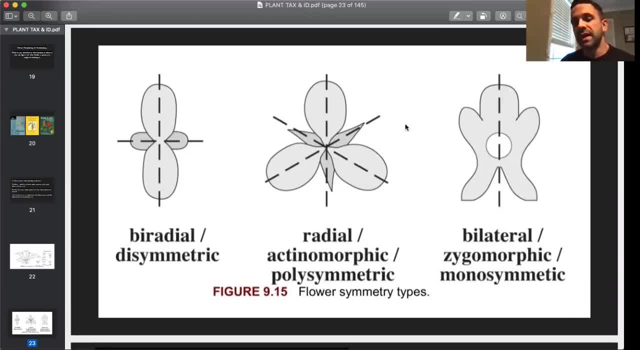 way. it will not, And this again just will help. This is important if you're identifying a flower like: oh, it's bilaterally symmetrical, Good chance. it's in the order Lamiales, the order of sages, just like Orobancaceae, Scrophulariaeaceae, Lamiaceae, et cetera. These are they all have. 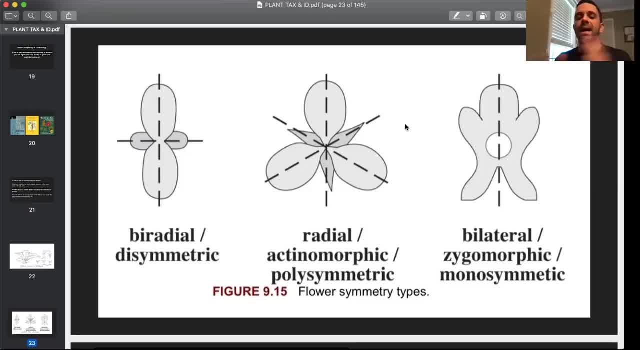 or Penstemon's Plantagenaceae. These are all bilaterally symmetrical flowers. They're all in order, Lamiales. People knew this before DNA. just by the way they looked, Of course, when we went and looked at the DNA, it was true. They were all they were. that was a monophyletic clay, They all. 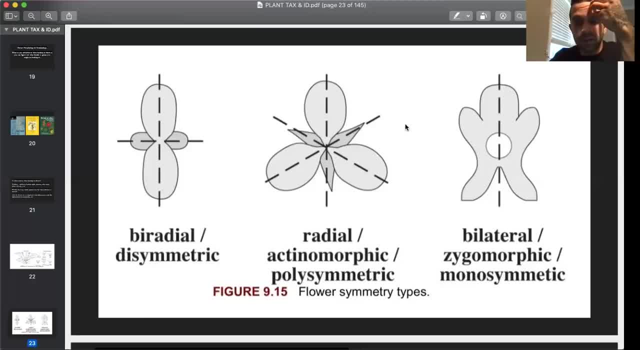 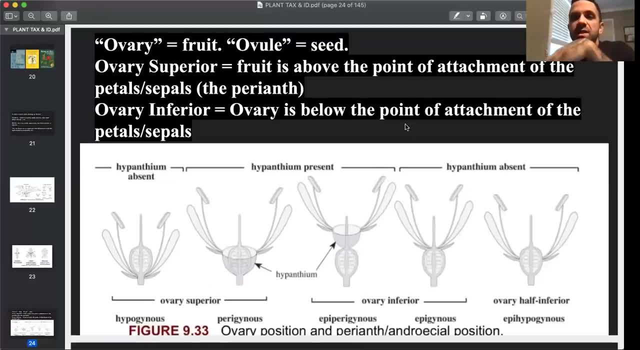 emerged from the same ancestor in Lamiales. They were all related. Ovary fruit ovule- sepia- we ran through. this Ovary superior fruit is above the point of attachment of the petal. sepals Ovary. 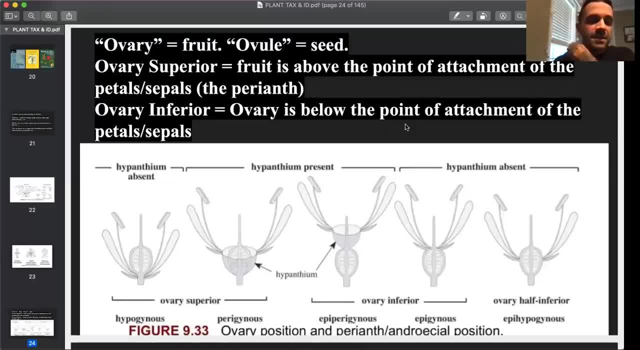 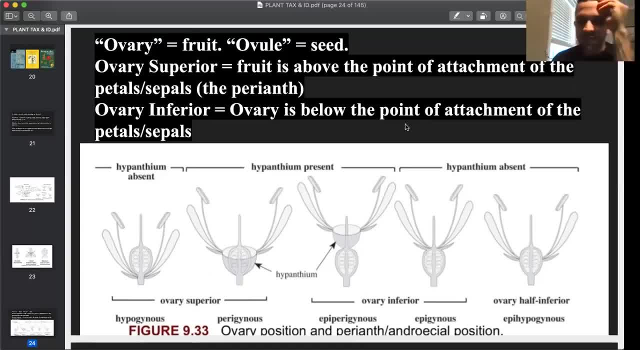 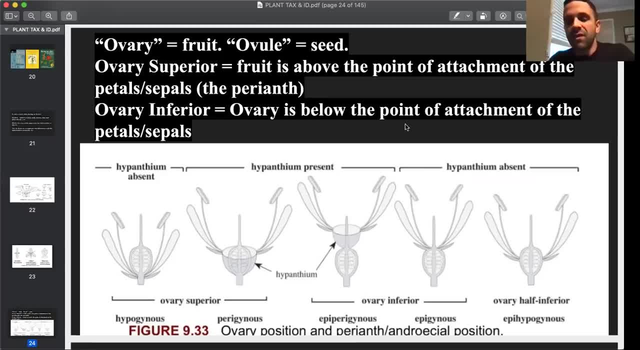 is by making mistakes, but you also got to observe it firsthand. If you're in a place where nothing's flying right now, go sneak into the conservatory. if you can, or pay, Pay, but if you don't have the money, try to sneak in. Because, again, all this shit, in my opinion- museums, libraries- 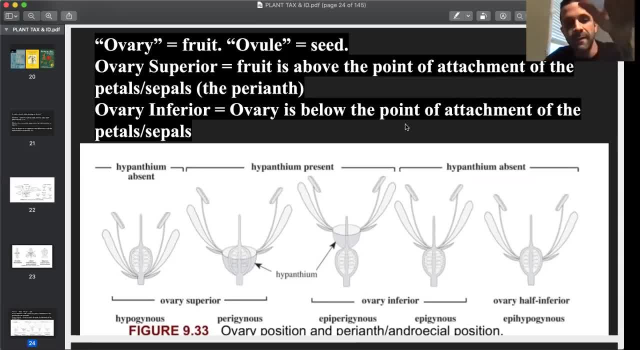 all that shit should be free. If you have money to support those institutions, do it. But at its root, this shit should be free. no gatekeeping. uh, here's examples of ovary inferior and superior. forget about hypanthium now. we don't need to memorize that, you know. and of course there's 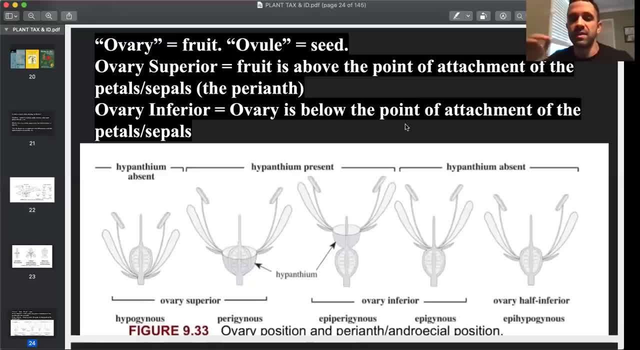 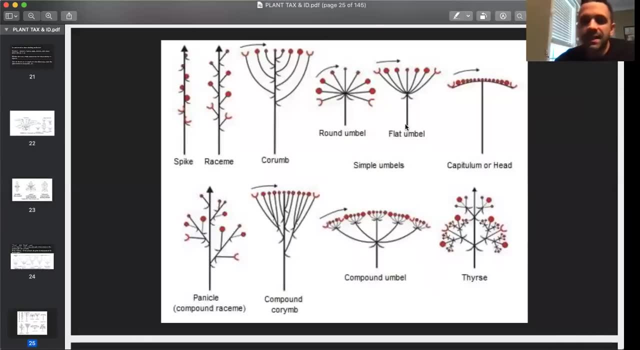 variations. sometimes the ovaries like halfway up the, the sepals and petals are attached halfway or whatever. it doesn't matter. just focus on inferior, superior, is it above, where the sepals attached to the stalk, or is it? is it? is it below? different types of inflorescences? again, don't fuck yourself. 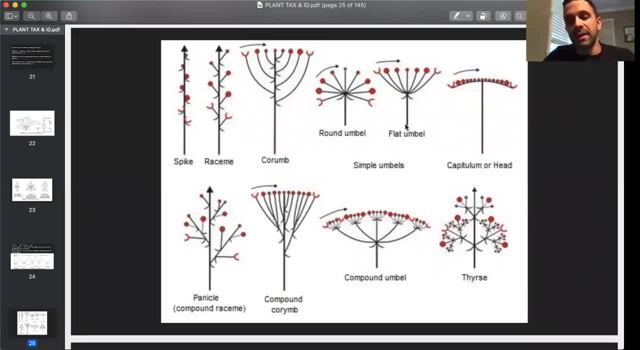 up trying to remember these. go observe them in the field and ask: what the fuck am i looking at? what would you call this flower structure? okay, you got spikes. a lot of orchids- uh, produce spikes. uh, racine corums, umbles- um, everything in the carrot family produces an umble, but it's not. 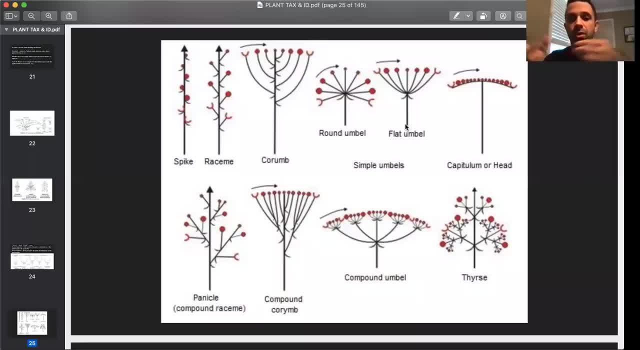 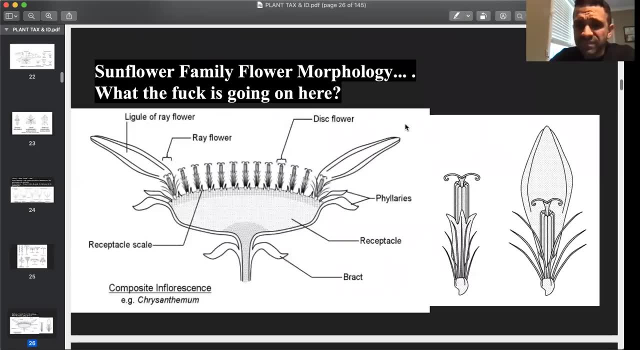 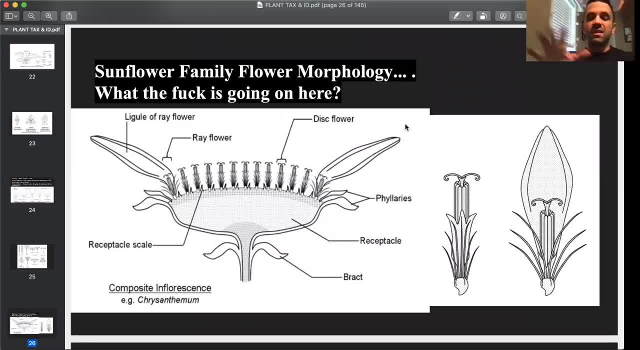 shit starts to get interesting. this is totally different from everything else. sunflower family is different. you know, i'm always ranting about asteraceae. i fucking love it. it's everywhere. they're so cool, they're so adaptive. uh, you know they're. they're the most ecologically successful. 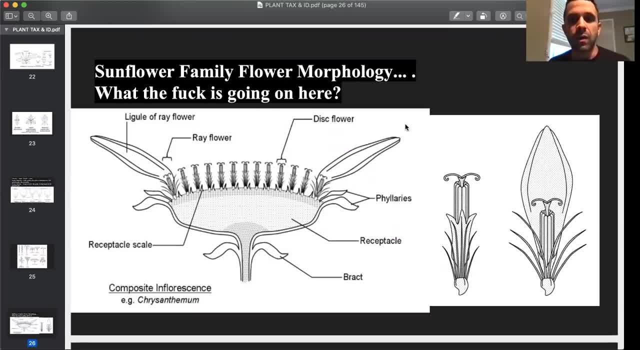 plant family on planet earth right now. uh, you know, orchids have more species, but orchids are most at lower latitudes. um, so what's going on here? you got a ligule of a ray flower. you got two different types of flowers: disc flowers, ray flowers. okay, it's not that this. 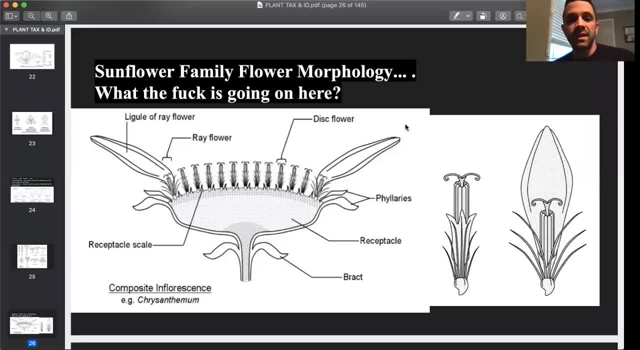 might seem intimidating at first, but it's not once you get the gist of it. you got disc flowers and ray flowers. okay, then you got receptacle scale, aka the palea. uh, receptacle, i don't even use that word, i just say capitulum or capitula plural, and filaries, these things that are. 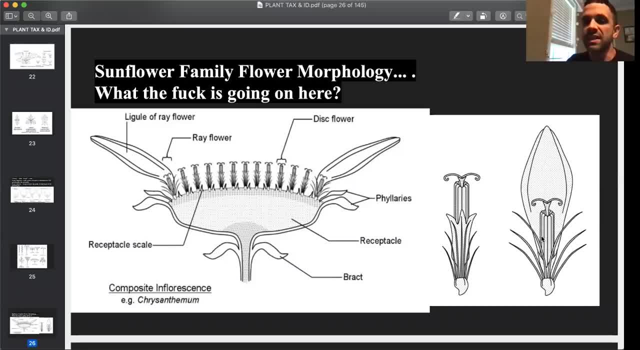 diagnostic and figuring out what species you're looking at. on the right you see a diagram of both a disc flower and a ray flower. um, this is really. this was a massively adaptive trait when this evolved, and the whole order astorale is not just the family- tends to have these compound. 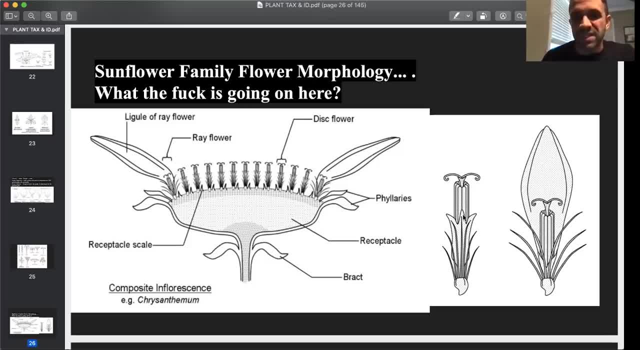 flowers, and not only that but tends to do secondary pollen presentation, which uh sunflowers do. so those styles, those little y-shaped looks like a bent y right with its branches bent back, those emerge. they are functionally stamina. first, they produce uh male flower, they, they produce they. 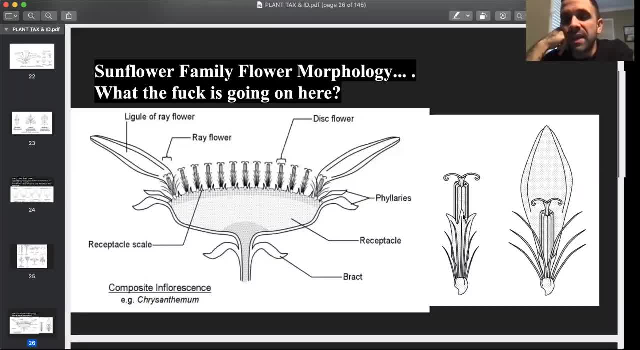 put pollen out first, uh, and then they become receptive to pollen afterwards. but this was so adaptive because it's a way you're grouping so many flowers together and because the way that the flowers mature in the disc that there's always a this thing: the single flower head, the 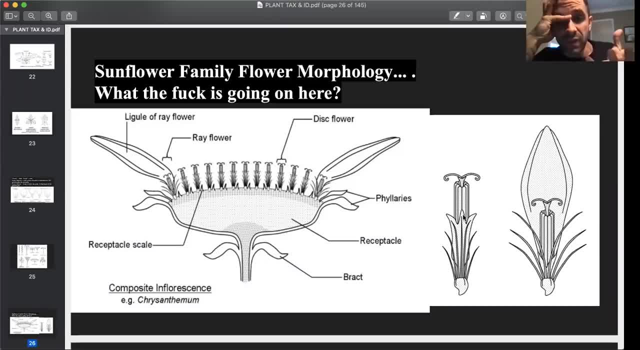 capitulum will be blooming, in some cases for a fucking month, you know. so, as the flowers on that, they start: at the outside, those mature first, on the inside, those mature last. and always, throughout that month, you know, there will be a flower presenting pollen and being pollinated. so 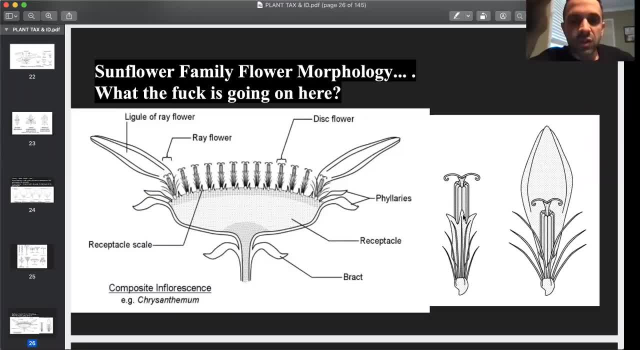 ecologically. they're providing nectar and a sugar source for insects and, in some cases, birds for a really fucking long time, you know, whereas some flowers only bloom for a few days, sometimes only a night, like saguaros only bloom for a night, so this is massively important for the fucking food chain, but also this is such an adaptive trait. 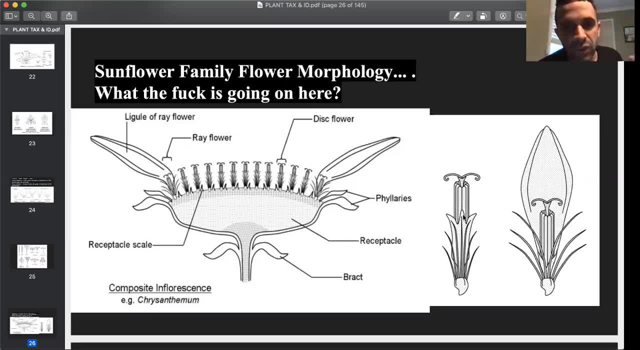 because it's you've got so many. i mean, one flower head can produce sometimes thousands of fucking seeds, right? so you've just made a thousand uh offspring. and not only that, but we'll get to this. unfortunately this doesn't show it, but you know that. then all this does that. 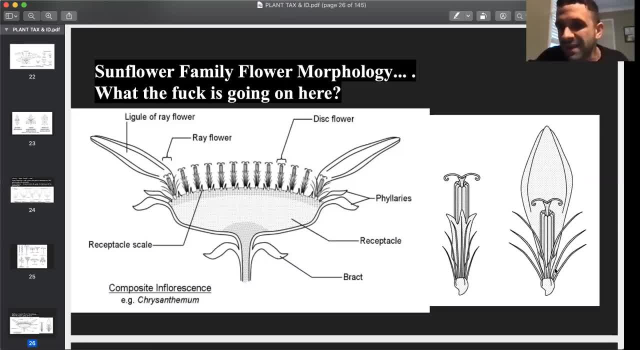 the ray flower does well. they both do actually see these elongated spikes at the bottom. so you got: look at the flower. everyone still with me, yeah. so you got these flowers in the right right. you got a disc flower. you got a ligulite flower at the bottom. you have a seed that that you know little. 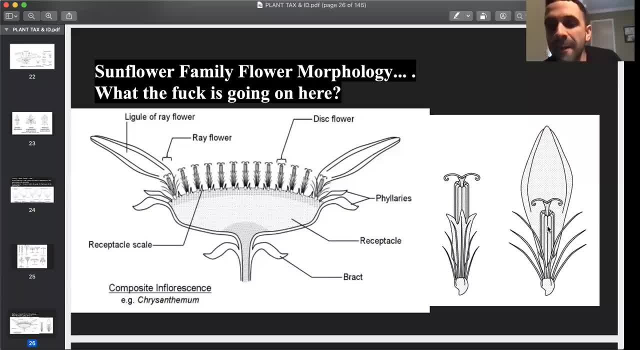 comma shaped thing, and then on top of that you have the pappus. okay, pappus can also apply to grasses, um, i think, yeah, that's right anyway, but but in the terms of asteraceae, the pappus is that that dandelion fuzz it would? it acts as a dispersal mechanism and it's a dispersal mechanism. 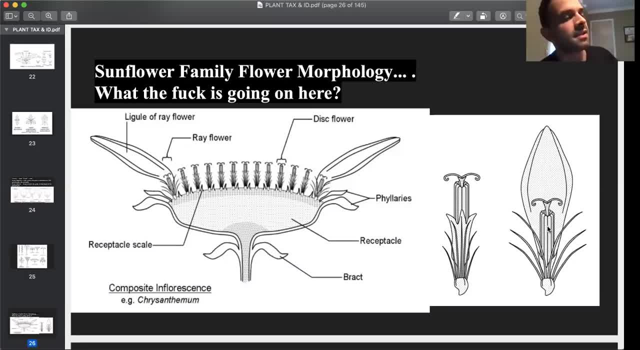 sometimes the pappus has been modified to stick to other animals and then you know later, it gets brushed off somewhere and dispersed somewhere else. you know, in the case of a lot of members of the sunflower family, it's it, uh, it picks up wind currents and it gets transported somewhere. 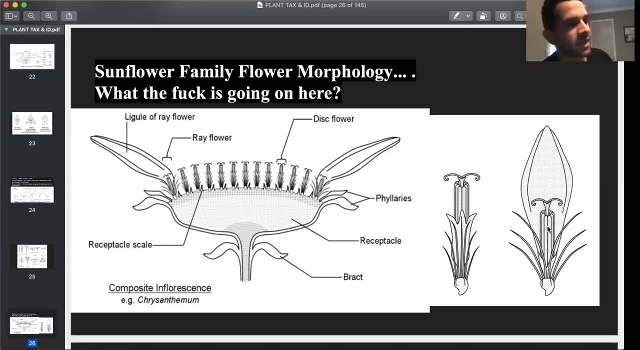 else you know. so i mean you've got- you're producing tons of seed and you got a way to get them around. they don't just fall and drop on the ground. so this thing- that's why this family is everywhere and a lot of weeds, a lot of non-native weeds can be. 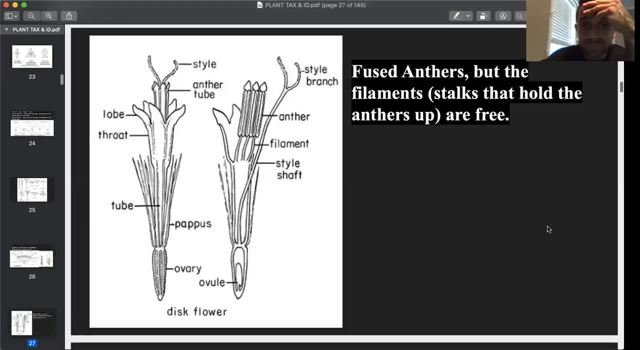 members of the sunflower family too. so the thing that's really weird- and this is hard to to grasp right here- is that, unlike most, most members, if you look at that diagram on the right most flowers you know you got stamens, pollen, anther filament. okay, that's easy to grasp. i get it kind of looks like a bug antenna. 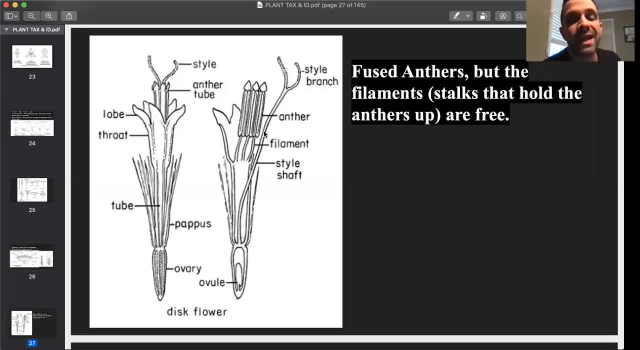 in the case of the sunflower family, though these have been, the anthers have been fused together. the filaments, the stalks that hold them, are not fused together. they're free. and you've got this structure. you can never see it unless you have a hand lens. you 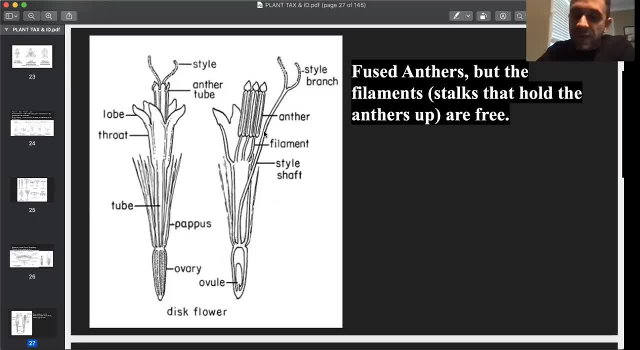 can't ever really see the anthers on a member, on a flower, of a member of the sunflower family, except for the one i'm about to show you, because they're fused together and inward facing in this little tube, and so this style, this is the secondary pollen presentation i'm talking about. 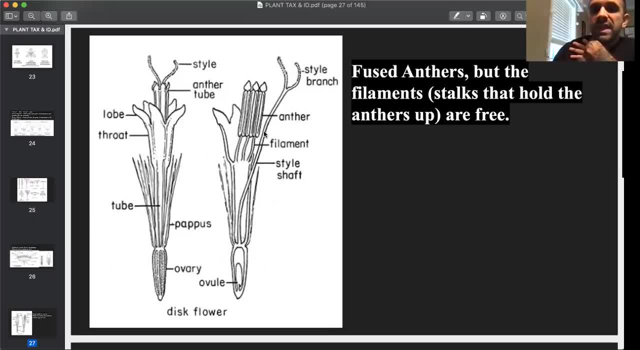 this style comes up in between: that fused anther tube pushes the pollen up, presents it and then, once it's been removed, then it branches out and opens up and becomes receptive. this is a massively adaptive trait. but it also makes them hard to study because- and it really fucks people up when you're looking at them, because you can't really see what's going- 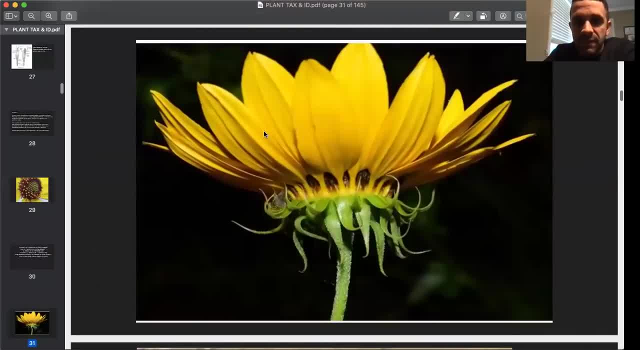 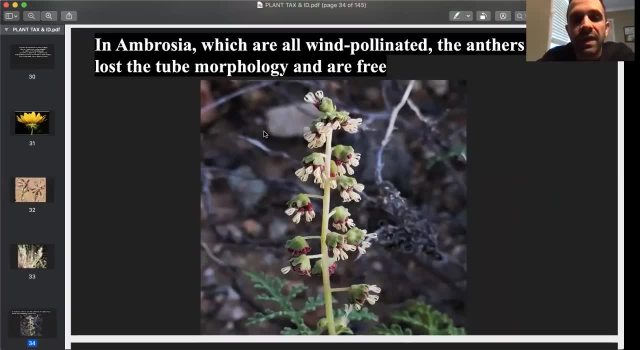 on, except in where the fuck? i don't think i put it here we'll go, we'll get here really quick, except in ambrosia. so ambrosia is one of the few uh clades in the sunflower family that's wind pollinated. it's not pollinated by bugs, so what good would it do to just have a fused? 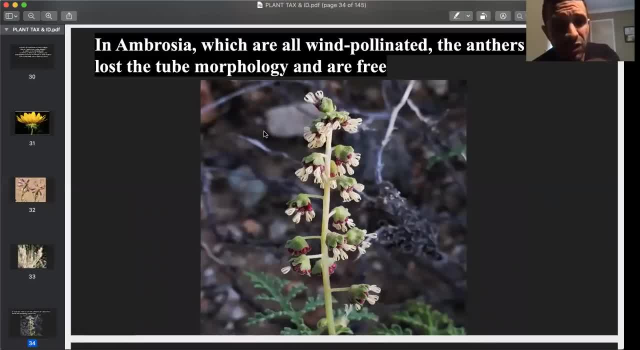 anther tube and then have the style: push them out right. also, these flowers are not bisexual, which is odd for the sunflower family too. they these- you know, ambrosia is such a fucking weird flower structure. these are the ragweeds. these are what irritate. 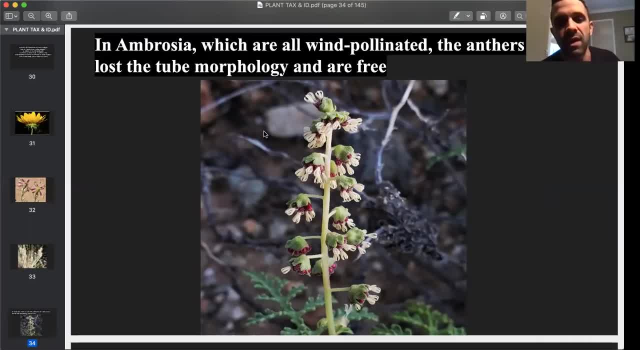 everyone in the spring and and through summer into fall massively, because they're wind pollinated. they just dump out tons of pollen, tons of plant sperm to, just, you know, irritate everyone's- uh, you know, make them sneeze like hell, itchy eyes, whatever. so these are animophilus. they're wind. 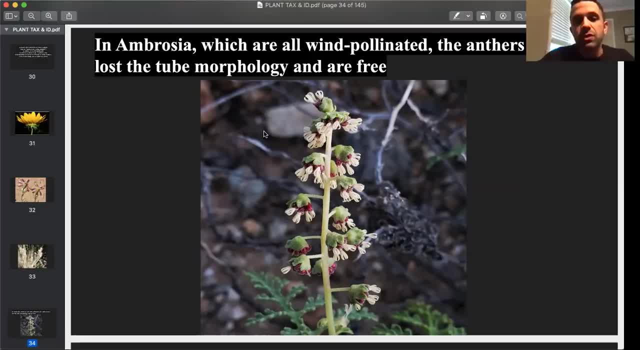 pollinated so because of that they don't want. there'd be no point in having a fused anther tube. that's not going to be an adaptive trait. these are five. these have evolved so that that anther tube is no longer fused and the anthers are free and so you can get a. the thing that's important. 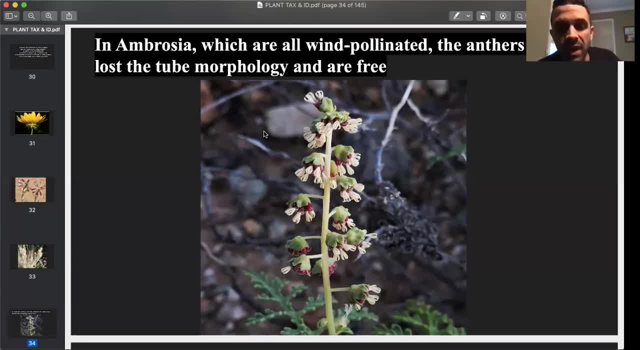 is. it gives us a close-up shot of what's going on with asteraceae anthers. i mean, this is one of the few clades in which you can actually get up close and see the anthers. so these are all staminate flowers down below, not in the photo or where the female flowers are. 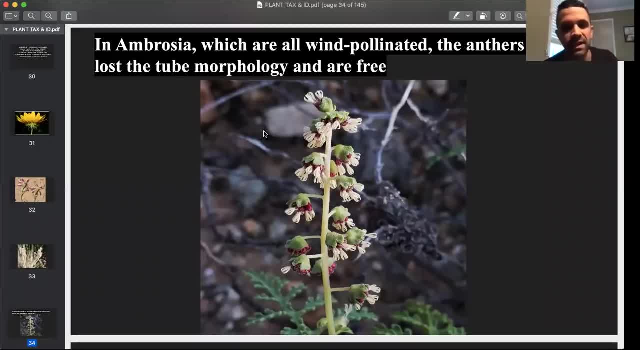 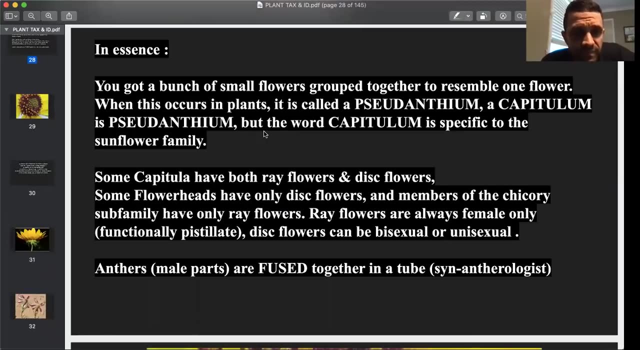 the pistillate flowers. but it's it, really it's. it's a cool example to see one of the few cases where you can actually see, uh, this family's anthers without a hand lens. so any questions real quick. no, no, uh, i have a quick question. yeah, what's up? um, so it, do you know of any books that are just? 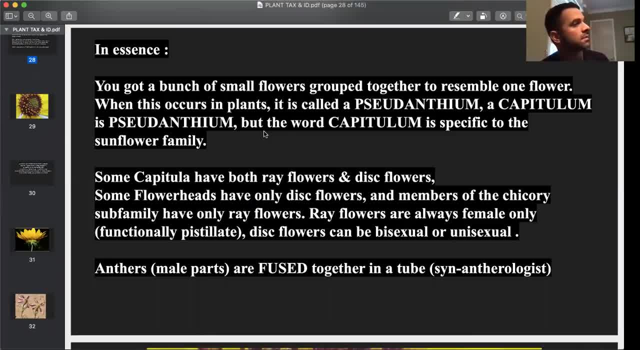 that the whole focus is on the asteraceae family. oh yeah, there's a shit ton. there's one online, uh, and i used to have it on that google drive thing that i would give out, but it's like a thousand page book. it's like. it's great, though, because the photos in it are. 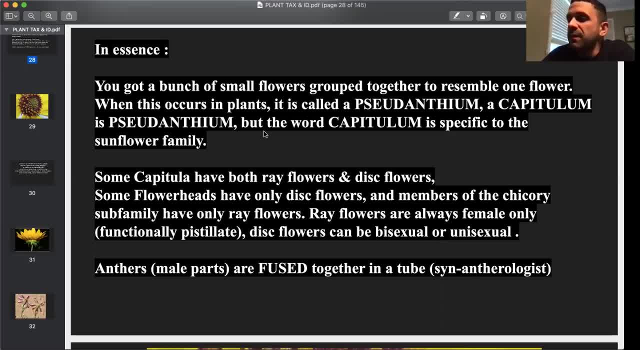 fucking awesome. it's in pdf form too. vicky funk before she died sent me one, but it's also available online. you could try googling all one word: comp book for distribution. comp as in composite- another word for the family- composite flowers. comp book for distribution pdf. 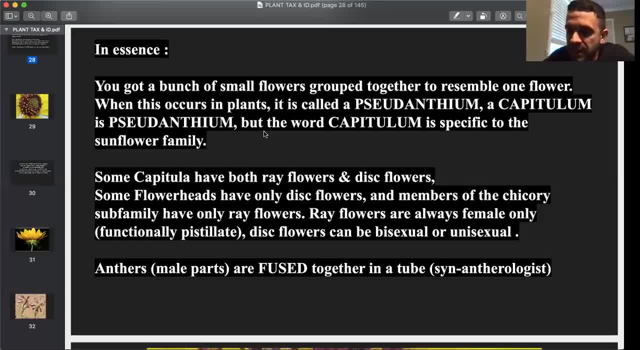 it should come up, or if you email me i can send you a copy. i can email you a link to a copy later, but that really gets into it and there's. you know there's. each chapter is like designated towards a different order or family or different sub family or or tribe, whatever, but it's got a great glossary. 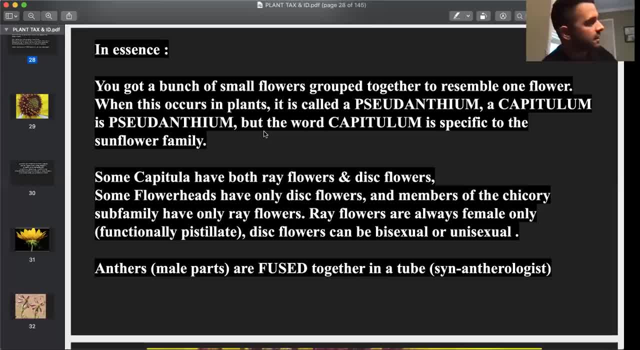 in the back, etc. there's also another book called uh, sunflower, the sunflower family in north america, which was put out by botanical research institute of texas. uh, they have a publishing company. that's a fucking great. that's a great book too. um, and i think it just came out, a 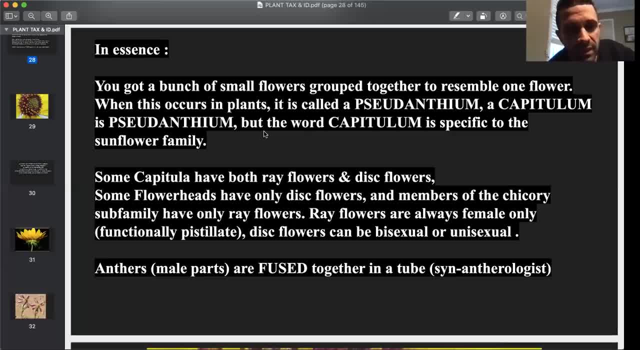 year or two ago and that covers every genus in north america and talks about habitat and you know, synapomorphies of of every genus and tribe. it's a great fucking book. but those are two to start. yeah, no, okay, thank you. yeah, i'm just, i'm tired of overlooking them. yeah, i know, i used to. 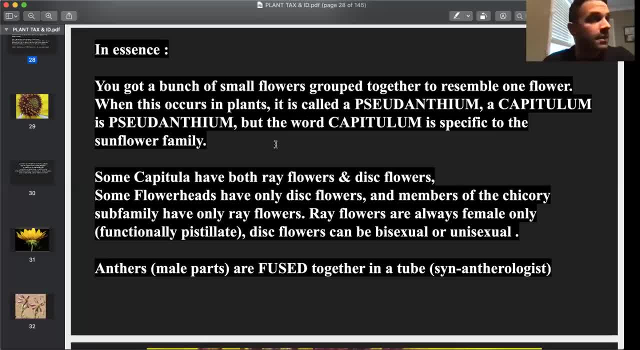 just ignore them. and then i i was like i gotta fucking figure these out, you know. and when i did, i was holy shit. and you see, some of the south american ones- and they're not just these boring little yellow daisies anymore, they're a lot of them- are pollinated by hummingbirds, they're. 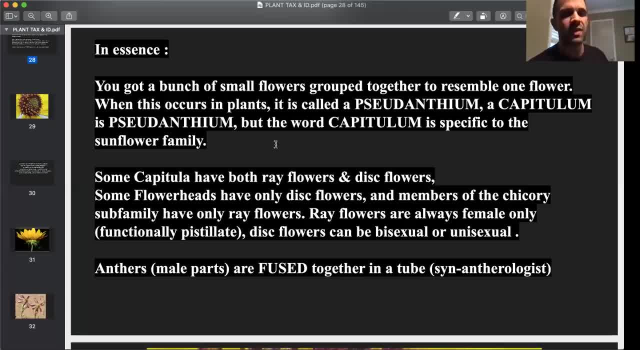 like radically colored. they're just the most fucking bizarre things. go to like: look at the tarweeds on hawaii. look at like- uh, i mean some of the other, some of the other- aster, aca, you know, all over the world. they're like south africa. there's members of senecio, which is a weed here. 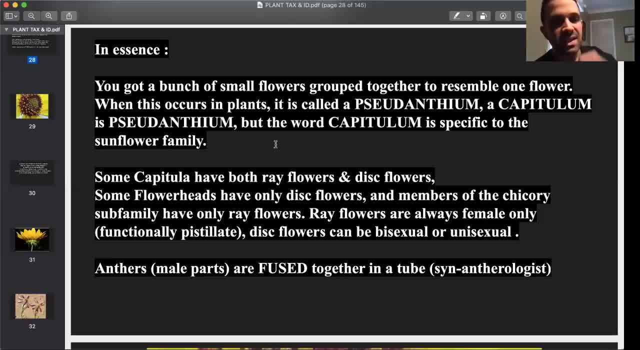 of the senecio tribe that are like 30 foot tall trees. mount kenya, you know, equatorial highlands at 16 000 feet. i mean, when you see the variations on a theme that evolution's produced in this family, that's when you'll kind of get hooked. you're like 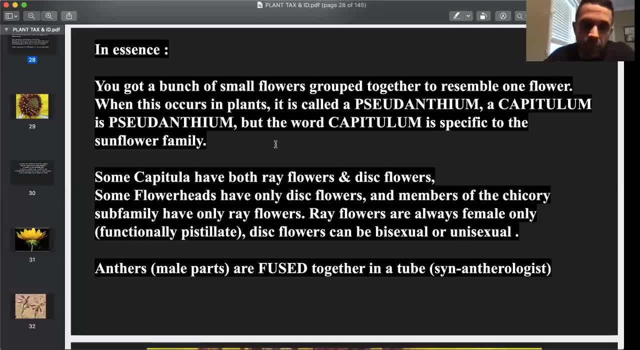 this is fucking wild man, holy shit. so it's the. yeah, they're cool man, but always get pictures of fileries. when you're taking photos and pictures of fileries and leaves, because, yeah, a lot in north america at least a lot of the flowers. look, the same sounds good. i'll be using i naturalist to 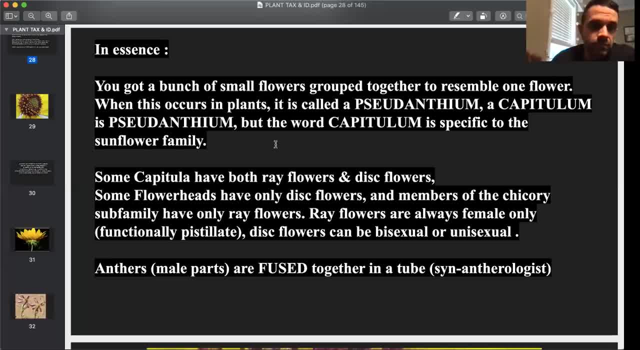 because that that seems like one of the only things that uh like, if you take some really, really detailed pictures, that's that's where i've had most of my luck identifying most of just those. you know, those dycs, yeah, yeah, yeah. and eventually you know you're into them long enough and you start to notice like you'll be able to look at. 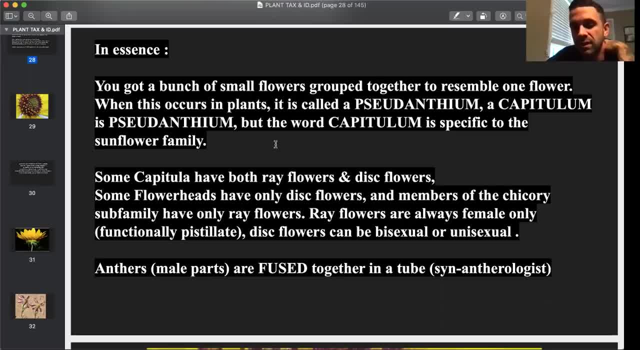 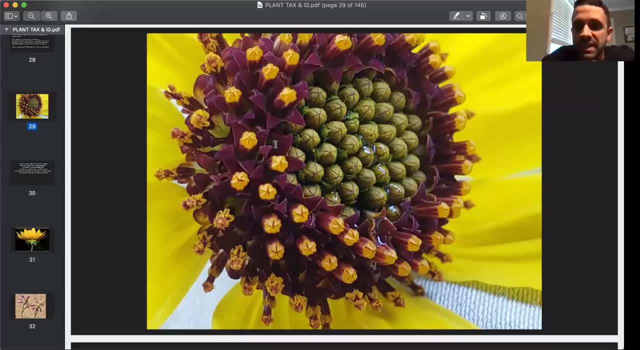 a flower and be like: oh, that's probably in this genus, you know, yeah, because there's apomorphies on every level: genus, subfamily tribe, so, uh, anyway, um, we already talked about all this stuff. here's a nice money shot of, uh, an encelia flower, brittle bush, uh, in the deserts. 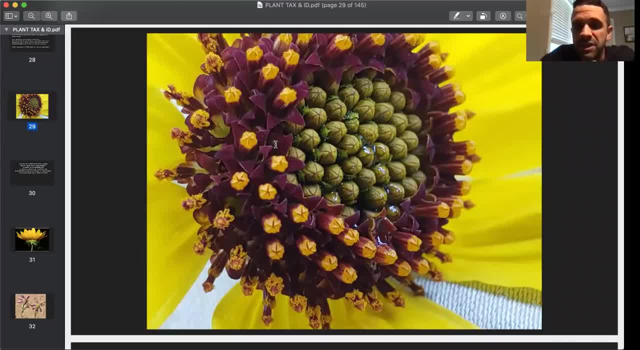 you know, super common plant, successful plant in the deserts of north america. you'll see them growing on the side of the fucking road and in uh arizona, southern arizona. the reason they grow on the side of the road is because they get all the immediate runoff whenever it rains, acts as like a. 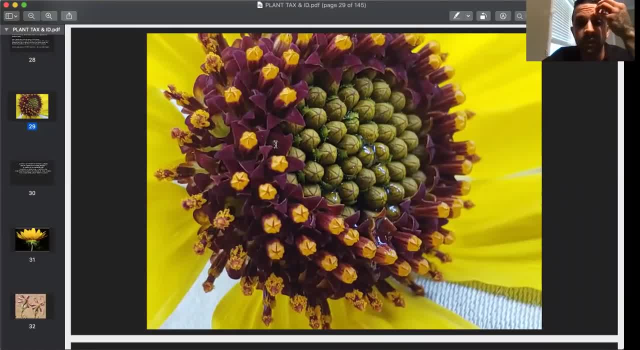 little feeder tube, a little funnel just funneling a moisture um. and here, right here, you can see the individual flowers. see the ones on the outside matured earlier than the ones on the. the ones on the closest, the center of the flower, haven't even opened up yet. those 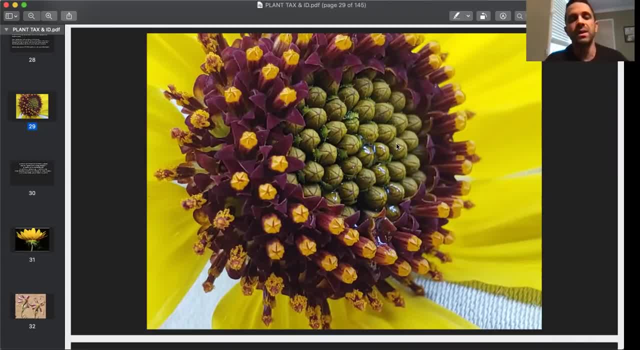 fused anther tubes have not even opened up yet. you've got the purple corollas- five lobes, so what would be petals are all fused together in this tube. you got an anther column poking up out of that tube and you got the flowers maturing cent, cent centripetally um centripetal maturation. 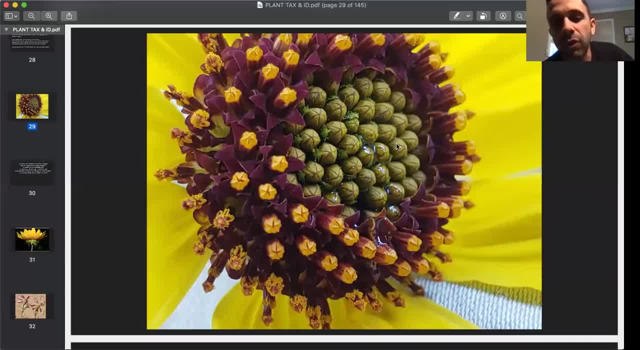 so this thing, these things will bloom for weeks. man, they smell great. there's a cool resin you can scrape off the stems. um, which is cool too. i mean, they were used as incense for a while by a lot of the spanish missionaries when they were committing genocide, you know, for the 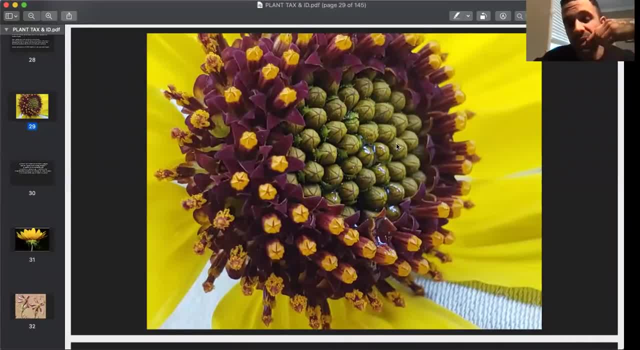 churches for the good catholics. nice, because that incense smells good when it burns. but you can see, i mean right here, i mean look, you can see the individual pollen granules on those outer flower, those outer florets. so that's. the other thing is, the actual flowers are called florets and the 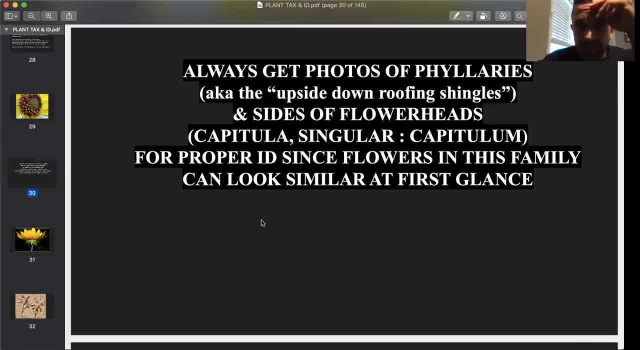 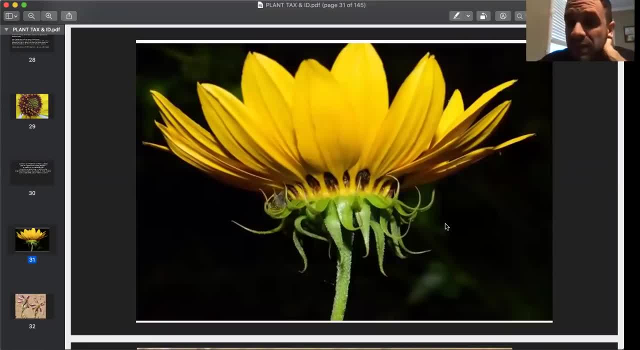 florets are grouped together in a capitulum. here's the flowers. give photos of filaries. here's the filaries. this is the case in which it's diagnostic, this fucking flower. this species is a texas endemic, south texas endemic, from the sand sheet. uh, helianthus praecox, i think it's a variety or subspecies. run yoni, i you know very. 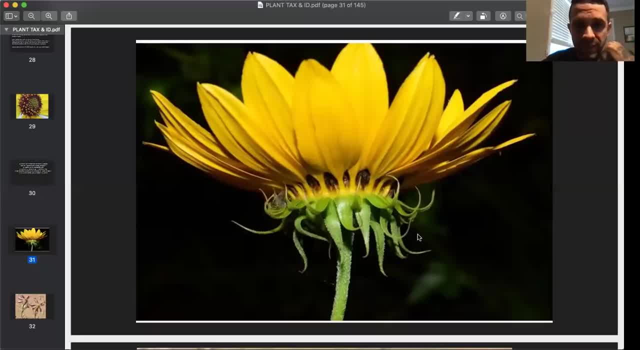 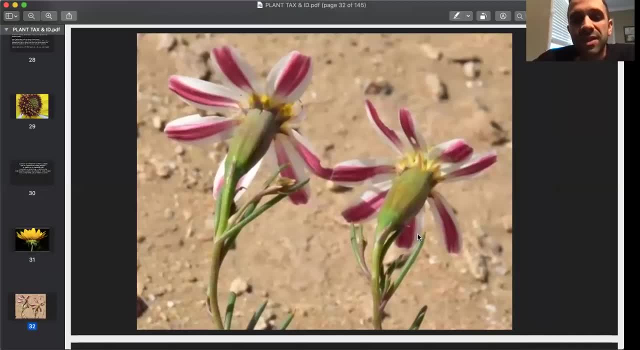 you can see the, the fucking filaries right there. i mean the way they're so elongated, spiky, the way they were curved. this is nicoletti atrifida from the deserts of baja. this thing smells amazing, like all members of the nation, and i'm going to show you a little bit of the flowers that i've got here. 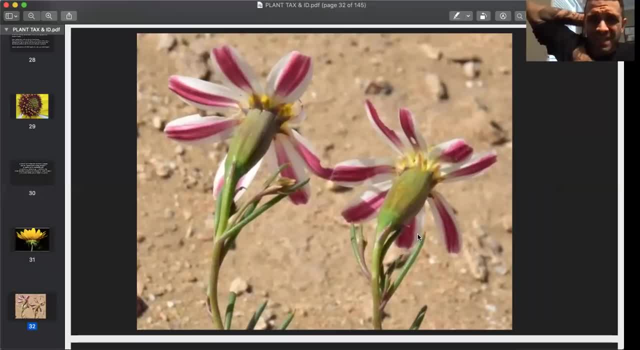 and i'm going to show you a little bit of the flowers that i've got here and i'm going to show you marigold tribe and it's also got these really bright colored and other species in nicolettia do this. have these really bright colored? uh, ligulit, ligulit, uh flowers, ligules, the kind of candy cane. 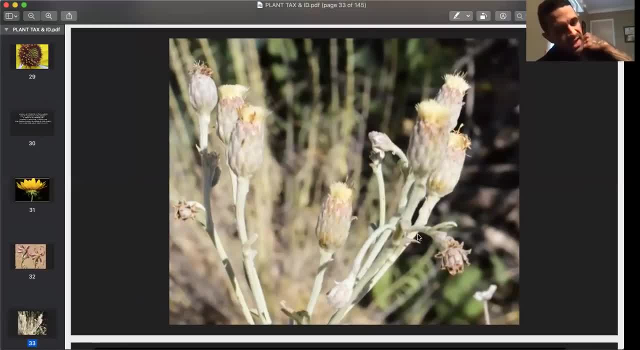 thing, vernonia larceniae. this is from near sanderson texas. this fucking thing. you know vernonia, aka the ironweeds. you'll see them in the midwest, you'll see them on the east coast. they're, they don't look anything like this man. they're fucking crazy. they're really. 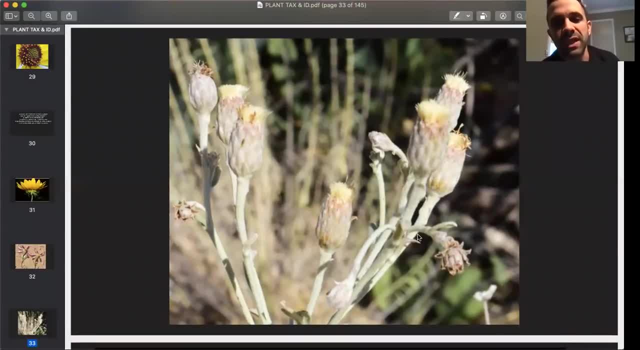 brightly colored. the corollas are like bright magenta and they're green and they got leaves. this thing almost doesn't have any leaves. the leaves are tiny. it grows in the desert. of course, if you live in a desert, you don't want to have big surface area leaves to transpire all that. 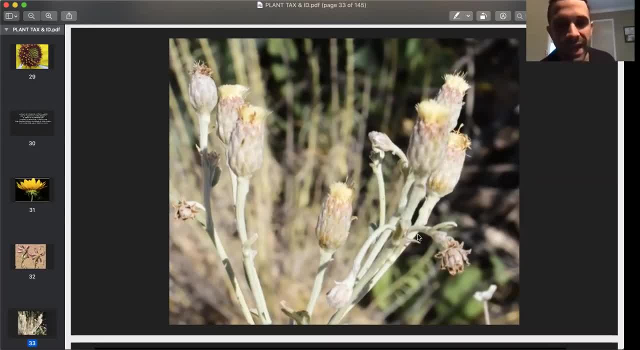 moisture, you're going to reduce your leaves. you're going to eventually evolve white hairs that cover them. uh, this is a pretty rare plant. it's from northern mexico and south texas in the chihuahua desert. when i saw this, i was fucking stoked. i got a bunch of seed of it and then i 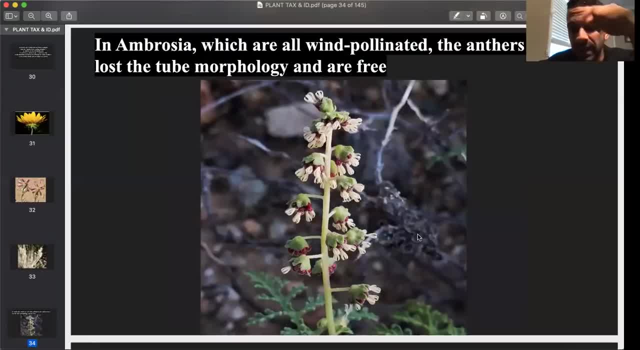 fucking lost it because i didn't miss, i didn't label it, so anyway, go back. already went to this. the ambrosias, some of the ambrosia. this is ambrosia camperata in in serpentine and this is a relatively rare plant in baja california, sir, ambrosia trifida, if you live in texas, uh is an annual that gets. 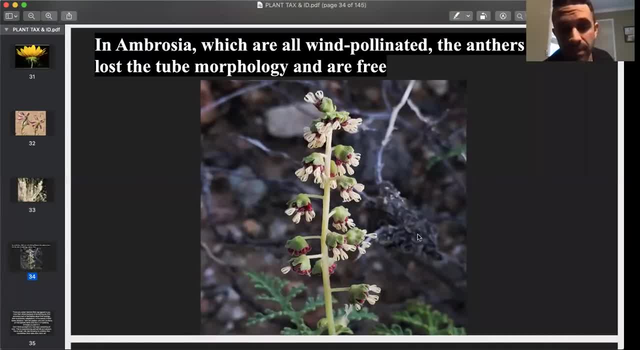 upwards of 25 feet tall in a single season. i mean, it's like fucking bamboo, it grows so fast. um, but the same flower structure, the same flower structure, different leaves: trifida, because it's those leaves, but it's definitely a plant, you know, it goes unappreciated because it causes. 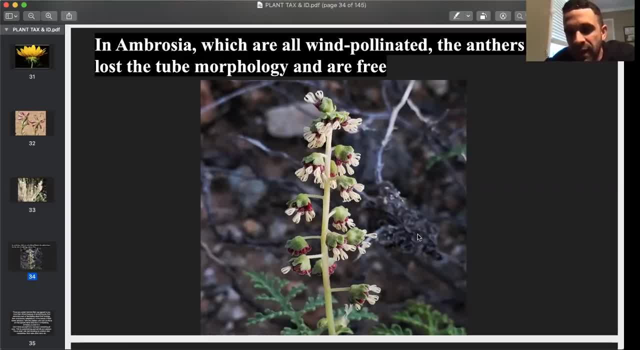 hell for people with allergies, and it's just a roadside weed, uh. but here in north america, where it's native, it's a plant you gotta, you kind of got to give some respect to, because it's so ecologically dominant and, uh, you know, they're sure a lot of things munch on it too. so anyway, 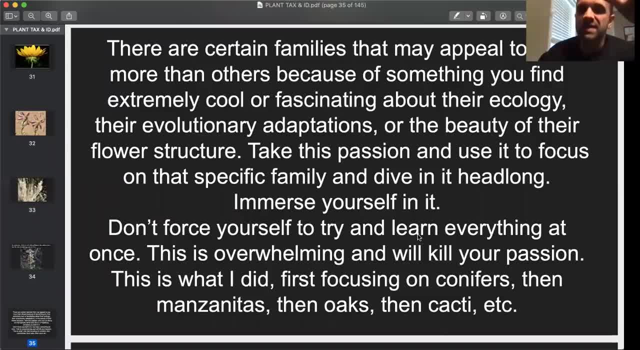 we already talked about this- certain families. this is how you really get into it. don't just try to memorize all this shit at once. find something you're you find really cool. say it's saguaros. say it's fucking sunflowers- probably not going to be, but most people aren't taking the sun, but you know. say: 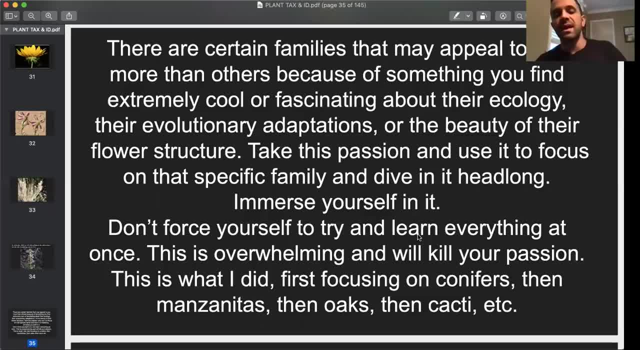 it's a uh uh members of the four o'clock family or say it's like the mustards, like they're really weird. the fact they grow in all this fucked up soil, uh, is odd. you and you just roll with that. just focus on that. don't try to learn everything. focus on that. you'll get stoked about it. you'll. want to know what are the different variations on a mustard or the different variations on a columnar cacti? for me, when i did this 12 years ago, it was conifers and it was cypresses. i was like this is so weird, the way that california cypresses grow there's, you know. 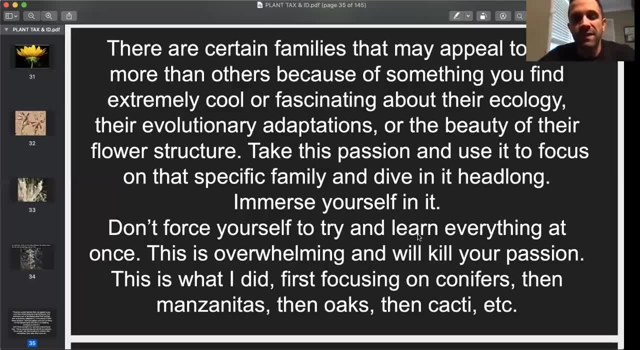 a lot of them only grow in these small geographic areas, often on really fucked up soil, and if you go to an area where there's a cypress growing, uh, there's also probably going to be a lot of other weird endemic plants, rare plants too, so that and then that kind of you know i'd be in the cypresses. 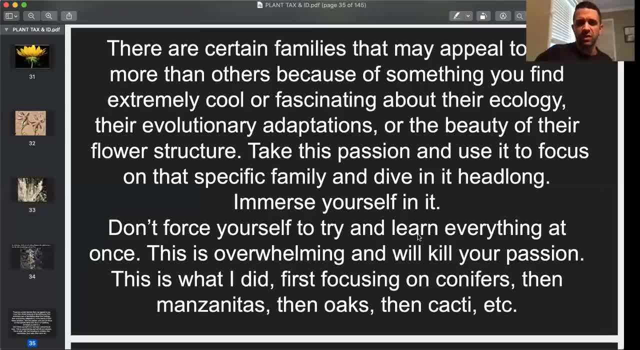 i'd kind of nail them down. then i'd be like, oh, this other thing that grows with them is really weird too, huh. and then i'd look a little bit closer and just have my mind blown and get so plus again, pleasant distraction from the fucking harsh reality of the modern day. just 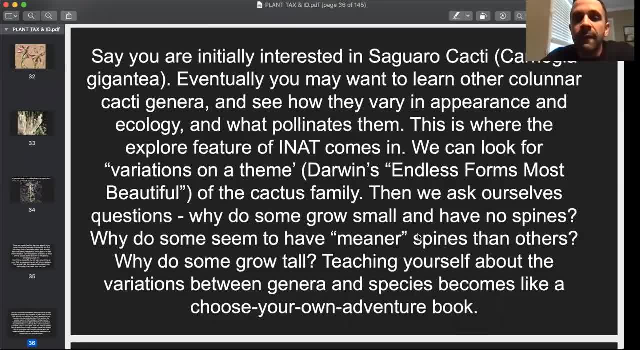 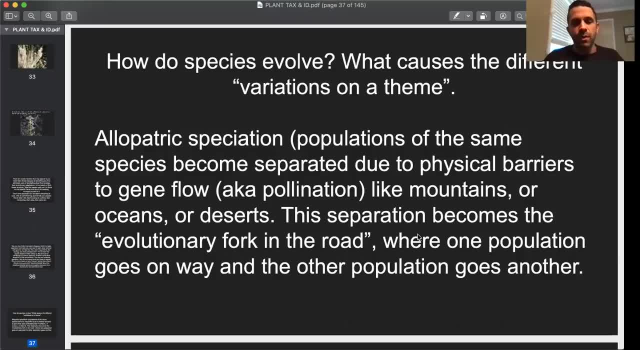 studying life. so, anyway, it's more what i just said. uh, so how do species evolve? is everyone people getting too bored, or is this good or what? you want to just look at some plant photos or what? okay, all right. uh, there was like a california answer. it was like it's cool, but it'd be cooler. 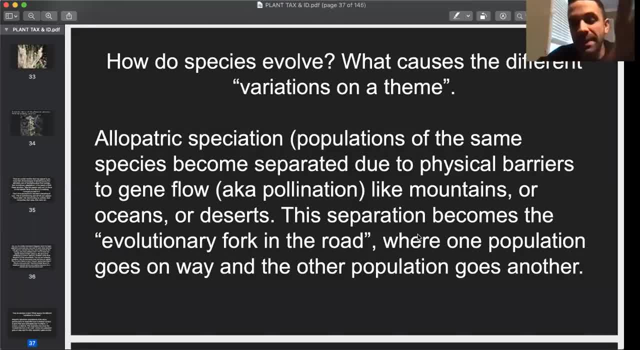 if it was no offense, but i'm just saying, if you want me to look at photos, we can go to photos, but this is the how species evolve is pretty fascinating too, um, but i'll try to speed it up a little bit. so how does species evolve? how do you get these? 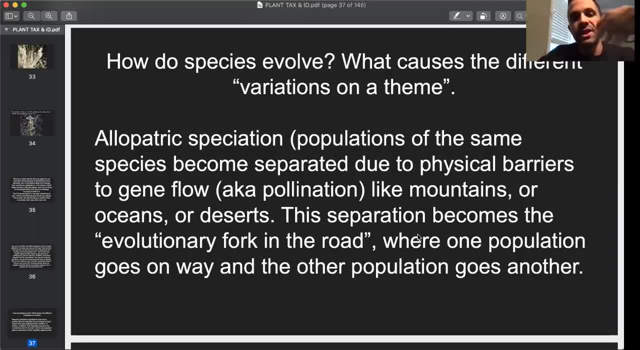 different variations on a theme. uh, you get allopatric speciation and sympatric speciation- allopatric is the most common species- becomes separate. a population becomes split in two by a mountain range or an ocean or a desert or whatever. uh, sympatric speciation, a population is. 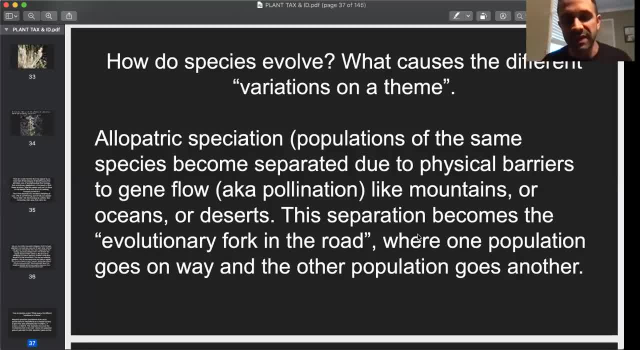 population is, doesn't get split into it, doesn't get geographically separated, so you get a different pollination time. they evolve a different phenology. this members of this allele. this allele arises and it causes these individuals to bloom in the spring and these individuals to bloom in- uh, the fall, the 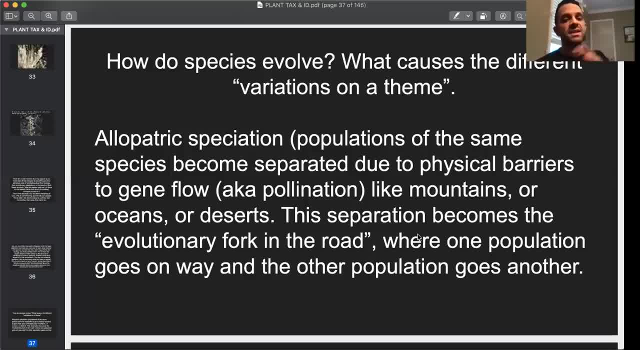 idea, though, is you get a a decrease or elimination of gene flow between the two populations. okay, so you're not exchanging genes and alleles anymore. you've got two different uh populations, and those eventually evolve into new species. okay, but vicarious barriers like mountains or oceans, or 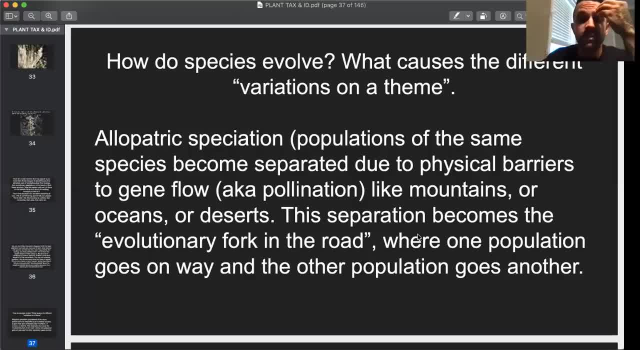 deserts. that's the common way that uh things speciate. but you can also get dispersal events, as happened with the hawaiian silver swords and the tarweeds. so hawaiian silver swords are most closely related, the plant they're most closely related to on the mainland. 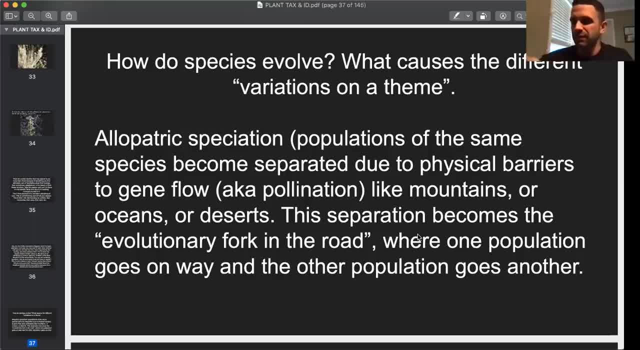 are the tarweeds, these like weedy little really glandular resinous. they're called tarweeds because they're sticky as hell. i think they smell good, but again, that that the that resin. they produce those really sticky glands, almost like cannabis. the point of that is to prevent things. 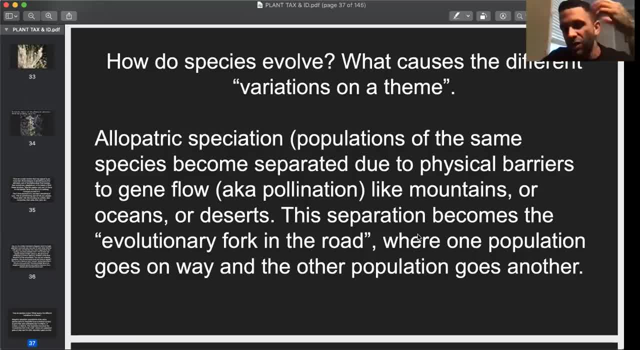 from eating them to get bugs stuck to them. whatever you know, the bugs will crawl in that and they'll get stuck, can't move right. so that's a really good adaptive trait to you know: keep yourself alive so you can produce offspring. so they at some point. one of these seeds, or maybe a few dozen seeds, got brought to the hawaiian. 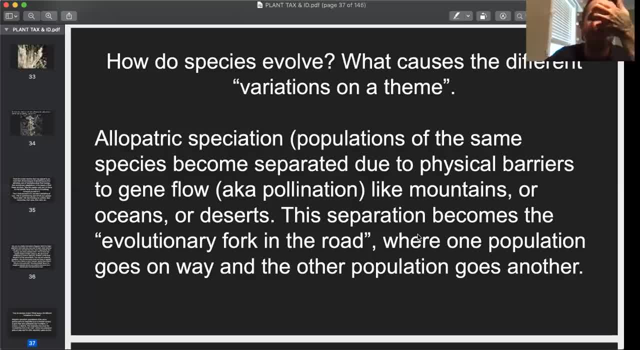 island archipelago, and you can actually. we've actually dated this at five or six million years, looking at molecular clocks, which is a whole other concept to get into, but a really cool one. if you have time, you should try to teach yourself it. uh, five or six million years ago, one of these seeds- 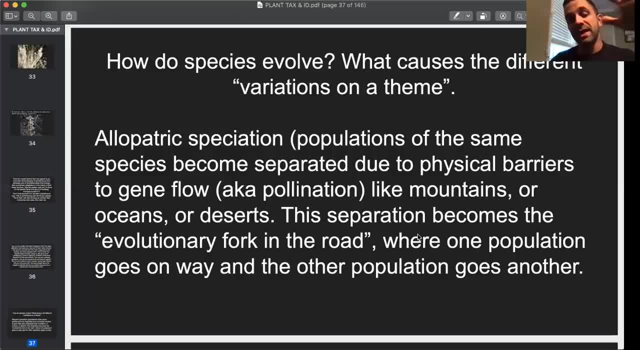 got brought to the hawaiian island archipelago and because of the way that plants speciate on islands where, uh, you don't want seeds that are not going to be able to grow and they're not going to do anything, just an pencils spots are consuming more seeds, or one of the reasons why so much. 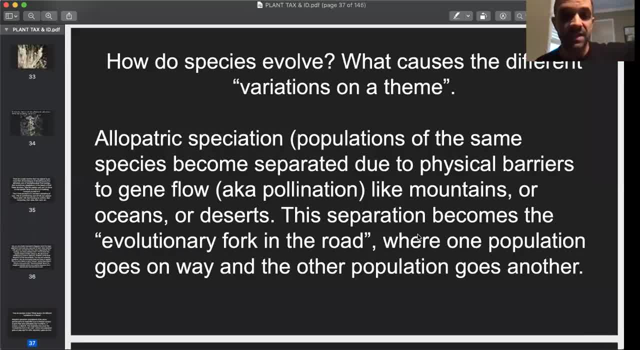 of this in one of the centers in Berkshire place are going to be to destroy those seeds- and there's only a large number of edible seeds that might get this thing- and you put them in their- that's going to be, you know, will hold up for better or worse, you know. 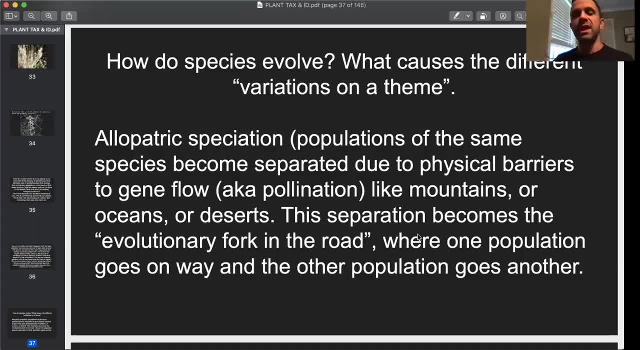 bit like any other weed rinsed from the center of the home. vitamin c readings, all the other belt leukamistoplavin and they you know, but this unit it. it's really hard to test and mutation might get. that's a big red flag, a big flag to herbivores. They'd gnaw it down It. 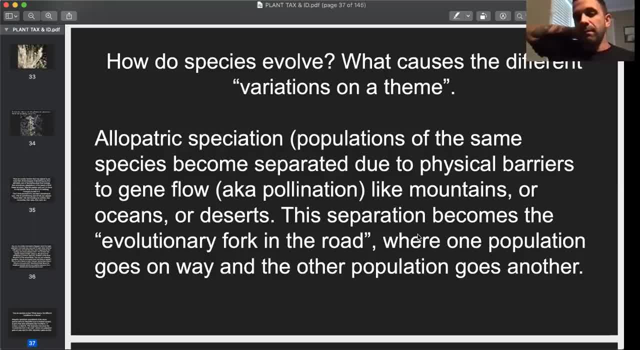 wouldn't survive. But on an island. you know there's benefits in growing big too, because you can make more nutrition for yourself, You can more service area to photosynthesize, You got more carbohydrates stored, So that what was a maladaptive trait- to get big and you know- become 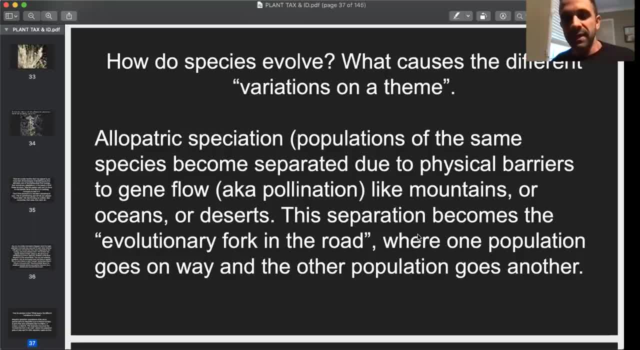 noticeable to herbivores on the mainland is now an adaptive trait on a on an island because there's no herbivores. So now these things grow bigger. The ones that don't grow as big over time just kind of get filtered out. They don't make it. They don't produce is what they're not as successful. 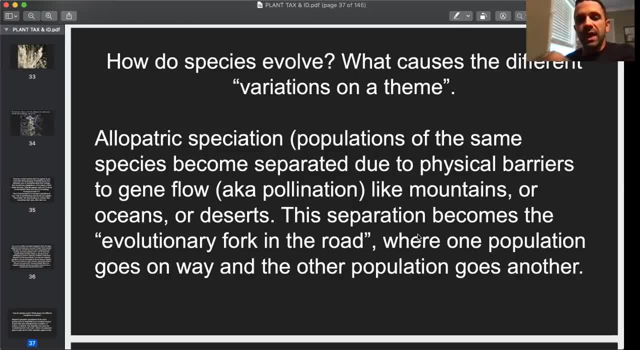 So from this tiny little fucking roadside weed that grows in California evolved this thing that lives now lives 30 years. Most tarweeds are annuals. They only grow for four or five months, produce a ton of seed, then die. Evolves this thing in Hawaii that can live for 30 fucking years. 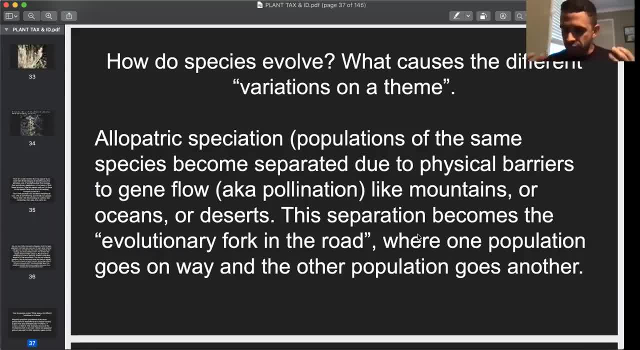 get eight feet tall in some cases, has these like really bright blue fuzzy leaves, grows on tops of volcanoes at high, high altitudes and just looks nothing like the thing that it evolved from, And it's immensely successful on these volcanoes where it grows It's you know. and how long did it take? 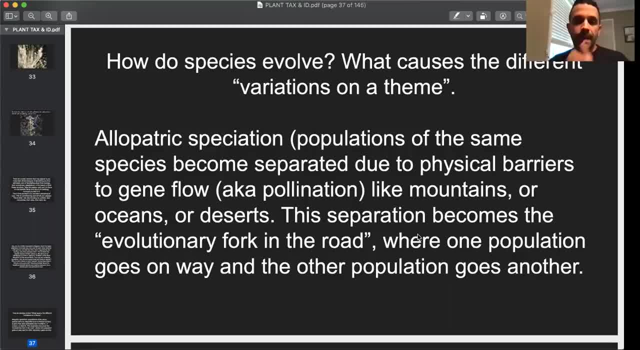 for that to evolve A few million years. whatever You know, this is the. the idea is you get this evolutionary fork in the road, the separation of two populations, And it can be because the seed was dispersed by an animal, or mountains arise, or continents separate, plate tectonics, et cetera. 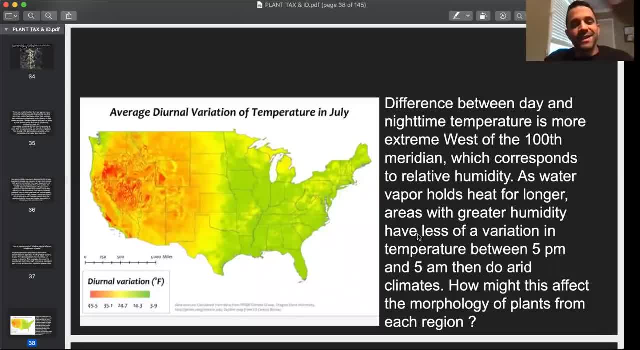 This is fucking unrelated. I just thought it. I just thought it was cool. This is why a lot of plants out West will be fuzzy And a lot of plants in the East will not. they'll have green leaves with few hairs on them, And this is because of this. this is a, this is a factor that causes. 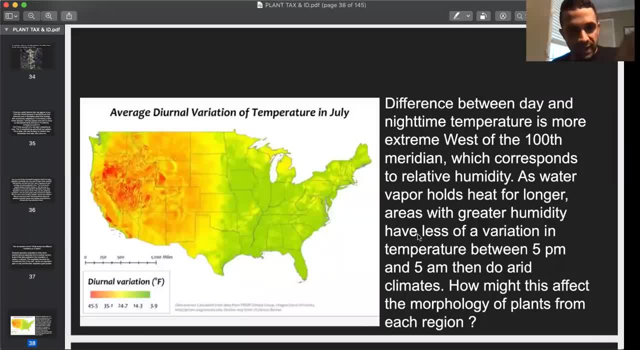 that is, you get much more humidity East of that hundredth Meridian, which you could see running through central Texas, where it's greener, And that's what causes the diurnal variation in temperature. The diurnal variation in temperature corresponds to humidity, because 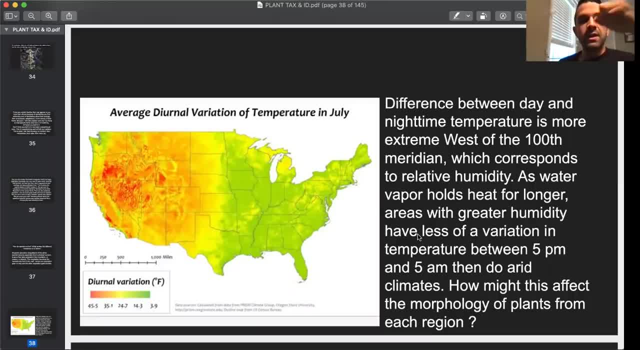 humidity. water vapor holds heat longer, So you don't have much of a variation between day and night in Florida in the summer because there's so much fucking humidity You could practically spoon into your lungs. You know it's not going to change that much. You might get 10, 20 degree. 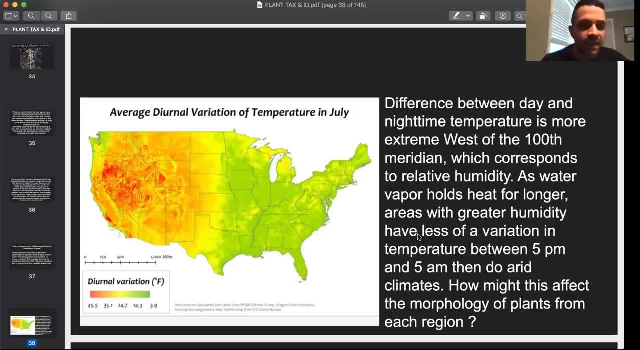 difference. but you go to the desert, go to like death Valley It'll in the summer, obviously it's a fucking 115 degrees. In some cases it'll cool down to sometimes the upper seventies at night. So you've got like a 45,, a 35 degree variation in temperature. 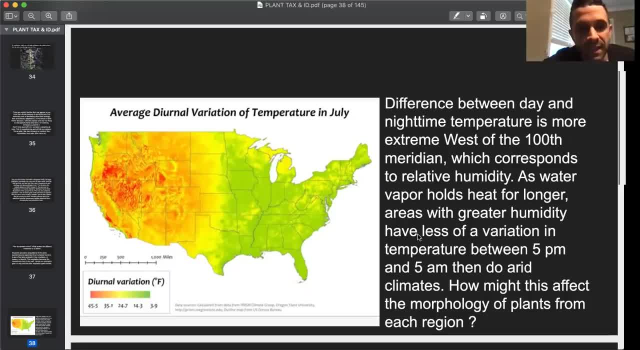 in some cases, much more. you know, and this is something you get in Highland tropical areas too, like Mount Kenya. where you're at, you're getting the full brunt of sun. You're at zero degrees latitude, but you're getting the full brunt of sun because you're at 17,000 fucking feet. 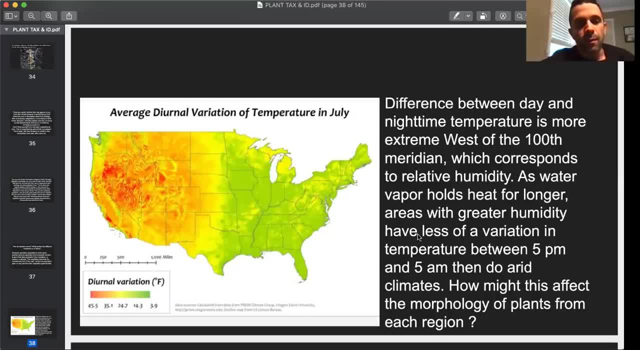 elevation. So it will be. it'll get upwards. you know what? I've never been there. but say 70 degrees during the day, then it cools down almost below freezing at night. I mean that's a huge stress on plants. 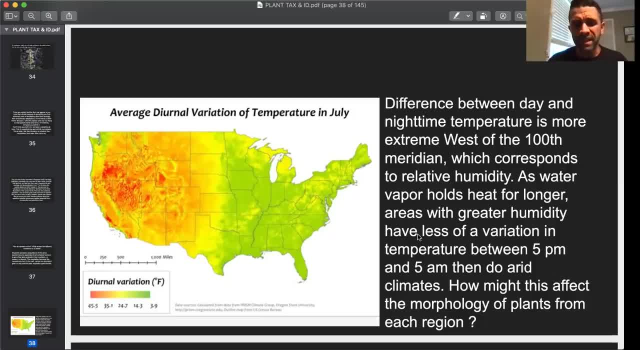 but again, evolution being what it is, they adapt. So you know same thing in like Columbia Highlands, I mean, you just get wild shit that happens. but also knowing this and how plants respond to this effect, this diurnal variation in temperature as well as humidity, you can see a. 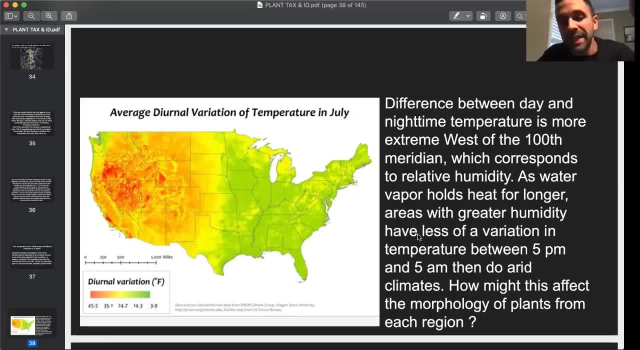 plant you've never seen before, And if it's blue and it's got fuzz boom, you know that plant is from a dry, uh, arid environment. It doesn't matter if it's Australia or South Africa or or the, the deserts of Northern Africa or whatever. I mean, you could see that and be like 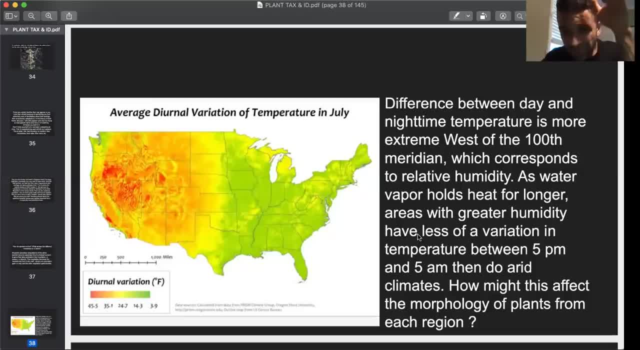 wow, that's. that's from a dry climate, Really fucking cool, Cause the, the moistures or the, the those hairs keep that moisture in. they keep the ultraviolet radiation from battering, uh, the leaf tissue. and getting the leaf tissue too hot Cause it, you know. 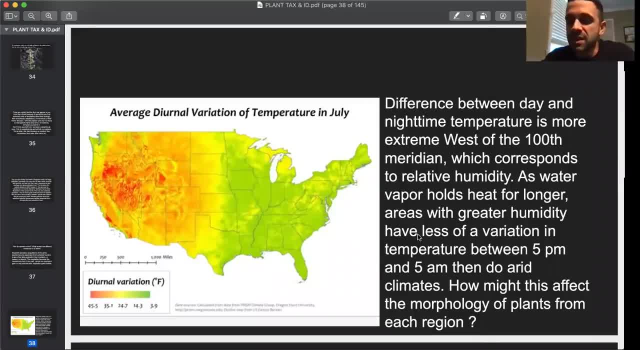 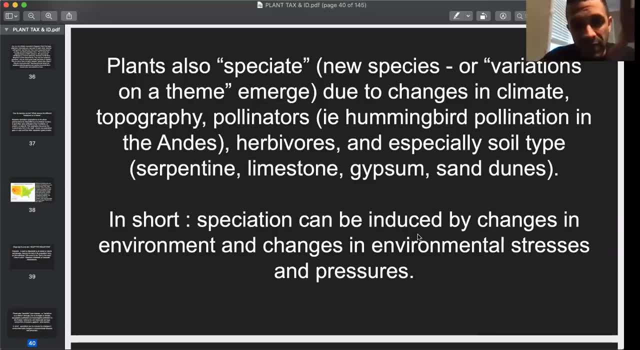 at certain temperatures, photosynthesis shuts down. So, uh, just another cool thing to pay attention to. dispersal events already already talked about that, And this is my favorite shit. This is what I'm really into. plants also speciate. Oh, this isn't nevermind, These are just different factors. but at the last one, 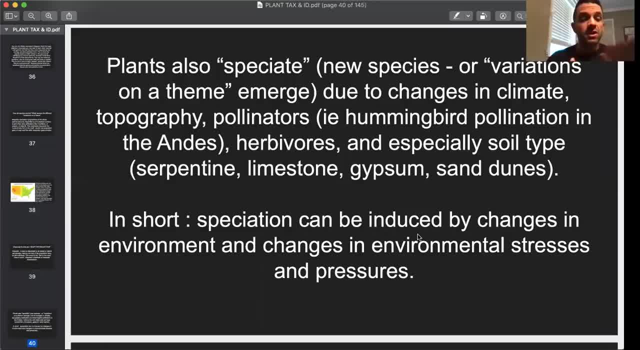 the last factor here, especially soil type right Can cause plants to speciate. You got serpentine, limestone, gypsum, each of these soil substrates And this is a. this is what's fucking cool, Cause this shows you how much geology affects evolution of plants. 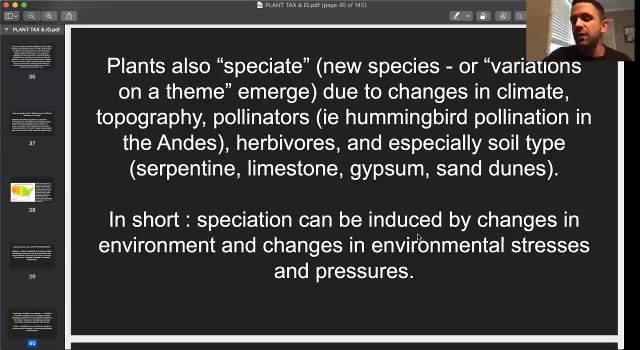 Things Most, most people don't ever pay attention to. when I see a new plant, Anytime I'm in a new habitat, I I try to figure out what the rock is. you know, and you only got- I mean crash course. 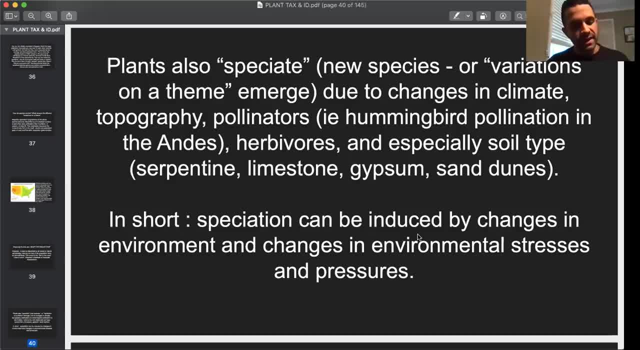 in geology you only really got three main different types right: Igneous: Is it volcanic or is it like granite? Did it cool from a magma, or is it metamorphic? It was, uh, altered at some point, ie cooked either by magma or by being buried at really great depths, or was it sedimented? 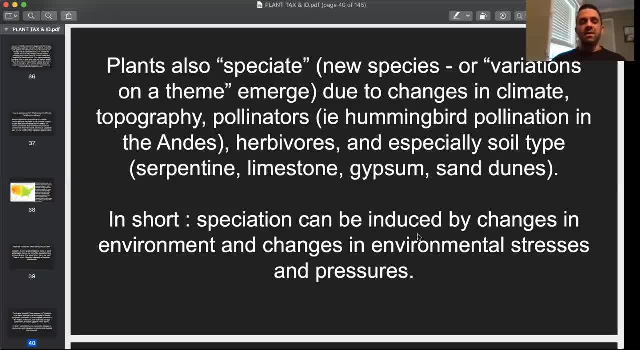 You know, if it's sedimented, it's all. sedimentary, you know, just sediments accumulating over millions of years, like limestone or or sandstone, et cetera. So these soil types, you know, or dunes, in the case of dunes, can affect how plants uh speciate and evolve. 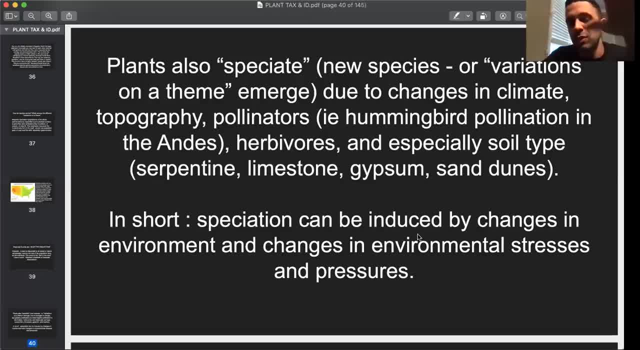 So you'll go to areas that are. the geology is gypsum. You only find gypsum endemic plants there, or plants that can tolerate it, but the gypsum endemics you won't find growing anywhere else. you know, and to see what effect that geology has on plants is fucking mind-blowing. 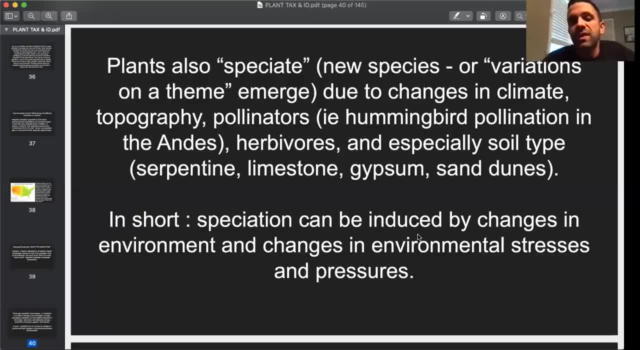 and really cool. so, uh, in places with uh more homogeneous uh geology- and i can see too much of this- you know, like in the midwest growing up, it was always it was all limestone and that limestone was buried beneath 40 feet of topsoil in some cases. i couldn't really study it as a kid. 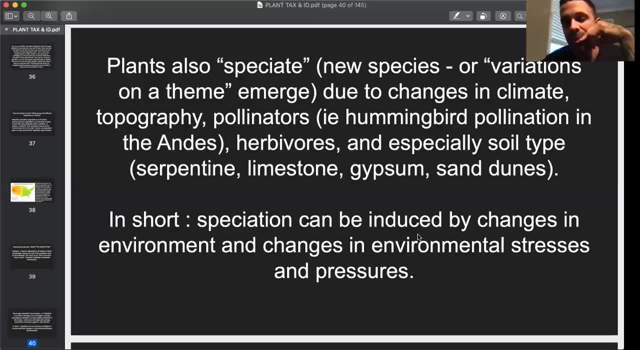 or pay attention to it, you know, unless i was driving by a limestone quarry. but in places with more diverse geology, you notice the stuff and it's you'll start to notice the differences, man, you'll pay attention to start be able to figure it out. so we'll go, we'll roll through uh. 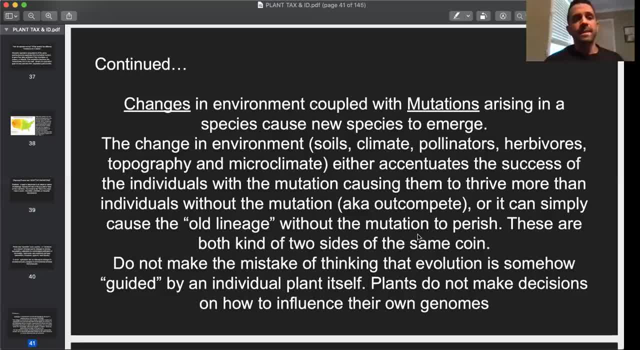 one more fucking slide on this. okay, go ahead. geology: what's the geology app that you mentioned a few videos? videos ago, you got i naturalist and then you got geology app that connects you to papers on your area. oh yeah, rocked r-o-c-k-d. yeah, okay, it's a, it's a geologic, it's a usgs overlay. 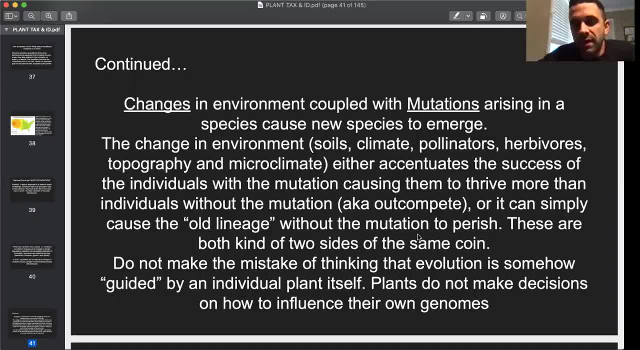 like a geologic map overlay of wherever you are. that's a good thing to have too. it can be buggy sometimes and frustrating, but overall it works out pretty good. um, you know, does that? does that only work for the united states? no, no, i used it in mexico, i used it in australia. it depends what their source of information is. you know, in some 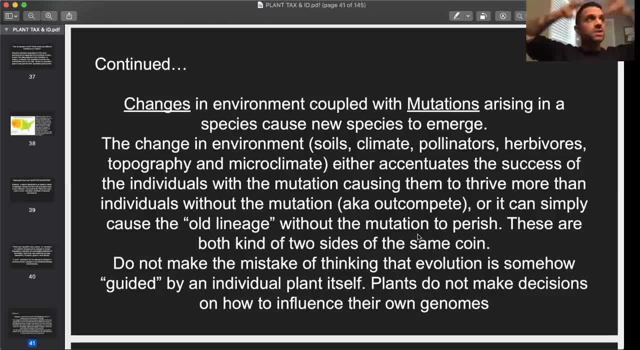 places. it's really general, like when i was in mexico. you had these huge areas that were actually quite buried, but the whole area would be grouped, as you know: cretaceous metamorphic rock lake, cretaceous metamorphic rock right, whatever. not very helpful, but in some areas, you know, it's really. 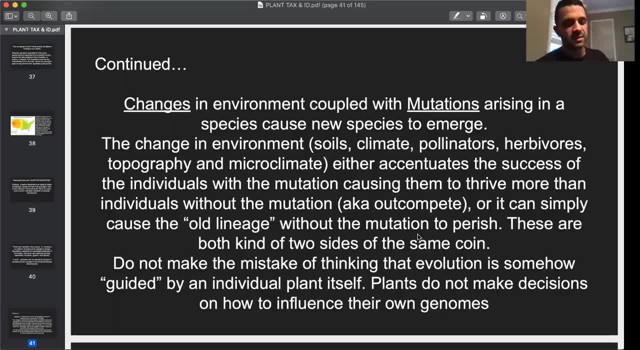 really uh, you know, like in texas, some of it's like really these maps. each different type of rock is color-coded on the map. it's really helpful, i mean, you can see, you know it's. it's really uh articulate, in other words. so that's a good one to have too. and then if you want to learn geology more, i mean 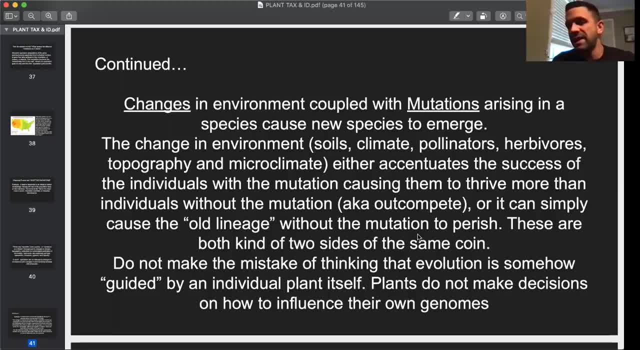 the easiest way to do it. yeah, you could read john mcphee books, you could do whatever, but really the easiest way to do it- john mcphee was like a pop science writer for me and he was like i'm going to, but the easiest way to do it is really just, you know, watch geology videos. uh, you know and more. 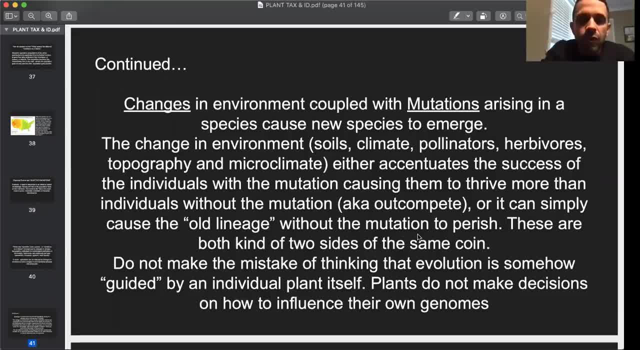 importantly, get like a used geology textbook. like geology overall, unlike plant taxonomy, has not changed that much in the last 10, 15, 20 years. so, uh, you know you get an old geologic textbook. you can find them probably online: 10, 20 bucks. you could download them on libgen. essentials of 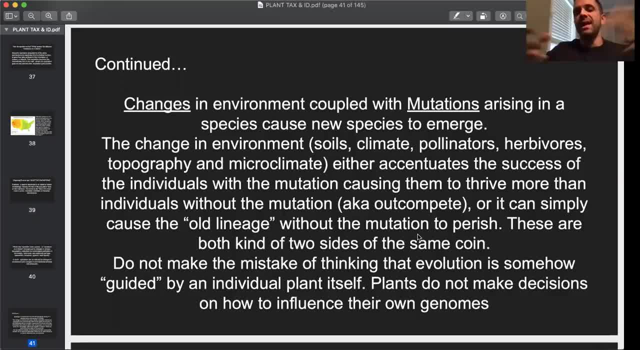 geology is a good one. you don't have to take the whole thing in, just get the base elements. now, one of three different types of rocks. how do you pay attention to it? okay, you got igneous, and then subcategories of that igneous- you know, cools from a magma. you got extrusive igneous rock and 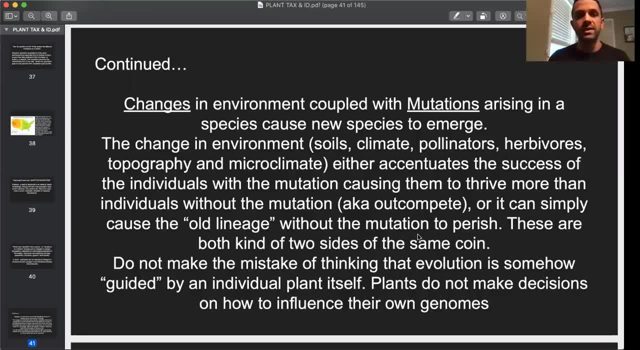 intrusive igneous rock, right. well, how do you? how do you tell which is which? by looking at the grain size, aka those crystals, the shimmery bullshit, as i call them in my videos of like basalt, like basalt. you look close and if you see little shimmering, those are the crystals. that's the. 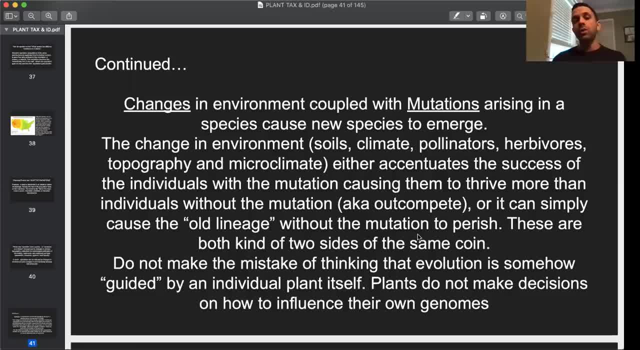 grain size. the crystal grain size, uh, and that cool. the reason those crystals are there is because it cooled from a magma. that cooled relatively fast in the case of basalt. they're going to be small if it cooled over a few million years in the case of granite. like you go to joshua tree national park, 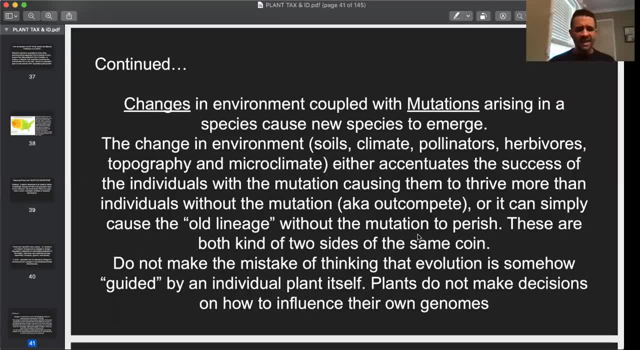 these are the geology there. uh, is these massive granite plutons, these masses of fucking rock, the whole? you know, the whole area was a mass of rock all relatively similar in, uh, in chemistry that cooled immensely slowly, like over millions of fucking years deep underground. because it cooled so slowly. 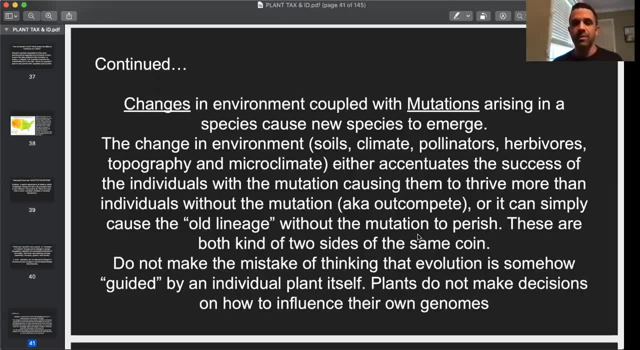 there's a larger grain size. those crystals had time to grow. you know, like if you make rock candy, it takes time for those sugar crystals to grow. so the longer, the more time you give it, the more homogeneous conditions you give it, like temperature and depth. for a longer amount of time, the bigger 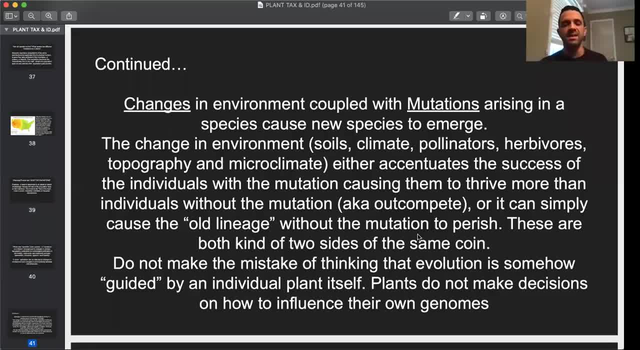 those crystals are going to grow. those gypsum crystals in that cave in mexico were at the conditions like 58 degrees celsius groundwater. they pumped the groundwater out to get in there, but it was 58 degrees celsius groundwater really. uh, gypsum and and sulfate rich groundwater- that, and it stayed like that for. 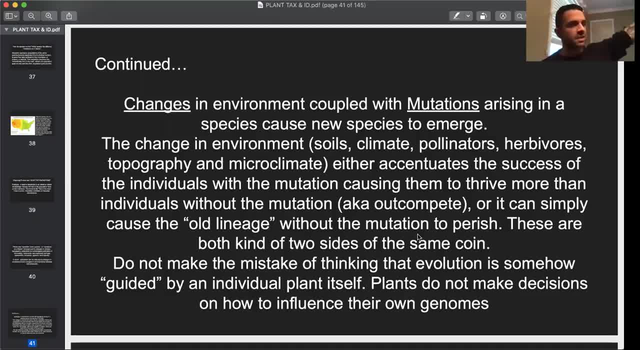 estimated like 500 000 to a million years, and that's why those crystals are like 20 feet long in some cases and eventually, when you know, people abandon that cave, it'll fill back up with groundwater and theoretically they'll keep growing. so, um, anyway, that's igneous rock, sedimentary rocks. 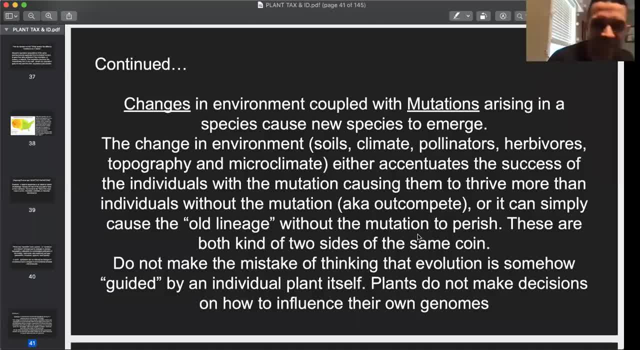 i mean same. you just learn the look of it. i know that sounds ridiculous, but it's not ridiculous. but you'll see a sedimentary rock like a sandstone and uh, you'll just eventually learn the look of it. but you always gotta check, you know. am i right? is this wrong? what is this? just ask questions. 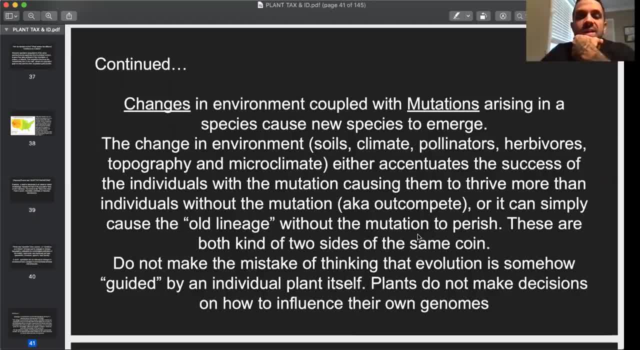 so, um, so it's, it's, it's ch what causes speciation changes in environment coupled with mutations. so this is the thing that the changes. things always mutate. you know, uh, we see this in the fucking coronavirus. there was a mutation, uh that occurred that made it more contagious. boom, so that that. 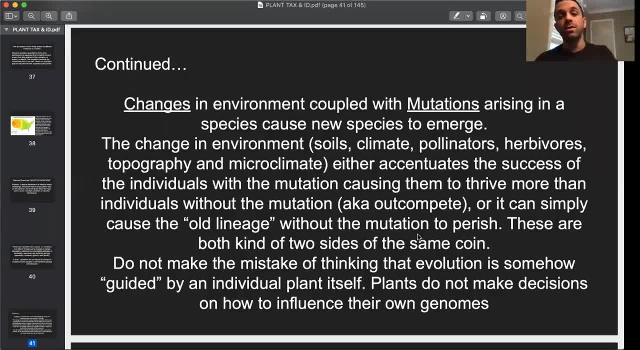 makes the individual's viral particles with that mutation and makes them more successful. okay, As viruses progress, as they evolve, they tend to get less lethal. Why? Because the ones that kill their host immediately, before they have a chance to spread, they're not going to thrive. 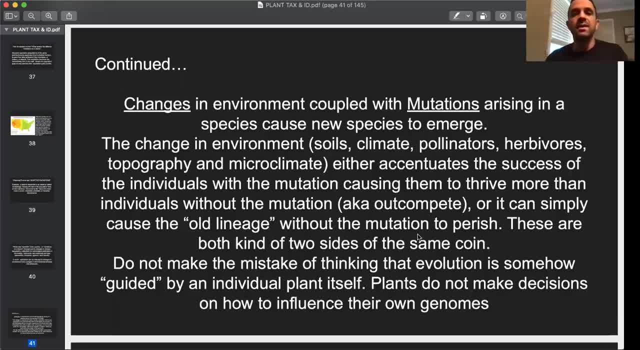 Those aren't going to make it If you kill your host immediately. this is why SARS-1 didn't make it that far. you know It wasn't. it was cases were symptomatic and it killed people. It had a. 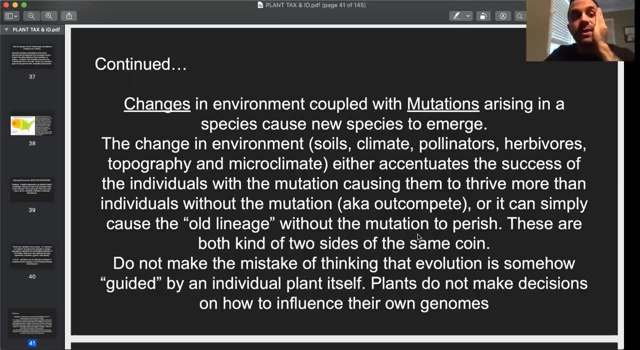 higher lethality rate. You know, the adaptive benefits for COVID are that it can lay dormant- and not dormant but asymptomatic- and it's extremely contagious. If COVID kills more people, that's not an adaptive trait. Your host dies. You're using your host as a viral factory to 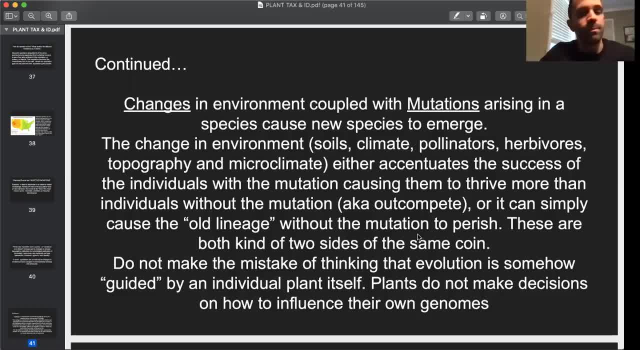 produce more viral particles. You know you don't want that. You don't want to burn down your house, right? So again, it's not, don't anthropomorphize, It's not benevolence of the virus, It's just the way. 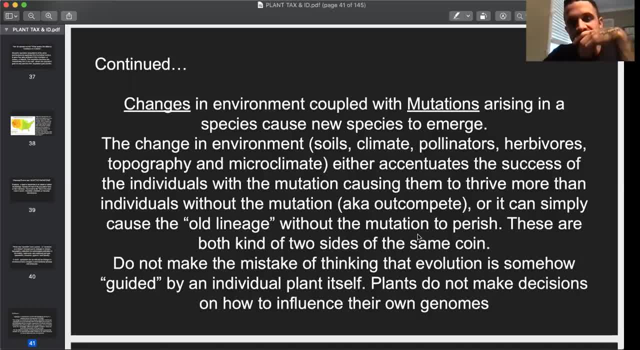 evolution works. So you know these mutations arise. Same thing happens on a more macro scale with with plants. Mutations will arise A certain you know. suddenly you get a flowers or a species that mostly produces purple flowers. Suddenly it produces white flowers. okay, Say the pollinator. 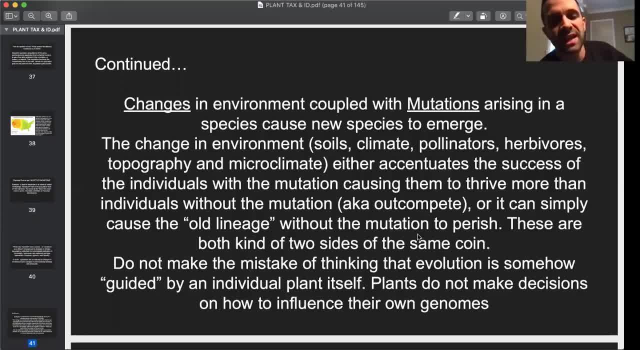 something in the environment changes, The pollinator that pollinates those purple flowers gets knocked out. Now you've got a pollinator that pollinates at night. Say it's a. a pollinator that pollinates at night is not going to see purple flowers, right, So it's going. 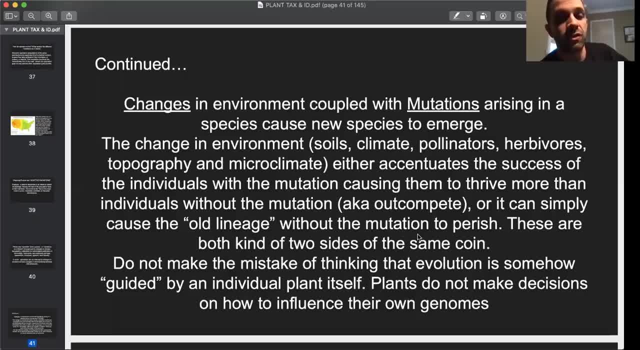 to stop pollinating them to such a large degree. But you've got these mutants. It's a recessive allele, say, but these mutants produce white flowers. right, White flowers stick out like a, like a fucking sore thumb at night when everything's dark. So that's going to cause. 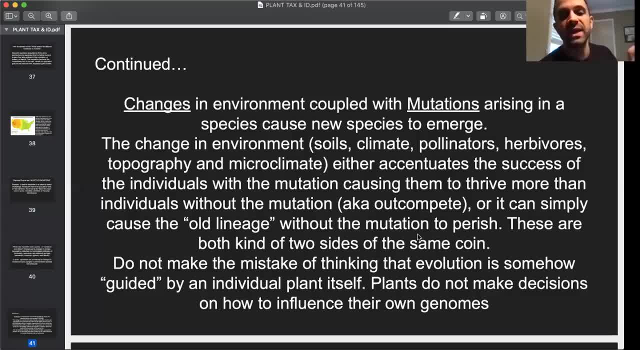 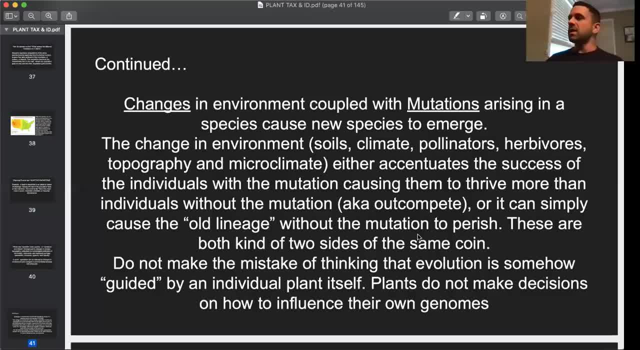 they accentuate that allele for white flowers. So a couple of generations, maybe a thousand, 10,000 years down the line, that species doesn't produce purple flowers anymore. I mean that allele has been filtered out. It's mostly producing white flowers, And this is the really. 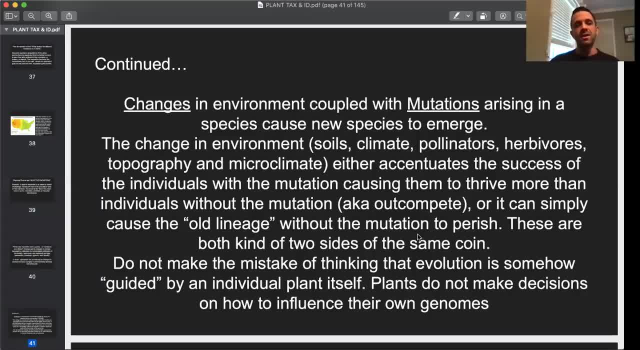 cool shit. I mean when we kind of have decoded how it works. you're mixing Mendelian genetics with Darwin's theory of evolution And now we have DNA to look at how this stuff happens. We can measure it, which also makes the fact that there's still people that deny evolution fucking. 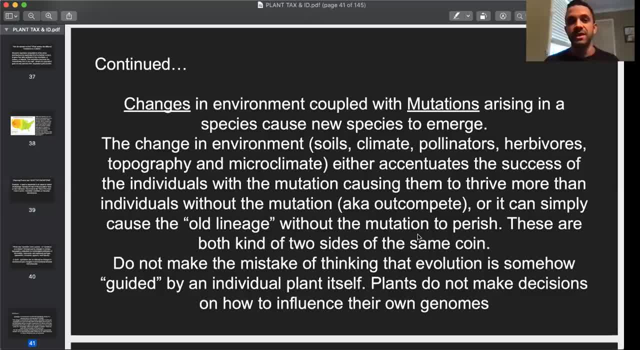 saying that belief. I went to, like the the evolution denier museum in Texas. I fucking had to go, didn't pay to get in. Uh, I wanted to do a video there, but it was kind of weird, Cause I'd. 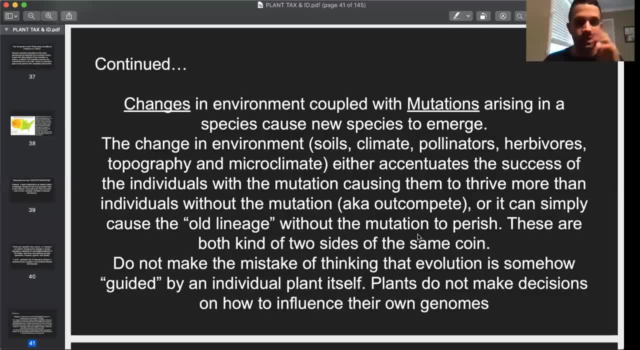 be like blatantly making fun of them- and they were right there, you know. but it's just. I mean, we can see how this stuff works. It's like looking at the gears of a clock and seeing how it works And then you've got someone telling you that the clock is false. It doesn't, it's fake, It doesn't. 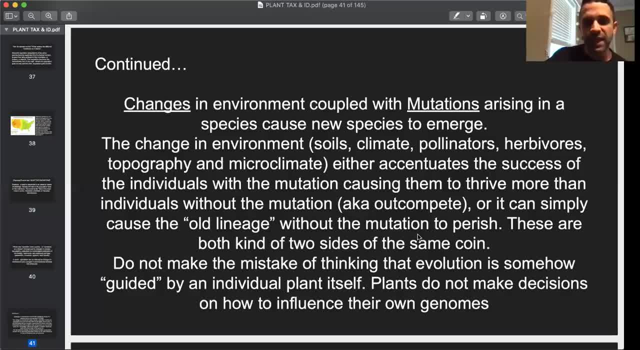 exist. So, um, anyway, cool shit, Any questions. I had a. I had a question about that, Like. so this is something that I struggle with, kind of on a moral sense, I guess. but speaking of like, invasives, like, do you think that plants that are being impacted by 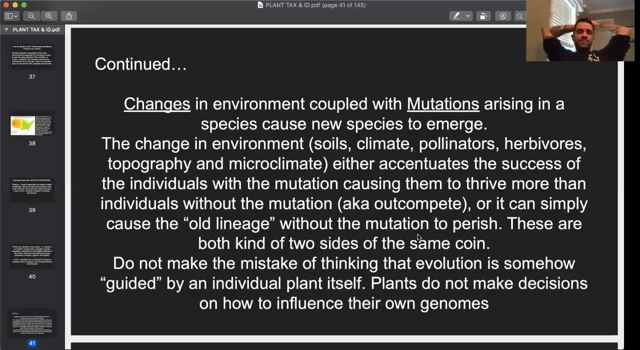 by humans are going to evolve in similar ways in response to the impacts that humans are making. Or do you think that we're moving so fast, fucking shit up- that the plants won't be able to to adapt? Like will some like will the, the invasives of today, eventually diverge and 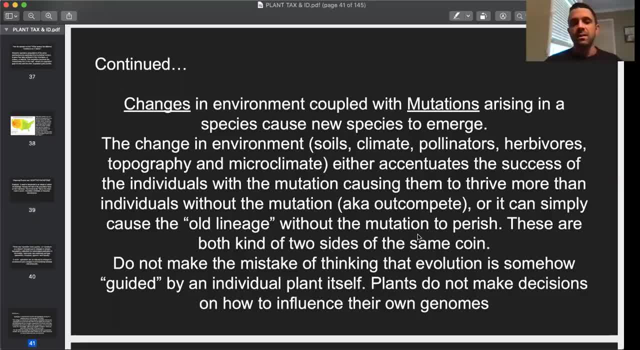 become natives on a, on a geologic timescale. Yeah, that I mean. another way to think about invasive species is they're just dispersal events. So, but dispersal events have never happened at this rate before. There have been hundreds of thousands of dispersal events of both plants. 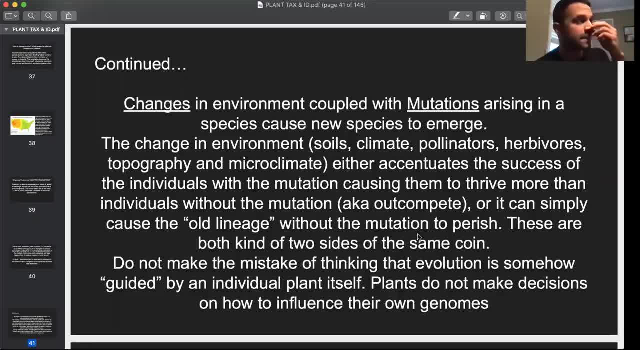 and animals and fungi and and insects. insects or animals, uh, in the last hundred years That's never happened before. I can't think of a case in which that's happened. Normally dispersal events will get one. They're very rare. 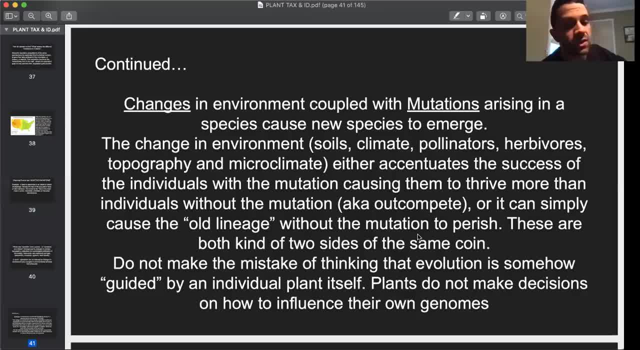 You know they're very rare, much more rare than this. They occur, but they're much more rare than this And because of how slow they are, the ecosystem has time to adapt. There may have been dispersal events- five, 10,, 50 million years ago that occurred, that that caused extinctions. 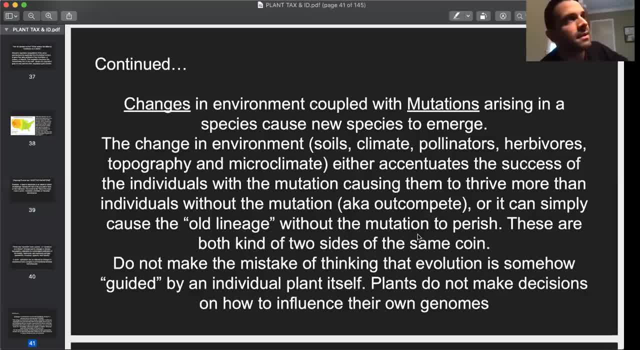 may have happened. We'll never know. Okay, I mean it's, it's thought that you know when, when dingoes arrived to Australia, to the mainland, that's what caused the extinction of the Tasmanian tiger, which isn't a tiger at all- uh, long before people got there. 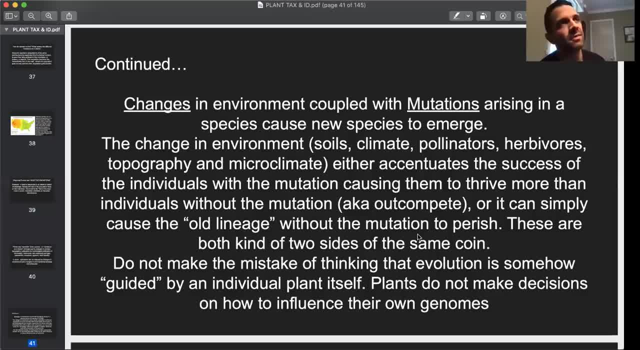 you know it's. I don't know. I maybe it was, maybe people did bring dingoes, I forget, but maybe the aborigines brought things. either way, The idea is: is there, you know these dispersal? 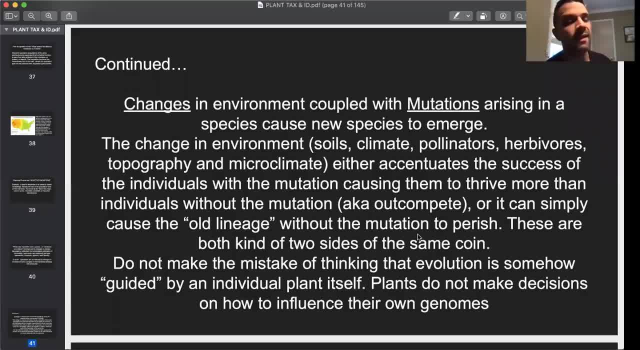 events happen, but they were somewhat. they were rare compared to today. So will these things evolve if we go extinct? Well, yeah, they will, but they'll cause a lot of extinctions. I mean, this is what this is. the idea to get across is there will be species that go extinct. 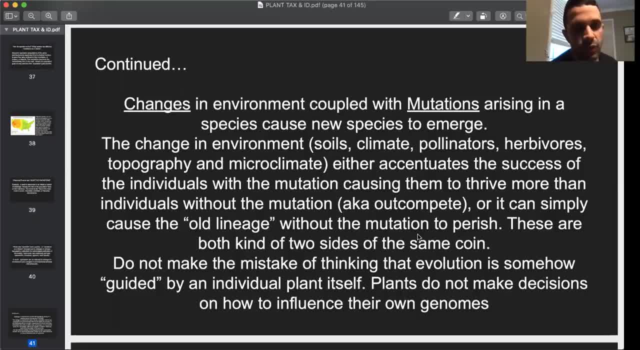 even with proper management. uh, due to invasive species. I mean, they just they don't have any checks and balances here. You know every- I always say this in my videos- to every fucking tree disease we have that's causing decline in a tree species in the United. 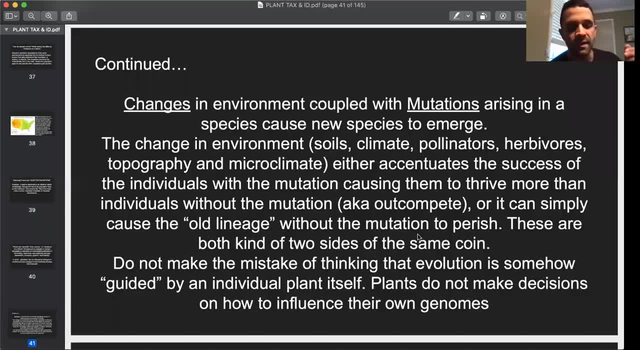 States, is an invasive species, It's an invasive insect, It's an invasive fungus, It's. it arrived here, Doesn't have any checks and balances, because it didn't evolve in this ecosystem. It evolved 8,000 miles away. And you know, over time, uh, things get checked, you know. 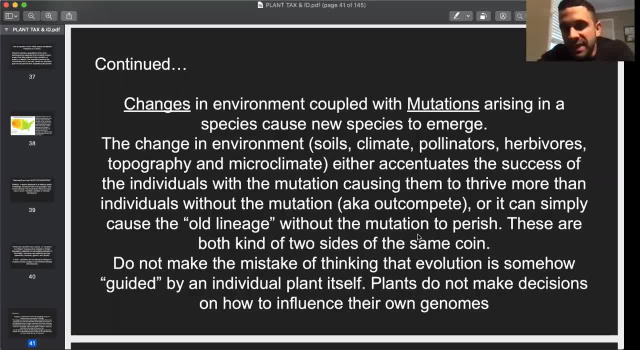 checks and balances right, There will be a far a bacteria that ends up, you know, checking that fungus, or there'll be an animal that ends up checking that insect, or there'll be an insect that evolves- It ends up evolving- to check that plant, but it takes a long time, And also you. 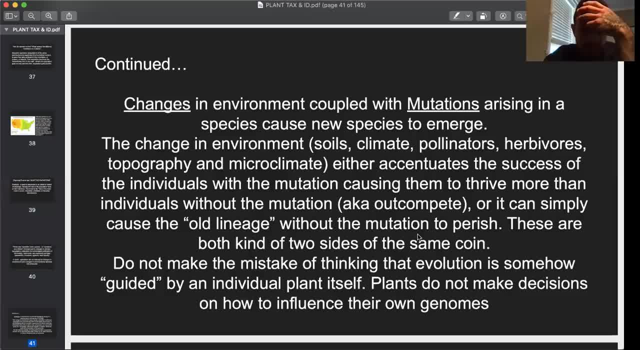 know, habitats carved up by people now, but uh, you know, in the meantime what will happen to the rest of the ecosystem. Things are going to go extinct, You know. there's just no way that they can't. I mean, when you see monocultures of uh, Saharan mustard in the market, you know. 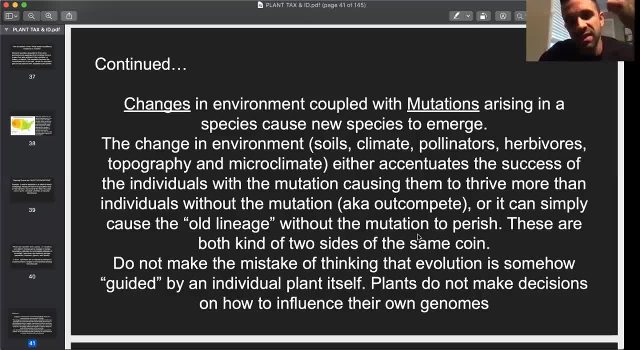 Mojave desert and they're just so successful there. I mean, you get this, you form this Kohlrabi like root, you produce thousands of seeds in a single plant and they spread. They're just really adaptive, uh, adaptive, uh traits in this new environment, And so that ends up choking out. 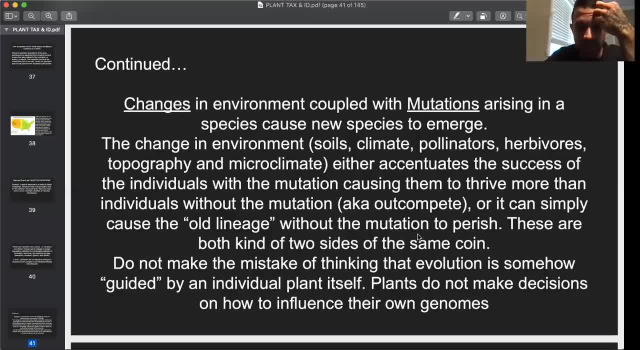 you know dozens, if not hundreds, of species of really cool annual little wildflowers. So this is why we need to manage it right. So it might be an uphill battle, but so is fighting cancer. If someone had cancer, would you tell them: Oh, you're never going to get it, It's futile, Fuck it. 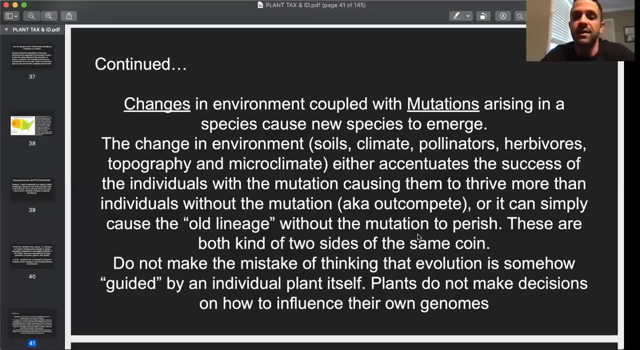 You know- I mean no, most people- are going to fight the fucking cancer. You know you don't do something because you know you're going to win. You do something just because it's the thing to do to preserve something you love. So you know, and a lot of people, a lot of these idiots- no offense- 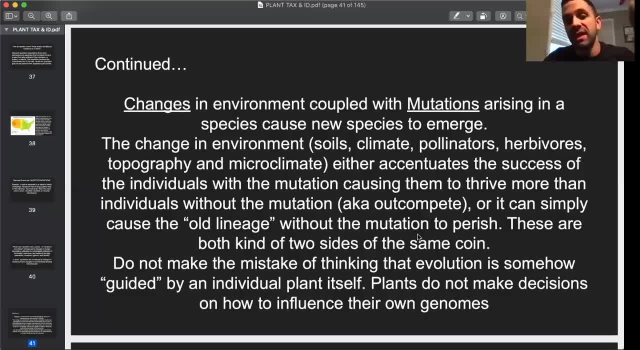 but deny the impact of invasive species. I mean, I've seen it firsthand. everywhere I've gone I see plants that are native here and don't get out of control here. but you go to Australia and they just run rampant and they lead to biodiversity loss and 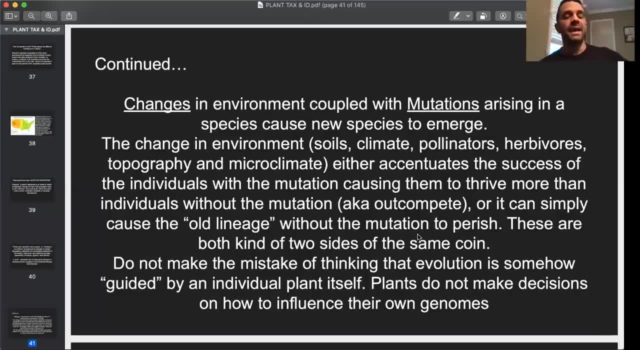 furthermore, they directly lead to extinctions. Will that plant, if humans went extinct and quit bringing new individuals of that species over to keep the gene flow going? will those eventually evolve and get checked by something in that environment? Absolutely, But the question is, what in the meantime? what's the cost? How many plants will go extinct? 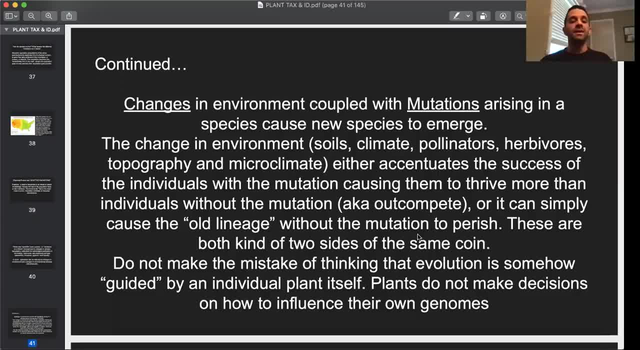 and further. how long will that take? So everything will eventually level itself out. but don't take solace in that, because a lot of there's going to be a fucking cost. There's going to be a lot of there's going to be a fucking cost. There's going to be a. 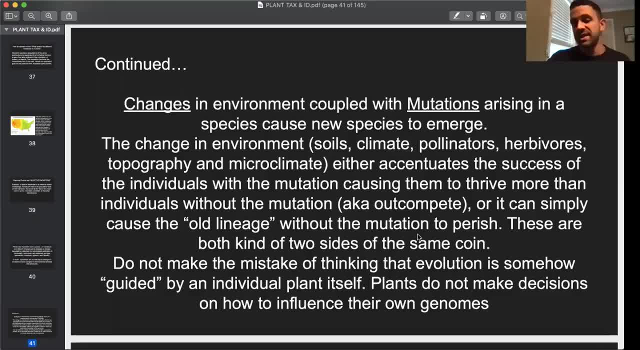 lot of things that go extinct because of that And, like I said, these invasive species dispersal events that we're causing are going to cause extinctions. There's no way, there's no way around it. I mean, this is a mass extinction. you know the invasive species are one of the 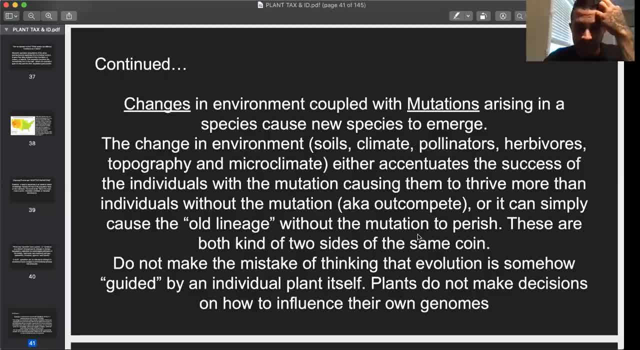 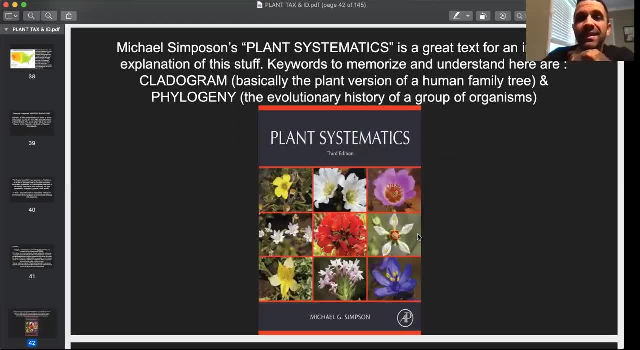 main causes of invasive species and habitat loss. So hopefully that answered the question. Anyone got any more? No, All right, here we go. Okay, There we go. There's that book: plant systematics. Uh, this is, this is the fucking. 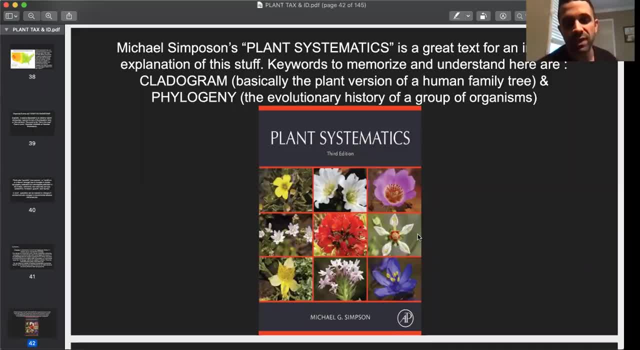 one of the most wonderful books for- and I, like I said, you, if you buy it, it's a reference book for the next five or 10 years, however long you care about this shit. Um no, it's like 60 bucks. 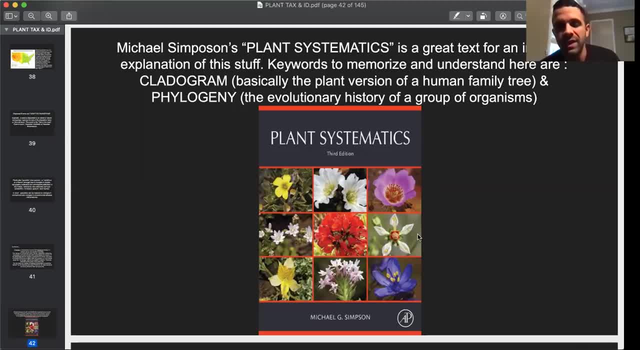 If you don't have it, fine, you can get on live gen too, But if you've got a chance to throw this guy some money, buy it, do it. Um, this really breaks it down. You know some of the the clay. 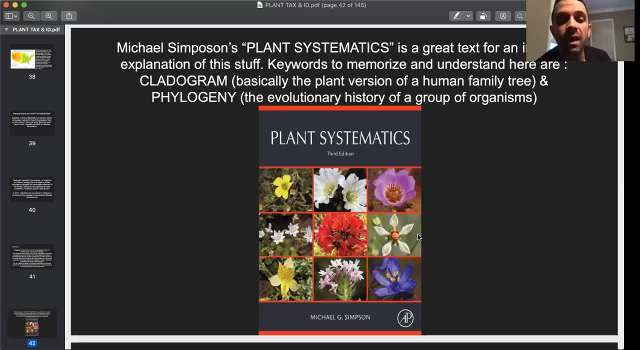 the grams I showed you at the beginning of this were were taken from, uh, this book. He's got a glossary in the back. He goes into order, He goes into families. It's not just on flowering plants. He goes into conifers and mosses and flying plant evolution. 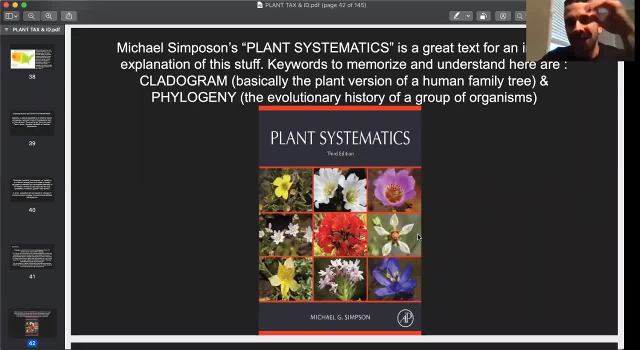 It's a really elucidating book to shed light on, uh, the rest of earth's biosphere, Um, at least the photosynthetic elements of it, and the concepts that you learn in this book when you learn about evolution can apply to mammals and bacteria and what it birds, whatever. 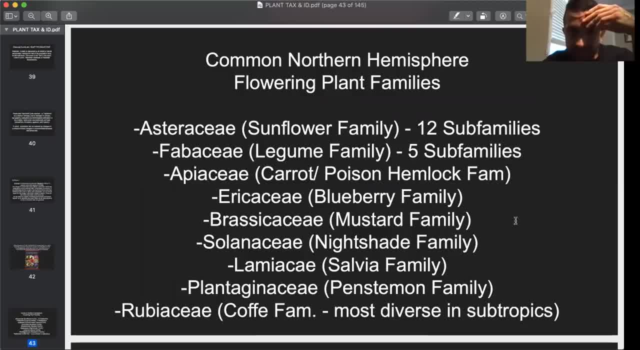 So, uh, let's see common North American uh flowering plant families: Asteraceae sunflower family. You've probably heard me rant about all these uh in the videos. We won't spend too much time. This is really important. I naturalist. I told you to download this before we started today. 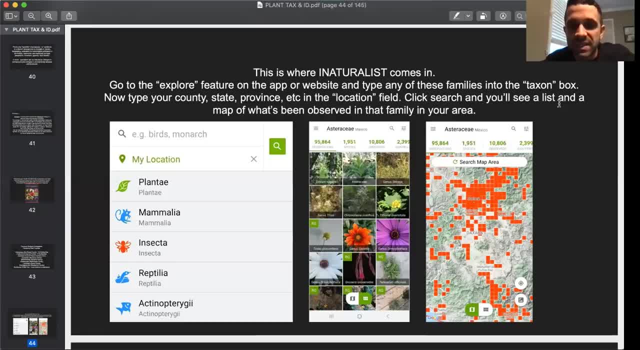 This is where you can really, uh, learn this shit. I mean, this: is you learn how to use that explore feature? This is on Android, I guess on I. on the iPhone, it's a little different iPhone. We'll just take you to the I naturalist website. 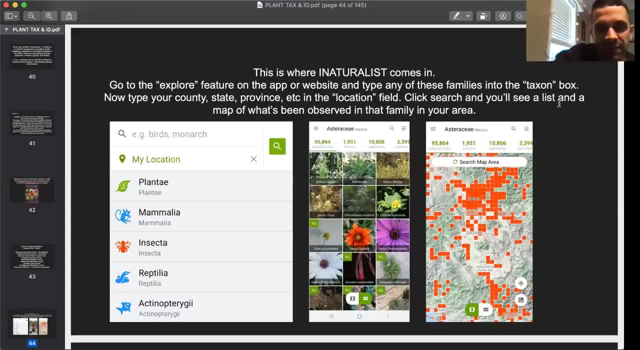 All this info is still there. You get you type in in that field on the left. you know the tax on that. you're looking for plants, type in plants. You got to wait for their suggestion to come up. You can't just hit search. It'll say: no, you know, we don't, we don't know. 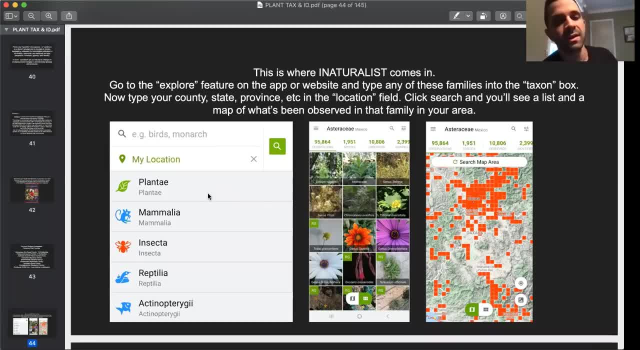 this way for the suggestion to come up. tap on it. my location, You got to know your county, your state, uh, your continent, and you will get. and you hit search, let the suggestion come up. hit search and you'll get a list of everything that's been observed in your area. Look on this. 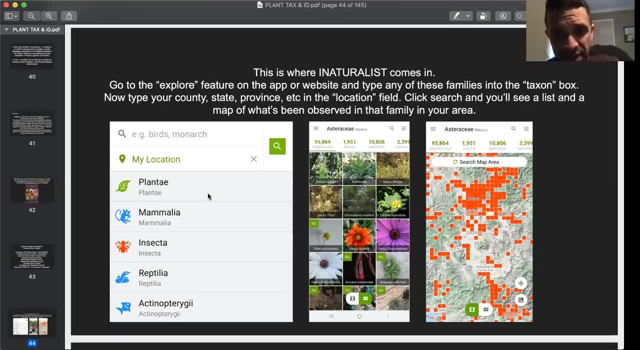 middle photo. You got how many observations, how many species, uh, how many observers. do you go to the on the bottom part of that. you click on the map where that little wavy line is with the two black bars on either side of a white bar. 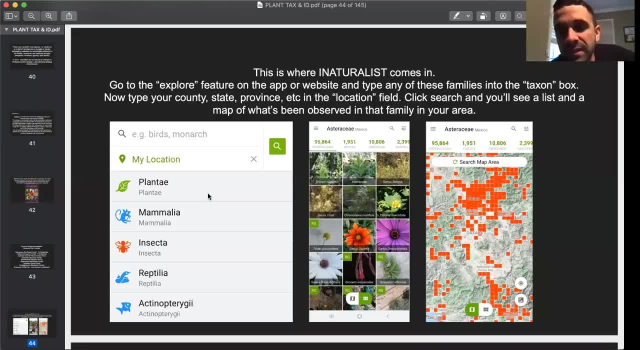 Then you get a map. So you, I mean it really it's pretty. it's a pretty fucking incredible tool Once you learn how to use it. you can teach yourself botany, You can teach yourself plant systematics using I naturalist alone. And even cooler, when you go to a species page. 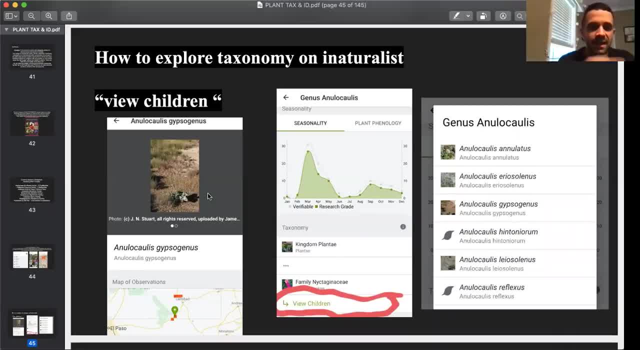 you click on, like you know, a new little call us chips- the genus. click on on the actual species page. It'll take you to the species page. That's what I was talking about before you view children, See, so you you go. you can click on Nick, Taj and ACA. They'll take you to the the uh tax on. 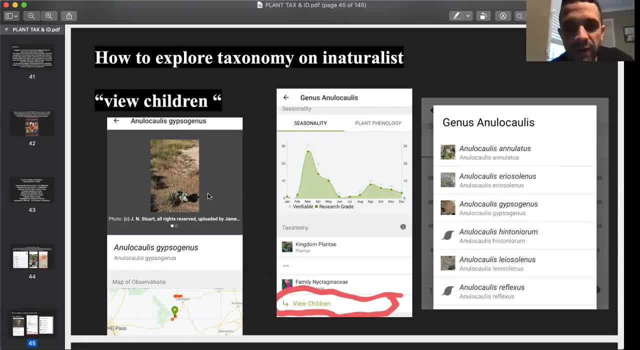 page for the four o'clock family which is in the order Karyo file, Ellie, same order as spinach and beast Um, you can click on that and it'll show you all the genera in the family. If you're looking at a genus page, like we are here in this center pick. 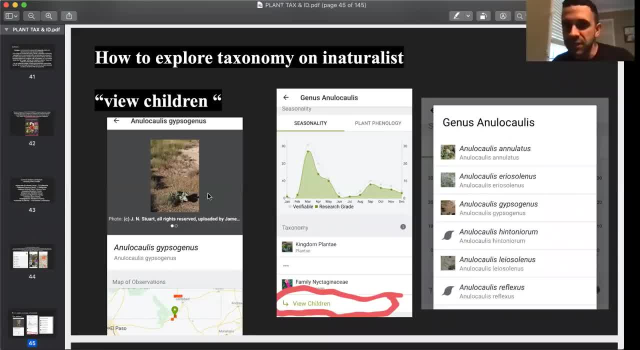 genus a new local is. click on view children. It gives you all the species of a new localis. I mean, it's it's like looking through a catalog of the different things that evolution has produced. It's fucking, it's wild. It's really cool. Uh, some of these. 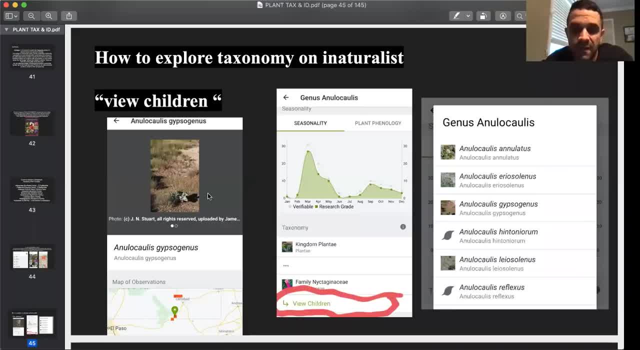 like a new localis. and Tony Orem, look at that. That hasn't even been observed yet. There's no, there's no thumbnail photo there. I mean it's that makes me that that you know that attracts my attention. Why the fuck are there? No, it must be really rare. Now I want to. 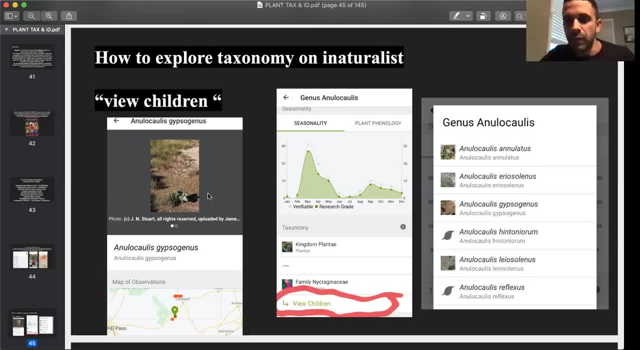 read about it. So maybe I'll go to Google scholar now and look up a new localis and Tony Orem- When was it named? How recently described as it- but you will probably- grows on gypsum in Northern Mexico because Hinton was a Mexican botanist. a new localis. a lot of the species show a. 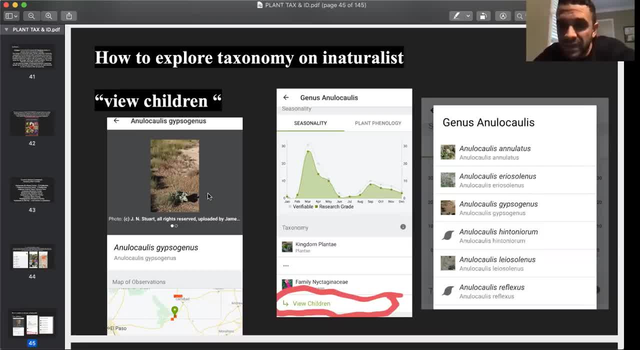 disposition towards gypsum, So I don't even know about that. but I'm willing to bet that's the type of substrate it grows in. And of course you know we'll go through these, these plant porn photos. later You'll see some of the examples of gypsum endemics are fucking wild. 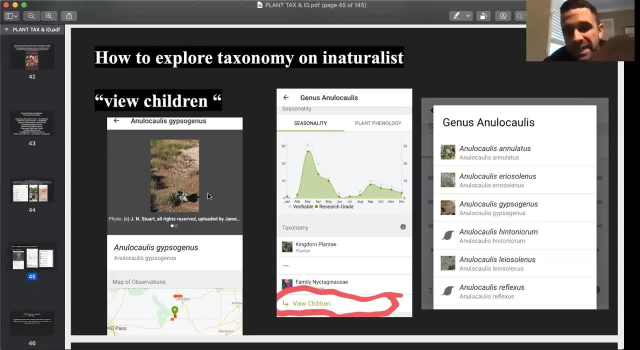 So that the thing to learn here- And I mean, like I said, you can click on plant a, you can do the same thing, You all the children in kingdom plant day, all the tax on pages of kingdom plant day. 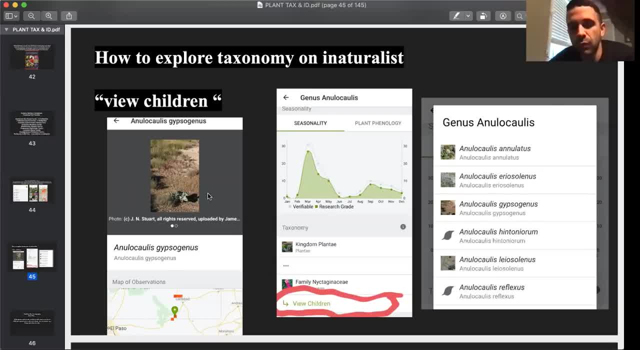 all the variations on the family and contagion ACA. then you can look at what order is Nick tagging ACA And it's a fucking, really cool tool And you can do this with reptiles, birds, anything you know, And so it'll show you how closely related things are. uh. 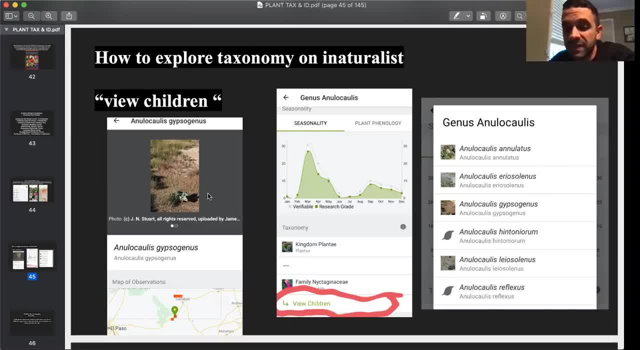 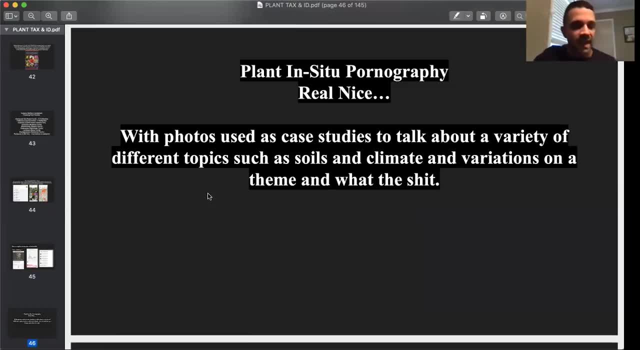 and how, how things have evolved, how evolution has worked. That's really fucking exciting and fascinating. So anyway, here we go. Here's, here's plant in-situ pornography. We run through some case studies, got the you know things to talk about. mostly this, we'll focus on socials. 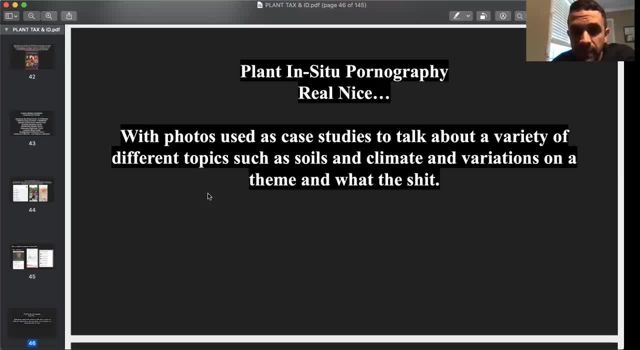 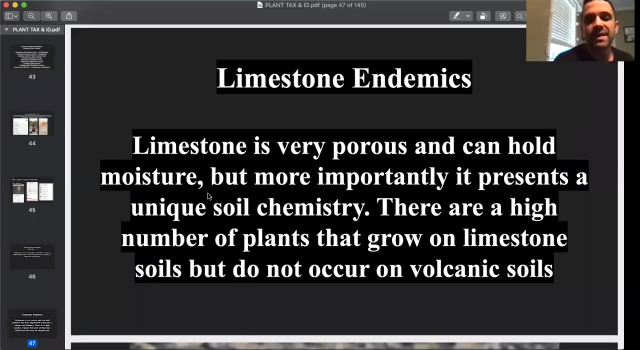 before we get into any questions from anybody. is everybody's still with me, No one's too hung over and no one's a confused or what. It's still here, Okay, Don't know doing bonkers after, So you don't lose your attention. spin. okay, i waited. yes, sir. so limestone endemic, so a lot of these rocks, uh. 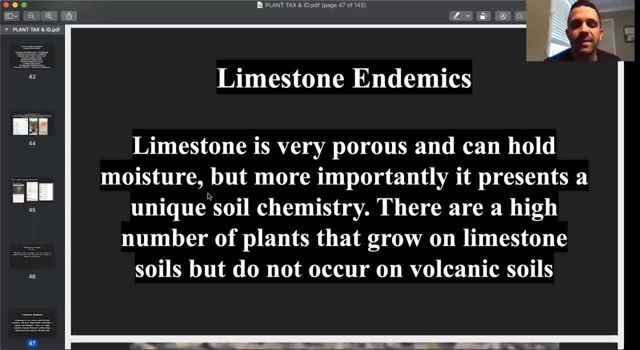 produce. they have both physical stresses and chemical stresses. stresses, i think, limestone- uh, i haven't looked into this too much, but i've read that it can be deficient in phosphorus, so you know, which of course affects roots. so you'll get uh, synapomorphies. that occurred because 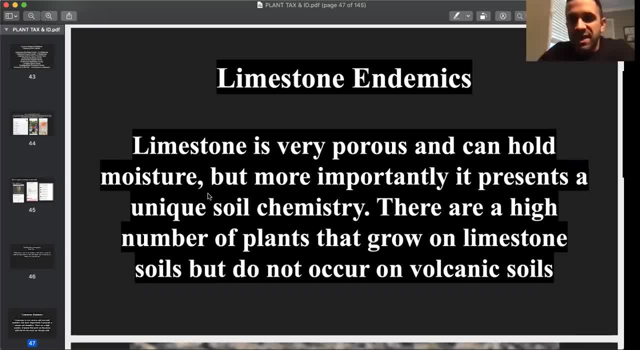 of that stress, but mostly, uh, in these areas, especially out west, where it's just limestone and there's no topsoil. you just get this bare limestone rock. you get plants that will grow out of the cracks in this limestone. so limestone is very porous. it uh tends to dissolve slowly. 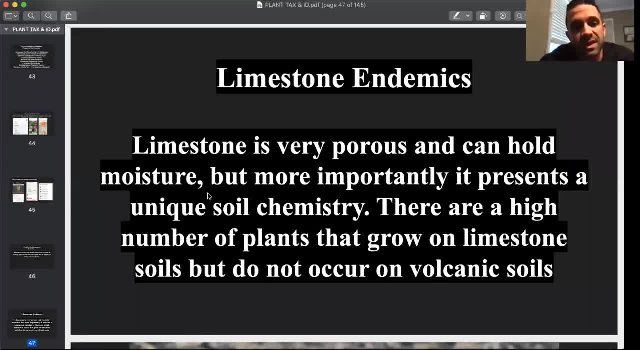 under rainwater. you know, like i remember as a little kid growing up in the midwest, you'd go to these old cemeteries. we used to go fuck around and these gravestones were all limestone. sometimes people died 120 years ago. you couldn't even read the names anymore because it was slowly eroding. 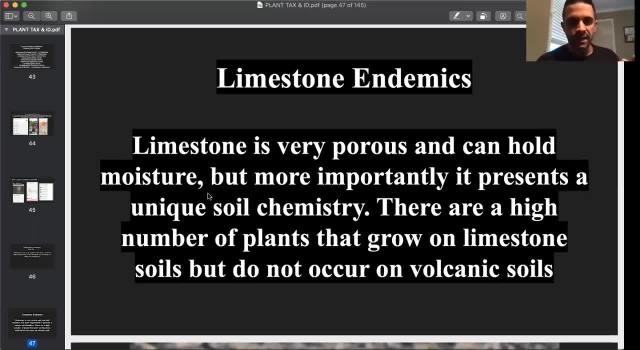 and i'll show you pictures of uh. you can see the dimpling and uh in rock that's caused by this, the reaction with uh, slightly acidic rainwater due, you know, due to the carbonic acid in there, due to the co2, and so that's why you get a lot of caves and limestone. 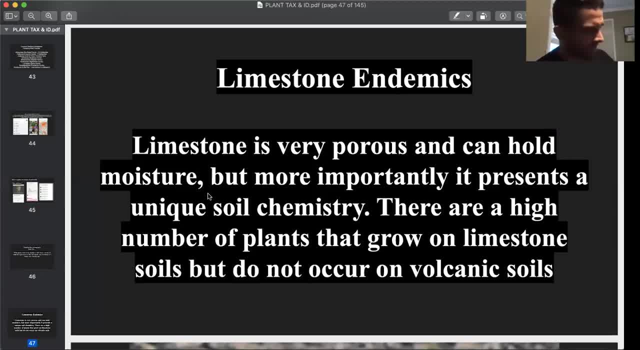 areas. i mean shit. when i was at el cielo biosphere reserve in mexico, the whole area is underlain by these massive fucking caves. you can go in one of them, you know, i did a video on it. just this huge fucking stadium sized cave- again the result of limestone, very slowly, uh, you know. 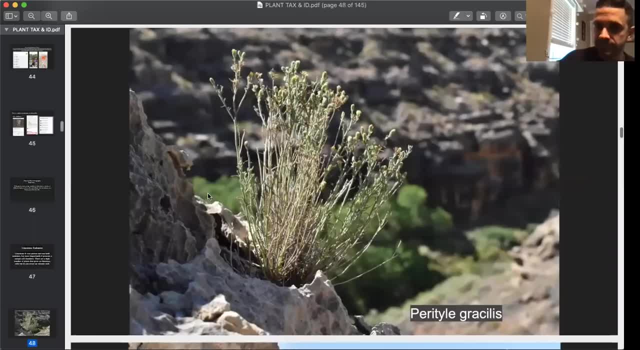 eroding and weathering with acidic rainwater. so here's a perfect example of a limestone endemic species. this is peritoneal grass list. this is at a place called uh canyon diablo, arizona, and uh, this, this is actually really cool. this is old limestone, it's you know. i found ammonite fossils. 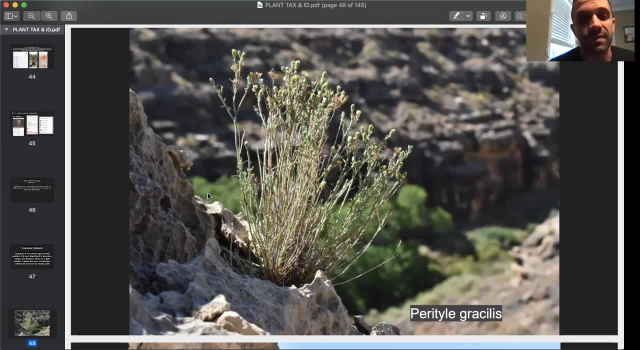 there. ammonites went extinct with that kt extinction, the meteor that hit the dinosaurs. so that tells you at least that rock is, you know, older than 66 million years. there were limestone, there were ammonite fossils everywhere. you know. ammonites like nautilus looks like an octopus with a curly q shell, um so, and you can see, look. 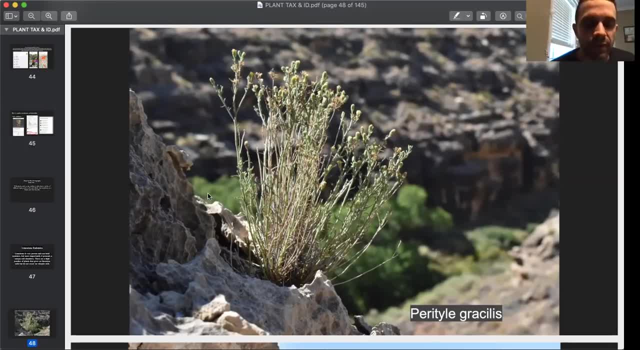 at the texture of that rock, see the dimpling. that's all because the way it reacts with right, with rainwater- and it doesn't rain here very much- it's the fucking. you know this is like central arizona, uh, but when it does rain it works. it works away at that limestone and over massive 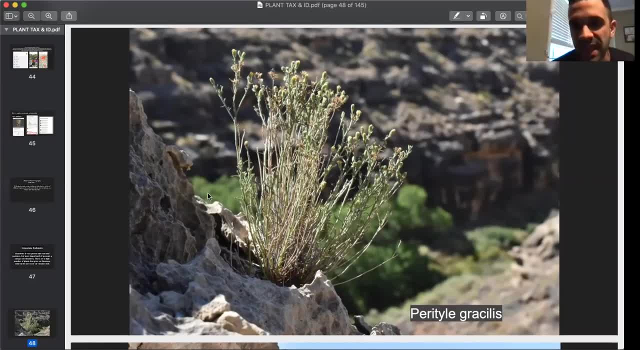 amounts of time. you know it creates caves. it's created this canyon that i'm standing on the sketchy edge of and it also with limestone it creates these really cool kind of staircase uh patterns which you can kind of see in the background there. see how like 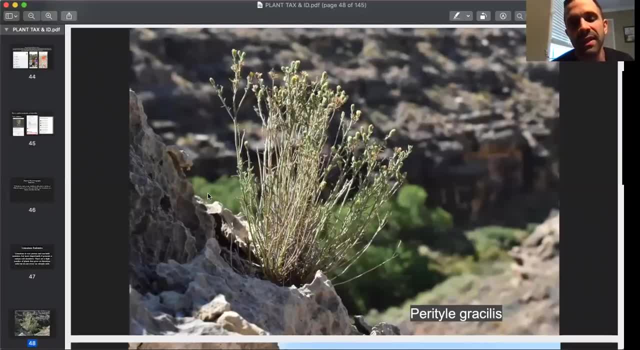 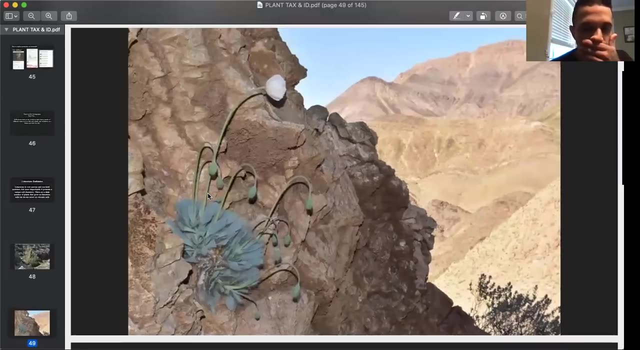 it's wider. the higher up you go, the wider it is. it's because that rock has been exposed for a longer amount of time, so it's had more time for that rainwater, or the, maybe the river in this case- to work at it and and chisel it out. uh, here's um, i was confused. 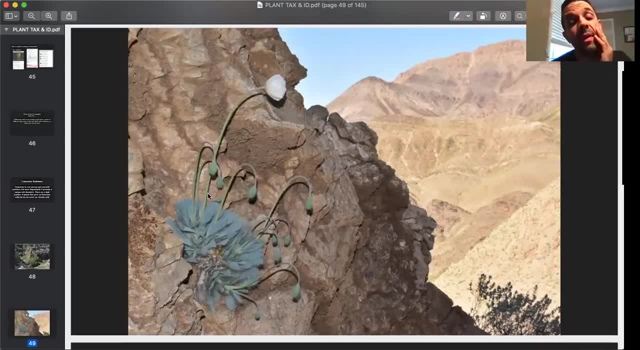 with our gemini, our arctomicon. uh, miriamii the bear poppy it's called, because the leaves apparently look like a bear paw and they're covered in fuss. this is from the fucking mojave desert. this plant grows a lot in death valley. uh, immediately, look at the blue color you got. 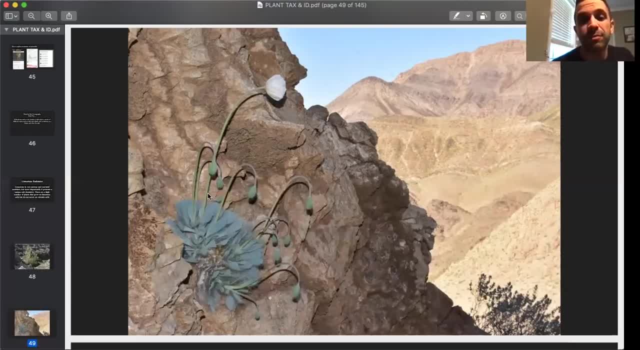 the hairs on it. boom, it's a fucking desert plant, of course. not only is it a desert plant, it's growing out of a fucking vertical limestone cliff face that actually looks like it might have a little bit of gypsum in it. uh, next to, uh, an abandoned mine. this was a fucking, really cool. 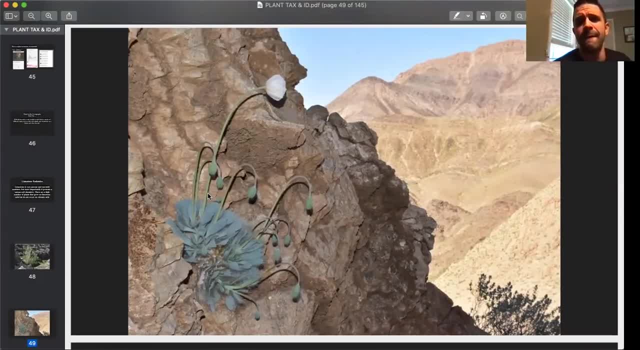 plant. i remember the minute i found this i was like god damn, this is like picturesque. you know, this is fucking insane. remember the poppy family that has evolved to grow out of i mean, there's no soil there. like: how does that? what are the conditions that it takes for that seed to? 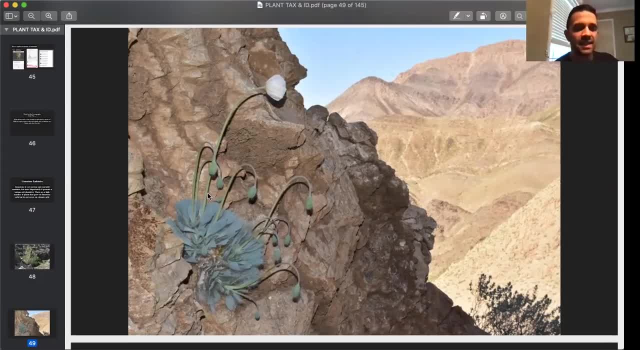 germinate? does the rock have to be wet? is there a cryptogamic crust that holds that seed in there? uh, how old is this plant? this plant could be fucking 20 years old. you know who knows um and you know it's quite likely that a lot of the limestone has. you know once it. 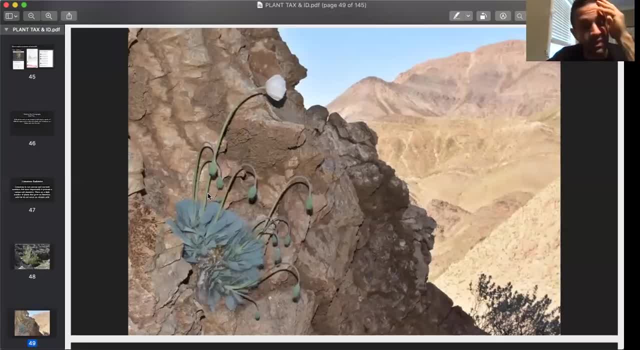 rains. it kind of holds on to that moisture. it's a porous rock where there's cracks in it. uh it it maybe it behaves like a sponge and holds on to that water uh longer than like rhyolite, which is just silica, you know, and water will just run right off. limestone, of course, is. 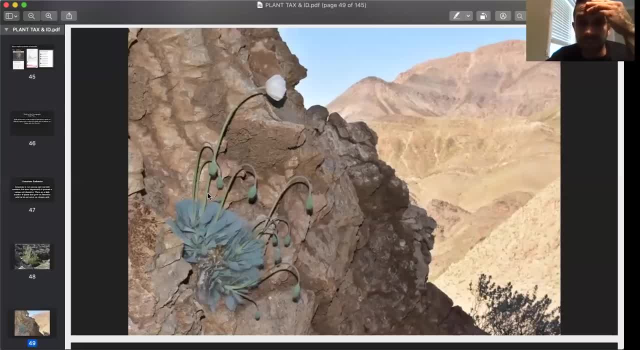 calcium carbonate. that's why you get that uh reaction with the, the carbonic acid diluted in rainwater. so there's uh arctomicon mariammii, all species in this genus, and there's only three of them. uh are endemic to either limestone or gypsum. 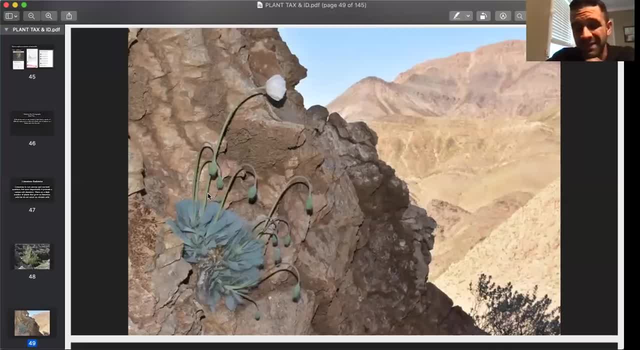 there's two other species that grow in gypsum. they're equally fucking wild. i think i got a photo of one, but i mean they grow in areas where it doesn't seem like a plant should be able to grow. you know, gypsum when it's wet kind of spongy, kind of soft, when it's dry it's got the texture of bad. 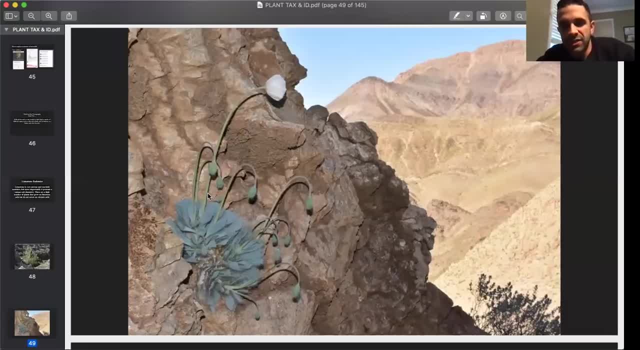 concrete. it's brutal to kneel on seeds, can't penetrate it. uh, you know, it's like a radical or a root emerges from a seed. it cannot penetrate that crust, but then it changes texture when it's gypsum, of course, is what we make drywall from. 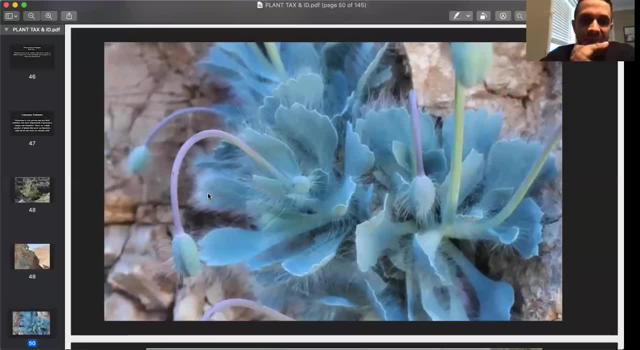 look at the leaves on that man: just blue and so fucking hairy. uh, the blue color, also called being glaucus, uh helps reduce, uh, it helps reflect ultraviolet radiation. the hairs keep the moisture in also reflect ultraviolet radiation. the whole point is to keep the leaf temperature down and keep the moisture. 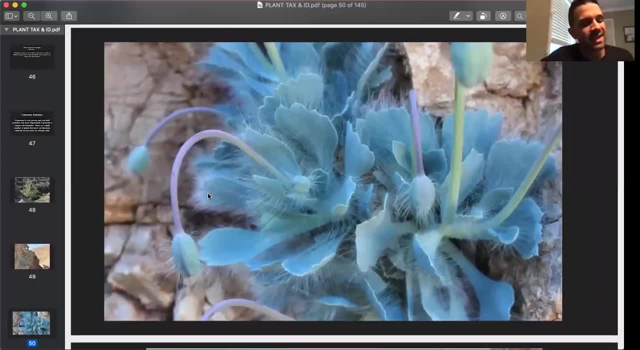 inside, moisture transpires from plants and those tiny little pores, often on the undersides of the leaves, called stomata. you have to have those stomata open, uh, at times when you're photosynthesizing to bring in, uh your building blocks, your co2 uh, but that's the. the bummer too is when you got them open, you're also losing moisture. so how do? you cope with that. you evolve hairs. you evolve a thick wax a lot of desert plants will have just have. they won't have hairs, they'll just have a really thick cuticle, aka the wax on them too. another cool limestone endemic. you're only going to find this growing on limestone. 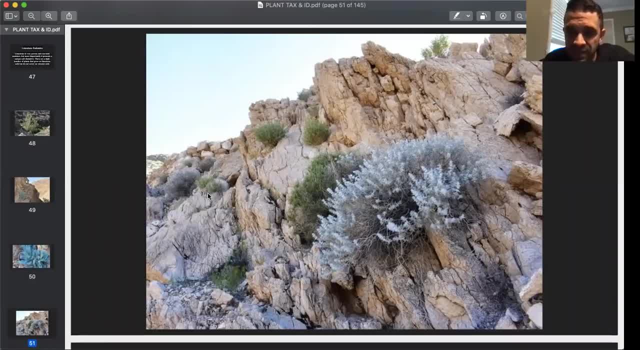 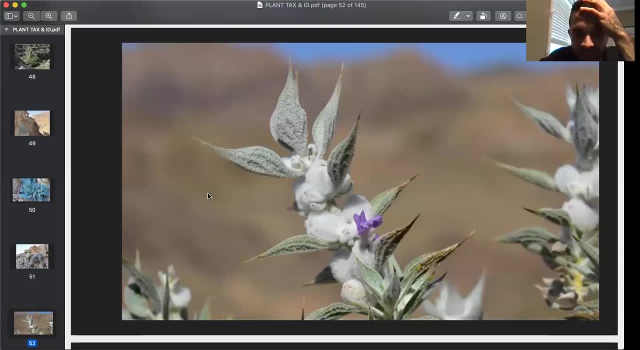 salvia funeria, the funeral sage, also from the mojave desert. there's the flowers, i mean the calyx on these are look like cotton balls. i mean it's like the mojave desert, of course, is the driest desert in north america. as you proceed east, you get a. 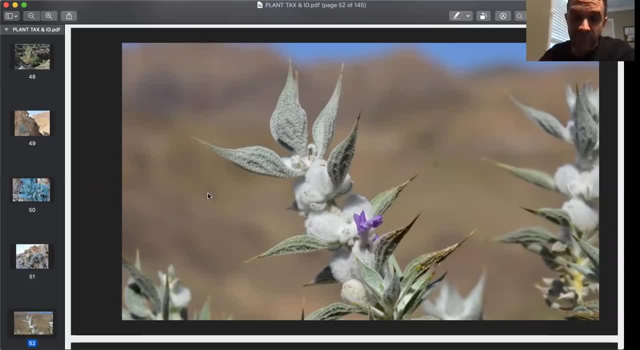 little bit more summer rain. when, when you end up at the chihuahua desert, you get a lot more summer rain, it's still a desert, still really hot, still really dry. you still have that, those descending high pressure systems at that latitude, uh, causing the aridity. um, but you get a little bit more summer. 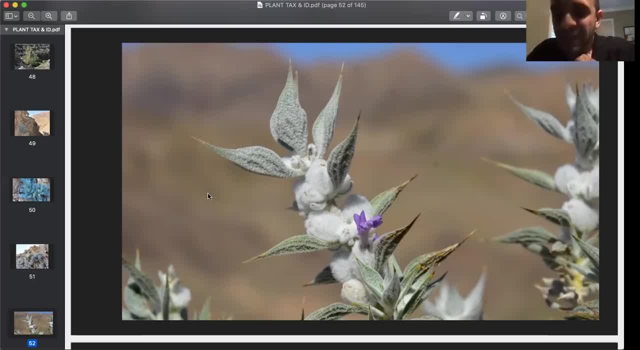 rain, you get the summer monsoon, not so in the mojave desert. it's so fucking dry. i mean, the mojave desert has the biggest assemblage of white and and like sky blue plants i've ever seen. it's fucking incredible and spiky. look at how these leaf tips have been modified. 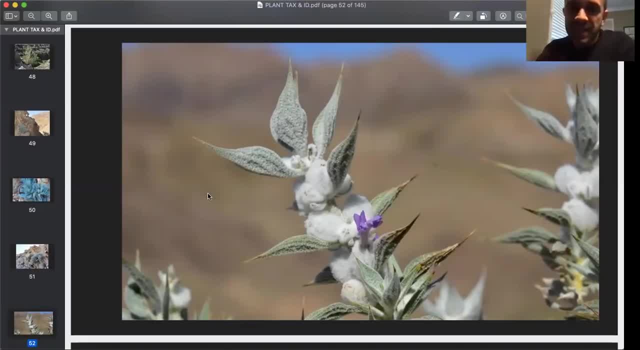 to be, to be spines. i mean, it's fucking, it's so. there's a story there. that's what i'm trying to teach you. there's a story there behind that morphology. it's not just: oh, look at that, it looks kind of cool. i'd like to take a photo of it put on my wall. or, oh, i can make a potion, put it. 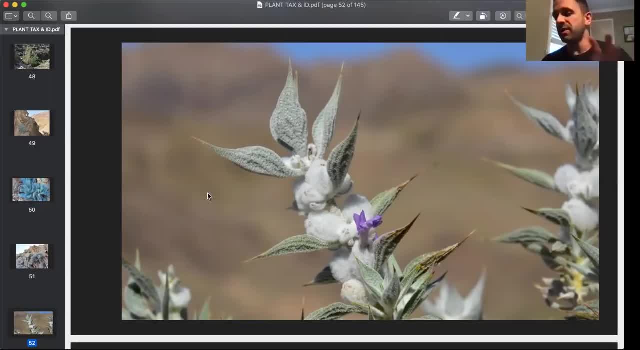 in my ass. there's a fucking story there that relates to geology. there's a story there that relates to plate tectonics and how the uh deserts have evolved to to what what you know in the earth's atmosphere is causing there to be a desert at that locale. um, you know, plate tectonics in some. 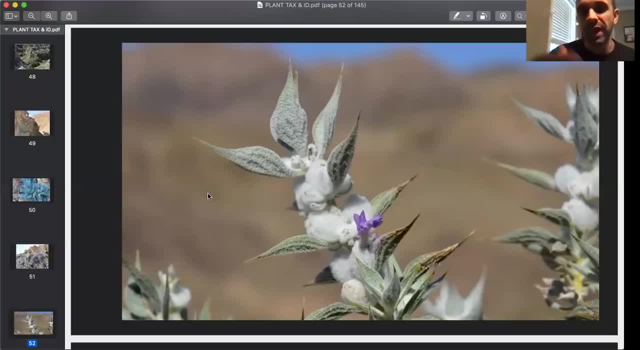 cases. you know what mountains have arisen and that caused the rain shadow. you know the that all that air rises, that moisture-laden air rises. when it hits that mountain it's forced upward, dry out, loses all its moisture and everything on the east side of that mountain you know, become their. 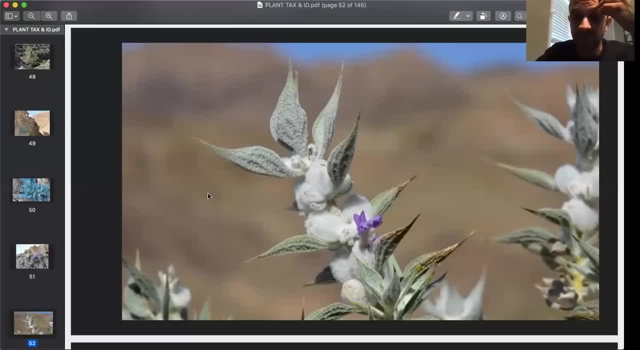 landscape becomes super dry, so new species evolve. this is a fucking great plant and it smells great too. it's a- i mean, it's a sage, it's a salvia. uh, and look how small the flowers are too. just big enough to get noticed by pollinators, but not too big that they're going to lose. they're going to. 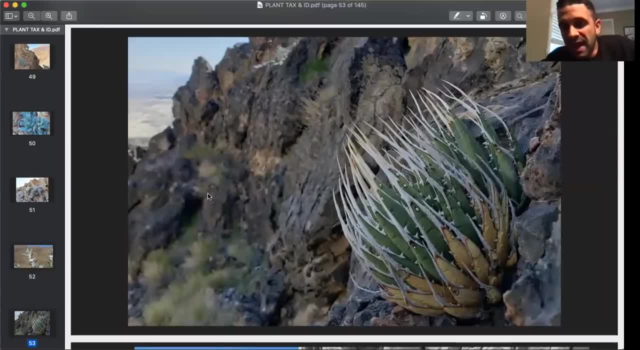 be a source of a source of moisture loss. agave utahensis- there's like three different species of this. i've never paid much attention or cared to, not species varieties of this. i've never cared to figure out which ones they are. ebora spina- is it subspecies and evidences, or variety and evidences? whatever? it doesn't matter. 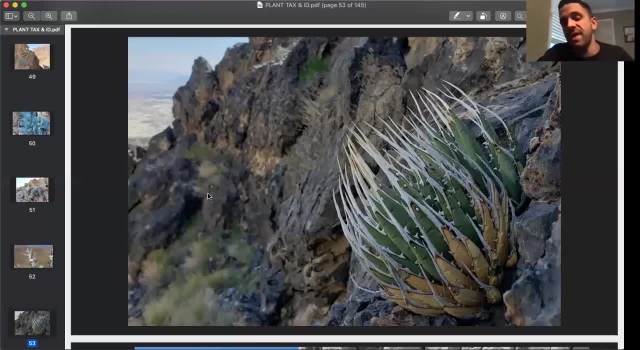 just a cool plant got another limestone endemic. you only find this growing on limestone. is it because of the porosity? is it because of the the uh, different uh, cation and anion structure of the, the rockets growing in because of the lack of phosphorus, and this is adapted to a lack of 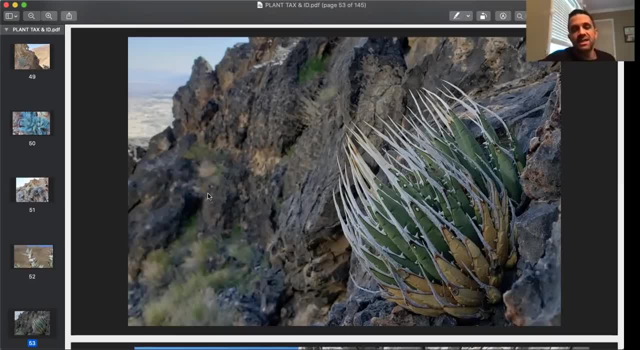 phosphorus. i don't know. you know who knows and you'd have to investigate that, study, that individual plant to figure out why. but you will never see this growing on volcanic rock and i've seen it all over southern nevada and southeastern uh california. not once have i ever. 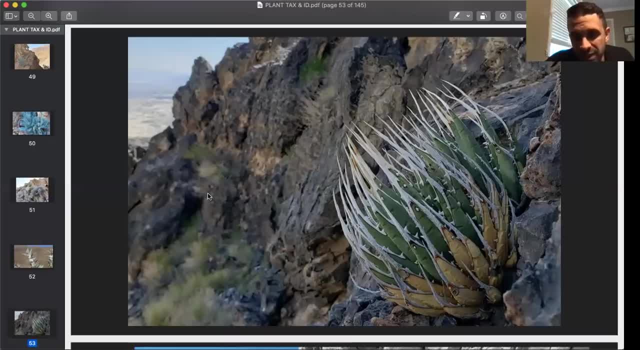 seen it on a volcanic rock like rhyolite or andesite or especially basalt. it's only growing on this really old limestone, like some cases three, four hundred, five hundred million years. uh, that's got the texture of really harsh sandpaper, so i can see a limestone hill from. 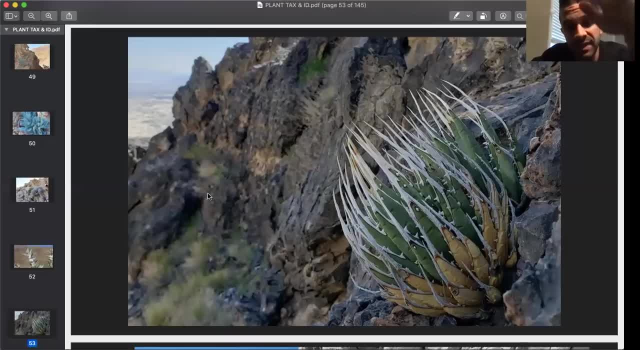 there, but i can tell you what plants i'm probably gonna find there, you know, if it's in the mojave desert, which i'm familiar with, you know. and this is where you start to see these, these similarities and these traits, and again they point all point to the same story of how this thing evolved. 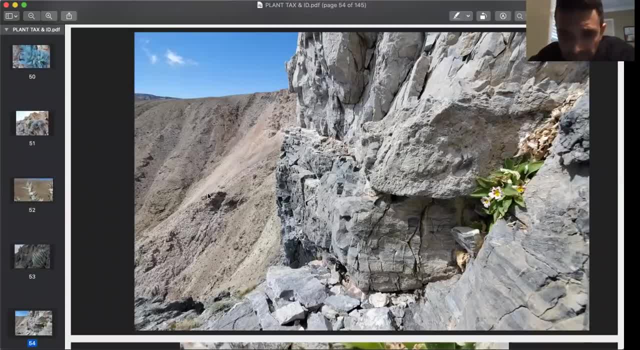 this another favorite death valley monkey flower, the placus rupicola, only find growing on limestone, only find growing in the cracks of limestone, very rarely. well, you'll never find. you'll never find it growing in an area where there's like a soil, even if that soil is limestone. 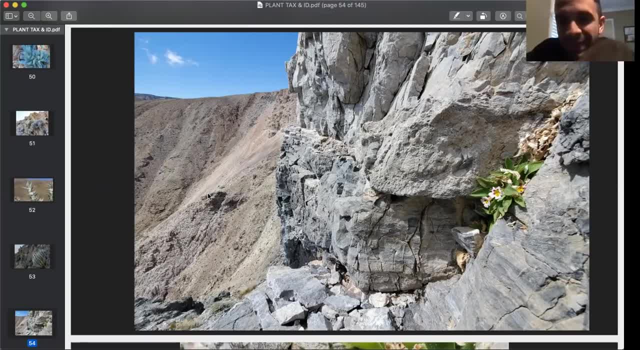 based limestone was a parent rock. you'll only find this growing in crevices of fucking limestone rock, and the habitat here, as you could tell, was really fucking cool. i had a great time. this isn't the fucking janet jackson- uh, at the start of the pandemic- crawling around on these limestone. 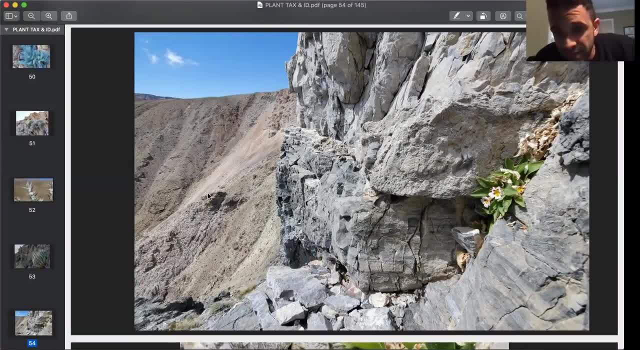 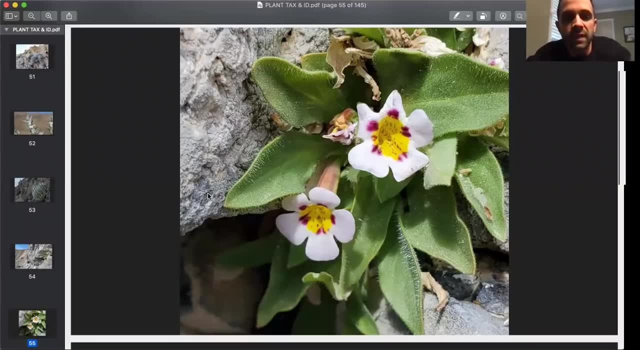 rocks, almost breaking my ass and just being fucking stoked. i was like this is epic man, this is awesome. there you go see the hairs on it. you get closer it's it's bright green. but when you get closer, not only do you see hairs, but you can see little glands. that's why it's got that kind of. 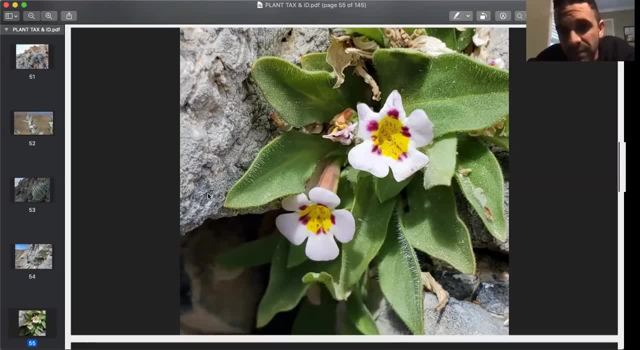 shiny nature to those leaves. the fucking flowers are beautiful, totally incredible, and the the habit of how this thing grows just out of cracks and limestone rock, only from a few mountain ranges around death valley, is what makes it so uh exciting. i think it's a california endemic and 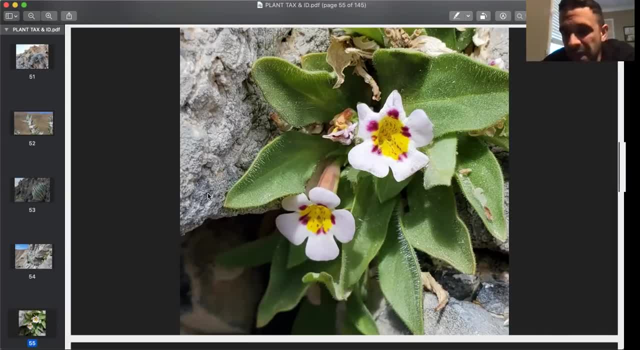 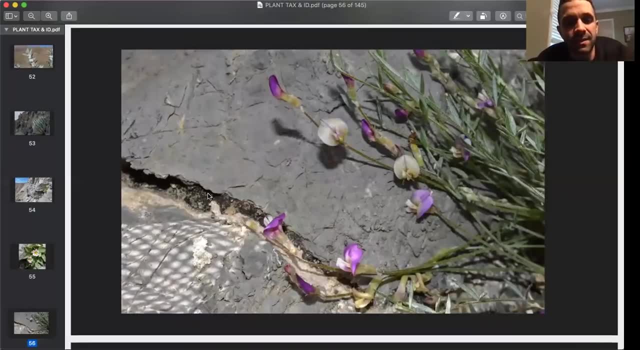 maybe it occurs over the border in the valley greater, in a few limestone uh ranges too. but astragalus panamintensis that netted shadow on is my hat this was. i would like crouch over it to get a good low contrast photo. um, this was growing again out of straight rock. you know, astragalus, aka the loco weeds, it's all. 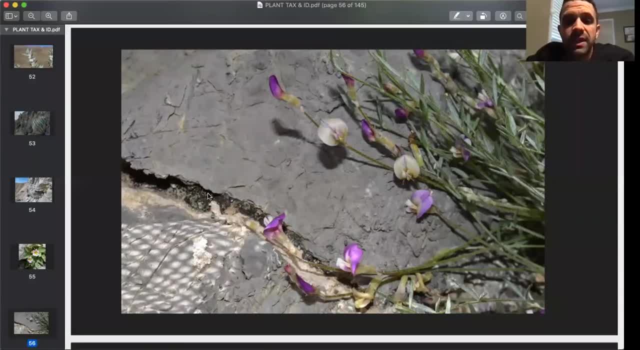 they're all over the fucking globe. there that's been a very successful genus in the pea family. you got a typical pea family flower right there, a banner wings and keel. the is that big posterior petal right there, astragalus. if you know what it's, this is a really cool. 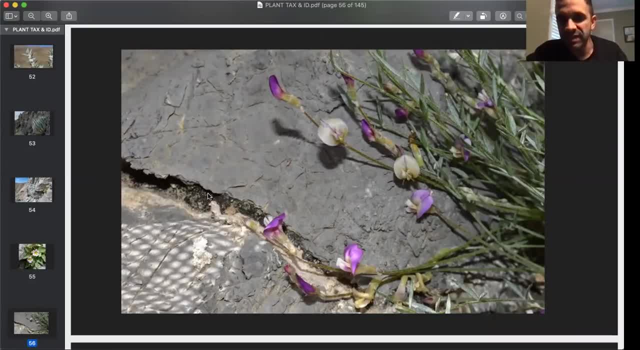 variation on it, because astragalus normally has these big leaves, pinnate leaves, you know little leaflets opposite each other. on the rachis that's the stalk, but this one it's from such a fucking dry environment. not only are the leaves blue and covered in hairs, but the leaves have been so. 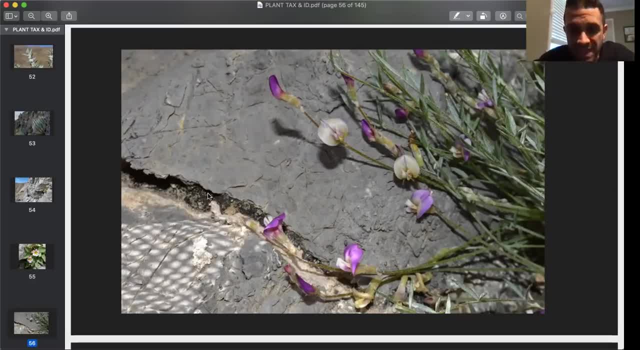 reduced that the, the fucking. and it's photosynthesized to the stem, that it just looks like it, the leaves, this thing wasn't blue, it almost looks like a grass and that's another synapomorphy. uh well, not a synapomorphy because it's. it's a convergent trait, you know plants can. have this trait without being related, but that's another thing you'll see in a lot of desert plants is stem photosynthesis most. the obvious example is cacti, but you'll look at palo verde, the palo verde tree in arizona. i mean that thing. can have leaves, but uh, at some point there was a mutation where that thing uh started producing chlorophyll in its stem. that proved adaptive and beneficial. now it could lose its leaves and save all that moisture. you lose your leaves, you're not losing any moisture anymore, but you also can't. 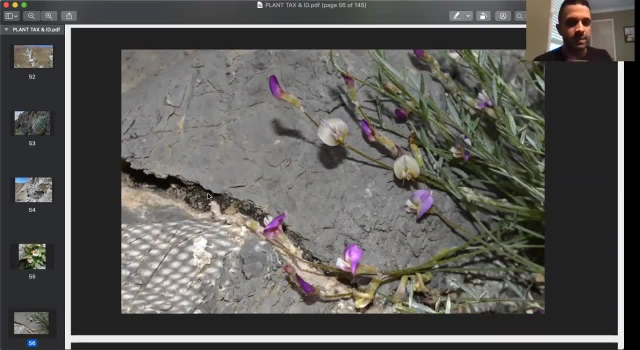 photosynthesize, but this can the palo verde- not this plant, but palo verde in the pea family. it's a leguminous tree- can uh photosynthesize through its stem tissue, so it's not an issue if it loses its leaves. it's an adaptive trait. 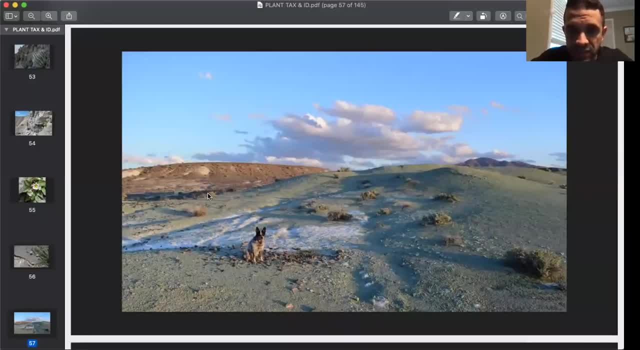 this, uh, is not limestone, i just want to show it. it's cool, it's looks like snow. this is, uh, in nevada and southern nevada, technically the mojave desert. still, what is that rock composed of? who's got a wild guess what that shit is? gypsum, nope. 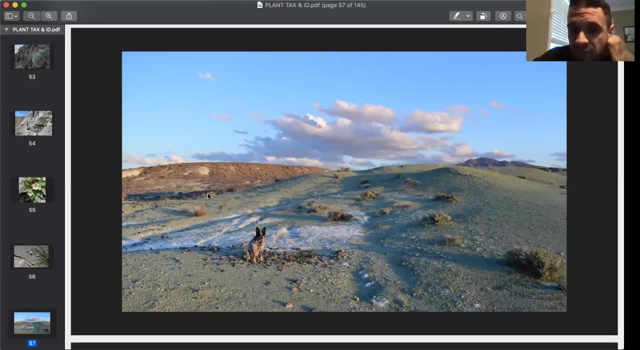 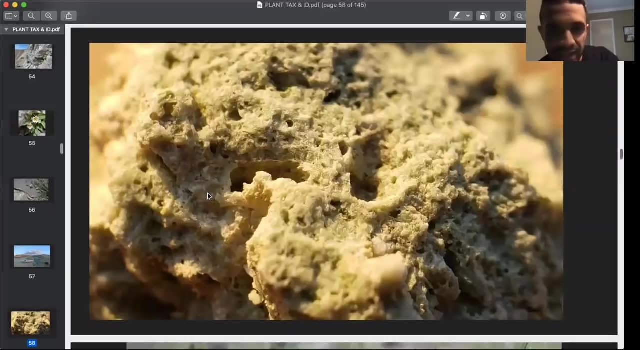 anyway. this is why you get titanium. what's up serpentine? no, no, serpentine is always like blue or red. maybe it's salt, could be some, maybe gypsum, maybe let's get up close and look at the rock with a hand lens. it's fucking. it's ash, it's volcanic ash. you see that texture looks like a piece of pumice. 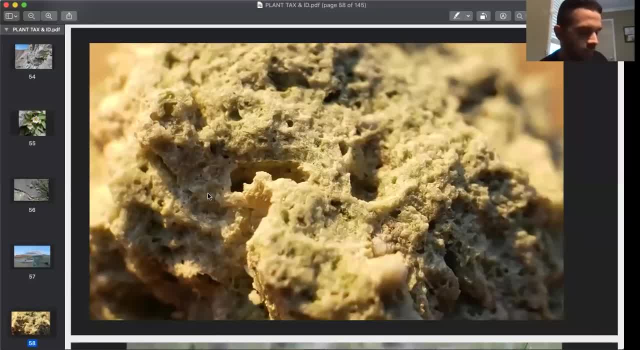 this is probably the whole screen is maybe one millimeter across. uh, you see the the, you know the gas, the gaseous nature of this high silica rock. remember pumice and and obsidian are the same thing, just occur. they're chemically the same thing, they just different environments. 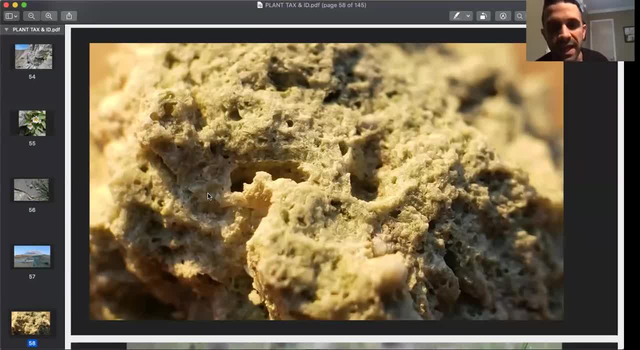 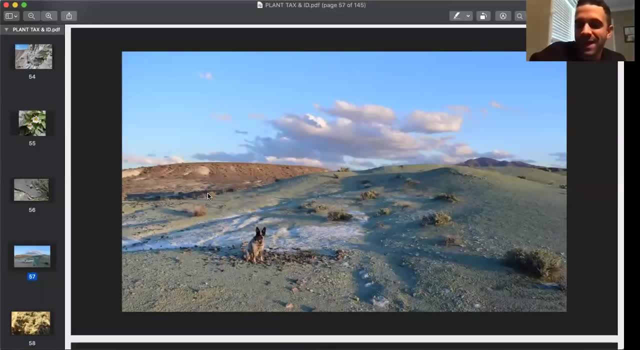 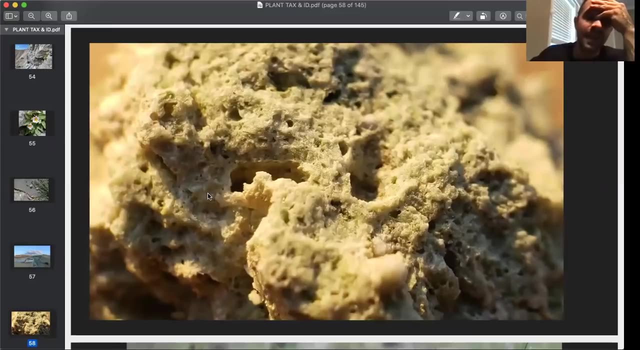 create them. uh, this thing was filled with a lot of gas, it was very frothy and that's what this was. so this was. this is volcanic rock. this is volcanic rock. it's it's volcanic ash. um, i haven't seen how this really affects. i haven't seen too many endemics to volcanic ash. um, obviously, the stress. 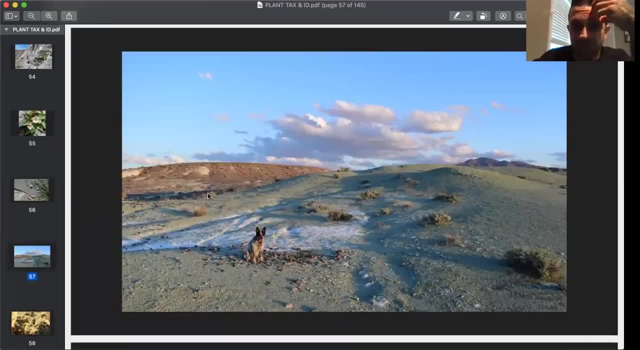 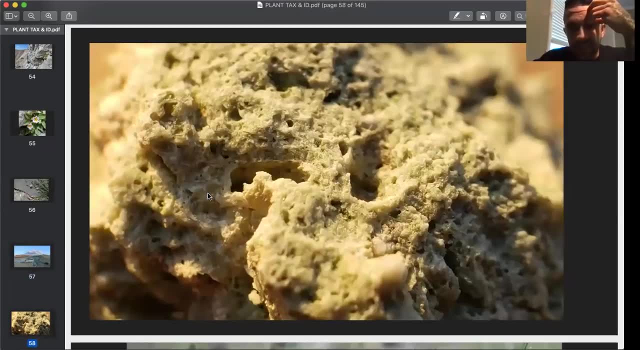 is there. it creates a barren environment. it can be hard to grow, it doesn't retain moisture. but it's the mojave desert. everything is pretty barren, um, but again, that's another great thing- that use a hand lens. i mean, right there, you look at that and you're like, oh, 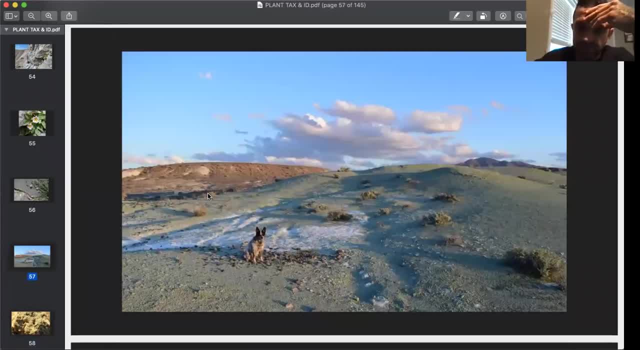 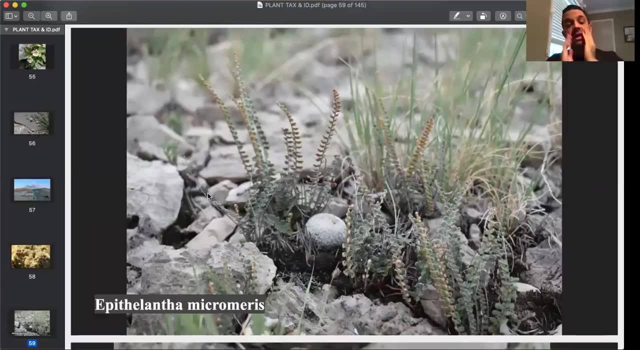 this fucking pumice. it's like a tiny grain of pumice, no shit. oh, okay, cool, you can see jack patiently waiting for a sausage right there. uh, here we go back in the limestone. epitheliantha micromaris- this thing's fucking incredible too. uh, you got um astrolipus, the fern on either side. 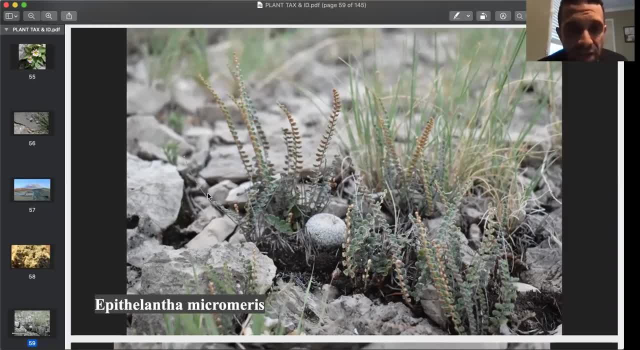 pterodactyl is the family on that. one of my favorite desert ferns, xeric adapted ferns. that just means dry this thing. this is in new mexico, you could see. this is another cool thing about cacti: spines are not always defensive. spines can be for- uh, crypsis. spines can be for camouflage, which is what this guy 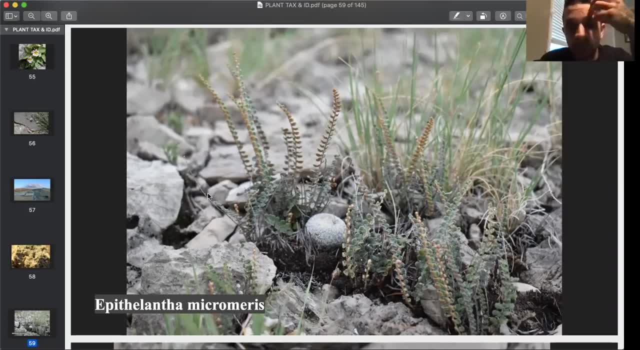 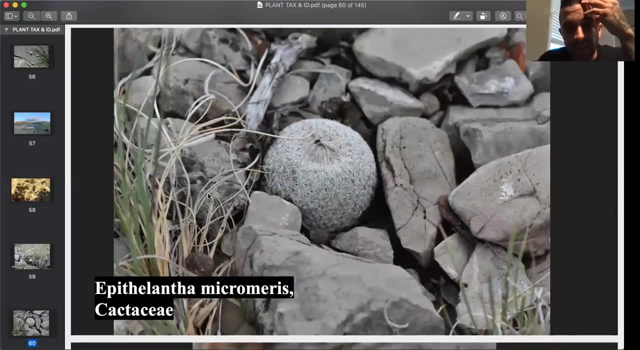 is doing this is: you can touch this and it doesn't hurt. there's not. they're not going to poke you, but those spines have been modified in such a way that it basically makes it blend in with the- uh, with the limestone. nice money shot up close. as you can see, the 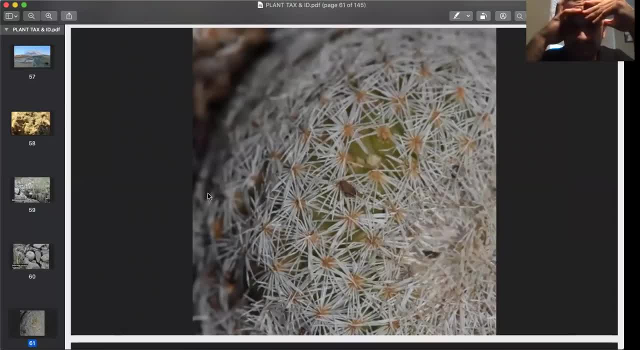 the tubercles there, the, the spines also keep that, that uh, epidermal tissue, the temperature that epidermal tissue down. could someone turn off that mic, whoever, whatever it is coming from, sorry thanks. so those spines, you know, can serve multiple purposes if it's an adaptive trait to 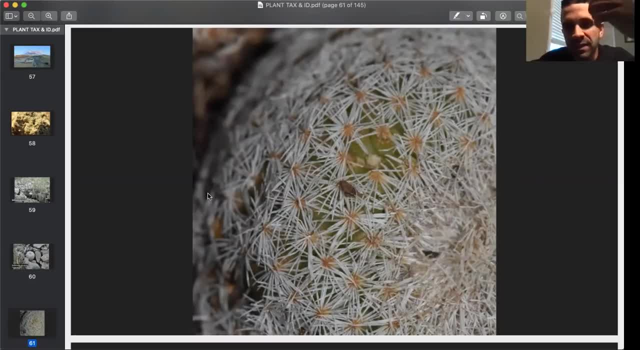 have spines like this, that that aren't pokey. don't waste that energy putting out these central spines that are going to poke herbivores. if this is enough, half the time the herbivores won't even be able to see you. you know, rabbit won't be able to see you, and also, 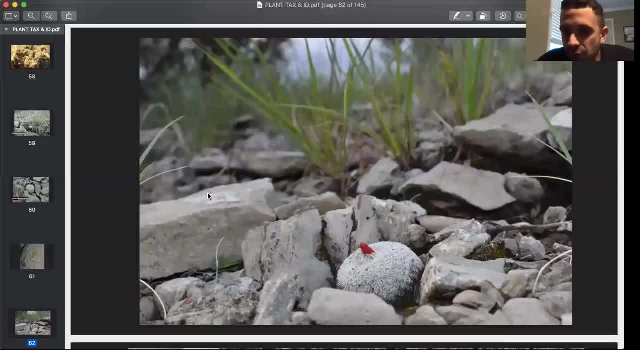 you're mitigating that ultraviolet exposure. but then when you want to get noticed, you want your fruit to get dispersed. you make it bright, red or not make it. of course evolution is not a conscious decision. certain alleles get accentuated uh over others. the allele to produce red fruit is the basically the standard now for this species, and a lot of cacti do it. so a bird will come by see that, pick it up, fly off with it, eat the skin and drop those tiny little poppy seed like cactus seeds out somewhere new and disperse it. another cool limestone endemic. petrophyton stays pitocin rose family. this thing is closely related to rose? well, not. it's more closely related to roses and cherries and strawberries and raspberries and almonds than any other plant, okay, than plants that aren't in the rose family. this thing is thought to be a. 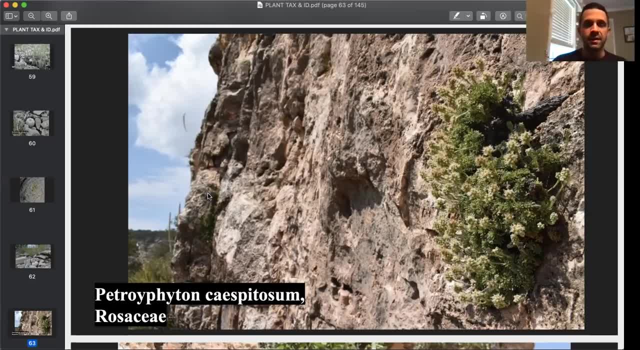 basal member. ie. it evolved relatively early, early in the early 20th century, and it's been growing on the history of the rose family. uh, and this thing only grows on rocks. it only grows on vertical rock walls. sometimes if the limestone's been tipped, you get a limestone boulder. it'll grow. 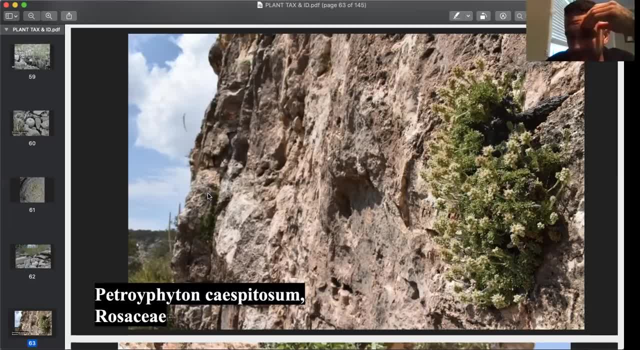 on that too, but it doesn't grow on soil and these things can last for hundreds of years. another pretty basal member. basal just means you got to think of a cladogram, right so? or a family tree. so a basal member would be at the base of the family tree would be one of the early diverging. 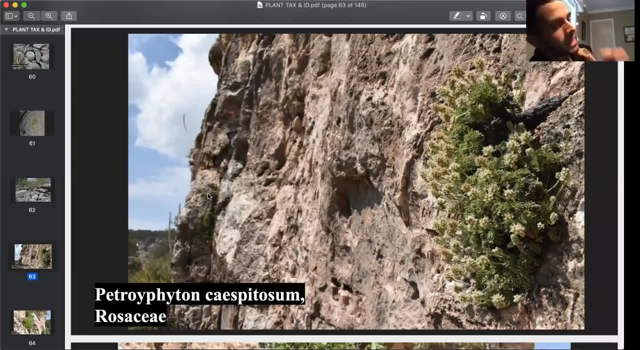 early branching lineages. uh, like ambarella is a basal member. uh, is a basal lineage of angiosperms, of flowering plants. um, you know, it just means that it branched off those long lonely branches i was showing you in that cladogram before. um, common ancestor? uh, perfect, not necessarily, but shared, yeah, it's, it's. 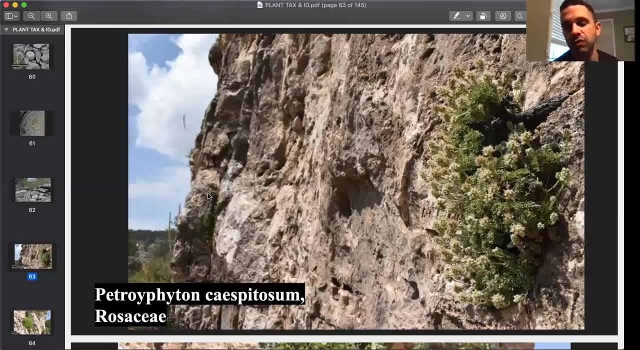 in the rose family, so it shares a common ancestor. it's more closely related to roses and strawberries than it is to any other plant, so it's a common ancestor. it's a common ancestor, it's a common ancestor of the plant family, but it still stands out, stands almost alone in the rose family itself. 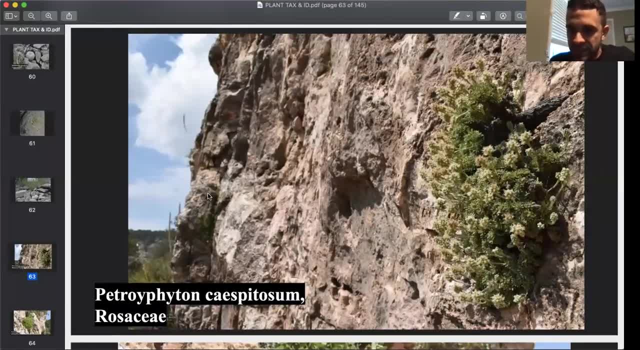 okay, but and of course, if you were to get down and look at those flowers, the hand lens, you'd see the rose flower, the rose family, flower, synapomorphies, you'd see a few of them. uh, that it shares with other rose members of that family. so here's, here's, paredale kinkoflora asteraceae. 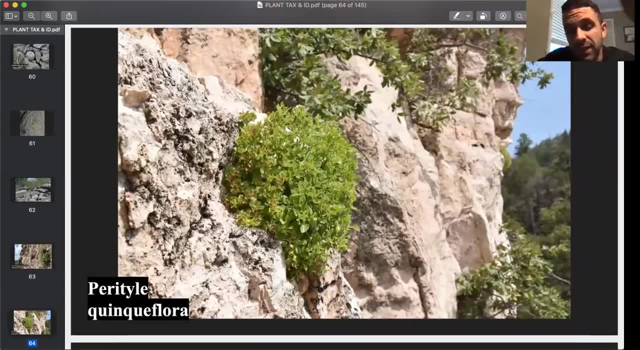 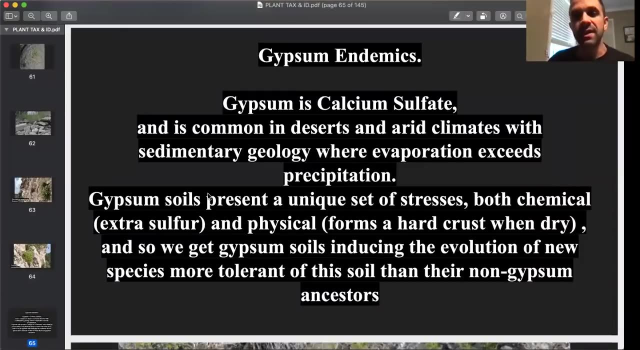 another limestone endemic, uh, another rare and uh narrow distribution only known from a handful of uh limestone mountains in, uh, i believe, northern texas and southern new mexico, near guadalupe national park. here we go: gypsum, calcium sulfate- so there's a lot of sulfate dissolved in the oceans. 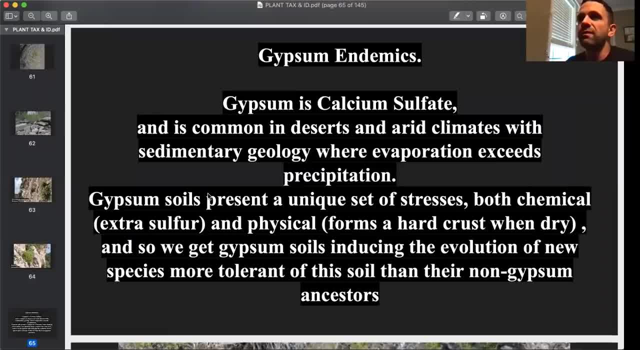 i think for every like liter of of seawater, you have like 2.5 uh, what is it? milligrams of uh, sulfate, um. so it's, it's there and eventually, you know, when you get shallow seas where water evaporates more than in really deep seas where evaporates faster, you get these gypsum precipitates. 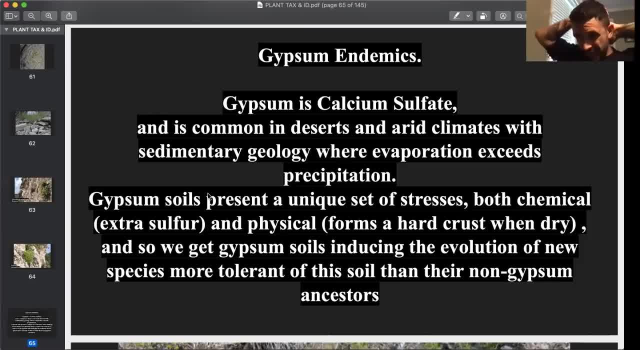 so gypsum uh is like limestone in the way that it weathers and uh reacts with acidic rainwater really easily. it becomes mobile, if you want to think of it like that. it's you know it dissolves readily in water, more so than limestone does. it's it's become, it's like a mobile uh uh mineral. you. 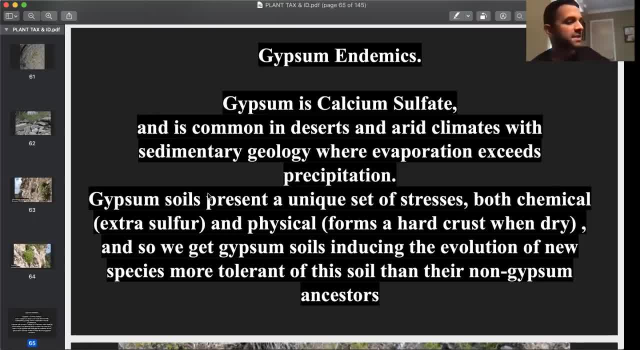 know, mobile with water, so it'll get weathered with rainwater and then get deposited out somewhere else when that rainwater dries. so it's originally, uh, the result of shallow seas. it's a sedimentary rock, the result of shallow oceans, limestones associated with deep oceans, but uh, you know, in in areas you mostly get, 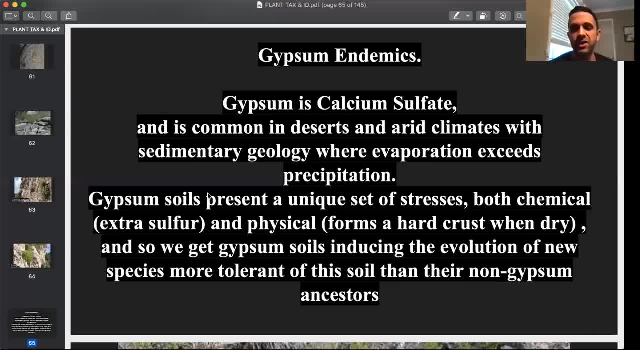 the gypsum where you're going to see. it is areas where evaporation exceeds uh precipitation, where it's hotter and drier and that water evaporates more than it. it falls in the form of rain. right, because if you got, if you had gypsum in like florida, it would just 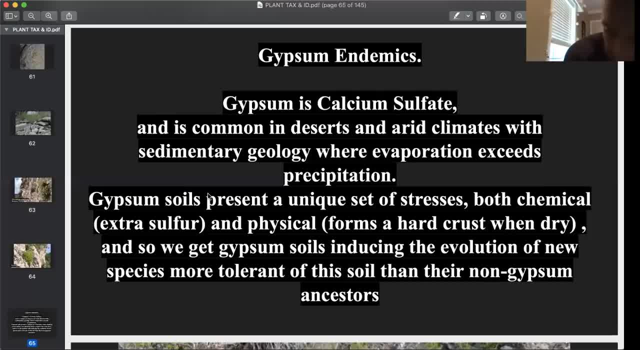 weather away and that would be it. once it was exposed due to plate tectonics or the layer above it getting eroded, the geologic layer above it getting eroded, it would just weather in the it corrode in the rainwater and just it'd be gone. that'd be it. but in areas where it's so dry you. 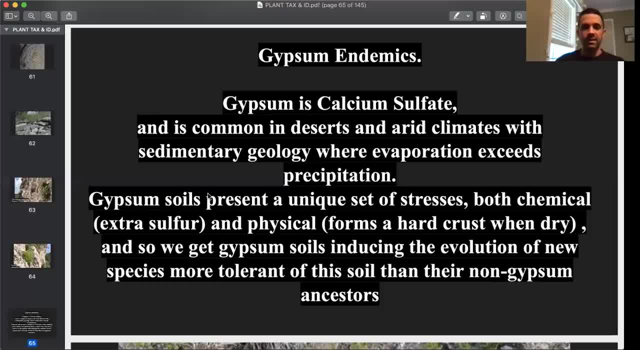 don't get much rainwater. that's where gypsum sticks around a little bit longer, and so this is fucking cool. there's a huge gypsum belt north to south of here and it's like it's like it's like a. there's a huge gypsum belt north to south of here and it's like it's like it's like a water. 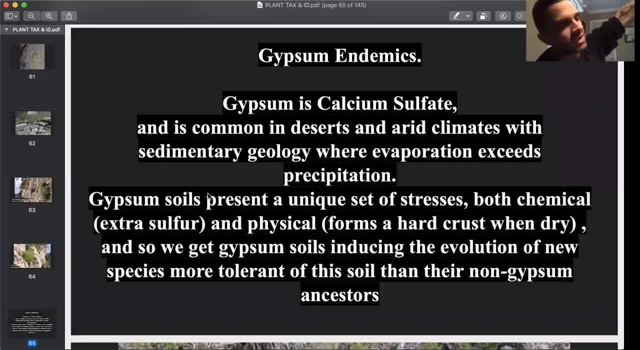 gypsum belt, sporadically occurring from like northern new mexico, just northwest of albuquerque, all the way down into nuevo leon, through coahuila, the mexican state of coahuila, etc. and and over time, what that has done the plants is fucking fascinating. it's similar thing as serpentine. 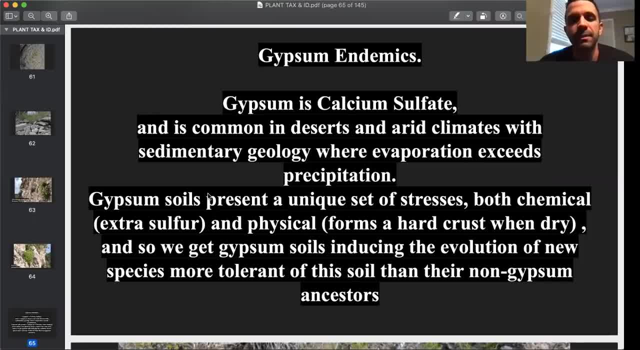 and sandstone and limestone, you get plants that are gypsum endemic. some plants, uh, will grow off gypsum and but they'll tolerate gypsum. and then there's a handful, a lot of a lot of species that actually only grow on gypsum. they're endemic to gypsum. the question, of course, is: do they grow? 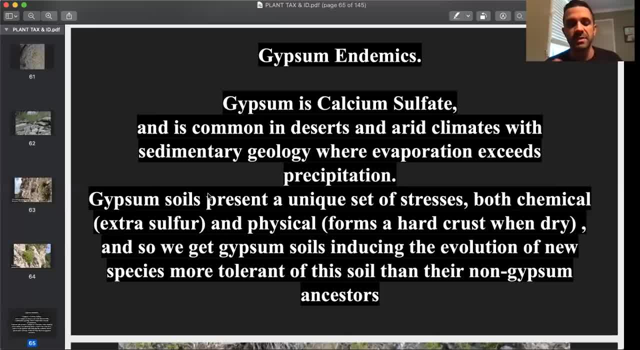 there because they need the gypsum, or do they just grow there because nothing else can compete? gypsum soil is so fucked up and there's no topsoil there and it forms such a hard crust when it's dry then nothing else can grow there and so these have a competitive advantage. it's, it's mostly. 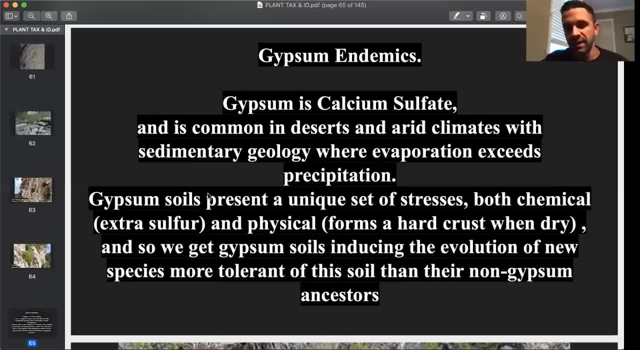 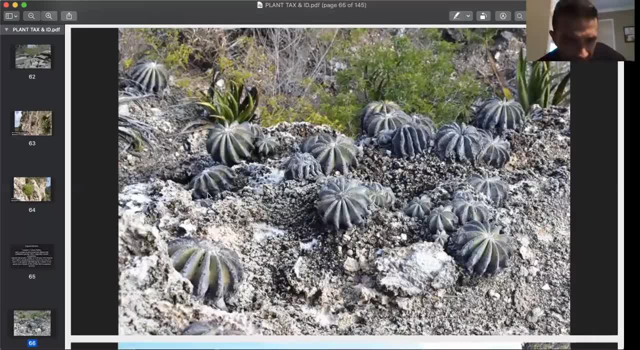 the latter. they have a competitive advantage because of their adaptations to it, but there's exceptions anyway. moving right along, here's, uh, everybody's favorite super rare cactus species only discovered, uh, a decade or two ago. this is astichium hintonii. looks a lot like geohintonia. 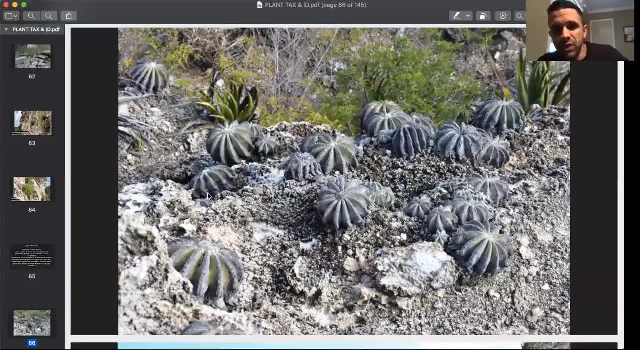 mexicanum, which it is sympatric with. but you could see here it's growing on what looks like someone, like a fucking cement truck exploded right. it just dumped this stuff out. there's no soil, these things are just growing straight out of the rock. it's wild and this is a kind of a rare case. 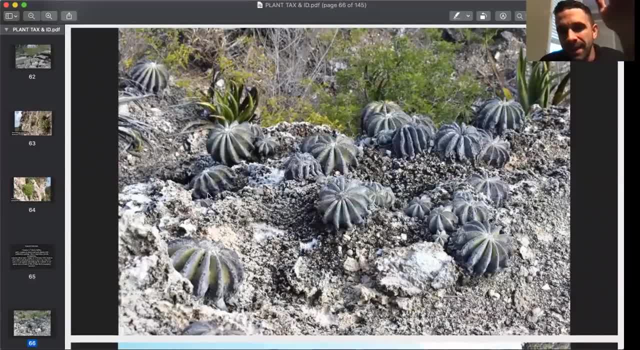 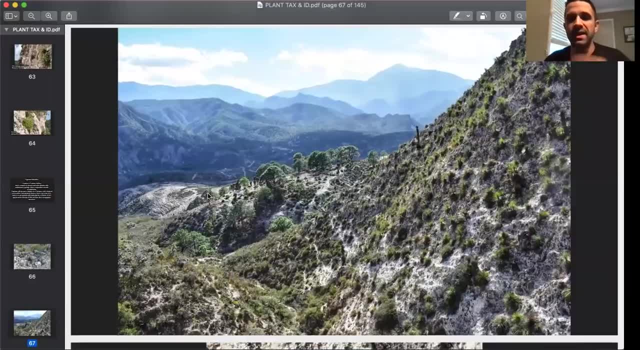 they're growing on almost a horizontal substrate right here. but uh, you know, in most cases these grow out of fucking walls. they grow out of rock walls. the craziest shit i've ever seen. here's the habitat. you got pinus arizonica in the background. uh, in the foreground you got a lot of yucca i. 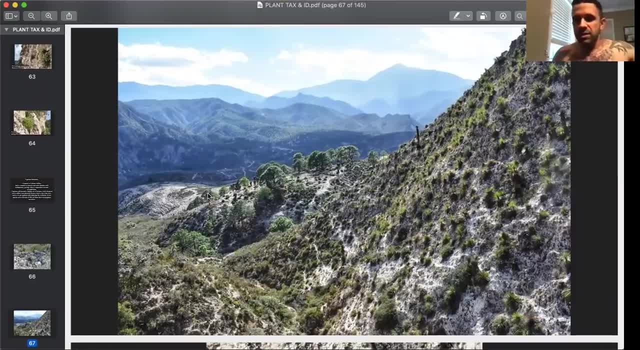 think it was yucca carnerosana, a bunch of other species that are adapted to, to growing on gypsum, but you have almost, uh, you know, like a 70 degree slope of fucking gypsum. it's wild, um, you know, and it's at the correct latitude for a desert. it's in the rain shadow. 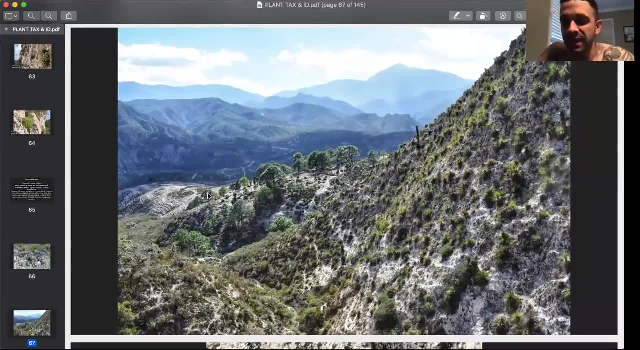 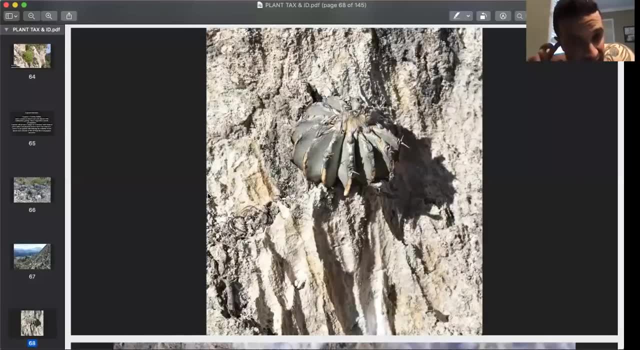 of the sierra madre oriental, most of the rains coming from the east, from the atlantic ocean to the east, from the gulf to the east, etc. uh, here's geohintonia mexicana, other species that grows sympatric with it, that is, they grow together in the same area and you can see that gypsum just. 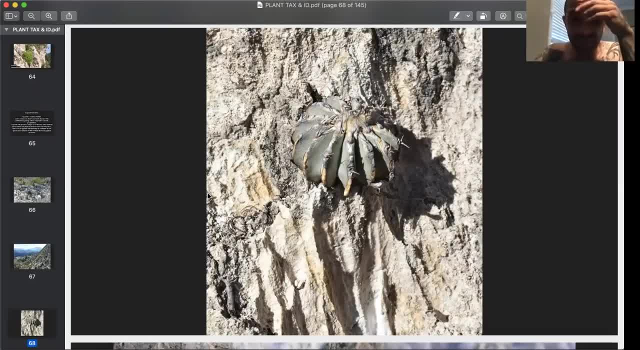 corroding again. you see that dimpling, you see that ridging the way it reacts with rainwater looks a lot like that asthecium but- and you couldn't tell from the photo so much- but if you look at that that looks like half a cd, a half a compact disc coming out from that central. 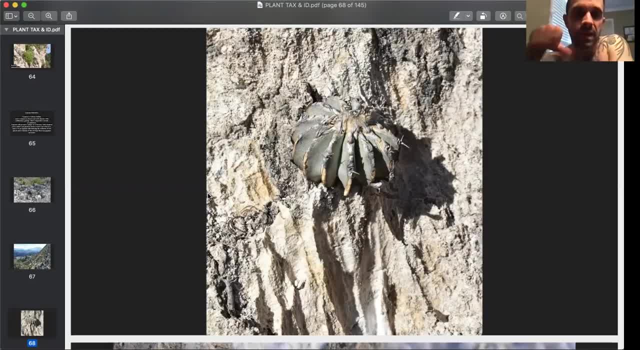 area. each one of those ribs doesn't have uh ridges on it, right? if you look at the other asthecium, it does, and of course, when they bloom they look radically different. the flowers look radically different. there's more geohintonia. you could see. uh, what is that? i don't know if that's. 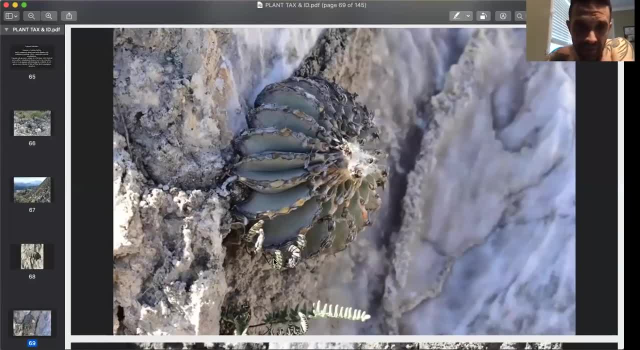 a myriopteris, or a palea- that fern down there- or gyrocosma, another cool xeric fern, the xeric ferns with a p pterodactyl- really cool family. uh, i believe it's all over the world, but especially the north american deserts have some wild fucking members of that. so there it is growing out of. 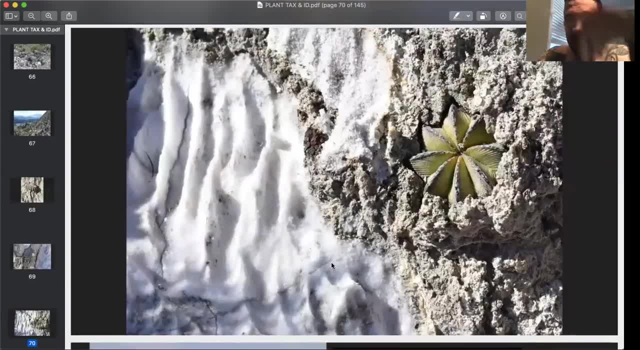 vertical rock wall. this thing gets poached a lot too. there you go. you could see those ridges on the individual ribs of asthecium cantonii. and look the fucking rock here. it looks like. it looks like a salt, lick like it's. so it it. and you know gypsum is a salt. i mean it essentially, you know. 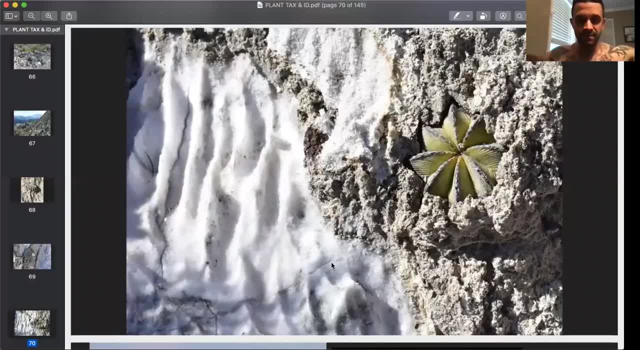 as salts are classified in the field of chemistry. you know it's and it's super soluble in water, so you can see it looks like it's nested in that rock. uh, my guess is that that little nest kind of grew around that uh seedling right there. that seedling is probably 20 fucking years old. that's it, and 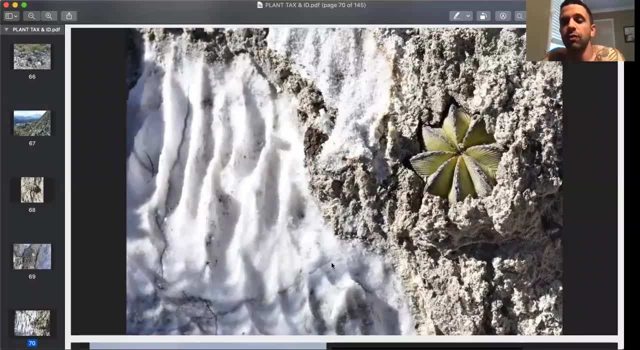 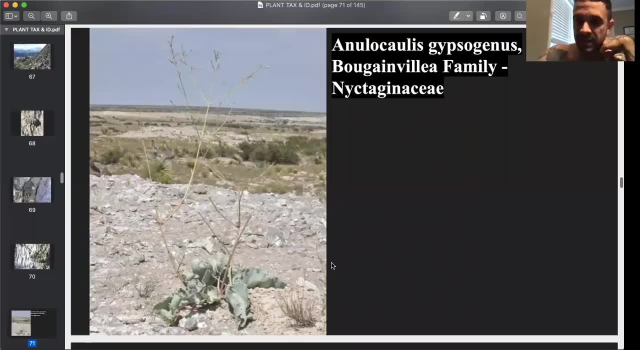 it's like smaller than a penny. so these things grow really slowly and they live for a long time. so it's more you know, more testament to the desert's fragility and how easily people can fuck them up. okay, this is from uh, southern new mexico. this is that a new localis gypsogenus. families: nyctaginaceae, the four o'clock family, same family as bougainvillea, which is almost a horticultural atrocity. you see, you know, fucking home depot plant right there the bougainvillea, the home hummingbirds love it. it's cool. it does provide nectar for them, but whatever, but it's. 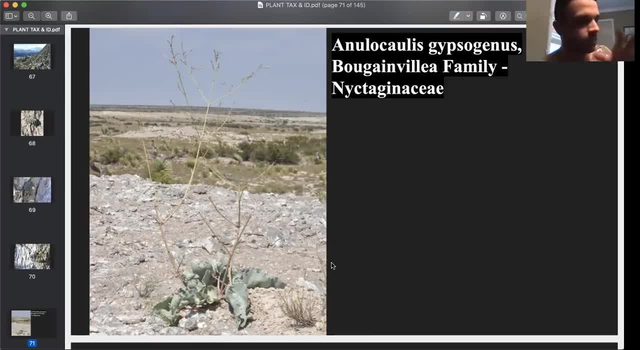 in that family, nyctaginaceae, and nyctaginaceae, of course, has its own synapomorphies. you know, they have petaloid sepals. they don't have true petals. they've only got one series of those floral appendages, that being the sepals. but don't focus on that, just look at how. 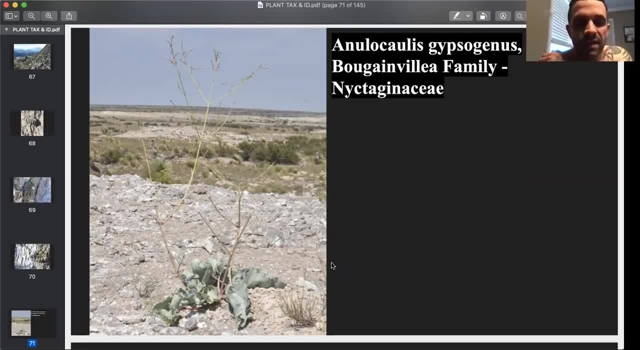 look at what, uh, the gypsum substrate has done to the evolution of this plant, which is a gypsum endemic, over however many millions of years. it's got these leathery like blue basil leaves, really tiny flowers on these stalks that you know have such a small surface area, uh, so they don't lose. 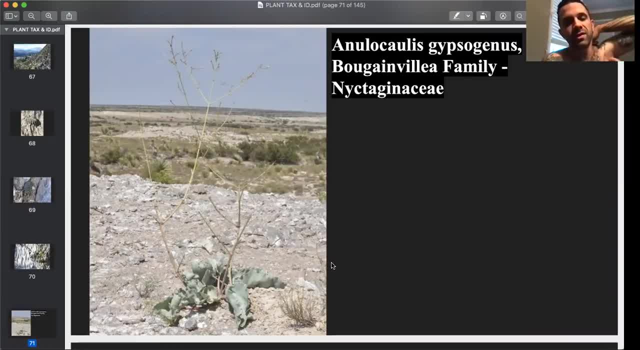 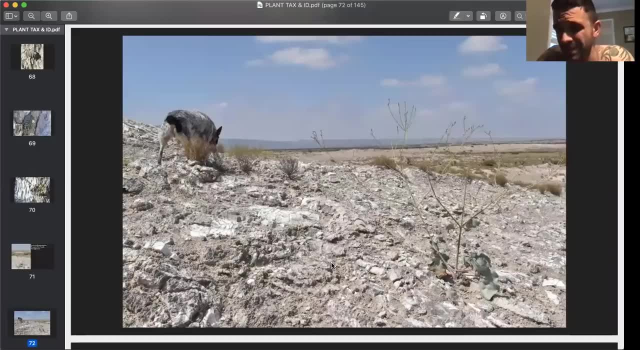 so much water, i mean you can barely see the stalk. you know, once you get 20 or 30 feet away from it, you can barely see it anymore. it's just so thin, um, they're perennials here. really cool fucking. i saw this thing and i was like this is the. 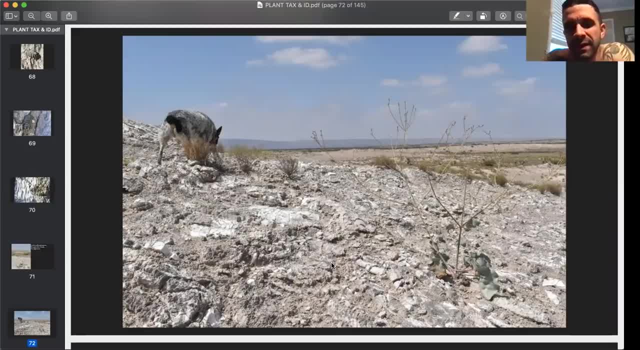 weirdest shit, and the reason we found this is we were driving, uh, north. it just crossed the texas- new mexico border and we saw this area and we're like what the fuck? that's crazy? barren environments always produce some really cool plants. if it's barren, because it was. 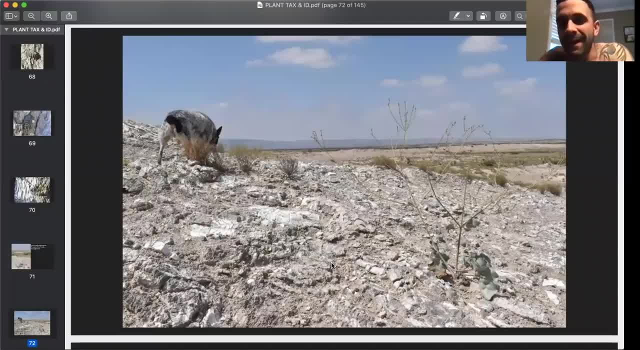 naturally barren, not disturbed or bulldozed by people. uh, there's always going to generally be some cool plants there, if it's barren because it's serpentine, or if it's barren because it's gypsum, or barren because it's sand dunes, whatever. so we went there and we found a ton of cool plants. 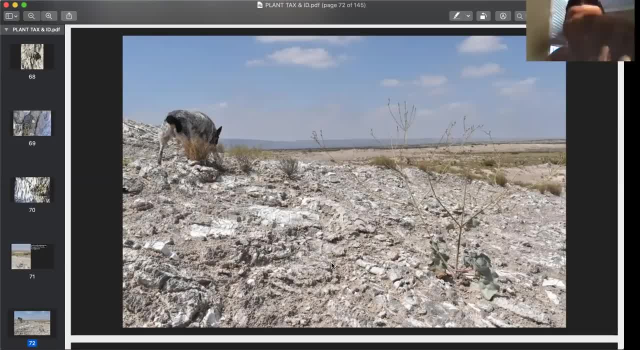 we'd never seen before like this. anulo, call this and look at the soil again. you get that vinnie mixed a bad batch of concrete thing. going on, it's kneeled down on this shit. it tears your knees up really hard, but when it's wet turns kind of spongy and uh and comes to life. there's those. 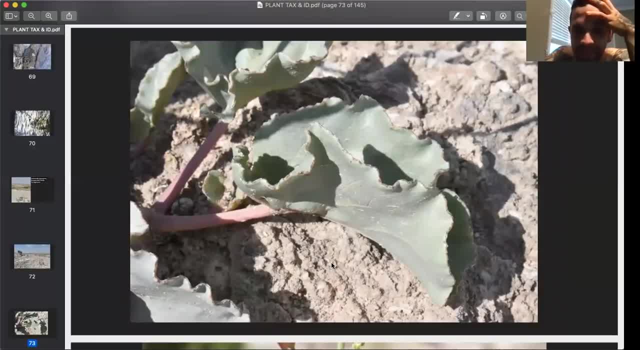 leaves- coriaceous is the word for that- leathery, leathery and waxy. you'll notice that no hairs, they're glabrous, but they're. they have so much wax, they're so much hair, they're so much hair, they're such a blue color to them. you know they can reflect a lot of that light. another edit now. 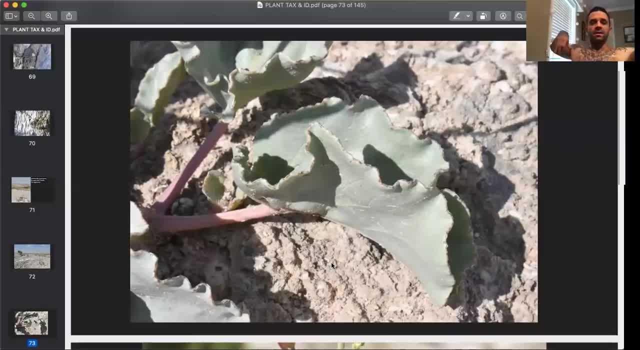 that red on the uh, on the stems there? would that be example, an example of that pigment you were talking about earlier? yeah, betalains, exactly yeah, so betalains and the rest of flowering plants, uh, the equivalent of the betalain pigment in every plant that's not in caro phylales is generally: 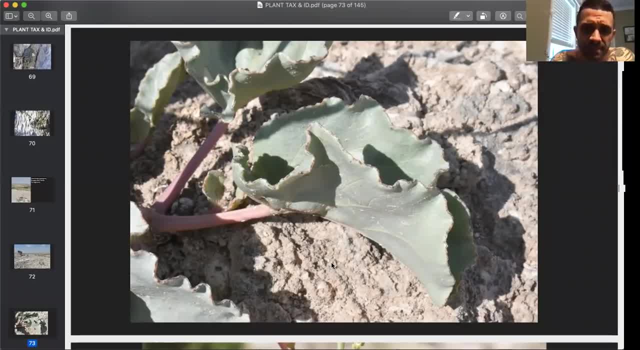 anthocyanins, uh, carotenoid pigments, and they look different. they just have a different look. i don't, i know that's kind of a shitty way to put it just looks different. but if you really look at the, the color of that red pigment, it's- i don't know how to describe it- it's often, maybe kind of more. 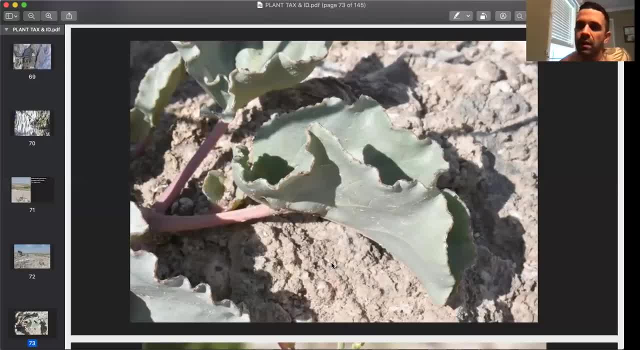 pink, uh, more. uh, the way it reacts with visible light when you're looking at it, the way the visible light reflects off of it, is different than if you look at like a strawberry. like the pigments in a strawberry, that's anthocyanins, carotenoids, uh, the pigment on, like the red. 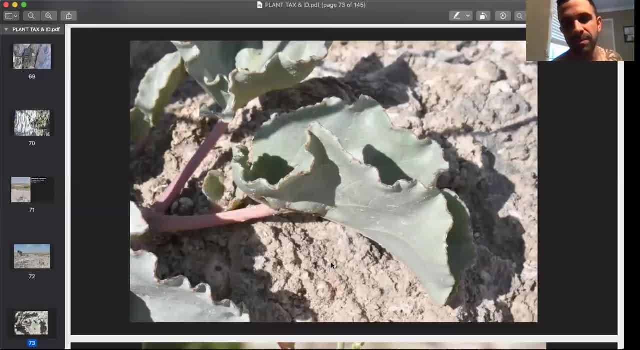 margin. the poinsettia is another pigment that's kind of like a red pigment, that's kind of like a good example, like they, the pigments are notably different from betalain pigments. okay, so, but remember, like you know, i think like five percent of the order, caro phylales doesn't produce betalains. 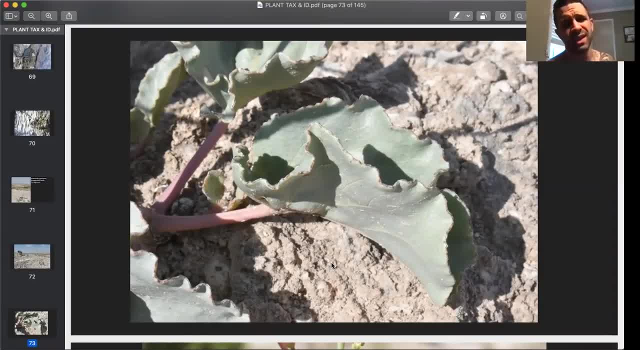 they, just they lost it. i don't know if they evolved anthocyanins. i think they evolved anthocyanins on their own, secondarily, but you know, these are all just the molecular toolbox that plants have to create these things. and so, uh, betalain proved adaptive enough, and i'm not exactly sure why. 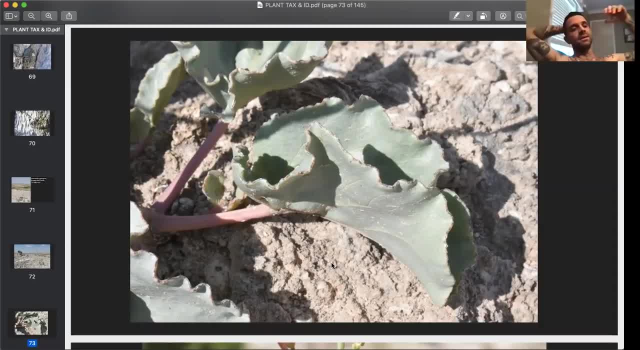 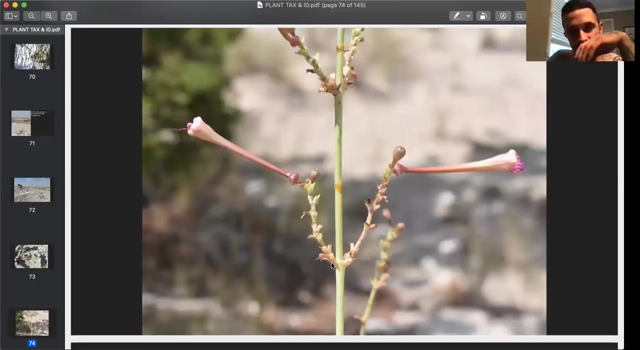 but it proved adaptive enough that every uh descendant of the, whatever lineage, whatever ancestor, that pigment evolved, and proved adaptive enough that every descendant it stuck around. you know almost every descendant, so. but yeah, you could see the betalain pigments right there. that's again cario phylales, the order of beets and cacti. there's the flowers tubular uh, almost. 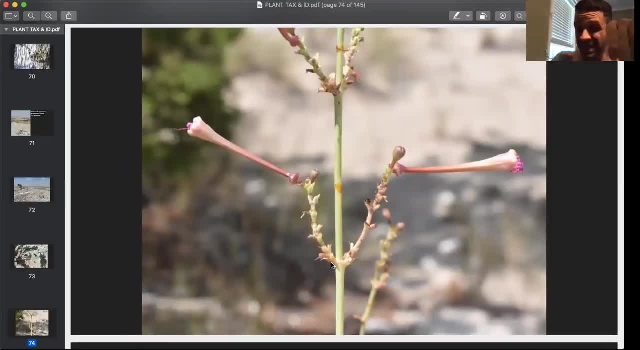 red, pollinated by sphinx, moths or hummingbirds, something that's got to get in there, right, because all flowers produce nectar at the base. is it attractive? not all. some orchids don't, other, you know other plants don't? they rely on mimicry, or some orchids will even produce pheromones to. 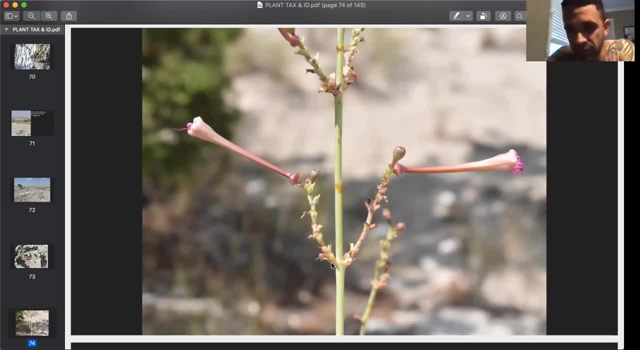 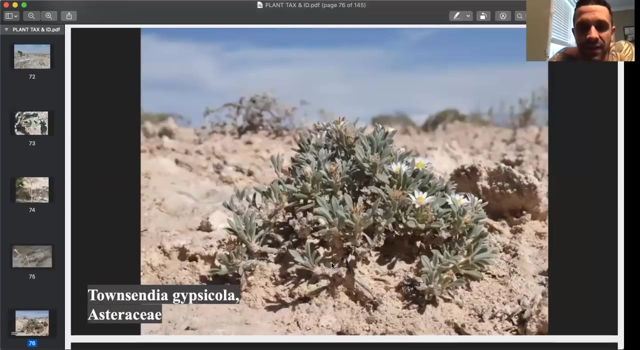 attract pollinators, but generally 95 of flowers produce nectar, so the nectar is in there. get a little food reward for whatever pollinates that, probably hummingbirds in this case, or sphinx moths too. they got a long proboscis. more money shots to that another. this one is: 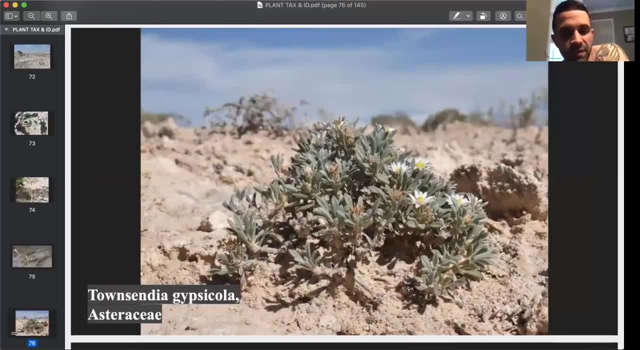 from up. uh, this species is from up near the gypsum areas off of uh Northwest of Albuquerque- maybe it's north of Albuquerque, I forget. it's a popular mountain biking area, thankfully not like a dirt bike or ATV area, so it can't get too up. but uh, uh, this time Cindy, a gypsicola again. 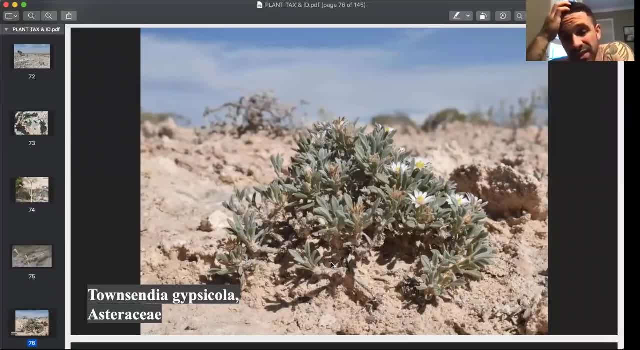 another gypsum endemic, not only from a handful of spots, never seen it growing off of gypsum town Sandy is a cool genus too. it's got quite a few species in it. uh, all Western generally high elevation- I mean this is the elevation here- was like four or five thousand feet, whatever elevation. 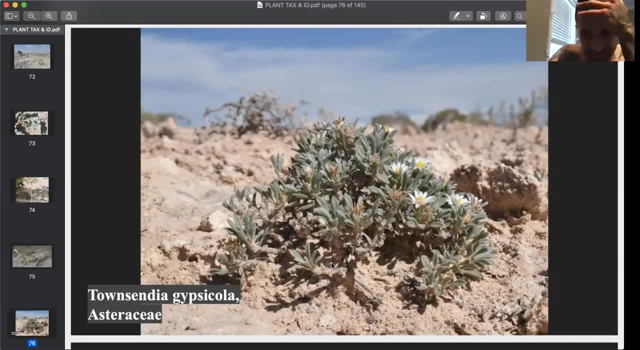 Albuquerque's at um, but uh again, yeah, just another cool variation on a theme: the flowers you know, bright, white a lot of other town standards can have, like orange or purple or pink flowers. this one, uh, has white. it's a weird thing too, you'll notice. sometimes too is like plants that. 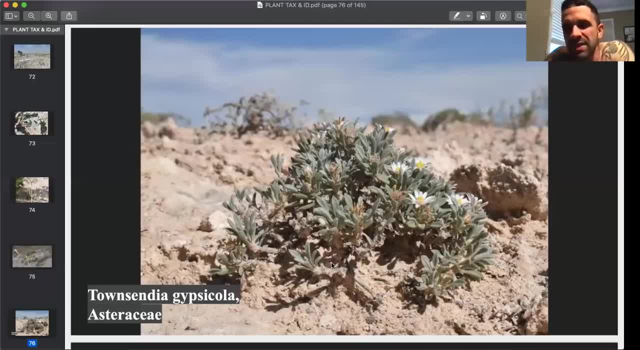 grow on these white substrates, you'll often see more white flowers in plant species than not. so like same thing with limestone: you'll see limestone endemics that have white flowers. it's really bizarre. I'm not sure if that's just the coincidence or if there's an adaptive benefit. 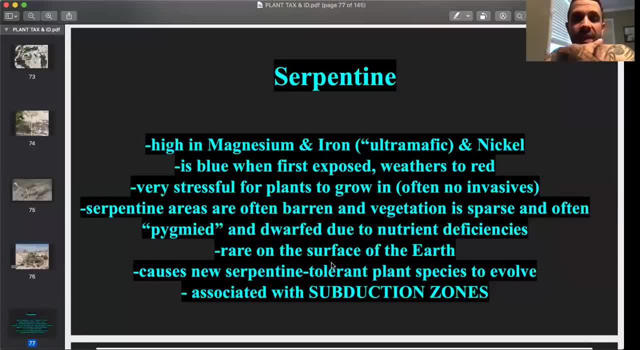 and uh producing white flowers or whatever. um, anyway, serpentine, one of my favorites. so serpentine, this is where geology and botany really, and the theory of evolution really come together. you know, uh, so serpentine, uh is a relatively rare rock on planet Earth. 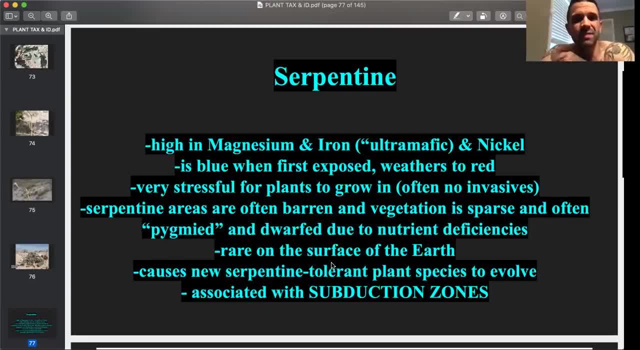 in New Caledonia, you get it in Cuba, you get some, even some in Texas, but it's not enough to really affect the evolution of the local flora. it's a small exposure and you get some in Pennsylvania and you get a ton in California. because relatively recently- and I say that in quotes- 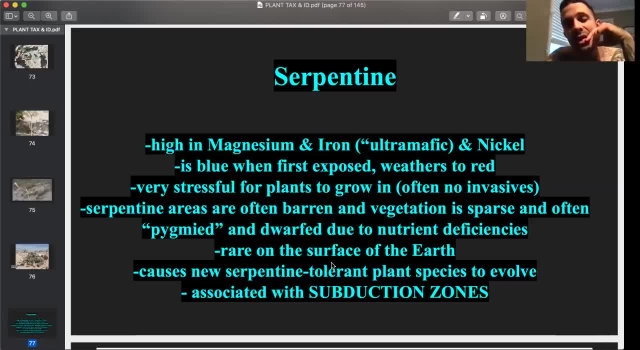 like 20, 30 million years ago, there was a subduction zone off the coast of California. gypsum, or serpentine, is associated with subduction zones. you can basically uh, synonymize the two. if they there's serpentine there, it it had to get there by either being subducted or abducted you. 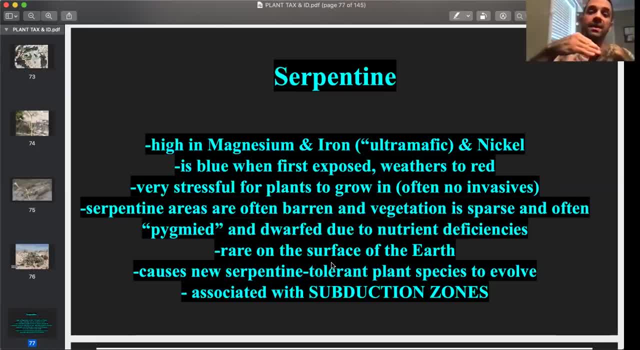 know, slapped on by a descending oceanic plate beneath the continental plate. this is another thing to read up on if you want to learn geology, because it's how the convection currents in the Earth work and it's how plate tectonics work. subduction, uh, the opposite of 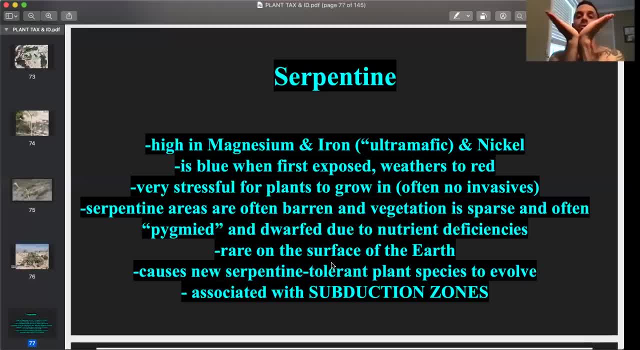 subduction zones or seafloor spreading centers where new rock is being created and pushed out in a different direction to the left and the right. um, so that's the thing to read up on. obviously can't get into it too much here. I'll around and try, but she got her porch time too. 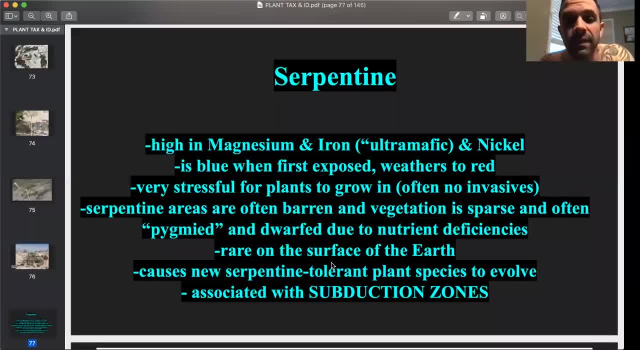 is that a question or did someone forget to mute their microphone? I've forgotten mute sounds like someone forgot to mute anyway. uh, okay, so serpentine, the things you got to know- high magnesium and iron- that's the chemistry right there, and you get a lot of nickel. so, uh, you got these harsh chemical situations. uh, magnesium and 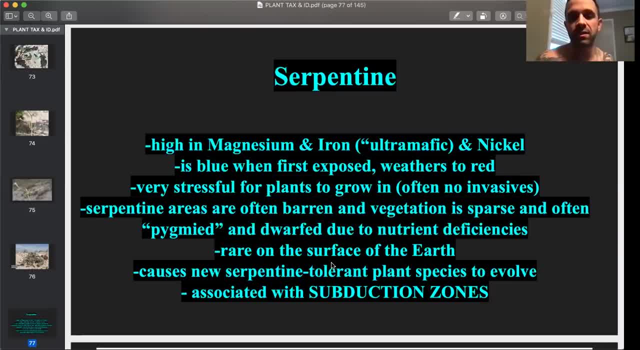 iron in excess amounts, and especially nickel, can be hard for plants to grow in the heavy metals. okay, they're also serpentine. soils are deficient in calcium and nitrogen. I mentioned all this in the videos. if it's redundant, speak up and let me know. um serpentine areas are often barren in the 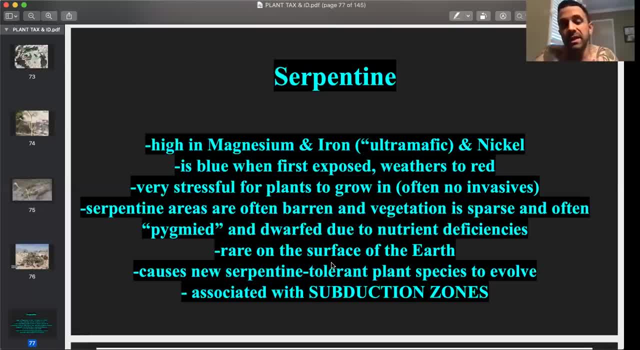 vegetation is sparse and if the where there is vegetation, it's often pig meat it grows- it's dwarfs, compared to if it's a plant that can grow both on and off serpentine. uh, that's tolerant of serpentine, but it's abundant off of it. you know, you'll see, the versions on serpentine are dwarfed. 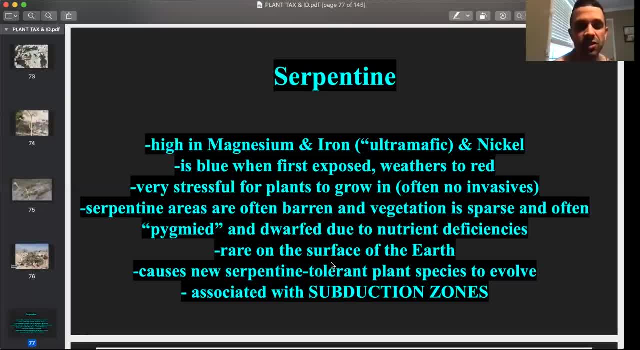 and I got some really nice examples I'll show you of serpentine in the deserts of Baja California. sir, the elephant tree- one of the another reason not to use common names- refer to two different plants, but the elephant tree that's in the poison oak and mango family. 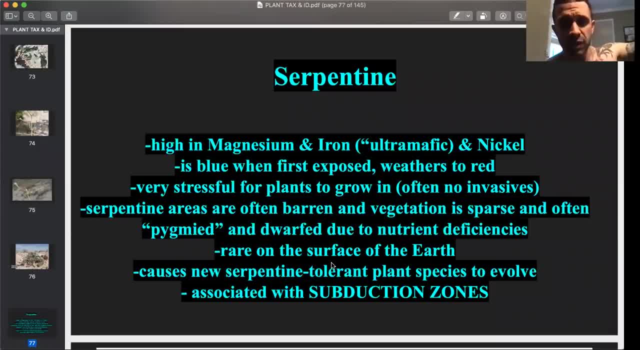 will grow if it's old enough and conditions are right. sometimes 20- 30 feet tall, uh, in other, like on volcanic rock, but you take it to serpentine. it'll tolerate serpentine, but they barely get taller than two or three feet. so you end up with this like sprawling- really crazy- bonsai. 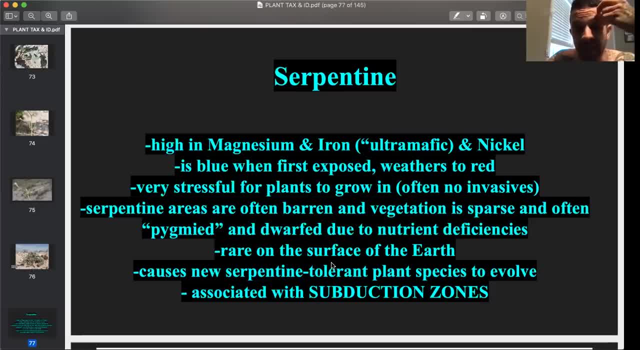 succulent tree. so, uh, anyway, serpentine's around the surface of the Earth. that's why you need it needs to get basically kicked up by a subduction zone. uh, it's mostly, uh, serpentine's basically metamorphous peridotite. peridotite is one of the main constituents of the 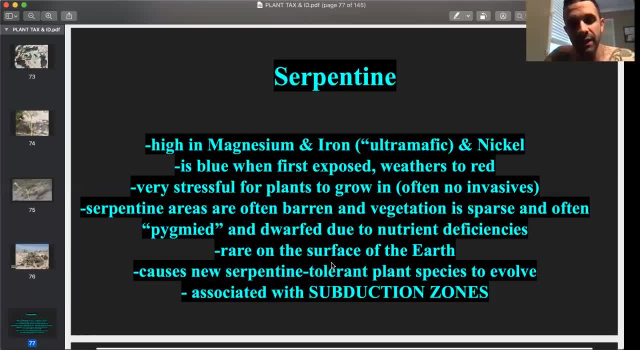 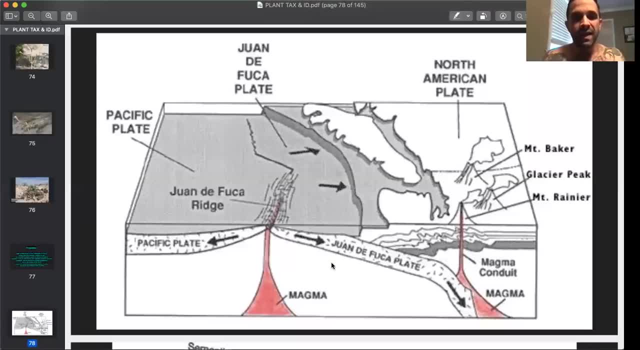 mantle so deep. these are normally deep rocks, okay, which is why, again, why it's rare and why it's associated with subduction zones. there you go, you got a nice little uh example of what's going on in the center, near where it says Juan de Fuca Ridge. that's a seafloor spreading Center, the opposite. 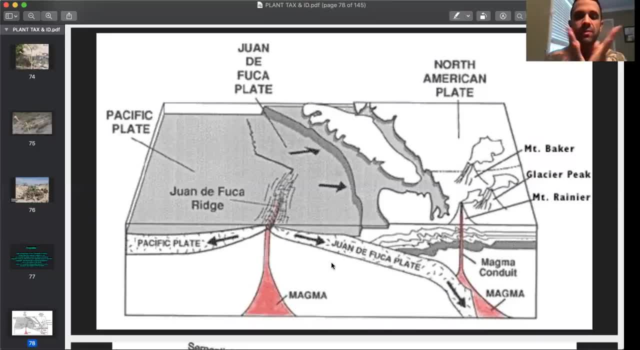 of that uh is the subduction Zone. so the magma comes up, new crust is created at seafloor, spreading centers- oceanic crust is and it goes back in to the depths- and a subduction zone. so, like convection currents in a pot, they come up at the center, then they spread to the sides and they go back down along the sides. 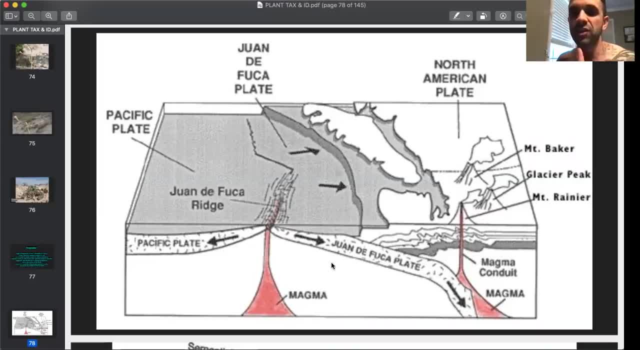 of the pot, etc. convection current- that's what is going on here. convection currents on a much more grandiose scale, not of water, but of rock. that's so fucking hot. it's liquid or plasticky. uh, in many cases, if it's got a lot of silica, it's plasticky. it doesn't really melt. it's not fluid like basalt. 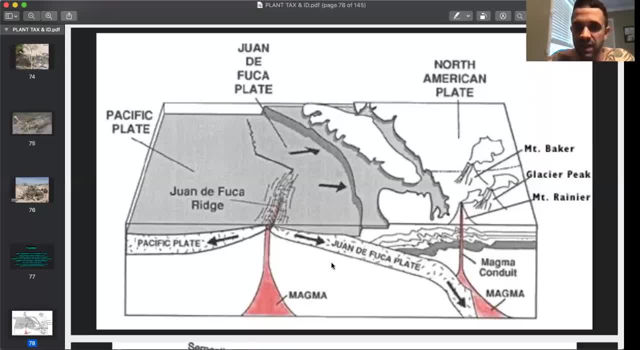 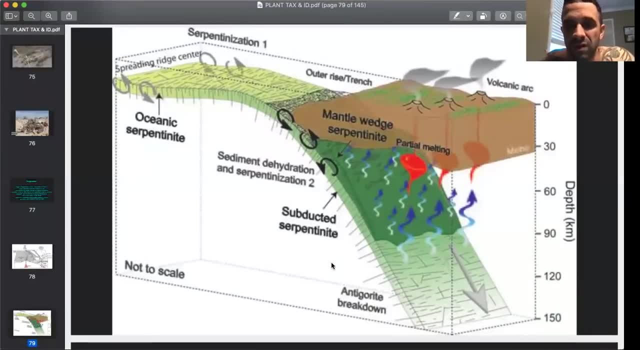 would be. silica means viscosity in terms of igneous rock. so anyway, there's that. don't fuck yourself up too much on this, but just grasp the general concept. uh, there's subduction zones, also called cause volcanism, too. this is from a paper on serpentine. uh, you got that. um, you can see where. 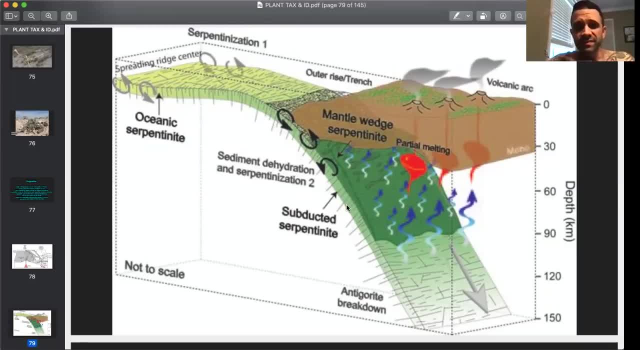 serpentine is created, so, or one of the places it's created. uh, it's that peridotite. as it gets buried again, as a subducting plate starts to go down, it gets heated up, ie cooked, but there's water present in it. so it's a little bit more of a peridotite, but it's a little bit more of a. 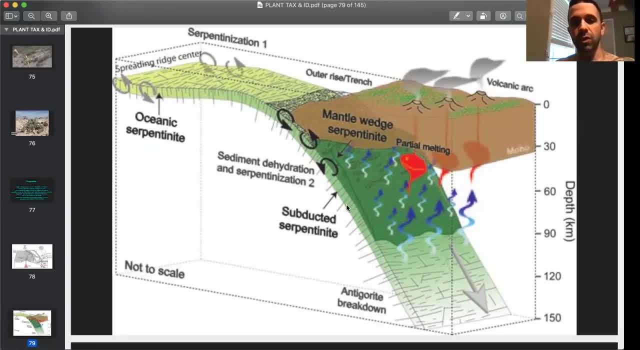 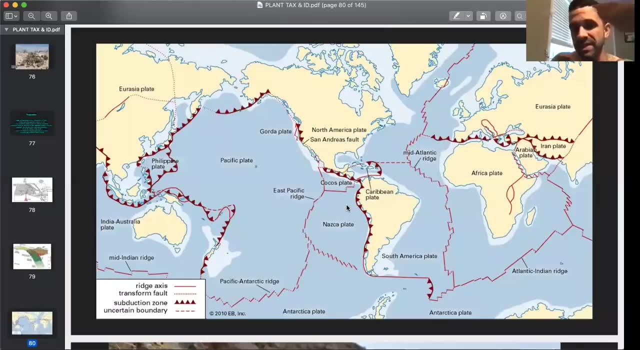 so it becomes a little less dense. uh, it's a more lighter, brittle rock, and then, of course, eventually it gets pushed up to the top. so tectonic map. i always tell people this is more important than geopolitical boundaries, because this is the fucking, this is the tools you got on. 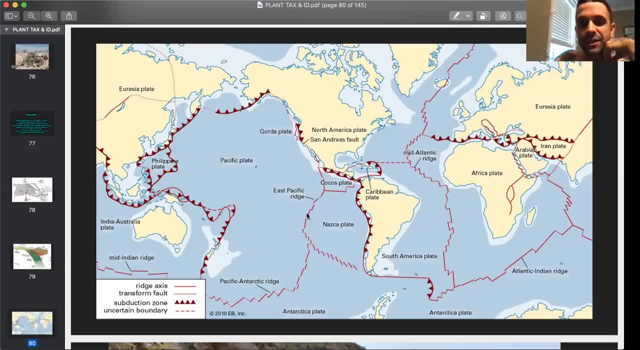 the on plate tectonics. right, the dashed lines with no triangles are the seafloor spreading centers. the uh, the lines with the triangles are the subduction zones. uh, you got transformed boundaries in between, like the kind of the way a baseball is stitched right because it's a the. 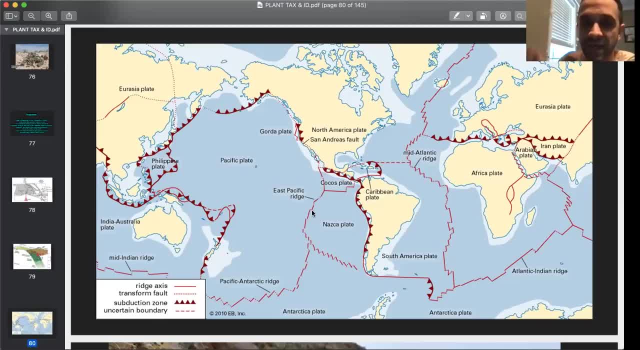 globe is spherical, you can't get straight lines. they gotta, they're gotta be breaks at some point. so that's why you get these kind of stitching zigzags. you'll notice here on the western coast of north america, just below uh, where it says gorda plate, where the triangles are. that's the. 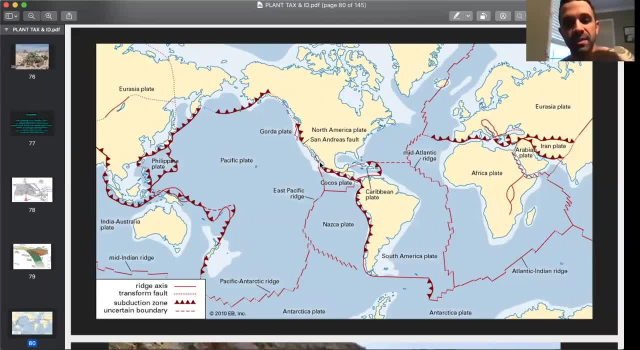 san andreas fall, you'll see a discontinuity between the subduction zone- the triangles near the cocos plate- and subduction zone- the triangles near the gorda plate. that discontinuity is the san andreas fault and which is a transformed fault, and to have a transformed 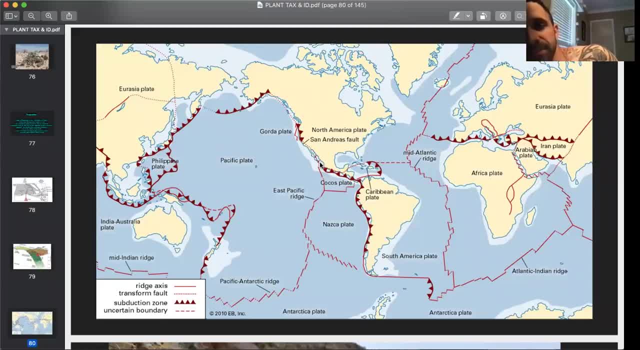 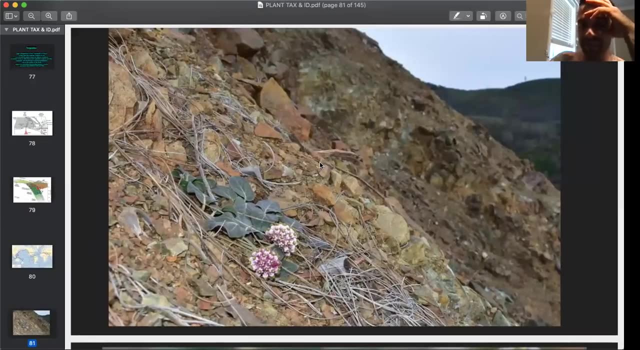 fault that big on earth is pretty rare, okay, and it's caused, but it also causes some really cool things geologically. in california you get rocks that have been transported by that fault. you know 200 miles from where they originated. some wild shit anyway. uh, don't fuck yourself up on that. 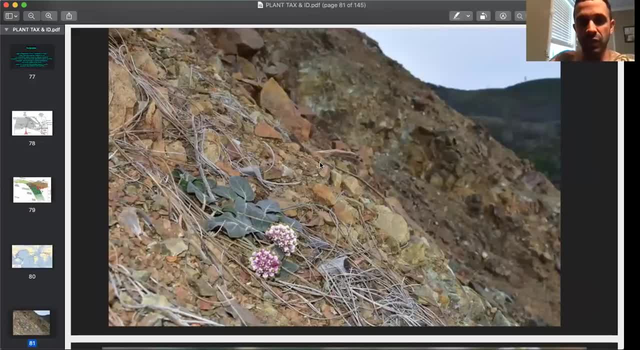 well, let's just look at what serpentine does to plants. so here's what serpentine does to a milkweed, right? so because serpentine is so toxic, it's so toxic to the milkweed. it's so toxic to the milkweed, it's so toxic to most plants. it causes these barren environments and and these desert-like 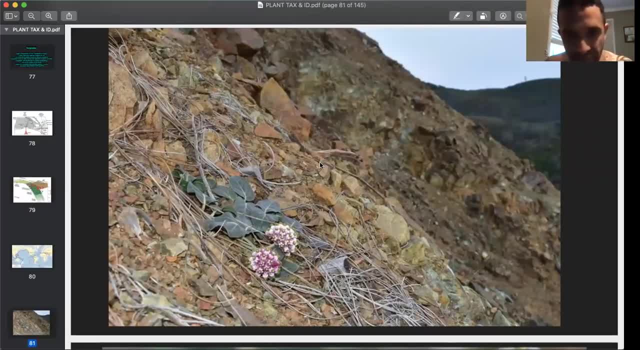 environments and what are otherwise, areas that get enough rainfall to not be deserts, but they're still barren again, because that soil chemistry is so fucked up: there's not much calcium, not much nitrogen and there's a lot of heavy toxic metals in there. so this is how, uh, the genus. 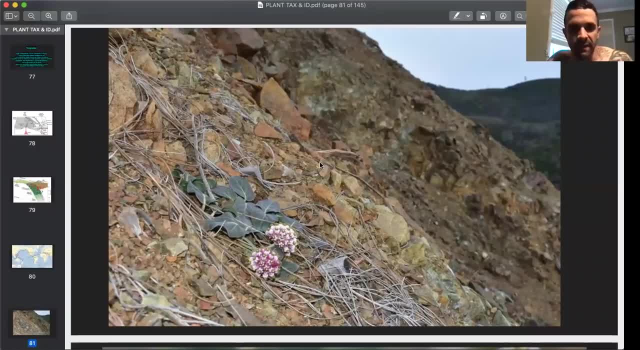 asclepias the milkweed responds to it one of the ways. uh, this is asclepias solanowana. it's a super northern california endemic and you'll only find it growing on serpentine and it doesn't get tall, it just lays prostrate on the ground. of the adaptive benefit of that there's, you could come. 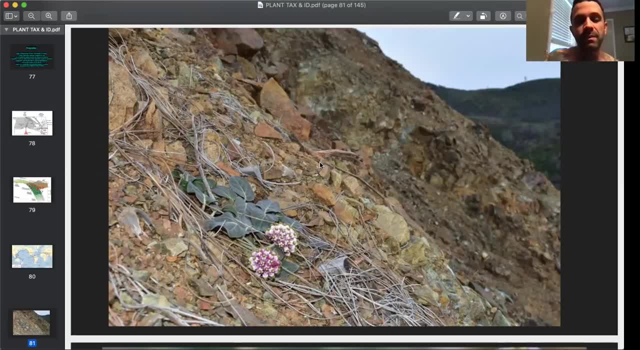 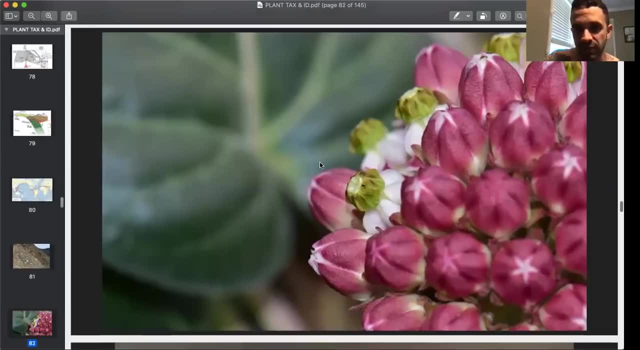 up with your own theories. you could imagine whatever benefit there might be in that. that's part of the fun and learning about this shit. but this is uh. there you go, and then those flowers again are just so fucking bright, so like spectacular. so you got, you know, pink petals. 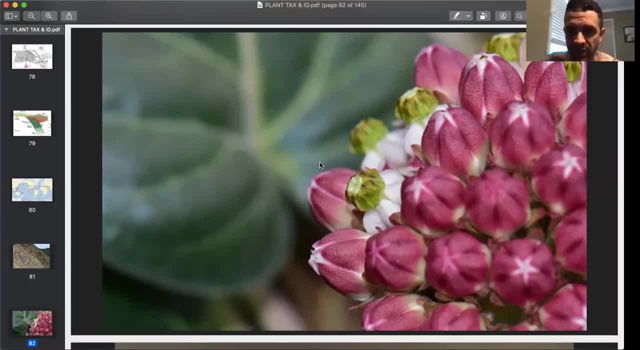 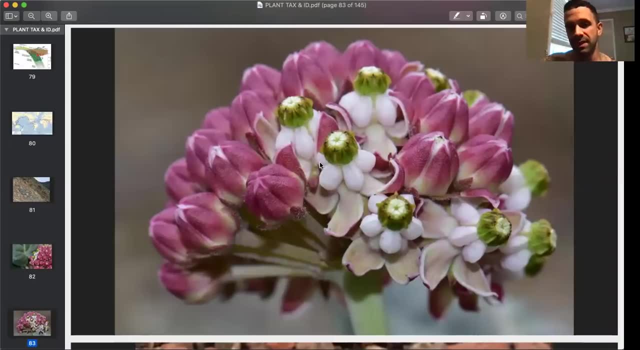 the sepals are already reflexed, can't quite see them. and then again, this is just the variations on a theme, uh, that geology can, can you know, throw into the mix with plant species. so really, really, unlike other milkweeds, here you don't have any horns, the hoods, 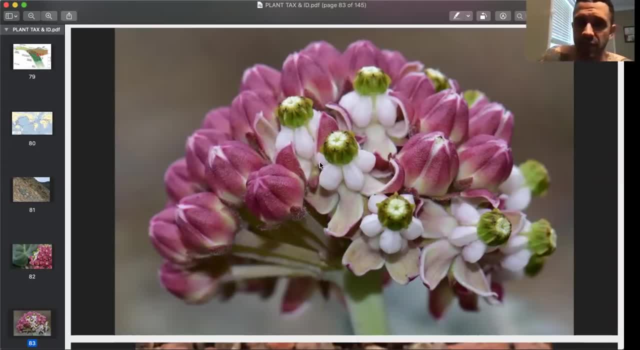 those white things, those teeth looking things, are not hollow. the, the corona itself, the, the, what you call maybe gynostegium is, is so much it's almost at a different level than the, the hoods, normally the hoods surround that, but it's not like that. it's not like that, it's not like. 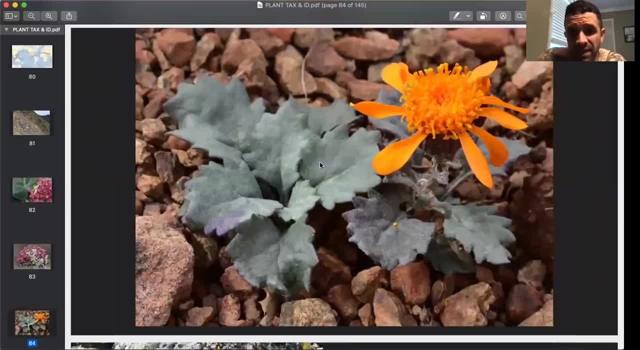 that gynostegium. it's just a fucking weird plant, man. another plant you only see on serpentine: pacara greenii. uh, things you'll notice about serpentine plants. they often have these like psych ward green colored leaves. uh, you know, i'm not sure if it helps them blend in with. 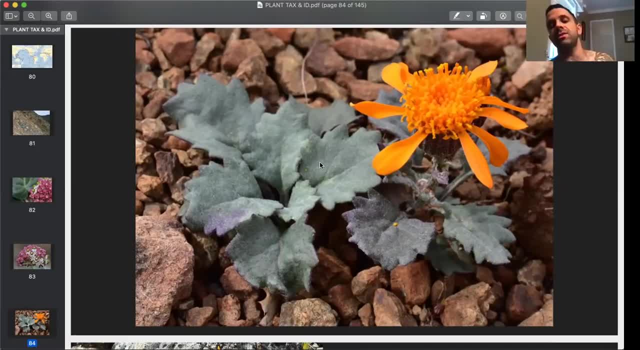 uh, serpentine, the serpentine, the blue serpentinite minerals, or what blue and green serpentinite minerals? serpentine is blue when it's first exposed. it weathers to red later on as the rock is oxidized. remember it's got a lot of iron in it. so here's pacara greenii, the minion of little. 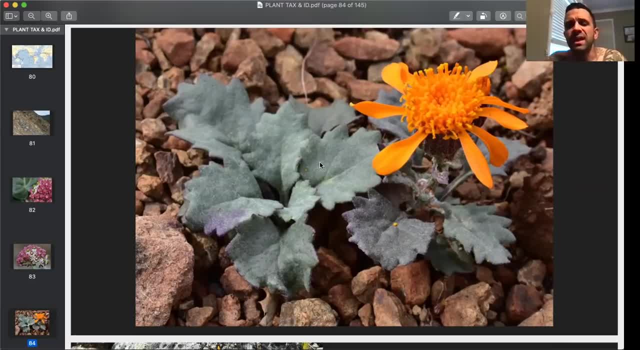 fucker, this one's only like four feet four inches tall. they can be upwards of uh. i've never seen them taller than eight or ten inches, but either way. but that bright orange flower, one of the only composites, one of the only members of asteraceae to have a bright orange flower, at least in north. 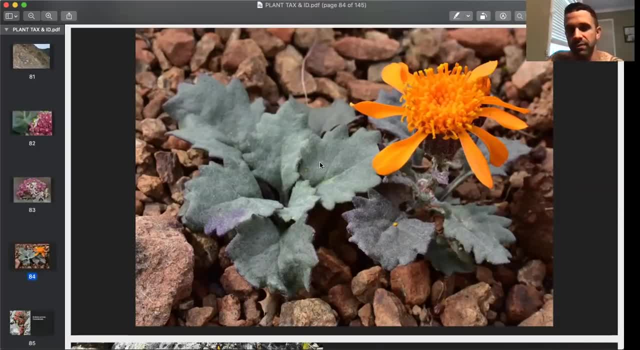 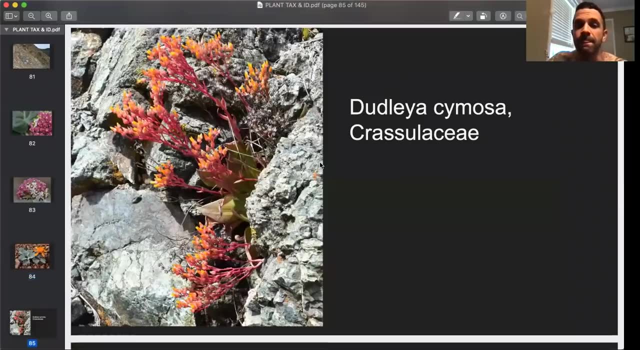 america. and again, you'll never see this growing on on regular soil. i've only ever seen it on serpentine- supposed to be a pain in the ass to grow too. i know a guy at the botanic garden is going to grow it. dahlia simosa. this is not a serpentine endemic, it just tolerates serpentine. 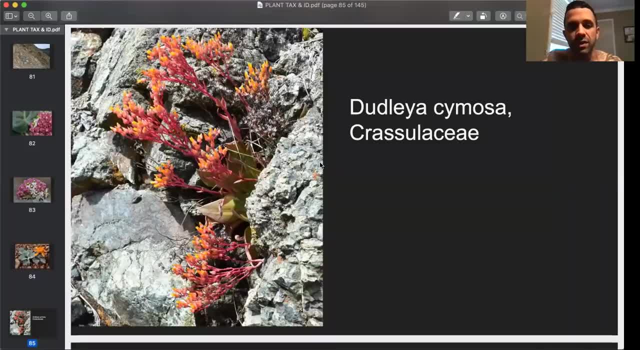 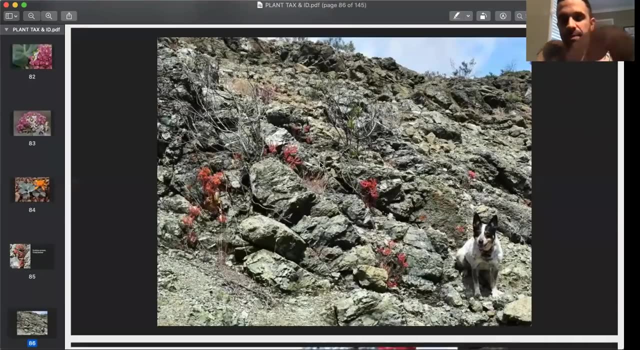 uh, who knows if it'll eventually evolve into a serpentine endemic species, whatever. but because it's intermediate, because it's tolerant, you can see, we're kind of afforded a glimpse of, you know, the intermediate evolution maybe, who knows? uh, the thing, i the reason i put this here. 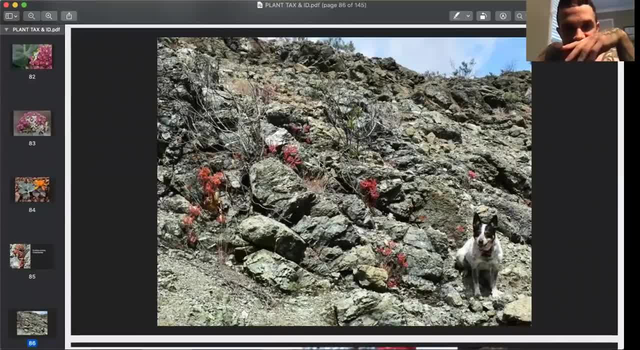 is. i mean this: these things blend in so well with the rock. um, this population does. dahlia simosa is a common dudley. you'll find that, like i said, growing off serpentine, but here it was growing on serpentine. and, uh, this population, if you were to compare it with a population growing. 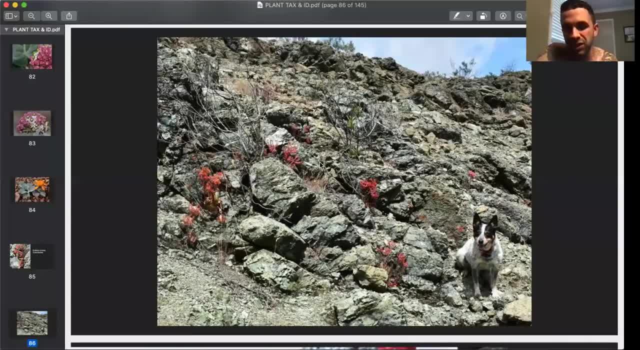 off of serpentine. it's not enough. it's not different enough to be a new species, maybe not even a new variety, but i'm i almost guarantee you, if you compared those dna barcodes you would see slight differences in this, maybe in the alleles, that code for leaf color or leaf texture, whatever. 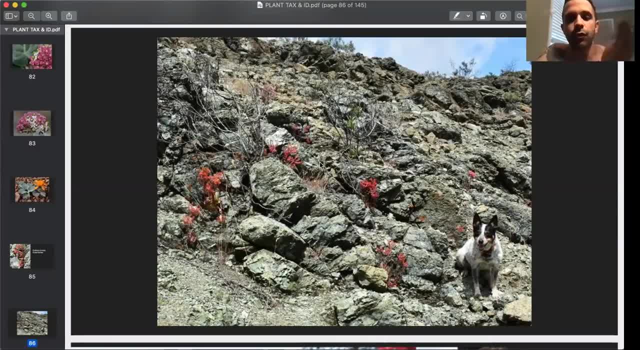 there's a benefit in in having a leaf color that's like grayish blue, because you'll blend in here. i mean, look, you can't even see these fucking things right until you get closer. the only reason you can see them now is because they're blooming. they're conspicuous, they want. 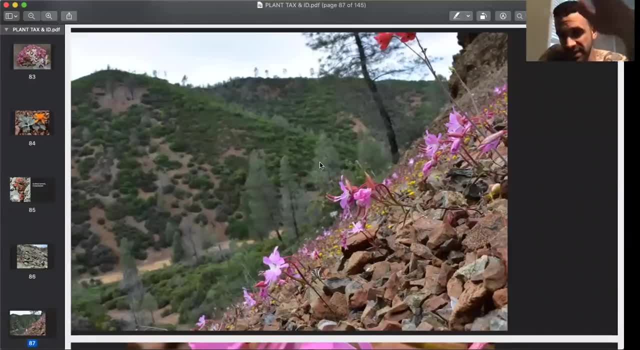 to be pollinated by hummingbirds? this isn't. this is a serpentine endemic. another really cool northern california species in the genus clarkia. member of the evening crimrose family. uh, this was. this is serpentine. you can see there's blue and red rock in there, so it's 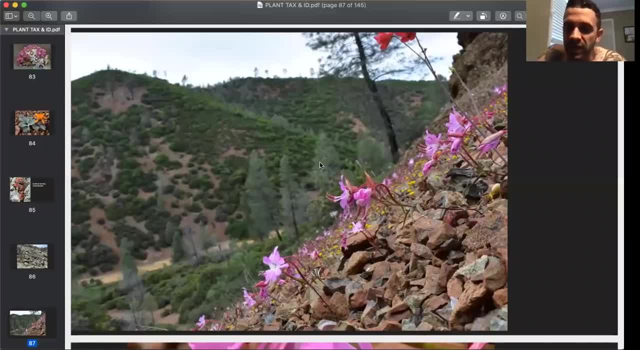 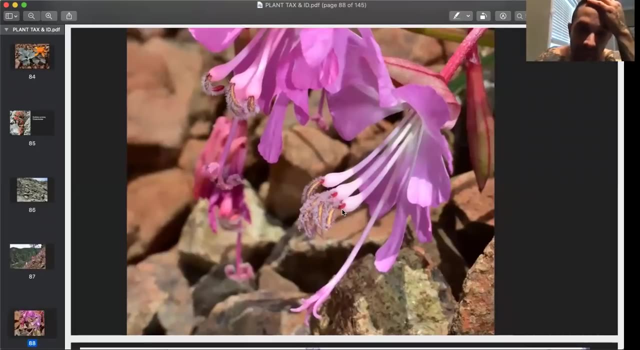 just weathering. uh, this thing is one of the only clarkia species. clarkia is a really cool genus, really showy. uh, i believe they're all annuals, um, but this one has the fucking hugest petals, i mean, and this shows, this is another good example to show you how, uh, one of the synapomorphies that's. 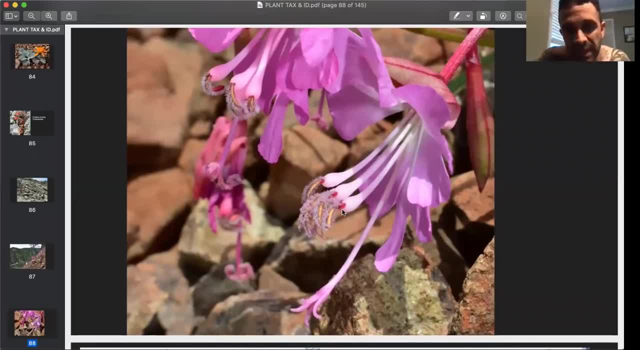 not a hundred percent, but most many members of this family have it. of the onogracia is they got this cobwebby like pollen. so see that these pollen threads they're they're technical term for them is uh, viscent threads, which just means like cobwebby pollen. so the 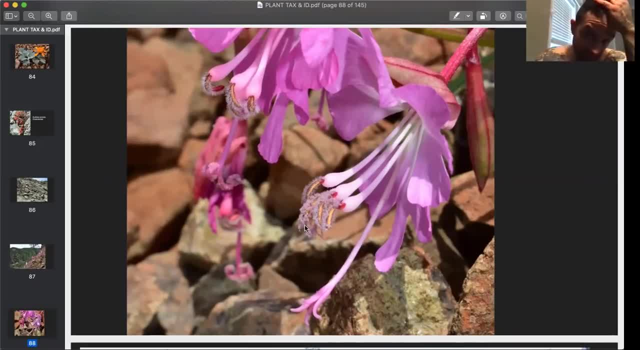 pollen granules stick together in this cobweb, uh like physiology, and that, of course, obviously has proved the benefit to uh these plants in terms of what pollinates them. so, uh, in this case these are pollinated by sphinx moths. uh, that's probably why they smell too. um, they're pollinated by sphinx. 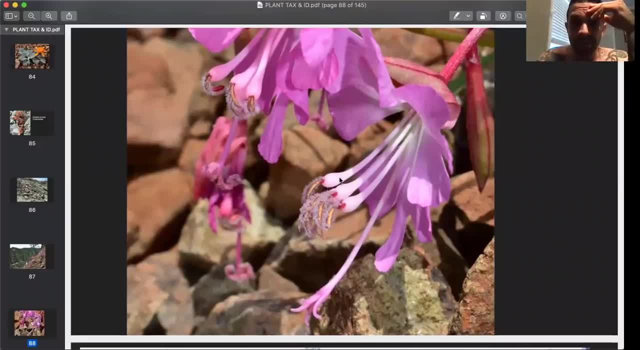 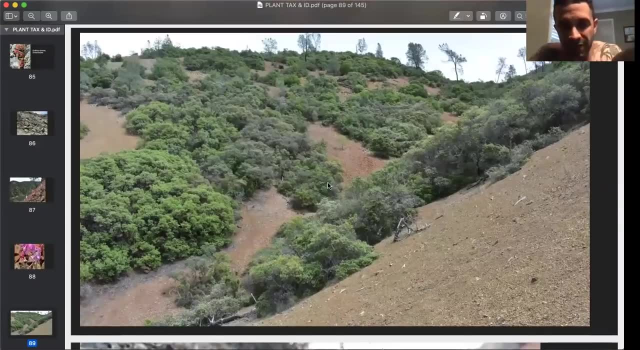 moths and they've got these enormous. look at the fucking anthers or the- uh, the filaments they get all swollen at the end. really bizarre and again only known from the central coast: ranges on serpentine, and here again you got that barren environment and what shouldn't be a barren 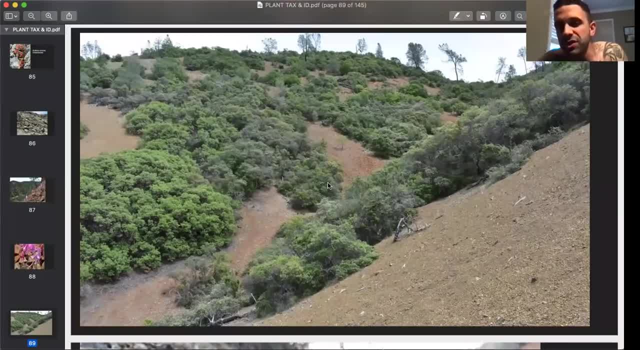 environment because it gets, i mean like 30, you know 30- inches of rain a year here, a little bit less last few years because the climate's so fucked up, but uh, but the rock is just so so fucking nutrient poor and shitty and stressful for plants to grow in. 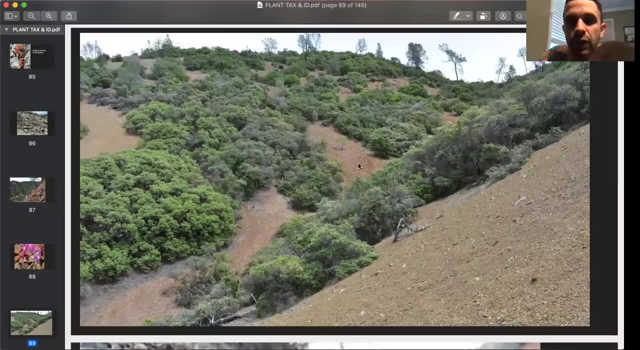 that it's entirely barren here. so this like over here: look in the distance where it's barren, like in between those two uh shrub lines, right that looks like just a barren environment. when i got up close i found like three different fucking rare uh serpentine endemic. 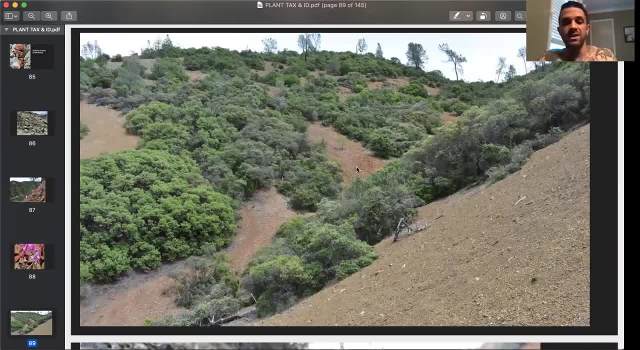 plants growing there. so it's always, it always, you know, works to really check out these barren environments a little bit closer, scope them out, see what's growing. there's going to be small stuff there, but and you can see a little bit of the green here. there was another cool member of the 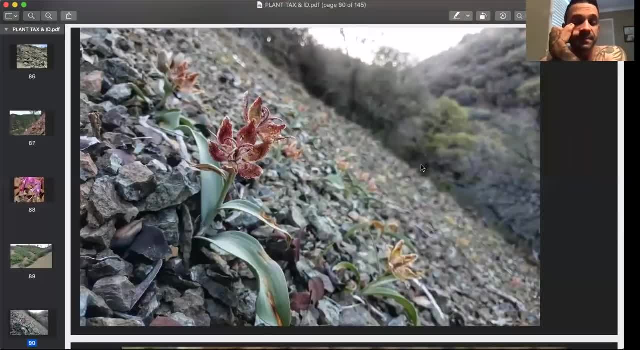 family growing at this exact spot, this guy area, falcata. this thing only grows in serpentine, and more so. it doesn't only grow in serpentine soil chemistry. it only grows on talus slopes. you'll never find it growing on flat ground. it. 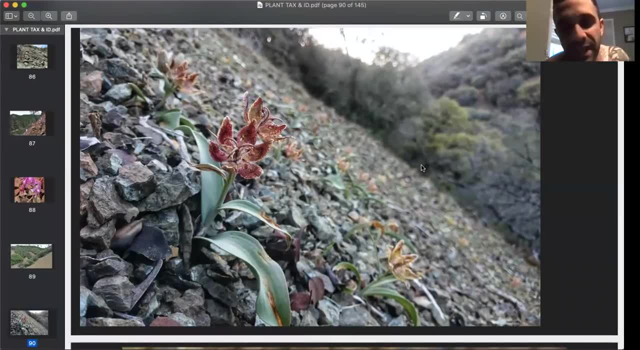 only it only grows well because of the way serpentine and ultramathic rock, which are somewhat synonymous, the way it weathers. it breaks up into these little like inch to two inch size square chunks, geometric chunks, and so because of that it forms these, the way the rock breaks up in. 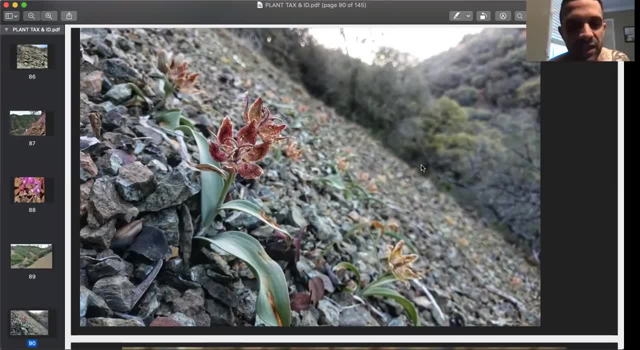 these little structures. when it's weathered and eroded, it forms these talus piles. so here's this. this is a phenomenon that's been going on long enough on the surface of earth, in this area, in this region, that you've had a plant species that has evolved to this specific trait, which is: 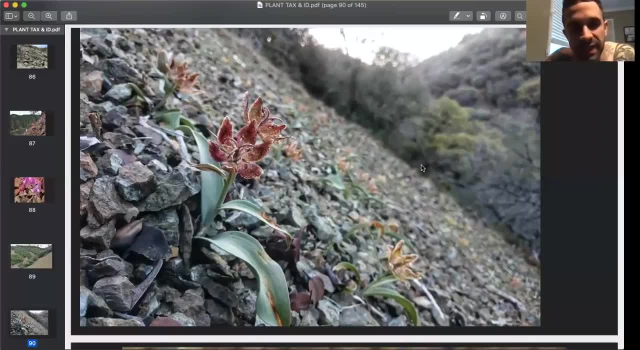 serpentine talus so deep and these are geophytes, they're lilies, right. so you got a bulb down there, so they're. they come back every year and there's a bulb eight, ten inches below that talus. it's. it's incredibly fragile when you're walking on these two. i mean, it's like a. 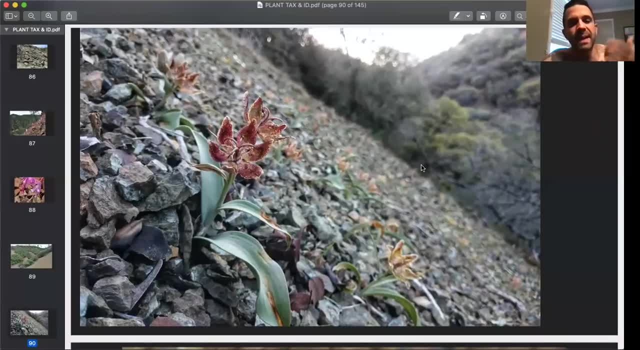 fuck, i almost hate myself because i'm like, ah, fuck, every step i take, this shit crumbles. you know, not only am i going to break my ass, i'm going to destroy something beautiful too. fuck, but it's fine. you know that that bulb will will come out. the bulb is still down there. you might 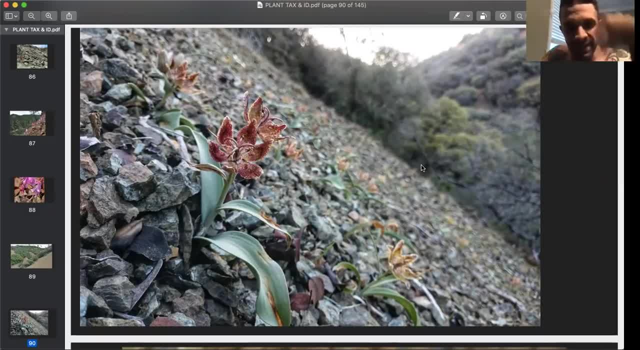 fuck up a generation, which is not ideal either, but so anyway, of course it's a lily, it's a monocot. flower parts are in multiples of three. you can see that three branches to that style you get up. the stamen's already mostly gone here, but there's. if you were to look closely you'd see. 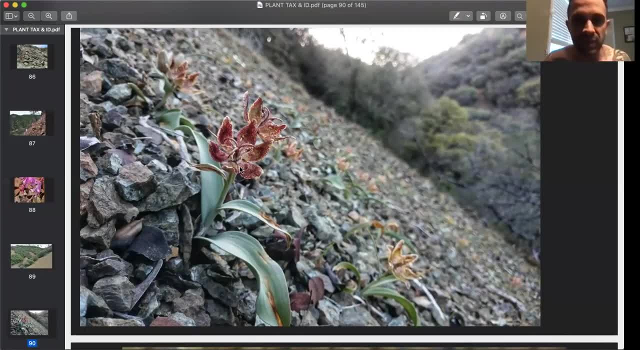 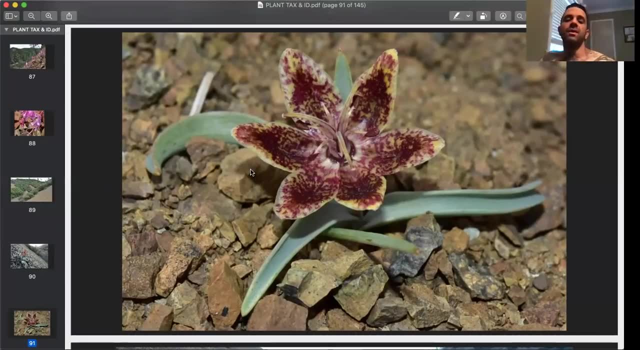 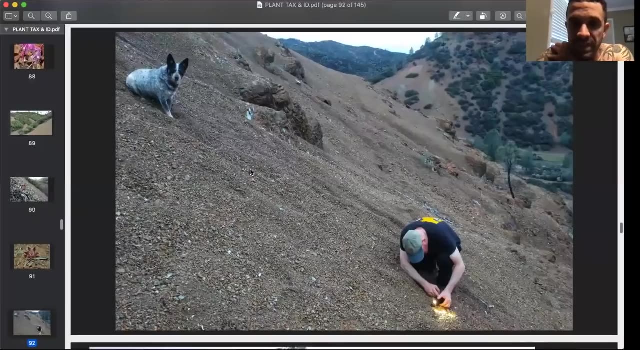 stamen. so flower parts in multiples of three, six tepals. so another favorite. there you go. boom and the. these things are so inconspicuous too, they can't be those again. you got that blue texture, that glaucous texture to those basal leaves. there's my friend alan rockefeller, taking 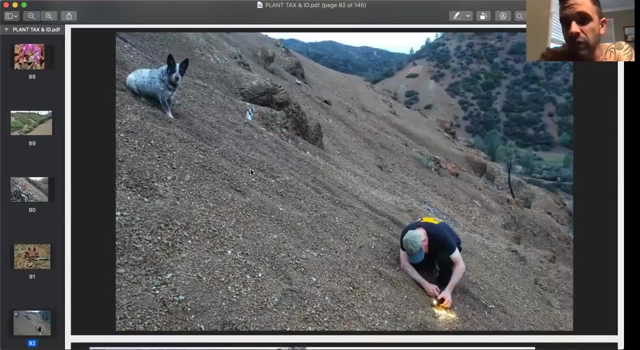 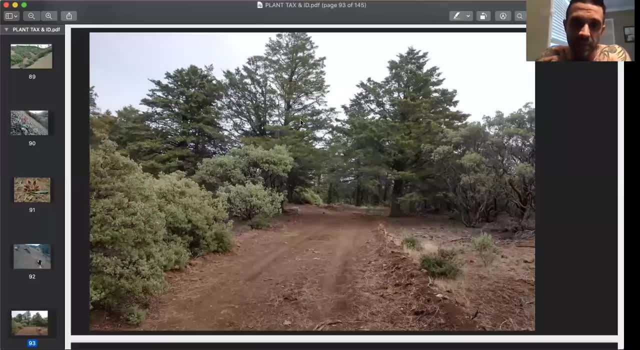 pictures of one. you got that ghost pine in the background too- pinus sabiniana, not a serpentine endemic, but it's found on serpentine a lot. here's a serpentine endemic: cypress hespero cypress uh sargentii sergeant cypress, one of. one of two or three cypress species that are highly restricted in their distribution, so they're only known from small areas and they're they only grow on serpentine, only in serpentine. okay, genus streptantis. we'll get into this really quick, because the point of this is to show you. 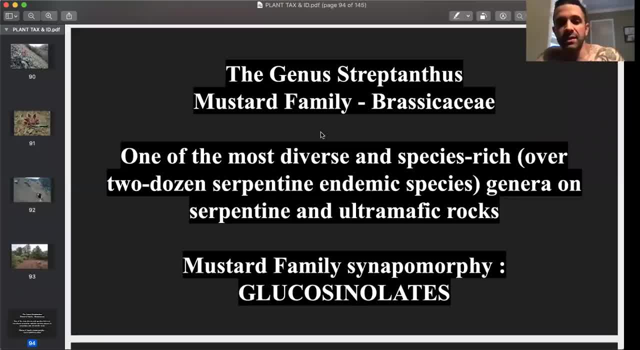 that this is a genus in which it's in the mustard family. so you got the glucosinase, but this is a like five or six times. so serpentine tolerance has convergently evolved in this genus five or six times. they are closely related, but if you take it to the next level down of taxonomy they didn't. 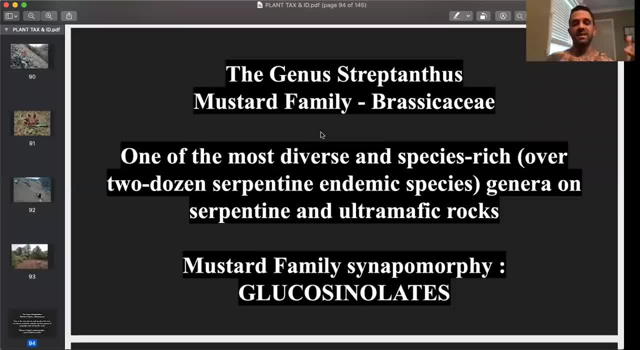 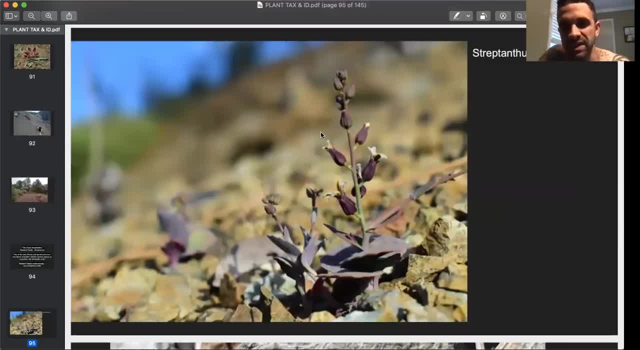 everything. every streptanthus, that serpentine tolerant, didn't necessarily gain that serpentine tolerance from the same common ancestor. so these are called the jewel flowers. they're, you know, for a fucking mustard which you normally associate- i normally associate- as being a boring plant. it's a. 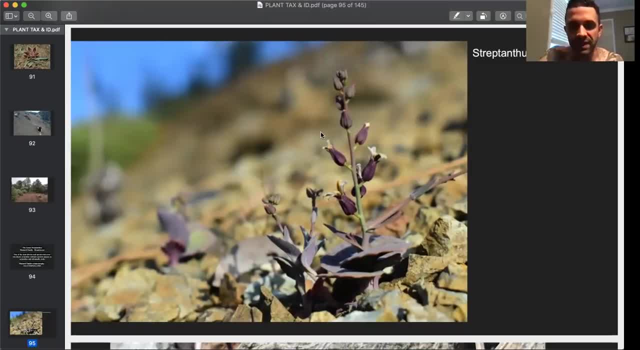 i get it: green, green leaves, yellow flowers, whatever uh, this, this thing involved, it's got purple. look at the leaves. the purple leaves blue in some cases. so you've got a little bit of crypsis there, a little bit of camouflage and the, the, but the flowers are just fucking incredible. 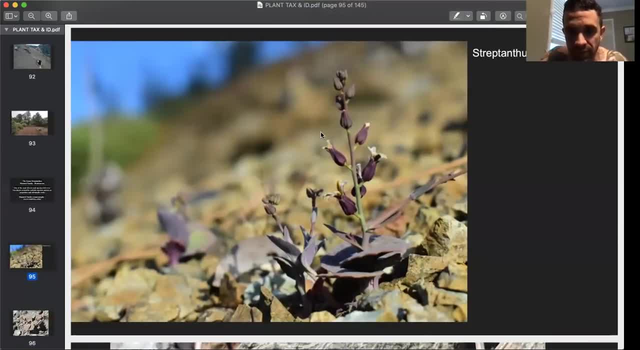 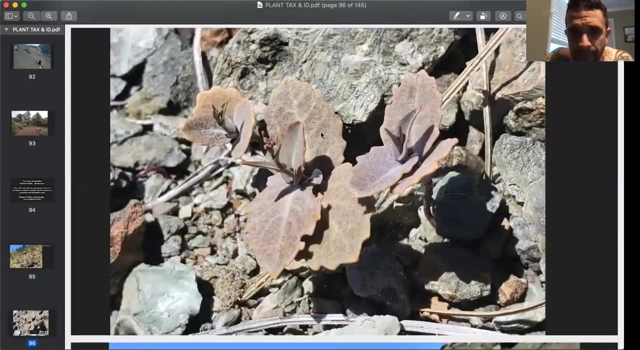 but we got uh, petals and multiples of four or multiple right, yeah, four petals, uh four sepals, etc. um, i think it's six stamens, so it's a little bit different, but either way, uh, there you go. there's the leaves when these things are just coming up and even cooler. 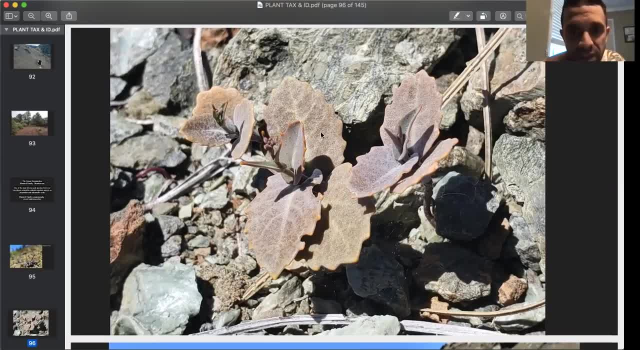 if you look at the ridges, the margins of those leaves, you see those little orange dots. the adaptive benefit of those is that they mimic butterfly eggs so that discourages butterflies from laying eggs on there because they're like: oh, this spot's already taken, i'll move right along. 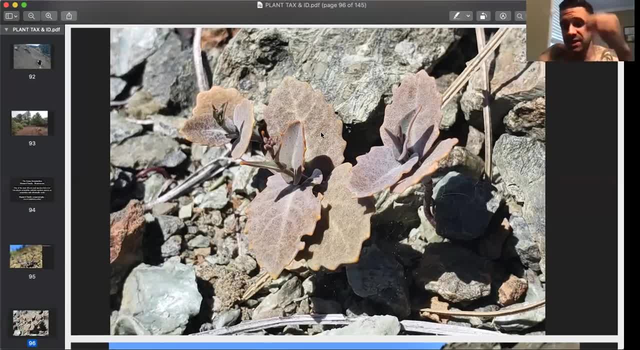 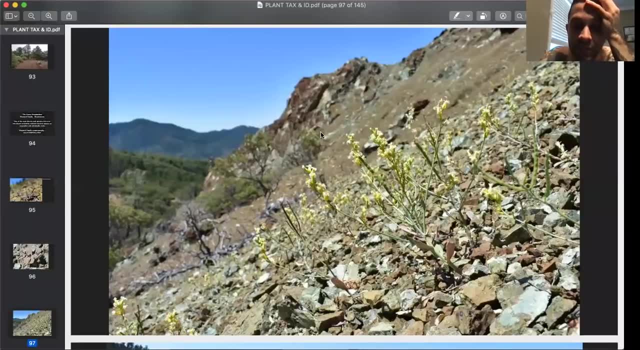 um, yeah, it's fucking wild. i mean these things. you could be standing right on top of them and you wouldn't notice them if they weren't blooming. this is streptanthus vernalis. species was only recently named in the last 15 or 20 years- vernalis, because it's one of the 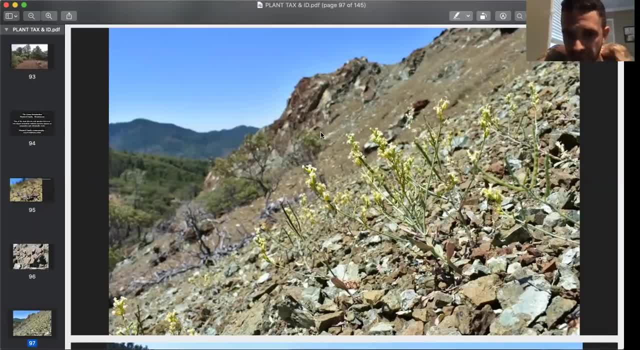 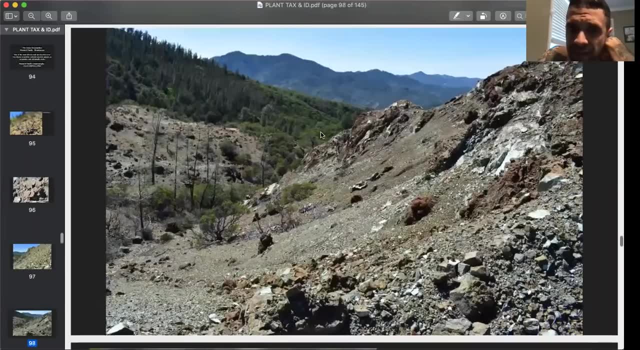 earliest blooming streptanthus. it blooms in the spring again, growing on serpentine. you can see that harsh blue serpentine talus right there, and this is in uh napa county. there's, there's the environment. i mean it's just like like a desert where there shouldn't be one a streptanthus. 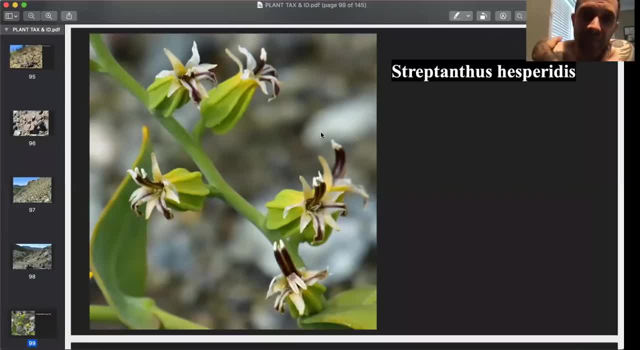 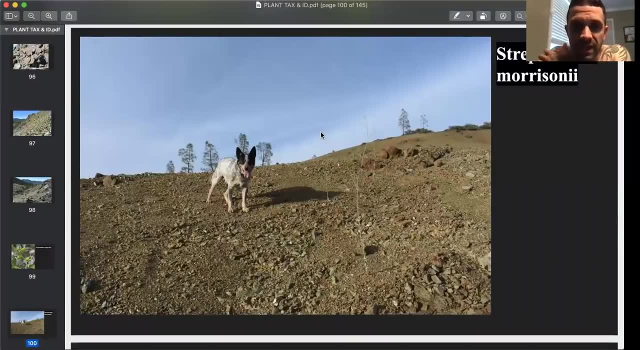 asperitis, another serpentine endemic. you know, it's just variations on a theme. look at the ridges in the middle of the netherlands. like the sepals, this is streptanthus morisoni. i i mean again really dry, exposed environment. it's northern california but we're inland a little bit, uh. so 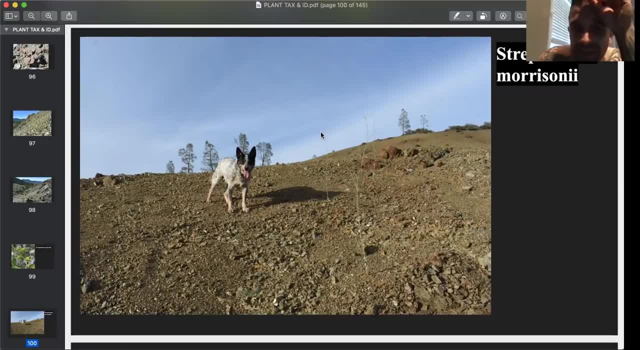 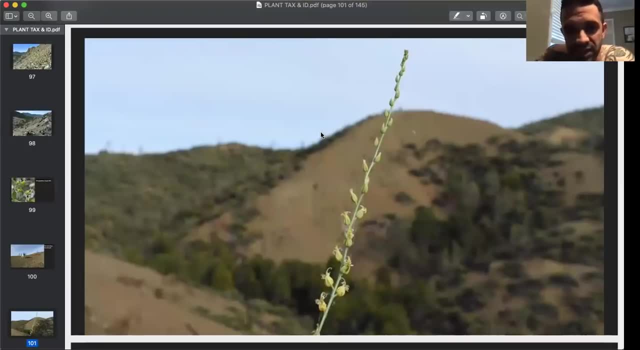 it gets really fucking hot here. you don't want a lot of surface temperature exposed. you got thin stalks, thin leaves, and then there's your flowers, but you get like three or four feet tall. another rare endemic, you know. who knows when it speciated, who knows when this species evolved? you know. 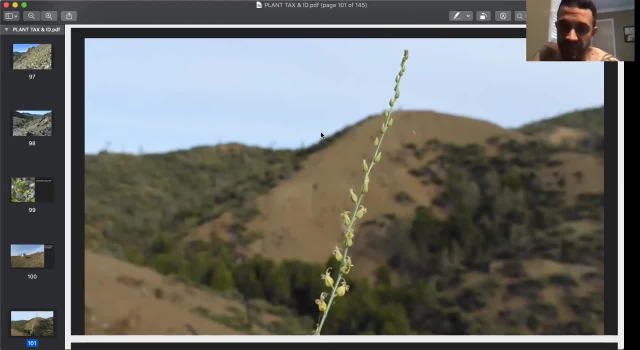 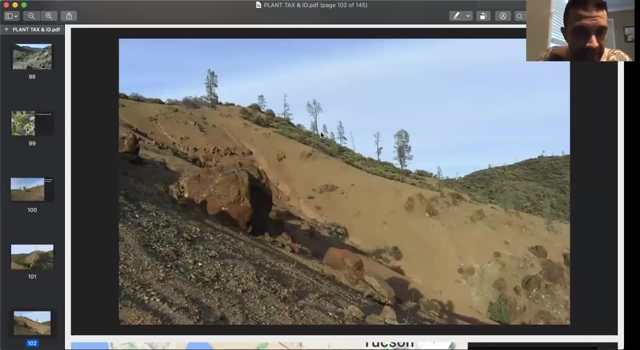 three million years ago. but either way it's restricted to this small area. just a barren serpentine. i fucking love this habitat, man. and these look like blocks of almost raw peridotite, maybe slightly metamorphous peridotite in the background, but again red or blue. 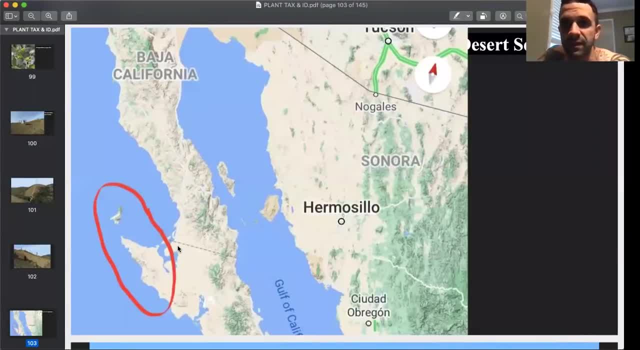 here's desert serpentine. it was a fucking fucked up. the uh, that covered the text a little bit anyway, this is where it occurs. so i i first- you know what was thinking about. i was like: well, everything, a lot of areas in the west coast of north america have serpentine, because that's. 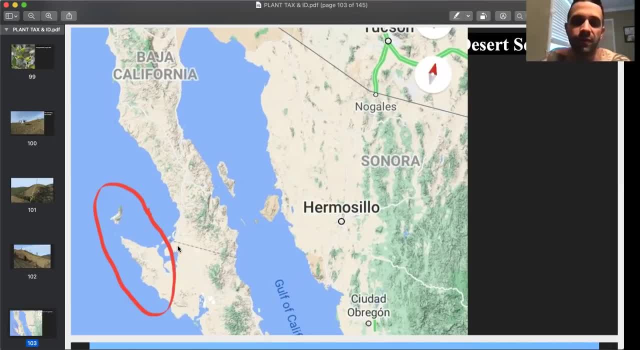 where the subduction zone was. i wonder if any ever occurred in baja. so i wrote a friend of mine who was a botanist down there. i was like: you ever get baja, you ever get serpentine in the on the peninsula, the bop peninsula. he said yeah, actually also i just found a new species down. 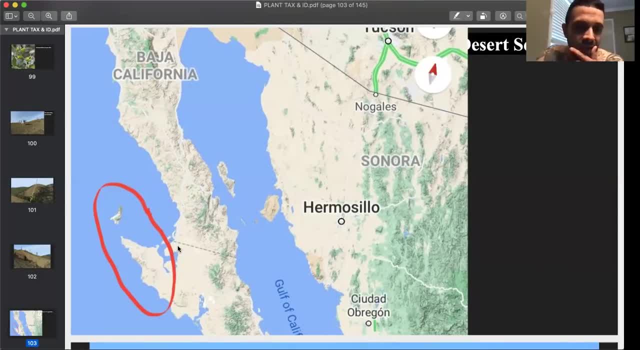 there haven't described it yet- which i'll show you the pictures of. so there's serpentine here, there's gabbro here, which is not metamorphous, it's. it's a another igneous, intrusive igneous rock with like, but it's like a black igneous rock, like giant. 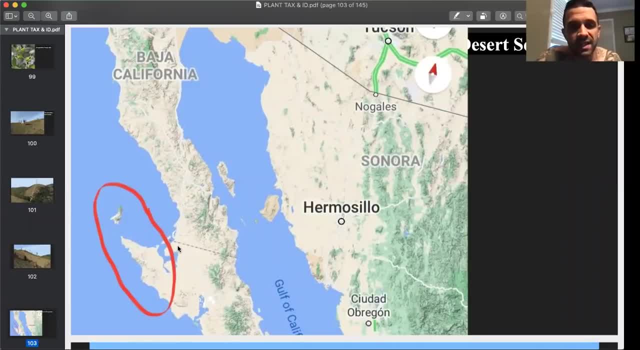 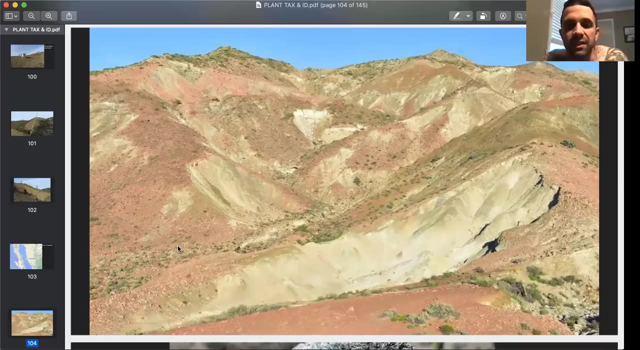 black crystals and it's fucking beautiful rock. it's the intrusive equivalent of basalt. so same chemistry, but different conditions, cooled much, slope much more slowly, and this is what it looks like. so it's it's. this is what the not what gabbro looks like, but what serpentine looks like. 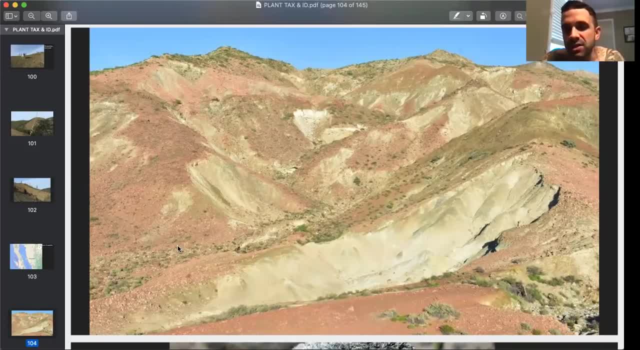 in the deserts of baja. so you take the climatic uh stresses of, really you take the climatic stresses of really you take the climatic stresses of really low rainfall, high aridity, uh, but you also get fog here too, which helps a little bit, helps the. 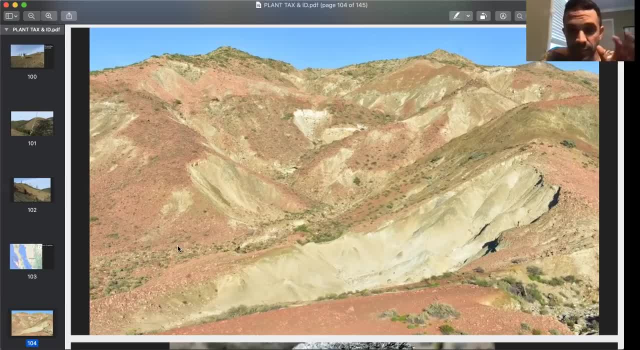 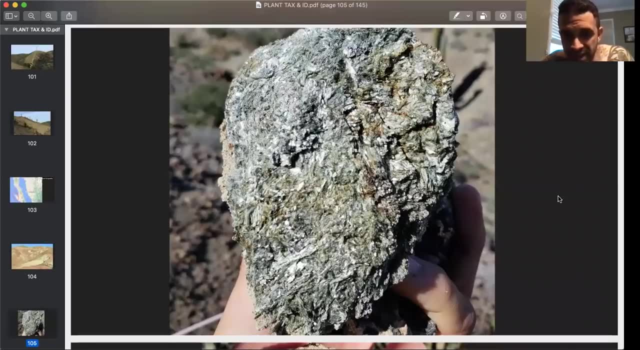 plant life and you mix it with the chemical stresses of serpentine, you're going to get some wild shit evolving, and indeed you do. there's some of the rock. this almost looks like chrysotile asbestos. uh, again this- these types of rocks- only occurred in certain areas that. 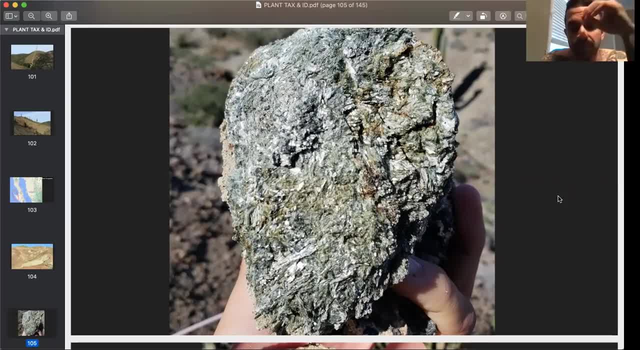 these weren't uniform throughout the the whole landscape, but where you did find them, i mean, this thing i took home too. i wrapped it in a bag so it wouldn't break off, because you get asbestos sometimes in serpentine too. serpentine is a really general term, it's a 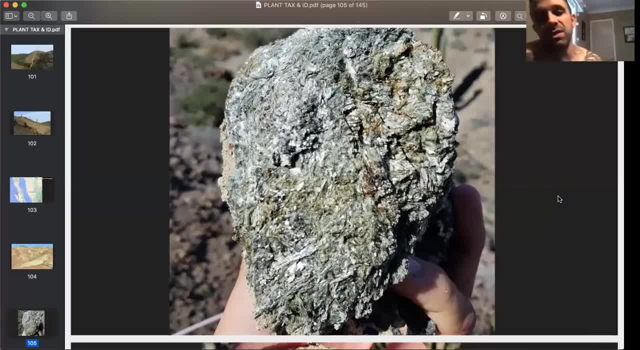 broad term for a bunch of different minerals. they're all composed of the same same, the same chemistry and from a similar- uh uh, origin environment. you know metamorphosed um. so they're not all uniform. you get a bunch of different versions of serpentine um, but with 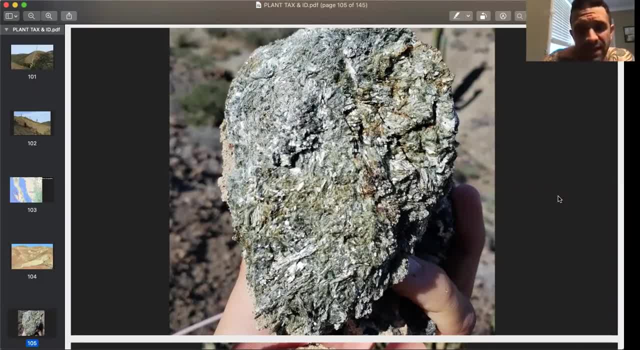 the same. you know chemical similarities of high magnesium, high iron, high nickel- like sixty percent of the world's nickel comes from serpentine. uh, exposures from serpentine areas anyway. uh, sometimes you'll see areas where there's asbestos and there's a spot on the beach. 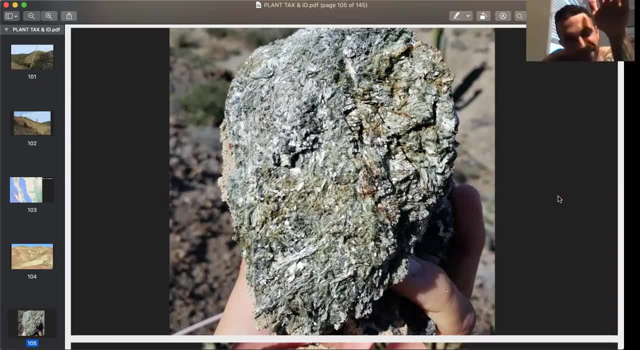 near big sur where it's like it's all, it's all fucking asbestos. it seems like it looks like these blue sandy slopes of what is technically all chrysotile asbestos. it's not as dangerous as you know the asbestos that they use to manufacture. it's a little bit more raw it. 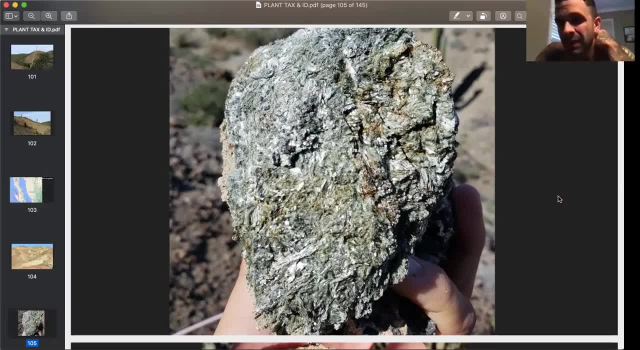 it's not airborne as easily. but technically it's asbestos, it's chrysotile. um, it's fucking crazy. it's really cool too, but just you know you expose to it once you're not going to fuck yourself up. but if you spend a lifetime working in a factory that manufactures asbestos roofing shingles, you. 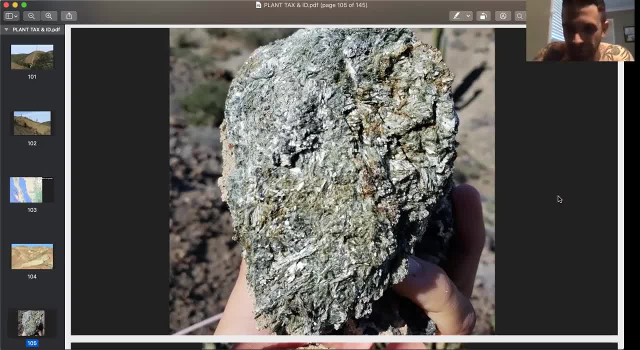 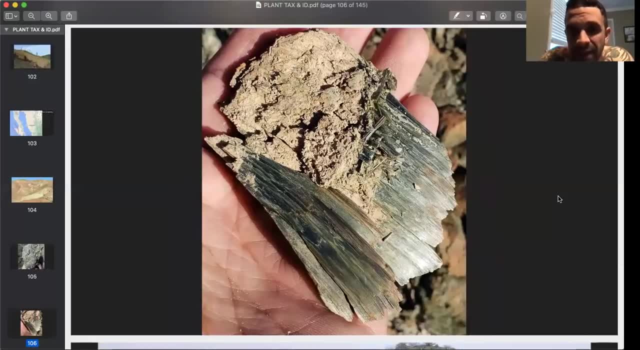 might get mesothelioma and you might get you know in on one of those lawsuits they advertise on late night tv. but anyway, there's the chemical structure of the rock. i bagged that fucker up, took it home and uh, there you go. there's that nice fibrous nature of some of the more chrysotile. 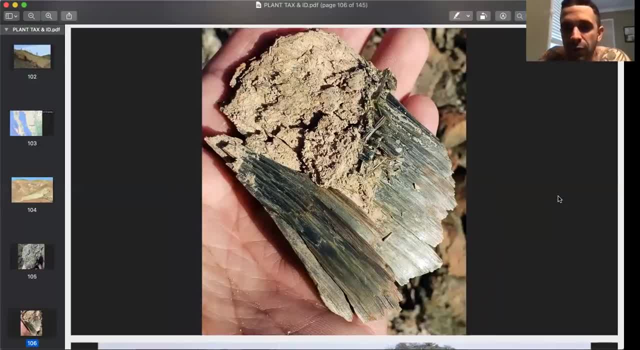 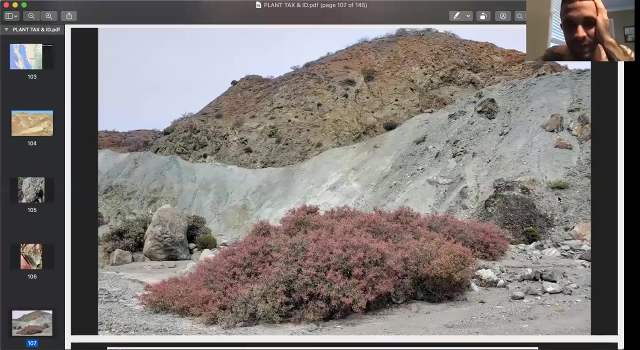 uh, serpentine. so you see, you got that dark green to light blue color and it's just, i mean it just looks like fibers there. it's great. i don't know if i took this home that might that's a little bit more, a little bit more too close to, uh, asbestos, but uh, anyway, moving on to the flora, this is a. 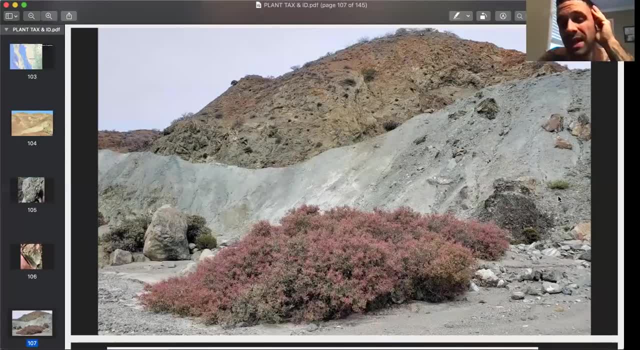 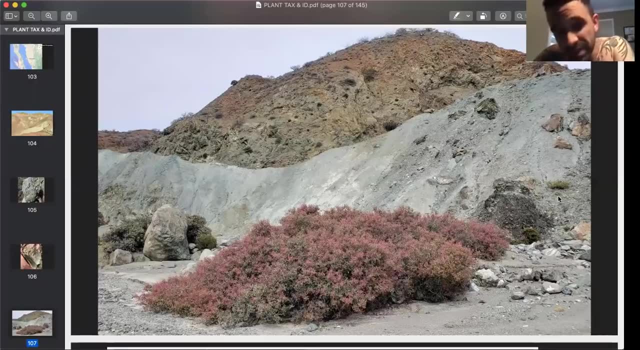 serpentine endemic. this is a type of sumac, this is ruse lentii. so it's in the sumac poison oak and mango family, uh, the pistachio family, anacardiaceae, but it's. you'll only find it growing on the serpentine of cedros island. 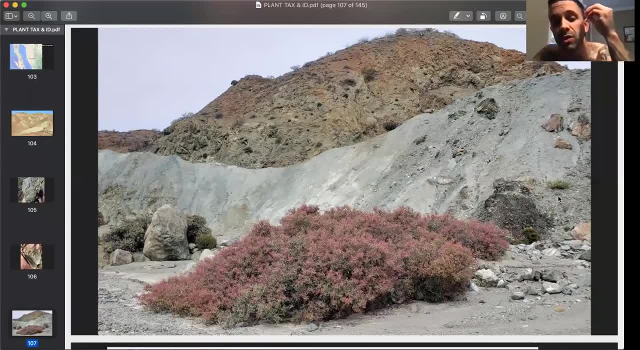 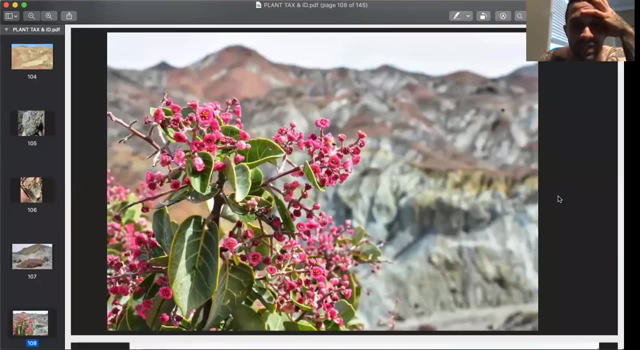 and the immediate uh baja peninsula coast where there's serpentine and this thing was fucking covered in bees. man, there were hundreds of bees around this thing when it was flowering. there's a nice up close money shot so you don't have hairs but you got a really waxy. 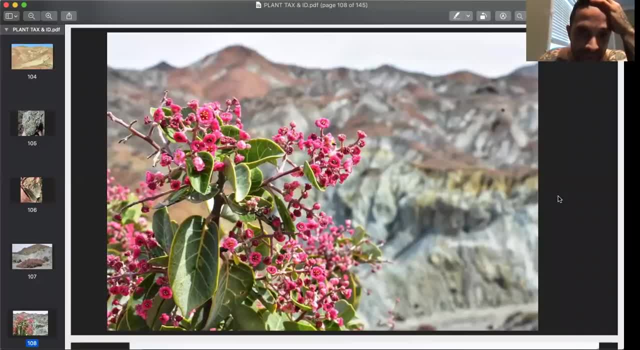 blue leaf with these bright pink, intoxicating uh flowers on it, and you can see in the video that i'm showing you here. you can see the background, notice how the tops of the, the, those cliffs over there, are red and the sides are blue. why do you think that is anybody? iron oxygen: what oxidation? yeah, oxidation, right, because the surface. 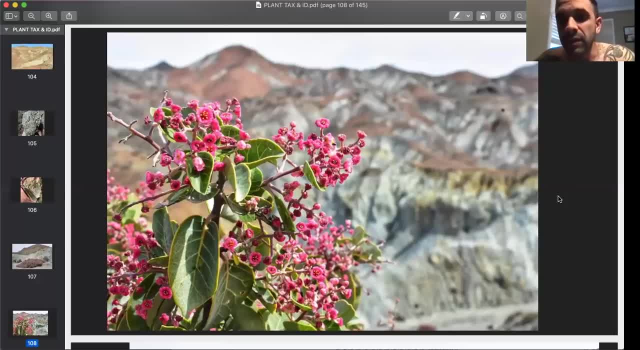 has been exposed technically longer than those slopes have. so you know, the slopes are constantly eroding. there's. it's an unstable rock, it's brittle, it's not that strong. it's constantly new material over eons, uh, you know, falling off and falling into that wash down below, whereas the tops 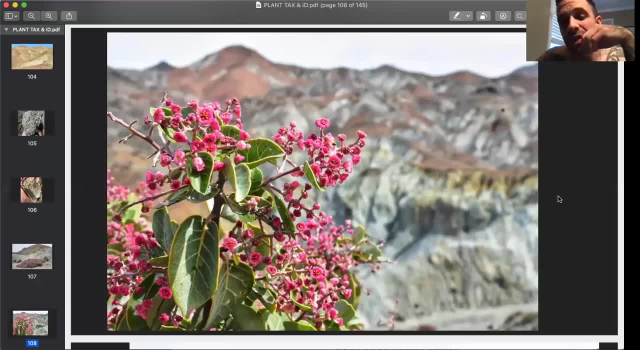 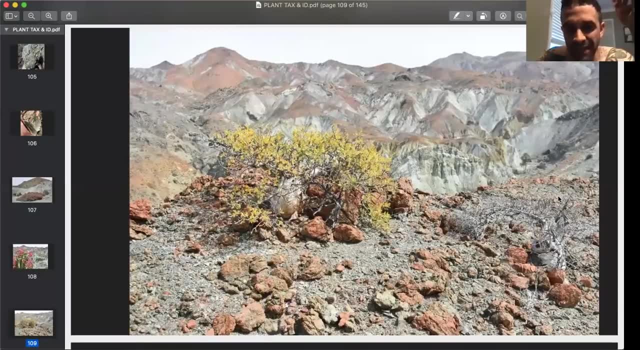 stay relatively, uh, stable, so they've been exposed longer. it's been exposed to the atmosphere longer and that's why it's it's more red. this is the elephant tree, so this is fucking cool. these were everywhere two feet tall. this thing tops out at and you can see that huge caudiciform trunk. 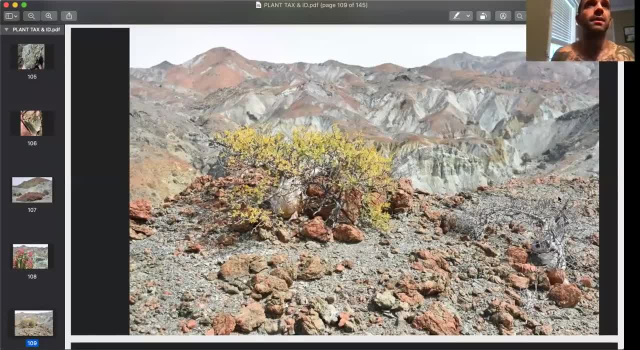 caudiciform is just a word for like you know, like a baobab or like a uh, you know, whatever you get the idea, just like a big swollen trunk, a big swollen stem, and there it is growing on. just volcanics. so that same species. 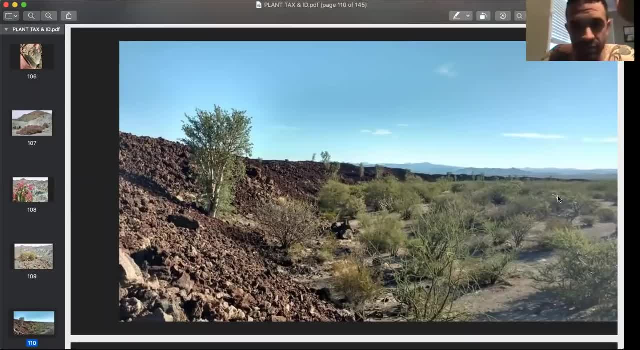 right here is getting 30 feet tall and forming this you know big tree, and then here it's just this tiny little. they might even be the same age, but here it's just this little tiny fucking bonsai. this is another spot. this is elsewhere on the baja peninsula, growing on uh, volcanics on. 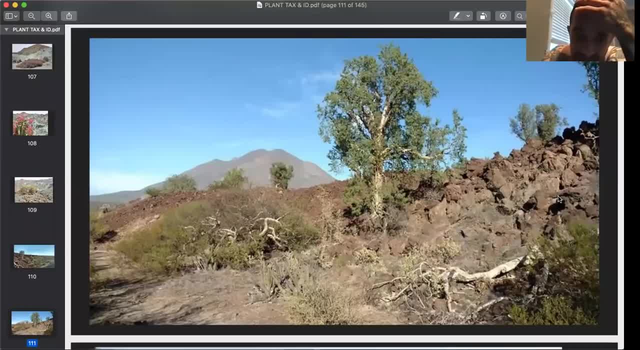 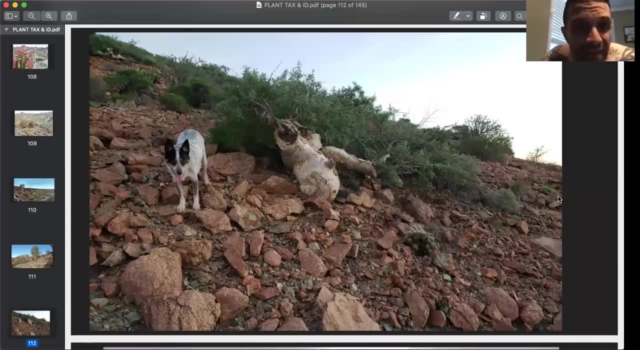 looks like, uh, pumice, just pumice, and maybe a little bit of a salt. i don't know, i didn't forget what it was. so anyway, here's that serpentine again. i mean, the flora here is just fucking so cool. you got a little cactus, uh, down there. it's a species of echinocereus, i forget which one. 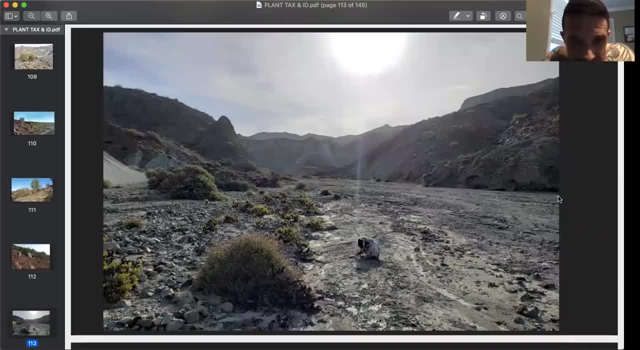 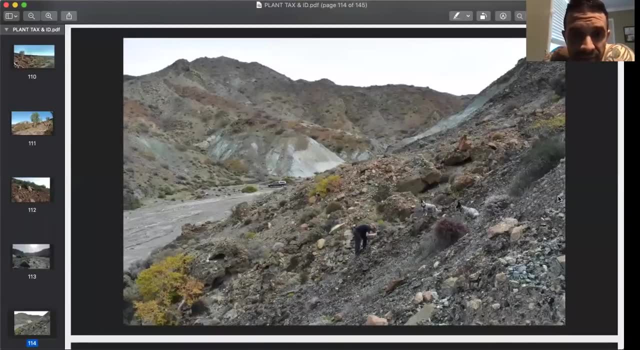 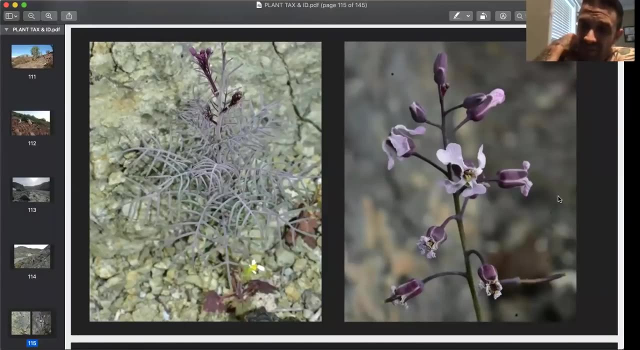 there's the wash. tons of cool shit coming up here, lots of endemics that only grow from this tiny fucking area. and this one, this is sibara angolorum. see the four petals. that tells you it's either going to be in- probably onigraciae or brassicaceae. this is in brassicaceae, the mustard family. 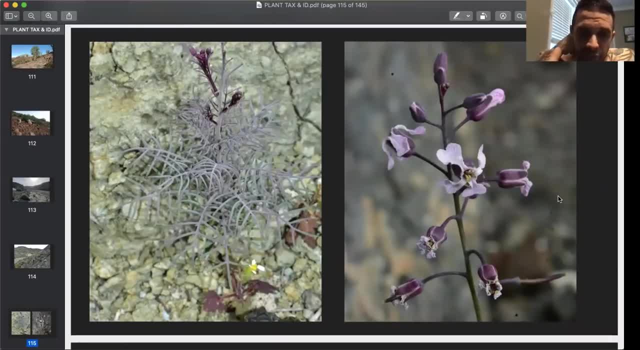 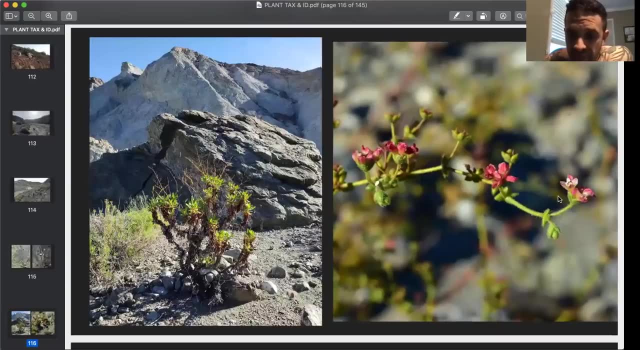 uh got purplish bluish leaves. uh reflect that uv light. blend in with that substrate more and then when it goes off, it's just boom- incredible. another endemic is an endemic buckwheat, just to ultramathic serpentine rocks and baja. this is uh. 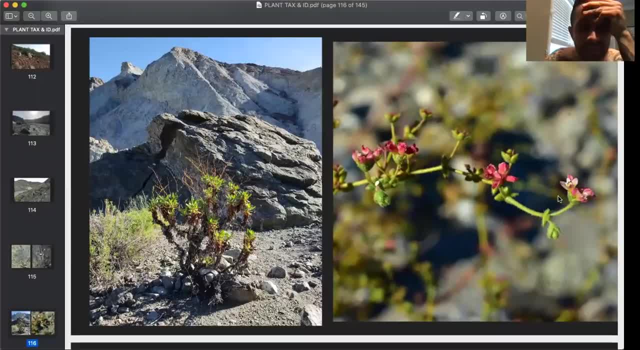 ariagonum. oh fuck, i can't remember this. i can't remember the species name. uh, oh fuck, i have to look it up. there's like three different ariagonums from this area. uh, that uh are endemic to serpentine. you get another one, ariagonum and celioides. i couldn't. 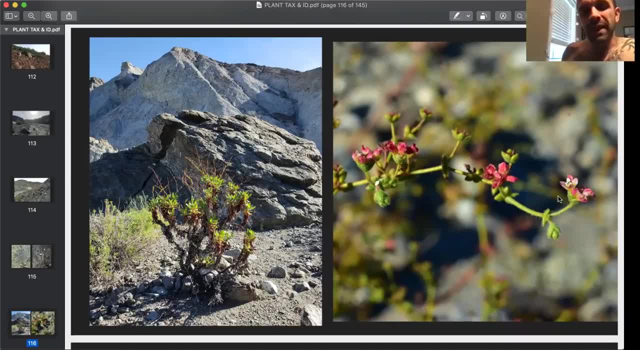 find any. i think i put some photos online. if you look up like ariagonum and celioides online, like my photos are like one of the only few that come up. i tried to create a video about it but i couldn't find any of them, so i'm going to. 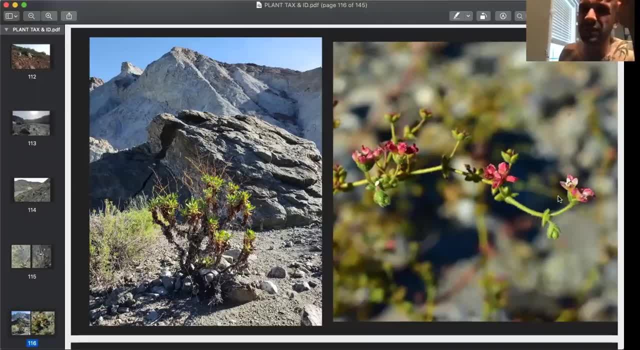 make a wikipedia page for it because it's such a cool plant. but someone- one of the checkers there was like you- didn't cite your sources or your. i couldn't find the paper that described that ariagonum, so i you know whatever they took it down, but the photo should still be up and it's. 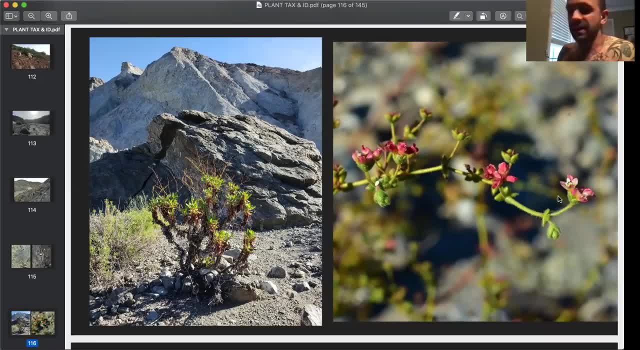 called in celioides because it looks like: uh, and it's yeah, this was ariagonum pre-clarum, another serpentine endemic. this thing's a long-lived perennial. you could see it just keeps growing. the old leaves die. that's what forms that candelabra shape and it just keeps growing. 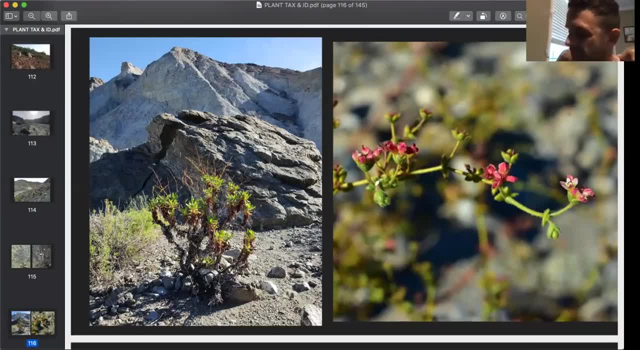 when you get up close you can see the old leaves die and it just keeps growing and it just keeps growing. you see that even the leaves just get smaller and just get bigger. down here the old leaves are looking great. they just keep growing and they just keep growing. so 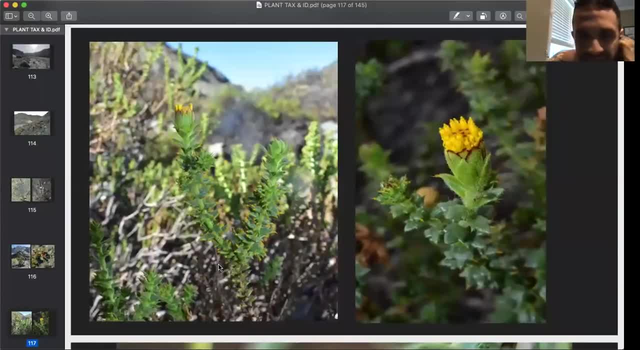 i don't know if you can tell in that photo: super glandular, super sticky, tons of tiny little hairs, each beaked with a gland, just like cannabis. same thing going on here: lots of tiny little hairs beaked with a gland. this is baja calia, moraniae, probably one of my. 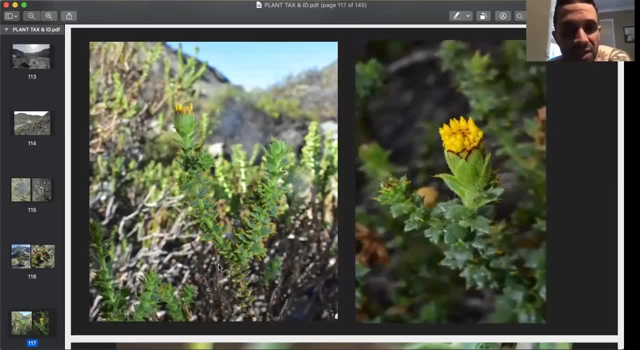 favorite members of the composite family. in, uh, the deserts of baja, california. it's a serpentine endemic. the leaves have been modified through the filter of evolution to be spinose. they're a little spiny. uh, the thing is also in the marigold tribe, so it stinks, uh, like turpentine. it's got those pungent volatiles. this thing smelled. like lemon and turpentine. it smelled like some fucking lemon herbal tea mixed with paint and it was the most bizarre shit. i i got some seed. i germinated one of them, but it just wasn't hot enough in my greenhouse and i couldn't give it the right conditions. you know, in coastal calif. 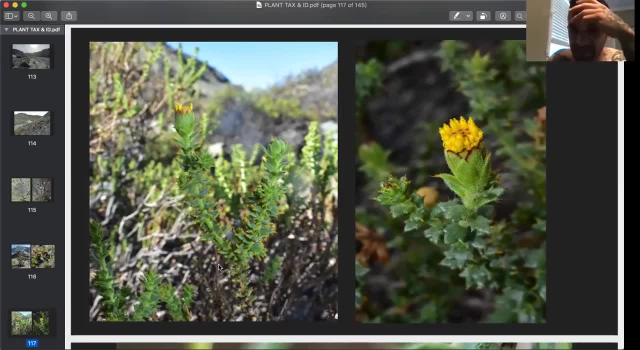 northern california, so didn't make it. i still got seed of it, but uh, you know i haven't tried germinating. yet another thing about desert seeds that's cool is a lot of these seeds are long-lived right, because anything that wouldn't, any seed that wouldn't last that long in an area where 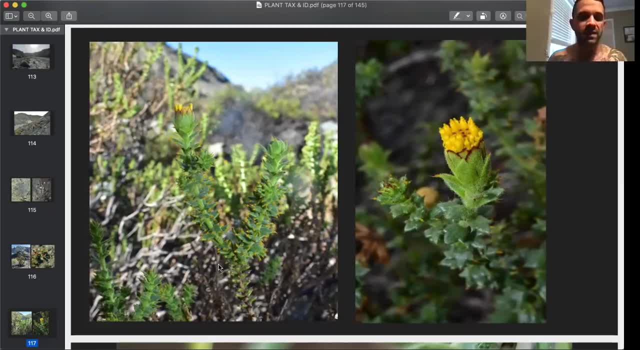 rainfall might only occur, or substantial rainfall might only occur every few years. any seed that wouldn't last that long, that's only got a short shelf life, would perish. so that would be filtered out by through evolution. so it's an adaptive trait to have long-lived seeds. 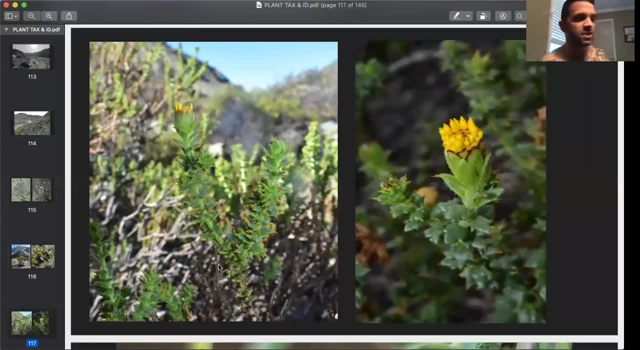 in some cases you know 50, 60 years. that's why you get these super blooms. you know, when you get all the fucking instagram influencers going out to take selfies in, like a field of california poppies or or or death valley super blooms, you know those seeds are there the whole fucking time they could be there. 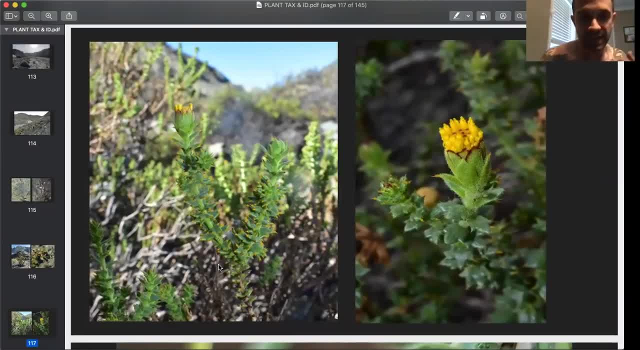 for four decades and it takes. you know they've got inhibitors in them, often chemical or physical inhibitors. chemical inhibitors would be like, uh, you know, chemicals that prevent the seed from germinating until they've all been dissolved or washed away by water, diluted by water by enough rain. uh, physical, physical inhibitors of seeds might be just a really hard seed coat. 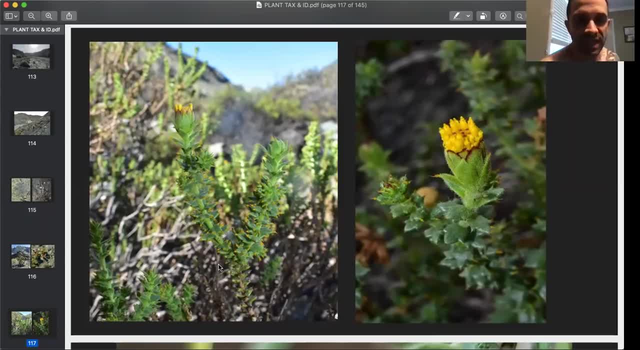 the genus erythrina, the coral beans has a really hard seed coat. they look like the seeds are like these bright red beans with like the texture of plastic. to get them to germinate you got to clip the top with a nail clipper to scarify it in essence, to get the water to get in there. so 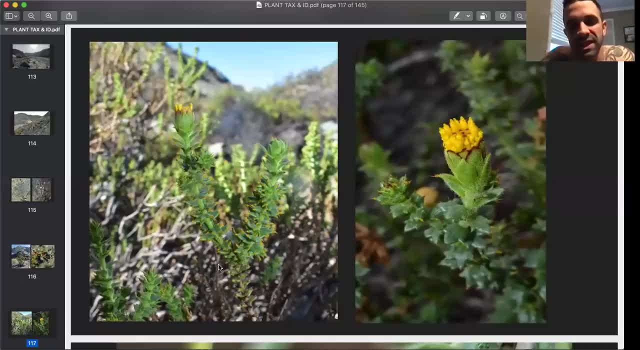 that's an adaptive trait you'll see in a lot of these seeds. not all seeds will germinate at the same time. some will lay dormant, some will germinate with the first rain, first big heavy rain, some will take a little bit longer and again, that's just. you get that genetic recombination. every seed is a. 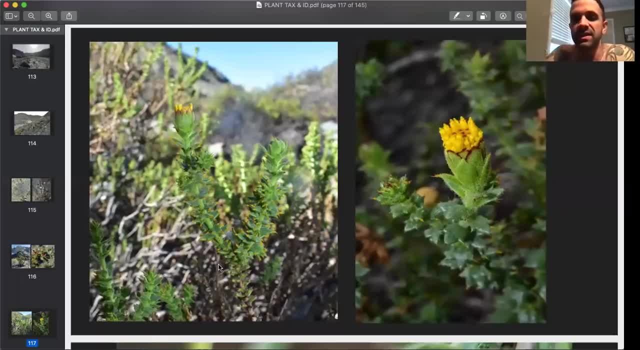 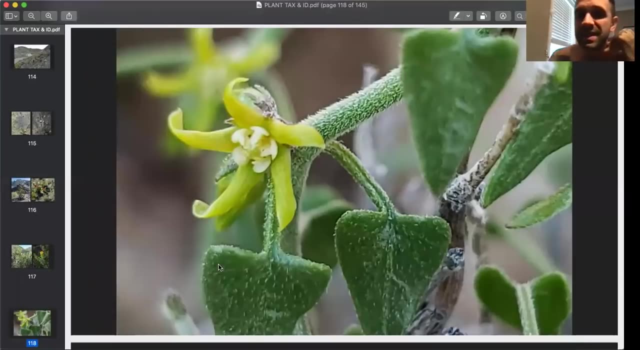 different, uh, a different combination of genes and alleles etc. and so some will germinate right away, some won't- really cool trait to think about with plants. so let's see, the plants tend to be there the whole time just waiting to germinate. so anyway, there you go. bah kelium urania, another endemic, this. 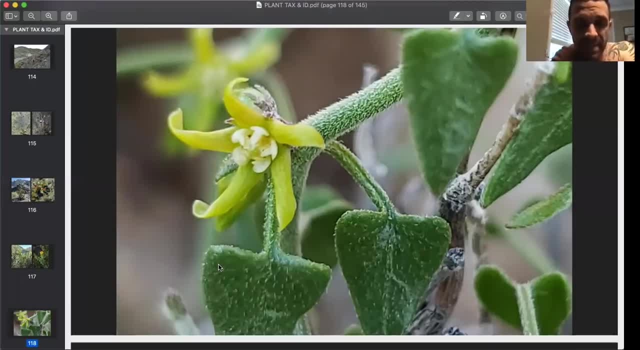 is that new species in the milkweed family. it's a species in the genus modelia uh, that hasn't even been described yet. Redmond, uh, at UC or at the San Diego Natural History Museum, just discovered this, like five years ago, and, uh, we went there looking for it the first day. we couldn't find it because I thought 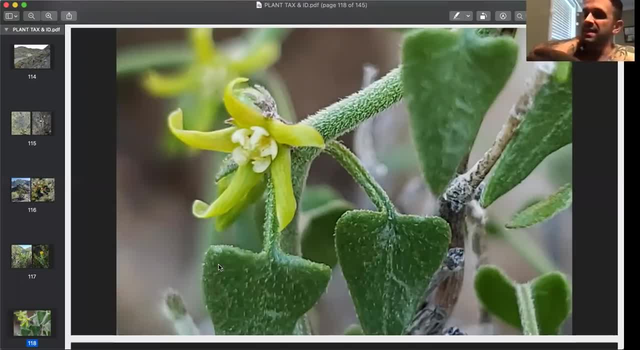 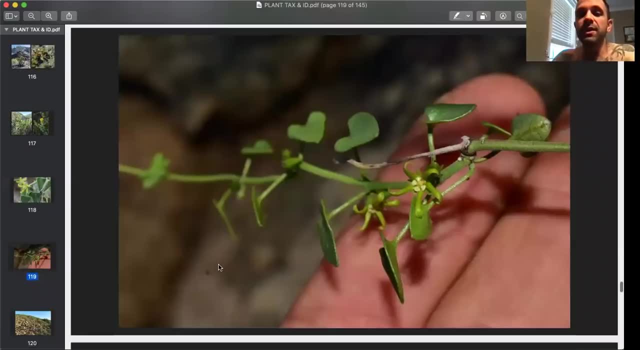 it'd be in the wash right, because it's where all the plant life is going to be, that's where the most moisture is. it wasn't growing on the wash, it was growing on the ridges up here, just totally diminutive. and you know, a fucking species that's never been, quite likely never been seen by people. 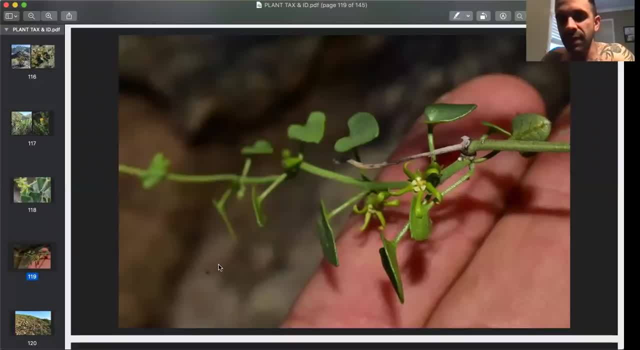 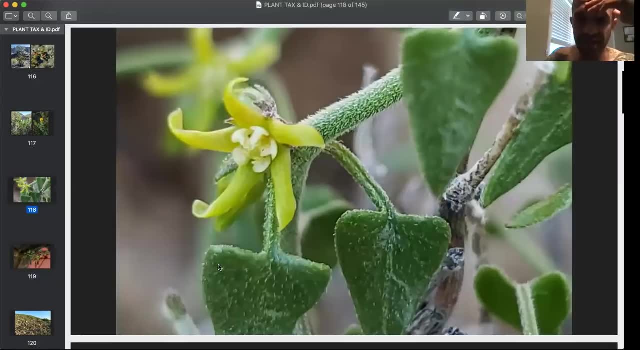 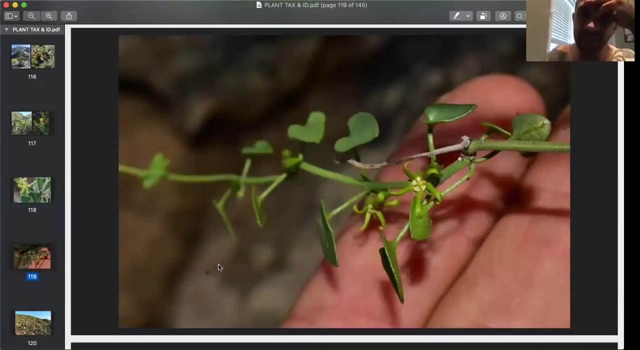 before. maybe it was noticed by Native American people, but there wasn't a use for it. uh, and totally new to science, you know, just hiding in the desert, sabaha, look at how hairy it is, those tiny hairs. tiny little flower, tiny little milkweed like flower, pentamerous flower. numbers of 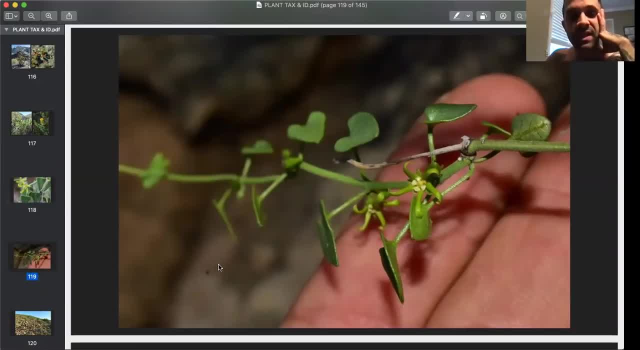 multiples of five, numbers of number five, five mares, little heart-shaped leaves. I don't even know if he wrote the paper on it when he actually he asked me not to show these four years ago. he asked me not to make it up, post about it and I was like, yeah, yeah, I won't because I still want to describe it, but whatever. 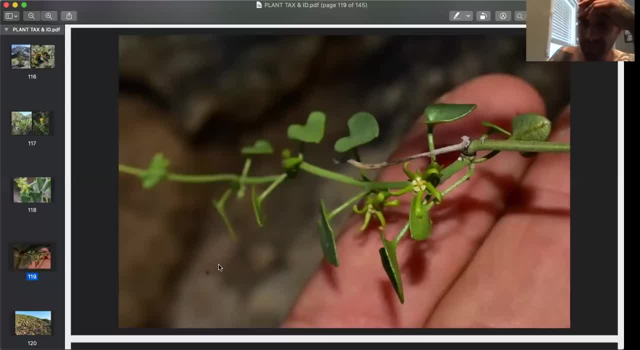 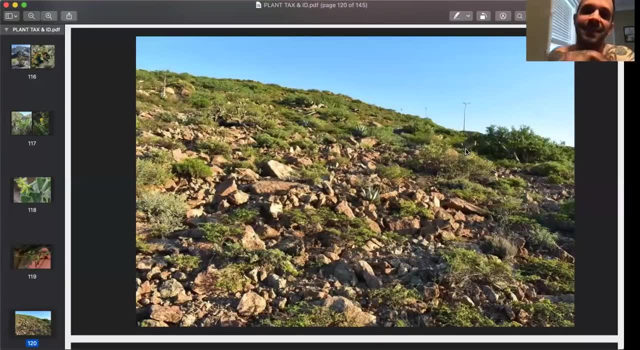 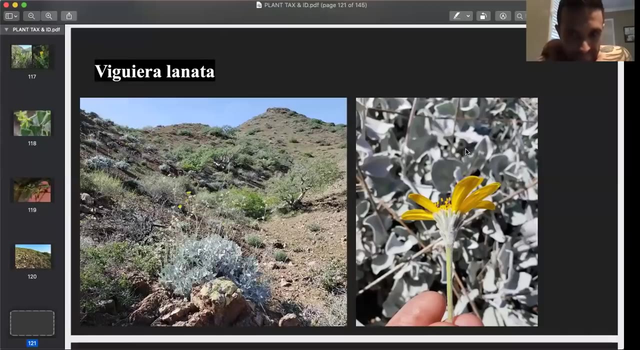 he's had enough time. if he hasn't done it by now, fuck it, I'll show it to you. so, and that's the habitat. look, you got fucking agaves back there. that's not a telephone pole in the background, that's an agave stalk. such cool habitat. this is viguera lanada. so fucking woolly, so woolly and so. 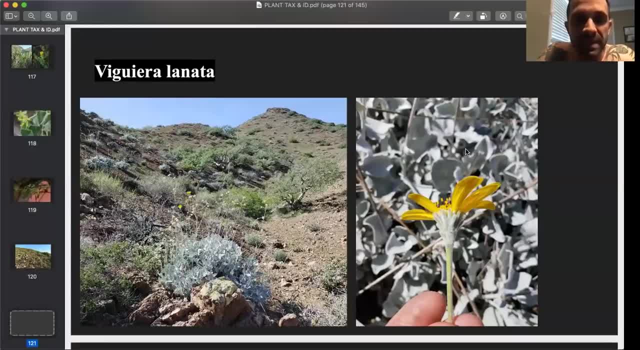 blue and just adapted to that. you can see that the serpentine's eased up, the chemistry's eased up a little bit here. the elephant trees are getting. they grow a little bit taller, so that's probably a younger elephant tree in the background of the one I just showed you, but the soil is not as fucked up so it can. 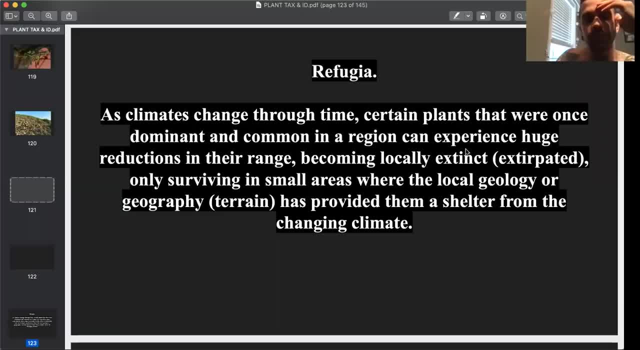 get bigger. the fuck, was that? okay, refugia. this doesn't really have much to do with soils, but you know, refugia, just the idea that, as climates change through time, uh, the geography can act as like a safe house, uh, for certain taxid species and even entire plant communities. so you know. 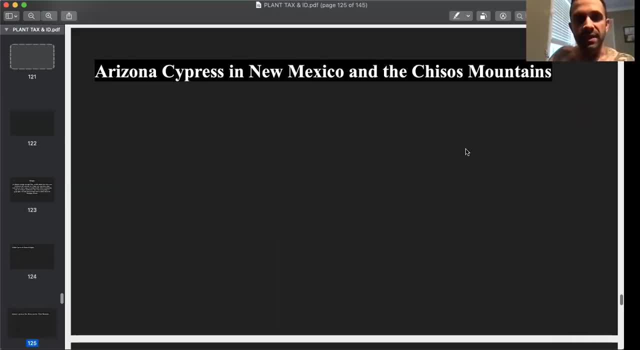 what I'm going to show you here. oh on, here, on on it, uh, on on where I know if that's what I'm on, um here, on misnomer, common name in eastern oregon, which is like 400 miles from the nearest population, and that's because the geography, though, if you look at like a terrain map, you can see how the 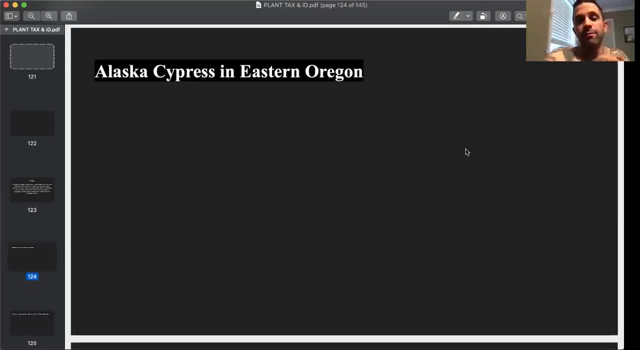 geology, the slope and the little, the way the mountain is carved out. it provided this little refugia for this plant to kind of hide out while the climate changed. it dried out around it like or eastern oregon's, like high desert man, it's like high desert with volcanic substrate, uh, and. 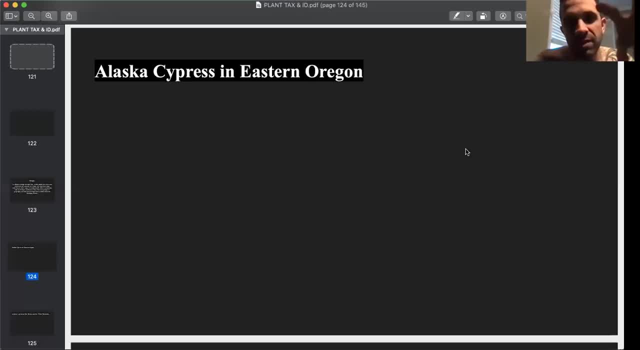 but here in this population, alaska cypress, which is a really moisture, demanding shade- demanding uh- needs an intact forest to grow in. there's a little population there still. it actually just suffer a fire. it's kind of fucked, might go out in our lifetimes, but it's still cool to see like oh. 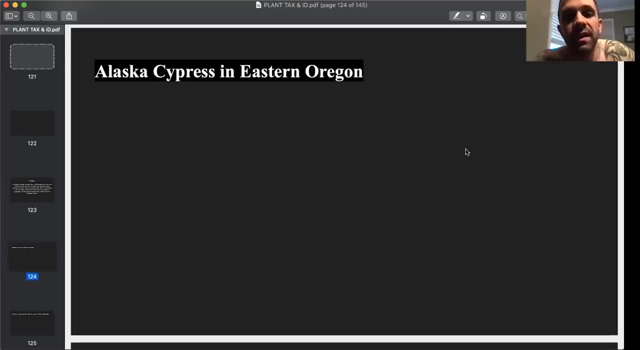 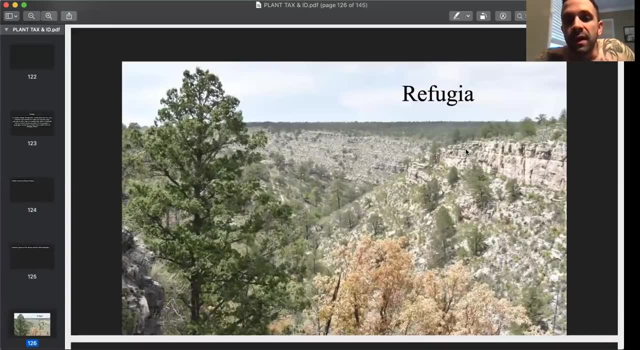 this is a remnant of the fucking pleistocene, you know, of when, uh, the eastern oregon was a little bit cooler and a little bit more, uh, wetter got a little bit more rain. okay, here's the first example of refugia. this is a. 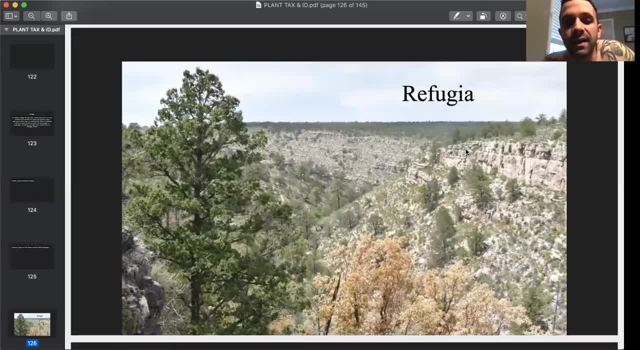 cool little canyon in southern new mexico, kind of near where that uh, a new localis gypso genus was. it's the doug for growing in this little limestone canyon up top on the top up here on the mesa. it's all juniper steppiana. it's all alligator juniper, relatively drought tolerant, low diversity up on. 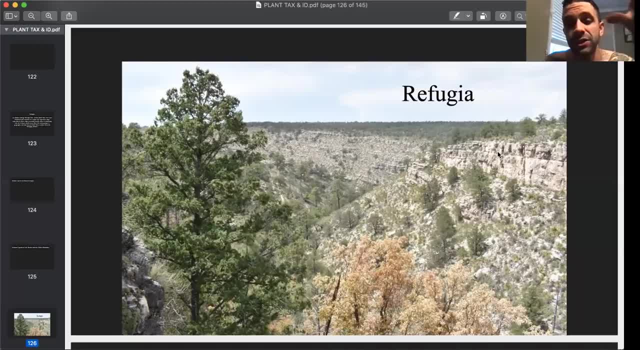 top. but in this little canyon we found all kinds of wild shit that would not, could not survive up top. it needed. the canyon provides shade because of the slopes on either side and it also acts as, like that, pavement effect. uh, for the desert, brittle bushes, you know funnels all the 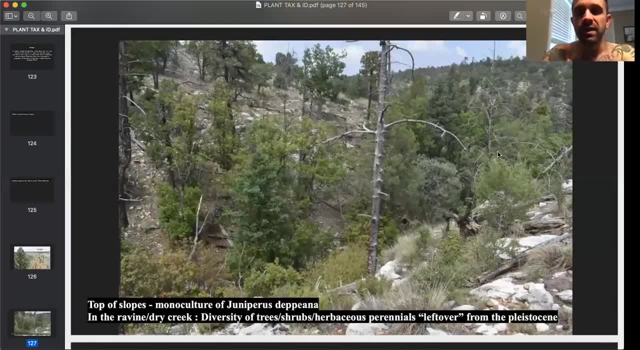 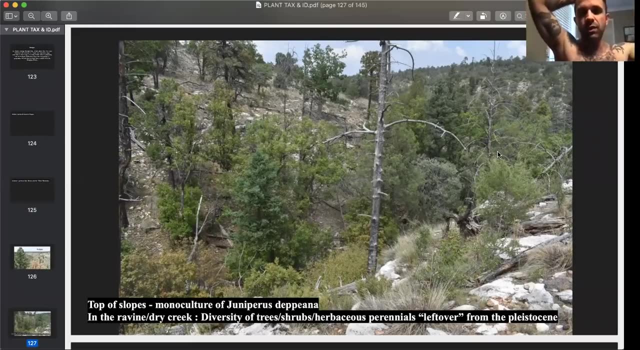 water into it. so we found maples there. we found, uh, our madrone there. we found cool members of the hydrangea there. we found monument plant there, the member of the gentian family, gentian aca, and frasera- that really cool fucking phrase there. anyone who's from the rocky mountains? 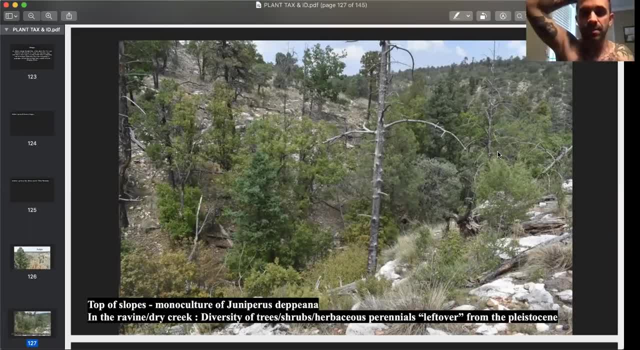 knows monument plant. anyone who's from the rocky mountain area and pays attention to botany and likes plants would know the monument plant. okay, and this is a big disjunct to find it growing in southern new mexico and the fucking what's technically the chihuahua desert. so here's. 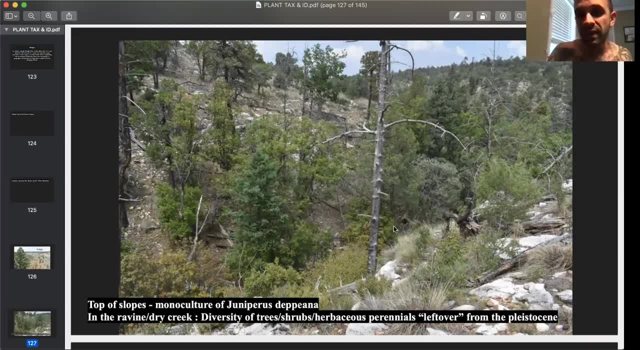 a good example you can see down in this. this is where this is, further up the canyon from the photo i just showed you. so this little arroyo eventually opens up into that big canyon. so these are like the headwaters: they were totally dry, but when it rains they funnel water. these are the 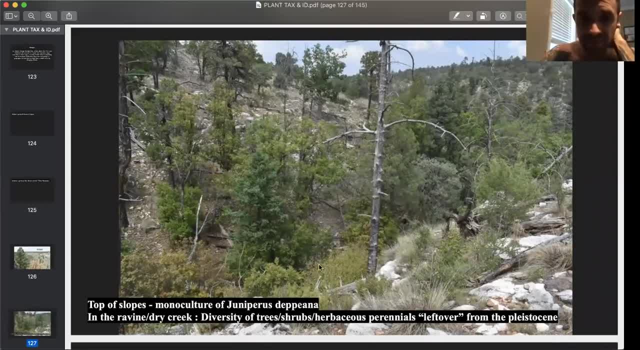 headwaters of that canyon and you can always already see you got rocky mountain, doug fir, a lot of different things here that seems like the well. this is the first one here. i'm going to point to it. last year when i did this, i took the first one from theolitical park. this one was up in the 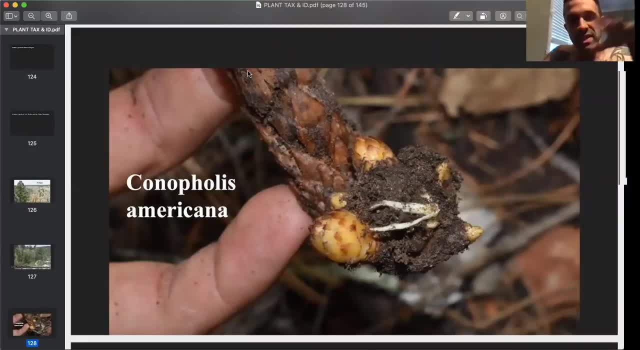 knee of the valley and this is a big regular suet, whereas here we see the yellow plant. there's a lot of green stuff on it and there's an apple flower in there here with the maple flower and the red- all the wide yellow food. but it was like so many peaches. 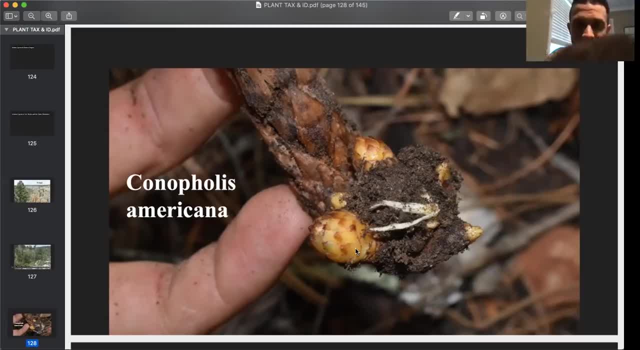 on there. and then the other one. when we dug it from the river i figured it was like the juke nada was trying. i figured it was dead so i pulled it up, but it actually fucked up. the plant, like i put it back- but it's you know, of course- got to be attached to its host, so it probably died. 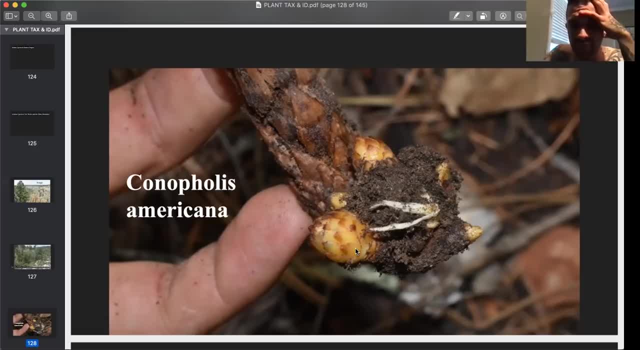 my bad, but i got a good photo out of it, and there's plenty more there, canophilus americana growing in the chihuahua desert, which is, i mean. if you know this plant, you know the habitat it's found, and it's not real. it's very strange to see it, uh, and on the map of what is technically the. 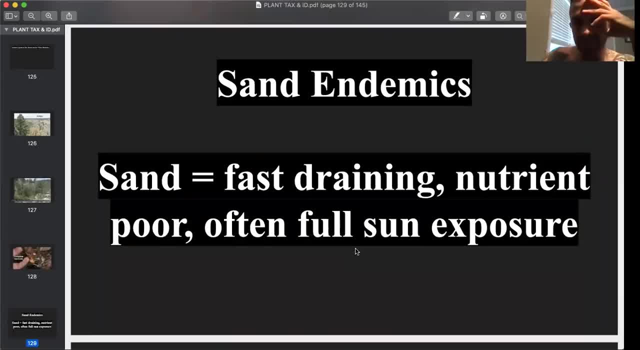 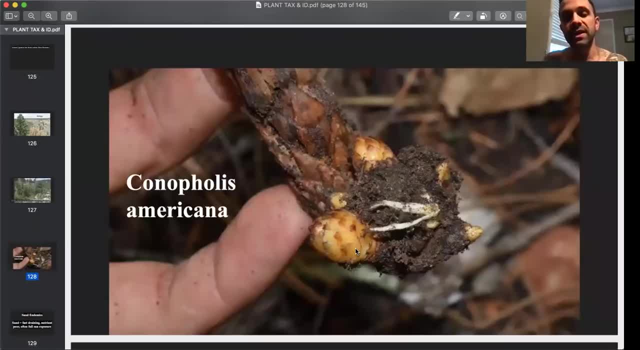 chihuahua desert, but again it's growing in this refugia, this tiny canyon, you know. and one thing i'll say about refugia too, that's cool is i mean i can look at a topographic map, at like google terrain layer, and and see how the topography, uh, is laid out and see, you know, what is gonna what's. 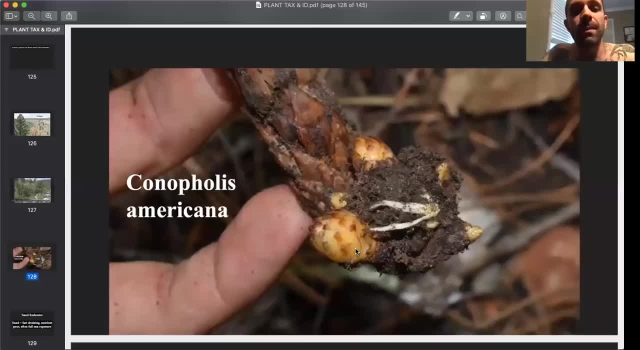 gonna what areas might have cool plants. i call it masturbating, like: oh, look at this little nook that's carved out. it's a north-facing cirque, a north-facing glacial cirque, so like a three-sided means it collects all the water and it's shaded to the south, at least in the northern hemisphere. 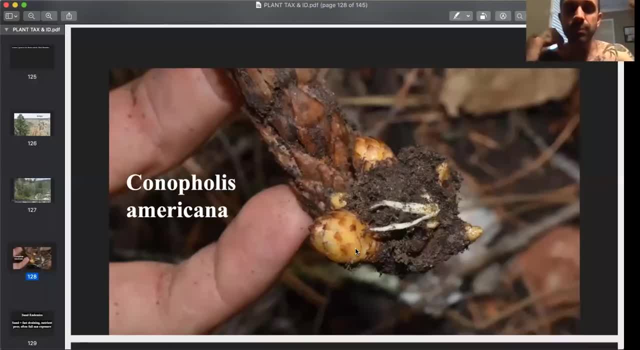 it's shaded to the where most of the sun comes from, to the south, so there's probably going to be some relictual shit in there. you're going to find stuff in that little glacial cirque or in that ravine that you're not going to find in the rest of the open exposed habitat up on the mesa or 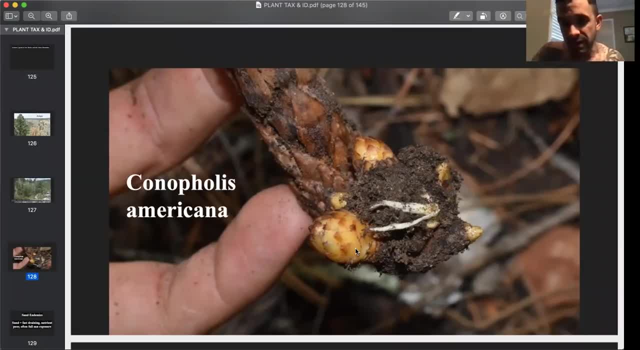 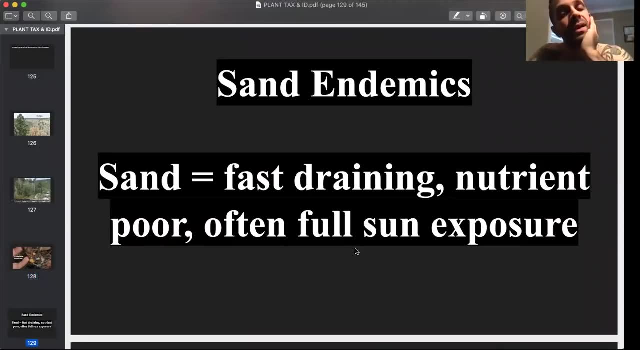 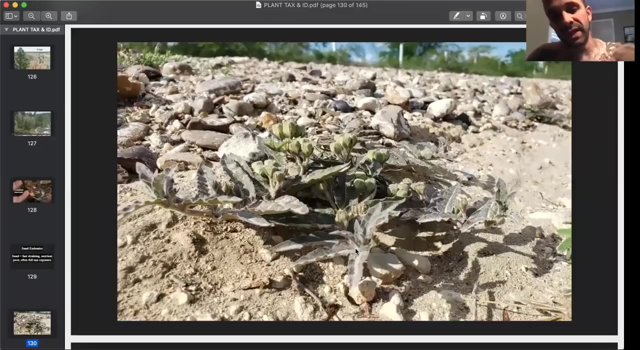 in the more you know south-facing uh air, you know alluvial fans or whatever, so it's always good to masturbate. become, become familiar with uh google terrain layer sand endemics. another example: asclepias prostrata, super rare milkweed that only grows in sand from the rio grande valley of south texas. this plant's kind of. 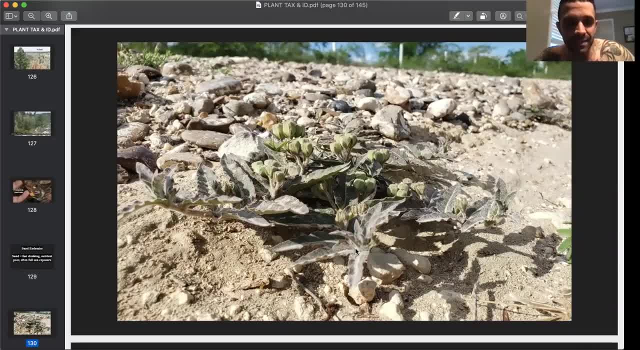 fucked. you know, state of texas is not. they've got no plan in place to protect this thing or preserve it. luckily there's some people growing it. i mean, in texas the most of the botany conservation work falls on the hands of private individuals. the state just doesn't care, you know. 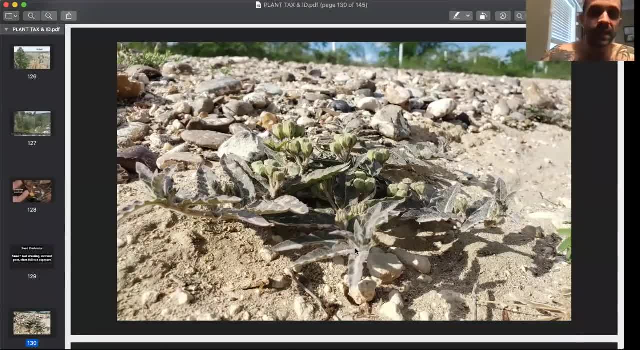 it's, you know, devotes a lot of money to it and there's all these fucking intense laws about you know you got to do environmental impact reports etc. but uh, anyway, there's a couple private individuals i know who are growing this plant. uh, san antonio botanic gardens growing it. 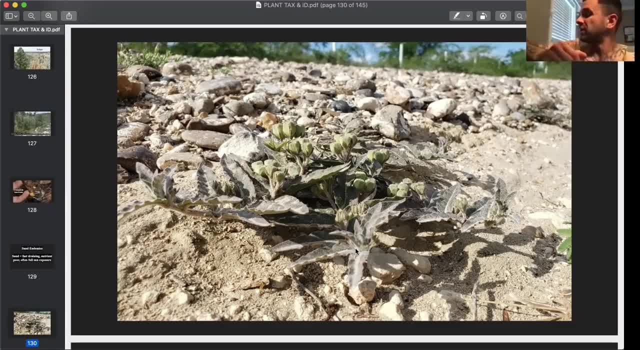 again. the seed was sourced by a friend of mine who's one of those private individuals. but this thing, it only grows in pure sand. again, you got that prostrate habit, just like the asclepias solanoana, from the serpentine of not not spending much time on it, but it's a. 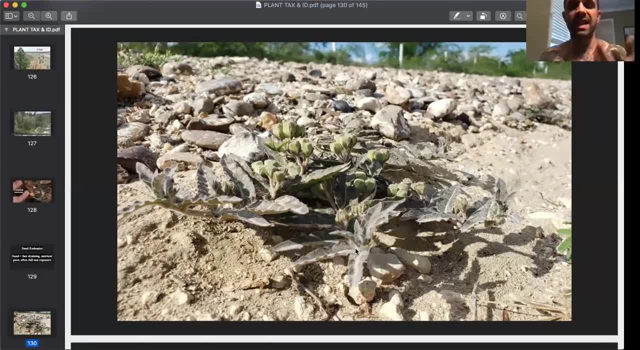 time forming, uh, you know, a stem, an aerial stem, because it's maybe it would just, maybe it's because it would just get gnawed down by herbivores, maybe because it's more adaptive for it to just be laid out sprawled on the ground- conserve energy. but either way, yeah, this thing's fucking right. 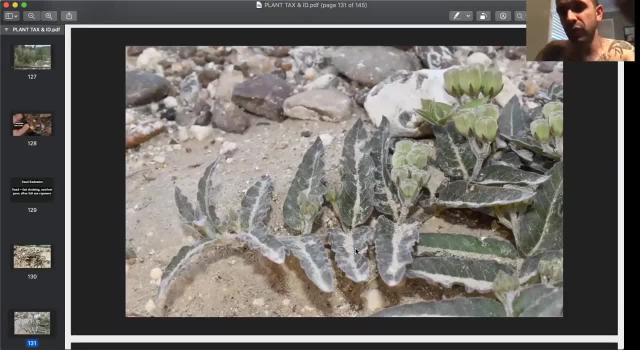 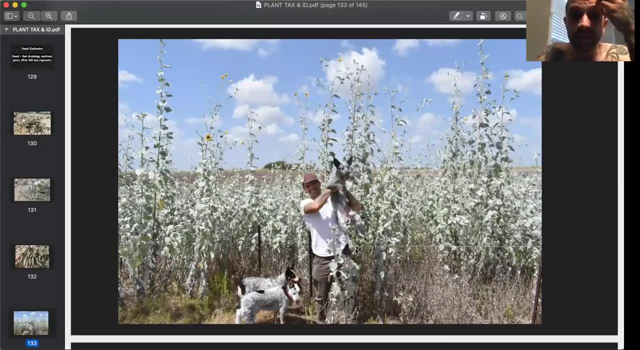 i've still never seen it in bloom. i i this thing bloomed two weeks later and i had to leave town. so, uh, another sand endemic right here. helianthus argophilus. i just put out a video on this. this fucking thing is incredible. these are annuals, so they only grow for one season, then they die. they grow really fast. 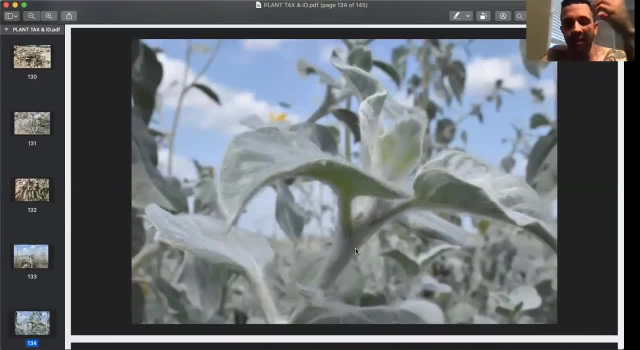 they're covered in fucking wool because again they're on that fast draining sand. so sand. the stresses of sand are that it drains really fast, doesn't hold on the moisture that well surface dries out, gets really hot. there's no topsoil there. uh, it's in a, it's in essence just. 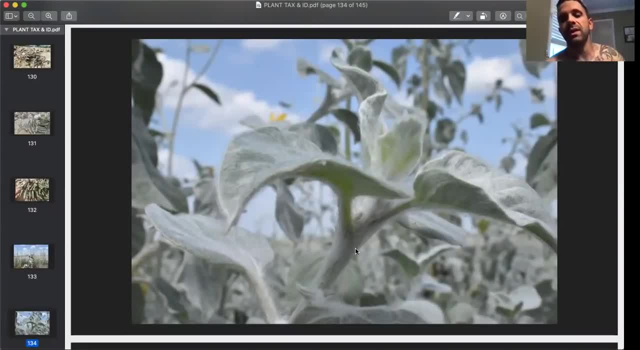 growing. in pure silica, there's no very little organic material in most cases, and so, as a result, you can't grow, you're there's no shade, you're going to be fully exposed, there's no trees to grow under. so you've got to cope, and one of the ways this sunflower species coped is by 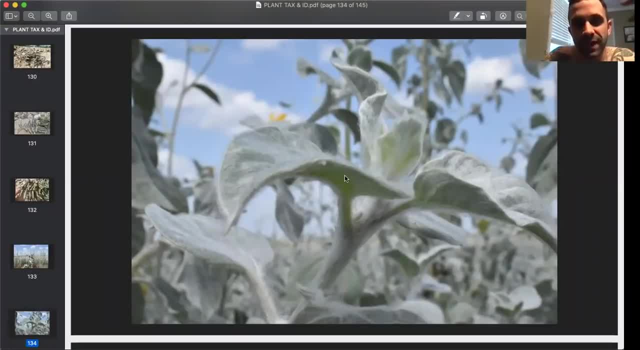 forming this intense indumentum of fucking wool. it looks like a cotton ball. i mean, it's incredible. um, so you know this and this thing can grow. it doesn't need to grow on sand. you can propagate this on regular soil, i've done it, but in habitat it it only grows on sand. maybe again because it. 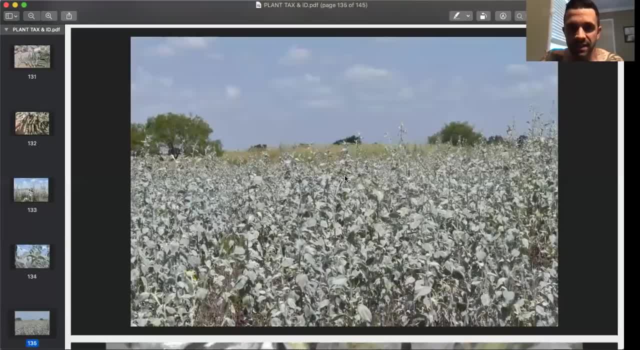 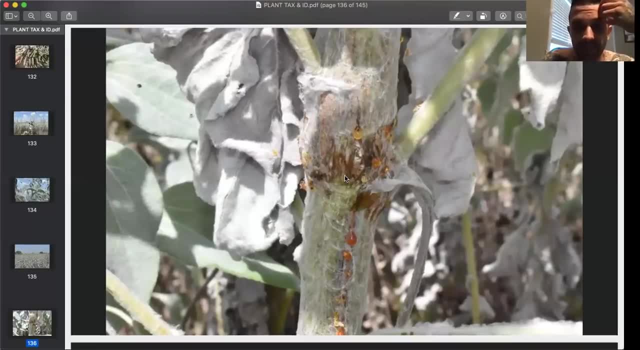 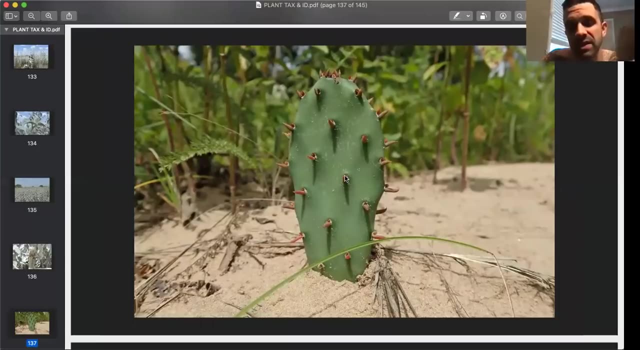 out, competed on non-sand substrates. so helianthus argophilus, silver-leaved sunflower, and it also leaks a lot of resin for any boring insects. so you know, we plug them right up. this is. this photo was taken 20 mile, 30 miles south of chicago. it's a cactus that's native to the. 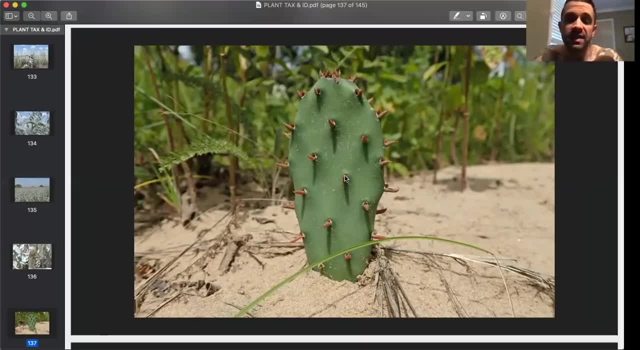 chicago region, but again, is only found on sand. and the reason the sand is there is because a glacial dam broke 15 000 years ago. uh, a glacier, the dam to a glacial lake broke, so you had this mass, uh almost instantaneous flow of water, and when it finally uh settled down, when the current finally settled down and all the energy, 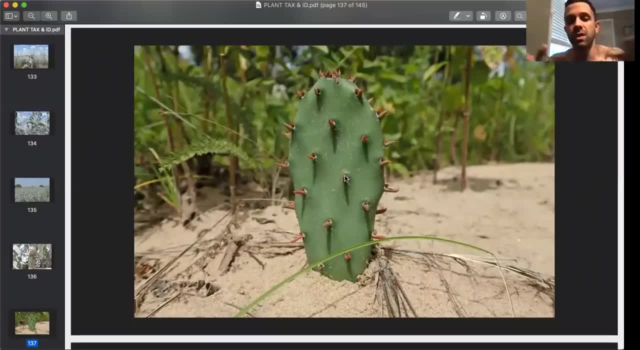 from this flow was was gone, and the most of the water was gone. it deposited this sand right here, just south of the city of chicago, and so, uh, this cactus opuntia humifusa thrives on it, because nothing else, not a lot of plants, can grow on this fucked up sand. it doesn't hold up. 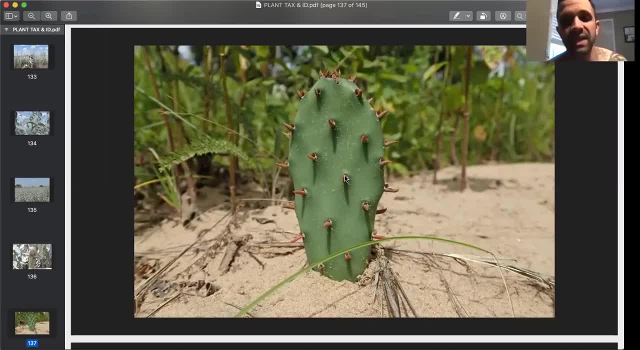 water, that much it's. it's very nutrient poor again, like we said, but that's not a problem for a cactus, which is in effect like a little battery. cacti store carbohydrates and water. uh, you know, you could throw there's. there have been research papers on this. there's been species of 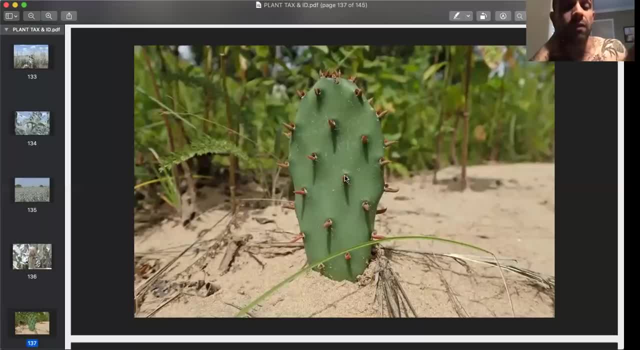 fucking barrel cactus that have been thrown in a closet for four fucking years, no light in the water, and when they're taken out of the closet, uh, they're put back in a medium and watered and given sunlight and they start growing again. i mean, these things can last immensely long and 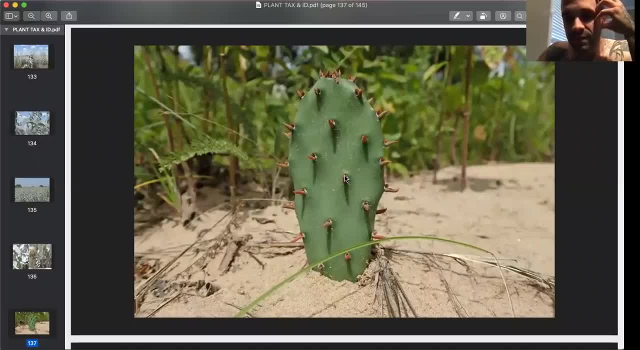 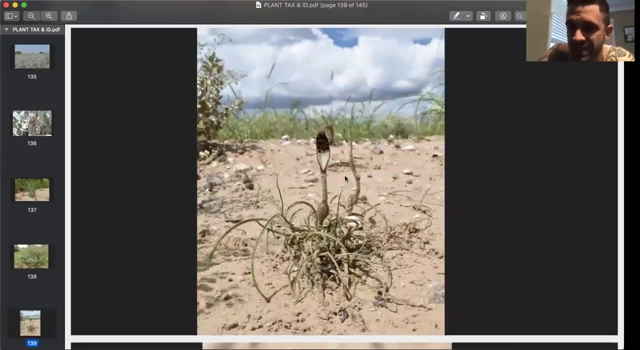 sometimes uh, with uh, you know none of the things they need to grow. so if you want to do a question and answer now- we're running into three hours and hopefully i still got your attention. i don't know how, but maybe i do- if you want to do questions and answers, just uh, let me know. do you know what's? 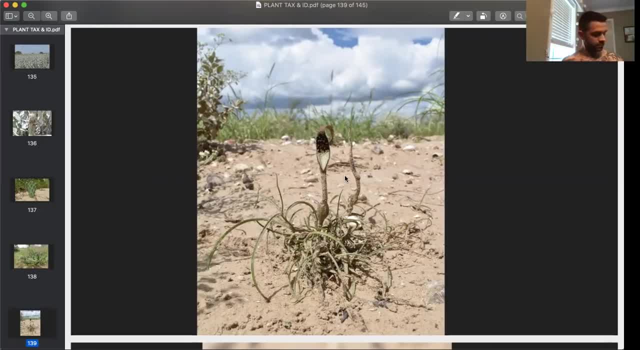 up with the um cypress that's sitting. butano, if it's still, if anything has germinated or anything, i'm kind of close to there, but i haven't really got up. if they're germinating, they would be doing it in the next few months. i'll take this down. that'll end the. 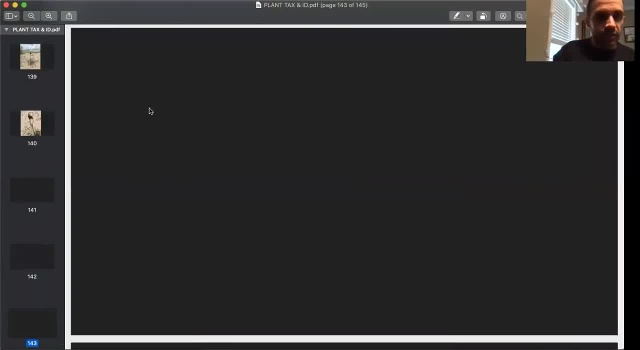 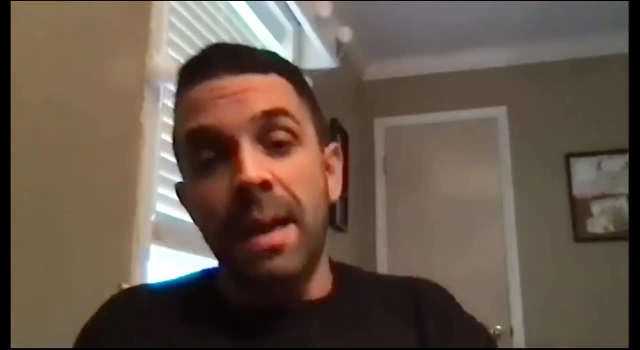 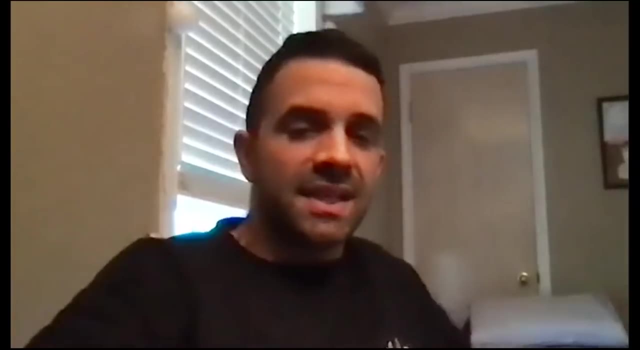 presentation. um, it's fucking over anyway, that was pretty good, uh, okay. so, uh, yeah, with the butano cypress i, i mean, i saw tons of seed when we were there. it was just, they were all over. i mean, you could squat down anywhere on that small football field, sand size, sandstone, uh, escarpment, and you'd 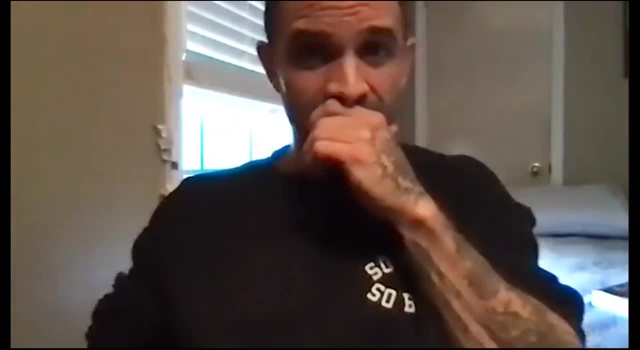 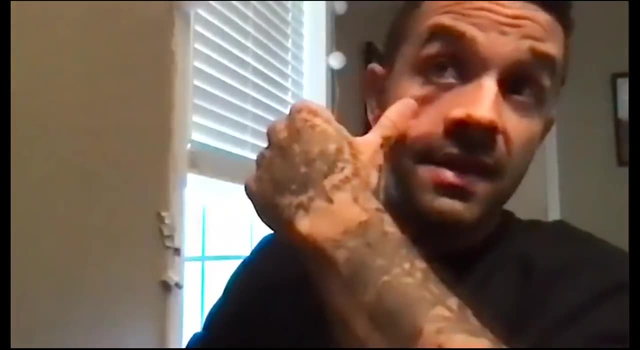 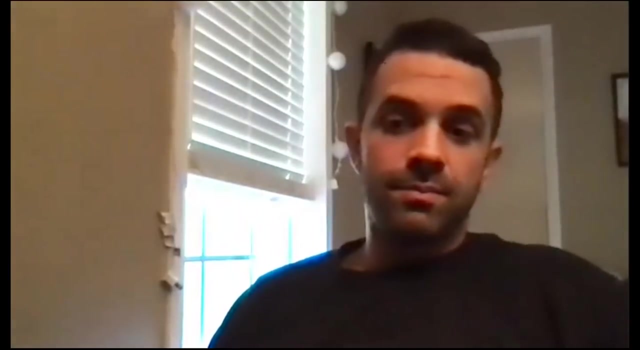 squat down and you'd find the fucking the cypress seed, you know. i mean, they were everywhere. so they're just waiting for, uh, waiting for enough moisture, and i guess they got enough. i dipped out of california last month, but, um, i'm not going to be back till april, but but uh, yeah it's. 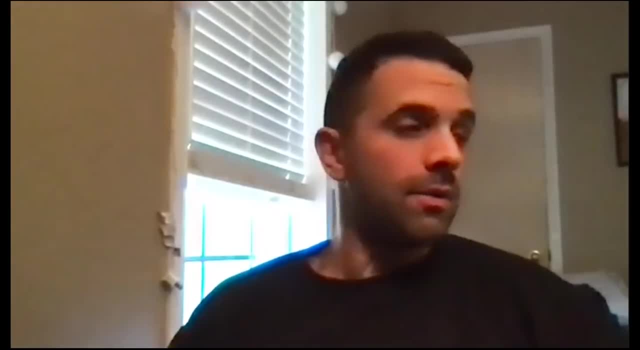 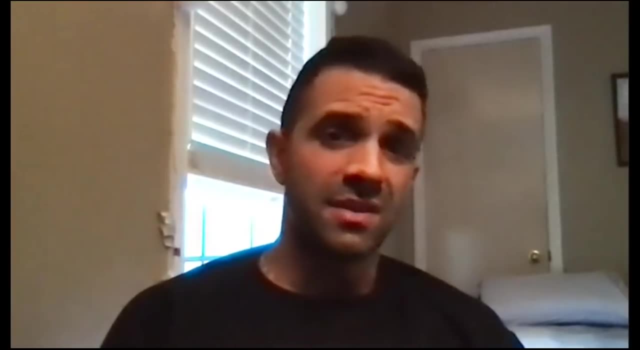 been raining like on and off the past few weeks. yeah, they'll be germinating, man. i mean that would be a cool thing. there's going to be a bunch of cool shit in that area coming back, because there's flannel bush in that area. i remember seeing flannel bush there 10 years ago. 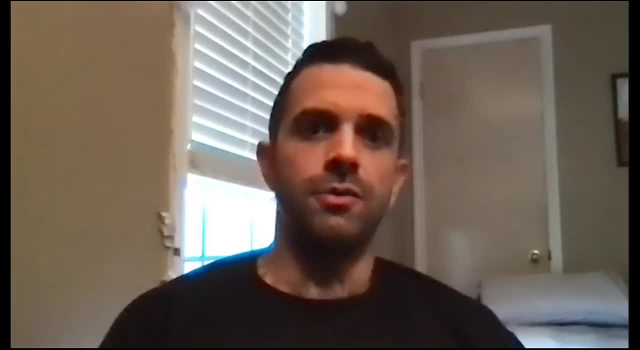 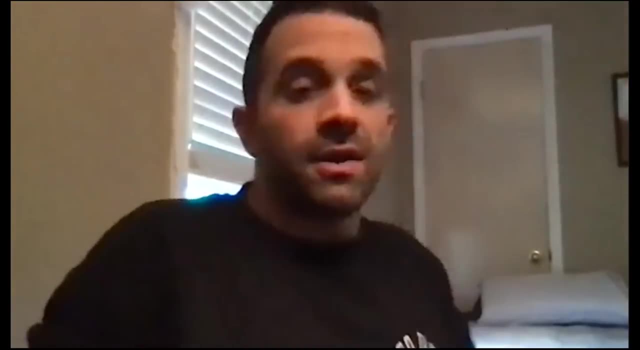 you know, not blooming but just the leaves and being like, oh no shit, there's formatted denner. i've talked to other biologists and botanists there and it's rare. like formatted denner is relatively rare for the santa cruz mountains, but that seed again, is still there. it's in the soil. 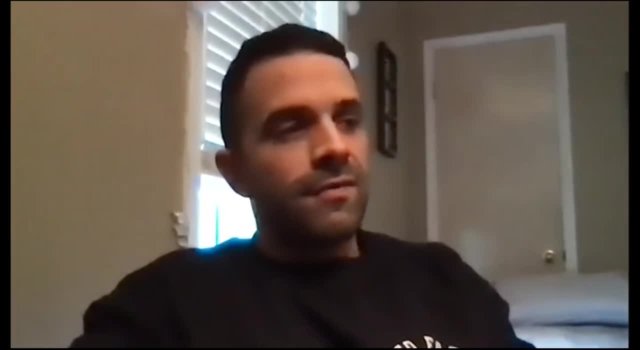 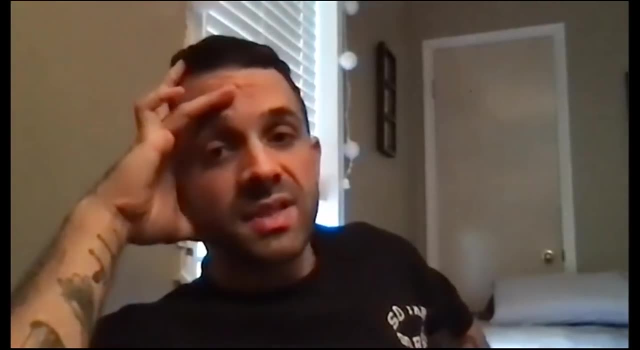 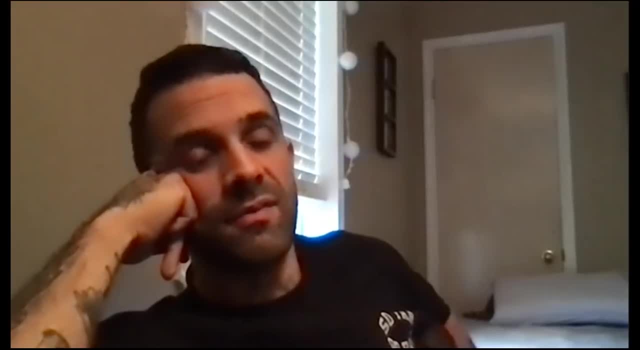 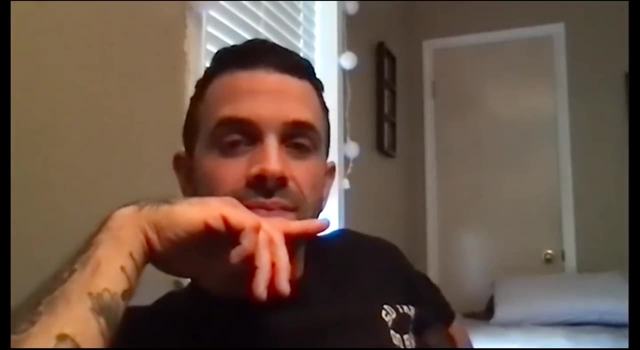 good shit coming back probably. i mean, it's going to be cool to see doing inventory there in the early summer. yeah, because i've seen like flannel bush down in monterey, but i don't think i've ever seen it in the santa cruz mountains. that's really awesome. yeah, yeah, let me say, do you really have? 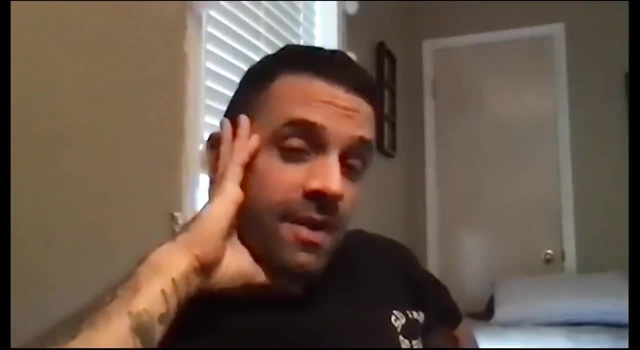 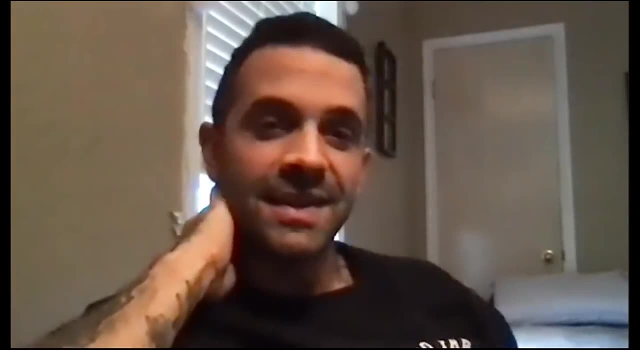 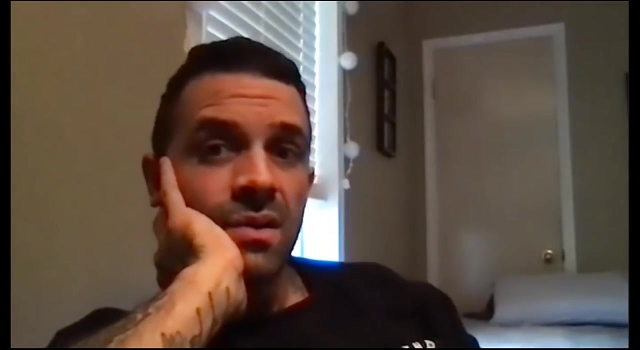 the ocean behind you, or is that like? no, it's just a background. my house is gross, so i have a pretty background. yeah, are you germinating any of the seeds that you showed us today in your presentation, like right now? uh, which ones? any of them? or? 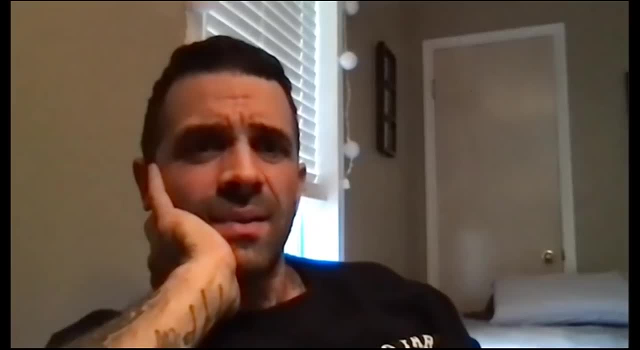 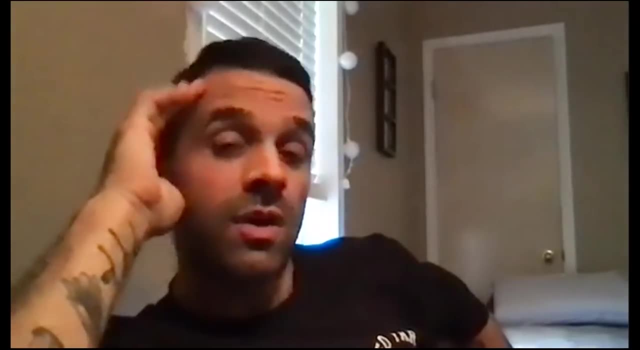 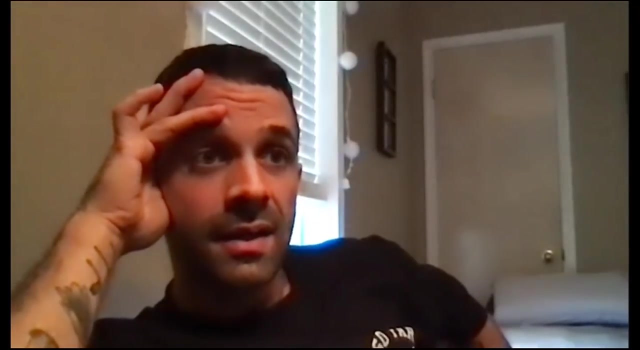 those lilies or tulip bulbs from the serpentine area. no, i didn't, i mean, you know, because i felt fucked up doing it, but i probably should have, because the that was trespassing on private land. i should have taken them and given them to a botanic garden. um, because the dude who owns 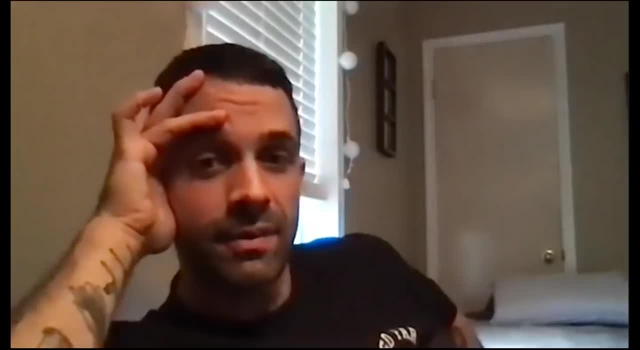 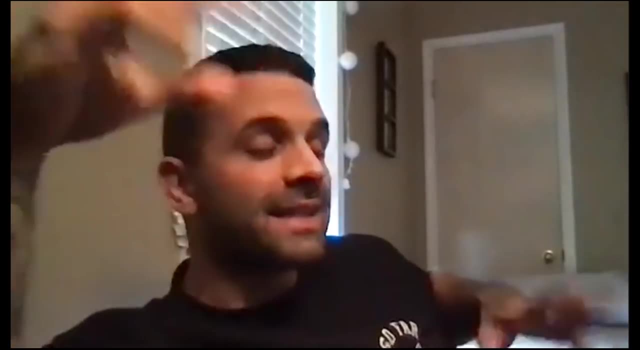 that land's a fucking dick. he's like probably one of the people that was storming the fucking capital two days ago. i mean he's, he's uh, and you know he's. that area is, like you know, california's all liberal, progressive, but like that area is super like fucking oklahoma. 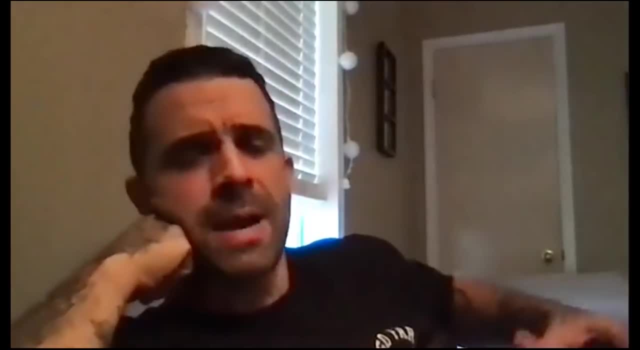 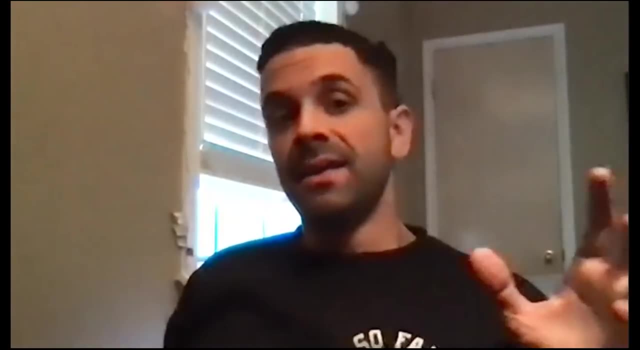 almost like super paranoid, super mine, my property, my property and uh, i should have dug up a couple bulbs, you know, because people do that actually a lot in texas- like a lot of the, the people, and that was something i kind of struck me when i first got here. i was like it's fucked up you. 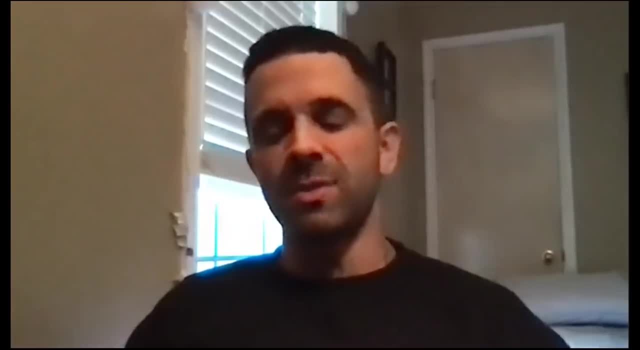 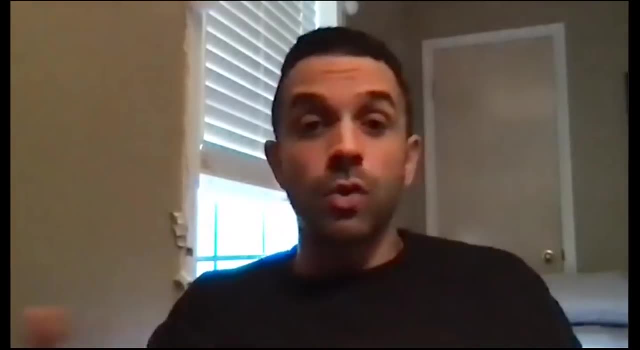 can't do poaching, uh, but in a place like texas where there's so much private property and a lot, i mean these guys were taking it not to sell, uh, they took it to to preserve. i mean, that's what we did in the fucking moving the cacti for the wall, right, i mean technically, we 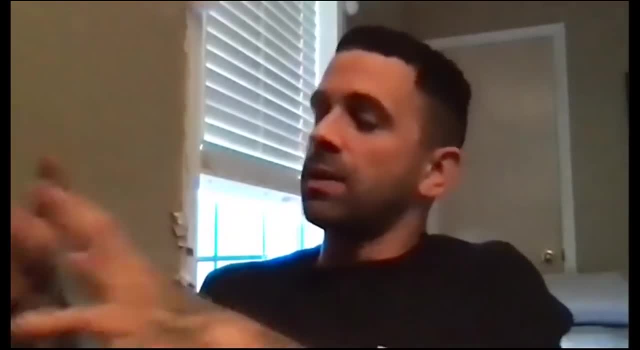 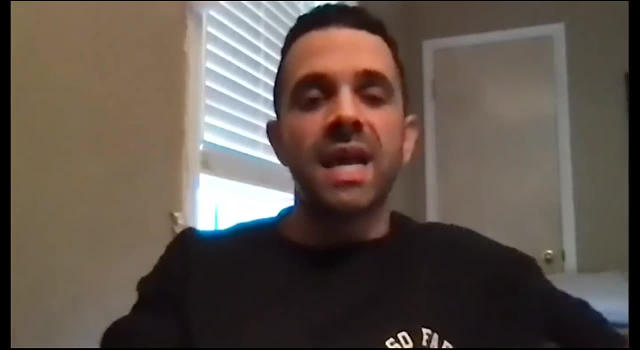 were fucking poaching. you know we're conserving those to give them to institutions that can take them or whatever. the plant should just be bulldozed anyway. but technically that's poaching and a lot of poachers will say, oh, i'm preserving, i'm updating the plant, it's just, it's a it's. 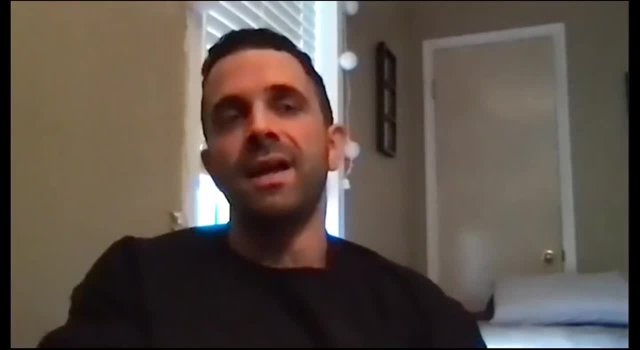 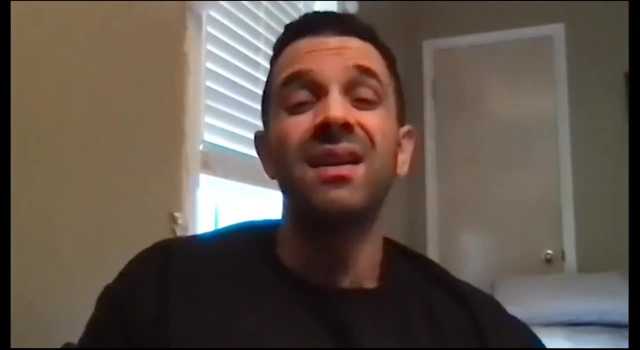 bullshit. they're not, but either way, i should have probably done that with that fertile area of. i mean they're, they're fine, but that area was getting trampled by cattle when we were there and that was something. i mean. a cow could fuck up that whole. a person steps on that habitat, those. 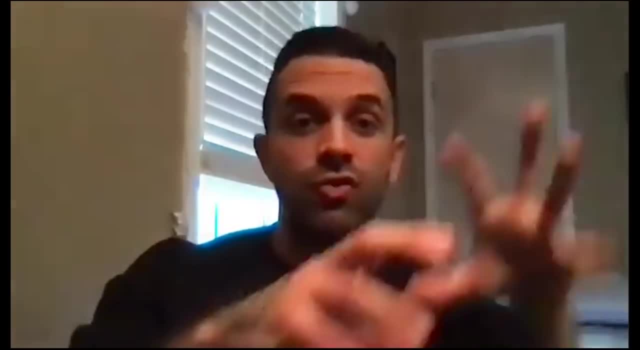 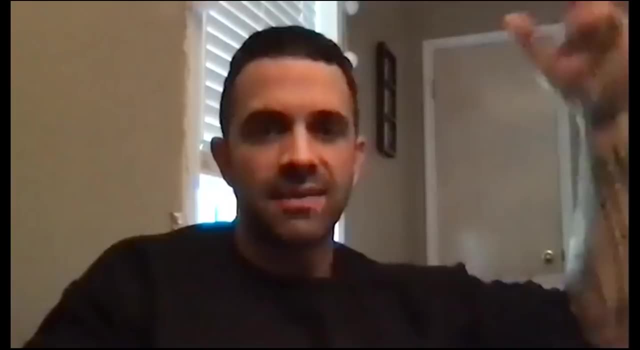 steep, talus, slopes and that shit just crumbles. i mean it just all falls down. i mean think of what a fucking thousand pound cow could do: just destroy it. i mean that guy doesn't give a fuck, the owner, he doesn't give a shit, he's flowers, fuck that. you know, i don't care about flowers. 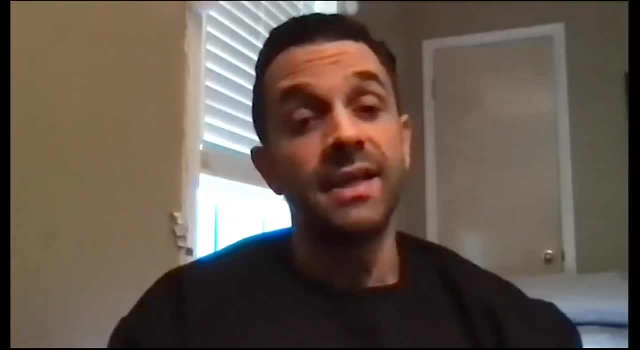 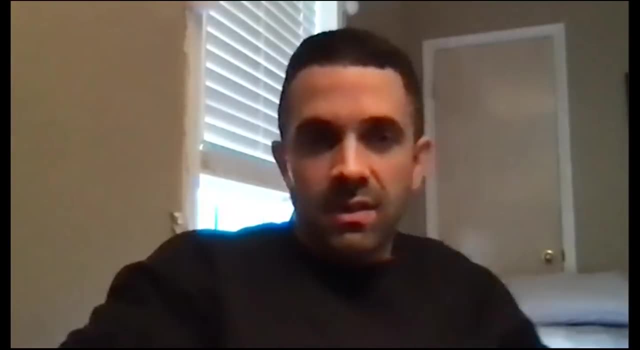 so, uh, yeah, i know i should have thanked him, but i didn't. um, but the important thing is, you know, as we see, because the tumor is not stopping- i say this shit all the time- the tumor is not stopping anytime soon. you know, plant conservation, uh, horticulture. 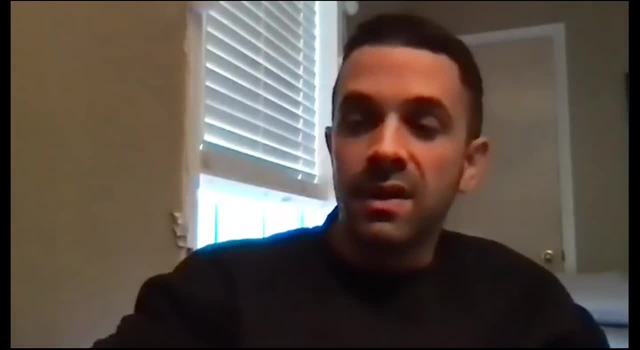 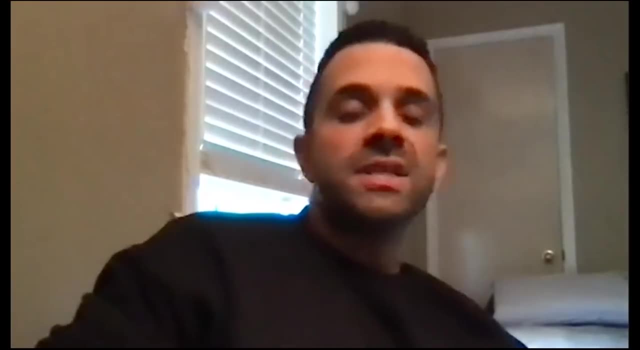 has a huge part in that, even if it's just horticulture in botanic gardens. that's not an excuse to poach, but it's. it's a thing to think about for those reference libraries of living plant material, material that are botanic gardens, you know. so that's, that's the thing, like i don't. 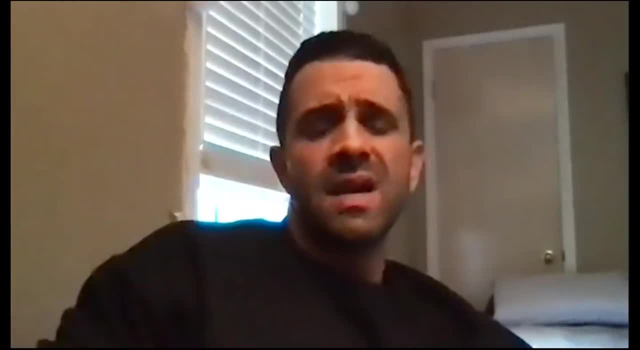 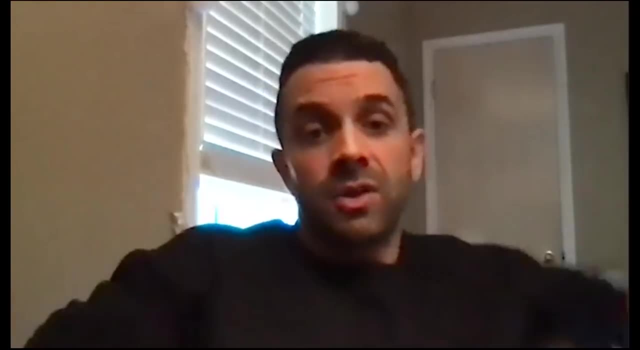 want to collect it, i'll germinate it, but don't fucking give it away, because i don't. i'm not home enough, i don't want to have to worry about it. if i kill it, you know it's- i feel like shit. so like i got an ambarella germinating now in back in california, when that thing's big enough, i'm. 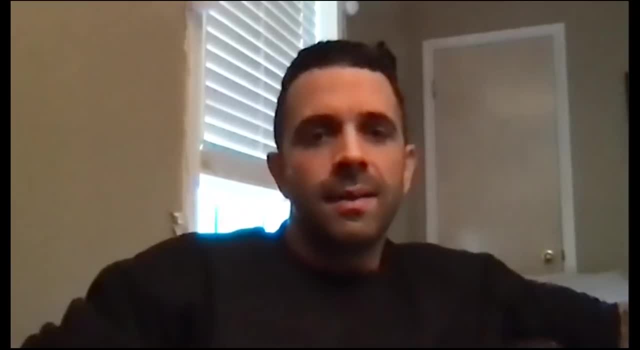 giving it to uc berkeley. i don't fucking want it. what am i going to do? what am i going to keep it in my, my little, my personal collection? it's mine, you know it's not. i want people to be able to enjoy it and learn from it. that's a really important plant to have. people can take cuttings. 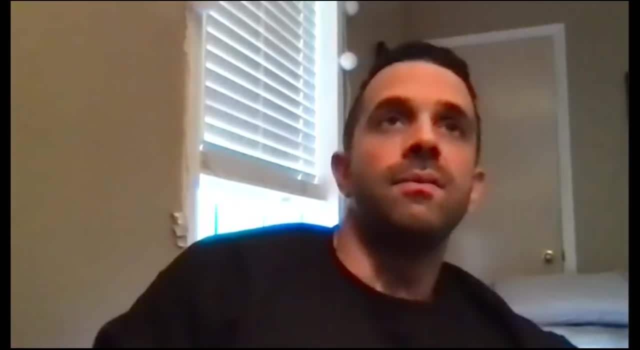 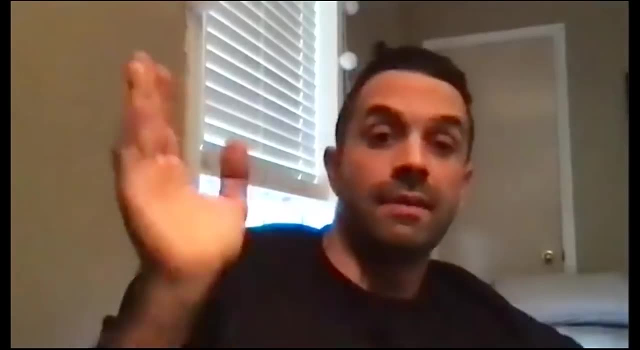 from it and, you know, propagate it. so but no, i didn't. i mean the stuff i'm germinating now, like i got a bunch of texas stuff that i'm just i just sewed in the, the ground outside because i was like i don't want to fucking deal with it. you know, i um, i got a. 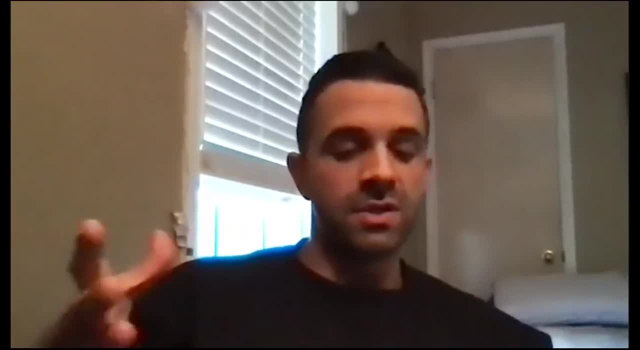 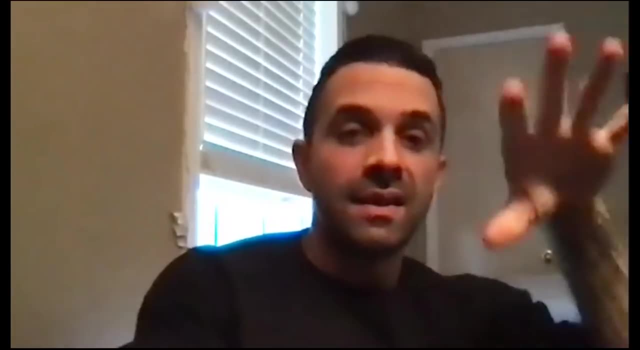 little grow dome. uh, i actually just bought like a storage thing at walmart's thing, kind of lifted one of them, uh, self checkouts your friend at walmart and uh, and got some led lights. and you know the purpose of that is to keep the humidity up. you poke some holes in it so you get a little. 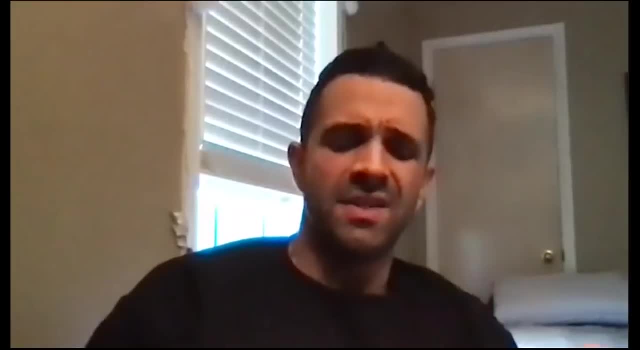 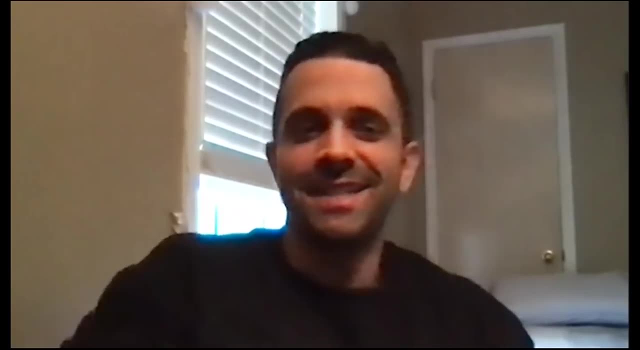 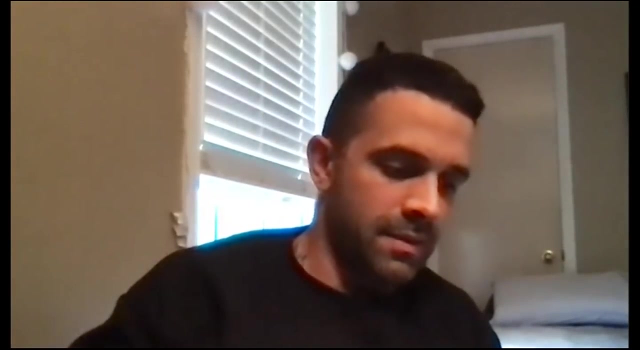 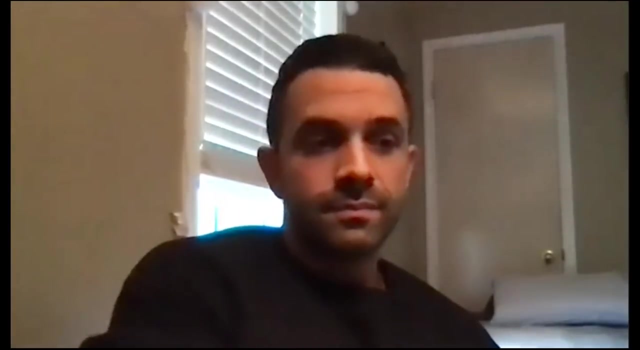 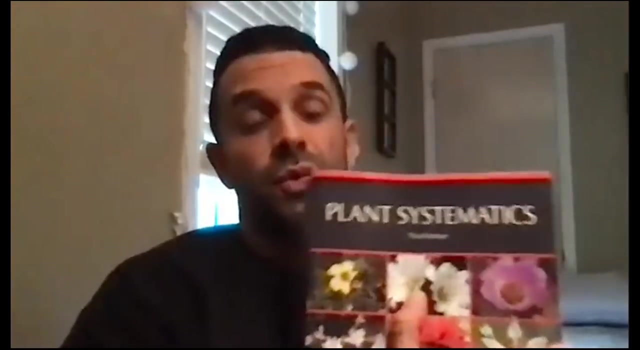 bit of aeration, you can grow the shit on your own. fill the bottom with soil, because the soil drops when you're niching. it's probably the same as when you're doing a big shelf. this one, the 2018 man. get this if you can, because with, like i was saying, geology, not a lot has. 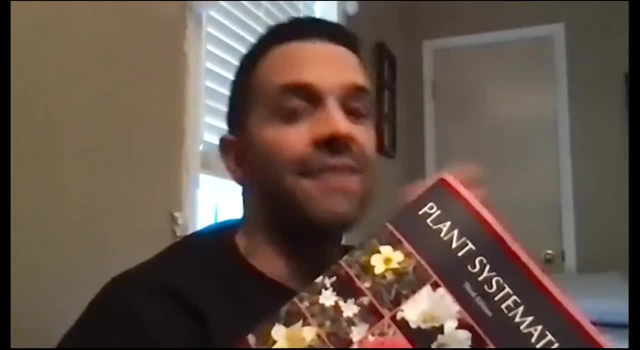 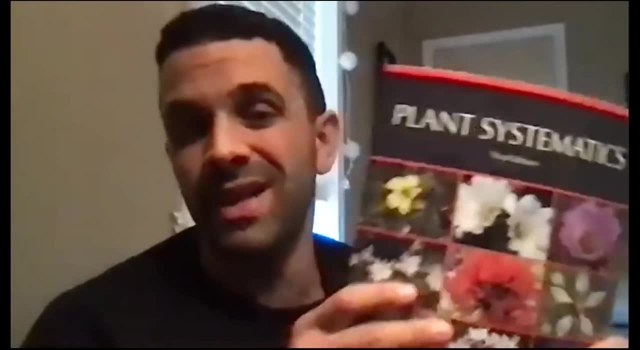 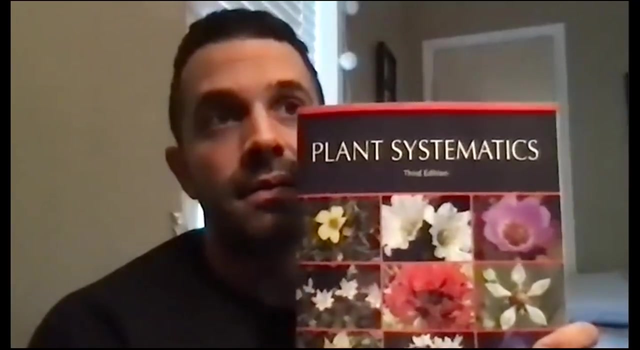 changed but with plants like, shit's really been fucked up in the last, not fucked up, it's been more elucidated and articulated, but the newer edition is the shit to get. i mean really either one. good, this is actually somebody put this on libgen, it wasn't me, um, but uh, another video. 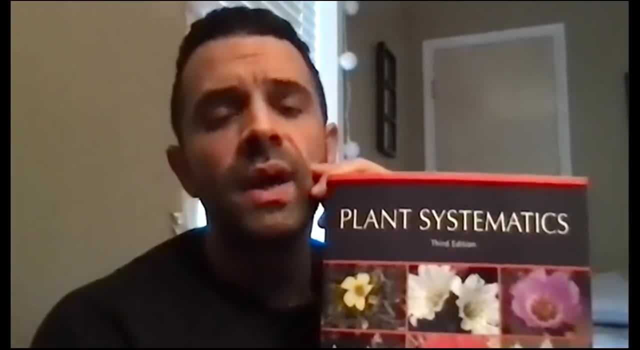 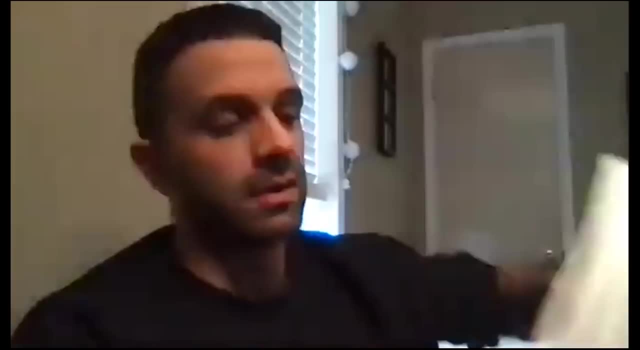 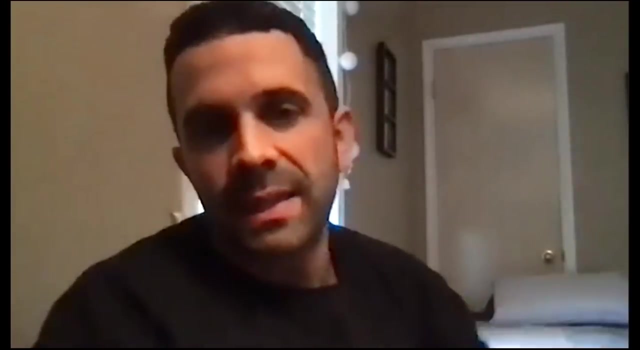 what i don't fucking forgot to mute the mic. anyway, i would get this one, um. like i said, hard copy is always better and mike simpson gets some of the money, but if you steal it on libgen, even just you know, find a way. maybe i can get venmo in 10 bucks. i don't fucking know. you know, um, because 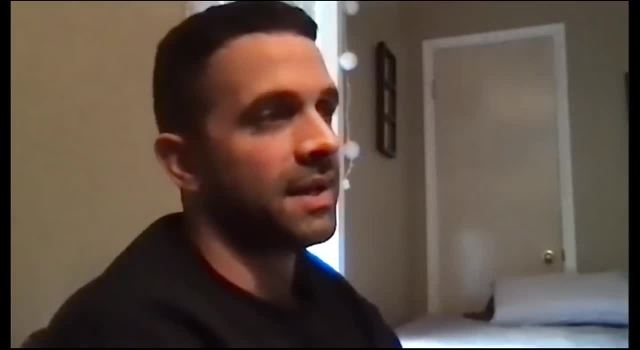 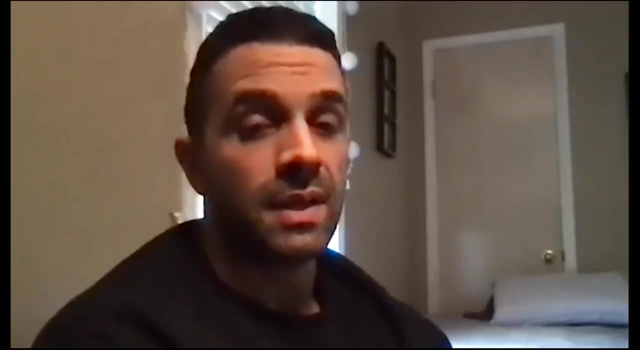 he's a cool guy and he's uh actually trying to do a podcast with him. uh, he hasn't responded. we've been emailing back and forth but he hasn't gotten back to me. he hasn't gotten back to me. he hasn't yet. once i asked him. but, uh, but that's something where, like, there's a lot of new, updated taxonomy. 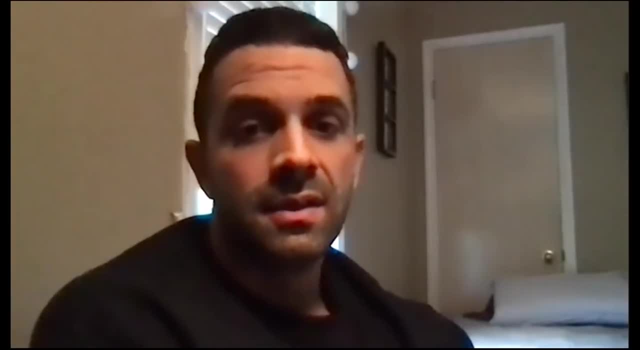 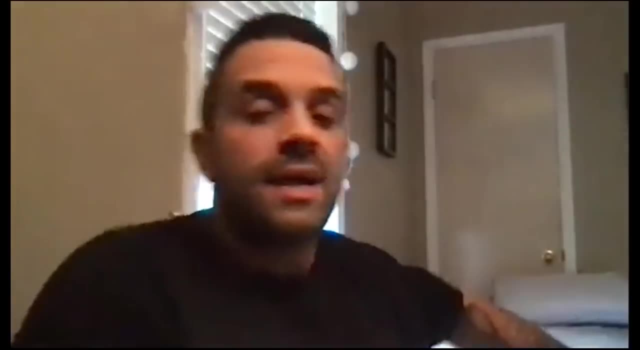 because taxonomy is still changing. it's still going to change. uh, as you know, there's a lot of families and taxa that haven't been sequenced yet. no one's done molecular phylogenam yet, and so, as as people do that, we'll gain new insight into these relationships. i would definitely get the 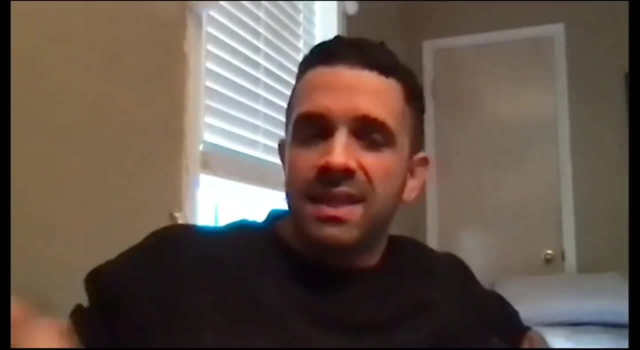 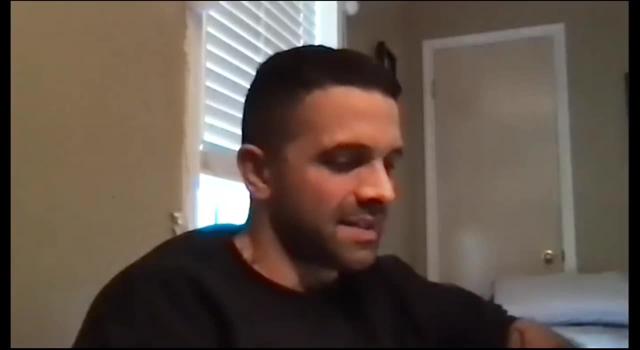 new one. i mean it's. it's on libgen, you can buy it on am. i don't even know how much it is on amazon, but uh, it's probably like 50, 60 bucks, but i mean 60 bucks. if you got on something you're going to use for the next 10 years, it's not, you're not. 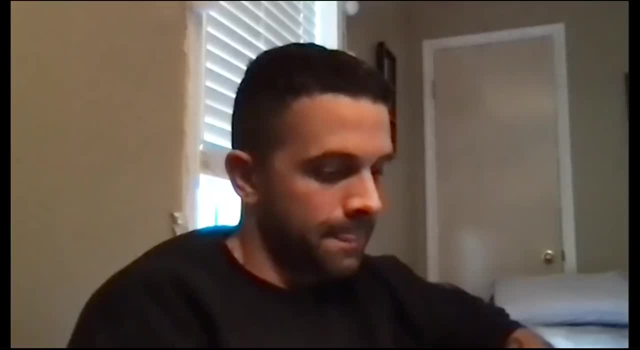 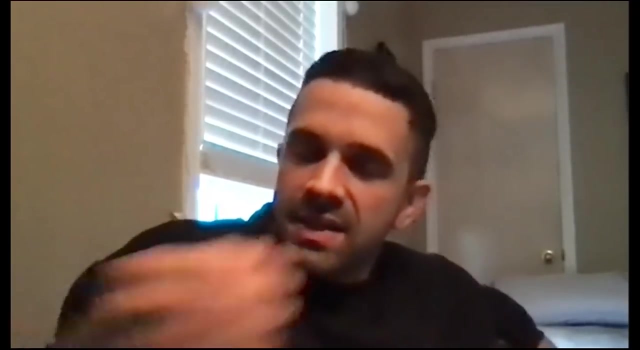 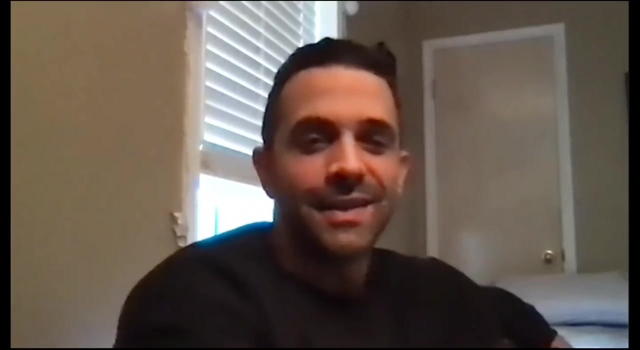 wasting money, you know. thanks, um, yeah, what's up? next question: um, do you have any information on the um escalopius prostrata growing on the mexican side of the river? no man, no, it's, and that's that whole side is like where it's like the base camp for coyotes, you know, for like coyotes and smugglers. 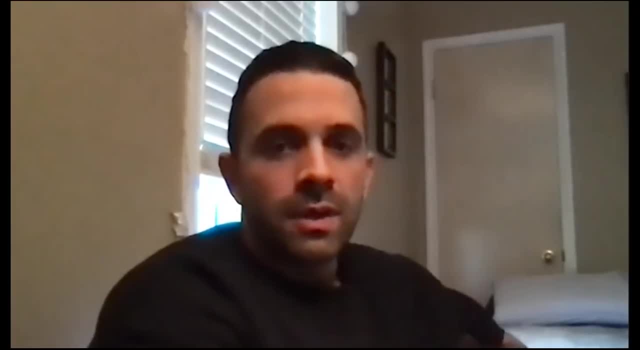 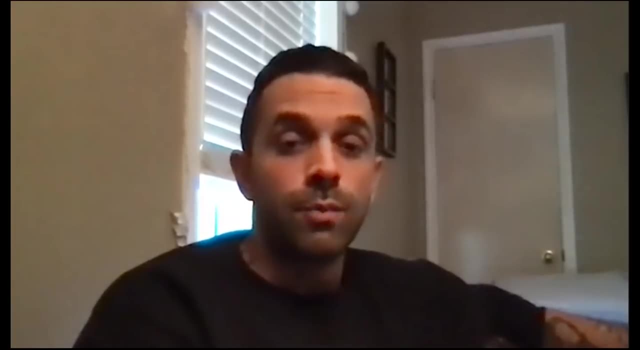 and i think you know, if they knew you were looking at plants, they probably wouldn't give a shit. but it's an area where, like no one's gonna think that you're there to look at plants. they're gonna think you're there to, like, move in on their business. you're trying to smuggle people too. you're trying. 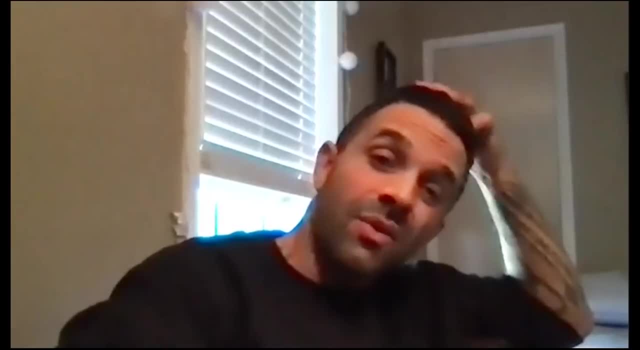 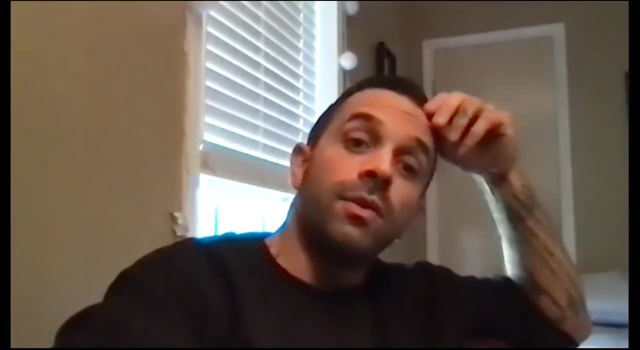 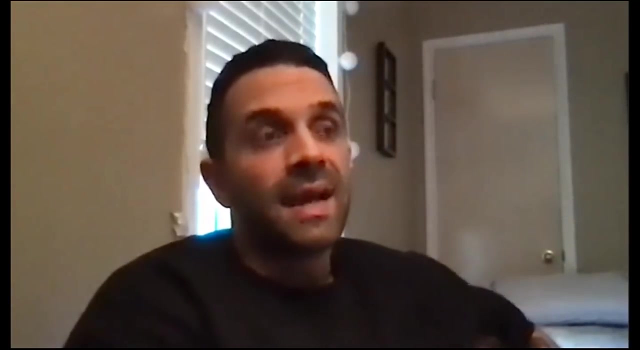 to smuggle drugs too. uh, you know so. no, i mean there's, there's a whole wealth of fucking plants there: astrophytum- uh, kaput, medusa medusa. medusa, i would have fucked you just pronounced it, latin it pronounced, i never fucking went. but that's another really wild fucking cactus. i mean, it's a weird. 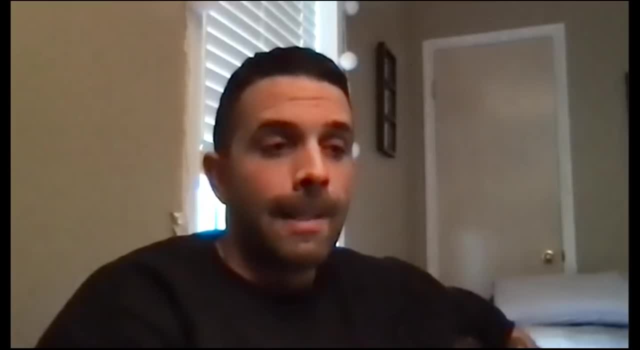 fucking variation on the genus astrophytum. you can't. i mean you could get there, but it's. there's a little bit more risk involved. it's just a fucking hot area, you know, and that's the again the result of poverty and inequality and all that shit, that the gravy seals don't want to pretend. 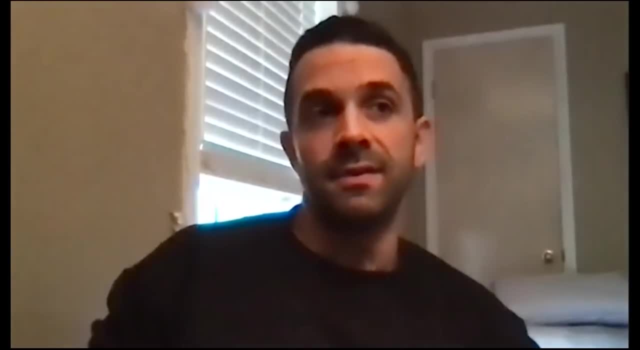 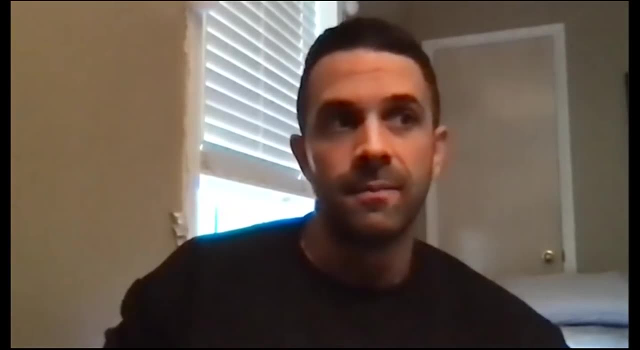 exist anyway. uh, without getting into that, yeah, there's a bunch of uh. hopefully one day shit will die down a little bit. you can go botanize there, but right now it's no. i have no, i have no clue. i mean, there's a couple people in inat. lex garcia is a cool one he's. he does a lot of. 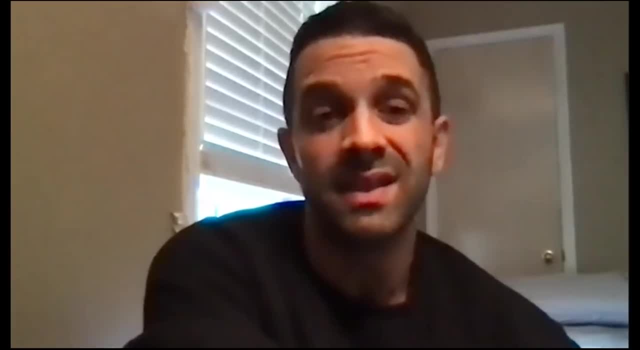 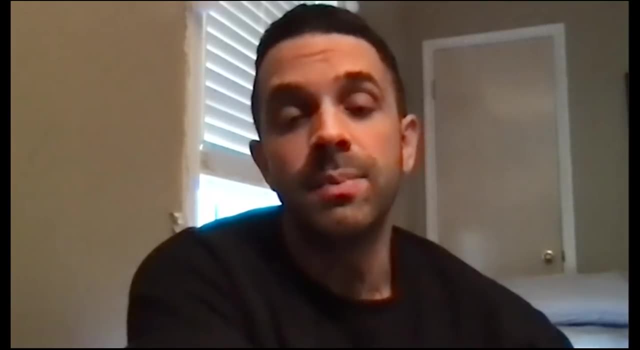 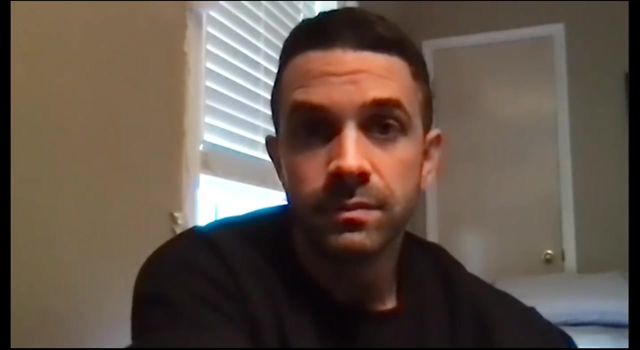 he's got a lot of observations in that area. you know, i would check. i natural that'd be the thing to do: go to explore type in asclepius and type in uh, tamalipis, which is the state that it's in, see what comes up. yeah, i mean, like um with inat, i think when it like when the observation obscures. 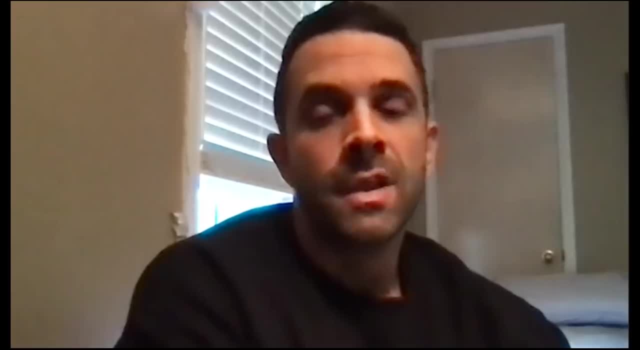 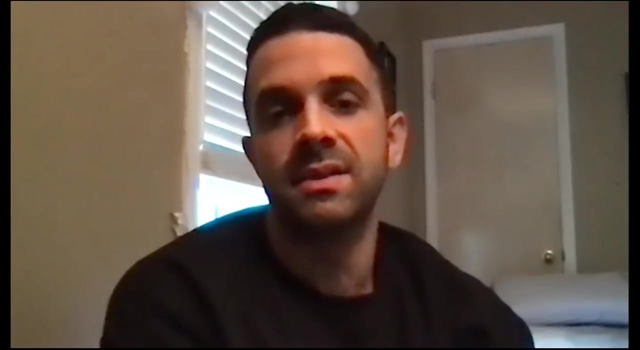 from texas go over into tamalipis and it, um well, the border does, the rectangle does. but if you type in tamalipis in that field, it'll only give you things that have been observed in tamalipis. so that obscure, blurry green rectangle will maybe cross into texas, texas, but it'll only be the. 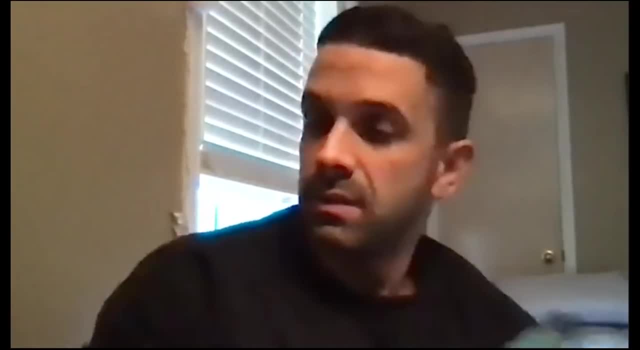 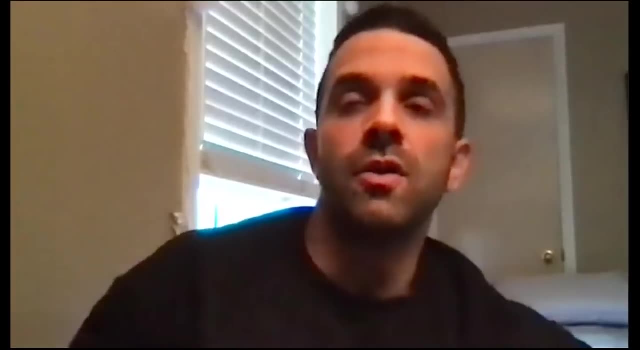 shit that's been observed in tamalipis. so yeah, but that's the cool, i mean fucking. yeah, that's a cool, but we just discovered another population of that, which i guess was known by one or two people already, but uh, and it had a fruit, but this fucking dude, i know, picked it not. 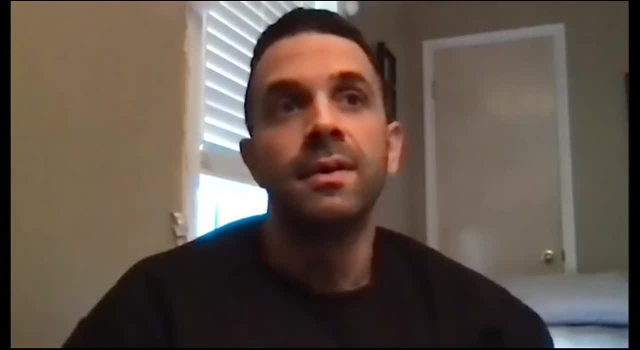 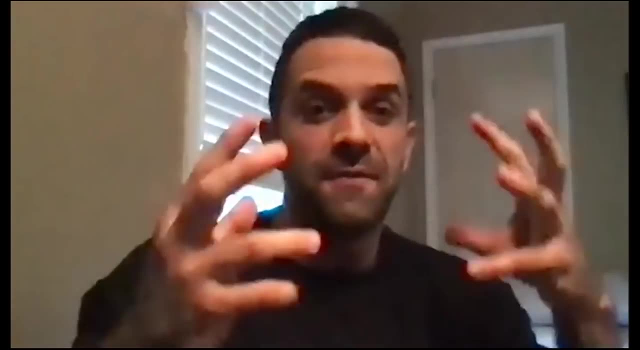 a bad guy, not, not, not, you know, not shitting on him, but he picked the fruit, uh, prematurely, and i remember seeing it and i'm being like it's not ready yet, i'll come back. and i came back and it was gone. i was like, ah, fuck mother, fuck you know, and i thought, oh, i picked it. i thought it was. 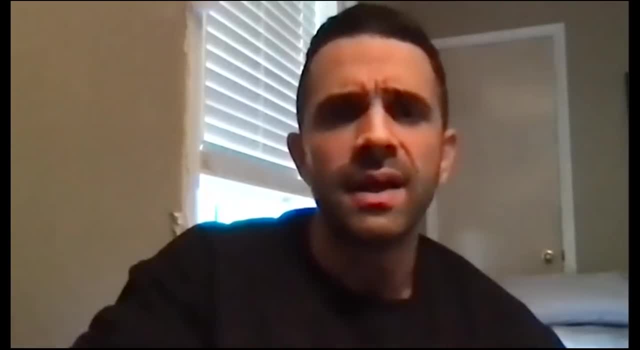 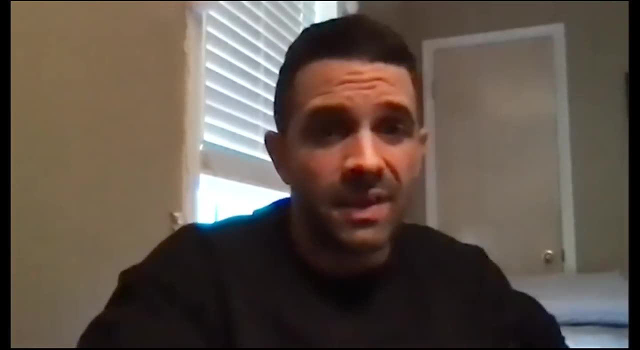 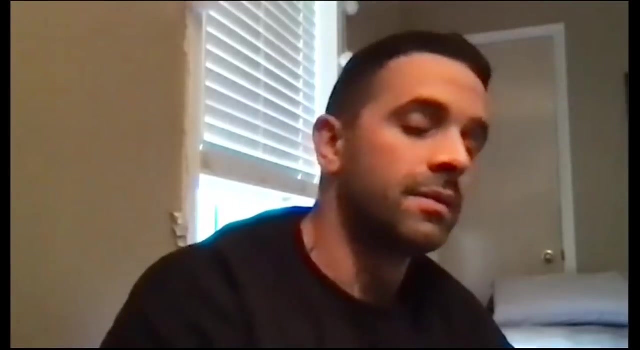 great, you know, and seeds were still white. they weren't brown yet. uh, they were still. they needed more time. you know, i'm just like, oh well, oops, and they're trying to build the wall right through where that population is too. hopefully it'll, it'll stop. i mean, because fucking wall was just a performative effort for, uh, you know, pig dick. 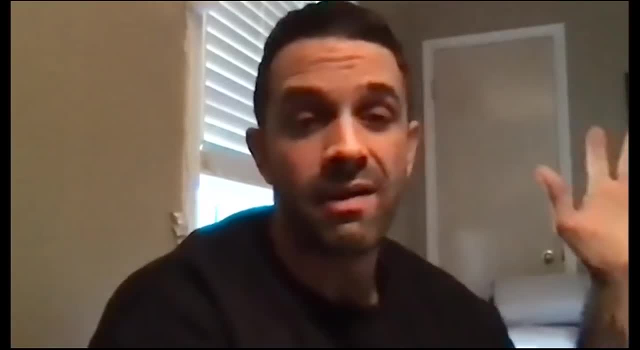 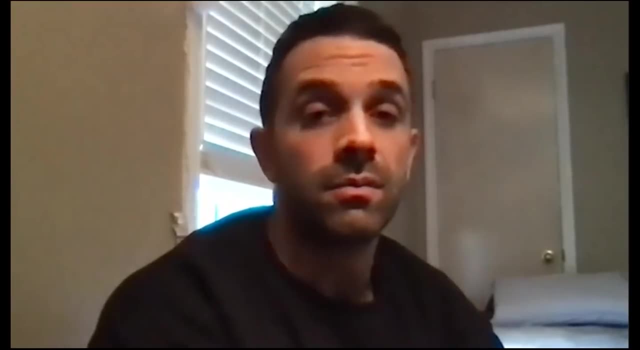 anyway. so i don't know. but there's other areas. they're speeding the wall up. they're like we got to get at these sleazebag constructioners, like we got to get it done before, uh, you know, before our time's up and biden cancels it. so, um, i don't know. i don't know what's going to happen, but it's. 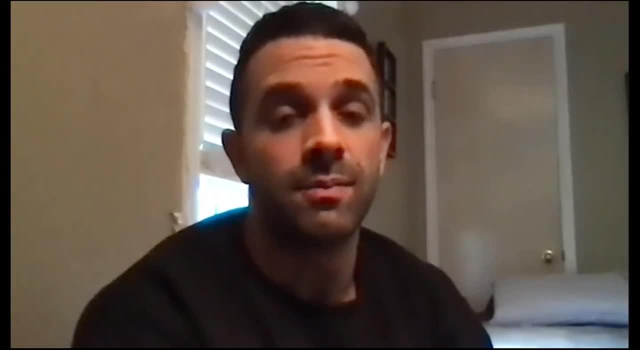 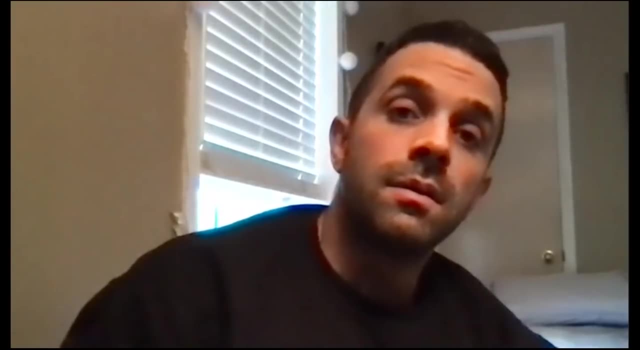 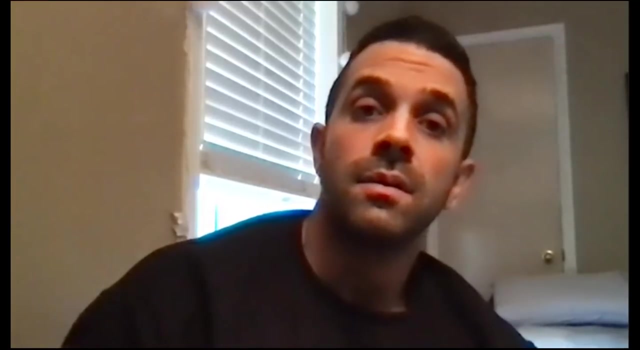 where that grows. that the one i just found is like one of my favorite places in south texas. it's cool letting people on there. so, um, i found one, like i was down there and i found a. i found one of those liquids with the follicle had just burst open and i thought about taking. 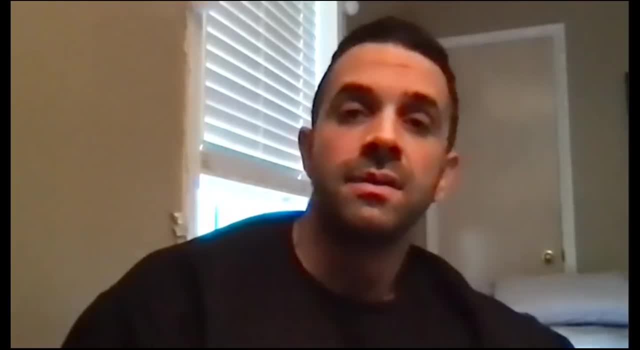 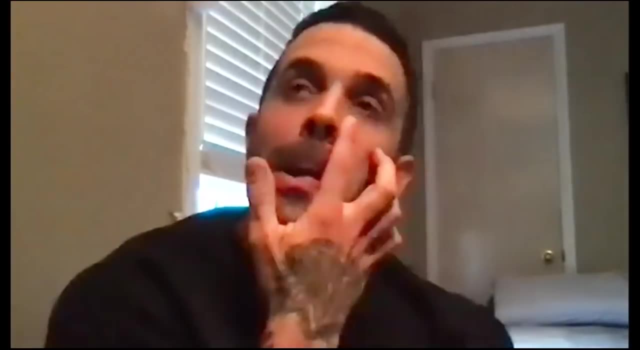 the seeds and i was like no, i shouldn't do it- of prostrata. yeah, i mean with that plan, almost it's like maybe, man, maybe you should have because for whatever reason that you know you should have, and then give it to someone who could propagate it, like i know i, i feel like i feel like such a. 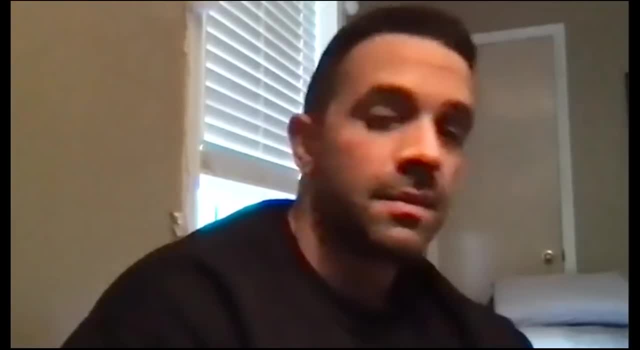 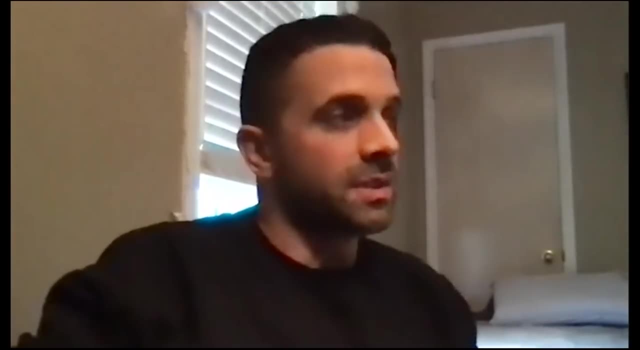 because like wait, where's the, where are these seeds gonna land? and eventually you shouldn't- i mean eventually you shouldn't- take seeds of rare plants unless you're gonna conserve them, you know, or give them to someone who's not gonna fuck up growing them. but you know that's a good thing to. 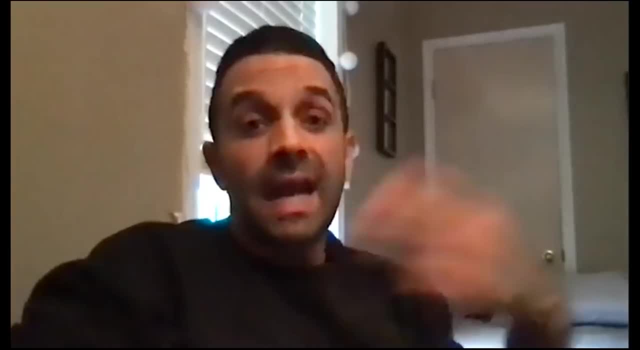 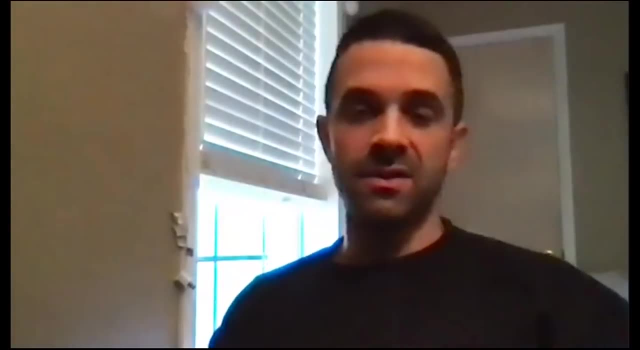 keep in mind. but i mean there's of course exceptions. i mean i've thought about that too. i was like like i was gonna go back and get that uh prostrata fruit for my friend michael eason, because he works at san antonio and works them a bunch, and i was like you know, and 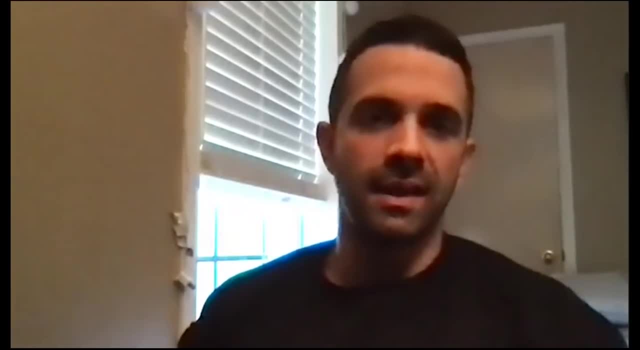 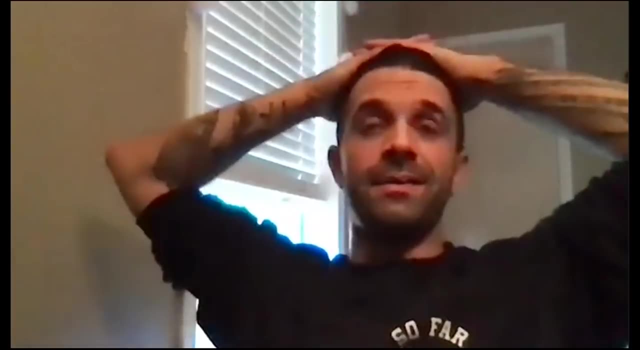 he was like: oh shit, okay, i told him it was there, like let me know, and then i went back to get it and it was fucking gone. i was so bummed, um you know, but there's, there's always next year or next rain. so yeah, you know, i carry, like i said, i carry those little drug baggies. 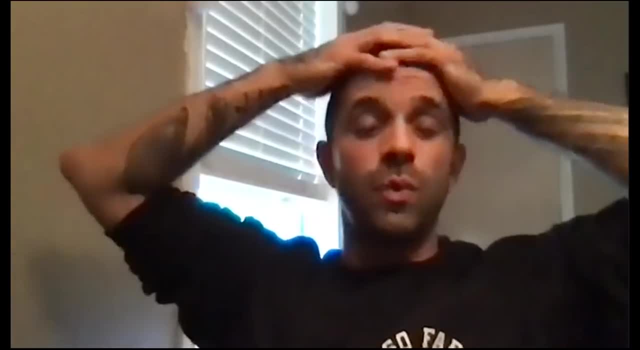 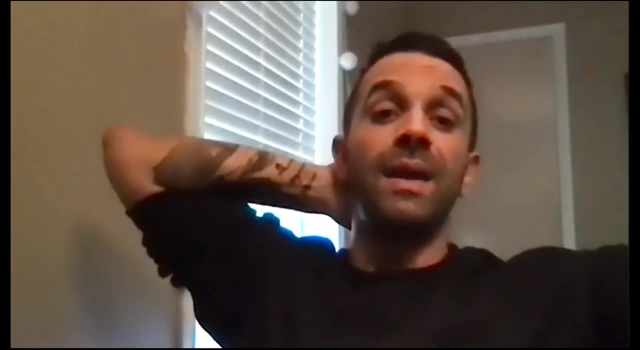 around with me. uh, that only works on dry seed. if, like, the fruit is still wet or the seed is like it's a cactus seed, it's still wet, i put it in the drug baggie and bring it back with me, and then, of course, when i get home, i'll, you know, find a way to air it out, dry it out. i'll take it out of the. 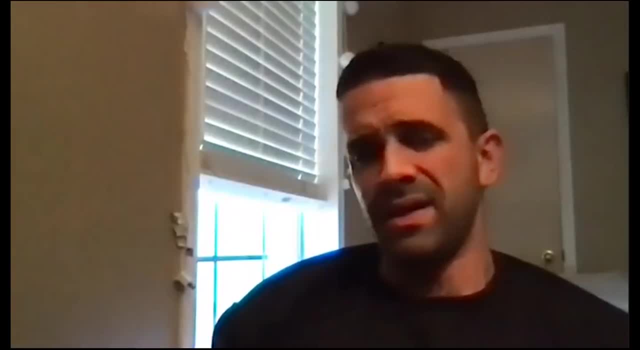 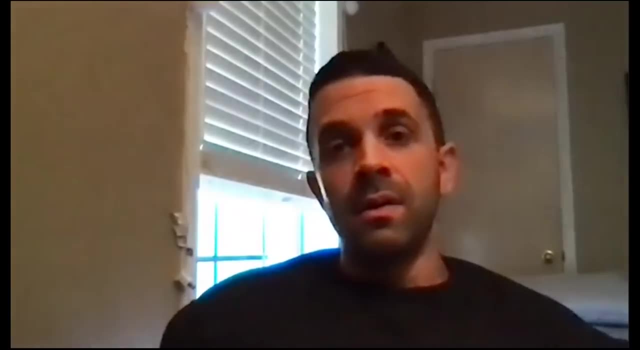 baggie. put it in paper. paper is generally better, but uh, the baggies are fine, you know, so anybody else? i received some seeds of various astrophytum from mexico and i'm about to sprout them, sourcing limestone and rocks that they prefer. how would you go about that? i live in. they don't need to grow on no limestone, except for pigs junction. yeah, they don't need. they don't need limestone. i mean, it's anywhere like peyote, like peyote seeds and habitat only grow on limestone. uh, but you could grow them on anything, i mean, they're just you just got to provide the. 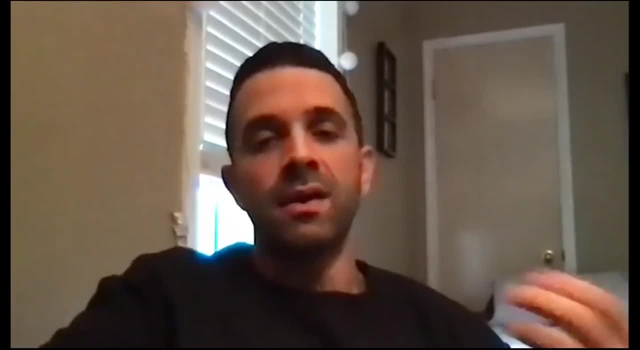 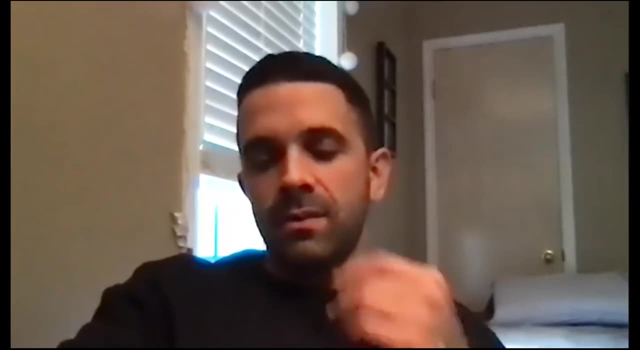 right conditions. again, it's one of those things that do they need the limestone, or is that just where? uh, they have a competitive advantage and they're evolved to it. um, there's different. you know, whatever, when anything's in cultivation, you can baby it, you can. it's not the same as 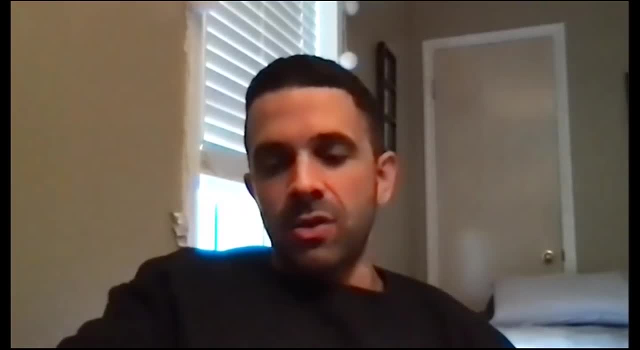 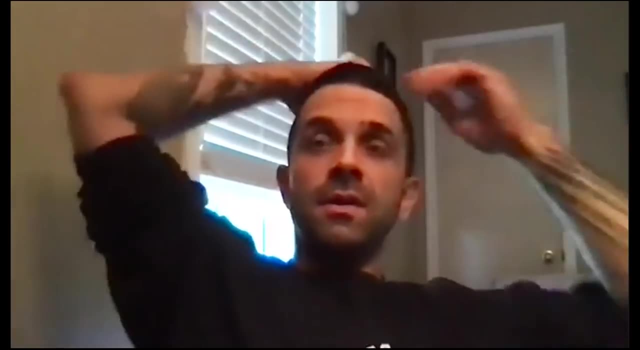 environment, obviously. so you don't need limestone. you could. just what you will need is a fast growing species. that's going to be a lot easier to get things down, but i don't think it's going to be that easy. but if you have a lot of things that you have to be able to get them from seed, i mean. i 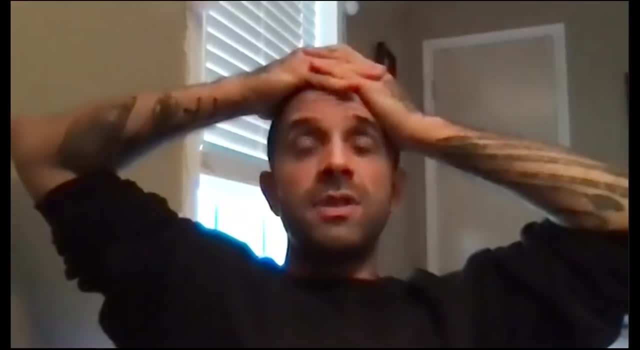 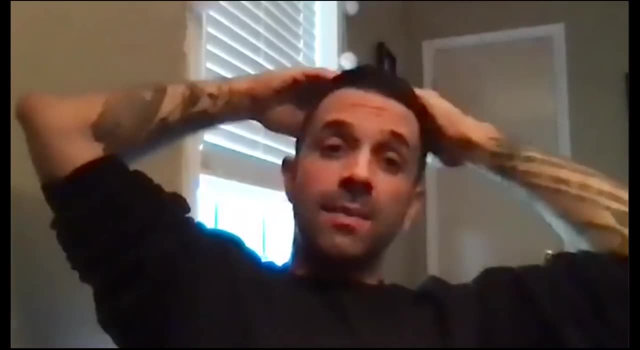 was just over at his house few days ago. he's got like trays of these. things are like bursting out of the. it's crazy, i mean he's really figured it out. he waters them from below so he like puts them in a tray, waters the tray so that they don't rot up top. he doesn't even give them humidity. but like when i've grown small spine this cacti. before i've kept them covered with like saran wrap to keep the humidity up, but then you run the risk of that first month or two it's a really fine line, Or are they going to dry out? Because before they've bulked up and turned into that battery that cacti are, and they've got enough carbs and moisture stored up. they're really sensitive. They can dry out easily, too, you know. So it's kind of like that fine line. ways to mitigate it are just, yeah, growing like. 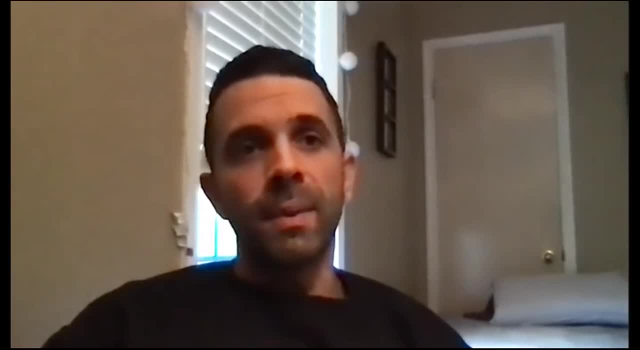 a humidity dome watering from beneath. So, like the capillary action of water draws the water up, You're not getting that tissue wet. But there was a soil mix, some dude told me, for astrophytum. forget what it was, but there. 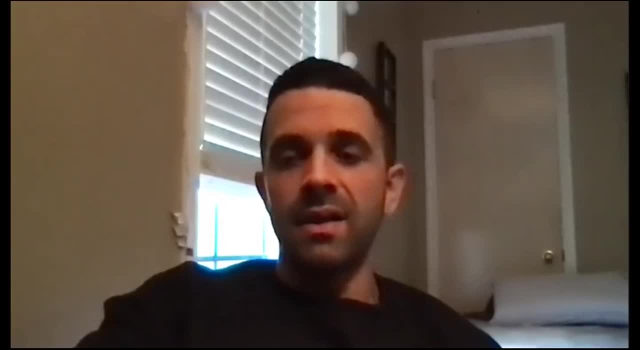 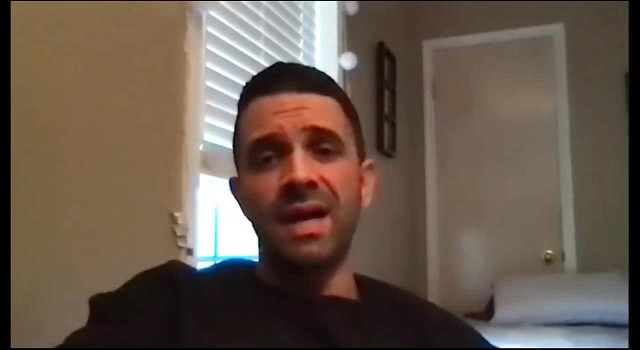 was like almost no organic material. It was like perlite or mineral base- Yeah, just mineral base, Like I forget what exactly he used. I mean, you can use a little bit of peat if you've got more heat, but if it's only like, 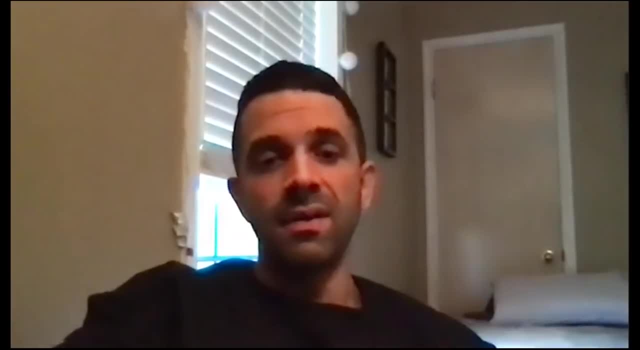 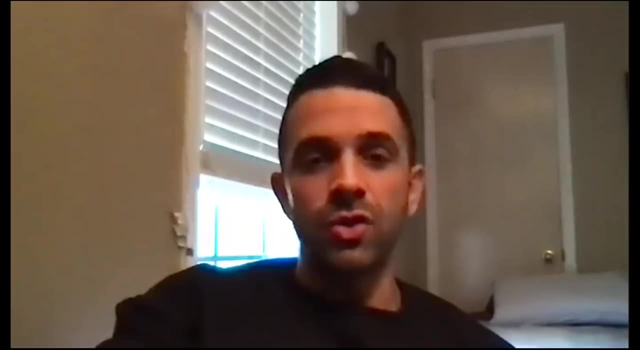 60 or 70 degrees in your growing environment. you want to stay away from the organic materials, But again everything changes Like when you're in a place where it's like 85 degrees and humid One. you're not going to need to cover those plants. 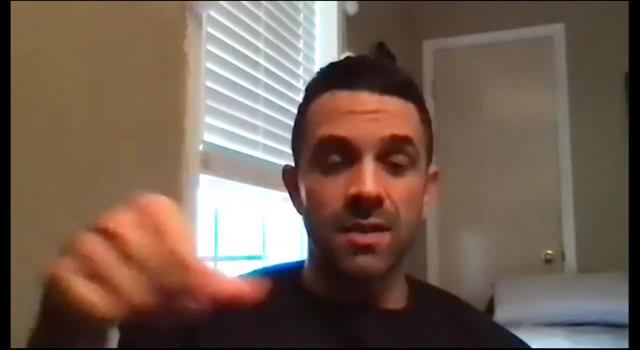 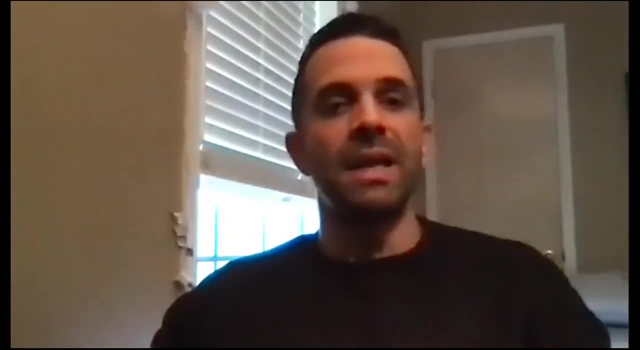 And two, you can use a little bit more peat because their metabolism is going so much faster than it would be. you know, plant. You have to think about the metabolism of the plant, how it's consuming, how it's photosynthesizing and then consuming its own energy, right? And plants that are from tropical and subtropical environments need warmer temperatures, because that's what their metabolism is adapting to And that's why, when you bring them to lower temperatures, they tend to rise, because they slow down, They're just. they're, in effect, living a sedentary lifestyle. They don't have the temperatures to metabolize and photosynthesize, And so they can't produce the compounds that fight off fungi as well as they might otherwise. So it's, you know, everything changes when temperatures change. But then again, if you get too hot, like above 90 degrees Fahrenheit, you know. 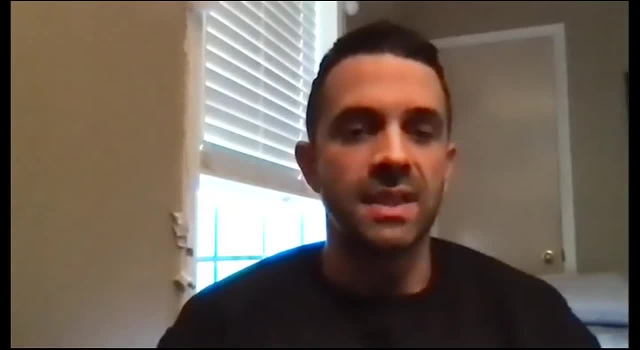 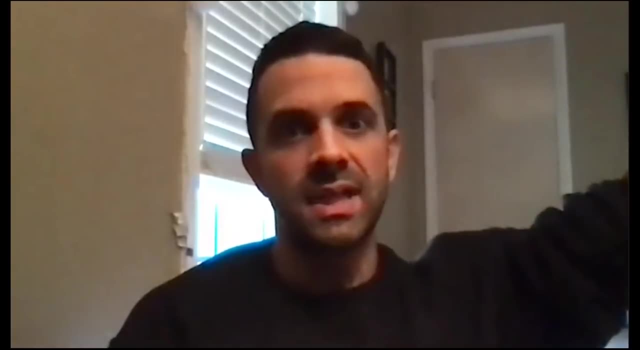 low phosphorus shuts down, It's not. it's not photosynthesizing, not actively photosynthesizing. Maybe it'll start photosynthesizing again later in the day, When temperatures cool off. maybe it won't photosynthesize for a few days, because it's 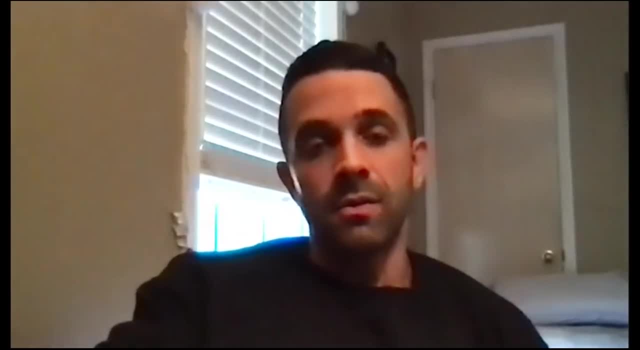 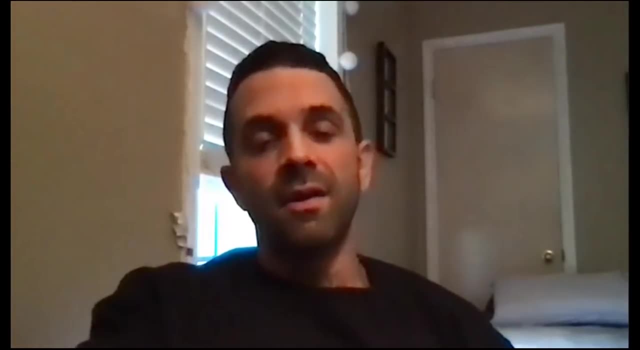 in a fucking heat wave. It just depends, you know. So if you want to read more about that- another great fucking book- I didn't put this Peter Raven's Biology of Plants, also available on LibGen- Don't start reading it from beginning to end. 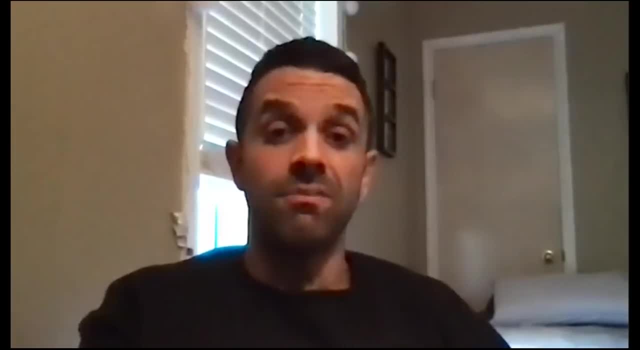 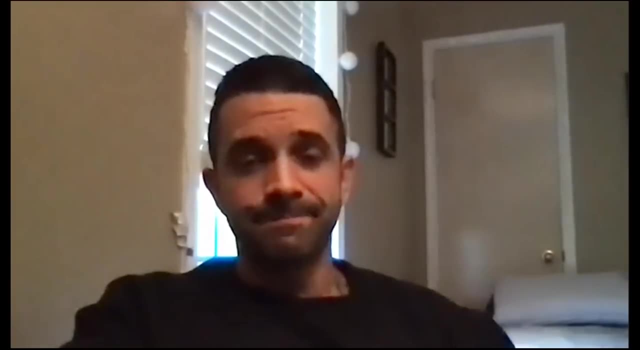 Just look through the table of contents and look up different chapters. There's some fucking great shit. It's like the plant physiology textbook. It's fucking awesome, you know, And you can pick it up anywhere and start reading, you know. So I live in like Cook Kane County border. 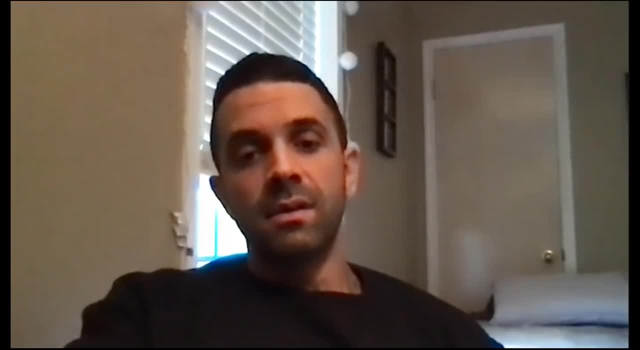 And because you're from the area, I was wondering what your favorite wild area is. Not like a botanical garden, but, Oh, Wolf Road. I mean there's a Wolf Road, Prairie, Braidwood Dunes- That's further south. 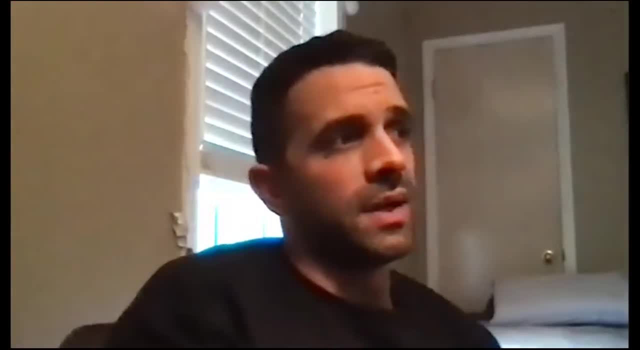 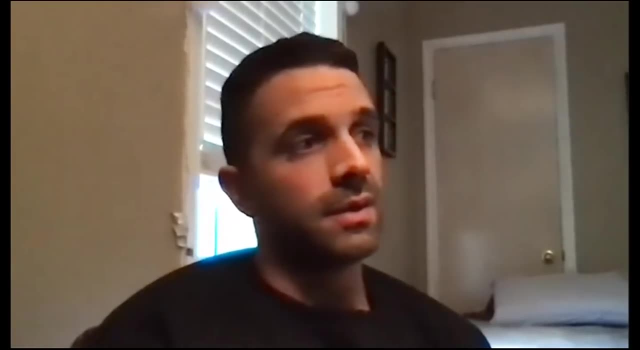 Well, yeah, that's closer south to you. You want to get to in the summer. if it hasn't rained in a while and the water is low enough, you could wade across the Kankakee River. go to langham island, check out that weird iliamna, which is super easy to grow from seed. super fucking easy. prairie, moon nursery sells it, but you know, each plant produces tons of seed. you could go over and take a couple. you know what i mean. you know i mean, take a couple fruits, give it the hot water treatment. man, i don't even need to, but i, i would wouldn't hurt. you know, don't get it. 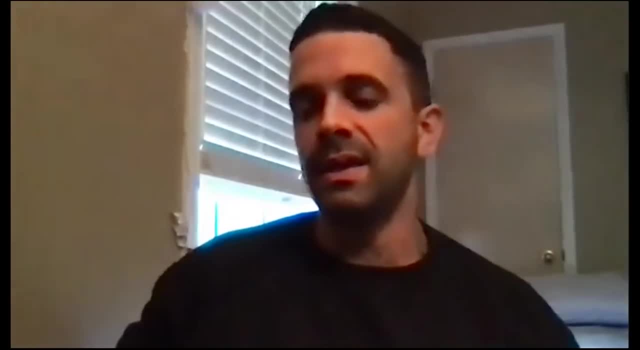 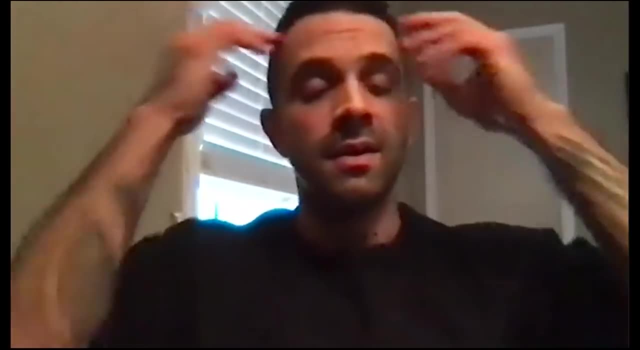 boiling but get it hot- you know, too hot to touch uh and then just germinate. i've germinated a ton of those uh plants. they come up like weeds, you know, if you give them what they need, and then they need full sun. um langham island's good braid with dunes, there's a bunch of sand prairies, i mean. 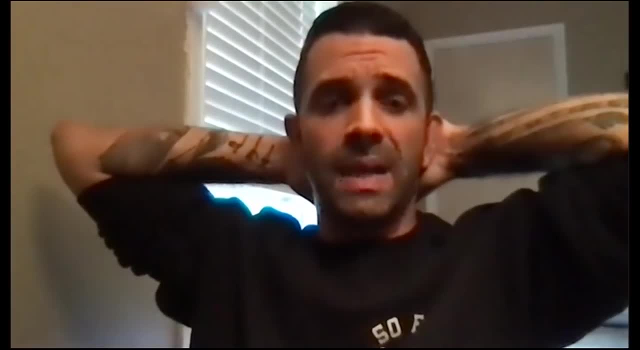 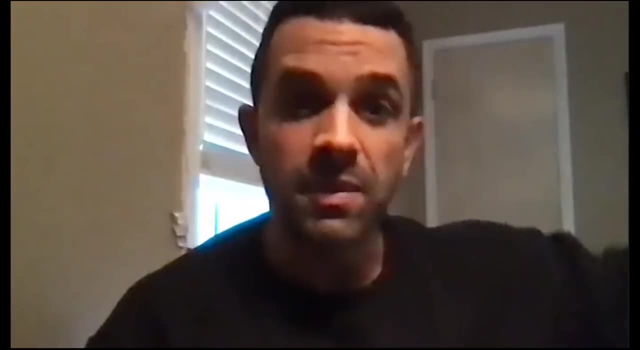 go to google terrain and uh, or google maps and just look at any green area and then zoom in on it and see if it's a nature preserve or a fucking golf course. if it's a golf course, go dump some garbage over there. just kidding, just kidding, and uh and uh, if it's the nature preserve, go check it. out and do like a species inventory. you'll see shit you never saw before. there's some really cool prairies down in markham too- nice blue collar suburb of markham. what was the name of that plant you mentioned, sorry, uh, iliamna. i l i a m n a remota. it's another weird uh narrow endemic only known. 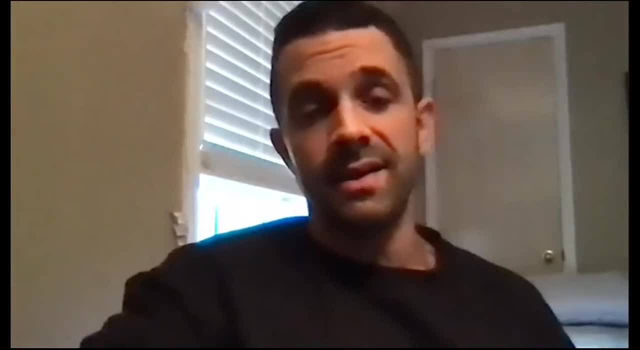 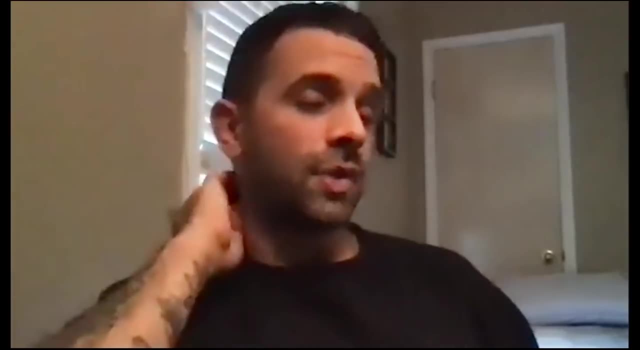 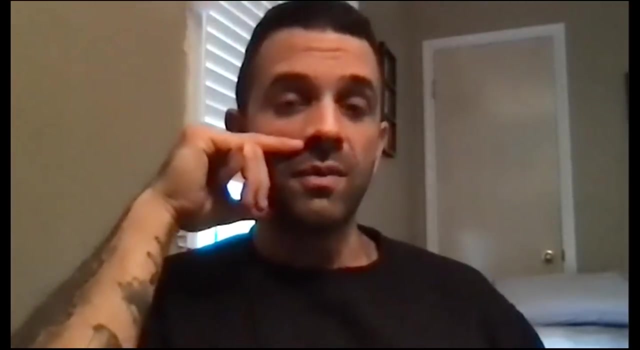 from that one island and supposedly on the side of some train tracks in indiana, and that's it. nowhere else in the world really. yes, remember the cotton family. uh, it's getting crowded. it was getting crowded out on that island by, uh, japanese honeysuckle invasives and quite a few invasives, and then a bunch of people started. 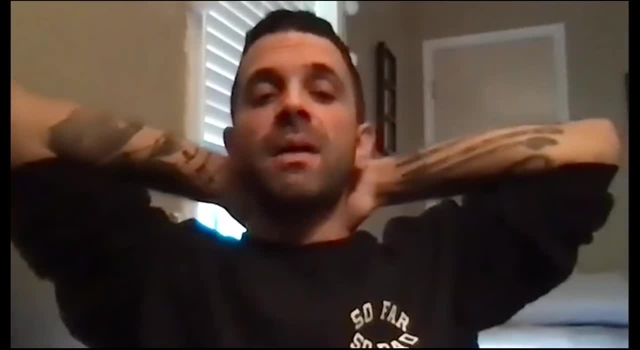 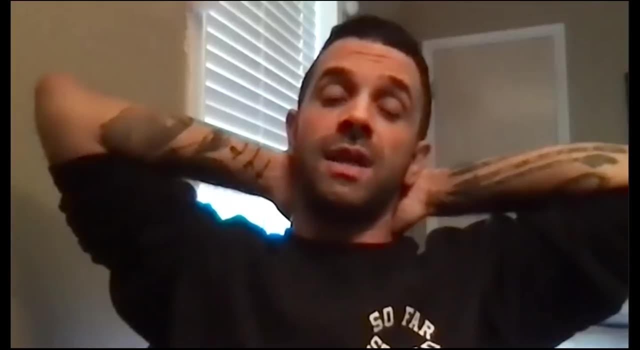 going over there like 15, 20 years ago and burning- they don't prescribe burns- and weeding out the honeysuckle and all the other invasives, and now they've. they've really done a fucking great job. i mean there's all this stuff there is thriving now, but that's probably a plant. i mean it's so. 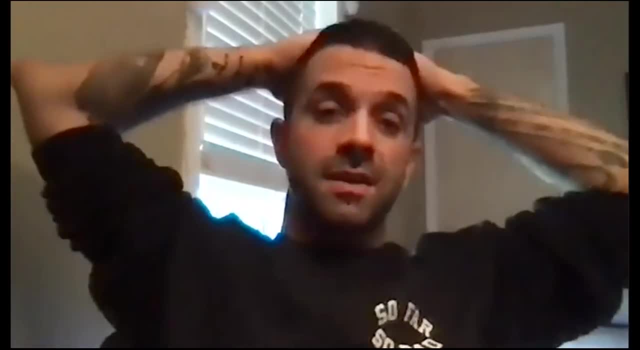 easy to grow. that's a plant that should be in every fucking midwest garden. i don't know why it's not like. i don't know why i never heard of it. you know, i don't know why it's not like. i don't know why i never heard of it. i don't know why i. until you know, i don't know why i never saw it at chicago botanic garden, which maybe because it's kind of lame, i don't know why ever, you know, i think morton arboretum has it, but uh, you know, it should be a much more common plant than it is. it's so fucking easy to grow. 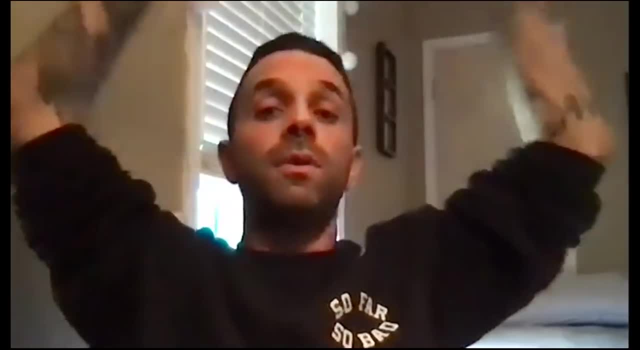 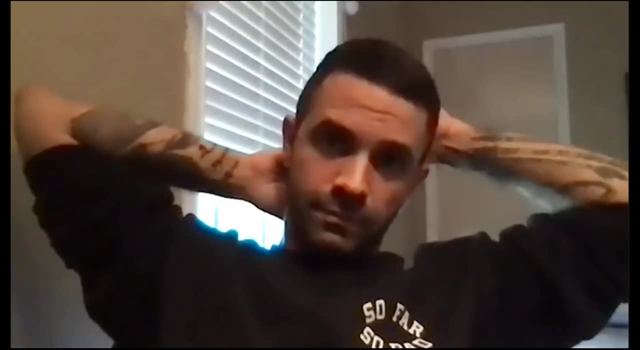 it doesn't require any special type of soil, it just needs full sun, just full sun, that's it. well, there's a couple of boggy areas and stuff near me that nobody goes to, so i'll uh see about helping it along. well, it doesn't like bogs, it likes fast draining soil. 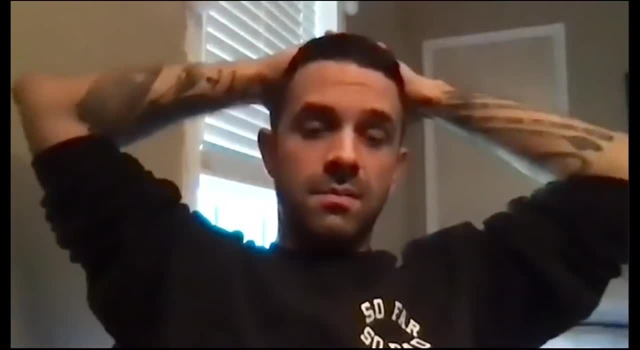 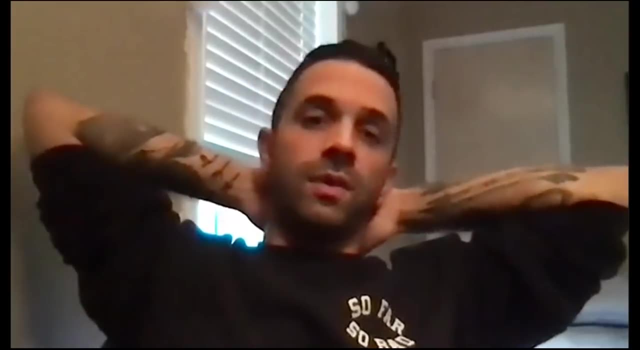 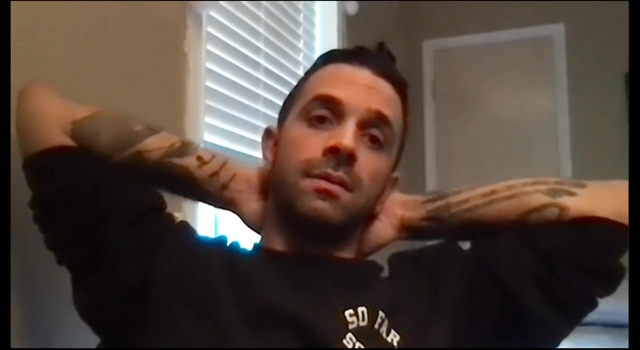 but uh, but yeah, i mean, are you with that? okay? yeah, i'll figure it out. yeah, you can email me after too if you need. you know any beats or anything. so anybody else got any more questions? all right, you can do another video. i don't know. i mean i'm doing this because, um, 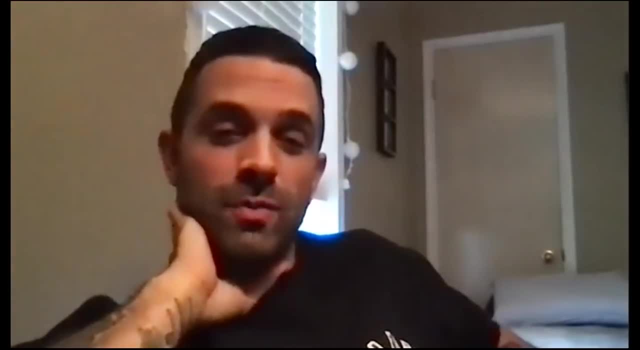 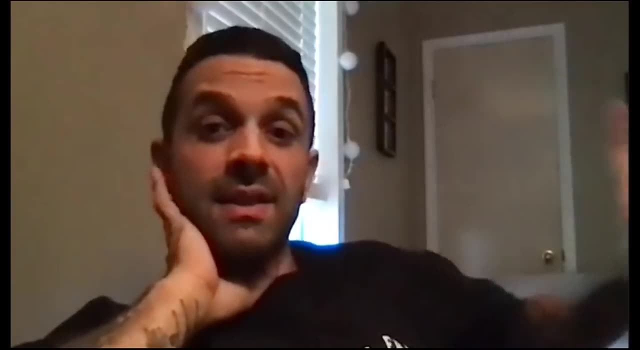 someone hooked me up with a, with like a pro zoom account, and they're leaving, uh, to go back to the dominican republic tomorrow. so this is you know, and she was cool enough. just be like, yeah, i'll help you out and she helped me. you know, do this, do i'll put this stuff together and maybe 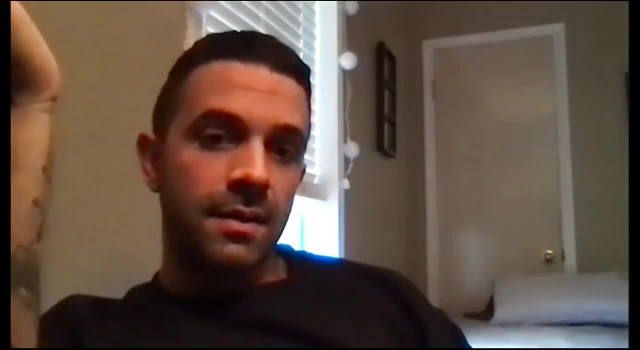 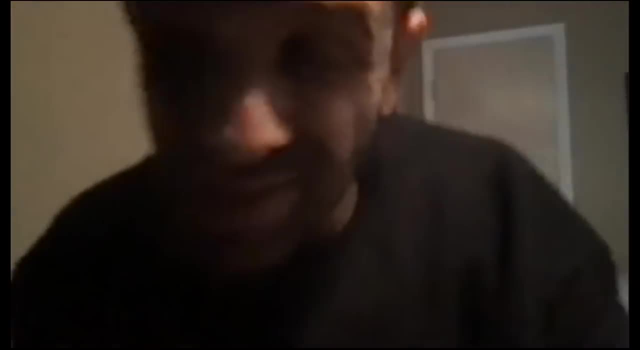 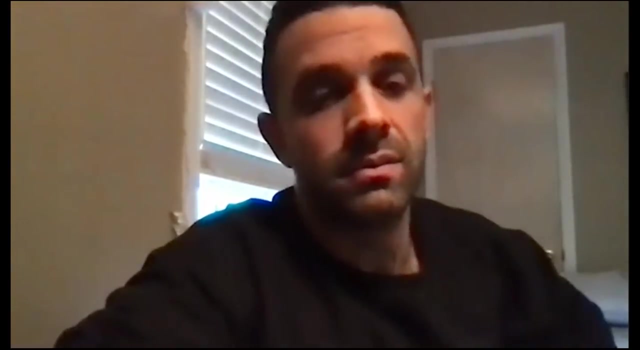 at some point i will, but if i do, it'd be, uh, it'd be limited to like a hundred, uh, a hundred people. i think the pro zoom account is like 150 bucks. when i looked into it it's like it's a lot of money. uh, you can get it for like 15 bucks a month, really, and you can get it to. they got like a 300. 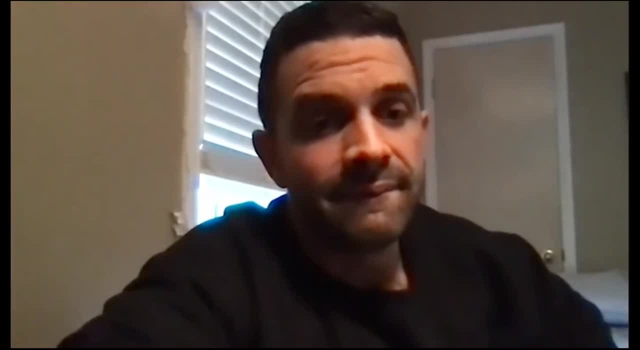 person limit or what. uh, i'm not sure, but when i went pro it was like 15 bucks, maybe more, yeah, yeah, that's what i would need to pay attention to is the the limit of the. you know how many people can attend. i think one and a half of us has to pay. 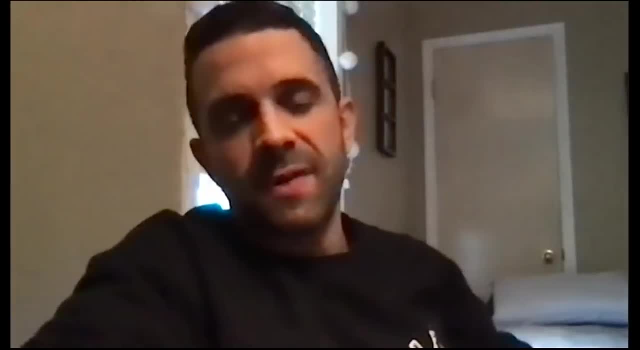 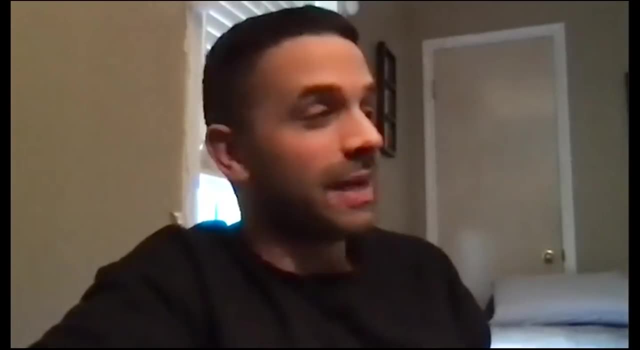 i'd only be limited like a hundred people otherwise, but that's fine. i mean like we're like 75 right now. you know, like half the people dipped out. i don't. i'm surprised there's this many people left. three hours is a long fucking time of time. anytime i do these presentations. 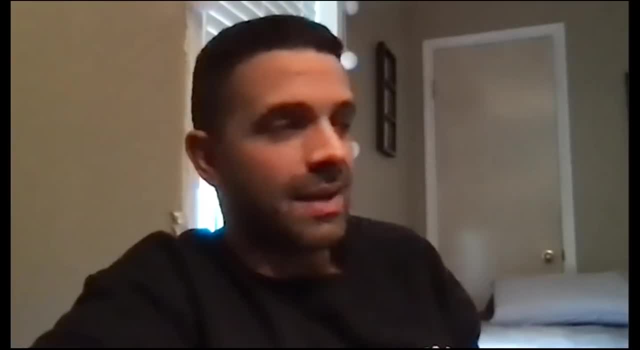 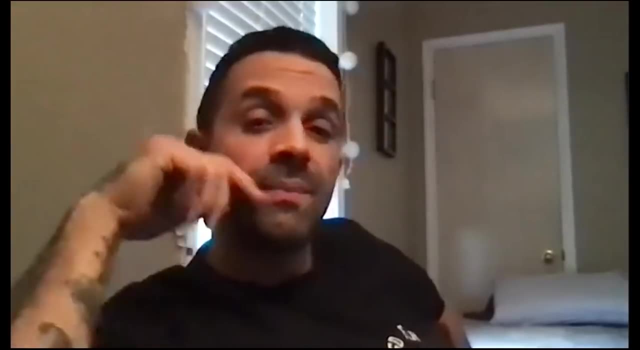 i'm always blown away how fucking long i can go before i mean i'm not like i gotta pee. but aside from that, i said i enjoy talking about this so much and, yeah, i like getting people excited about it, and you know whatever. um, any more questions, or is that? 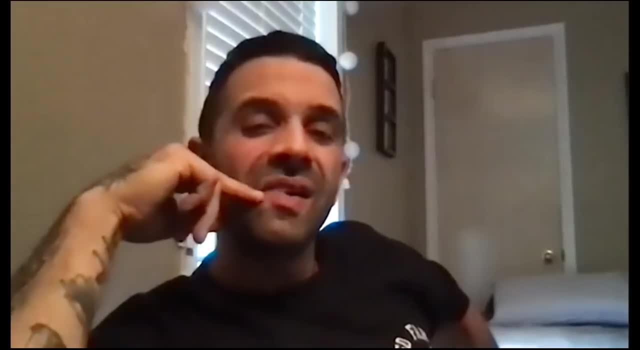 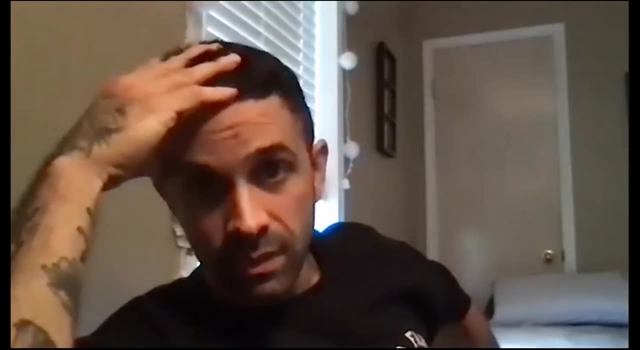 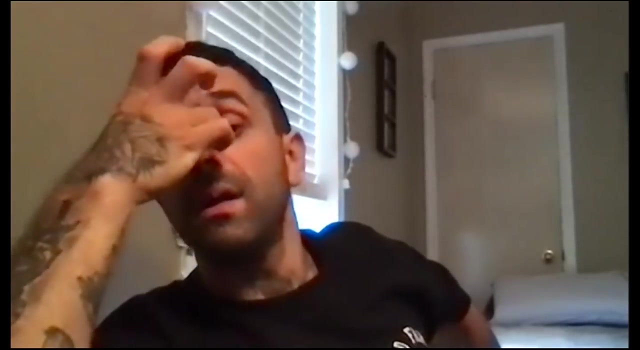 it. yeah, uh, but remember that support you found in. oh shit, go ahead, we, there'll be time for uh, the support that you found at the utah arizona border. i was wondering if you like any areas where you could find it, because i'm like in the res up here and it's just not that far. 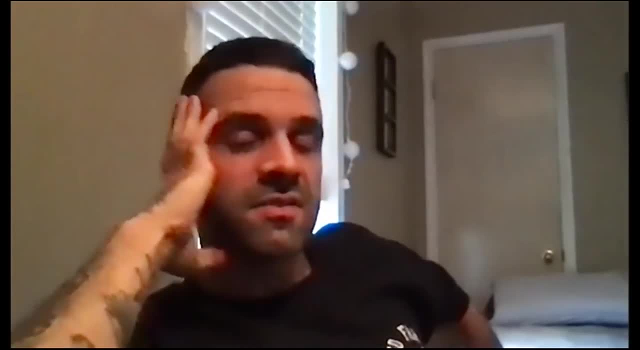 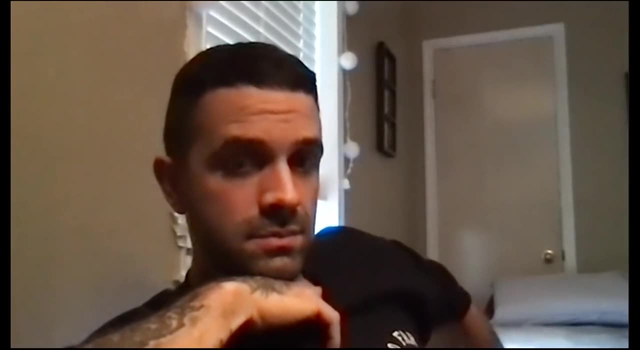 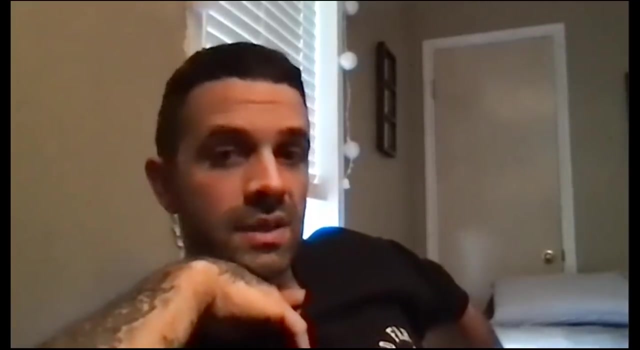 oh, just drive, just drive down there. i mean it's, it's from like a main it's- you wouldn't see it now because it's winter- but another, like warmings and like private areas, and uh no, i think it's, it's, it only grows in those dunes it might. you know what? i don't know, i, i. 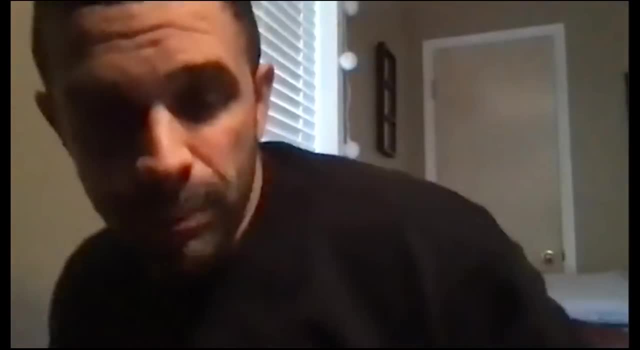 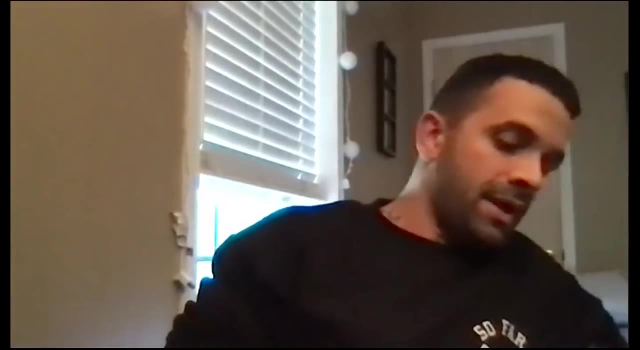 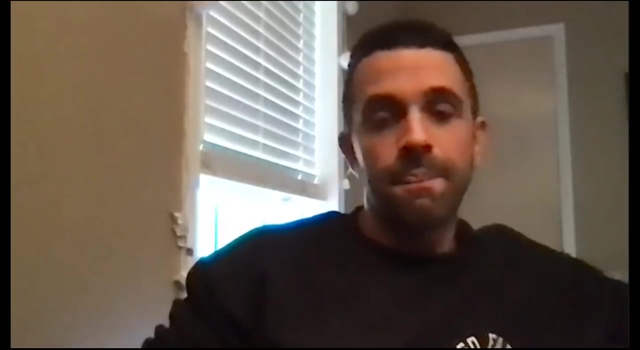 would have to look again. but again, look up on inat. it's not a rare plant. it'll be listed. yeah, here's the explore feature on inat. see where else it's been observed. uh, and barring that. oh fuck, this modem is about to fall. hopefully i don't disconnect myself again. uh, barring that, um. 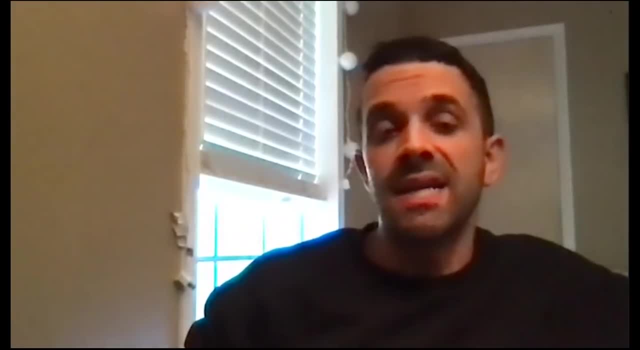 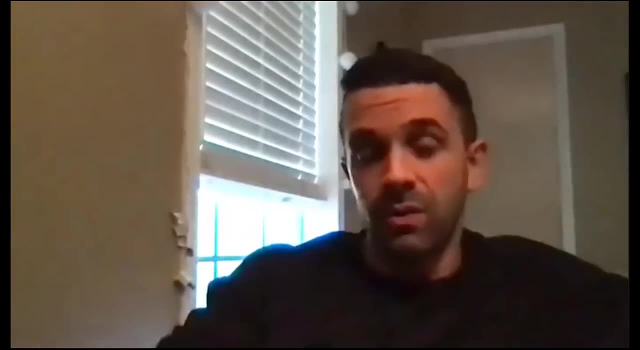 it'll be. you know, you could check uh sign at s-e-i-n-e-t. it's like the botanical research institution, um, you know, so it would be there too, but i i think it might be. it might occur in a couple other places, it's not. it's not as rare as that milkweed, but definitely that's. 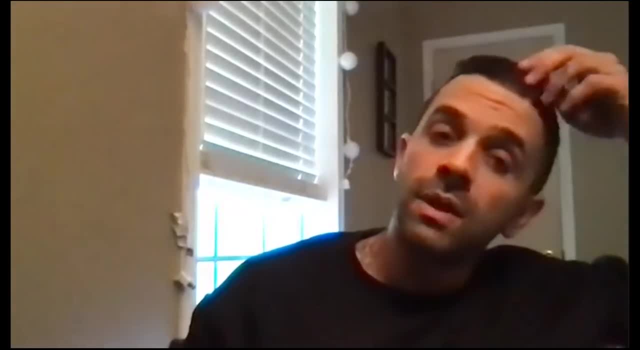 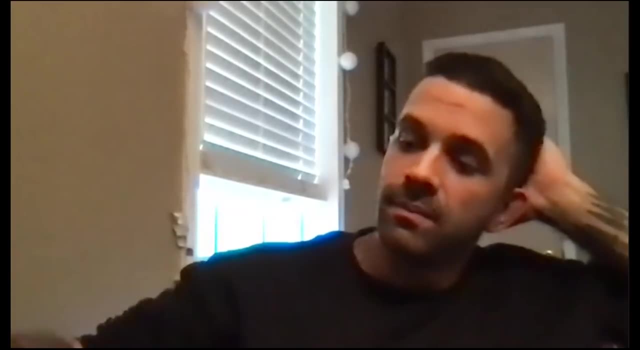 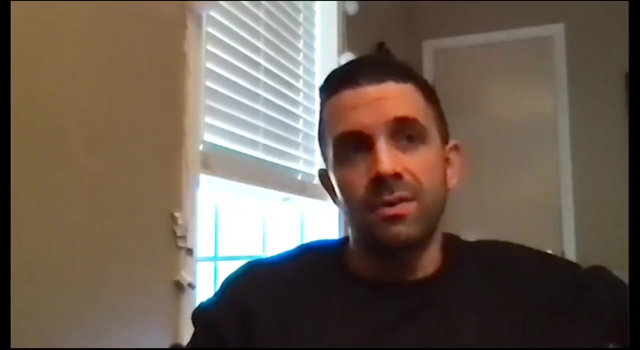 easy. so you should go to that. only grow in the sand. there's only, i think it only grows in sand. yeah, i'd be surprised if it grew anywhere else. but um, but yeah i would. you should go there anyway, it's cool and it's. you know, the fucking atv guys you know are well, they're restricted to a certain. 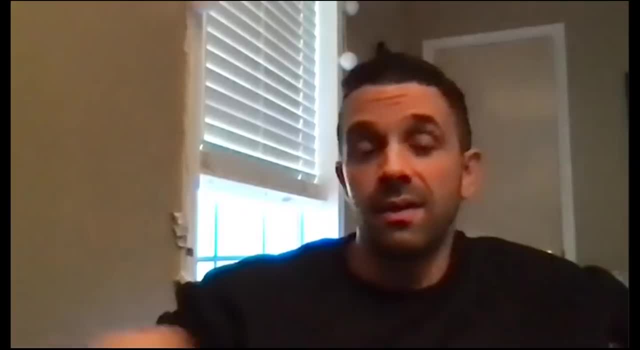 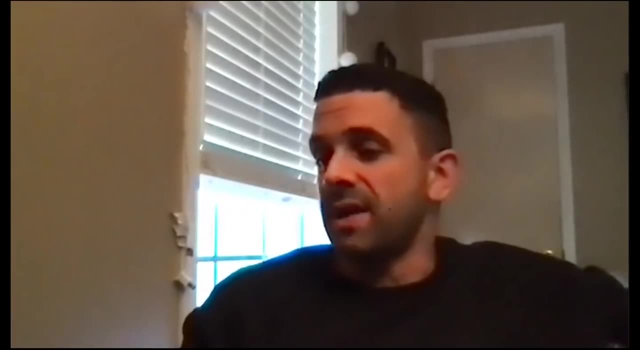 portion of it. they can't, they're not supposed to drive where the milkweed, all the other rare plants are, what they fucking do. you know freedom, uh. but yeah, check to check it out. it's right near one of the main parking areas and, uh, there's a ton of cool shit there. i mean, yeah, that's the spot to be in june. 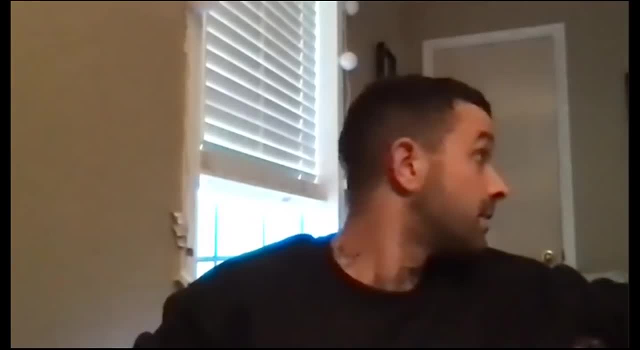 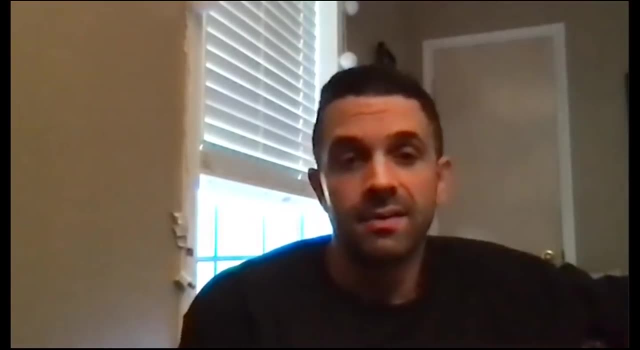 you know, if you want the more remote areas, you go to, like, the northeast end of that, um, you go to the northeast end of that uh little national park or mining, whatever the fuck. it is state park. so anybody else who else had a question? i've got one. so i was uh, as i've watched the videos, i've. 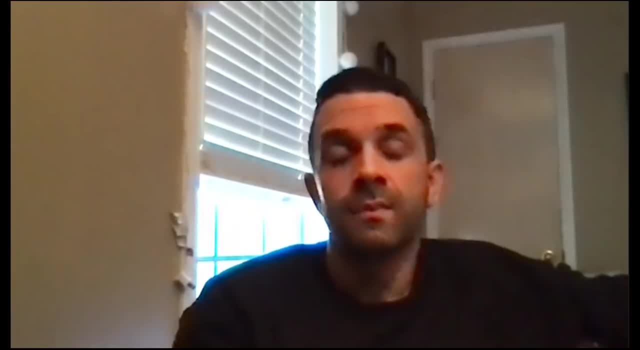 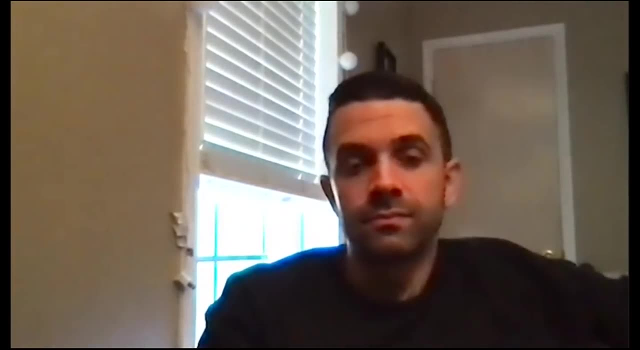 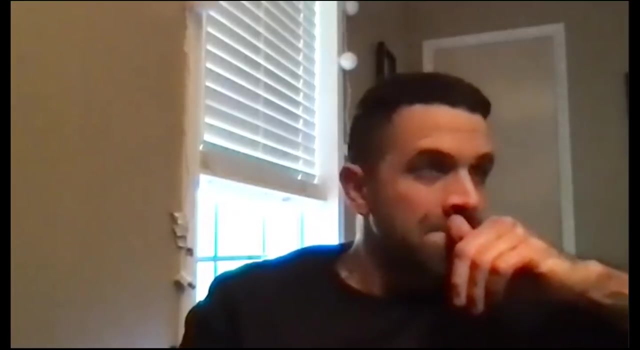 i've kind of been wondering if i mean, now that we've brought up the i naturalist sort of app and website, is this how you're mostly finding the kind of interesting locations with these rare plants or just kind of good places in general to find uh plants in your area? nah well sometimes, or if you're just like getting 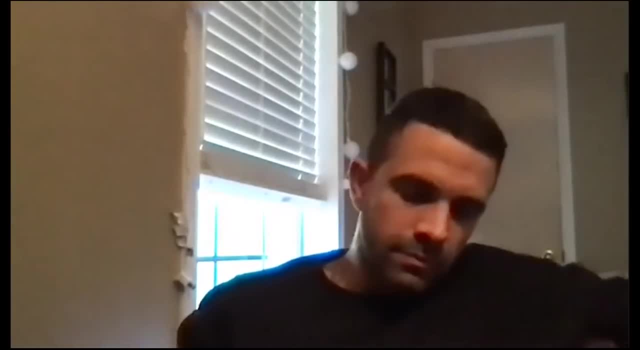 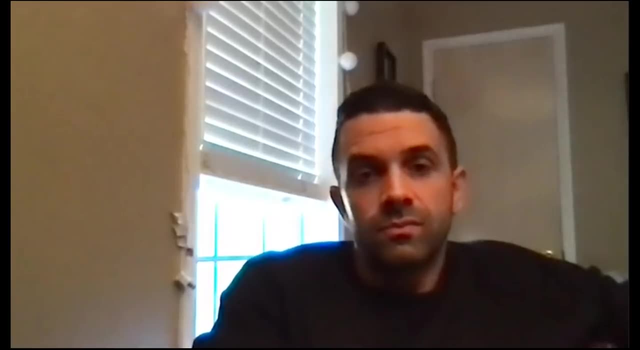 word of mouth, or if you're just kind of going out in random places and just hoping you run across something because you know, like you showed the, that fertile area. i mean that's a lot of uh a genus that i'm kind of interested in too, yeah, and i'm around some serpentine stuff, uh, in. 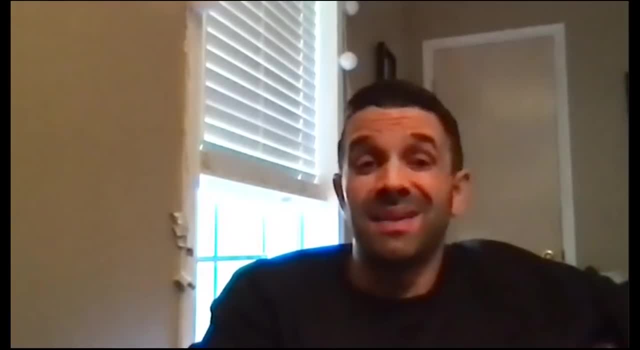 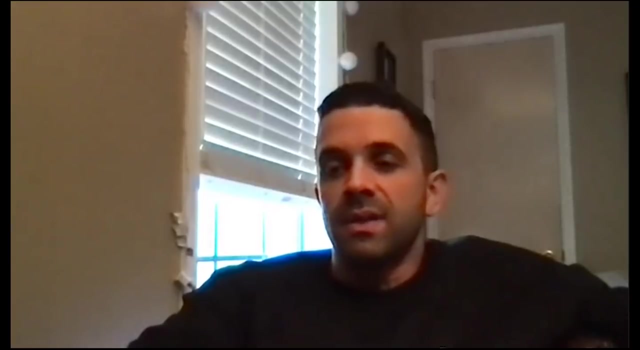 the east bay. how do you find rare spots? i mean, that's kind of a you know, that's the thing. if it's rare enough, it's obscure. you got to find word of mouth, uh, that population. one of those populations was actually found by a guy named roger rash, uh, who i'm friends with. um, i don't. 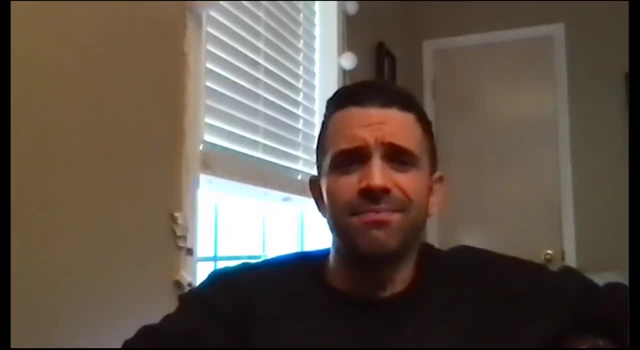 know if he's the biggest fan of the videos. he's kind of, uh, you know, he's kind of a, a square great guy, but he's kind of like the profanity offends him and she said whatever. but he found that, uh, on his own in like the 80s, you know, and he just there, no gps, he just. 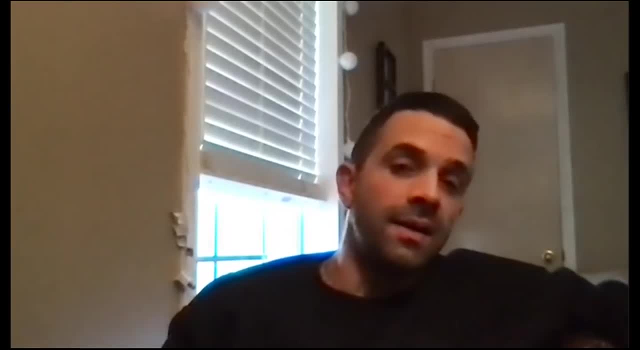 had really good location info and then a friend of mine uh went back based on a description of the area and searched and searched and finally found it and that's actually really cool. i mean, i showed you two different populations, that one of them is literally like 30 feet across. it's like 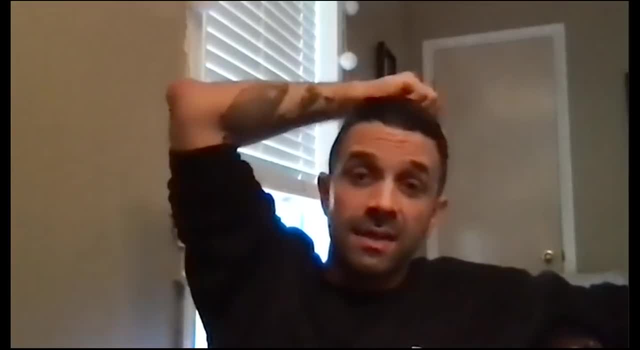 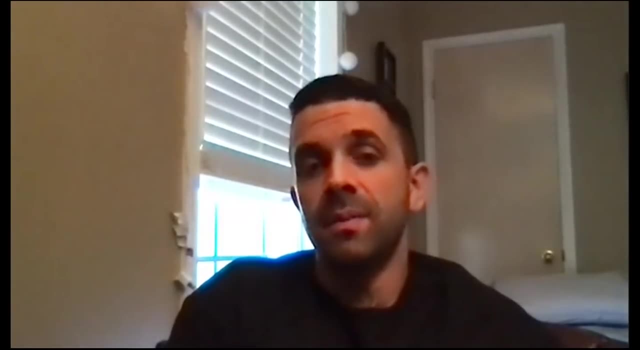 30 feet in diameter. that's it. nowhere else, for whatever weird reason, that's the only area that it grows um. but uh, the other population is a little bit more spread out. but but my friend found that and then told me about it. i just found roger race's, you know felcona population like oh i gotta. 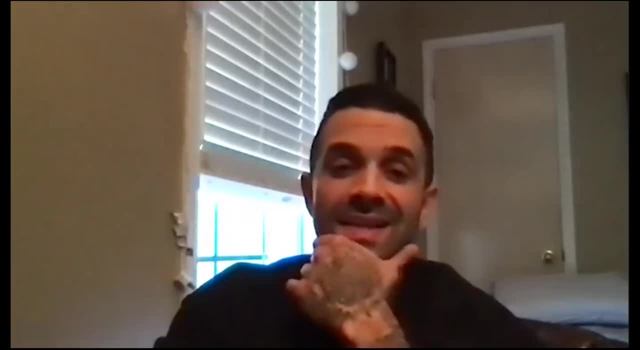 go check it out. and that was the spot that's trespassing, that's you know, the rednecks there, that's you know. i'm sure he would hate the idea of anyone coming on his land to look at a plant. but he's got like signs up and shit. now he- i think he knew we were going there and then next day he put: 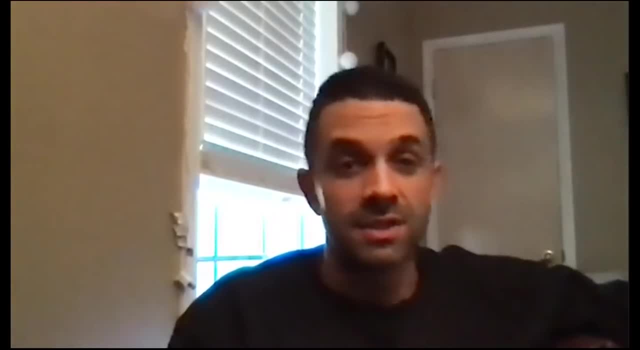 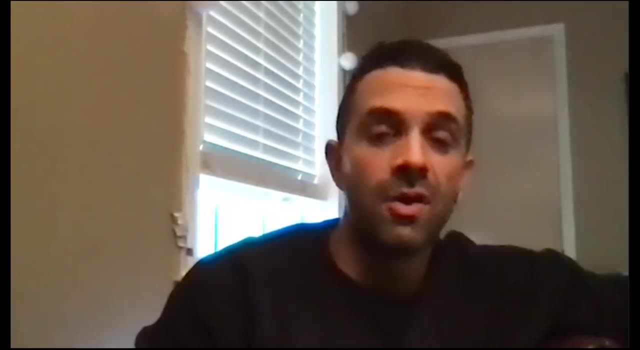 up signs and he put up a he like has some dogs that he just keeps outside. it's fucking brutal. he doesn't live there, but he owns the property. he just keeps these dogs, like now. they're like permanent residents. all that shit burned though, so i don't know what, uh, i don't know what. the 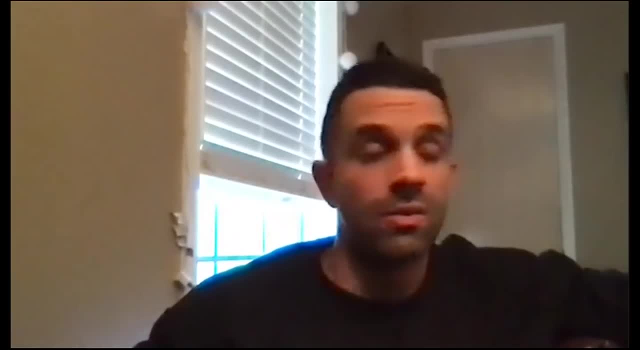 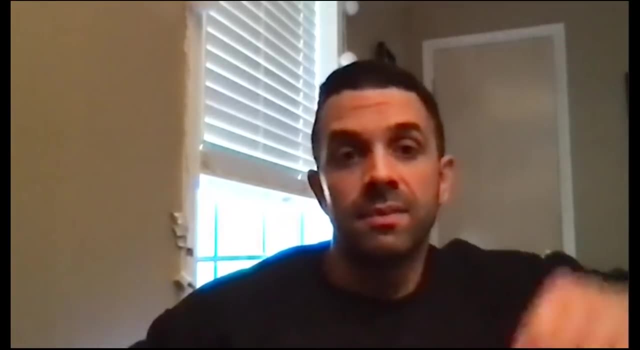 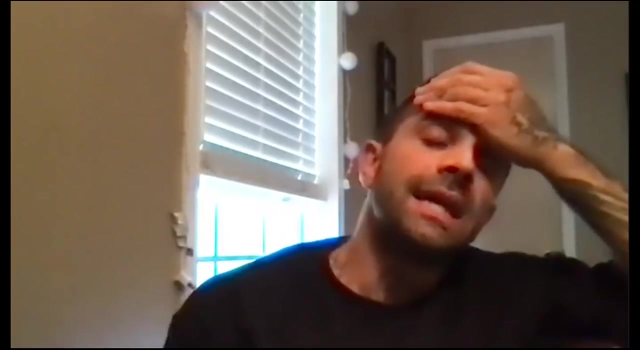 status of it is. i mean, it just burned, you know, seven months ago the whole fucking area went up. wouldn't affect the fertile area, but other locations. you know some. they're like that asclepias i just found on my own. i was, i was looking at the, at a, at the habitat, looked right. 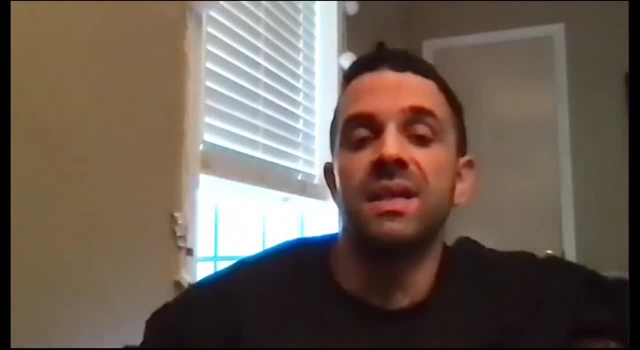 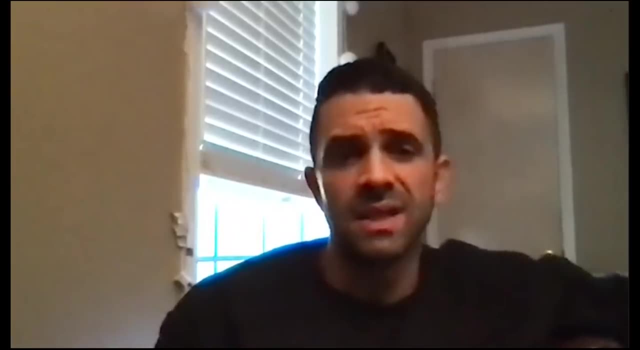 and i was like, well, this is too, there's too much vegetation around, but over there it's like bare sand. so i went and i was like, oh shit, there it is um other spots. yeah, friends have found. like my friend matt, sheriff woody goes out, he'll hike up in the middle of. he's like a. 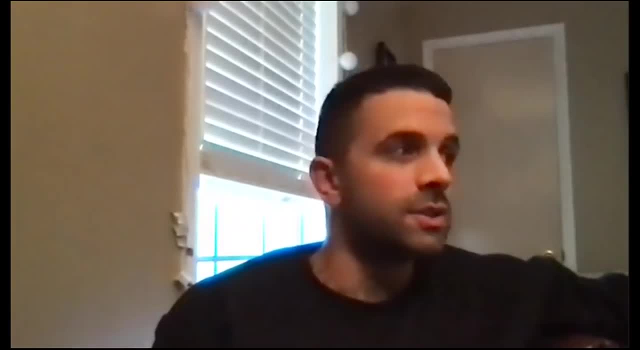 he loves hiking. he's like the surfer dude version of a hiker, so he'll just like hiking. 20 miles in a day is nothing to him like out and back so, and he'll find all kinds of shit. he might have found two new species of monkey flowers. um yeah, word of mouth you just. 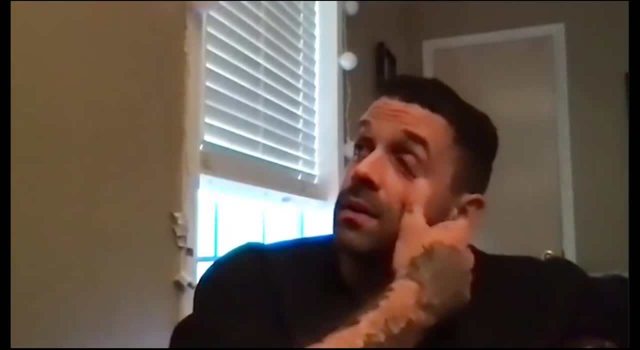 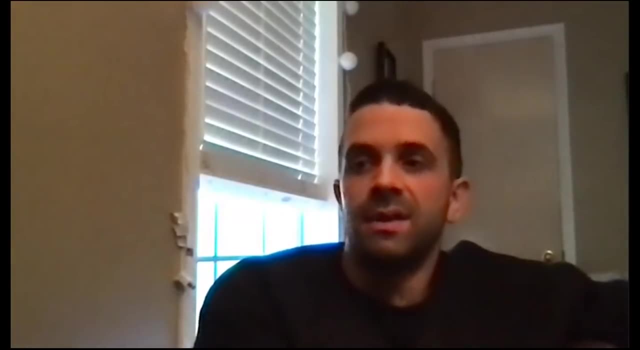 you come up on it, you know you're obsessed with something and you you are really into it. you figure out where to find it. so there's multiple venues, but it's mostly yeah for like the rare shit because it's obscured word of mouth- older barium vouchers, um, etc. so or just know what the 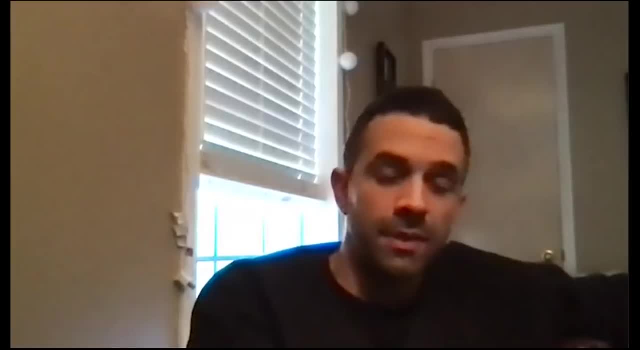 habitat looks like, you know, which sometimes you can even figure out from looking at a satellite map, like the burned areas? are you just like parking on the side of the road and like walking in because i want to go up there but i don't know where i can? like park, uh, you just find spots to. 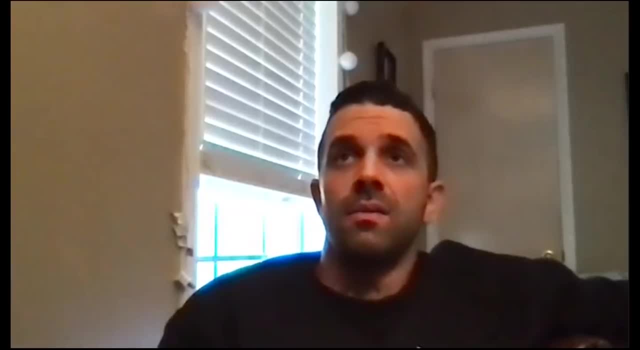 park. uh, you know places you don't think cops will with your car, the burn, i mean, like the tonneau ridge, that was. that's like a you know 14, 15 mile hike in and out. so, yeah, eight or nine, but and we weren't supposed to be there either, that was, you know, people were whining about. 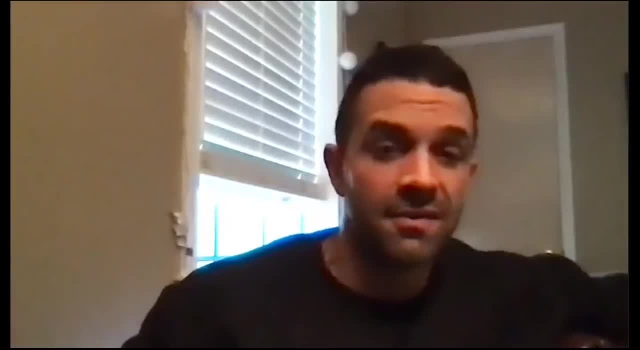 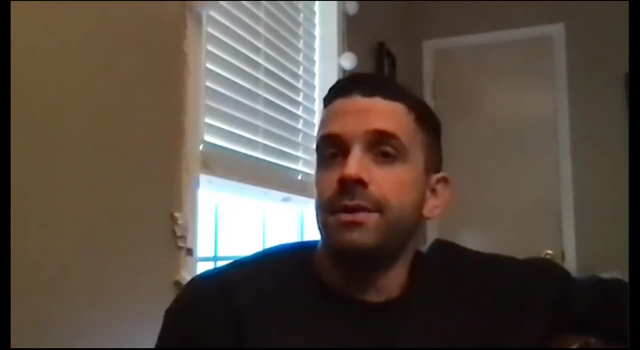 that on the it's clouds. well, yeah, it's close because of liability i'm not gonna sue of a tree falls on me, you know, off um, but uh, yeah, i mean you just you park where hours preferably. you don't want to have to hike that bar, but if you're like in a Honda fit or something, you're. 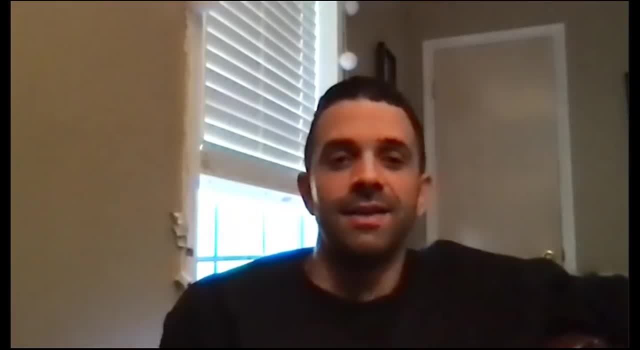 kind of up creek. you're gonna have to get used to hiking, you know it. just, it just depends, you know. but again, that's the point of masturbating. look at the map and you know, see what's, uh, what's available, what, what, the, what the area is like. so, okay, cool, i'm just gonna drive up in the big basin. 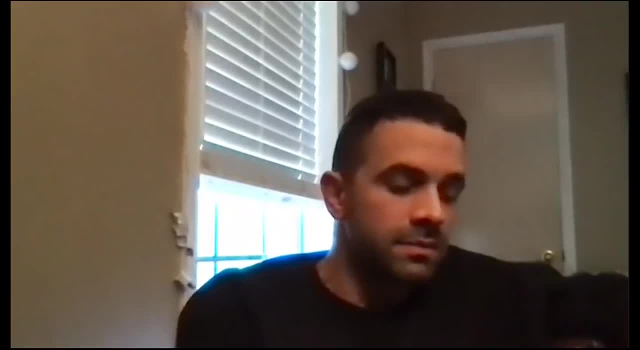 try to find somewhere to park. there's just i'm like scared of people with guns. i don't want to get shot. oh, don't be. i mean, i don't think in most cases, like a friend of mine who's a herper is always like: yeah, so and he does it in texas and he'll be trespassing and they'll be like it's. 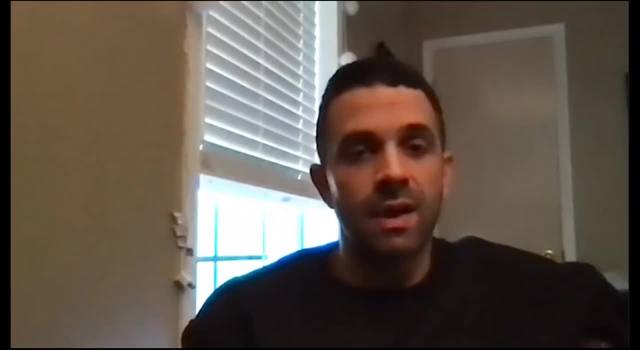 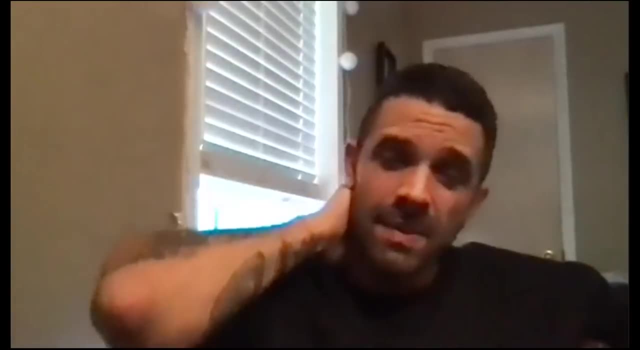 amazing what telling someone that you're looking for snakes- how quickly it changes them. and same thing with plants. you know, the only thing i'm worried about is, like a lot of you know, things are so polarized now people think you're looking for plants. they're that they're going to be more. 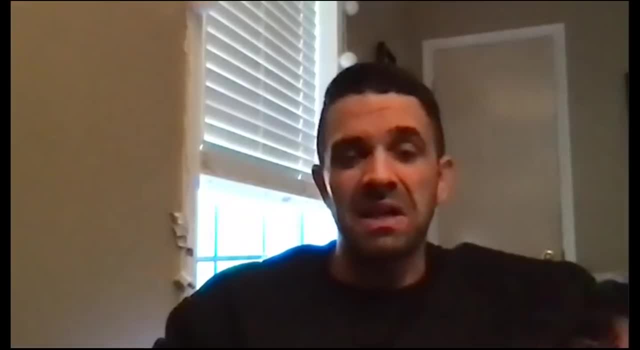 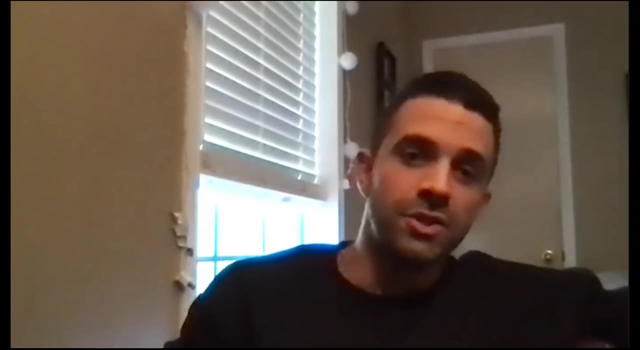 not in california but out here, so much they're going to be like: oh, you're playing, you're a hippie or antifa or what you know. it's just more of a political association with plants. it's stupid, but that's the nature of this. you know whole situation we're in right now. 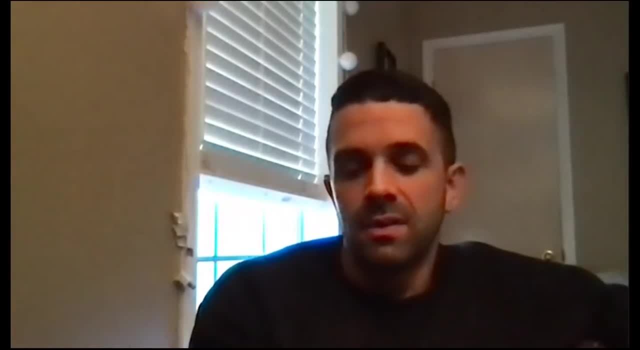 so maybe say snakes, but just tell them whatever you know. tell me you're looking for whatever. if they do catch you in so many cases they don't you know. i mean you're not doing anything wrong, really, like you're not being unethical, like proper private priorities are not ethics, they just people made up. you're not doing anything wrong. and if 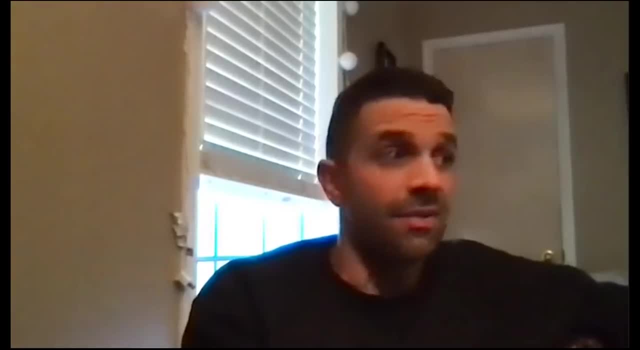 you're not doing anything wrong. you're not going to get into it with that attitude. it's whatever. you know, i got thrown out of some track i was running in less i like to run every day- had to have a fence to get in there because it's everything's gate. kept around this area. 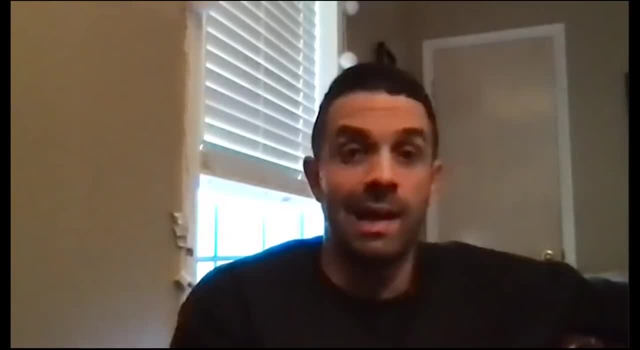 it's depressing. security rolled up and i just was like, yeah, what's up? i just talked to him. i was like, yeah, i came in here. how are you gonna have the fence? you know, i didn't think i got in. everything's locked, i'm just running, you know. and he was like, okay, we'll just get out of here. and i was like 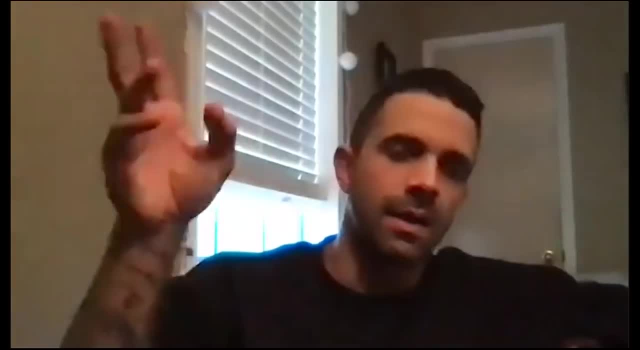 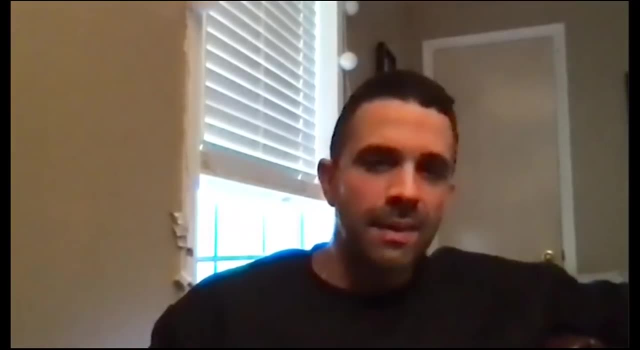 yeah, all right, i'm not doing anything wrong. i mean, maybe it's a lot and he was like, well, we can call all right, the cops show up. i mean, what were they gonna do if they take me to jail for being in a track running? i mean, i was in running shorts, i'd let my ass off and i'd go. 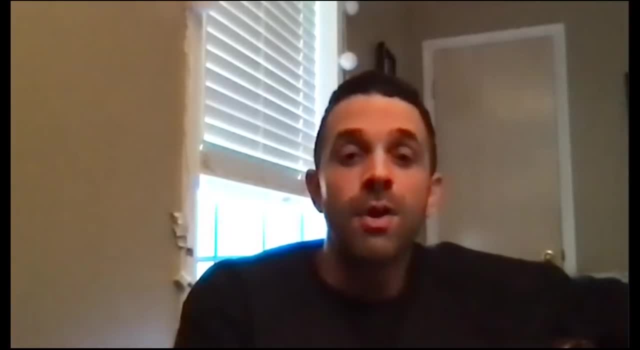 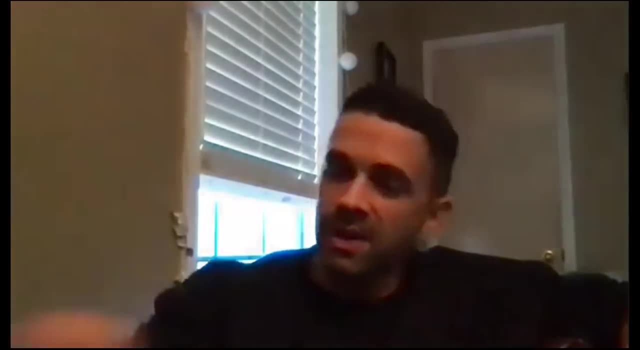 to jail. i don't give a. i've been there before. it's you're not gonna. you're not. the point is you're not gonna go to prison for it. it's maybe a small citation or something which is a pain in the ass, but but don't let the threat of you know legality prevent you from going to cool spots. so 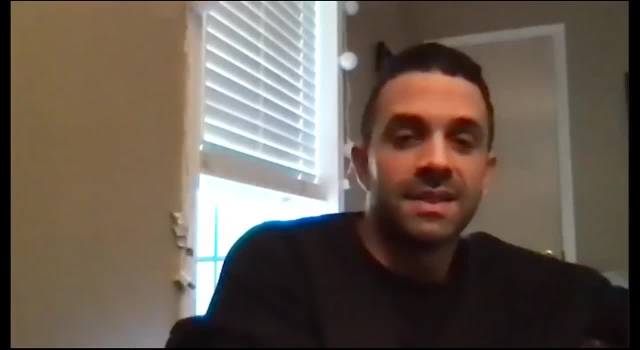 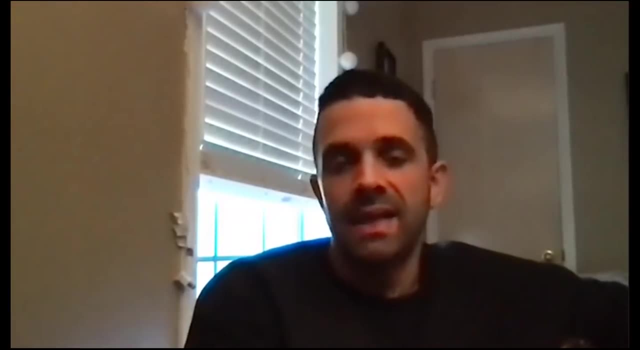 yeah, i'm like it's different though, but you know that's a different thing, and in california they they have to have signs of there's no trespassing signs, they can't even press charges and they're gonna be unlikely to shoot you unless they think you're stealing, you know. so there's just. 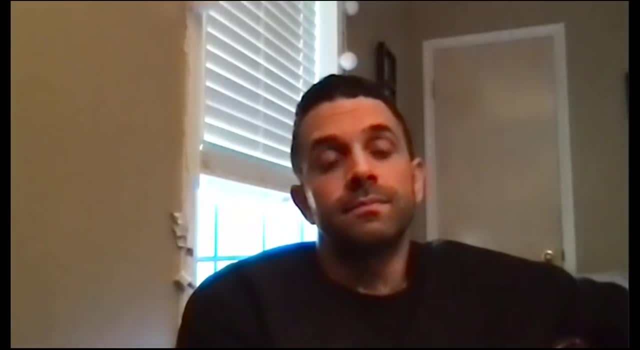 a lot of people that like they're very touchy because like everything burned down and i don't know if it's like people's private property, like i'll trespass, i don't care, but just yeah, there's a lot of people that are really like on edge right now. yeah, i mean try to avoid. 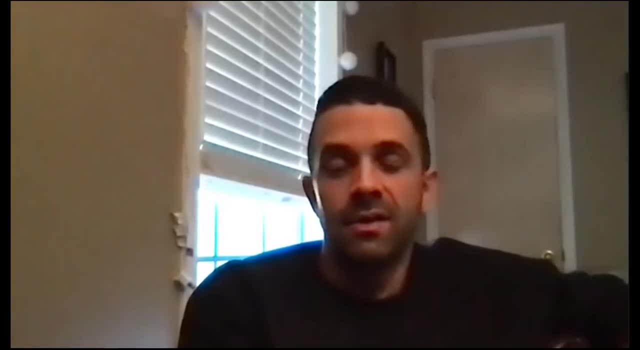 where there looks like there was a structure. you know, i don't okay, yeah, big basin, i haven't been there in a while, but if it's just a lot of the times things are shut down, especially in eric fire areas, because of the danger, there's nothing to be careful about too, because trees 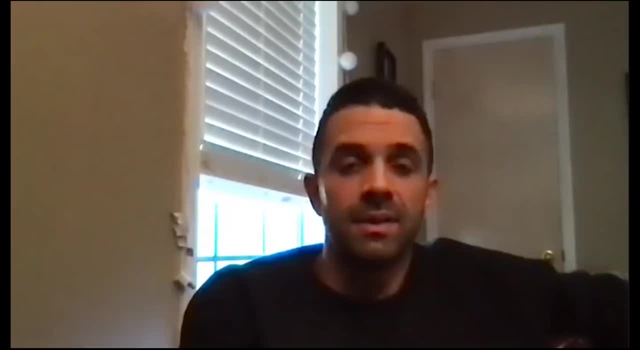 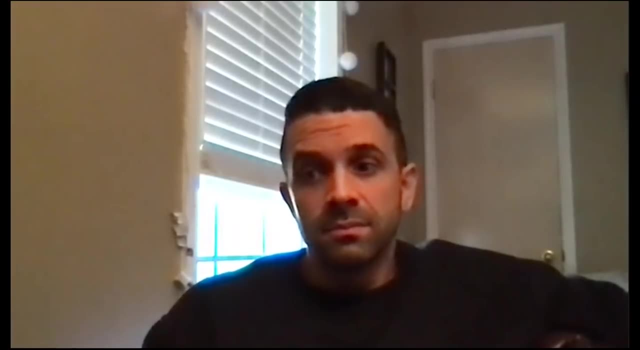 can fall on you, but they have to put those there because of liability issues. so i always encourage trespassing. what do you do about putting that stuff on? i know or whatever i have to. i obscure almost everything now, unless i want some somebody to find it, because 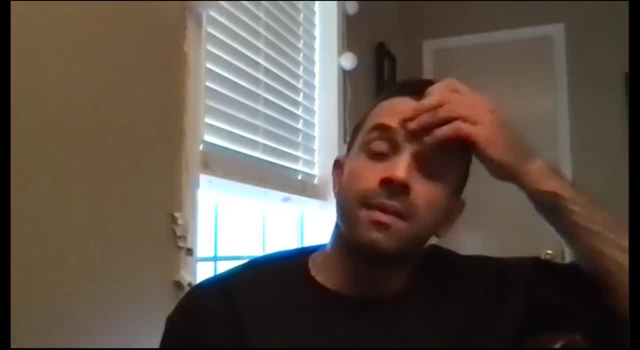 i think there's a lot of people, just because of the channel or whatever, that lurked that i. my naturalist is that i'm not going to put it on my page and so i don't want to blow up a lot of my spots, so i 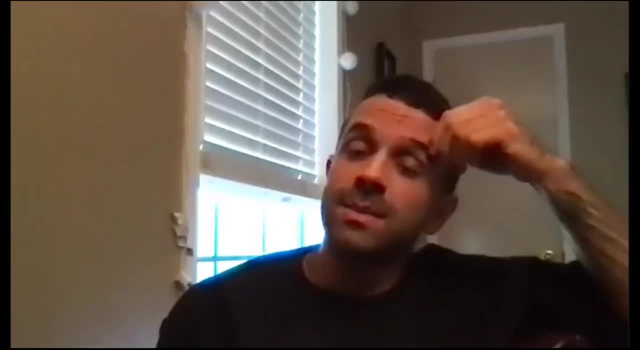 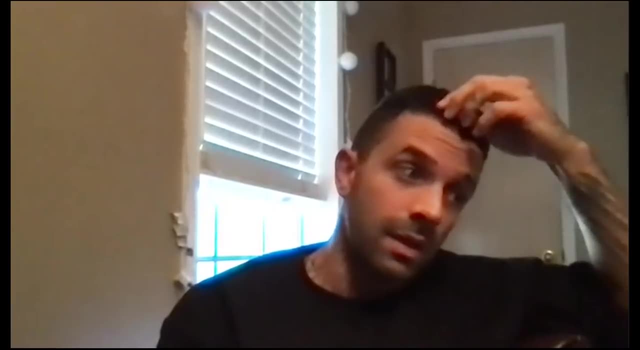 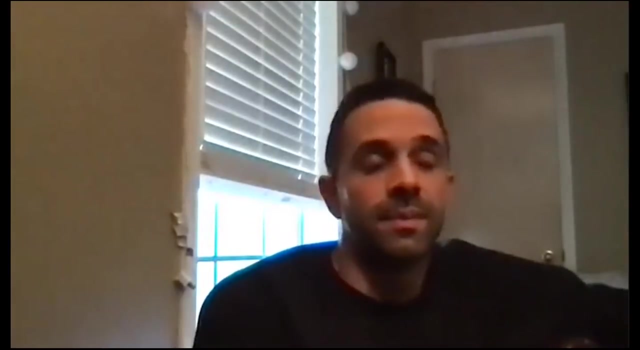 obscure them. but in some cases i think, you know, if it's not rare and it's not something that people are likely to poach, uh, i like having people know those things are out there. i like people, uh, you know, having a reason to go check things out and, you know, get excited. it's a pleasant escapism. 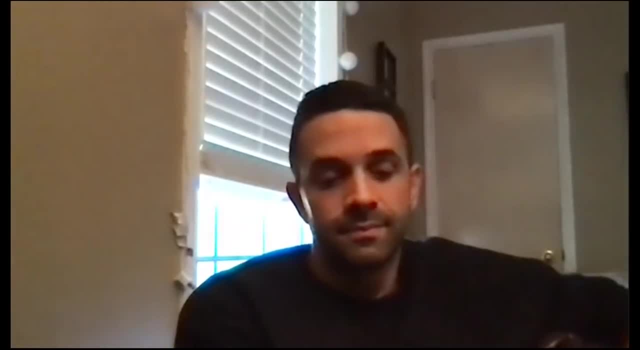 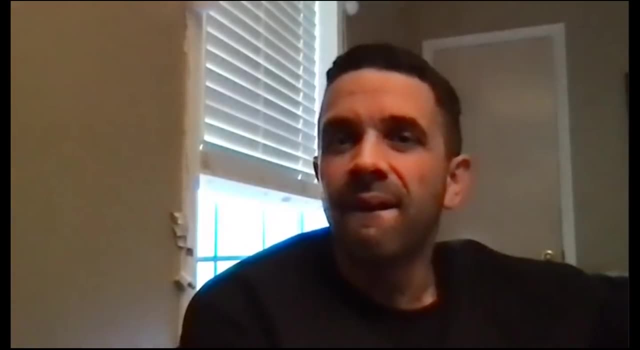 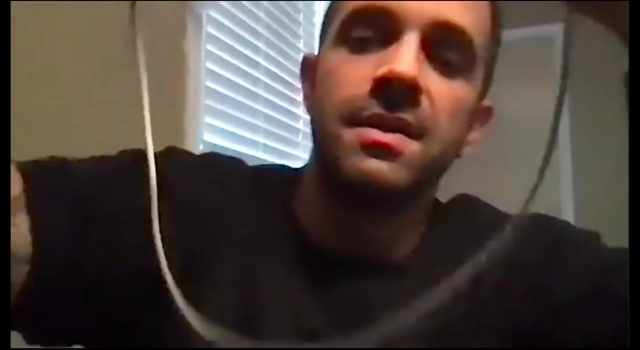 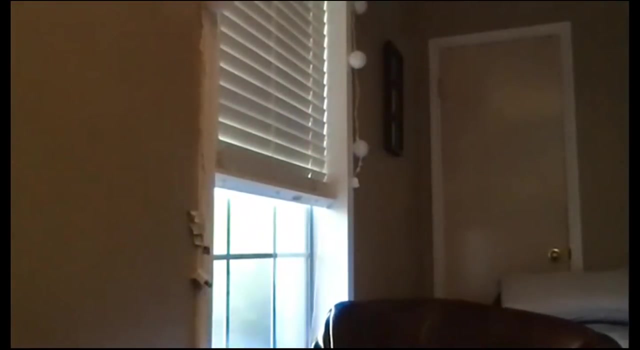 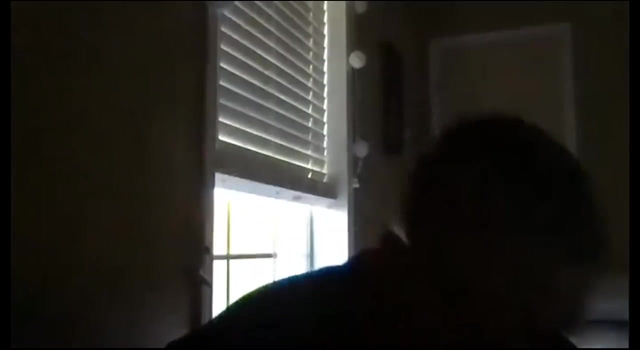 from: uh, you know the dystopia, so anybody else? uh, so yeah, i've, yeah, oh, oh, this might hold on. i gotta plug this uh laptop and it might croak if it goes out. sorry, you're still there. okay, something fell out, but okay, let's try this. 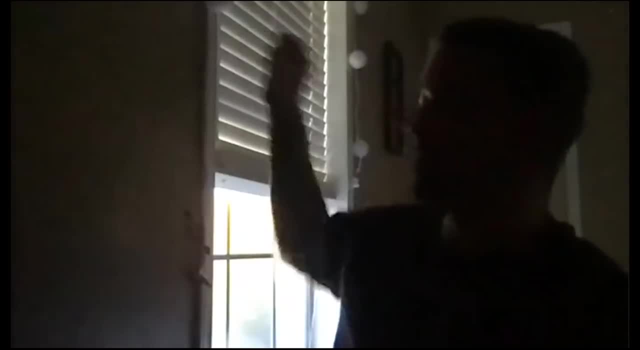 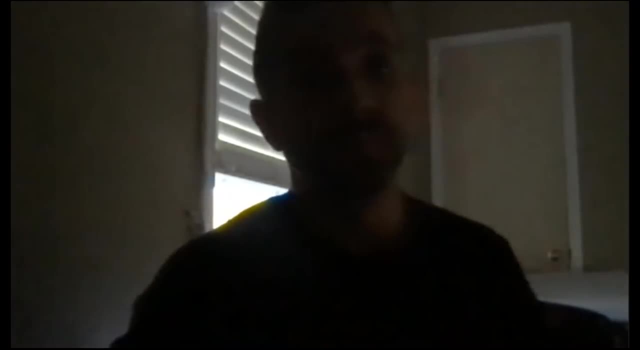 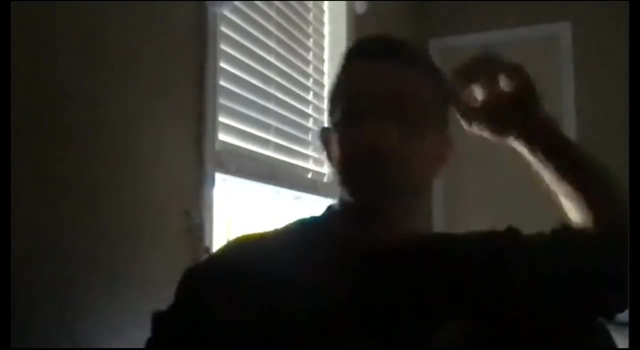 Okay, Charging All right. Yeah, What's up? Got a little darker, but So so yeah, I had a question about propagating. I think it's a cymopterus fenderellii, right? So it's a cymop, and and it's it's. I know your stance on foraging. 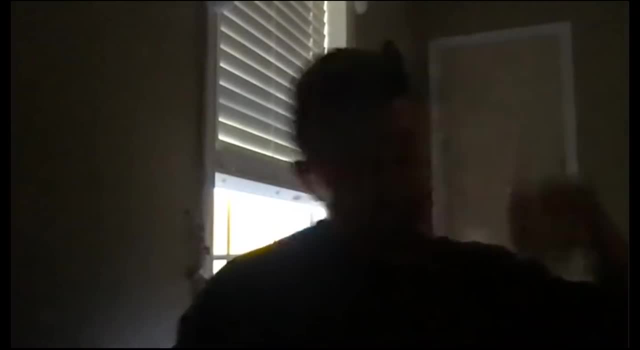 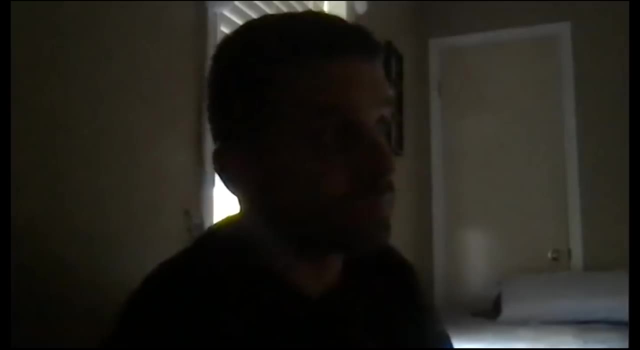 It sucks, And I thought about it before and I want to try to cultivate it. So what you know, if you know what, where do, where do I go to try to you know, figure out how to get this thing to sprout. 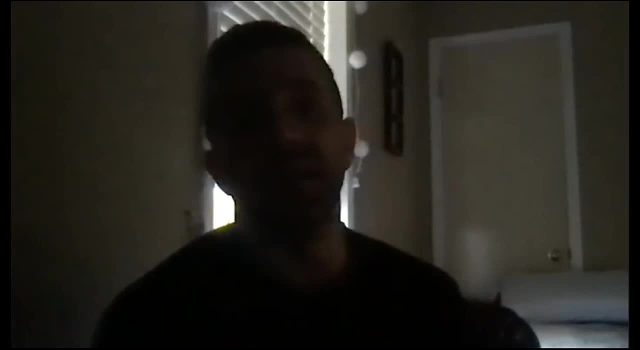 I would just well you could go to Google scholar and see if there's been any papers written on the germination. There's probably not, but but you know, I want to make clear like I don't. I. 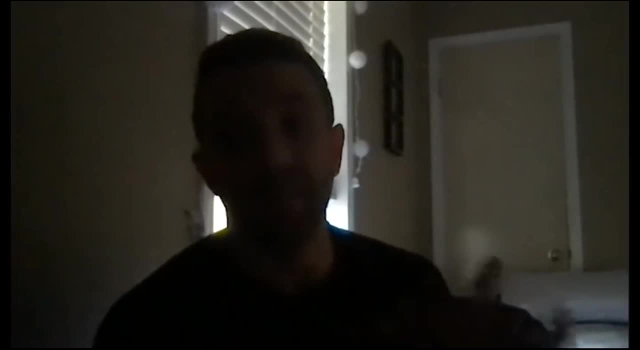 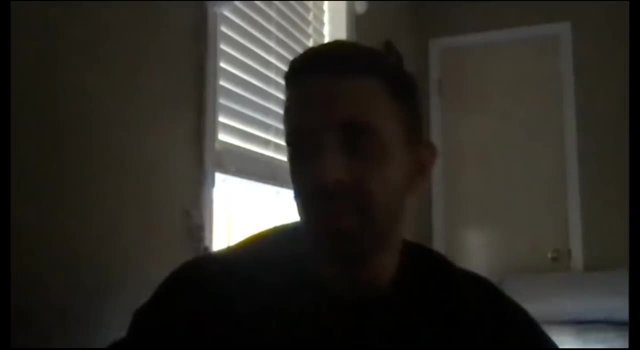 my own personal opinions on foraging. whatever I mean, I like the plants that have been through the 10,000 years of human selective pressure, but it's it's harmless if it's done in the in a harmless way, Right. 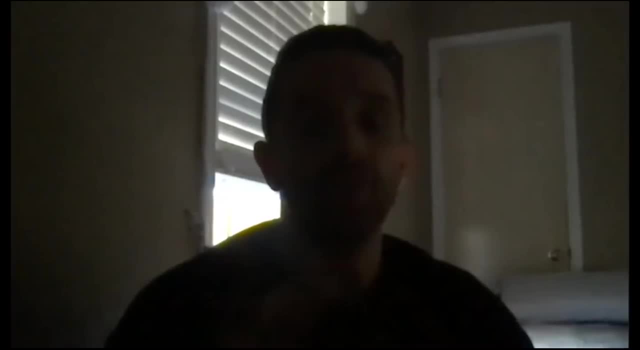 But it's when people just go out and they want to just get that consumer attitude and rip everything out, when it's you know, just for the sake, whatever it does, it doesn't matter. But if you want to cultivate some operators, 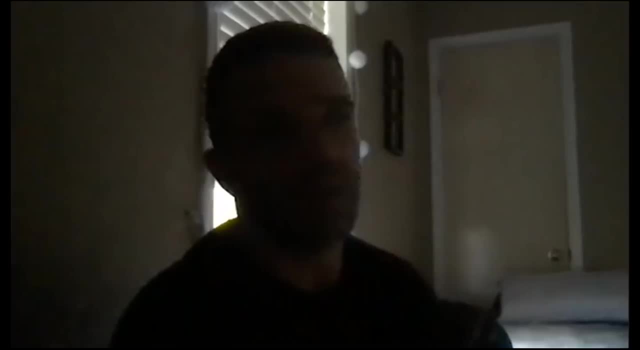 that would be cool when you could even breed ones, If you do long enough, that are more advantageous for human consumption. you know more bigger leaves, whatever the fuck. If I know where to germinate it, though, I would just look up just germinating the cymopterus genus. 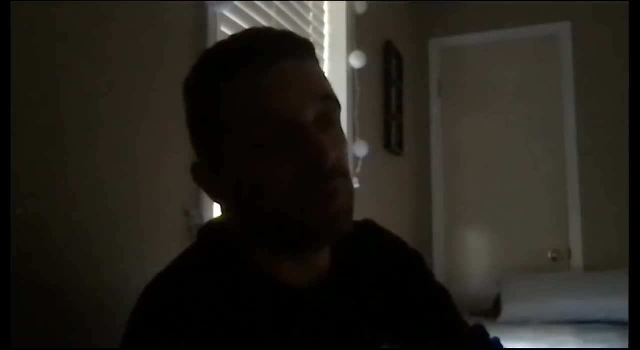 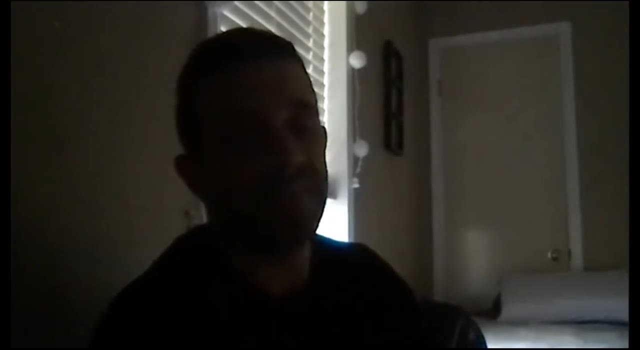 And short of that, I would just try- if it's from an area that gets cold winters, just try cold- stratifying it in a bag of moist- not soaking wet but moist sand in the fridge, And not that some of that moisture is going to you know. 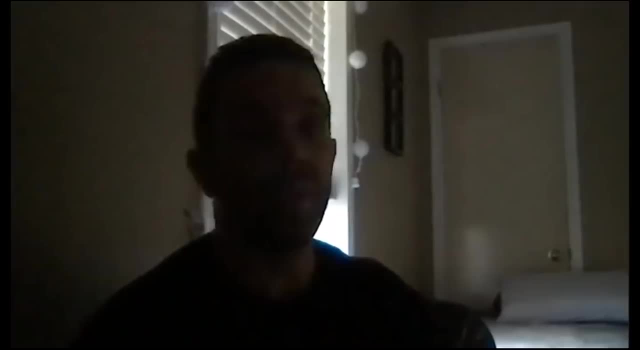 permeate that seed coat for a few weeks, for four weeks. If it's from like a desert area it doesn't need my. stratification Generally always improves things. Cold water always generally kind of improves things. but yeah, I don't know, I would just try it out, man. And if it's, look at the soil. if it's, if it's from a desert area- I'm not familiar with that species, but from a desert area where there's not much organic material in the soil, try a mineral, more mineral mix. You know, if it's like a desert plant, that's. desert plants tend to rot easily. easier. and in cultivation, if they get too much moisture of the substrate is too wet. So, um, let me try turning this light on. So I would just I would start there. You know, I mean the really the best way to do it sometimes is just to try and maybe that light. 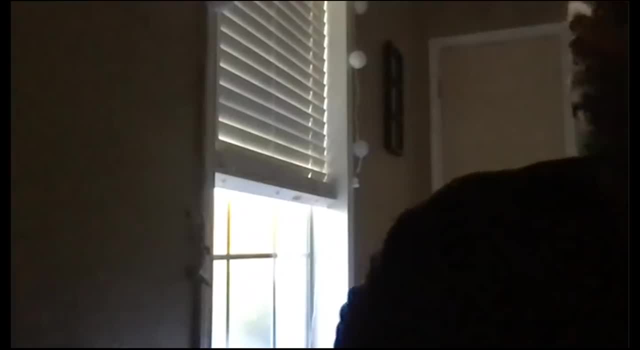 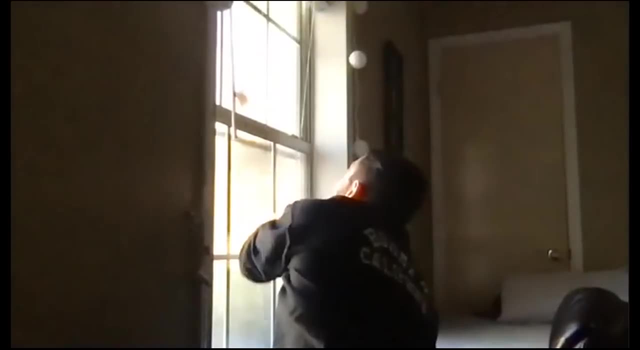 doesn't do shit. Maybe you won't. you won't get any germination, Maybe it'll work out really well. Uh, just try it and see, be your own fucking scientist. you know, Yeah Cool. So, uh, anybody else. 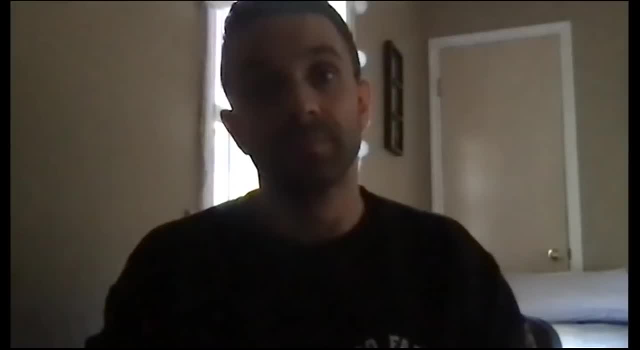 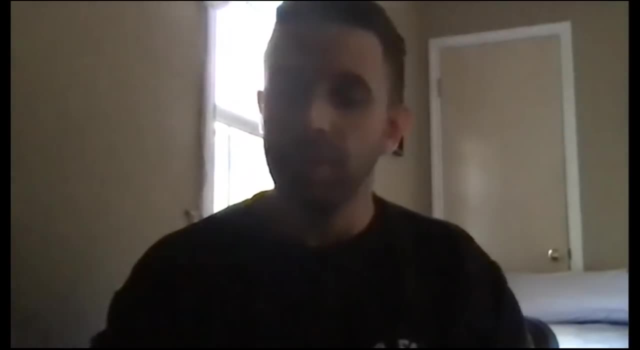 So I've been out several times and uh, uh, when I find like a new species and I'm totally stoked, stoked about it, and then I go to look it up, and then there's not really that much information on Wikipedia or or any other sites else that I'm looking at. 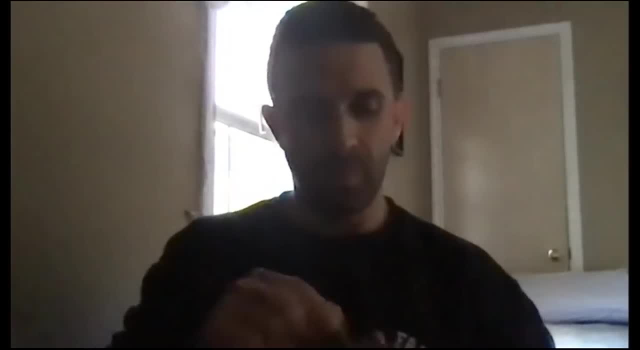 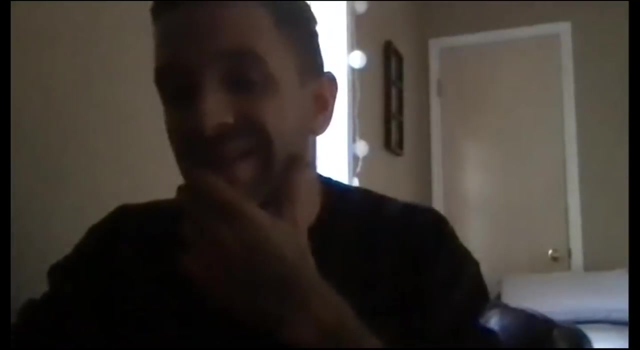 Are, uh, for specific species. are you usually looking at scientific papers, or are there any other resources that you'd recommend that are good for just- I don't know- learning more about the plant, about its ecology and stuff, or Yeah, man, that's a problem that that I really, you know. 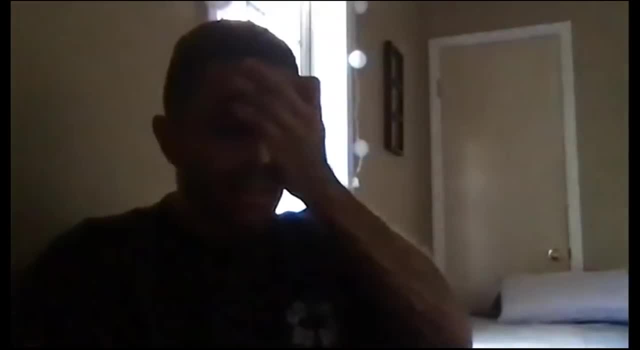 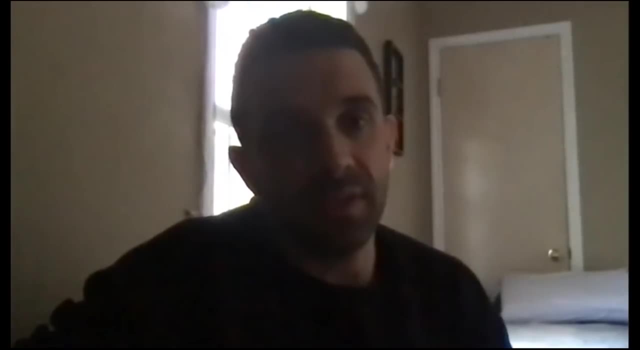 first encountered a lot when I was getting into this and that's, you know, uh, my friend Matt, the guy that's in defense of plants. that's what he mostly does. I mean he, like he's been in grad school for the last four years in Champagne. 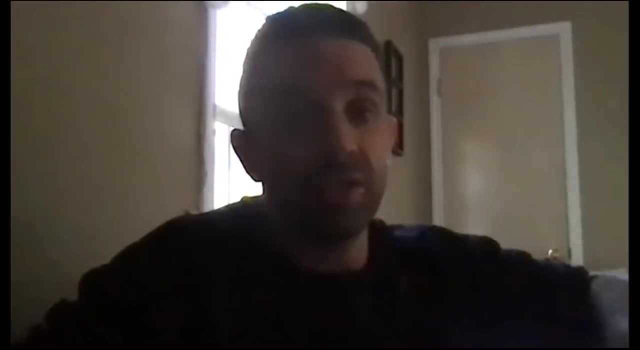 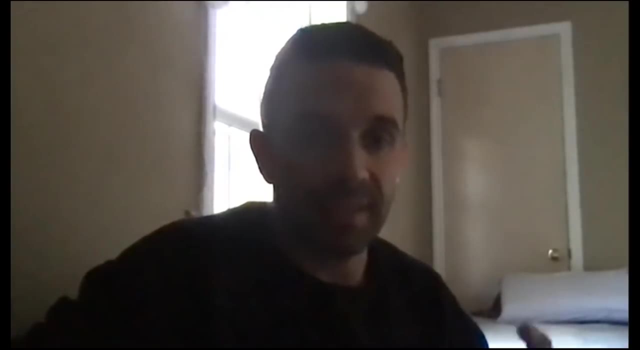 he's not traveling to these areas to see him. Uh, he just is really good at doing research and figuring stuff out and then putting it, digesting it into a really easily digestible, uh, articulate way with good photos, And I mean he's- he's excellent at that, you know. 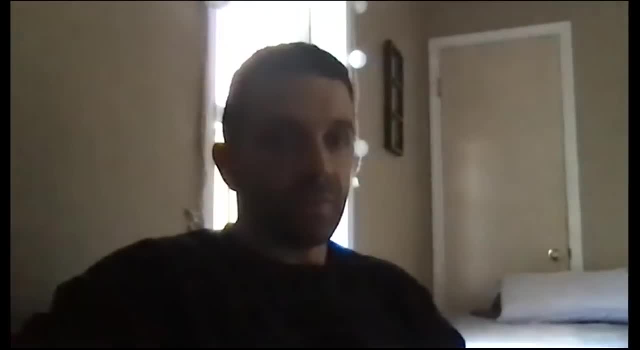 Um, so you just gotta- and I've always been good at doing research. He, when I was riding fucking freight trains, I was always good at figuring out where the fucking yard was, when the time when the trains left, what they looked like, you know whatever. 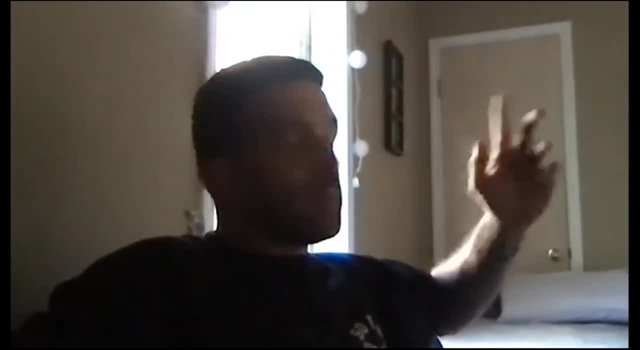 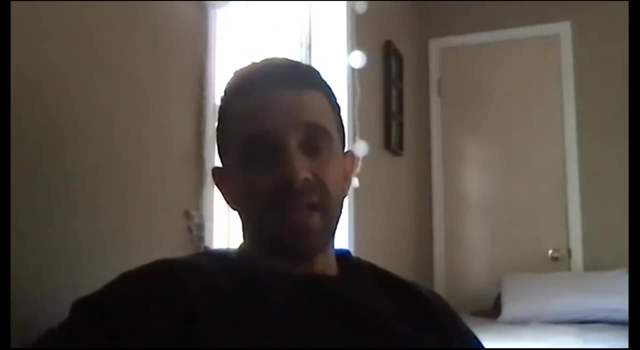 Um, so it's just, you know you're. if you're obsessed about something and that's everywhere you just find a way. Google scholar is your friend- scholargooglecom. I mean, even if you don't understand 90% of the words in there, there's going to be little. 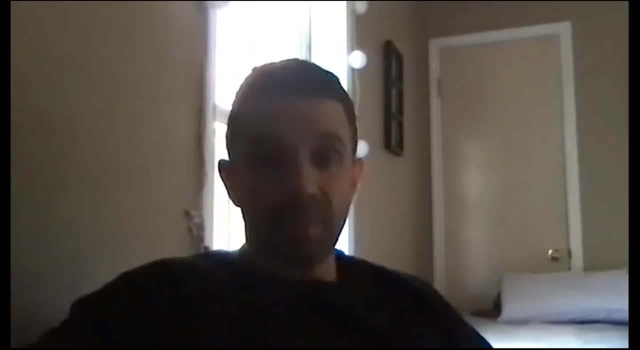 bits that you will understand it in the abstract. you know the introductory piece, whatever Um and there's, there's always an ecology there. I mean certain genera, certain families just have ecologies that are kind of written in there. 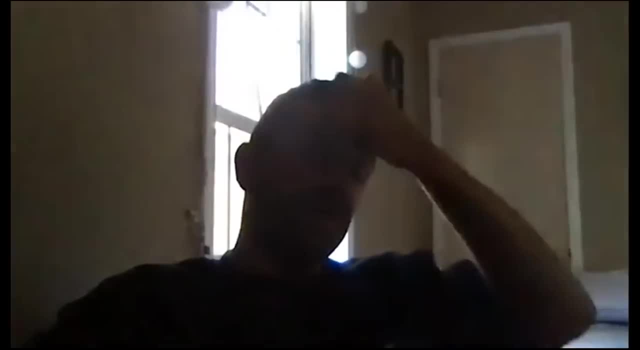 Like the footnote, like this plant normally grows, a lot of members of this family Grow on limestone. A lot of members of this family grow on serpentine, A lot of uh. this family has been really successful in the deserts. 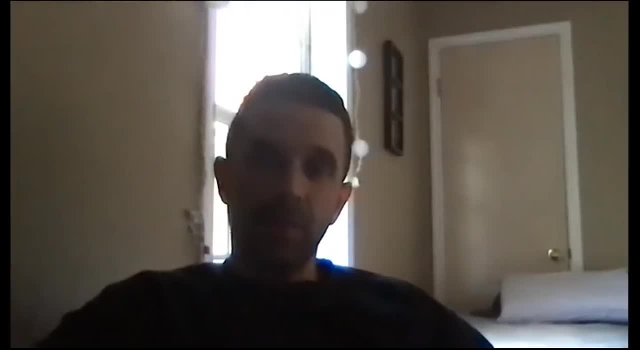 So there's always to get more of that story. I would do. yeah, Google scholar, Wikipedia can be good. Uh, if some schmuck wrote a book on the genus, cause they love it. You know there's info there. 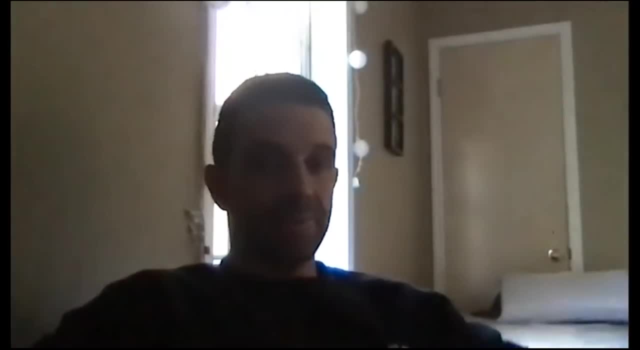 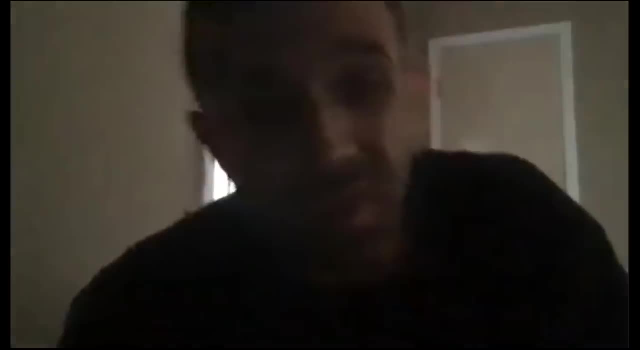 Um, nothing really beats going out to see it and kind of make observations, you know like an evolutionary detective or ecological detective. but but scholar Googlecom is definitely your friend. you know Cool Thanks, Yeah, sure Anybody else. 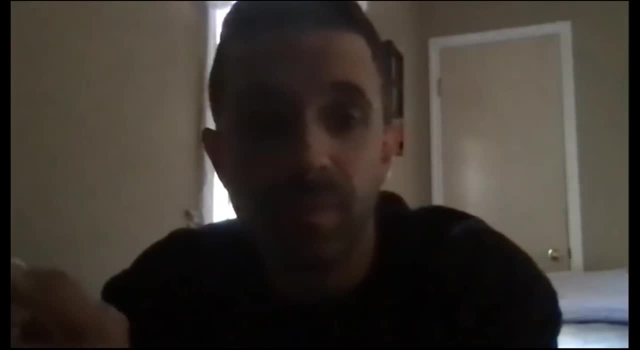 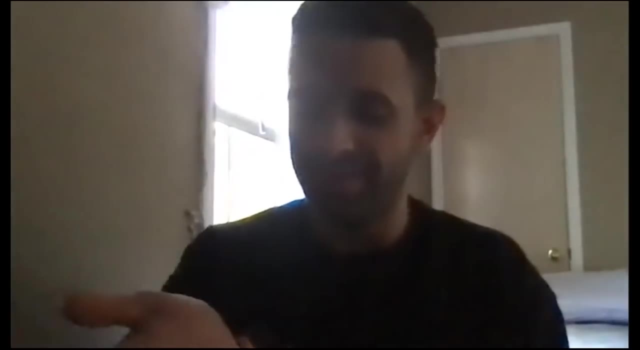 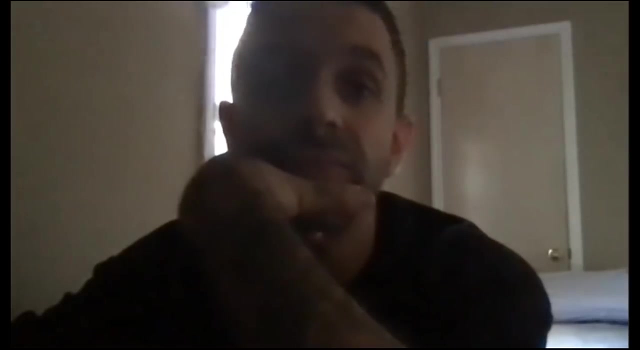 Um so around where I live. well, all over the United States, the um I land at LTC, the tree of heaven is a massive issue Um and I'm near Philly, So we recently got inundated with spotted spot Atlantis. 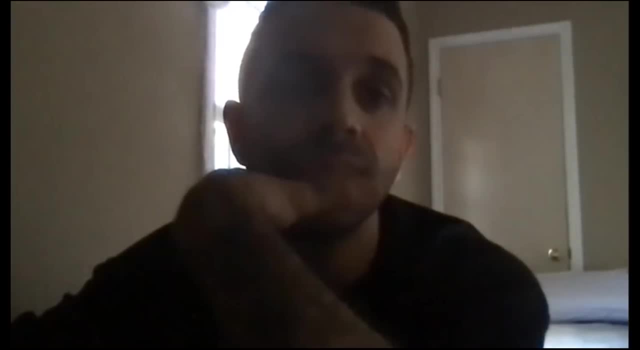 Yeah, So it's like a very long時間, And the reason why I'm near Philly is because of the tree of heaven. I see some lanternflies, gigantic leaf hoppers, And it just so it turns out that in Southeast Asia, where these things originate, um so 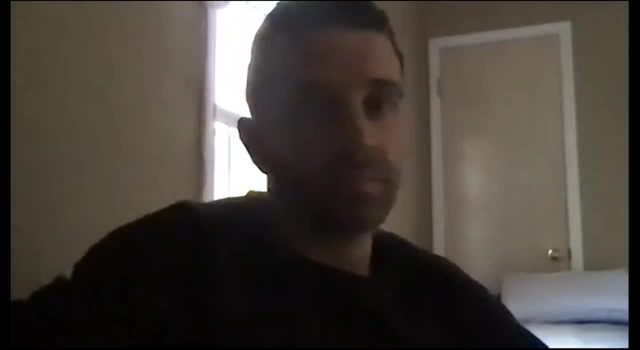 does the tree of heaven So in your opinion? well, and they, they brewed on them and they, you know it's essentially replication of their um natural Well, tree of heaven. I'm not familiar with spotted lanternflies. 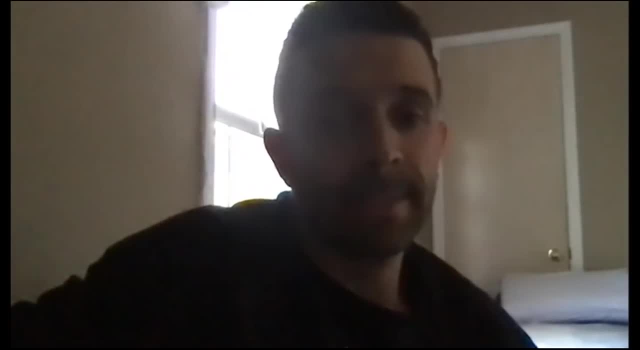 Tree of heaven is a host plant. yeah, um yeah, spotted, spotted lanternflies- are these big leaf hoppers? they're really pretty. it's a shame, but they're pretty destructive to crops. um, yeah, and we put all this effort into spraying down with pesticides and making sure all of the lanternflies are dead when we have. 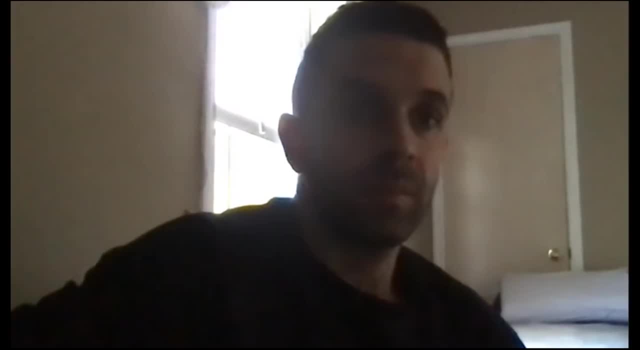 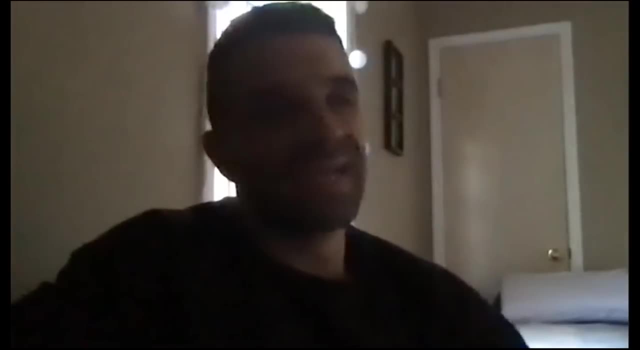 this massive population of host plants. you think we should be focusing more on the host plants instead of just bombing the area with pesticides. i mean bombing an area with pesticides again, it's that sledgehammer. when you need a scalpel thing, i mean it's. you know, i had like a, i was growing. 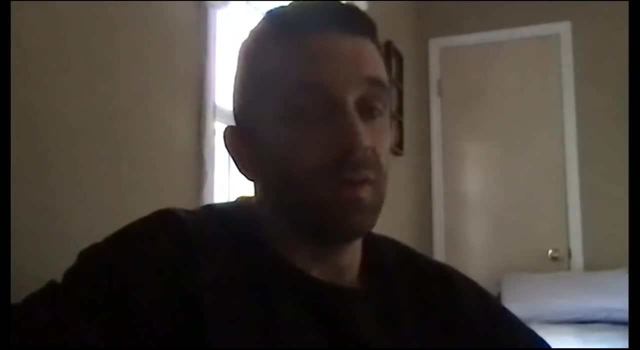 a bunch of shit in my greenhouse once and i had white flies all over like different species of salvia i was growing. i was growing, like you know, 20 different species of these central american salvias, and so i tried the organic pesticides, the pyrethrins- the quote organic- i tried everything. 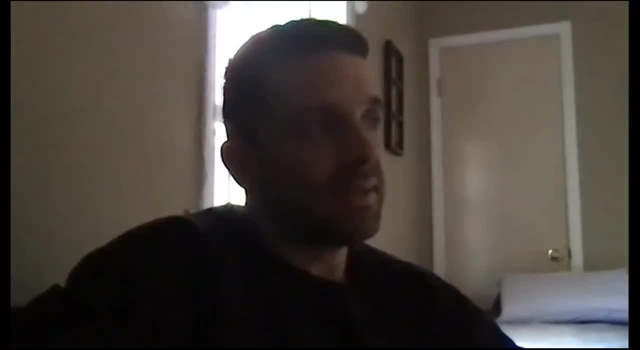 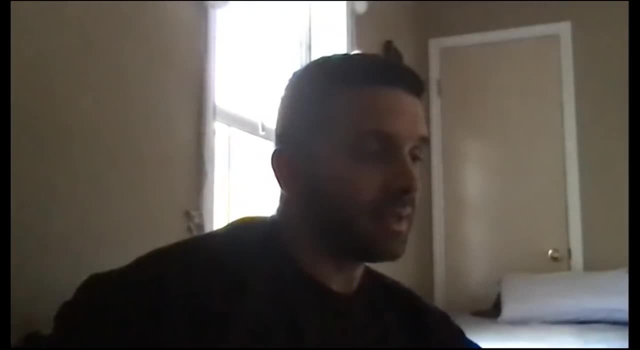 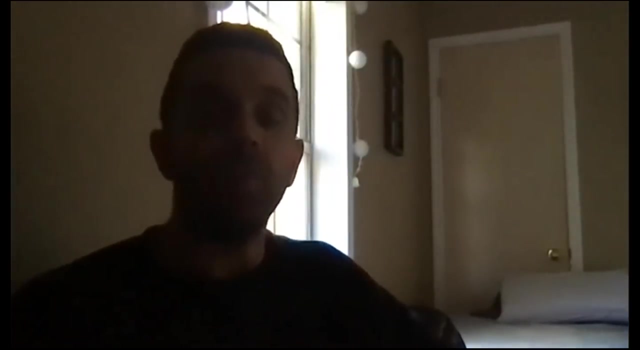 and the white flies get knocked out. they'd always come back, but then none of the other bugs were on. i was like this is fucking stupid, why am i doing this? what finally changed things was when i got- uh, some species of spiders showed up somehow in my greenhouse and then it thrived. there was a big food source for it- all those white flies. 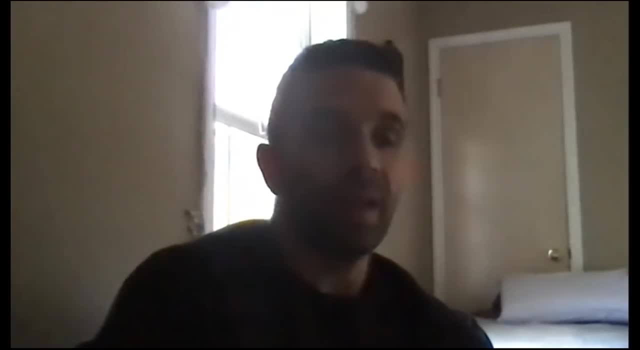 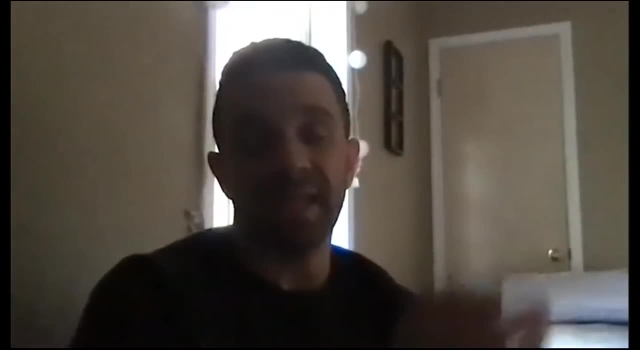 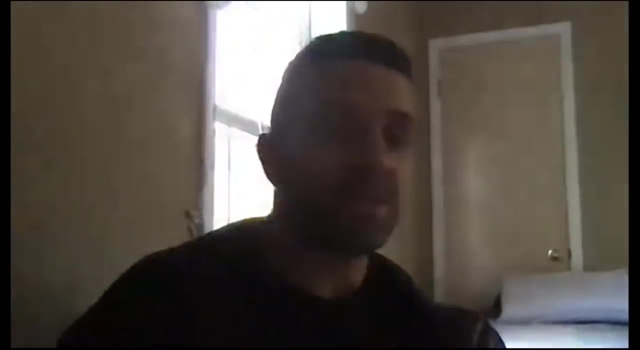 now there's this: fucking spiders are everywhere and i barely have any white flies anymore and they do great, you know. but but actually before that i stopped spraying the pyrethrins because i realized i was killing everything and then just started physically spraying the undersides of leaves with water. i got like a little mister attachment. so every, every other. 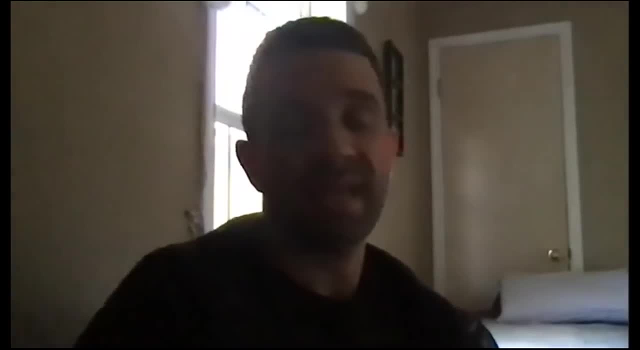 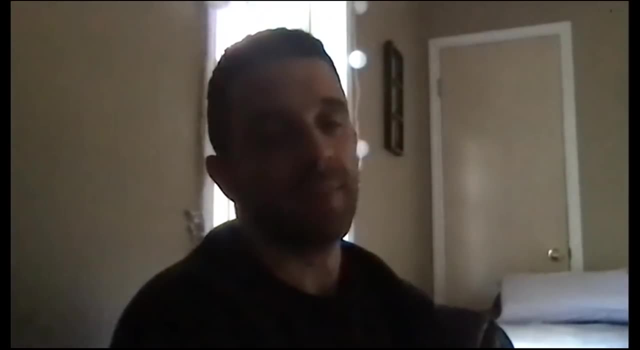 day, whenever i'd be out there watering, i just spray the undersides of the leaves, which is where the white flies hang out, and fuck them all up. you know, probably kill a lot of them, because once they get their wings wet they're done um, and then just let the spiders come in. i mean, it's always with. 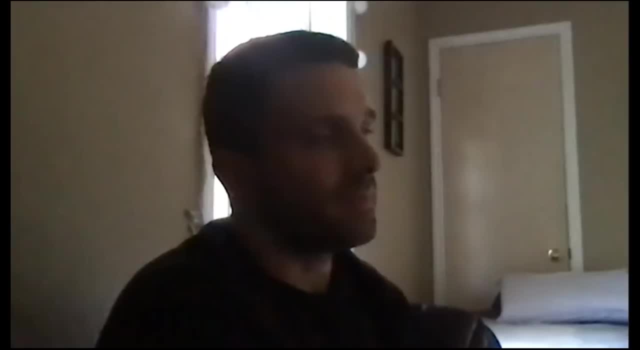 ohlantis. you know we used to climb that tree all the time, used to get on abandoned buildings and shit when i was a kid in chicago. but i mean it's always a good idea to get rid of ohlantis, man. i mean it's not so much a problem out west. you get to the bottom of the tree and then you get to the. 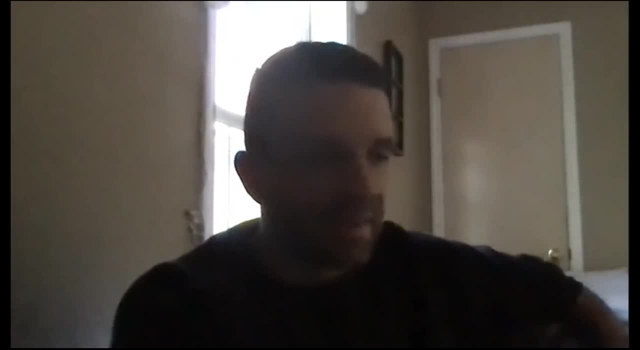 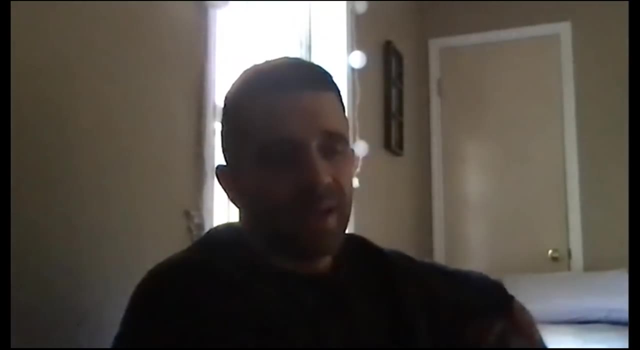 it in some areas, but it's generally too dry for it, our climate is. but in areas where you got those summer, uh, summer rain, uh yeah, atlantis does well- and that the way to do it is just, yeah, cut it and then spot, apply- uh, herbicide, you know, but pesticides are so fucked man, i mean really. and 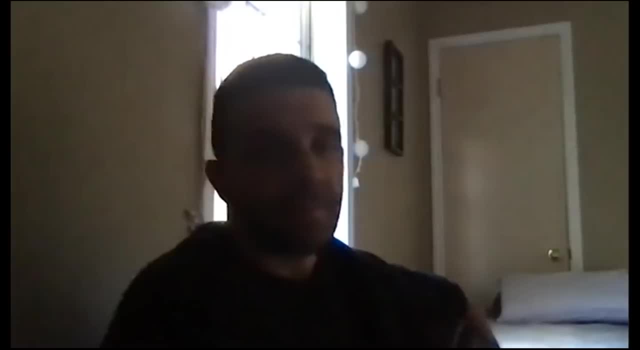 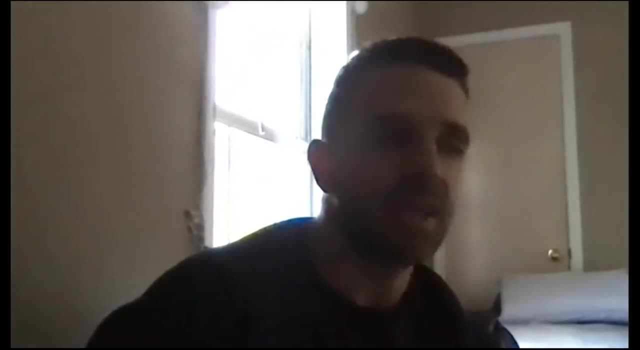 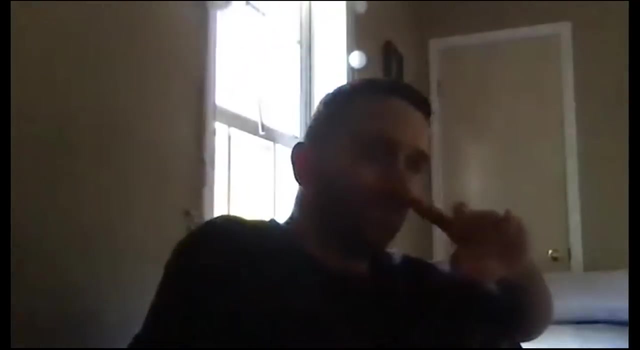 it's so crazy because you kill everything and a lot of insects you want around, you know. i mean, if it's bad where it's like malaria and you got to spray for mosquitoes, okay i understand it's not ideal. i'm actually in favor of that fucking genome that the suicide generation. uh, gmo mosquitoes. 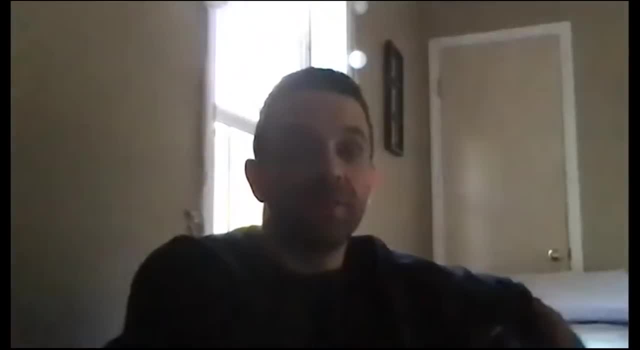 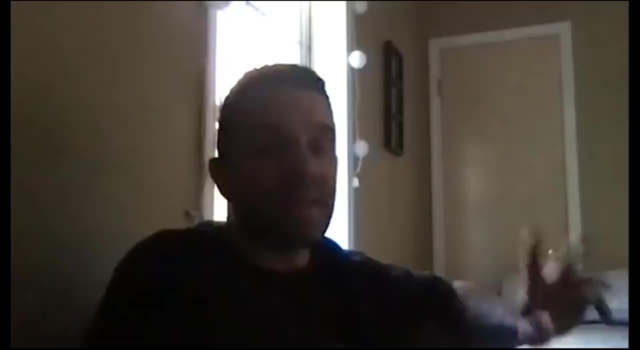 man, it's uh, you know, it couldn't be any worse than we're already fucking up the planet. that's really bad reasoning. but you know, i also understand how the genetics of a word seems kind of cool. but anyway, that that aside, i would, i would just, yeah, always get rid of atlantis, i mean. 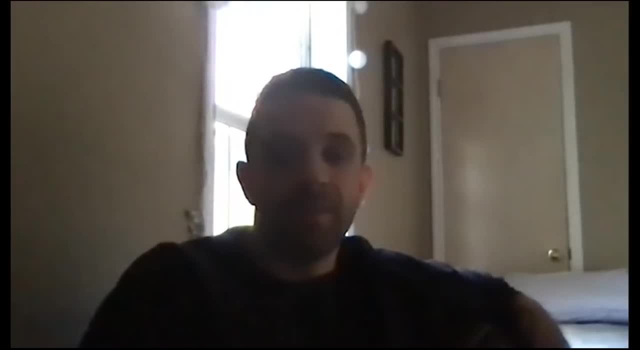 it's such a fucking. it's funny because it grows out of a you know roofs of abandoned buildings, but it can be a you. it's just kind of a fucker of a plant so, and i don't know the actual ecology, if it's like, plays a certain essential part in the life cycle of that. 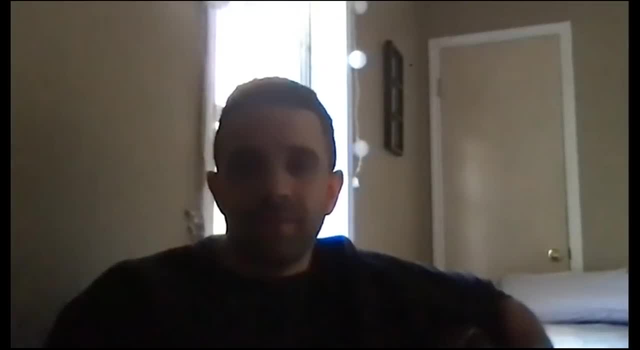 insect, but just get rid of it anyway, fuck it. and someone just chatted asking what the negative impact of lanternflies are. um, they're. they're crop eaters, essentially. um and their um nymphs put off this sticky resin that gets all over everything. it's just disgusting. 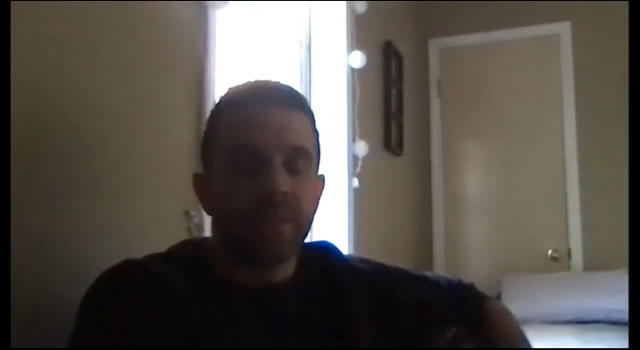 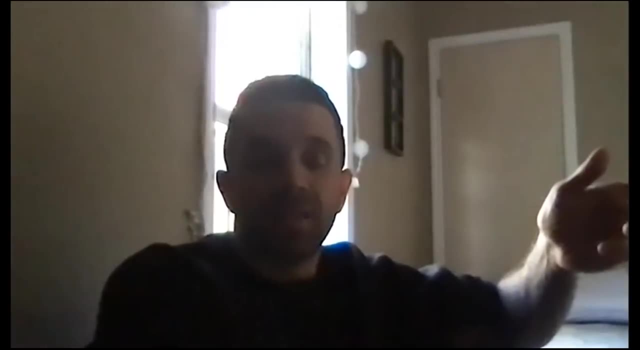 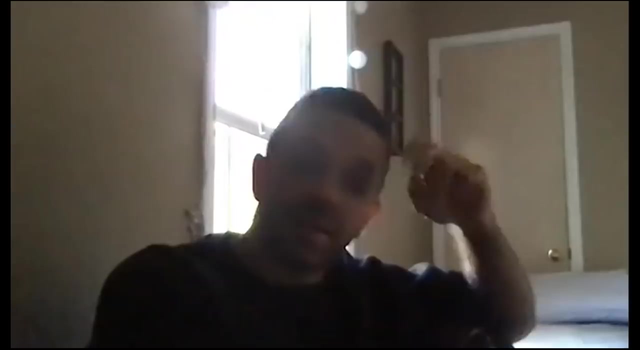 uh, and they multiply by the thousands. they're just, they're bad for everything really. yeah, damn man. but yeah, and of course eventually something will evolve to specialize on them or eat them. but how long will that take and how many extinctions will they cause in the meantime? yeah, not as fast. 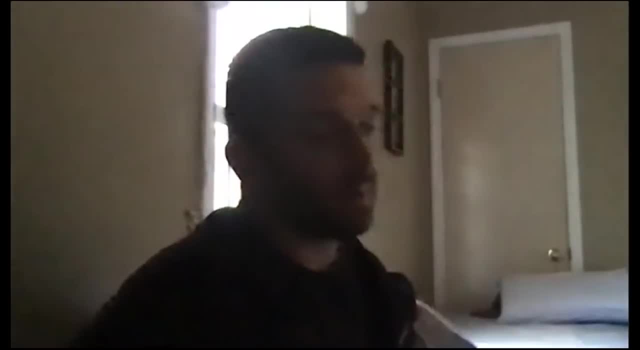 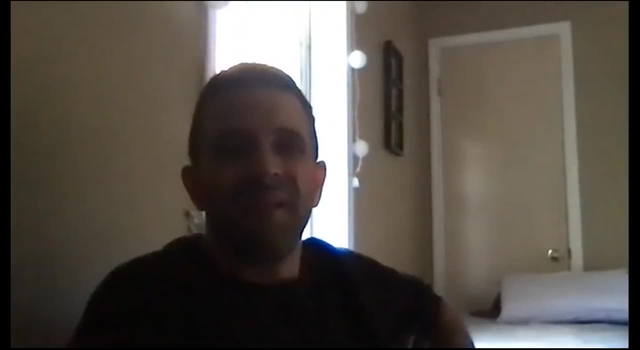 as they take over everything. right same thing with all invasive species, you know. so, uh, yeah, next person, hey, so, uh, i was out in the mojave the other day and i'm sorry if, uh, this might have been your episode about philisma, but i was looking around and i was wondering, like how? 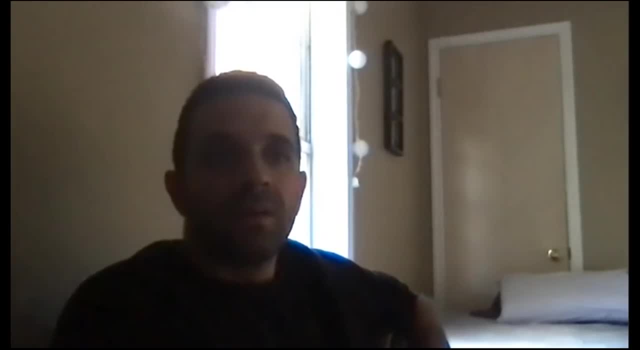 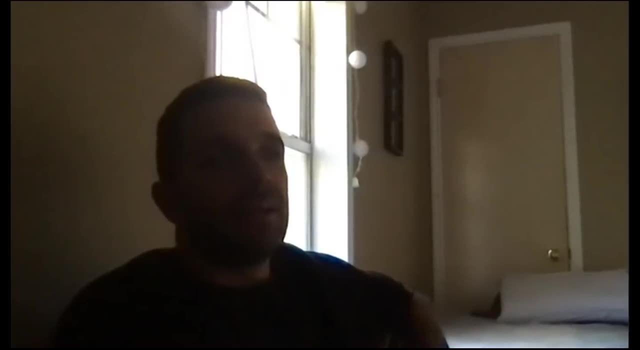 how did you, how do you find them? like they're underground, right, so well, yeah, well, they come up, they surface. uh, one species was up already. uh, the more common one, erinaria and cenoriae, was about to emerge. but um, but i, it wasn't up yet and the way i found it was like the same way you'd find a truffle: i. 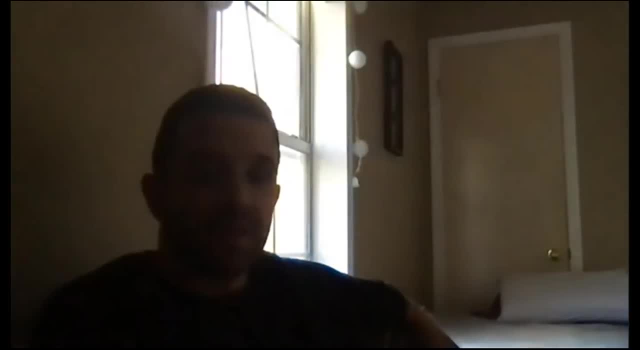 just i looked at the host plant, looked around the host plant, which was ambrosia, and saw a spot where, like, the soil was pushed up and then excavated it a little bit and there it was. i found like two or three more, you know, but that it's funny because that that area is fucking like, you know, it's like. 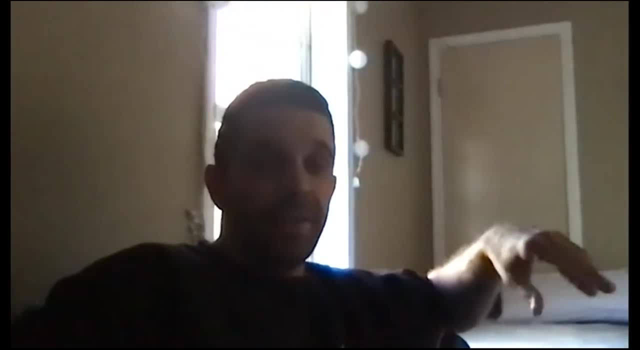 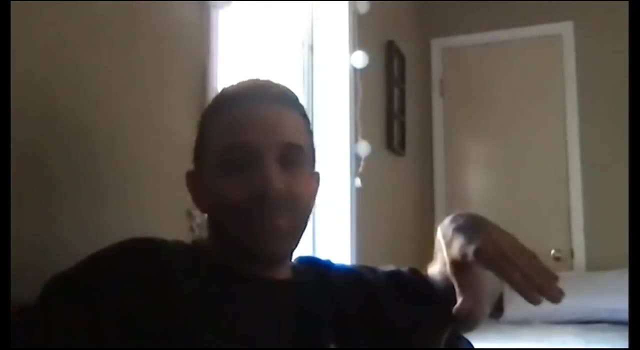 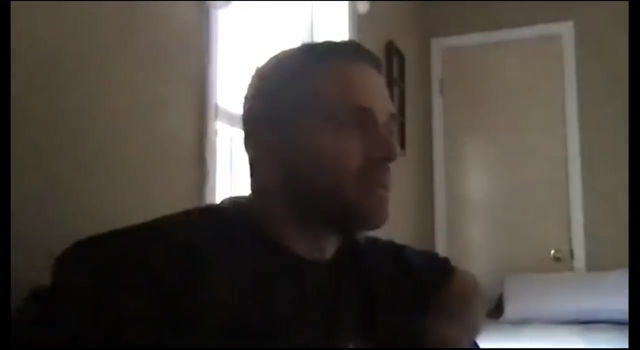 q anon atv. heaven right, it's fucking hilarious, you know. i mean it's horrible, yeah, like south of that road. it's just like some of the fucking worst, some of the worst people america can produce, and then the world it's all. yeah, it's like they. i feel like they're, like you know, fucking glaring. 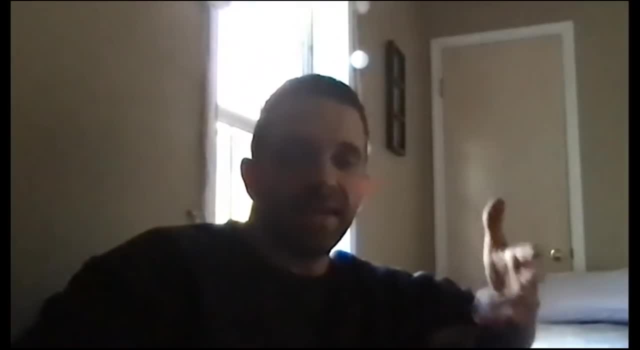 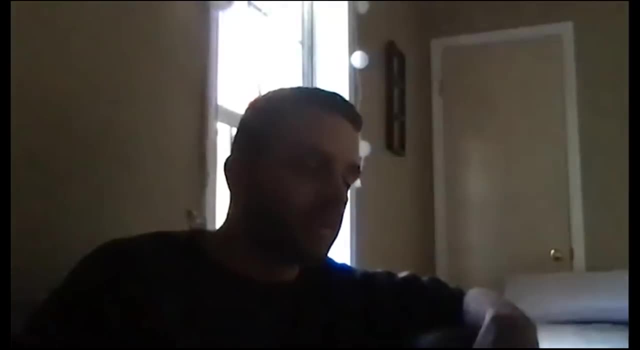 at you and calling you a fag for, like, stopping to look at plants. i mean, it's that kind of shit for brain. and the same thing they do when they see you wearing like a mask. you know, like, oh, i had. i had someone stop me and ask me why i was wearing a mask in my car. yeah, like, why do you give a? because 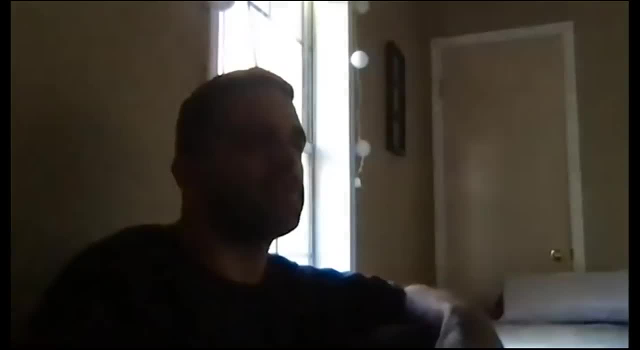 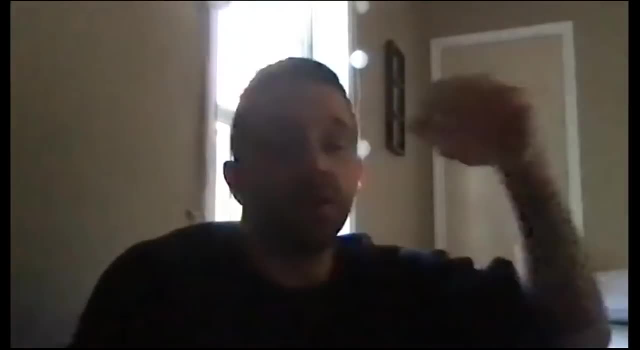 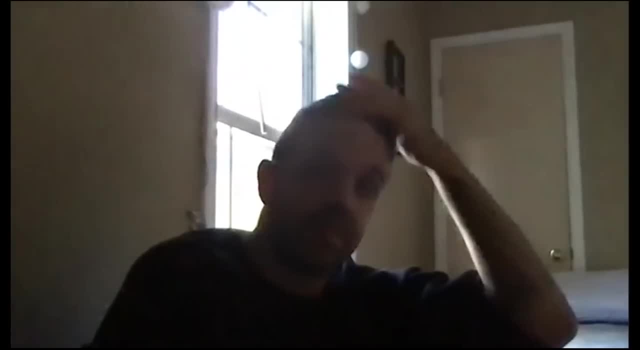 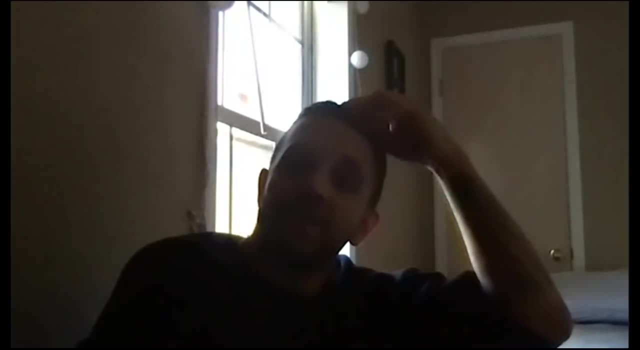 here is so fucking stupid. now i mean, it's just whatever. but but yeah, that's. uh, that's one way to find. it'd be cool to find new populations of it on sand and across the border in mexico, and that area is not too hectic, it's pretty chill, you can get across. but anyway, yeah, i don't know. 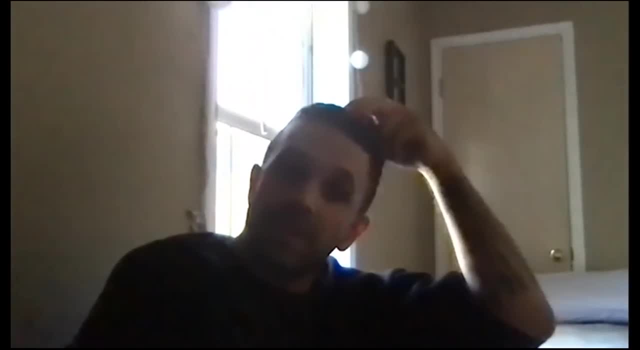 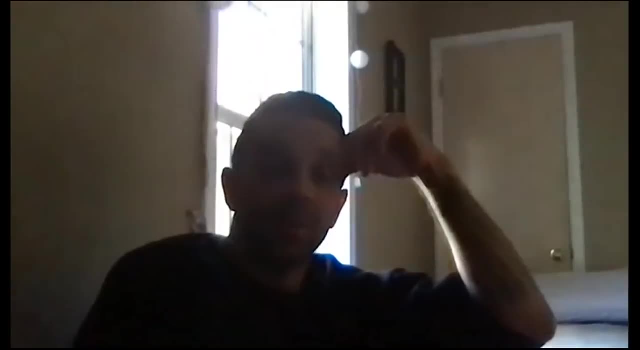 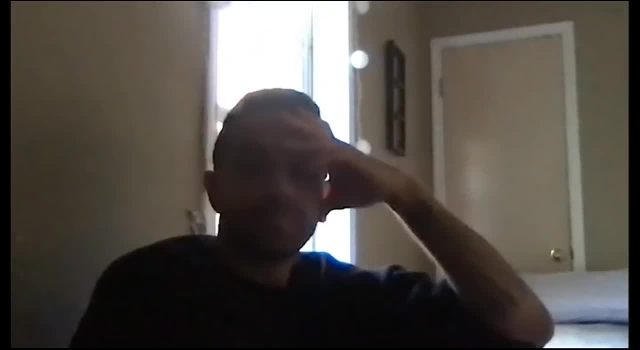 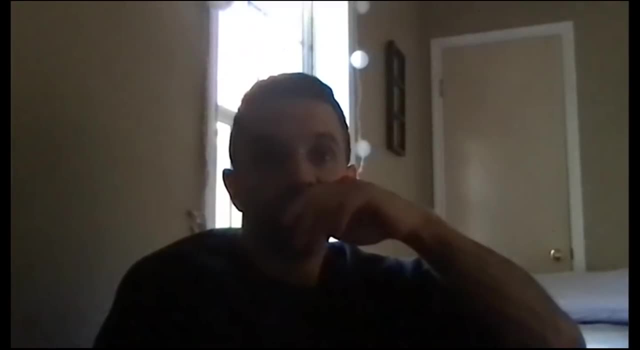 it, so got it, thank you all. right, one or two more questions, then i gotta pee. i got a question about, uh, serpentine. yeah, so does serpentine only occur, like in specific subduction zones, or do you, uh, does it have like erratics? basically like, will you find it in um? 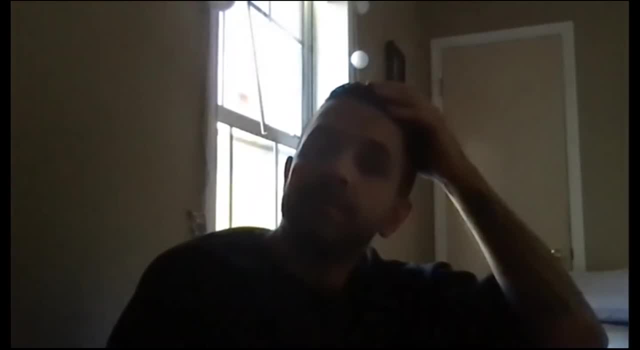 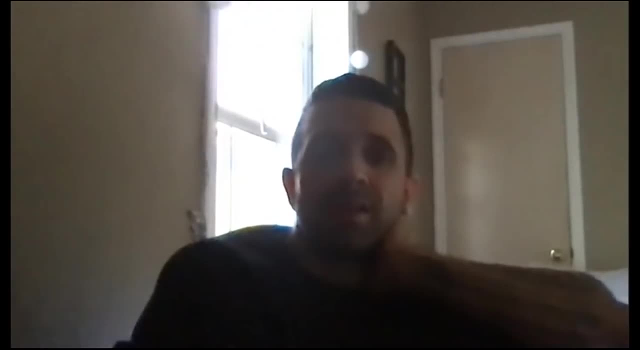 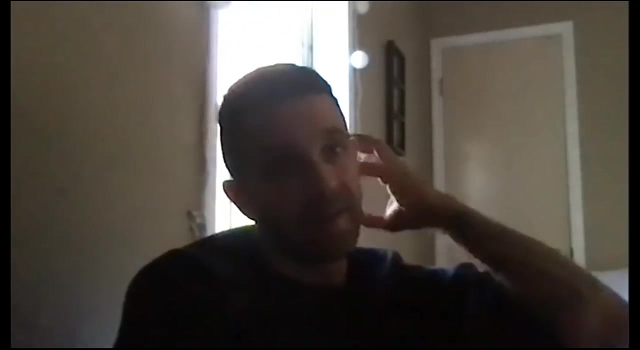 in a more random area, like maybe brought down by a river or something, uh yeah, you'll find cobbles. but in areas where the, the country rock, the base rock is, is not base but the that's not a. i don't want to confuse with basement rock. but in areas where 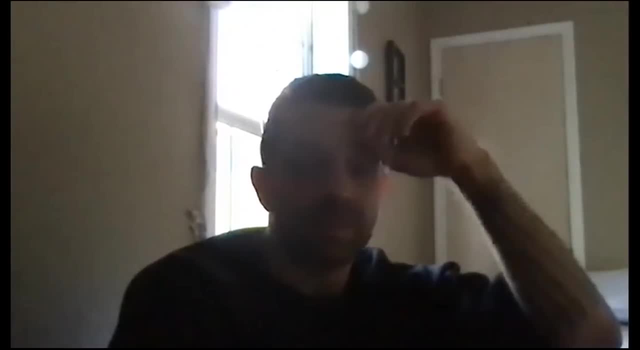 like the general region is all serpentine. it's always put there by subduction zones. but yeah, you could have maybe like there's a serpentine a few miles up up a river that was placed there by a subduction zone 70 million years ago and then 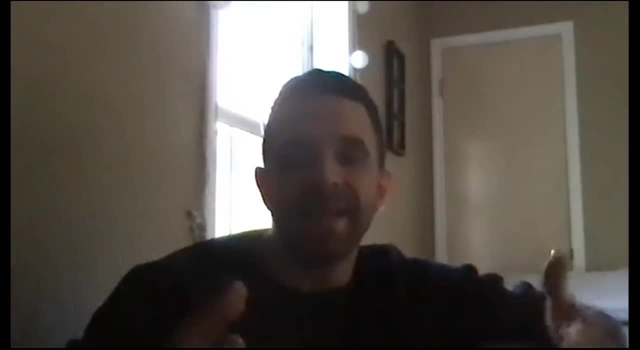 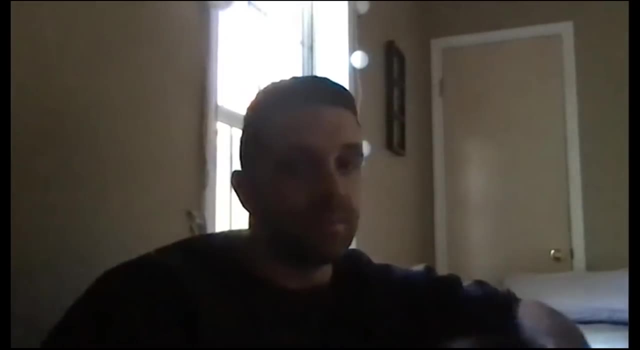 the rivers washed it down, but in areas where, like the- but in that case it's not the country rock, it's just cobbles that have been washed and moved by, uh, the river. they're alluvial deposits, you know, and any place it's the actual rock that is beneath the soil and composes the majority of the. 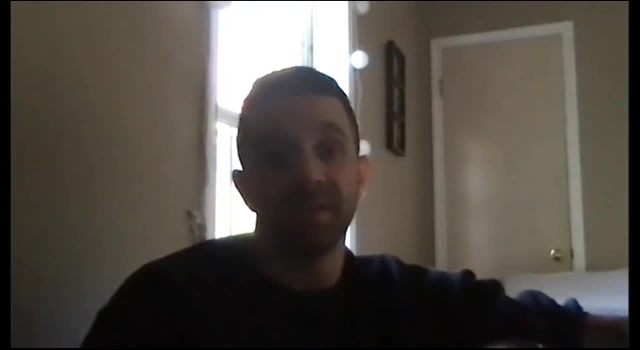 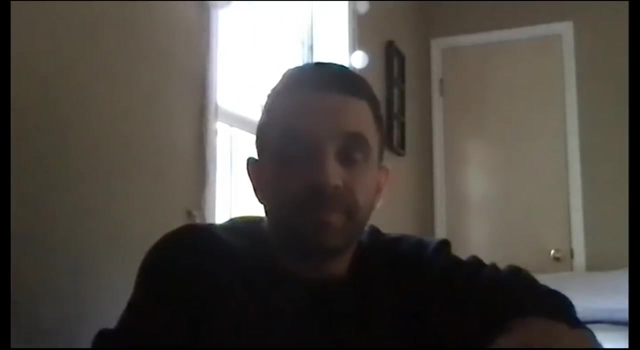 substrate. they're put there by subduction or abduction zones, so subduction zones going down, where instead of going down it gets kind of slapped up on top of the continental crust. Okay, thanks, Some of your cues about illegal planting and trying to get some more just plants in my local area. 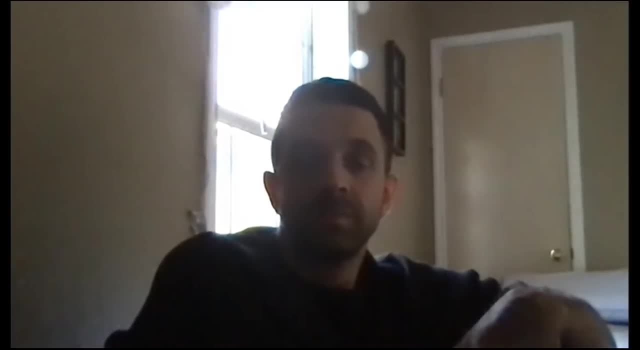 I'm in central Texas and I have some species of Quercus and Ilex going, but I mean the resources that I have for like, where I really should be out there planting and what's really good for local ecology and what's really beneficial. 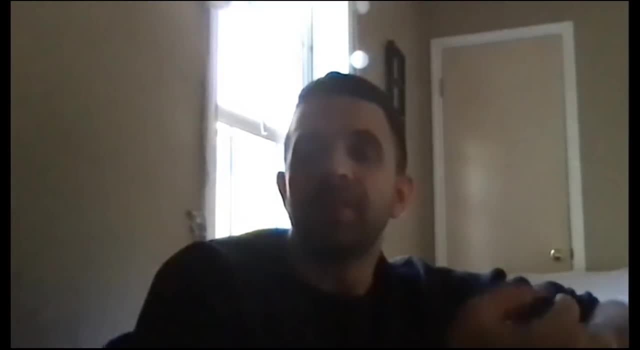 Like I really don't know where to begin there. What do you mean? to find out what you want? more diversity, basically, in terms of like stuff to grow? Yeah, exactly, And I know like trees and shrubs are a good place to start. 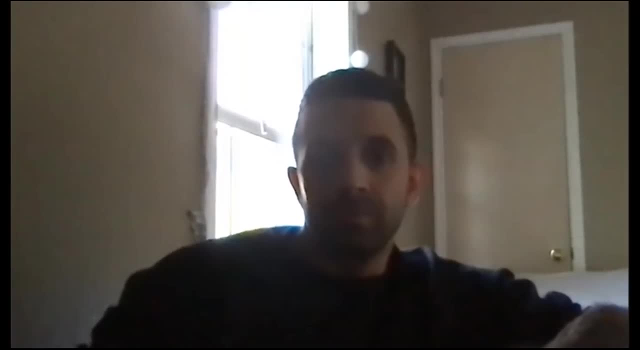 but I mean, that's really. I have a pretty narrow you know kind of expertise there And I really I need to expand my knowledge and, you know, gather more seeds, collect more seeds And I know like stuff that comes up. 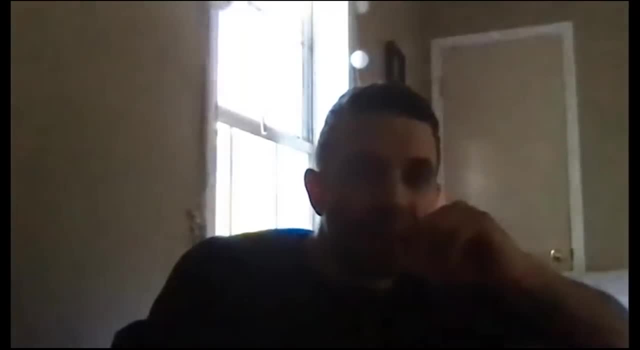 just collect and spread is beneficial. but I really like to, you know, target a few specific things and think plants that are really beneficial for pollinators and things like that. Do you have any resources? You want a good cast of species. You want to figure out what the rest. 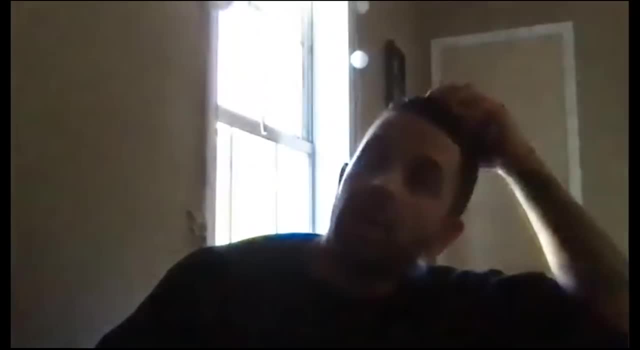 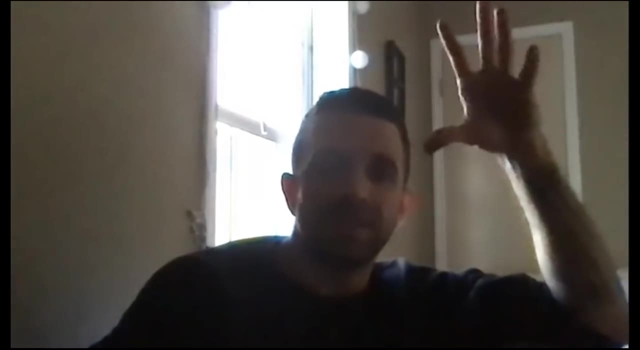 what are some more members of that plant community? So you could do a number of things. You can go to iNaturalist and explore. Most of the stuff that comes up is going to be native. Normally, if people post some shit that's planted. 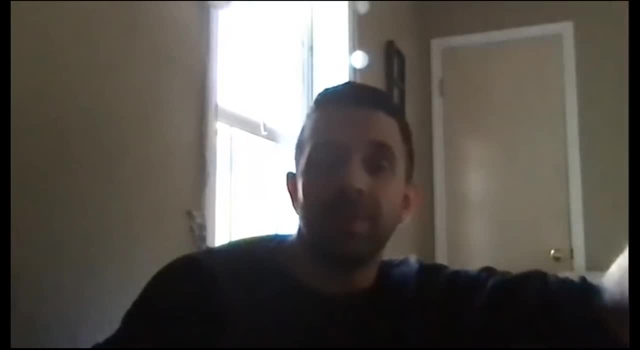 it'll be removed. If it's invasive and wasn't planted, you can go to the species page. It'll say where it originated. It's invasive. iNaturalist, I mean really. the explore feature is fucking great. Just type in a family you like. 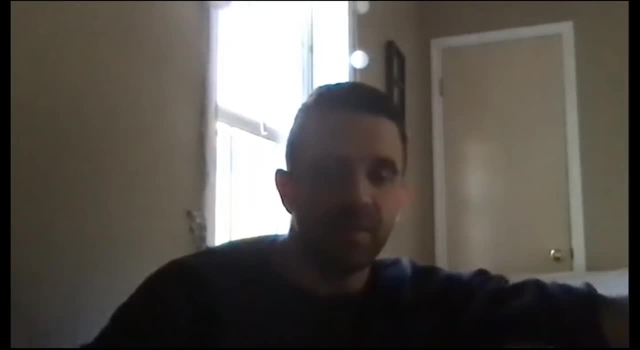 P, family Fabaceae. hit your county, Boom, you get a list of everything You know. it's Asteraceae- same thing. Salvia, family Lamiaceae- same thing. You could also do your own fucking species list. 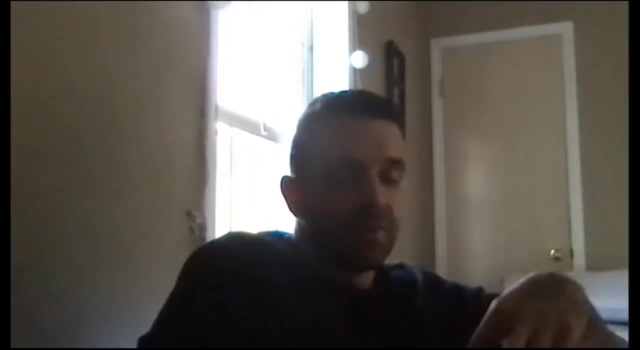 You know, go out to these preserves. what little crumbs of habitat have been left. Inventorium Surveium. You'll also be learning shit that you haven't seen before, Like there's a bunch of cool penstemons that grow around Fort Worth Dallas area. 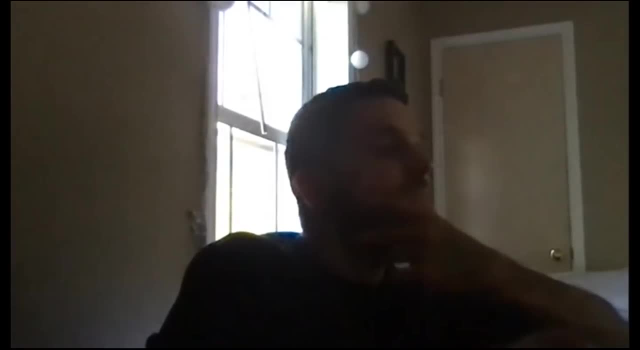 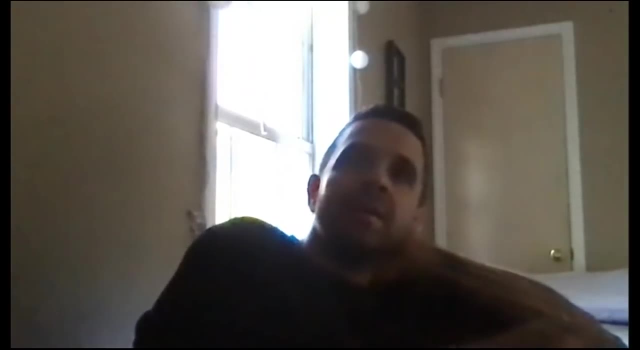 There's a bunch of cool limestone composites that grow on there, like that Silphium albiflorum and stuff. So you just go out and you'll see new shit. you don't know, You'll type it into iNat either- the artificial intelligence. 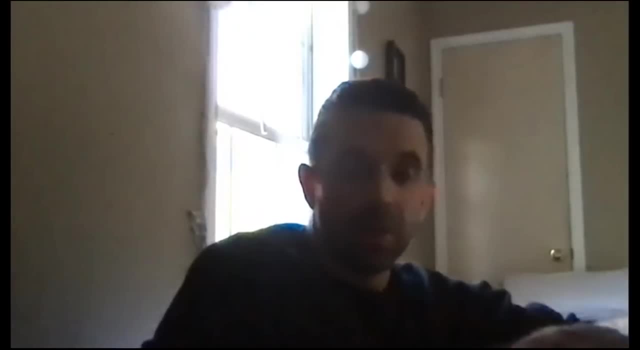 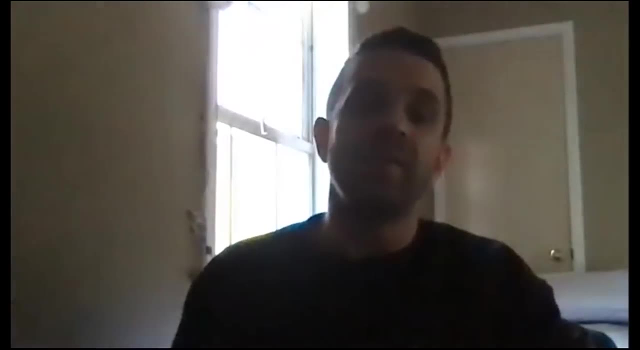 will identify it for you or somebody else will. There you've just learned a new species and now you can just go back to, whenever it's done, flowering, See if the seed is ready yet, if the fruit's ready yet whatever, and then collect your own seed. 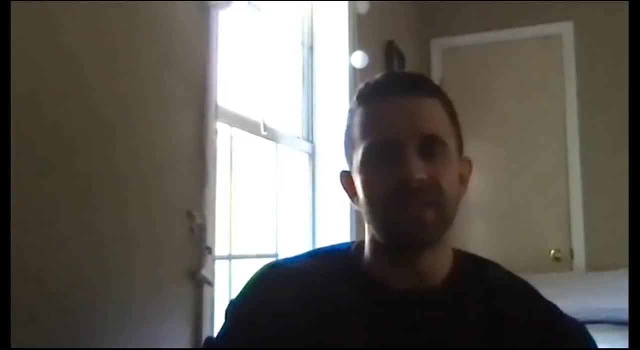 Or there's probably native seed. you know native mail or seed sources that would sell you seeds. So that's really the best way: Getting out in the field, checking it out, making a list. My list is on iNaturalist. 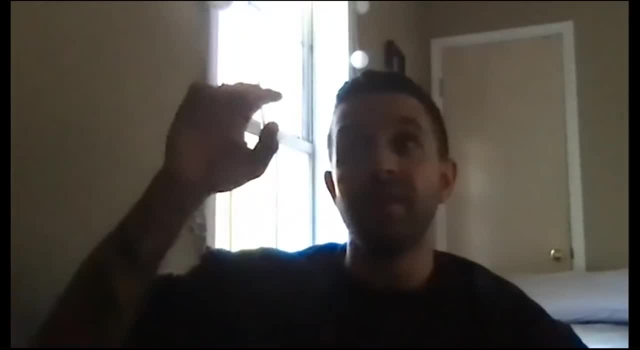 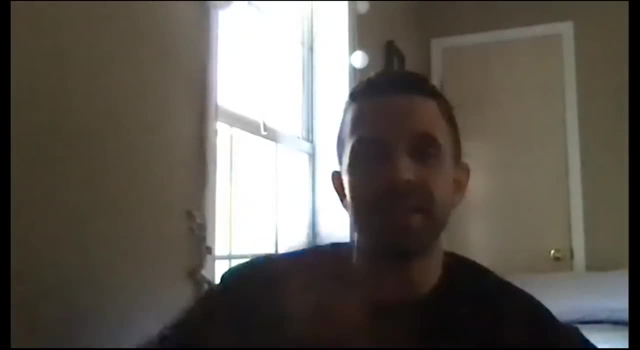 I don't feel like I'm out there with a notebook. I just have a list. I can type in family, location, and then there's a list- The location- and then there's another field where you can click: observer me? Only my observations. I can see everything that I've observed there. 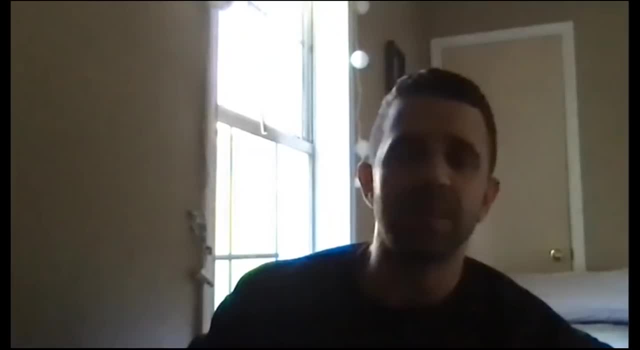 And you know that's helpful if I forget, like a genus name or species name. So yeah, but I would do that. I mean you learn your native flora and then you can grow all that shit, And that's the best way to get to know a plant is to grow it, you know. 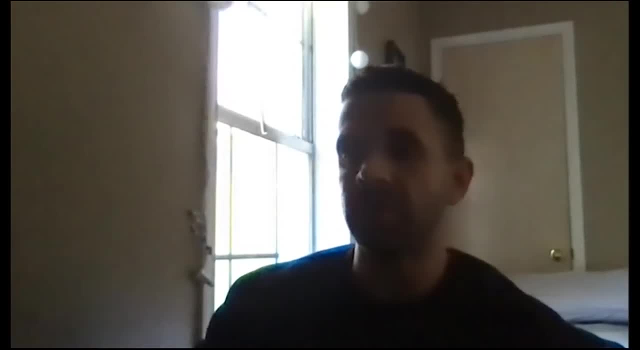 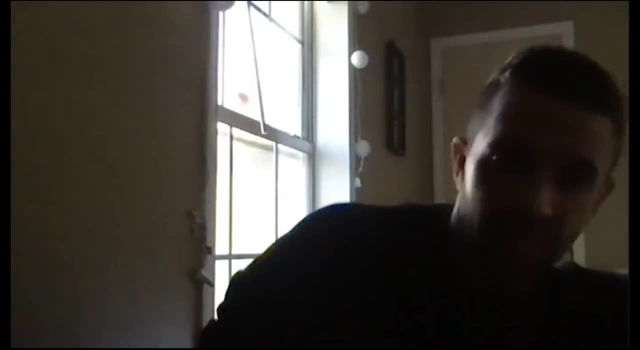 and you're like you see how it behaves and what it responds to And you know if it likes shade or sun, when it's young or when you know it's fucking cool. it's really rewarding Thing to do. 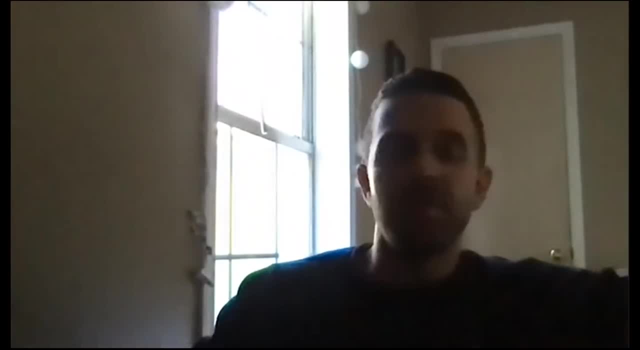 And then you go, when you grow a shit ton, you have too many- And then you go give them to people, or yeah, sneak them into a little landscape plant things or wherever you know. I would just give them to people. 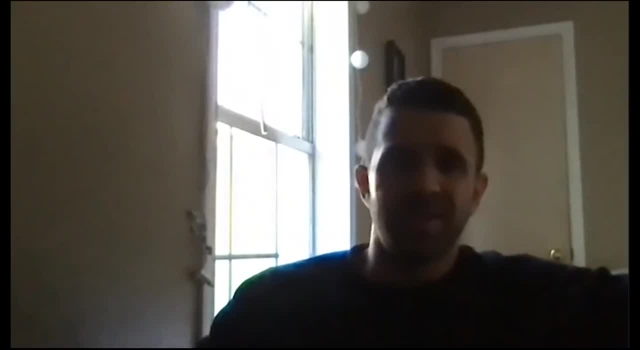 give them to other people that are in the native gardening in Texas. You know there's a shit ton of cool plants here, Yeah, right on, And there's way too many invasive ornamentals everywhere, And I'm just anything you do right. 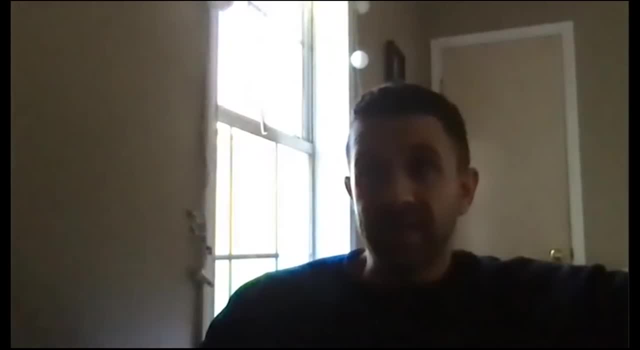 Yeah, Yeah, There's a yeah, So just you know. I think that's one of the things about Texas that kind of blows my mind is: like that They got such a cool flora here, But these people plant fucking crepe mortals and like, oh, like I. 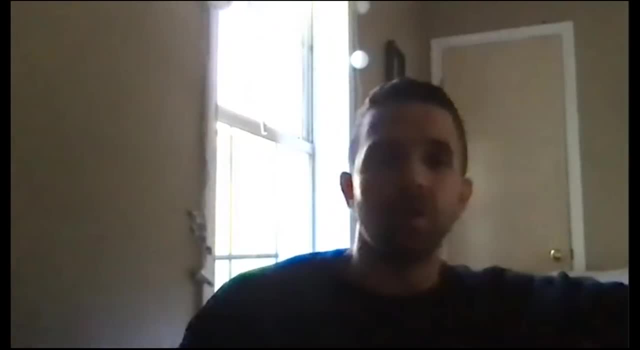 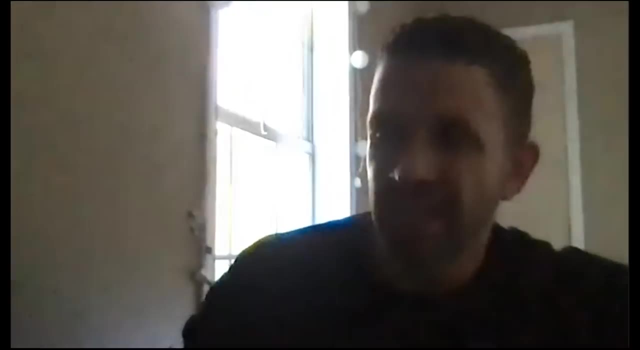 I see another crepe, mortal, I'm going to vomit, you know, just like goose drum which plant which is like terribly invasive and still being sold, like the Home Depot Garden Center, you know, and that kind of keeps in line. 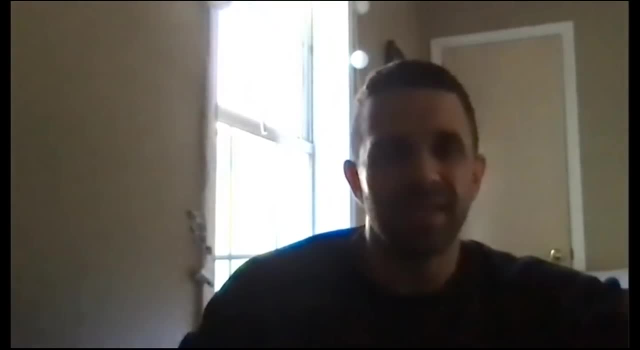 with, like, all the unimaginative fucking dead on the inside culture, the culture of the lawn, the culture of like: oh, it's hard work. It's hard work Like I'm going to be. I'm going to be a good boy and work 30 years. 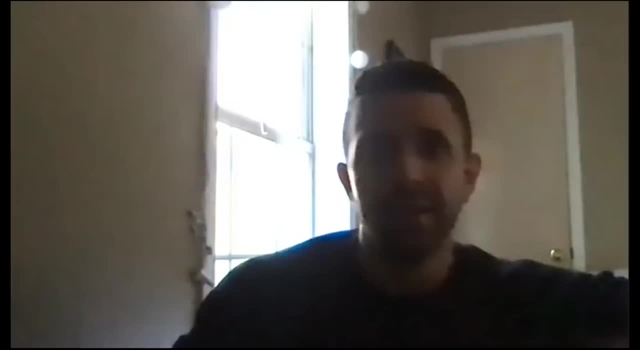 at a job I hate that doesn't pay me enough And get a little pat on the head. You know these people get older and turn 60 and realize the fucking system threw them overboard and they're fucked now. And now they're really pissed about it. 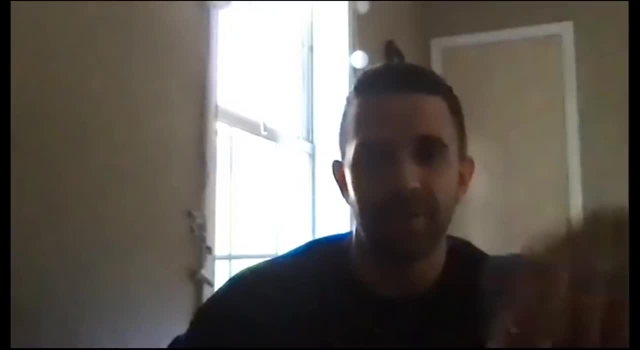 But you know, unfortunately the Facebook mega crowd got them first, before anyone that could, you know, tell them the real sense of what happened. So there's this whole, I mean there's this whole darkness that I synonymize with these fucking plant species. 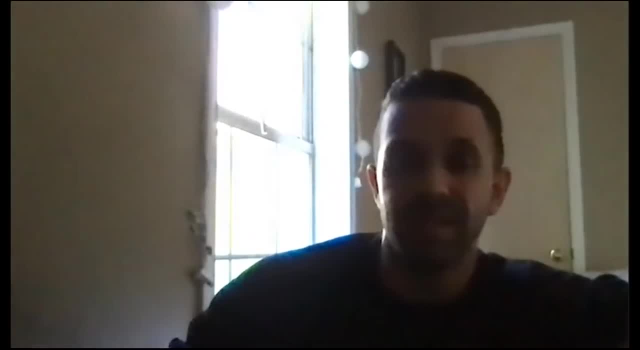 And that's not the fault of the plant species. Like goose, drum is probably cool, where it's made a really cool member of the olive family. only ACA, You know. Oleander is cool. It's a cool member of the milkweed family, apostasy, where it's native. 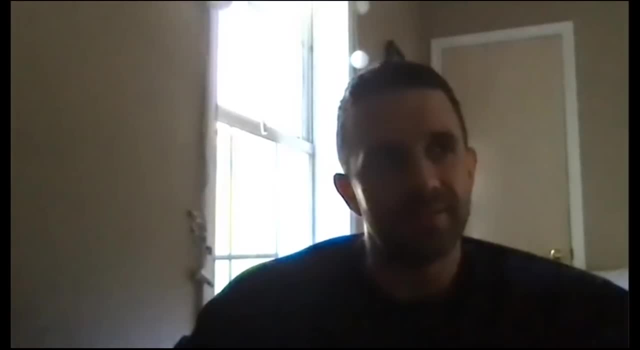 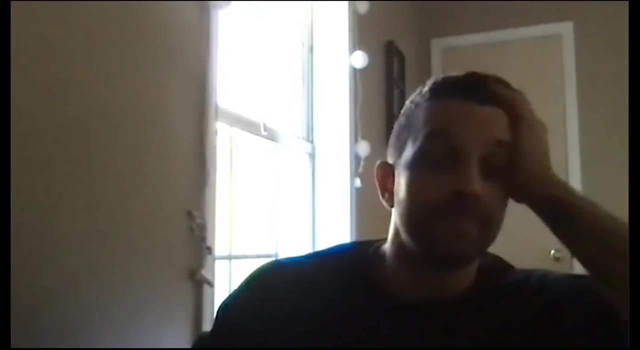 But I've just been beaten over the head with them by these bland, you know spiritually dead- human landscapes And I'm just like, oh God, I can't fucking do it now. So anyway, unsolicited rant. One more question. 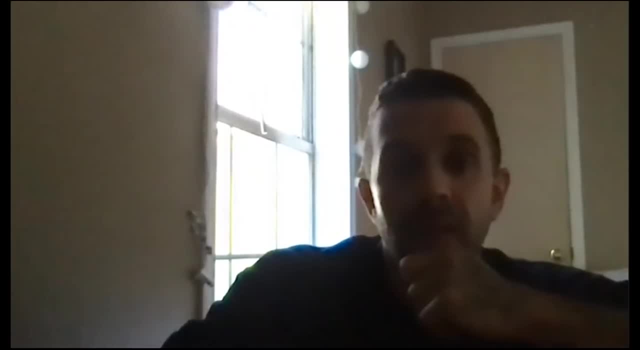 Anybody? Are you a? I got in here late. Was there a PDF Or anything? Are you just going to post this to Patreon later? Oh yeah, Well, it was like a Google Slides presentation And it will be written out- all the keywords and shit. 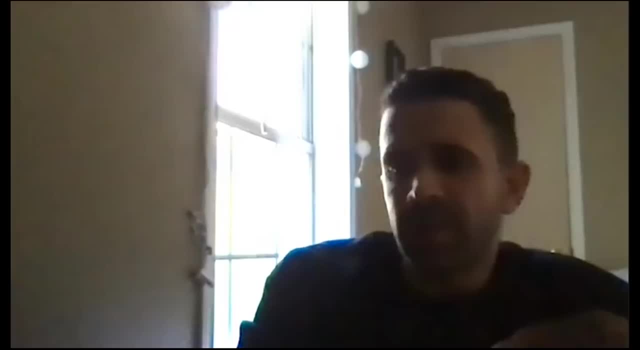 And yeah, you, could you get some out of that, I'll put it. I got to wait for it to finish on on a on Zoom, and then I'll put it up on unlisted and on YouTube, because YouTube is too much of a fucking toilet. 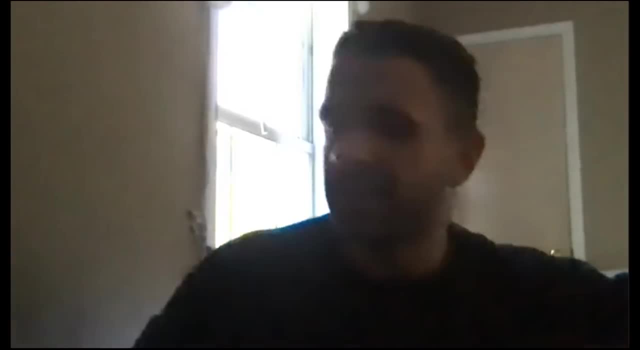 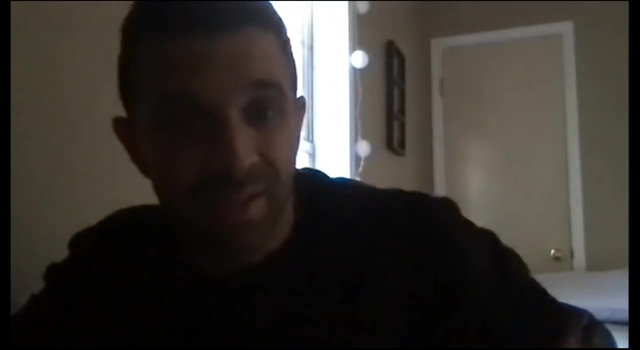 to put something like that. You know what I mean. You just get a bunch of bored fucking nerds, just you know trolls and whatever. So- and this is this will probably put a lot of people to sleep to the general audience So, but it'll be there unlisted on Patreon.